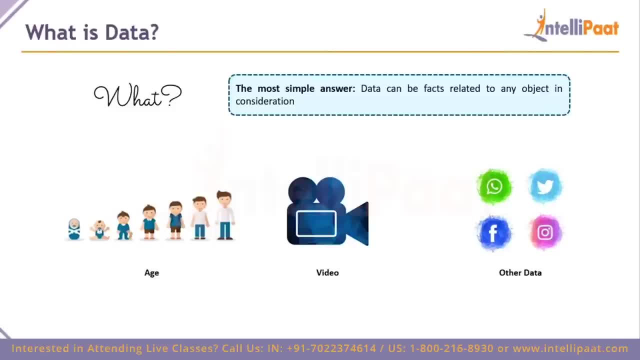 and then, if you're thinking about the other forms of data, again, we have video data as well. right, so video is what we call as unstructured data, but then if you do not know what unstructured mean, do not worry. uh, at this point you need to know that. at this point, you need to know that. pretty, 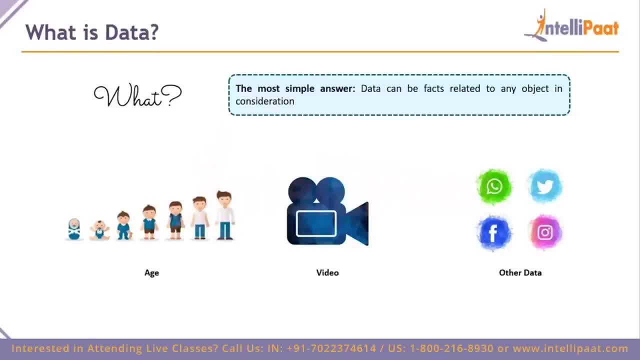 much. you know, video is a form of data as well, and then there are other datas as well. when you think about all the data we generate by, you know, leaving messages to each other on whatsapp or leaving tweets on twitter, uh, sharing photos on instagram or putting some updates on our timelines on. 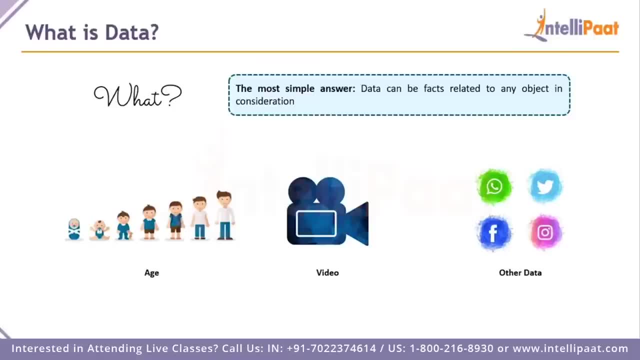 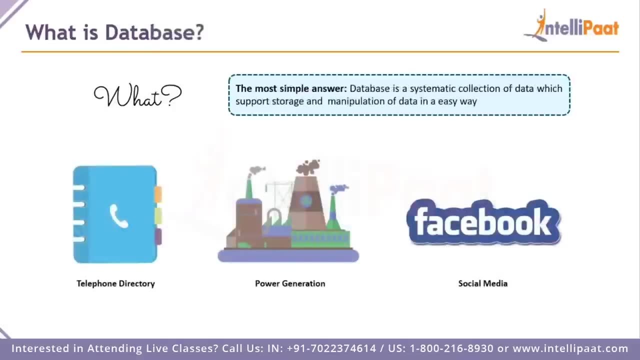 facebook, so all these stuff and lots and lots more is what we call as data guys. so this brings us to the question: what is a database? you might have heard of data, so if you've heard of database guys, head to the comment section and put down the comments as usual. i we all love an interactive uh session, so, and you guys are very 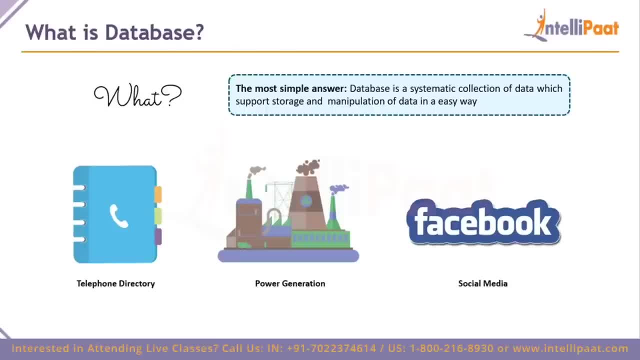 good at it as well, guys. so head to the comment section and put your opinions down. so what is a database? well, a database is basically nothing but a very systematic collection of data, in the most simplest terms. so why would we go about needing, uh, the systematic, uh, you know- collection of data? 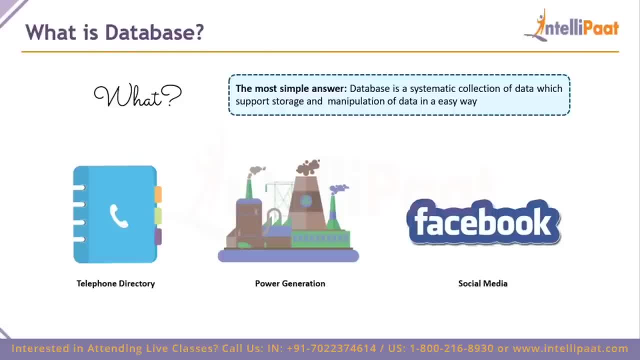 well, it's pretty much to you know- support some sort of storage where we can, uh, hold the data, maintain the data and eventually we can- you know, you know, we can, you know, we can, you know we can. we have to have the ability to manipulate the data in in a very easy way, to be honest. 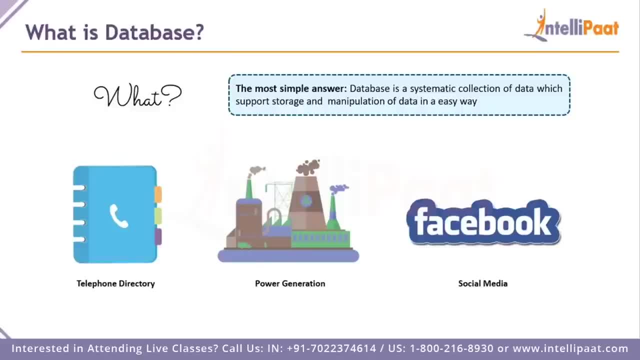 so to give you examples of what databases actually are, uh, if you guys remember, when we were, uh, you know, a couple of years ago, we used to get these telephone directories where they used to be all the numbers. it's called ello pages in a couple of countries as well. so 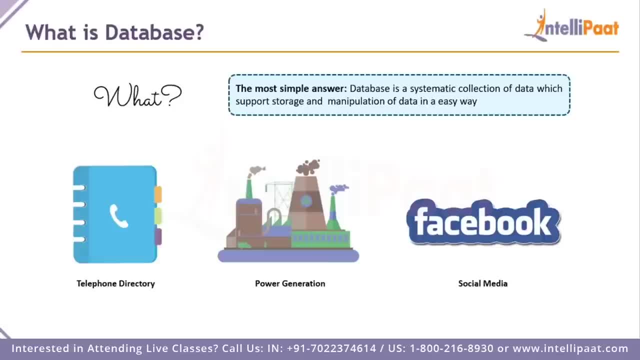 that is a very good example of a hard copy of a database, and the contacts option on your mobile phone right now is also a database. well then, coming to power generation, power generation you not know has a huge database of you know what power is being consumed by what house and what. 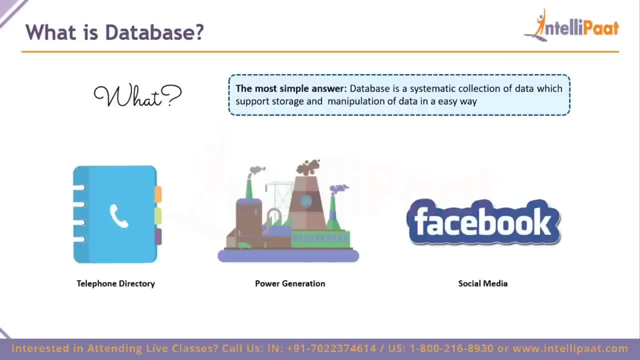 not, because again, at the end of the day, you get billed for the power you use and this data goes to your local electricity power supply board and again this forms a very big database as well, because pretty much they need to know what the power they're generating versus what's being used. 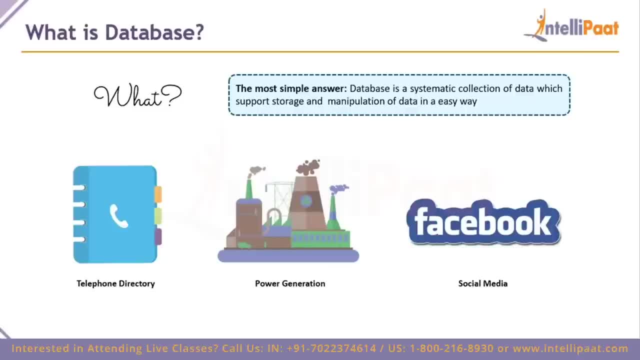 and many, many other details as well, guys. and then coming to social media, as i just told you, uploading images, uploading statuses, you know, uploading stories, what not? so all of these are stored in a database, in secure data centers, what we call, especially when it comes to social media. 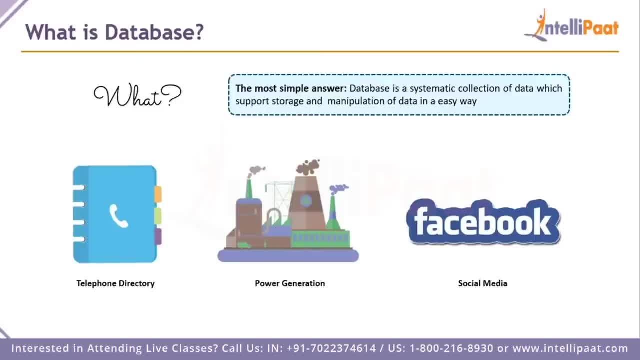 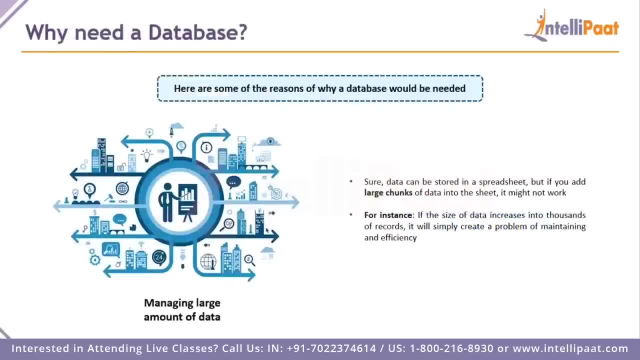 and the privacy things. so pretty much you know all of these are stored in in the database and it is stored securely, guys. so basically, this brings us to the question: why would we ever go about needing a database? well, i've pretty much tried to keep this session very simple, uh, and 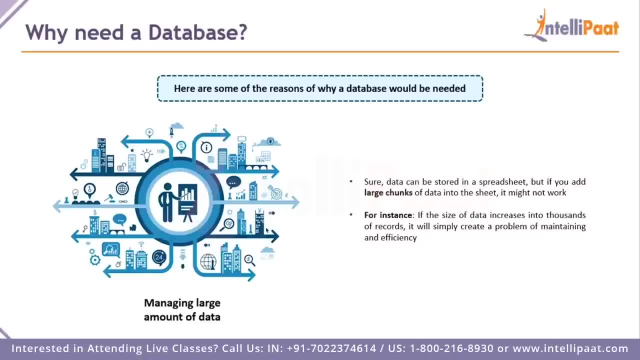 this is these. these are the reasons that i could you know, i've pretty much tried to keep this session very simple, uh, and this is these. these are the reasons that i could you know, i've pretty much tried to keep this session very simple, uh, and much think of of you know why, pretty much, we would need a database. the first thing in my 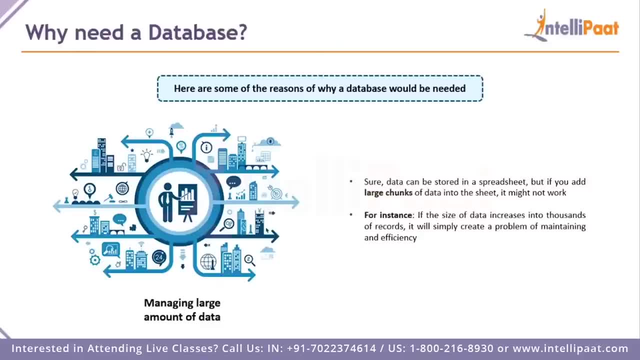 opinion is that we need a database because managing large amounts of data is a hassle, because you might say: you know what, i can store data in a, in a spreadsheet, and it's going to be fine. but then, when you think about very, very large amounts of data, large chunks of data, 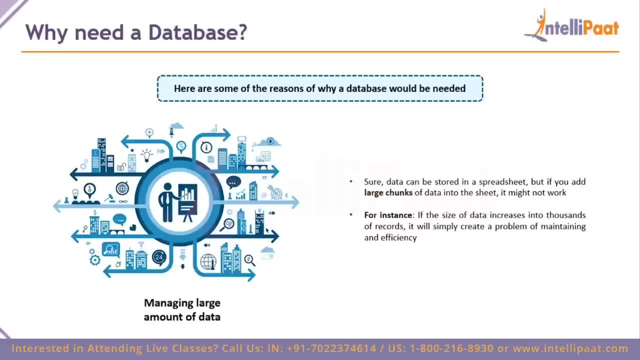 and throw it all into one sheet and make it work. it might not work or it might be extremely difficult, even if it works right. so, uh, you know, let's say, the size of the data increases. uh, from a couple of, you know, tens of hundreds of records to thousands. 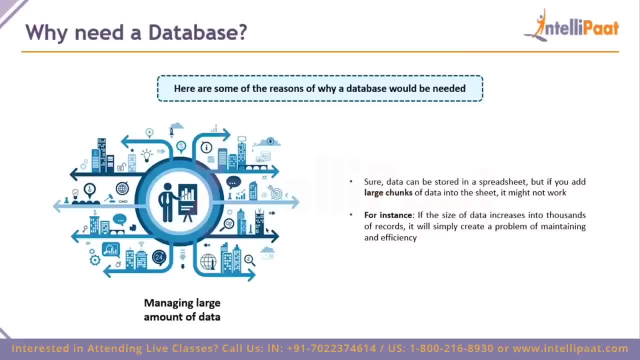 and millions of records. so when this happens, you know it will create a huge problem if you're using spreadsheets to maintain this data and, at the end of the day, it is going to hurt with respect to efficiency, time and whatnot as well. right? so this is the first point of why you initiate, why you 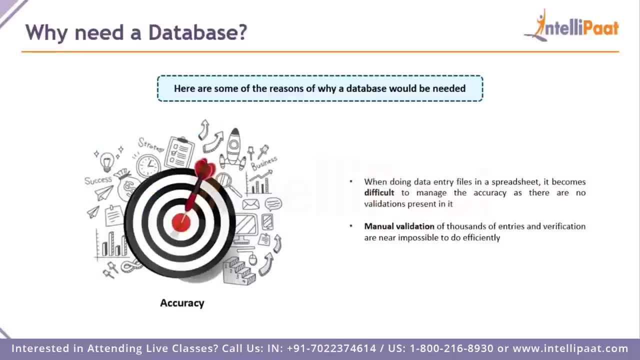 should need a database. and the second thing is the accuracy of the data, because when you think about it, doing data entry pretty much into a spreadsheet sounds very easy, but then it becomes extremely difficult to pretty much track how accurate the data is. uh, you know, on the spreadsheet, because at 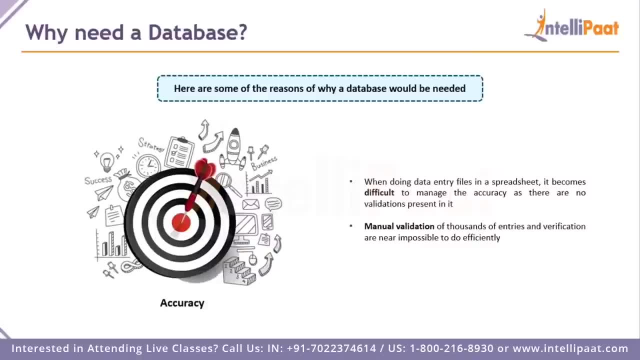 the end of the day, if you cannot have a method where you can validate the spreadsheet to find out if your data is accurate or not, it doesn't make sense. and again, think about this manual validation of thousands and millions of entries and verification of the same. it are pretty much. 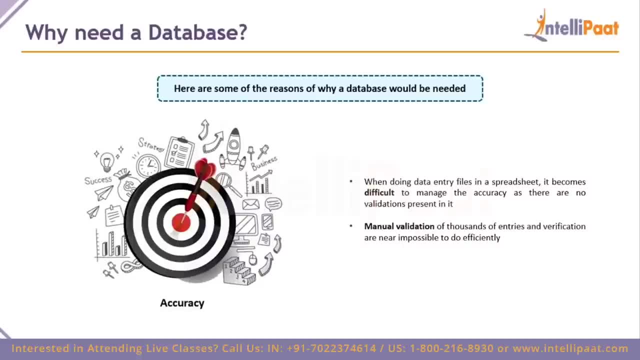 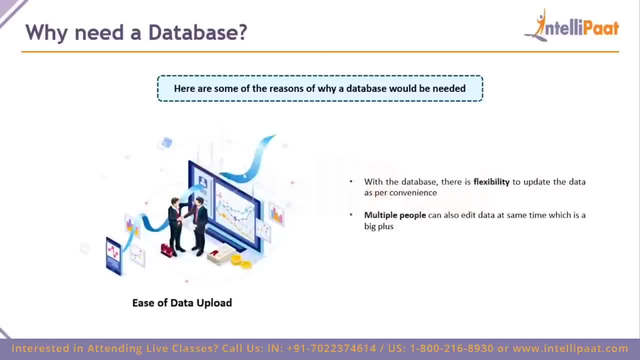 near impossible, and even if they were possible, pretty much it brings the efficiency right down to zero, right in my opinion. so this brings us to the third reason of why you need a database, guys. so, uh, in my opinion, again, it's the ease of data uploading, because with the database you have, 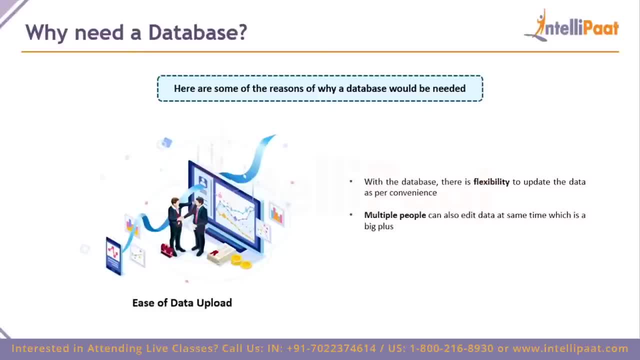 very good amount of flexibility to pretty much you know: update the, update the data present, manipulate it, play around with it, create and delete it whatever you want, at your convenience, so you do not have to wait for a the person who created the spreadsheet, go through millions of entries and do 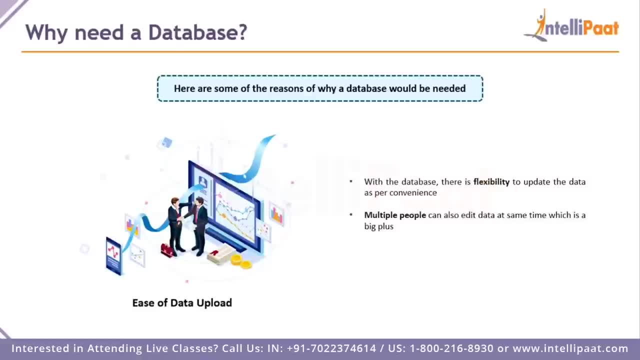 all of that. so again, you know, uh, the best advantage of a database is that multiple people can edit the data and you can use it for a lot of other things. so that's the third reason why we need a database. uh, at the same time, be, this brings up the efficiency and pulls it from zero to hundred. 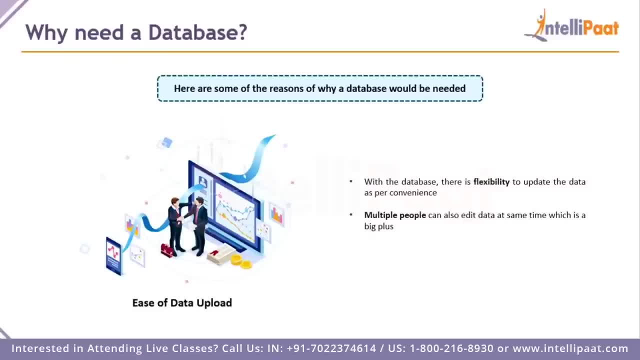 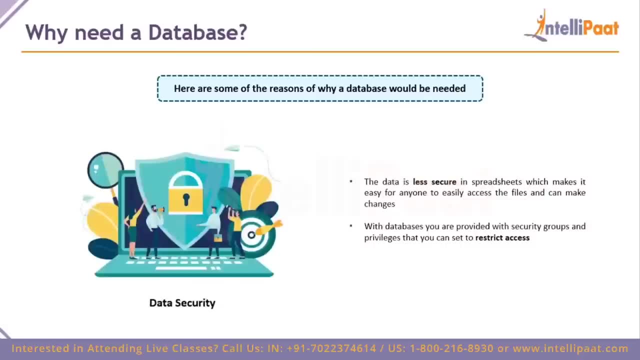 you know almost 100, in my opinion, guys. so what do you think about the efficiency when it comes to the database technologies of today? head to the comment section and do let me know. so on that note, this brings us to the next, uh reason why you should consider a database. that is pretty much because of: 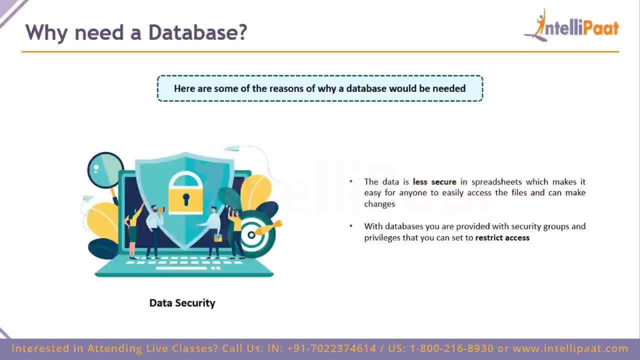 data security because, uh, you know, we do have passwords for spreadsheets and whatnot, but then the data is considered to be less, uh, secure and it makes it gullible because, you know, every gun can pretty much get access to all of these files. they can do some changes, remove whatever they want, or 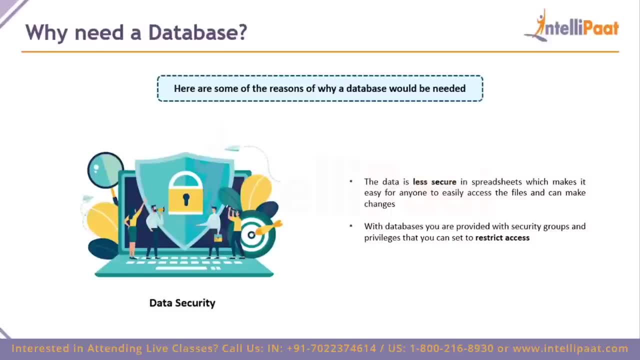 you know, add whatever unnecessary stuff and it hurts uh the data at the end of the day. but then with databases, pretty much, you can have something called as uh security groups, privilege accesses and so much more. so at the end of the day, here you can pretty much, you know, restrict access uh to a 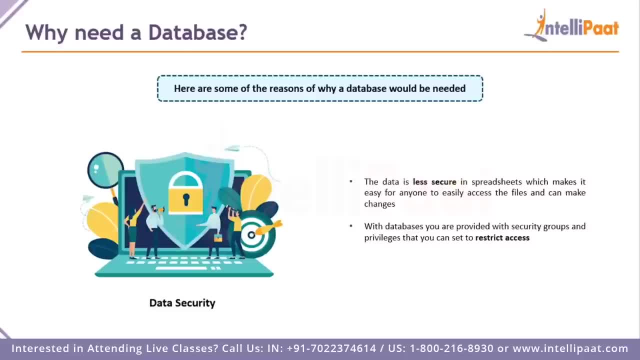 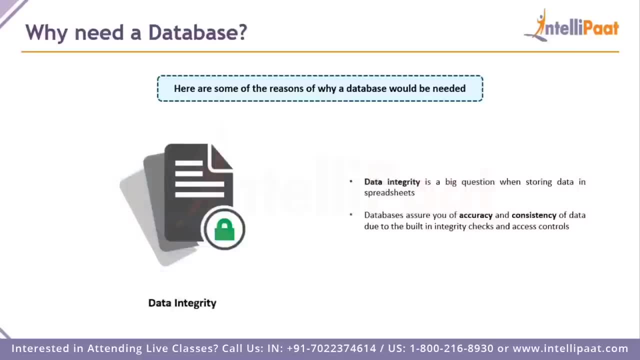 certain number of people, certain, you know people with the privilege to access the data, manipulate the data and whatnot. so your data will be in good hands at the end of the day. so what does that mean? well, adding on to that, this brings us to the next point, which is data integrity. data integrity is 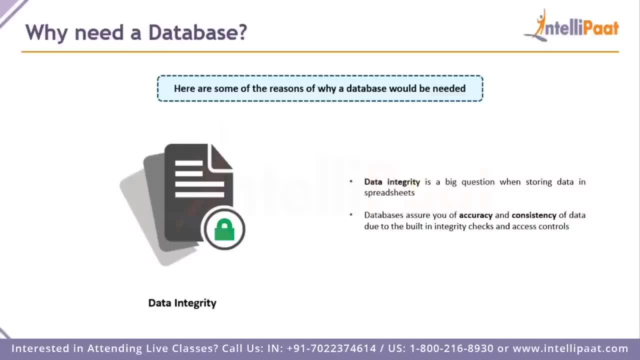 one of the big questions today. when we're storing uh, you know uh- data in in spreadsheets as well as databases- because, again, we've already spoken about how data can be gullible when we've put it in spreadsheets, but then when you put it in a database, you know, you're assured of accuracy. number one. 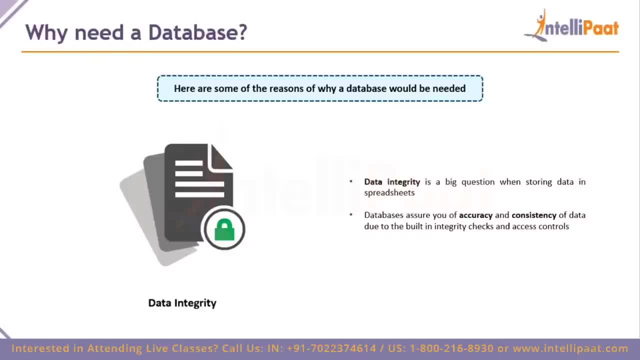 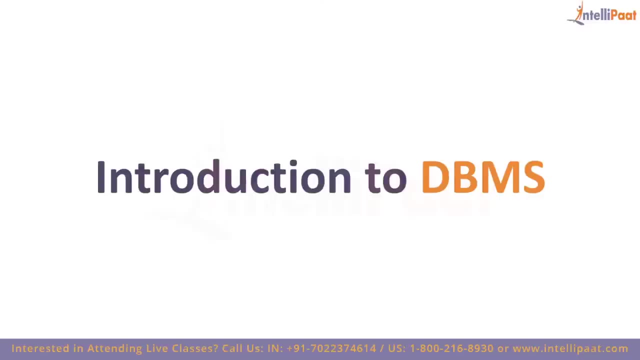 thing, it is extremely efficient. number two and number three: your data is consistent because databases- many multiple database service providers today pretty much you know- go about their work and they're going to give you very good integrity checks, very good access controls, privilege accesses, member accesses and so much more. 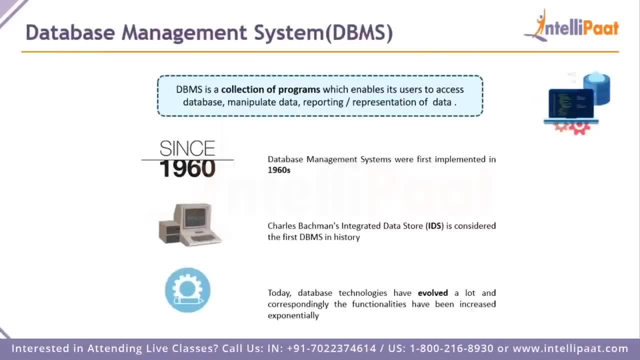 so this brings us to something uh, you know, you might have heard of, or you might have used in college, or you might not know as well: it's called as dbms. well, dbms pretty much means database management system, guys. so what is dbms? well, dbms, in the most simplest terms, is basically a database. 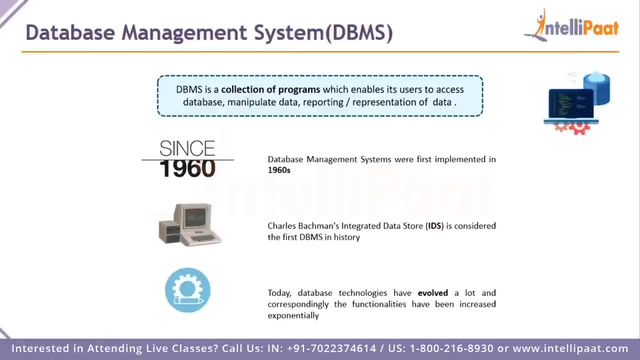 basically just a collection of programs which enables the user, whoever is using this particular dbms softwares, to go about accessing a database, creating a database, manipulating the data, you know, deleting the data. so basically, this gives the user an interface where he can, where he or she. 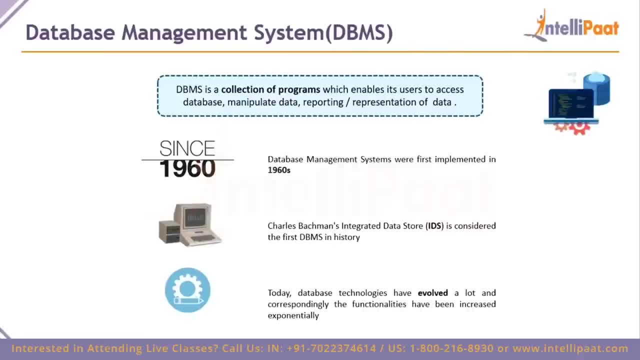 can, you know, talk to the database and pretty much work with the database, edit the database, delete the database and do whatever the person wishes to if he has the right access, and this basically gives the person you know a very good interface. guys, i have three facts for you, uh, with respect to the database management systems, and the first thing is: 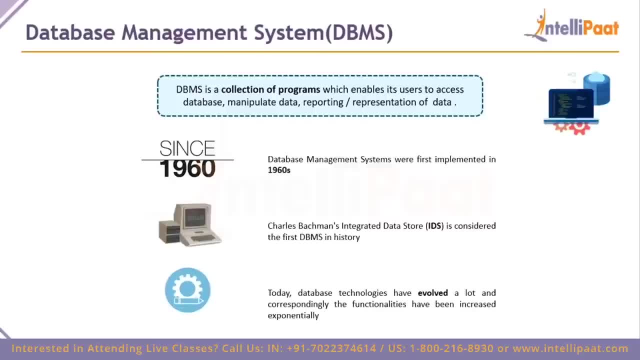 that dbms is not a new concept. it was first implemented pretty much in 1960, so that is how old a database uh management system uh is. and then, when you can think about it, uh, the person who pretty much uh gave us the first dbms system pretty much is called a charles bachmann and uh. 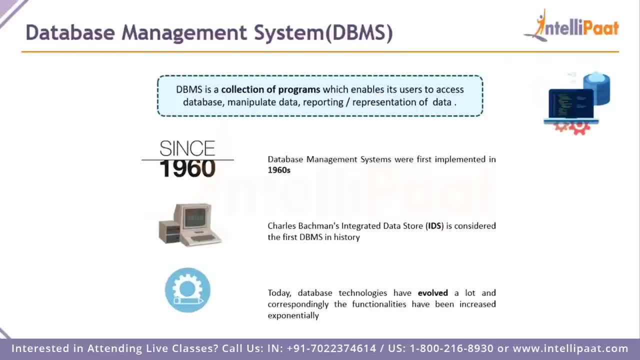 his ids is considered to be the first dbms. ids is basically integrated data store, is what mr charles call, uh, his first dbms machine, guys. and then, third important fact is that today, uh, we know that the database technologies have evolved so much and all of the functionalities have been given, and these: 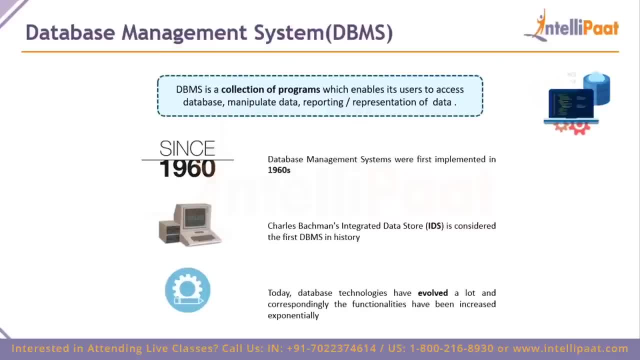 functionalities increase every quarter, every year, every month. and then the database systems today are so powerful, it drives, you know, millions and millions of gigabytes of data every single day. yes, millions and millions every single day. guys, i can say millions of millions as well, because the world 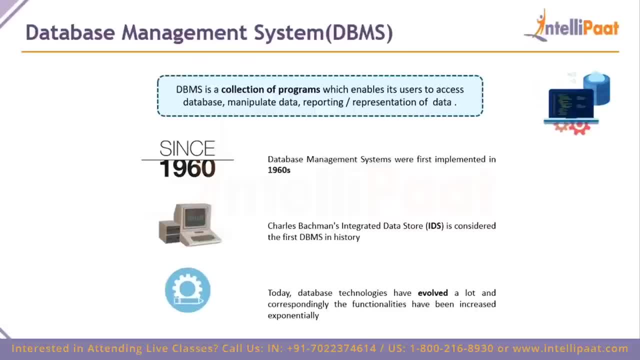 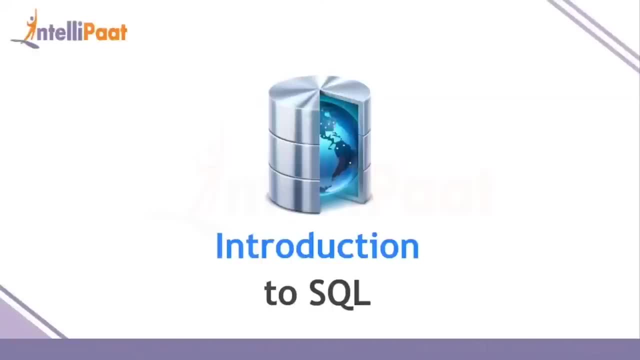 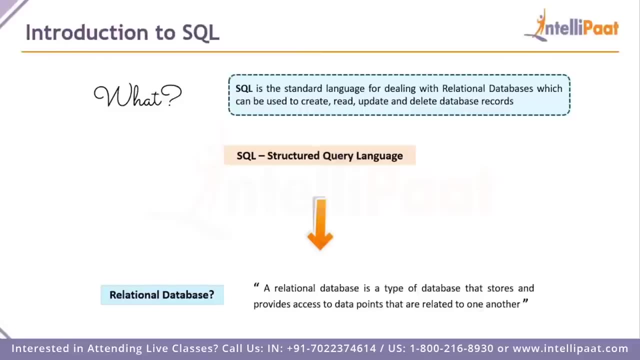 is basically a big data problem. so, uh, having a place where we can handle all of these, store all of these and manipulate all of these is always a blessing, guys. so this brings us quickly to, uh, the introduction to sql. well, so, what is sql? well, sql is one of the standard languages we use when we go. 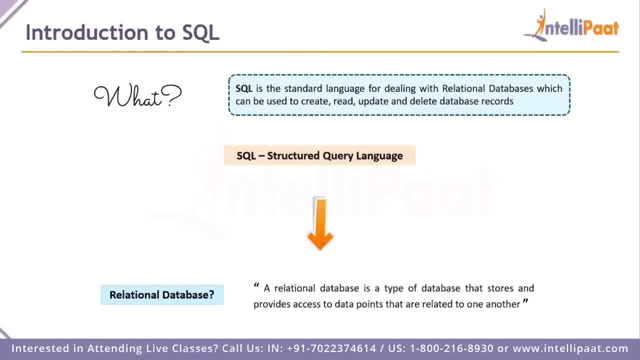 on about dealing with relational databases, which can be used to create, read, update and delete database records, guys. so these are some of the operations we can perform. so what does sql do? it's sql stands for- well, sql is simple, it stands for structured query language. guys, you're going to 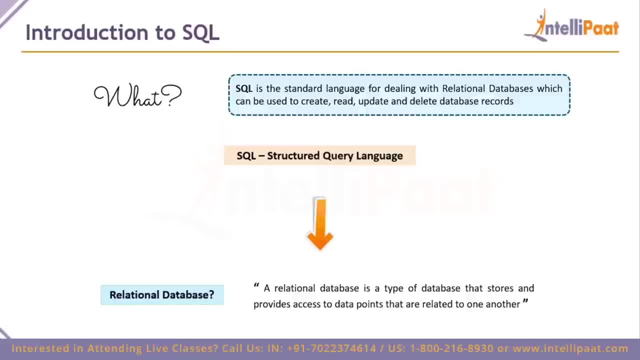 find out why we call it the query language in just a moment. but then you read the term relational databases. so what is a relational database? well, a relational database is basically just a type of database that stores and provides accesses to all the data points which are related to one another. 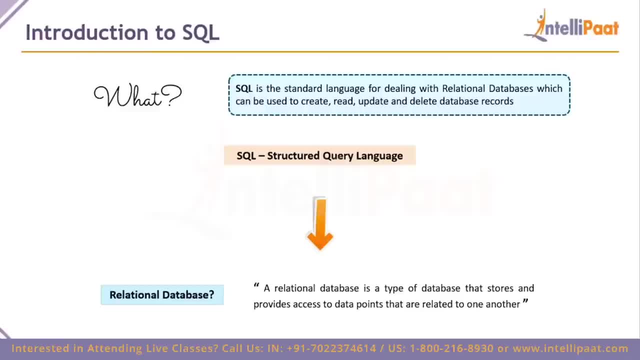 well, how are these data related to one another, guys? so, basically, when we call it a relational database, there has to be some relational database that actually votes to this data as well, as well relation with respect to the data using SQL and the. you know all the DBMS. we. 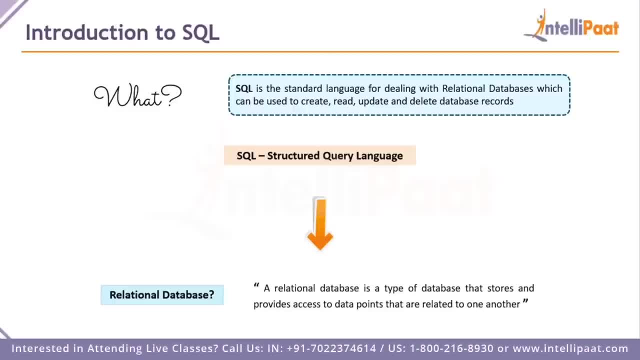 called the RDBMS because it's relational database management systems. here we have the data organized in tables, which you will see in just a second, and then we map the data so that the database knows what's important and what's not, and we do this using something called as keys. well, keys such as primary keys, candidate. 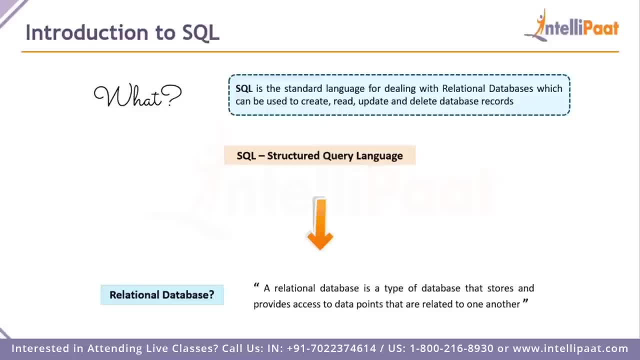 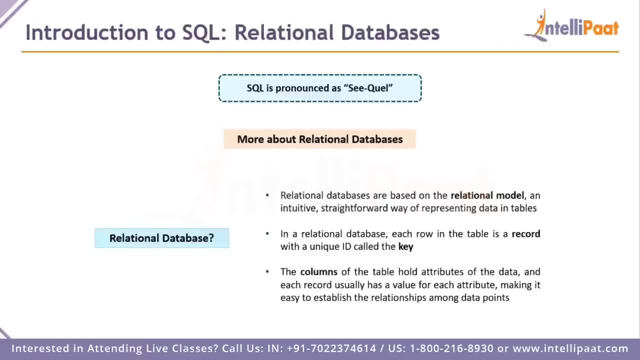 keys, secondary keys, all of these provide relation between one column of the data to the other column of the data. guys, you'll see all of this in a couple of moments. but then, coming to a little bit more about, you know, relational databases. well, relational databases are pretty much based on what we call as a 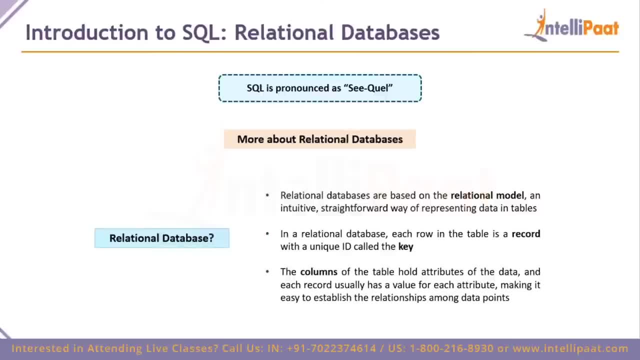 relational model where we pretty much map one concept to another, the other concept is mapped to another and we have this interdependency, interrelationships which are built throughout the data guys, and then this makes it very intuitive and extremely straightforward. you know pretty much, it gives us a very 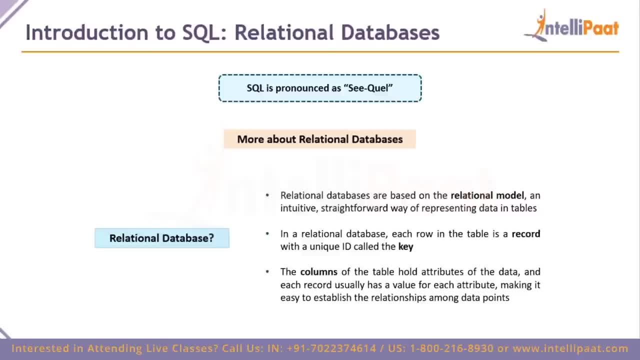 straightforward way of representing the data in the form of tables, as I just mentioned. and then the other good thing about the relational database as it, as I already told you, is that each row has something called as a record and there is some unique ID called a ski as well. again, 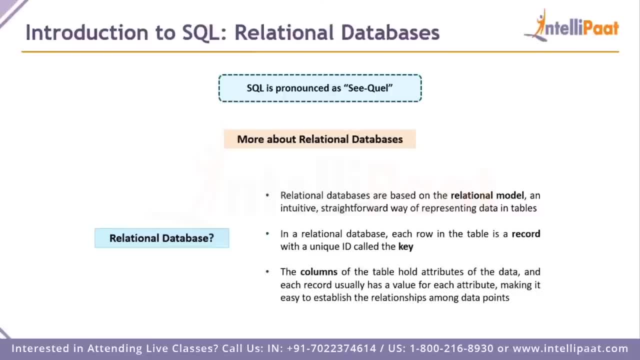 we're gonna check all of these in the upcoming slides, and then we have something called as columns, which any data table will have, and then these columns basically hold all of the data and each record in this column basically is mapped onto a unique thing, and then, you know, we go on about establishing. 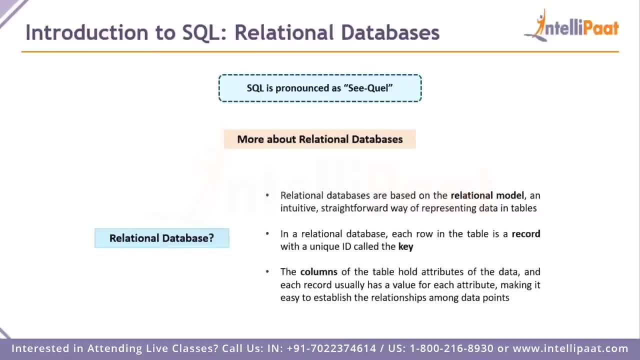 something called as interdependency relationships and much more among all of the data presently in the database. and if you're wondering how SQL is pronounced, it is pronounced as either SQL or it's called sequel. guys, pretty much you will find developers, enthusiasts and many others either calling it SQL or sequel. so whenever you heard of the term, 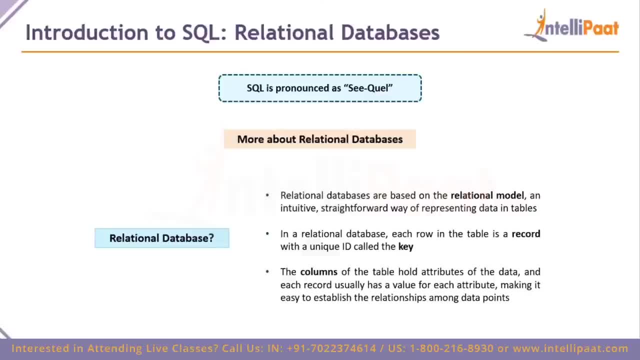 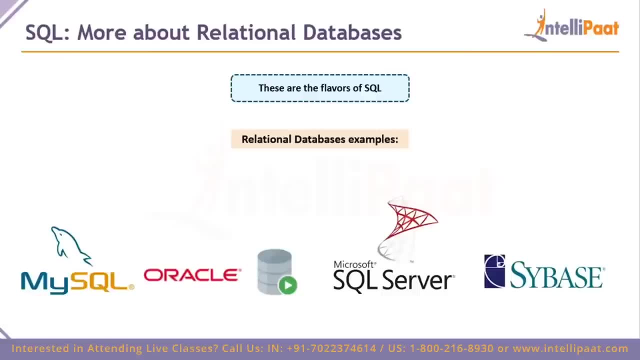 you know, whenever you hear the top sequel, make sure to map it into SQL, guys. it's. it's pretty much simple and straightforward. so, coming to know a little bit more about relational databases, there are some flavors of SQL that I thought I should tell you guys. well, here are some of the examples of 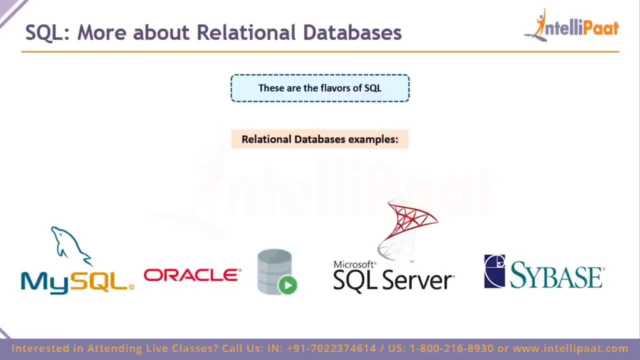 relational databases. we have mysql, we have oracle SQL, we have Microsoft SQL, we have Sybase and we have many more flavors of SQL as well. the subtle differences in between all of these providers are pretty much, you know, in in the form of syntaxes, of how we pretty much talk to the database, and there are 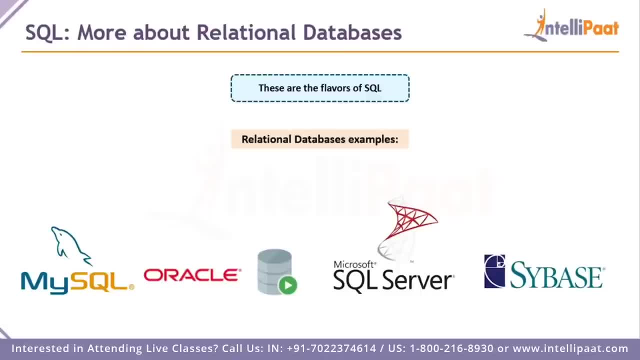 some proprietary syntaxes as well, where you know those syntax only works with, you know, Microsoft SQL server and it might not work with MySQL and so on. but then it is recommended for all the beginners to much go on to start with mysql and then pretty much you know, jumping to any of these other. 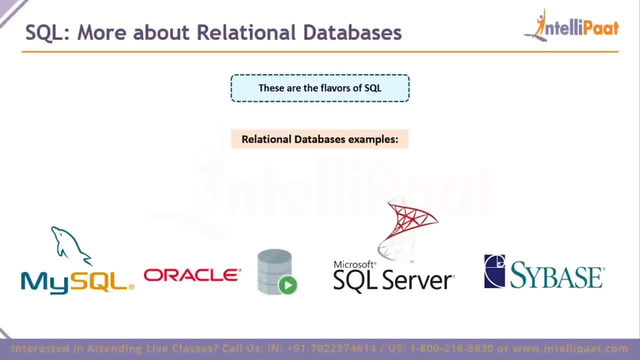 providers other flavors of sql. it becomes very easy if you're a master of mysql, guys, and on that note, make sure you stick till the end of the video, whereas, as usual, i'm going to give you a very attractive offer just for the viewers of this particular video, where you can fast track your way. 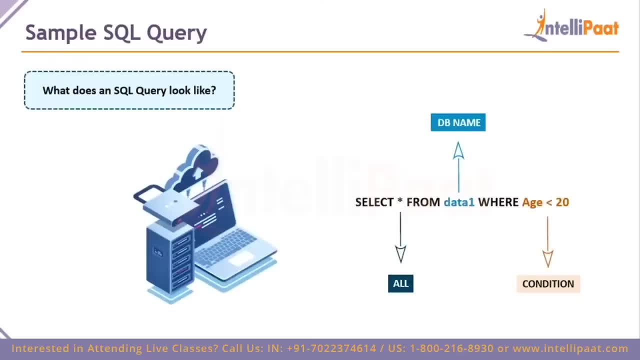 to becoming a mysql expert, guys. so, on that note, uh, we need to quickly check out, uh, what a query looks like. so a query is something very simple. it is the actual, let's say the code. we write, guys, in terms of, uh, sql. well, uh, a query will look something like this: think about you entering this in a shell. 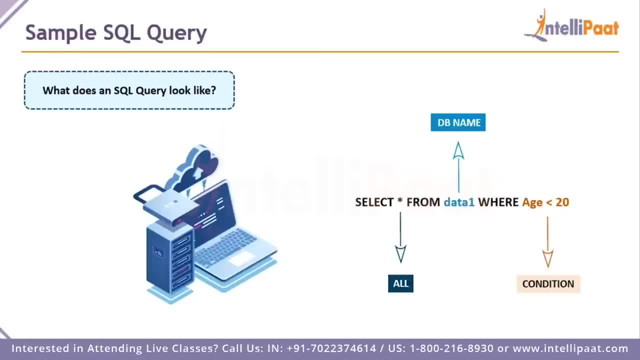 or in a particular workbench guys. so we have something called a select star from data, one where age is less than 20.. if you know a little bit of sql, i'm sorry. so if you know a little bit of sql then pretty much you can make sense out of this. but then if you do not, do not worry, because 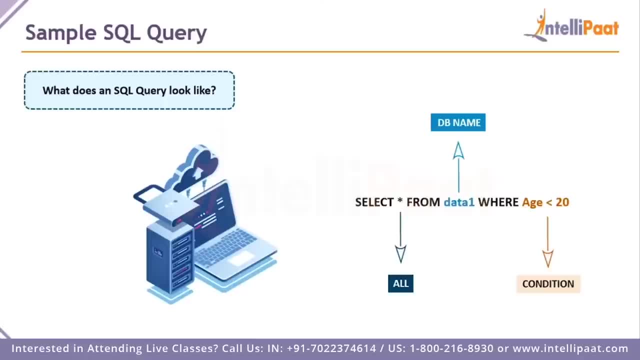 i'm going to walk you through what each of these means. well, so basically, we're going to be viewing a lot of data present in the database, right? so select statement is pretty much used to this: pick data from those actual servers and then show to us. star pretty much means that you know, show everything that is present, everything from where. 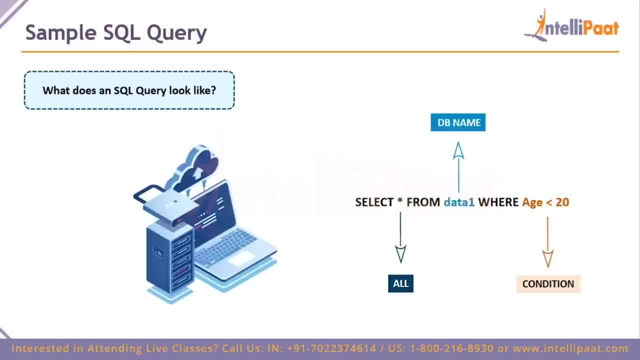 well, everything from a particular database that we have, and that database in this particular name is called as data one. and so do you want to see? just see everything from data one? well, no, i want to see some stuff from data one where the age of a person, let's say, we have talked, we're talking about a 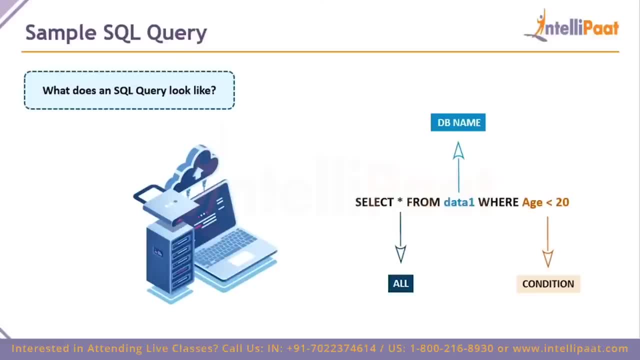 table which contains details about a lot of human beings or college you know, college people, uh, school people and whatnot. so we just want to find out who all are, uh, less than the age of 20.. so, when you think about it, uh, instead of just seeing millions or thousands of entries of 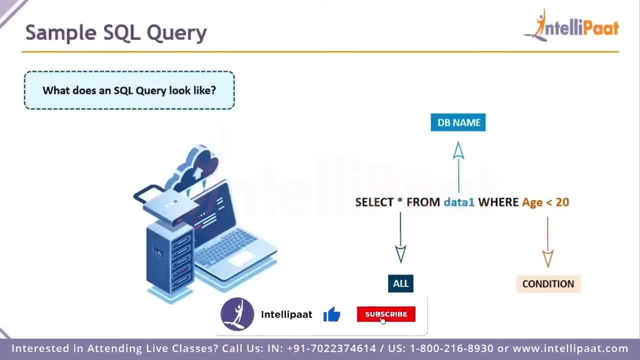 students who are, you know, aged various from, i don't know, 3 to 100 uh. but then when you're thinking about uh efficiency, uh, then you have to go to the data one which is uh, you know, like the data one where the age of a person. let's say, we've talking, we're talking about uh table, which contains a 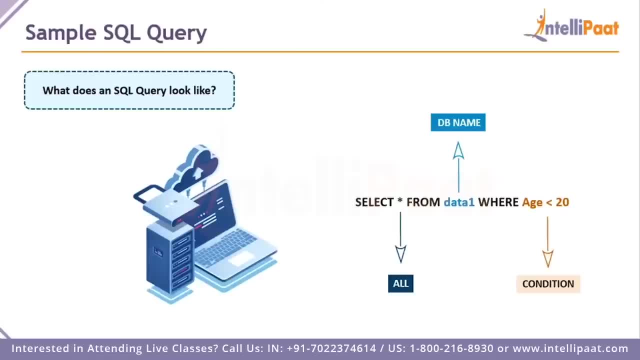 efficiency, then we need to bring it down to a certain condition where we go on checking it right. so instead of just seeing thousands of entries, let us say we only require 11, and we're going to see 11 entries when we put the condition saying age is less than 20, because there are only 11 people. 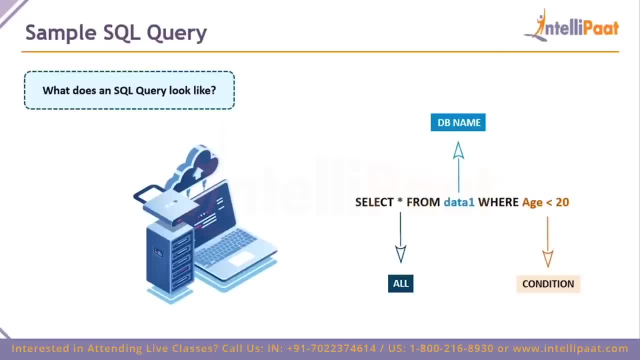 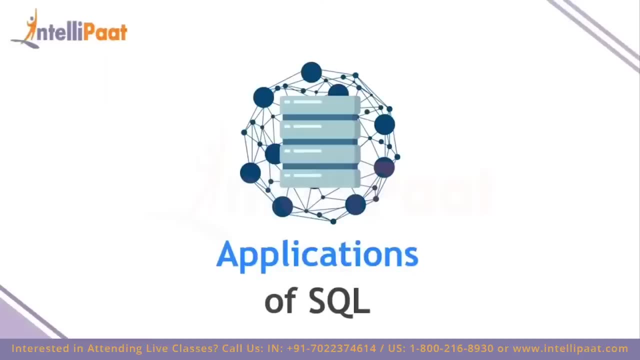 who are less than 20 years old guys. so pretty much this is what a sample sql query will look like, and we'll just be doing very simple operations at the end. you can follow along in. so, on that note, this brings us to. this brings us to the applications of sql. so sql has a couple of applications and 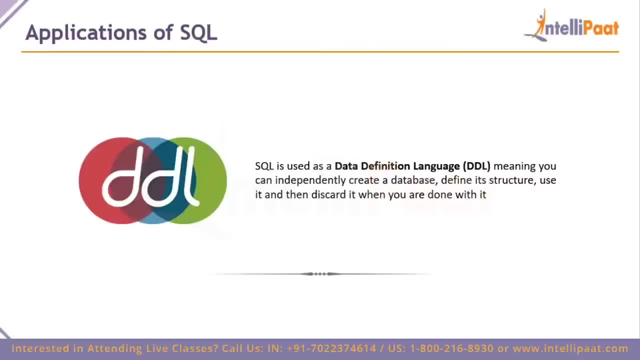 let me tell you one by one. sql can be used as a data definition language- ddl for short. uh, what this basically means is that you can- pretty much, you know- create a database on your own, define its structure on your own, use it on your own and, just you know, discard it when you're done. 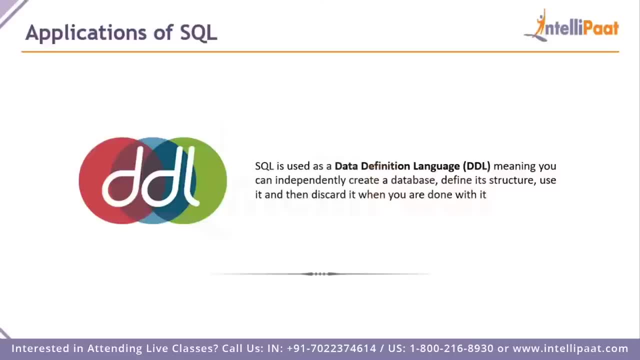 with it. so this, this doesn't have to be just you. this can be among hundreds and thousands of people. you can scale it obviously, but then know that you can scale it obviously, but then know that you can scale it obviously, but then know that, respect to data definition language, you have all the right where you can individually create a. 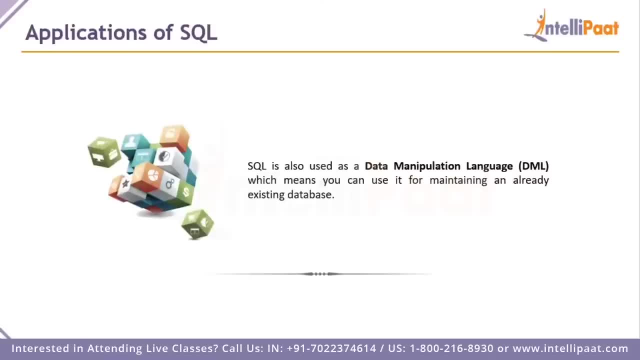 database, define the structure and delete it when you're done with it as well, guys. and this brings us to the next application, which is data manipulation language, because sql can be used as dml as well. so what it basically means is that that you know when we have something already in. 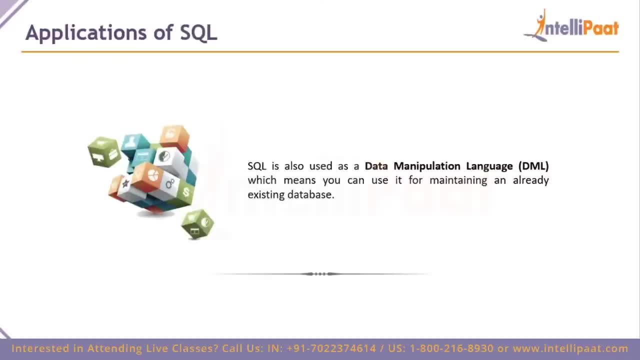 establishment, like uh data, which is already present in our database. we need to go on changing something in that database. we need to update a database, we need to delete a row, we need to update a column and so much more. so in that particular case, we can use sql as a data manipulation language where you can pretty much 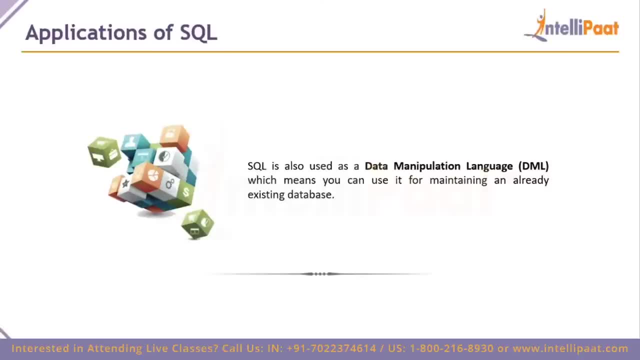 alter stuff in the table. you can go on adding, removing and whatnot. so this brings us to the next application, which is the dcl guys data control language. so data control language is mainly concerned with your data in terms of how you can avoid corruption and how you can avoid. 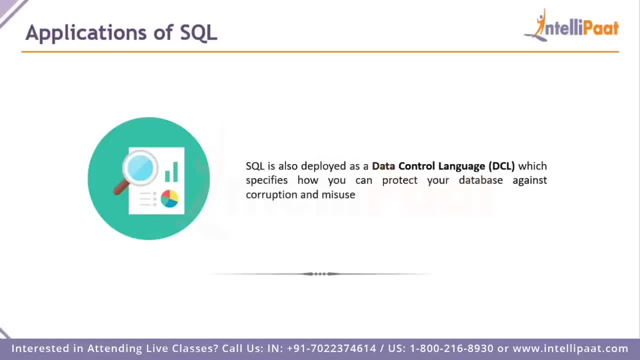 misuse as well. so, pretty much, as you know, data has to be protected and misusing data is extremely easy, uh, even though, with all the security measures, these tests. so, uh, you know, sql can pretty much be used in terms of dcl, where we can, you know, protect the databases against corruption and 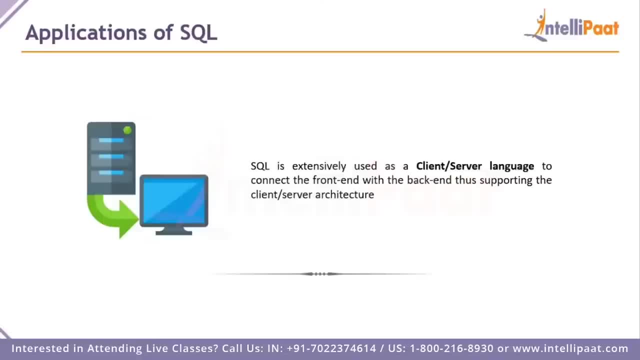 misuse in a very good way as well, guys, and the next application of sql is pretty much that it can go on to be used as a very good client server language. you can, uh, pretty much so, program on the client side and the server side, where you can, you know, connect front ends and back ends. 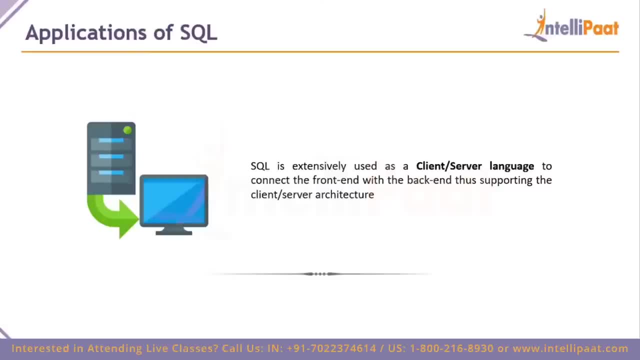 together, where we have an entire architecture which is set up, what we call as the client server architecture, where there is one server and then i know there are lots of clients, i'm sorry about that- there's lots of clients, you know, connected to that particular server and 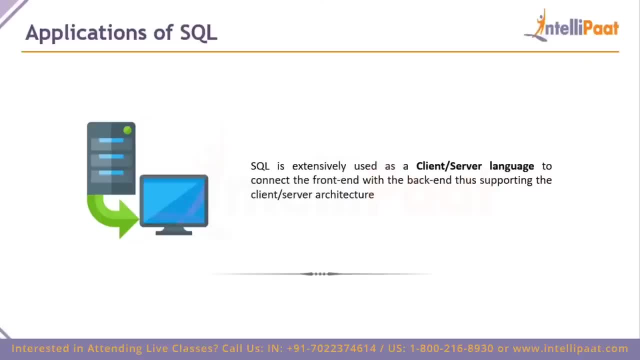 then we pretty much, you know, go on uh, querying and talking to the server, getting the details from the server for each individual client and more guys. so the next application pretty much is what we call as the three-tier architecture. the three-tier architecture is something very similar. 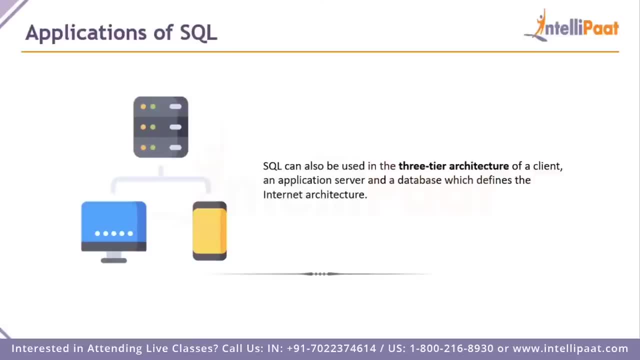 to the client, uh, server, client architecture where, you know pretty much, we have something called as an application server database and all of these together in terms of the server, the client and the database form, uh, the three basic, uh tier architectures, guys. so it's the client, it's the server and the database where? 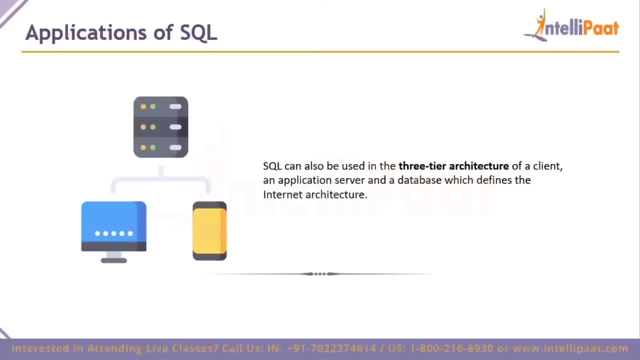 you know, the data is uh uh present and it can be. it can go through the server, where it can go to multiple machines or pretty much. you can have it come to the server and talk to the client directly as well, guys. so, on that note, what do you guys think about the applications of sql? 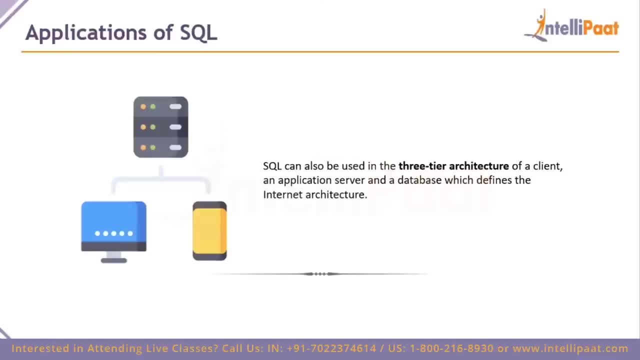 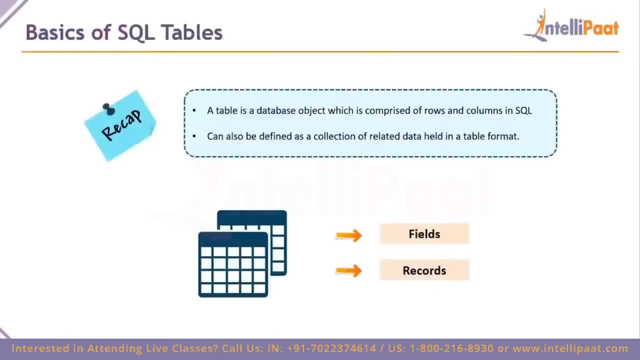 can you think about any direct uh applications of sql? if you can think of it, make sure to head to the comment section. right now. we can check out the basics of sql tables really quickly, guys. well, uh, as i've already told you, let's have a quick recap. a table is basically. 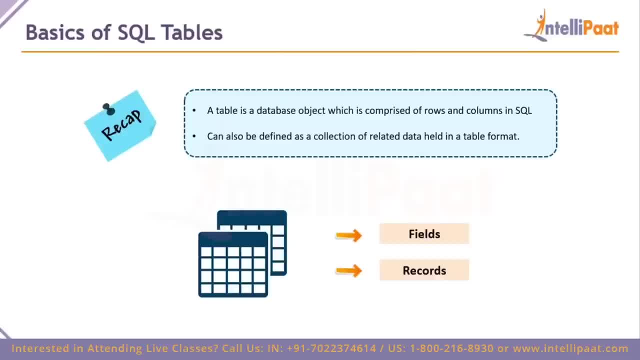 a database object which is comprised of rows and columns. in sql we already saw that it is the structured way of going about uh, using data or table, and then it can also be defined as the collection of, you know, related data held in a table. it is related by the forms of keys. 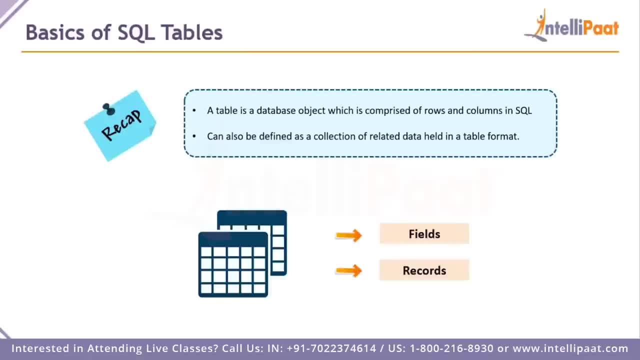 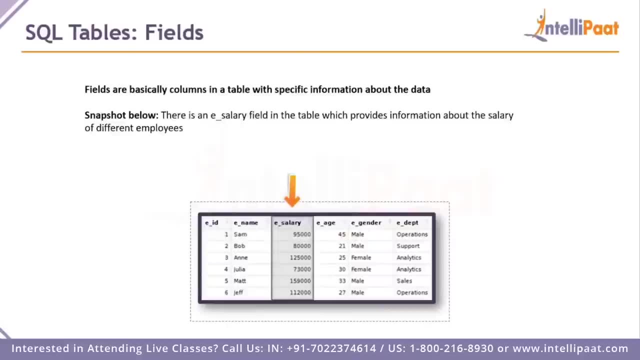 uh, which i told you, but then there are two things that i'd really want you guys to visualize, which are fields and records. well, fields are very simple, guys. fields are the column where you know we have specific data under that. well, consider the snapshot i have given in your screen. uh, we have some. we. 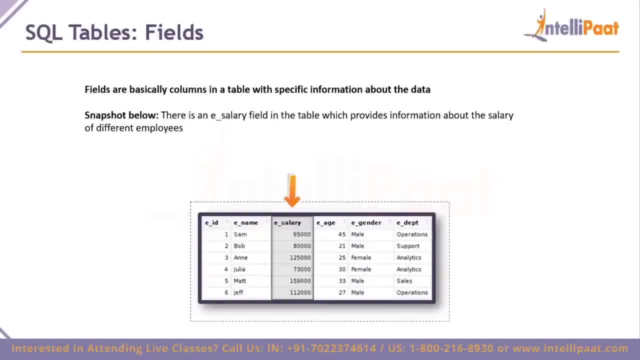 have a field called as e underscore salary, let's say it's employee salary, and this salary, pretty much, you know, uh, is- is the information which we provide. but then we have one header under which the salaries are all coded right. so this basically is: this is the salary field. this entire column is. 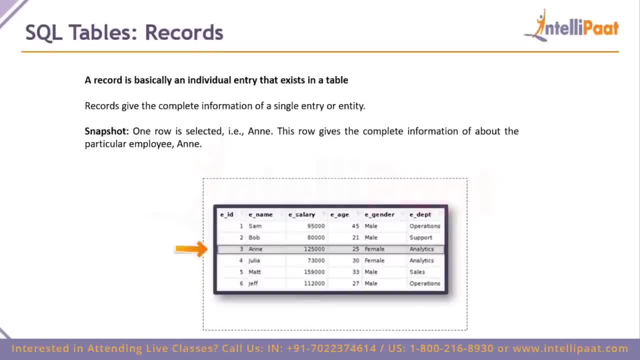 what we call as a field. and then, when we come to right now, let's say we have a table and we have a field called as e- underscore salary- and then when we come to records, records are something very simple, because what is the record corresponding to a particular field? uh well, let's say we want 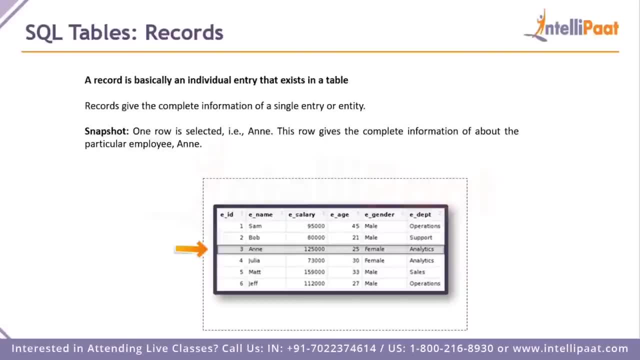 uh, the record of the employee name annie. here annie pretty much goes on to, uh, you know, be the employee id 3. uh, uh, it's under the employee name. we searched it through the employee name, right. so we said we want to find out annie. so annie is pretty much the employee's name and the employee's. 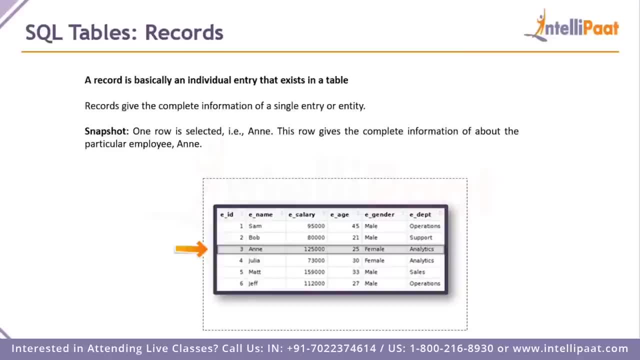 name was the field and the record was number three, right? so it's pretty simple. uh records are the field and the records are the employee's name and the employee's name and the employee's name is the entire description, a complete information of all the entities present in that particular uh data. 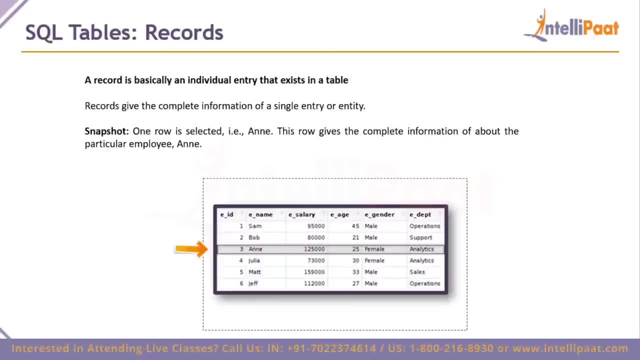 set, guys. so you know we already have a lot of data on the screen, but then when we highlight one row- uh, the annie's row- pretty much this row gives us the complete information about that particular employee, guys. so this is what we call as a record. let me quickly step back where you can see fields. 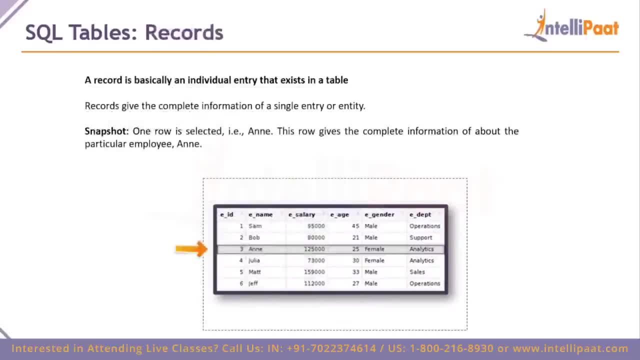 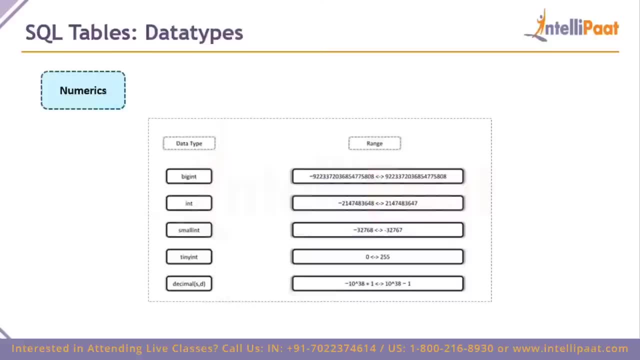 again. so this is the field, guys. the field is the column, the record is a single entity which gives us the complete information about the individual data types, and the data types are the data types which are present in sql, guys. so i will not go in depth, uh, because we need to keep this tutorial to. 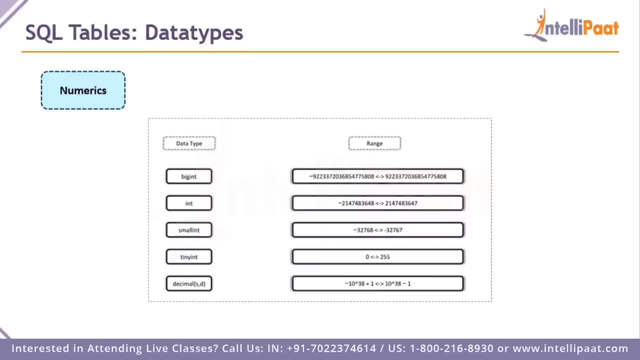 the scope of all the viewers uh or present uh tonight with our session. so, basically, uh know that you can have numerical data, character data, date and time data and much more. with respect to numeric data, we can have integer data, decimal data and all of these as well. so basically, what you have. 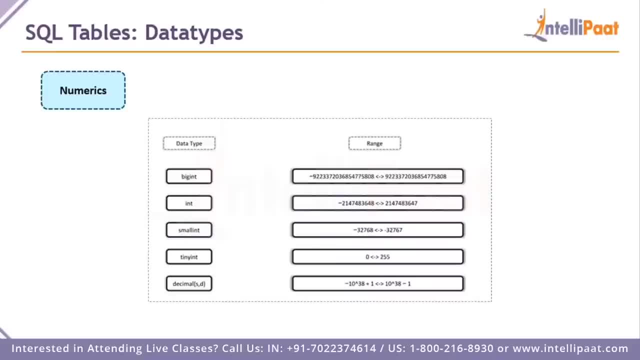 the corresponding range of the numbers that you can use. so you can see a big number there which is nine, two, two, three, three, seven, two, zero, three, six, five, four, double, seven, five, double, you know, five, eight, zero, eight, right. so this one particular number. if in case you want to put in a number, 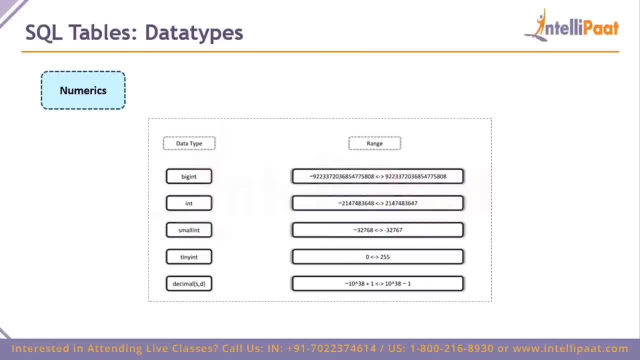 uh, you know, say you want to put a phone number, you want to put an address or whatever it is and you need this amount of number, the huge number. then you go on to use uh, the data type, what we call as the big int guys. then the normal integer supports pretty much uh in the data range that you can see. 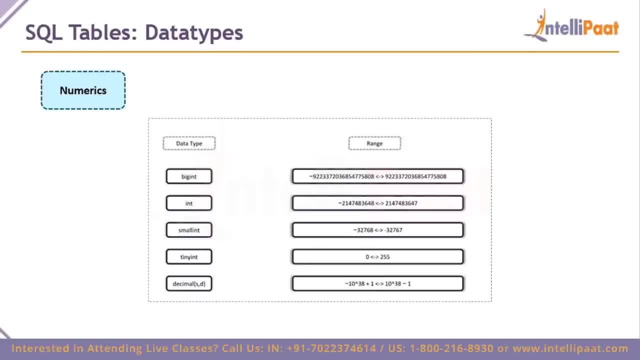 a fairly smaller number, somewhere around 32 000, and tiny int is even smaller, where it only supports positive numbers- between 0 and 255 guys, and then, with decimals, as usual, you have a huge number, access to huge numbers on the negative side and on the positive side as well, guys. 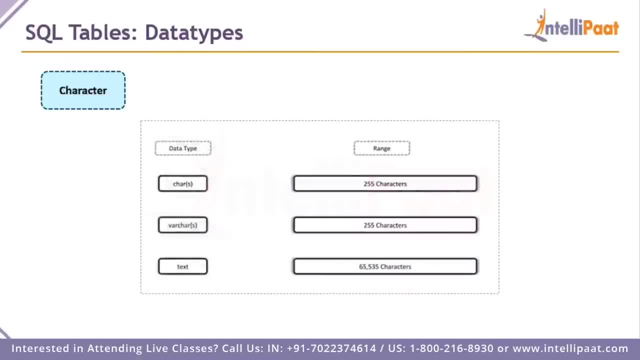 so this brings us to characters. there are three main data types: one is the car, one is the varchar and the text. again, pretty much, it is as simple. at this point of time, you need to know that you can have 255 characters at once. uh, when you're declaring something, when you're declaring the 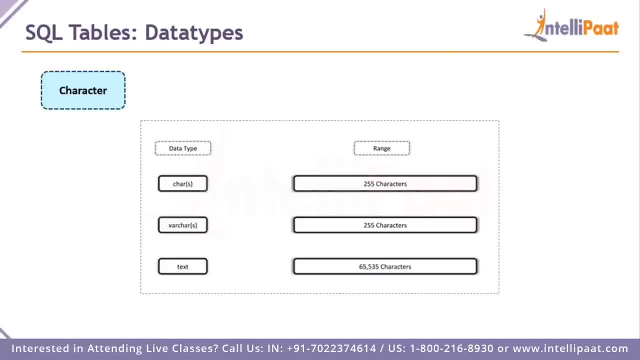 name of a data type, or when you're putting in the actual data for the data type as well. guys, so, but then we have something called as text, where let's say: you want to put in a description of something, so this, it will be a limit if we actually, uh say, 255 characters. right, so for that particular case, 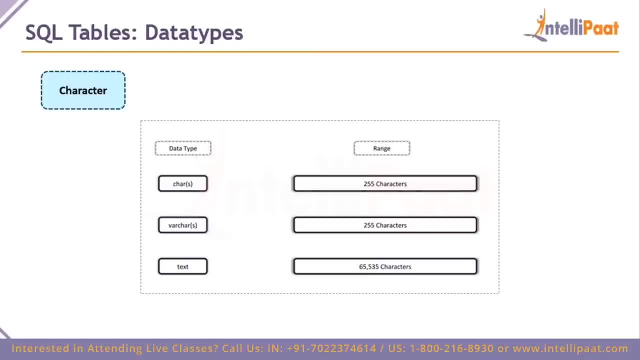 uh, you know, the standard sql manufacturers pretty much have given us a range of 65 535 characters where you can pretty much i think that should suffice. uh, you know most of the applications where we're using the data type text, where we are actually putting out some sort of description guys. 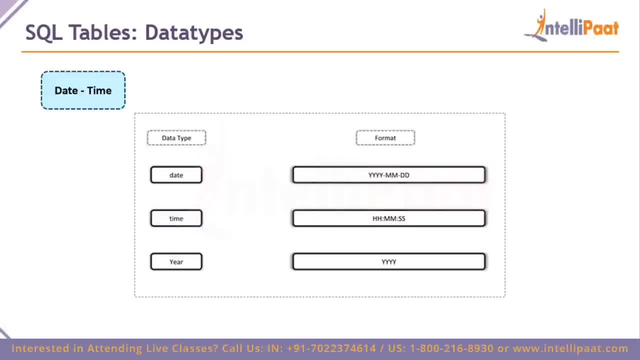 and then this brings us to the date time data type. well, basically, you can go on to using date format in the format your month day, and then you can go on to use the time as well- time in terms of hours, minutes and seconds as shown on your screen. and we can just use the uh data type- year uh- by showing 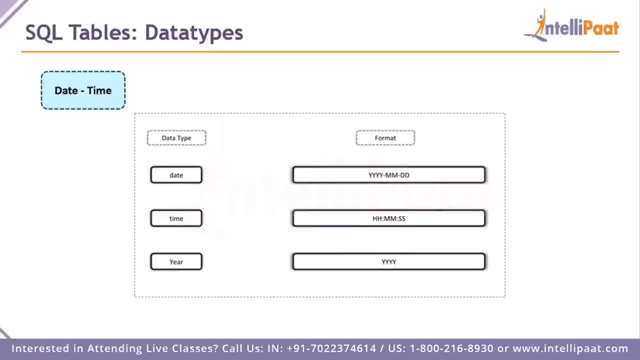 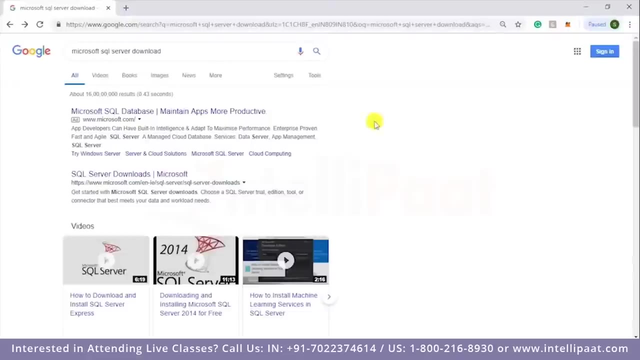 uh, you know by seeing the uh format on your screen as well, guys. so y y y y pretty much means four numbers. uh, if you have to put it down right now, it's 2019, so that'll be, uh, the format of the year. we'll be installing microsoft sql server, so all you have to do is go to google and then. 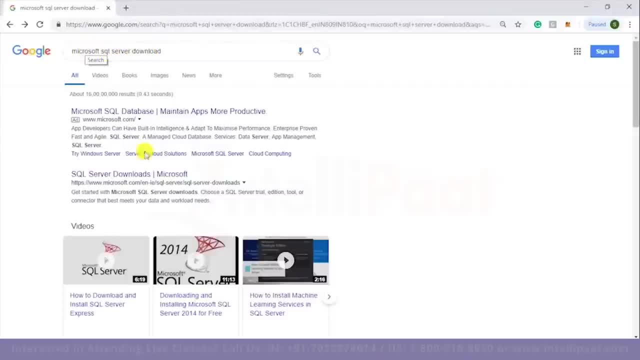 type: microsoft sql server download and you'll get these search results. now, out of these search results, click this one where you see sql server downloads from the microsoft site. so we are into the site. now, if i scroll down, we see two free editions. we have the developer edition and the 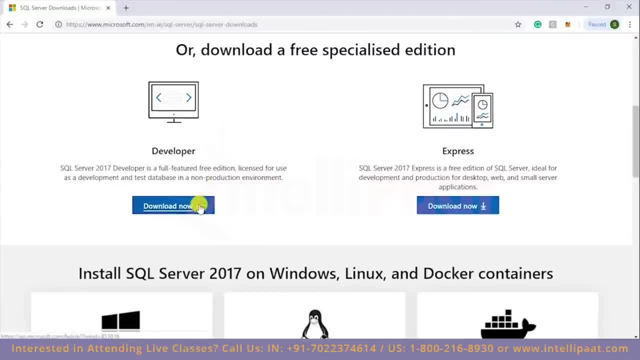 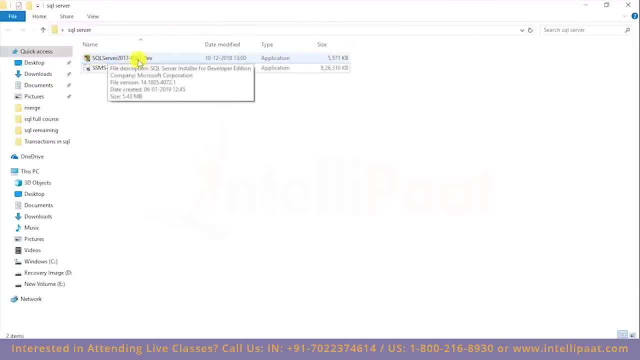 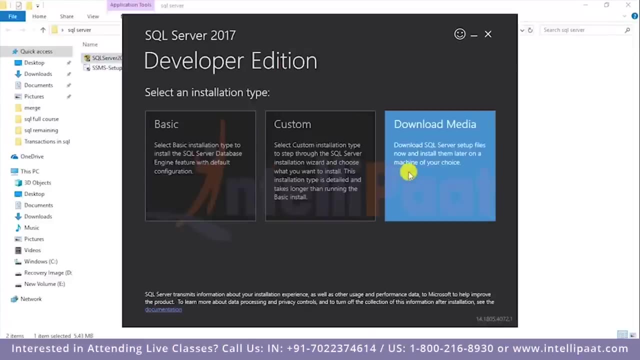 express edition, so i'd be downloading the developer edition. i'll click on download and the download. now this is the downloaded file over here: sql server 2017- ssei development. so we get this window over here and we have three options: basic, custom and download media. so i'll click on custom. 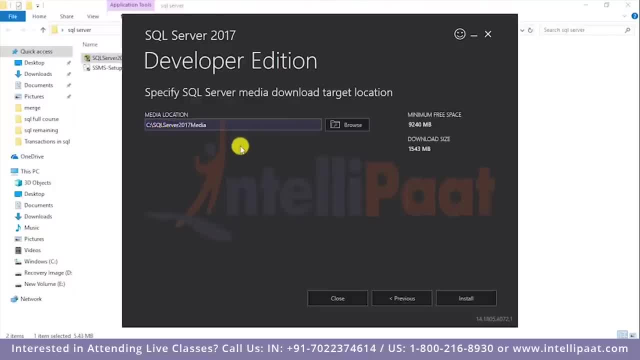 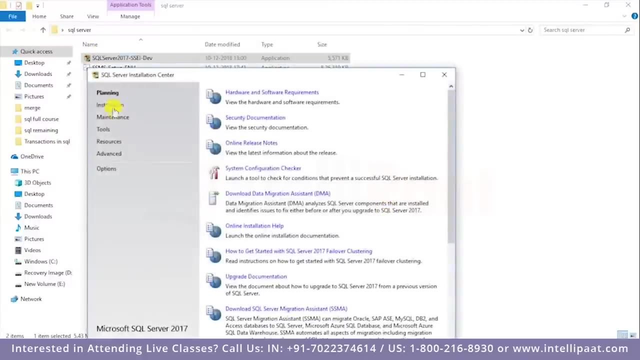 now we see that we have a media location where the sql server will be downloaded, and i'll click on install. you see that the download is successful and our installation will begin shortly. here i'll click on installation and i'll select this one, so i'll be installing a stand-alone. 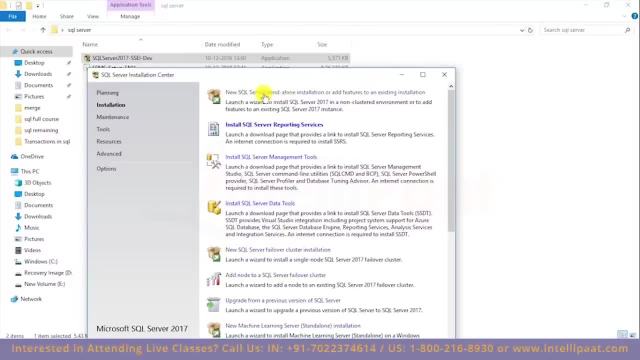 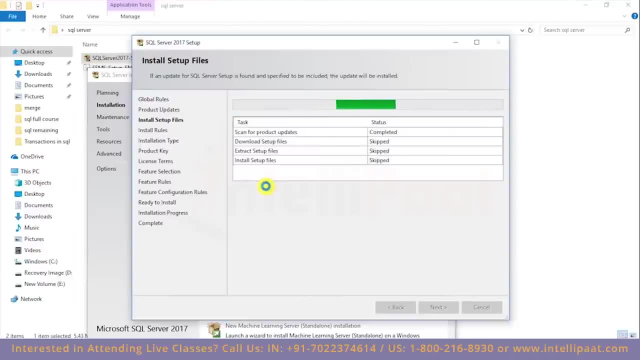 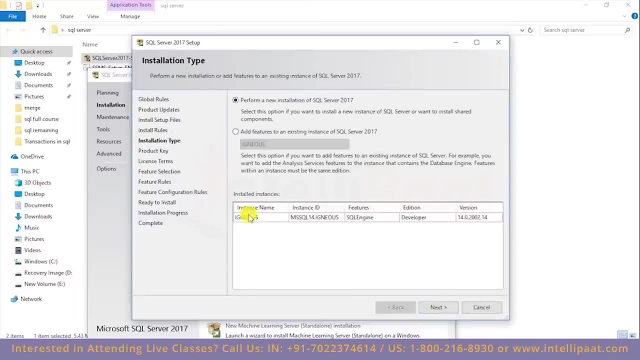 installation of the sql server. so let us wait for this to open. all right, so here i click on next. now i already have one instance of sql server, so i'll be installing a new one. so i'll uh click on next. select this: perform a new installation of sql server 2017, and then i'll select this free. 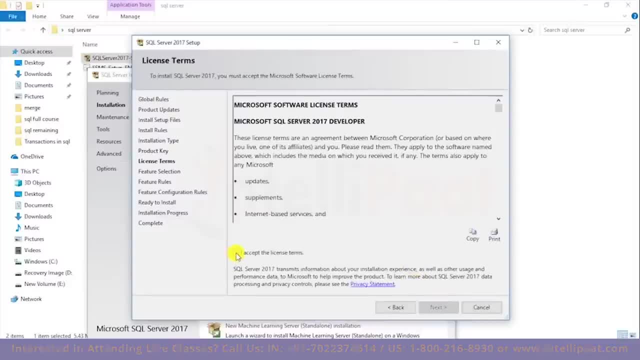 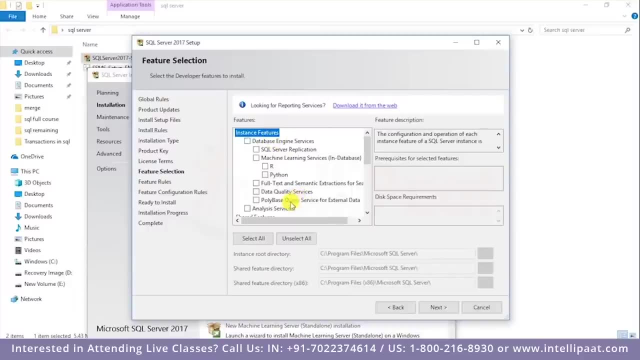 edition. i'll click on next. after that i'll accept this license agreement and again i'll click on next. so we have all of these features over here. so i would just need the database engine services. so i'll select this and again i'll click on next. 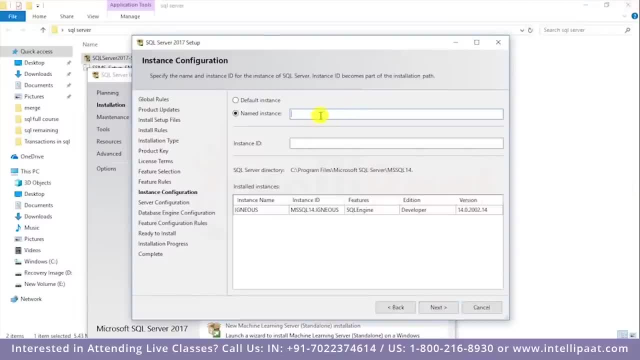 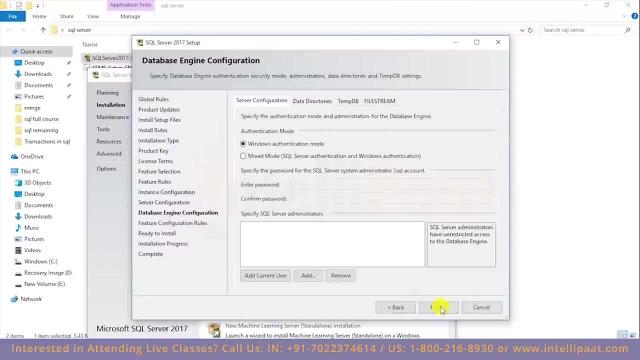 Bynum074Di boa the instance for the server which I'm installing. So I'll name this server as, let's say, Sparta. Similarly, I'll give the same instance ID over here. I'll click on next. So again, I'll click on next over here. So we see that we have two authentication. 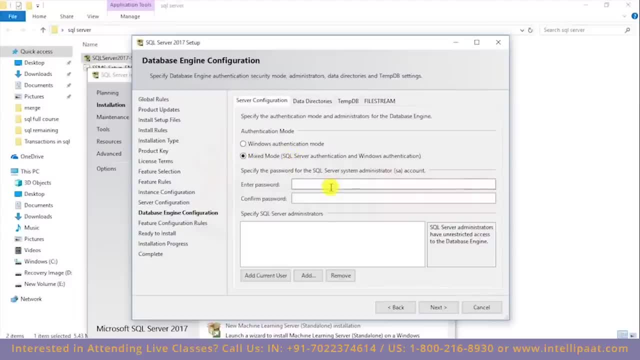 modes: Windows authentication mode and mixed mode. I'll select the mixed mode and then enter the desired password. Let me put in my password over here. I'll add the current user. So the current user has been added. Now I'll click on next again. 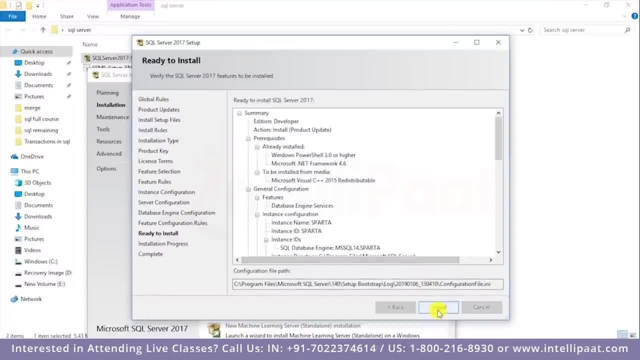 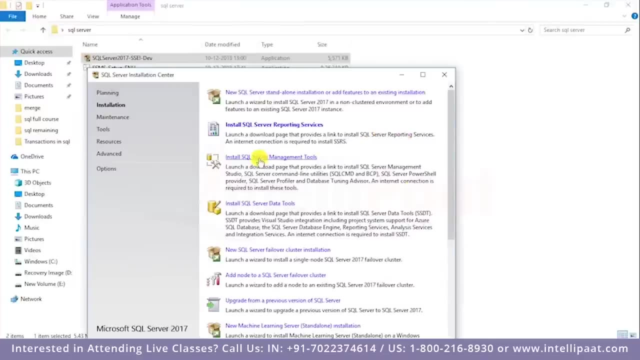 Right, so we are finally ready to install SQL server. I'll click on install Right. so once the installation is done, I would also have to install the SQL server management system. So the SQL server management tools basically help us to connect with the database. I'll click on this and this will redirect us to the. 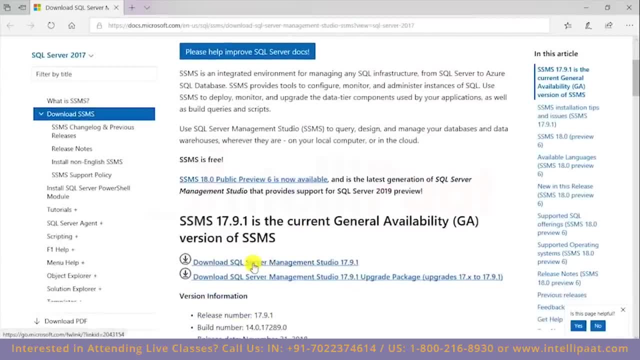 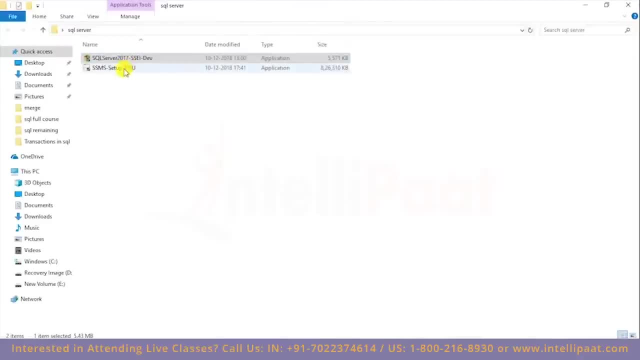 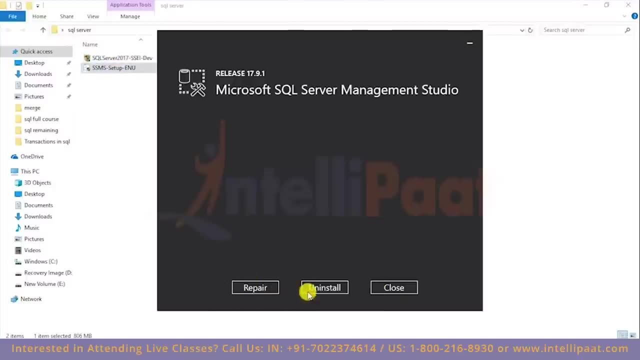 Microsoft web page and over here I'd have to download the SQL server management studio, and I'll be downloading the latest version And this is the downloaded file over here: SSMS setup- ENU. I'll click on this. So over here we have these three options: repair, uninstall and close. Now I have these three. 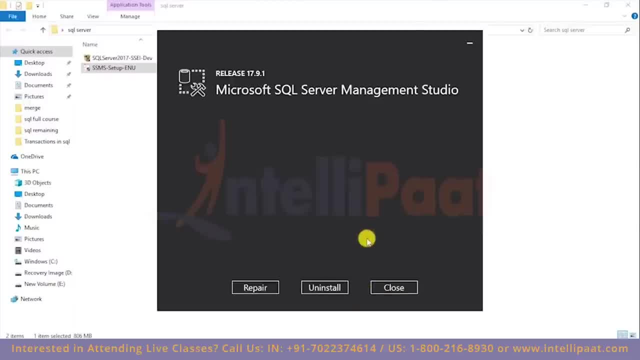 options, because I've already installed Microsoft SQL server management studio in my system and if you are installing this for the first time, you'll have the install button over here, So you'd have to click on install and the install would be done automatically, Right? so once you install the SQL server management tools, 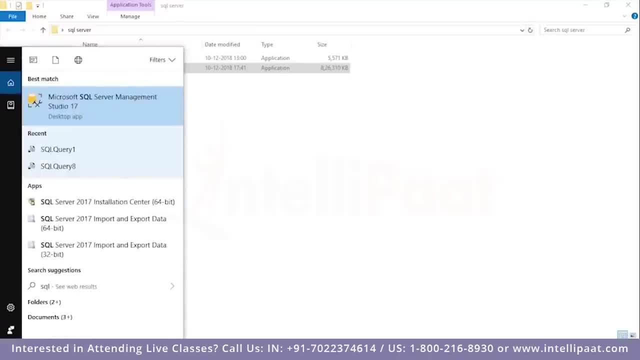 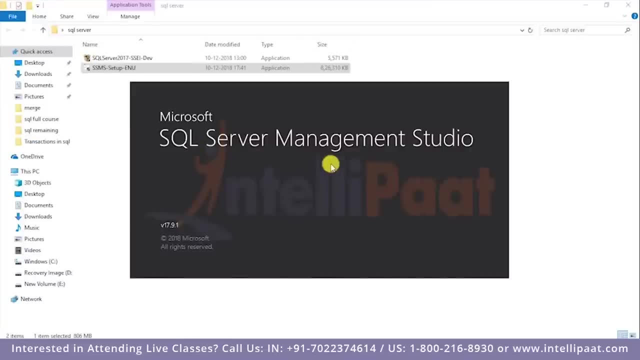 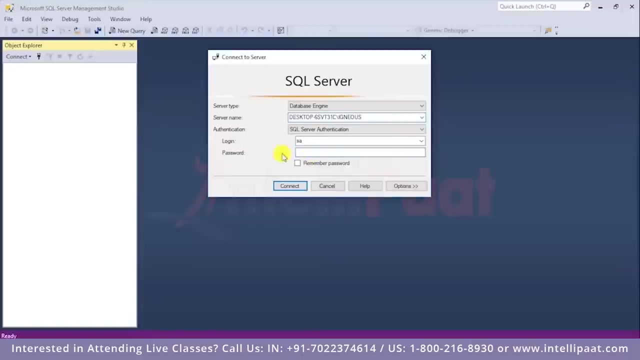 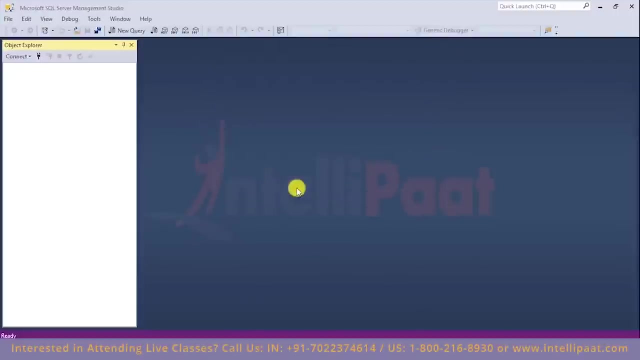 go to the search tool and type Microsoft SQL server management studio. Click on this and Microsoft SQL server management studio will start. So, over here you'd have to specify the password which you gave while creating the instance, And then click on connect And to start writing your SQL commands. 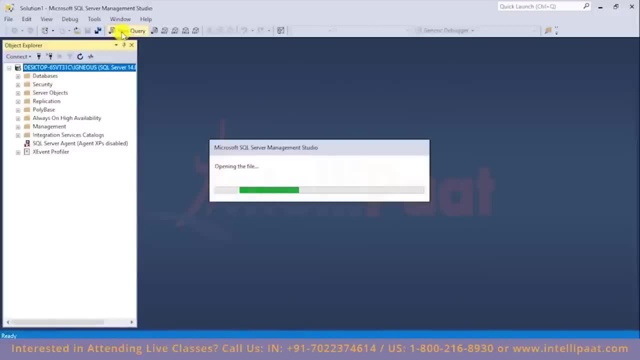 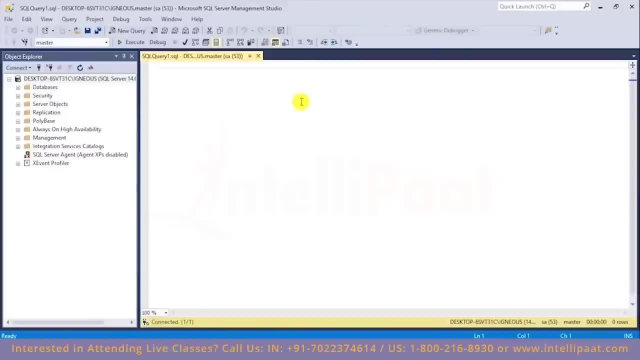 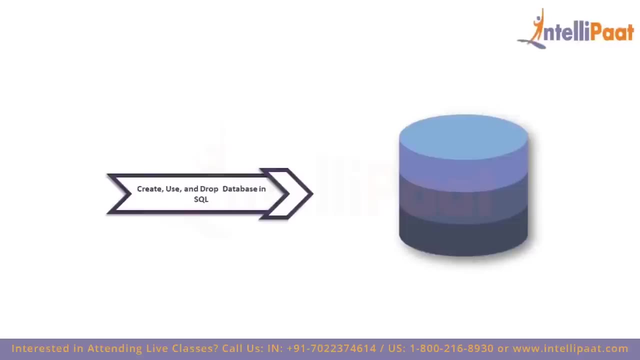 click on new query over here And then you can happily implement all of your SQL commands. Right? so this was the installation of Microsoft SQL server. How to create your SQL database. So this is the syntax to create a database in SQL. We will give in. 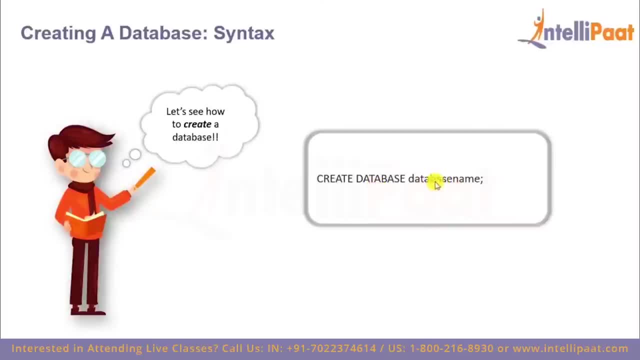 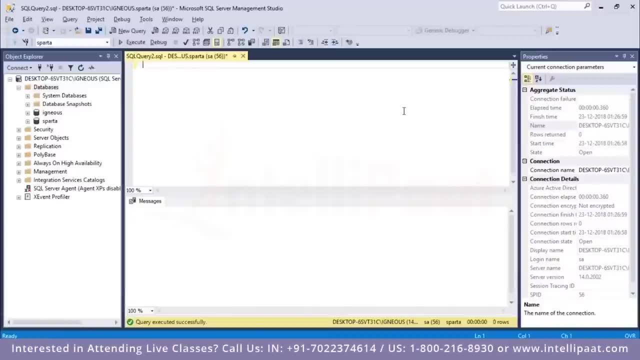 the keywords create database and then give the name of the database which you'd want to create. So let's go ahead and create a database in SQL, So let's create a first database, guys. So I will give in the keywords create database And let's say I want to name the. 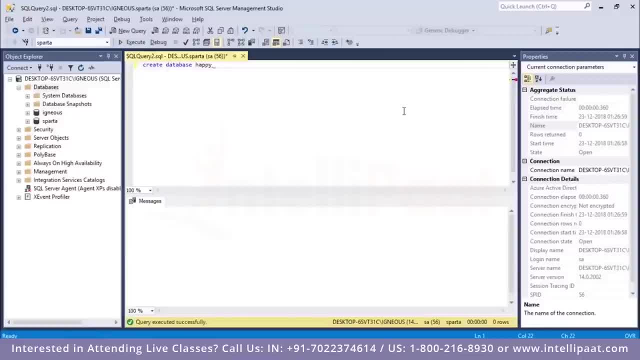 database as happy, Right. So I'll put a semicolon over here. I'll hit execute So see that commands have been completed successfully. Now let me hit refresh over here. So initially we just had two databases, igneous and Sparta. 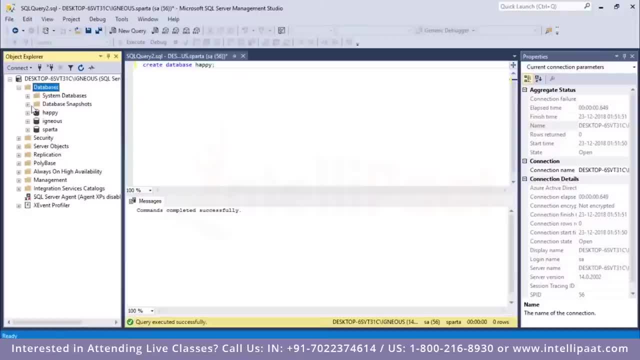 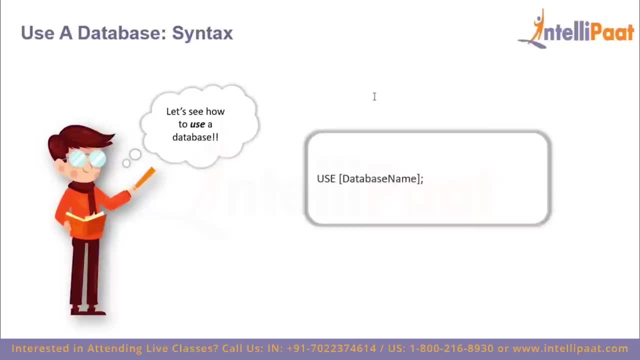 After implementing this command, create database- happy. we have successfully created a new database- happy. Now, after we have created a database, We need to know how to select a database from our existing list of databases. So we have the use database statement. for this, All we have to do is 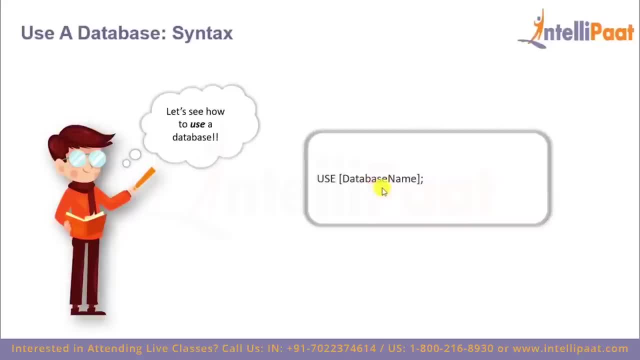 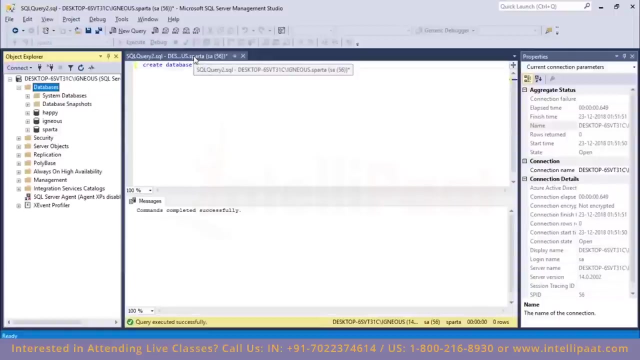 give the keyword use and then state the name of the database database. Now this database which you selected remains default until the end of a session or execution of another use statement with some other database. So if I put my mouse pointer over here, so you see that currently we are using the Sparta database. So now I 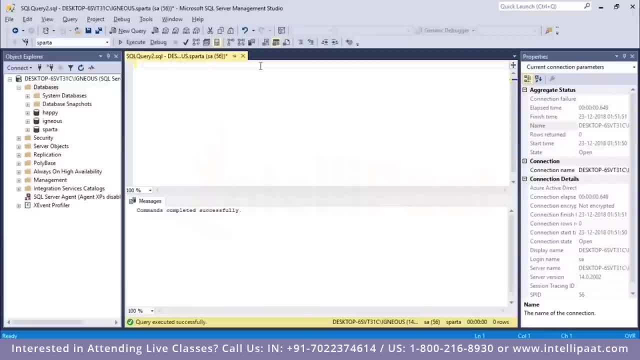 want to use the happy database instead of the Sparta database. So I will write the command for that use And then after that I need to give in the database which would be happy. I'll put a semicolon, I'll hit execute. So again, commands have been completed successfully. 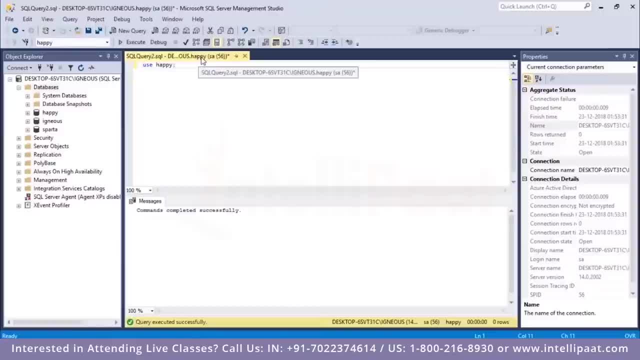 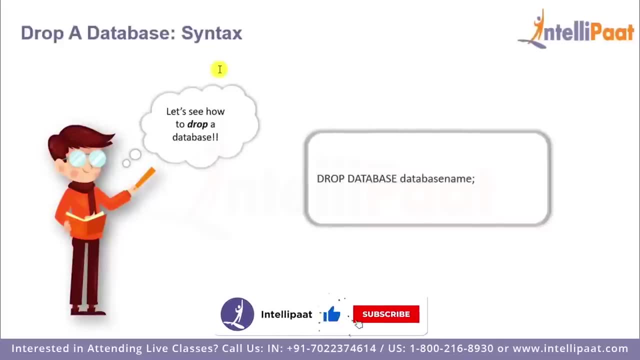 So now we see that the database has changed from Sparta to happy, So currently we are inside the happy database. Now we'll see how to delete a database, or in other words how to drop a database. So we have to give in the keywords drop database and then specify. 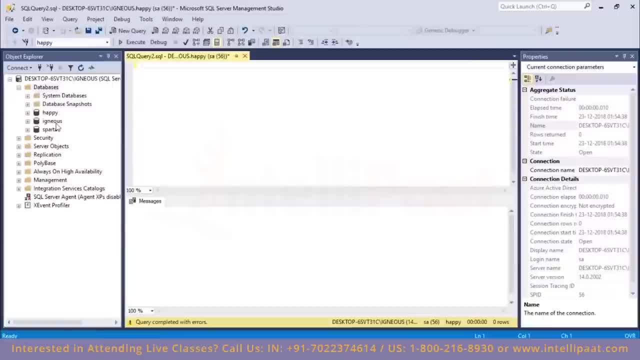 the name of the database which you want to drop. So now I'd want to drop this igneous database, So let me write the command for that Drop database, and then the name of the database is igneous, So I'll put a semicolon over here. 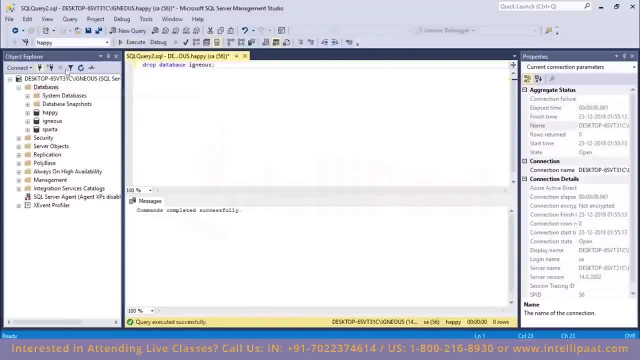 I'll hit execute. So again, commands have been completed successfully. Now I'll hit refresh. So we have only two databases: happy and Sparta. So database igneous has been dropped. So constraints are basically used to specify some rules on the data and limit the type. 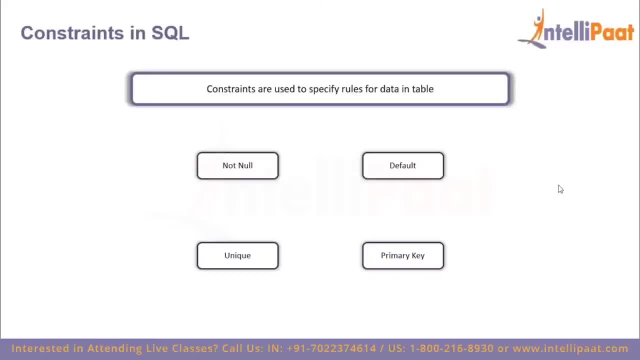 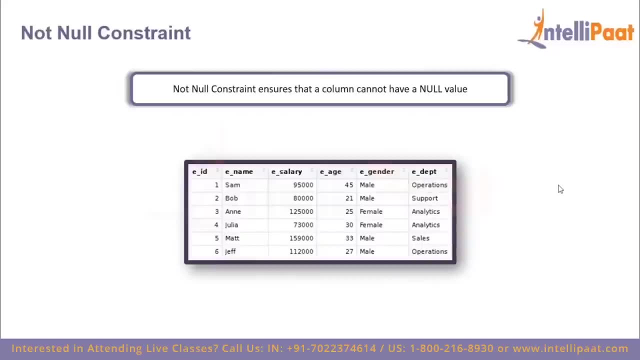 of data that can go into a table. We will look at these four constraints: not nil, but default, unique and primary key. Let's start with the not nil constraint. So by default, a column can hold null values And with the help of the not nil constraint, we can ensure 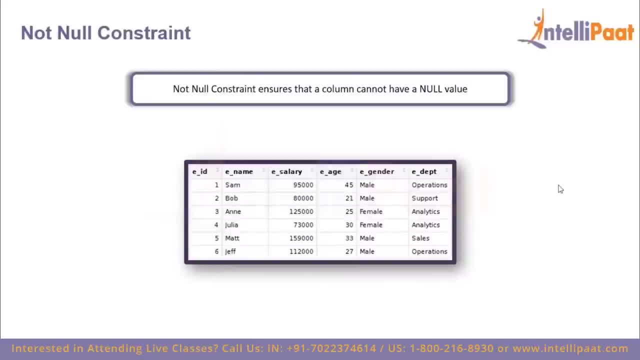 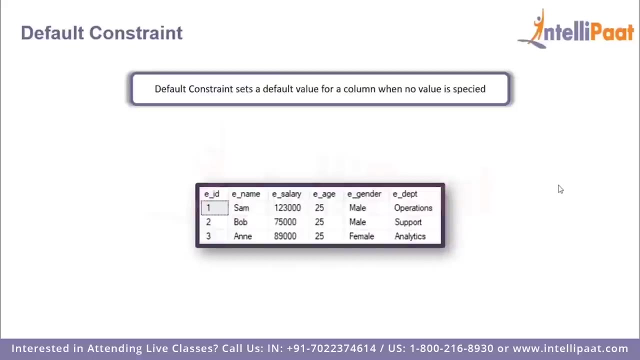 that a column does not have null values. So the not nil constraint basically ensures that a field always contains a value. For example, if we assign the not nil constraint to this ESALARY column over here, then every single entry of this column should have a value. 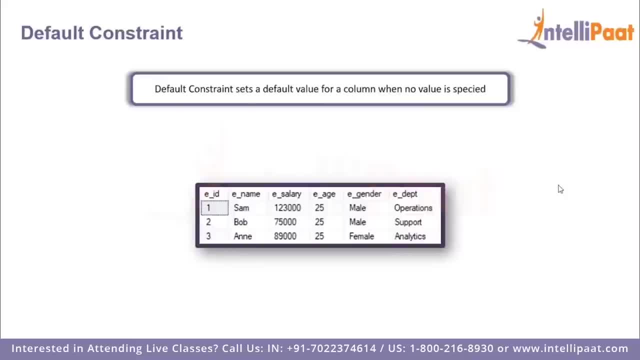 Then we have the default constraint. So the default constraint is used to provide a default value for a column. So the default value will be added to all the new records if no other value is specified. For example, if we assign the default constraint to the EH column and 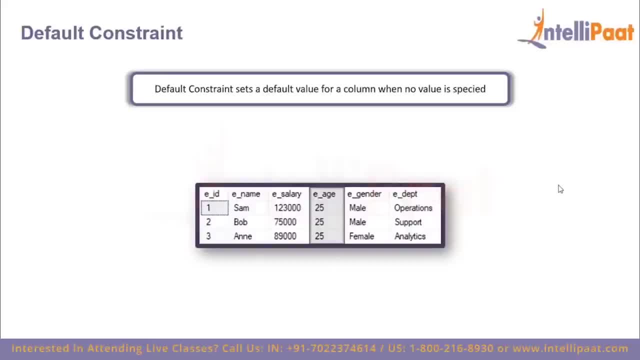 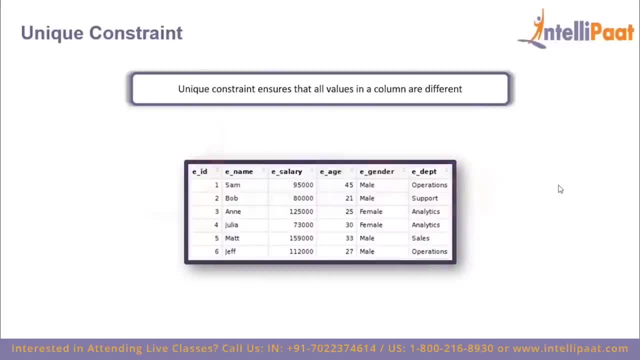 set a default value of 25, then all the entries of this column will have the default value of 25.. If no other value is specified during insertion, then we have the unique constraint which ensures that all the values in a column are the same. 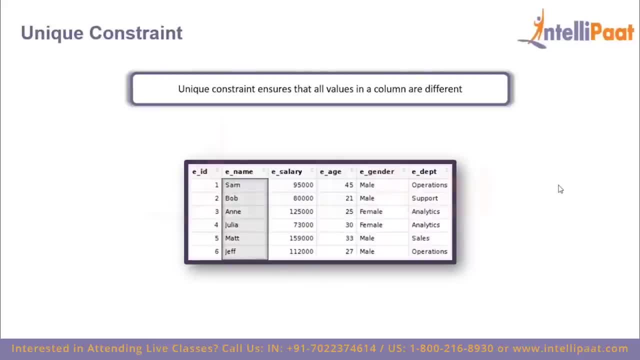 For example, if we assign the unique constraint to this ename column, then every entry of this column should have a unique value. And finally we have the primary key constraint. So the primary key constraint uniquely identifies each record in a table. Or simply put it: 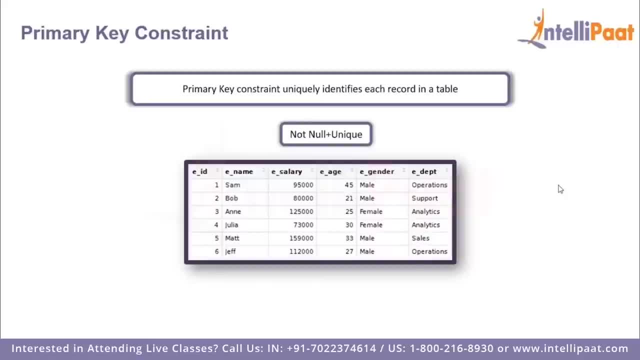 is just a combination of the not nil constraint and the unique constraint. So when we assign the primary key constraint to a column, then that column shouldn't have any null values and all the entries of this column should have a unique value. So the primary key constraint 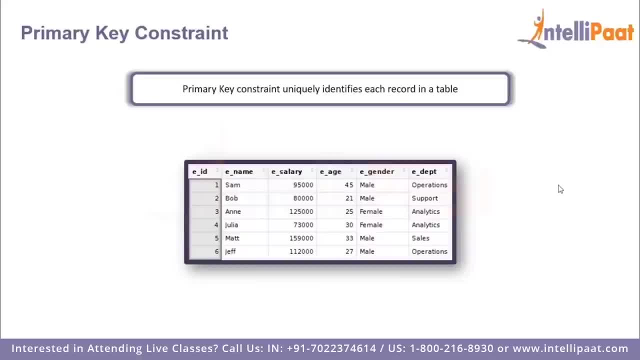 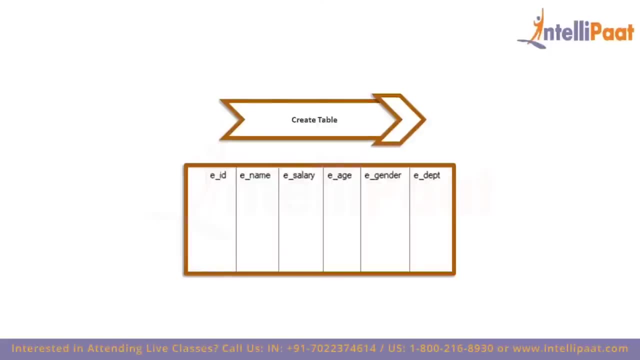 should also be unique. For example, if we assign the primary key constraint to the employee ID column, then there should be no null values in this column and all the entries should also be unique. How to create a table in SQL? So we'll be creating an employee table which would comprise: 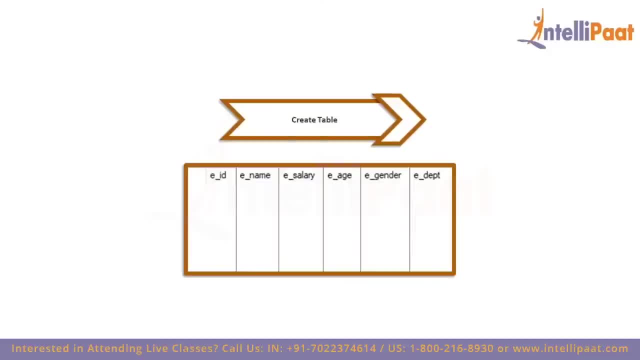 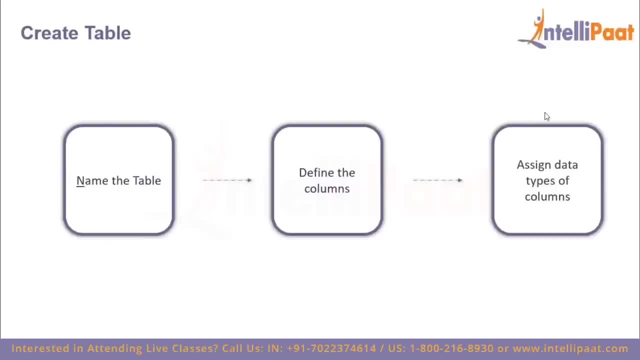 of employee ID, employee name, the employee's salary, age and gender and the department in which the employee works. So let's have a look at the steps to create a table in SQL. So first we'd have to start off by giving a name to the table. After naming the table: 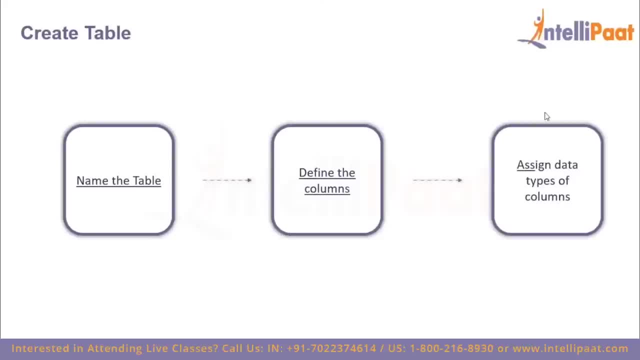 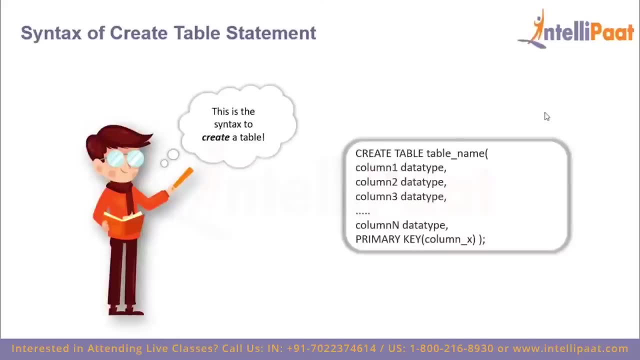 we'd have to define the columns which would be a part of our table And finally, we'd have to assign a data type to each of the column which we have defined. Now let's have a look at the create table syntax. So first we'd have to specify the two keywords which 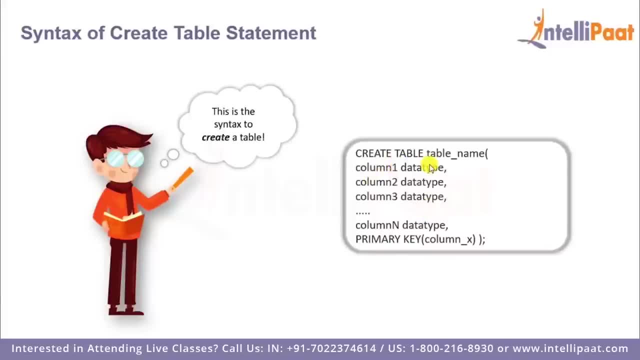 are: create table, and then we'll give a space and then give a name to the table And inside the parentheses, we will define all of our columns and assign them their respective data types. Now, finally, if you want to give a primary key constraint, we can do it over here. So, 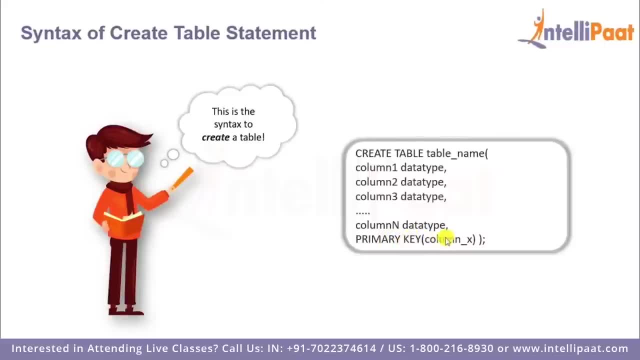 we will give in the keywords primary key and then given the name of the column which would be a primary key. So, as we have already learned in a previous session, a primary key basically helps us to uniquely identify all of the records in our table, And guys also. 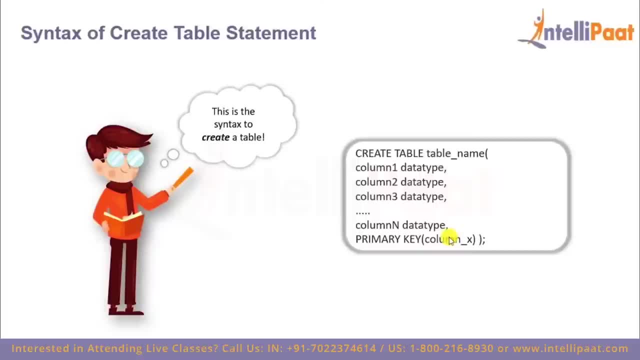 keep this in mind: a table cannot have more than one primary key. So now that we've understood the syntax of create table command, Let's go to MS SQL Server And create our employee table, Right? so this is MS SQL Server, So I'll start with the command. 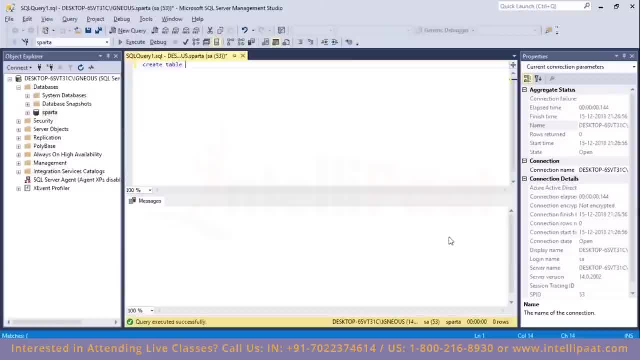 I will give in the keywords create table, then I will give in the name of the table, which would be employee, And inside the parenthesis I will give all of the columns. So the first column would be employee ID. So I will type E ID, which is the name of the first column. 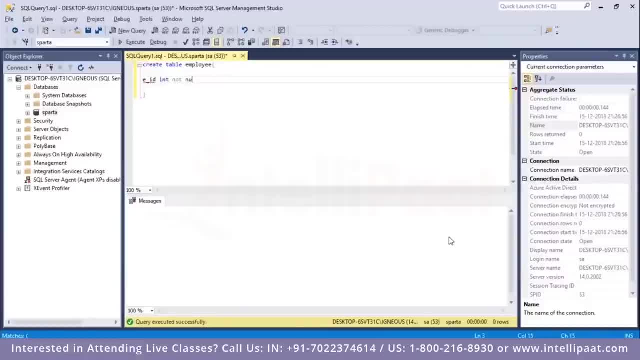 And this is of type integer. After this I will also put in the not null constraint, But all of the cells in this column should definitely have a value, And then I will give in the second column. So the second column is employee name, So E name, and this is of 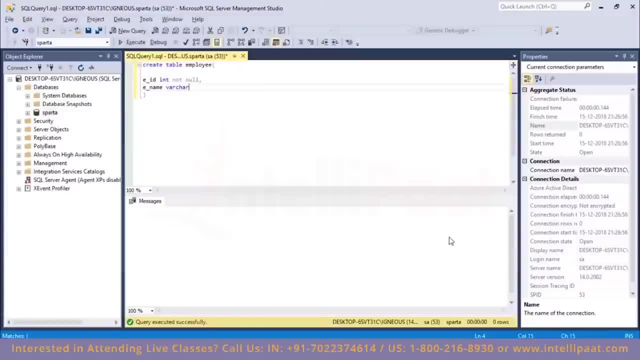 type varchar. So varchar stands for variable length character, and the maximum length would be 20.. Then I'll give in the third column. So the third column would be employee salary. So I will name the column to be E salary And this would be of type integer again After. 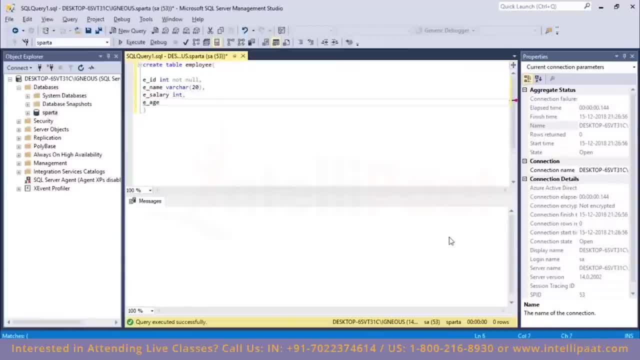 this. we have the employee's age, So the column name would be E age, and this is of type integer two. Then we have the employee's gender, So I will name the column to be E gender And this would be of type varchar. So this is of variable length, character and the maximum. 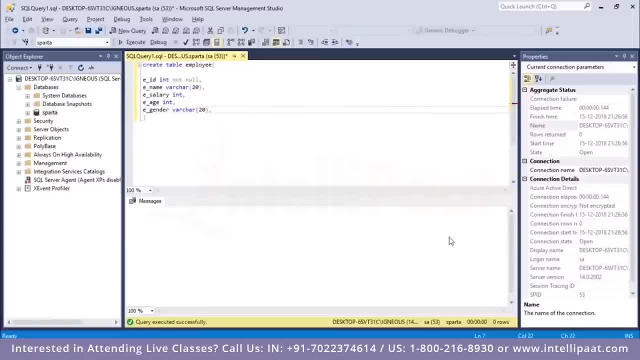 length is 20.. And then we will give in the final column. So the final column would be the department in which the employee works, So let me name it to be E, DETT, And this would be of type varchar, So varchar two and a maximum length of 20.. Now, after this, I can set in the primary key. 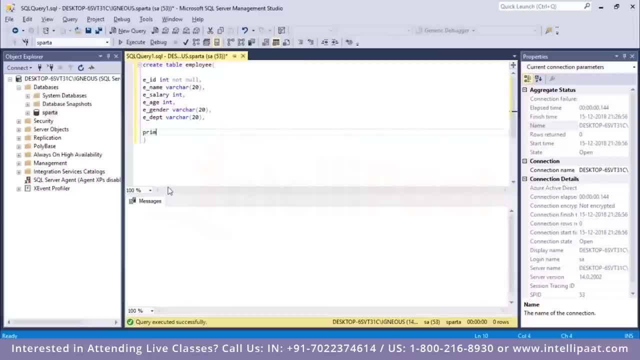 So I want this employee ID column to be the primary key. I will type primary key and inside the parenthesis I will give in E ID. Right Now. I will put in semicolon over here to indicate that this is the end of the syntax. I will select all of this and click on execute Right. 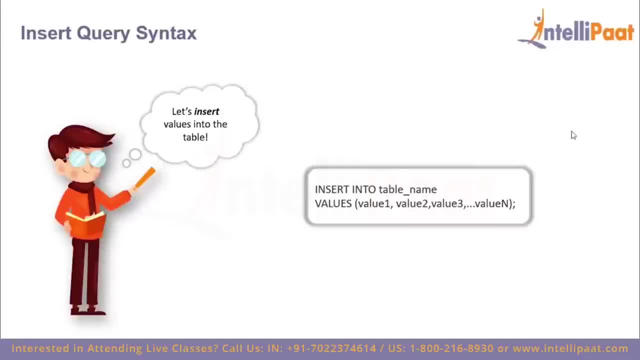 So we have successfully created the employee table. How to insert records into a table. We can insert records with this: insert into statement. Now let's understand this command properly. So first we'd have to type in the keywords insert into. then we'll give in the table name following which: 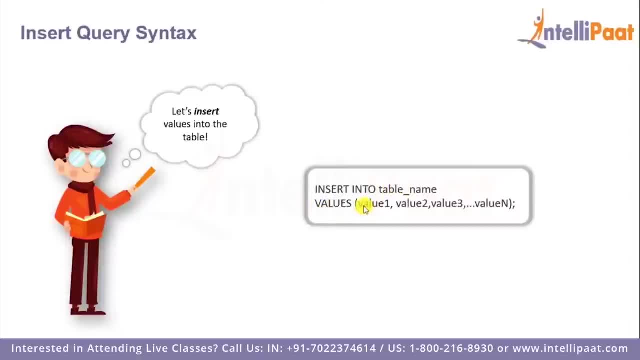 we'll give in the keyword values And inside the parenthesis we'd have to give in the values for each of the column respectively. Now let's go to MS SQL server and insert records into our employee table. So let me start with the command. So I will type in: 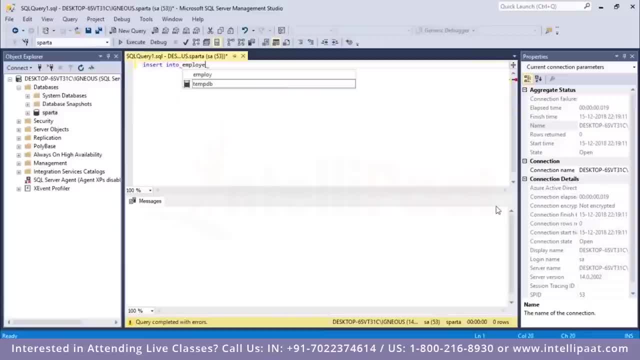 insert into, then I'd have to give in the name of the table, which would be employee, After which I will give in the keyword values And inside the parenthesis, I can give in all of the records. So let me start with the first record, Right? So we'll have to start off. 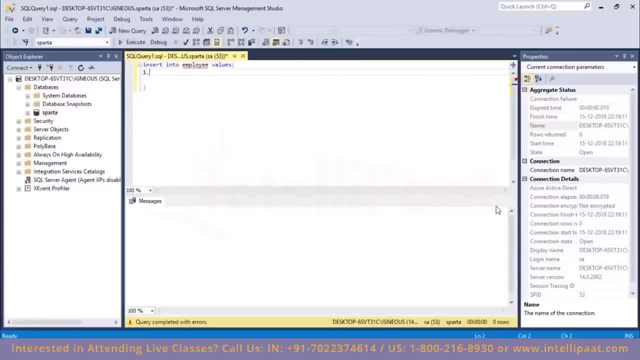 with the employee ID. So the employee ID is, let's say, one. Then the second column is the employee's name, And this is of type varchar. That is why I will give in the value inside these single quotes. So the employee's name is Sam. After this, we would have to give in: 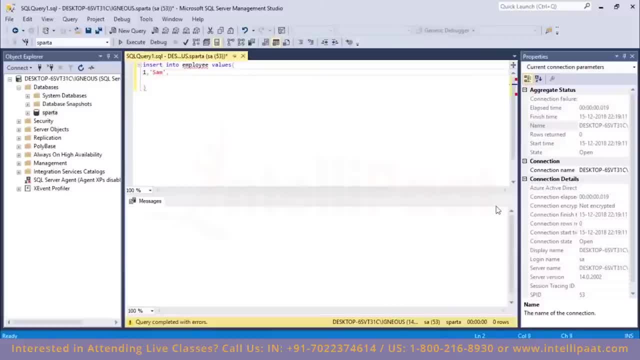 the employee's salary, So Sam earns $95,000 per annum. I will give in 95,000 over here. Then we have the employee's age, So Sam's age is 45.. After which we have the employee's gender, Again, since this is a variable character, so I will use the single quotes over here. 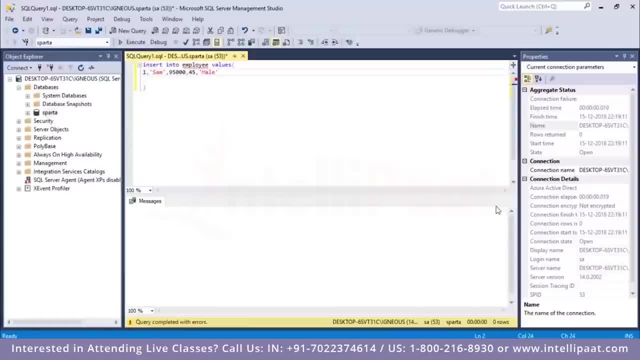 and Sam is male, obviously, After which we'd have to give in the department in which the employee works. So again, this is variable length character. I will give in single quotes and Sam works in operations. So let me type in operations over here Right Now. I will put in semicolon over here. I will 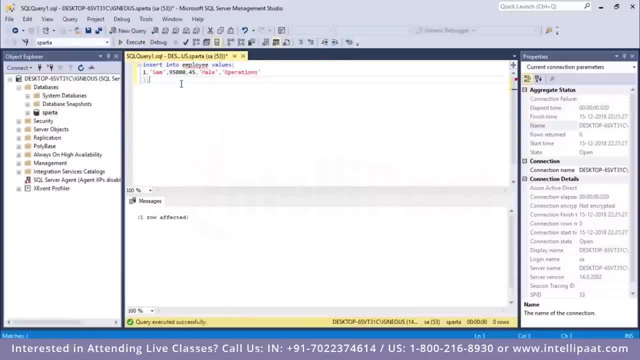 select all of this and I will click on execute. So we have successfully inserted one record into our table. Now let me follow the same procedure and insert another record. So insert into employee values And inside the parenthesis, the first column is employee ID, which would 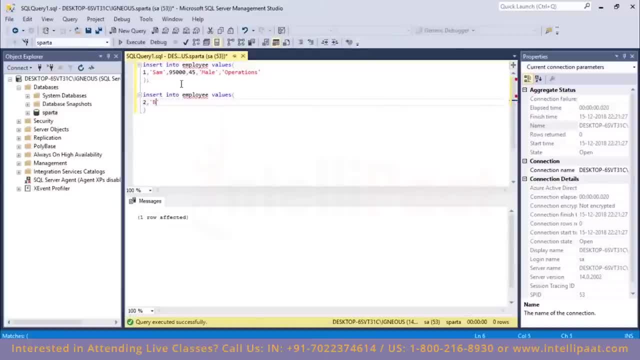 be do After this. I'd have to give in the name of the employee. So the name of the employee is Bob And Bob earns $80,000, which is his salary. So let me put in 80,000 over here. Then we have the employee's age, So Bob's. 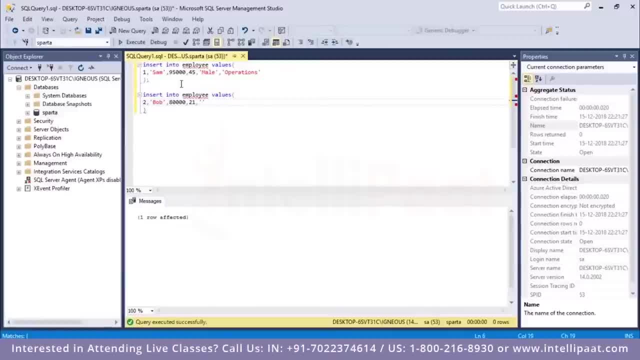 age is 21.. Then we have the gender of the employee. So Bob is male, obviously. again, Then we'd have to give him the department in which the employee works. So Bob works in support. Again, I will put in semicolon. I'd have to select all of these. Let me click. 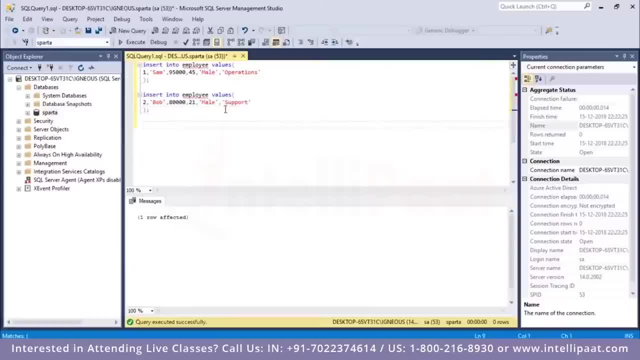 on execute Right. So we have also inserted the second record. Now let me insert the third record. So again it would be the same command: Insert into employee values inside the brackets. Let me give all of the values for the columns. So employee ID is three. The name is Ann. 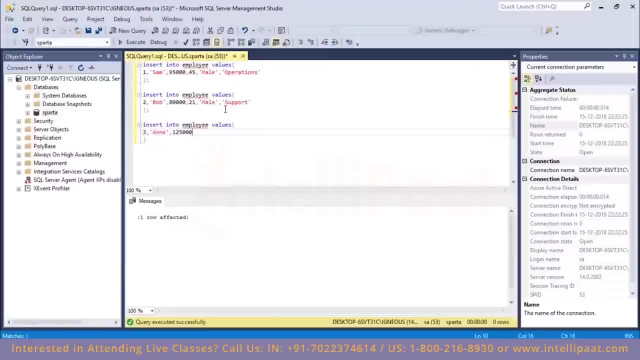 And Ann's salary is $125,000 per annum. She's quite rich, isn't she? And her age is 25.. And she's obviously female. Now, we'd have to give in the department in which the employee works. So Ann works in analytics. Let me type in analytics over here, So it seems like people. 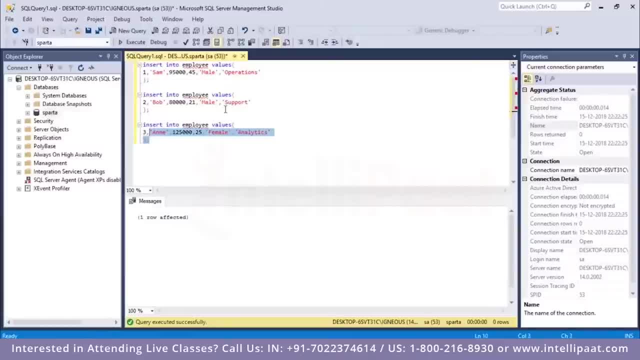 who work in analytics earn quite a lot, doesn't it? So let me put in semicolon over here. I'll select all of these and let me click execute. So, similarly, I will insert three more records into the same table. Right, So we have successfully inserted six records into our table. So, guys, this is how. 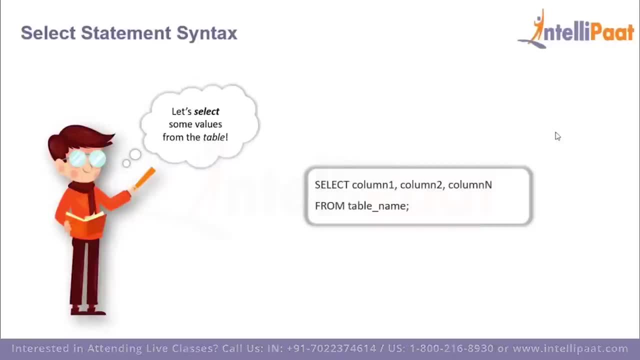 we can insert records into a table, How to select data from our table. So first we will work with the select statement and learn how to extract individual columns. Then we will work with the select distinct statement to select only distinct values. So the select query is one of the most important commands. 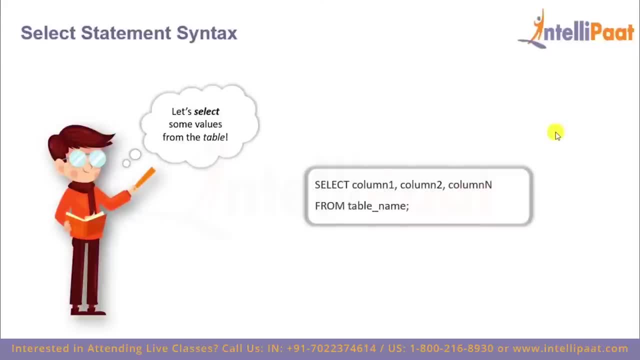 in SQL and it is used to get data from our table. So let's have a look at the syntax. So first we give the keyword select and then list down all of the column names that we want to select, Following which we will give the keyword from and then finally give the 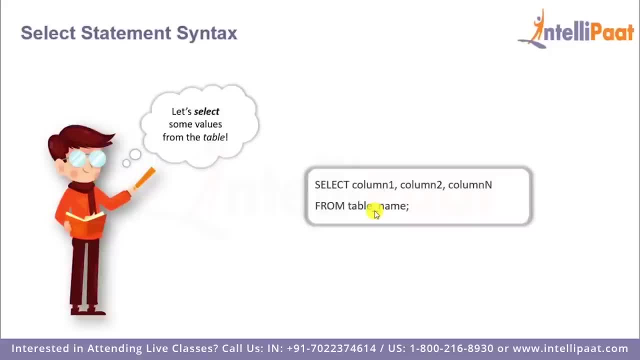 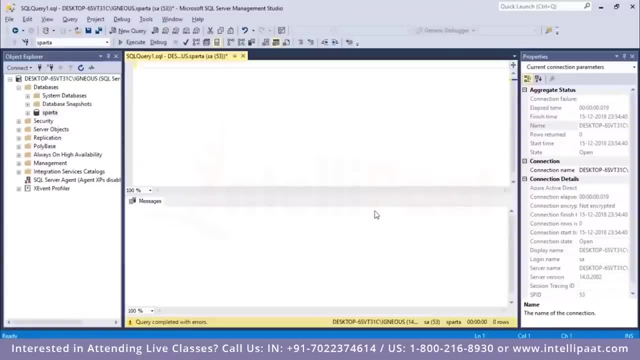 table name from which we are supposed to select these columns. So let's select some data from our employee table. So let's say I want to extract only the employee name column from the employee table, so for that I would have to give in select, and then I would have to. 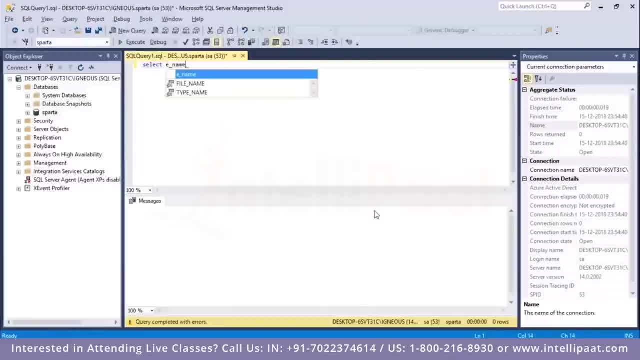 give in the name of the column. So the name of the column is ename, And then I will give in the from keyword, after which I will give in the name of the table, which is employee. let me put in semicolon and let me hit execute. right, so I have. 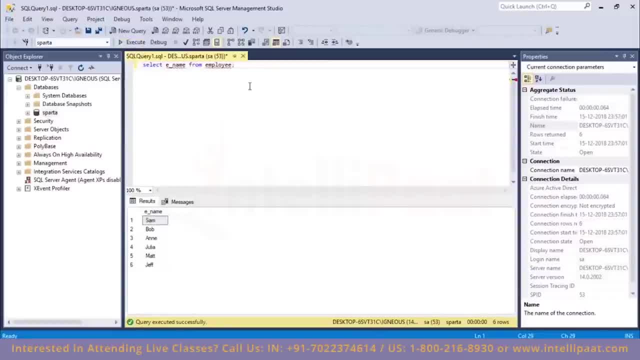 successfully extracted only the name column from the entire employee table. so similarly, if I wanted to extract only the age column from the employee table, we would have to put in a similar syntax so it would be select employee age from and the name of the table is employee execute right. so we 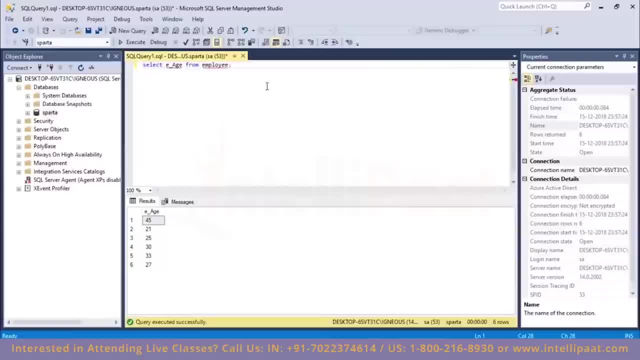 have extracted the age column from the entire employee table. now we can also extract multiple columns from our table, so for that we'd have to separate each of the columns with a comma. so let's say I want to extract the name column, the gender column and the salary column from the entire employee table. so let me write. 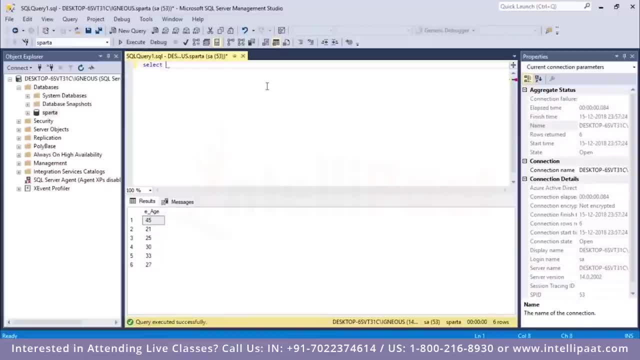 the syntax for that. so it would be select, select. I will give in the first column, which would be e name. now I would also want the gender, so I will put in e gender, I'll put in a comma, and then I would also want the salary column, so I will put in e salary, after which I will use. 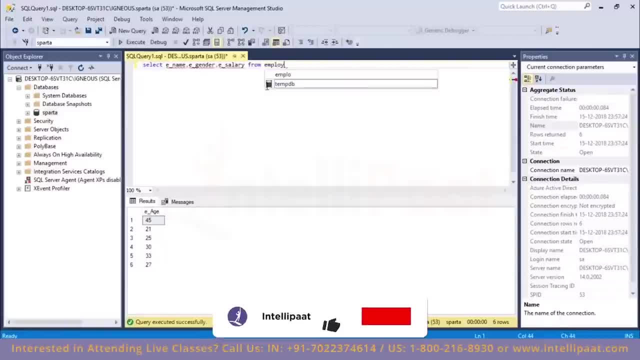 the from keyword and then I will give in the name of the table, which would be employee semicolon, and let me hit execute right. so I have extracted three columns from the employee table, and those three columns are e name, e gender and e salary. so this is how you can extract multiple columns from the same table. now we can. 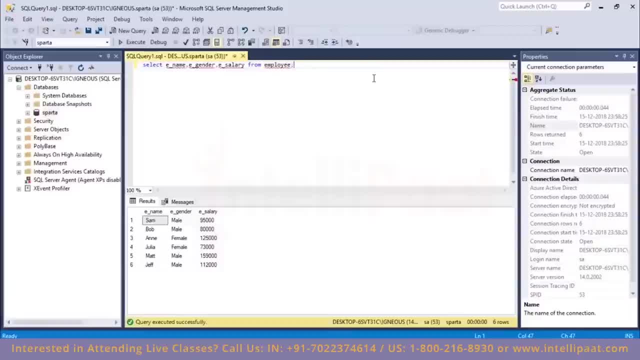 also extract the entire data from our table. and to extract the entire data from our table we have to use the asterisk operator. so let me show you, guys, how it's done. so the command would be select and then I will put in star, after which it will be from employee. so as simple as that, guys. select star from. 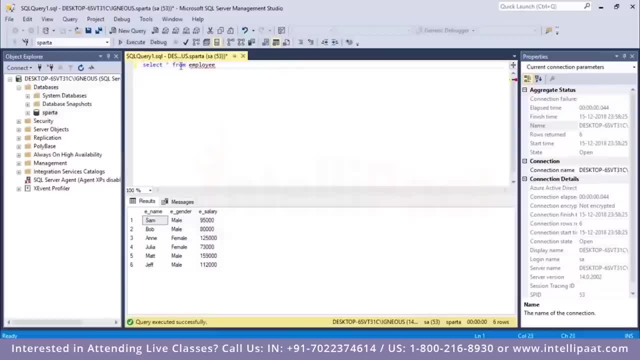 employee. so whatever table it is, all you have to do is select star from and then you would have to give in the table name. so this is extract all of the data from a particular table. so i will give in semicolon and let me hit execute right. so when i gave the command select star from employee, i was 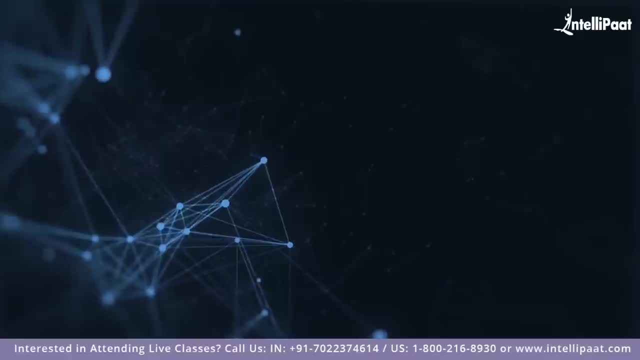 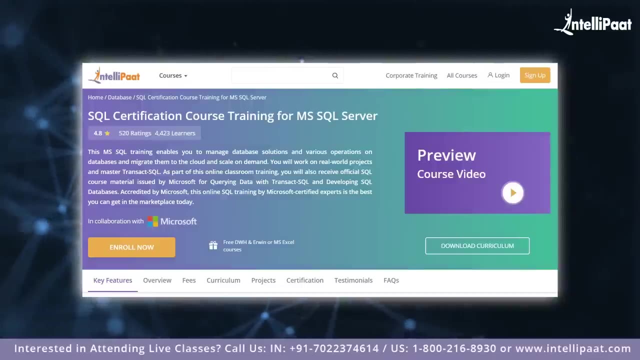 able to extract all of the data from the employee table. just a quick info, guys. intellipaat provides sql online training in partnership with microsoft and mentored by industry experts. the course link is given in the description below. now let's continue with the session. now let's look at: 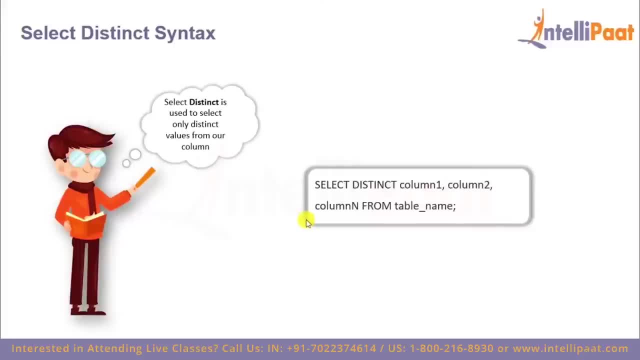 the select distinct statement. so a column often contains many duplicate values and sometimes we'd want to extract only the distinct values from the column. so this is where select distinct comes in. so the syntax of select and select distinct is pretty much the same. the only difference is we: 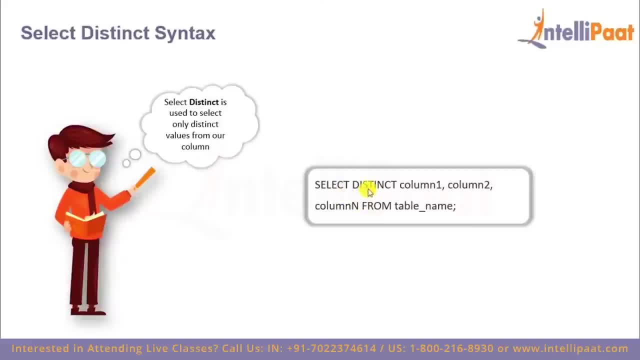 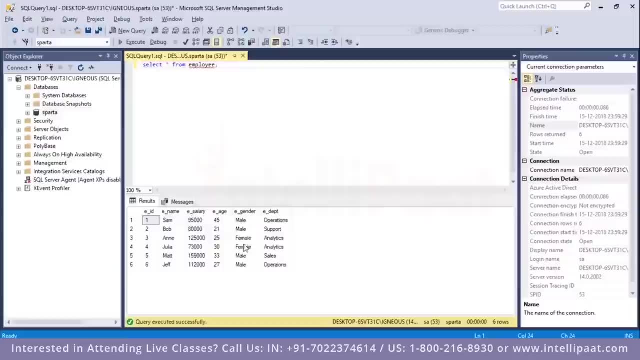 follow up the select keyword with the distinct keyword. now let's select some distinct values from our employee table. if we have a glance at this gender column, we see that these two values are being repeated. so we just have two values, male and female, and these two values are being repeated. so now, if i 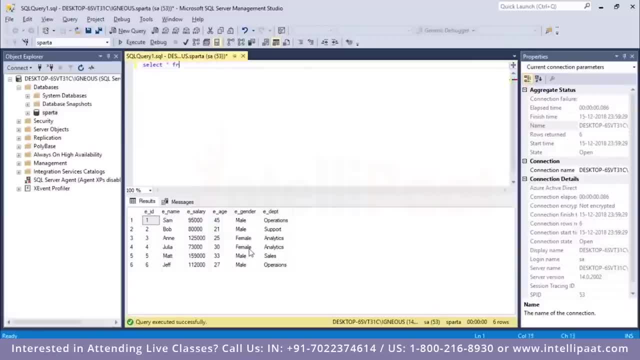 wanted to extract only the distinct values, so this would be the command for that. so i will type in select and i'll follow up the select keyword with the distinct keyword, after which i'll given the column name whose distinct values i'd want. so the column name would be e- gender, and then it'll be. 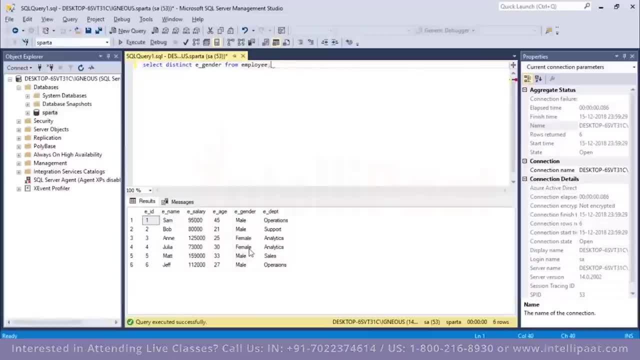 from the name of the table, which is employee. so let's see what do we get? select distinct e gender from employee, right? so we see that we only get the distinct values which are female and male. now let me actually remove this distinct keyword and let me execute. so let's see what is the 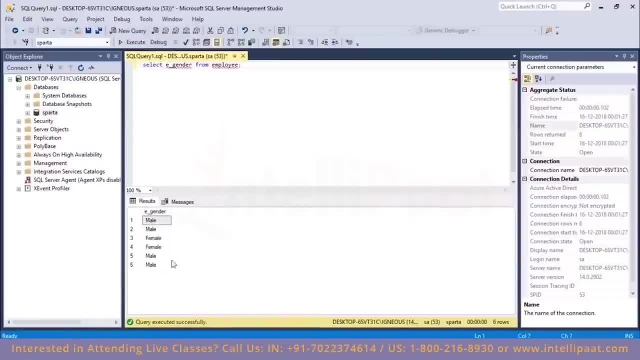 difference right. so if i remove the distinct keyword, we get all of the values. so male, male, female, female, male and female. now so if we use the distinct keyword, we'll only get the values which are different. so these are the cases where select distinct can be used. so the where. clauses used to extract only those records that are distaced values. so we'll use the whereas button ourselves. they are formed. Now I want to show you that the values of them are distinct values which are different than the other ones. Let's do the final application here. these are the cases where select distinct can be used. so the where closets used to extract only those records that are this like extremities. 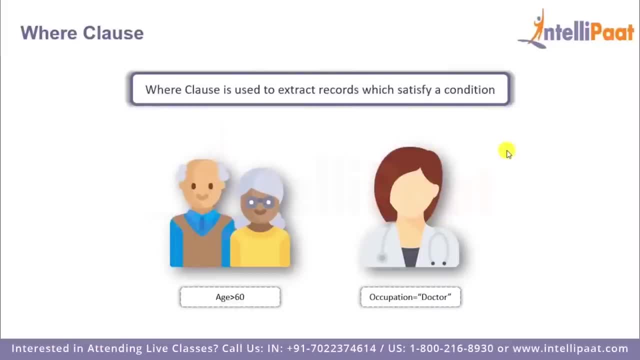 WhereS Creole AKA possible factors be expected: those records that fulfill a specified condition. For example, we'd want to extract those records where the age of the person is more than 60, or filter out those records where the occupation of the person is doctor. Now let's have a. 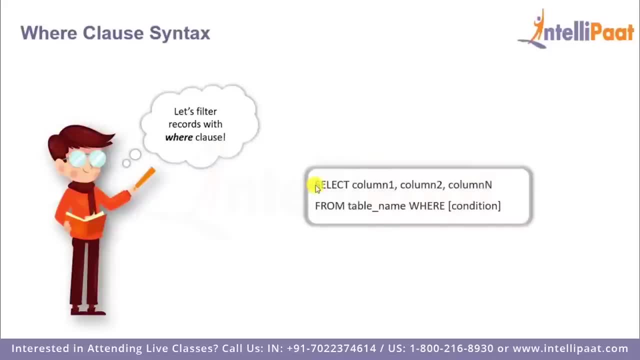 look at the syntax of where clause. So we'll start with the select keyword, then we will give in the list of all of the columns which we want to select, following which we'll use the from keyword and give the table name and finally use the. 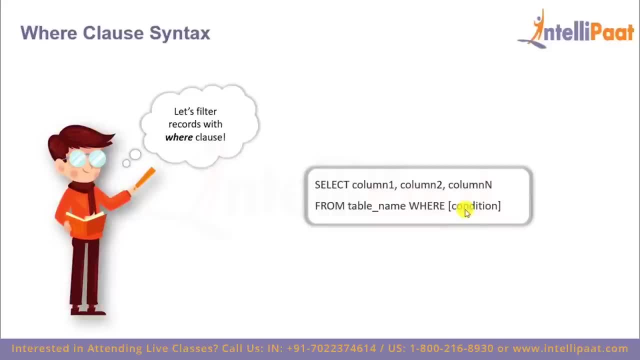 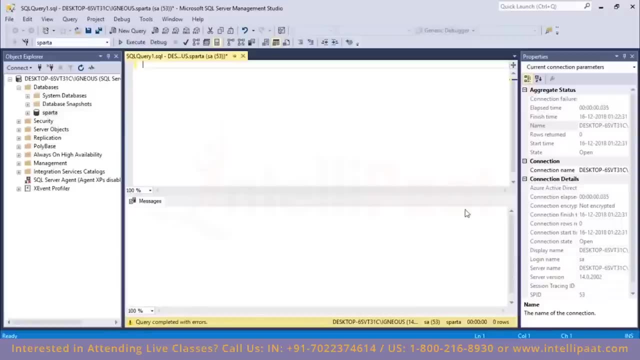 where keyword, and follow it up with a condition that would determine which records are to be extracted. So let's filter out some records from our employee table. Now let's say we'd want to find out all of the female employees of our company, So for this I'd have to extract those records where the gender equals. 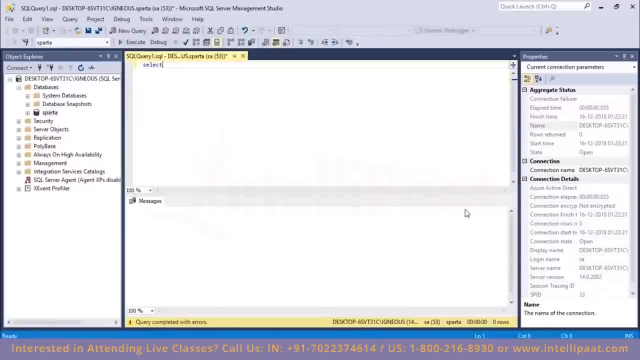 female. So let me go ahead and write the command for that. So that would be select star from: I will give in the table name which is employee, and then I will use the where keyword And follow it up with the condition. So the condition would be e. gender is: 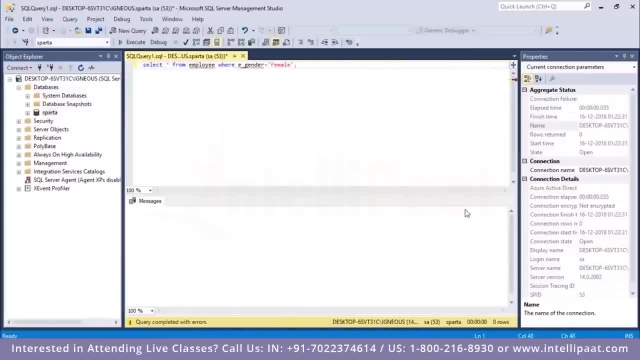 equal to female Right. so what I'm basically doing is I am extracting all of the female employees from this employee table. Let me hit, execute Right. so Ann and Julia are the only female employees. Now I'd want to find out those employees whose age is less than 30. So let me write the command for that. 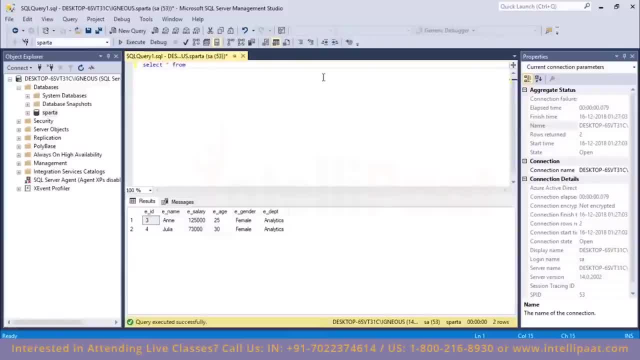 So I'm going to go ahead and select star from employee where I will give in the condition. So this time the condition would be: e, Age is less than 30. Right, so the age needs to be less than 30.. I'll give a semicolon. Let me hit execute. 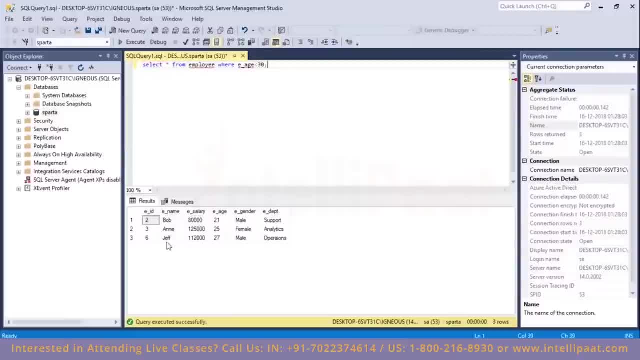 Right, so these are three employees, or these are the three records where the value of eAge is less than 30. So Bob, Ann and Jeff, these are the three employees. age is less than 30. Now, similarly, let's say, I want to find out all of those. 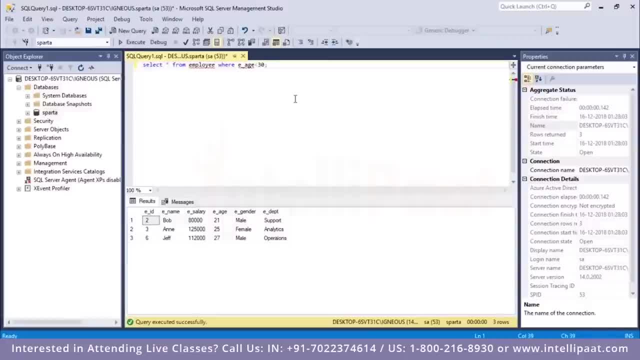 employees whose salary is greater than hundred thousand dollars. So let me write the command for that. So this time the command would be: select star from employee, where, so the condition would be: e salary is greater than hundred thousand, semicolon and execute. So, and Matt and Jeff are the three employees whose 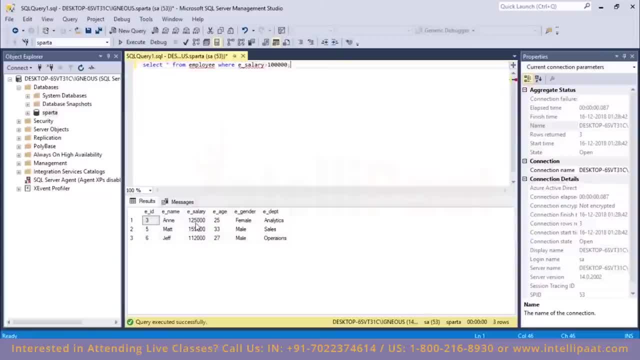 salary is greater than hundred thousand dollars. So, and salary is hundred and twenty five thousand dollars, Matt's salary is hundred and fifty nine thousand dollars and Jeff's salary is hundred and twelve thousand dollars. So, guys, this is how we can filter out records with a var clause. How to extract. 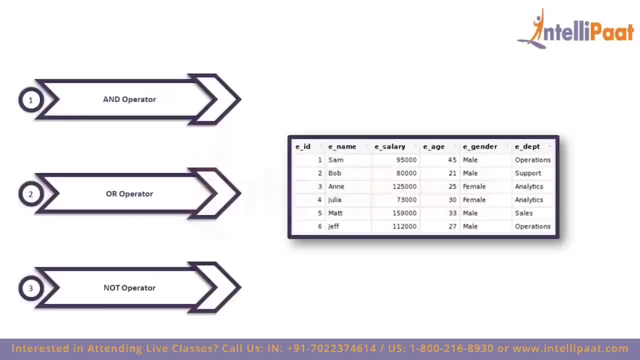 records on the basis of multiple conditions using the AND, OR and NOT operators. So we'll start with the AND operator first, then we'll filter records with the OR operator and finally we'll work with the NOT operator. So with AND operator we can basically fetch: 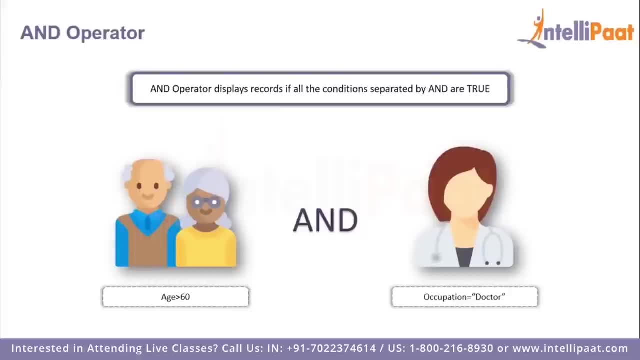 those records which satisfy all of the conditions separated by AND. For example, you want to find out all the doctors whose age is greater than 60. So there are two conditions over here. First, the age needs to be greater than 60.. Second, the occupation needs to be doctor. So we'll get only those records. 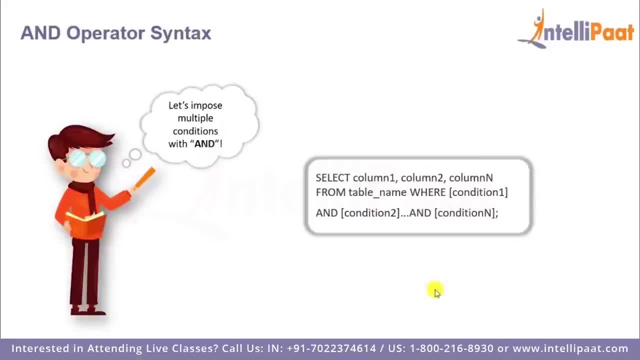 where both the conditions are being satisfied. Now let's have a look at the syntax. So here, after we give the first condition of the var clause, we follow it up with the AND operator and give the second condition. And similarly, if we have another condition to be satisfied, we'll again give the AND operator and. 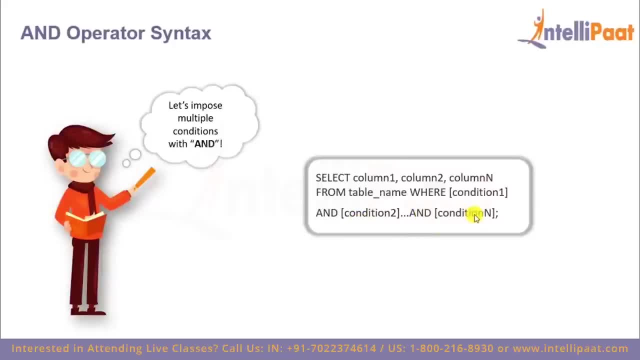 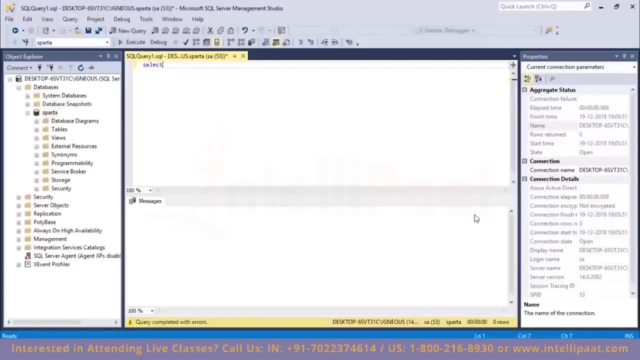 then give the next condition. So let's fetch some records using the AND operator. So I want to extract all of those employees whose gender is male and age is less than 30. So the command would be: select star from employee. I'll use the var clause and then give in the first. 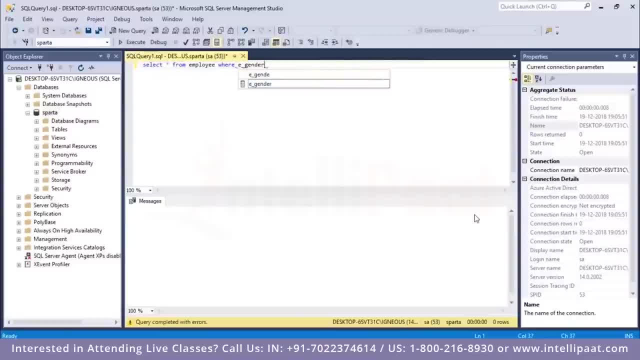 condition. So the first condition is gender needs to be equal to male. So egender is equal to male. I'll use the AND operator and then give in the second condition. So the second condition is the age needs to be less than 30.. 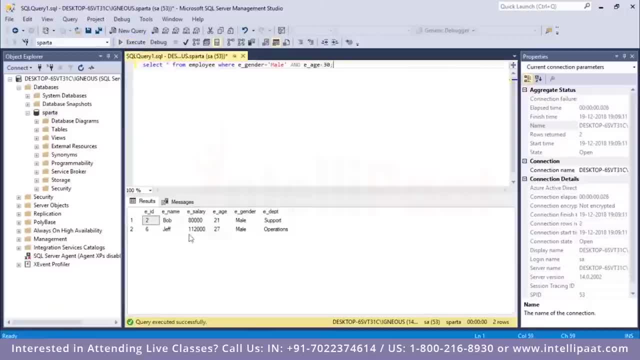 Let me hit, execute Right. so Bob and Jeff are the two employees whose gender is male and age is less than 30. Now, similarly, I'd want to extract all of those employees who work in the operations department and their salary is greater than hundred thousand dollars. So the command would be select. 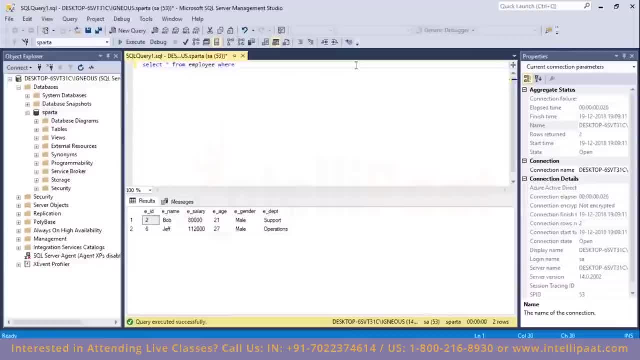 star from employee where I have to give the first condition. So the first condition is the department needs to be equal to operations. I'll use the AND operator again And then I'll give the second condition. So the second condition is the salary needs to be greater than hundred thousand dollars. Right Execute. So, Jeff. 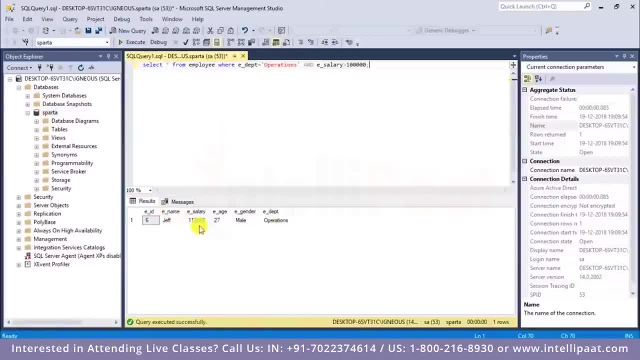 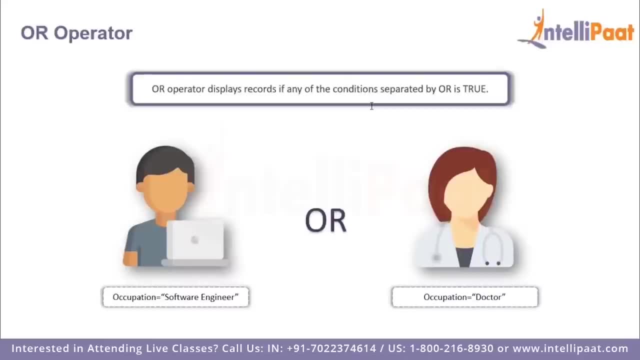 is the only employee who works in operations and his salary is greater than hundred thousand dollars. Then we have the OR operator. So the OR operator displays those records where at least one of the conditions is satisfied, For example, if we want to filter out either a software, 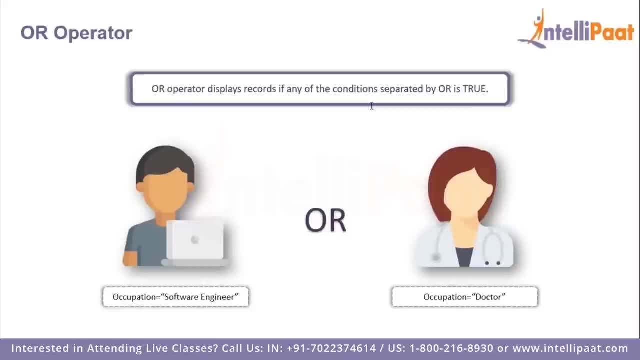 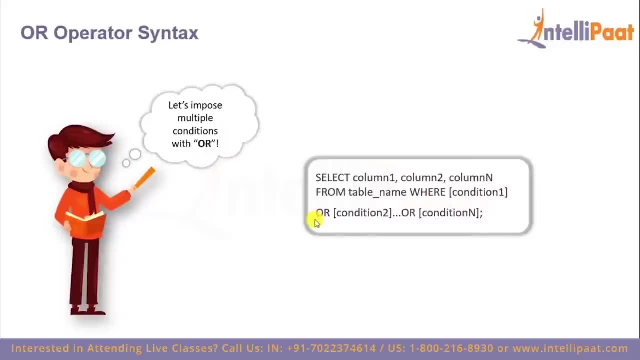 engineer or a doctor, then we can use the OR operator- And this is the syntax for the OR operator, So similar to AND operator. after we give the first condition, we follow it up with the OR operator and then give the second condition. Now we'll fetch some records from the employee table using the OR. 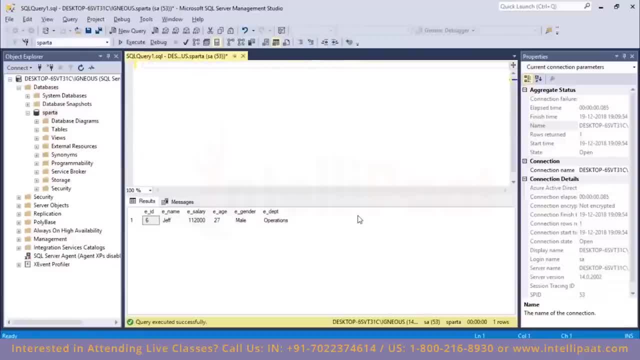 operator. So I want to extract all of those records where the employee works, either in operations or in analytics. So the command would be select star from the top right corner, and then it would be different to this one. Now we have an operation number which is equal to the first condition, and we'll add the 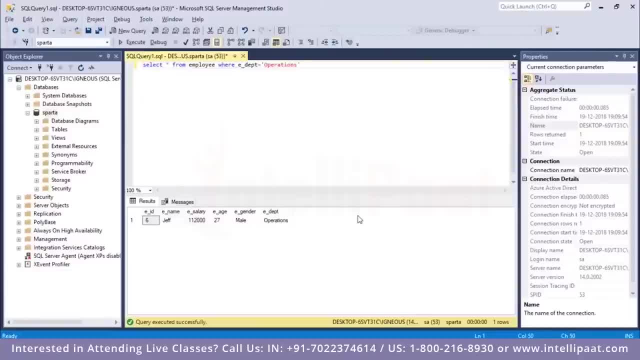 list in the function. Now let's add another requirement, which would be equal to the OR operator. So from there we get the first condition. So the first condition is department should be equal to operations. I'll use the OR operator now and then the second condition. So the second condition is the department needs. 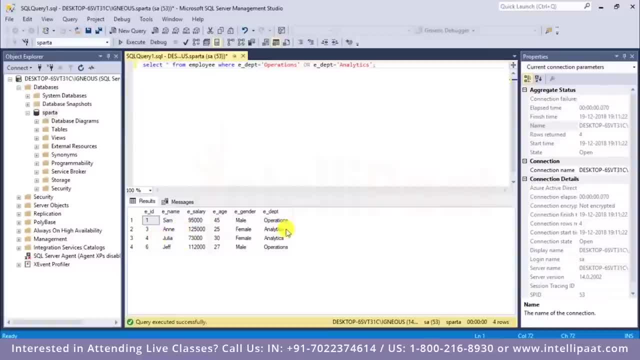 to be equal to analytics, works in analytics, Julia works in analytics and Jeff works in operations. so there are four results, all of which two people work in operations and two people work in analytics. now, similarly, I'd want to extract those records were either the salary is greater than $100,000 or the age is greater than 30. so 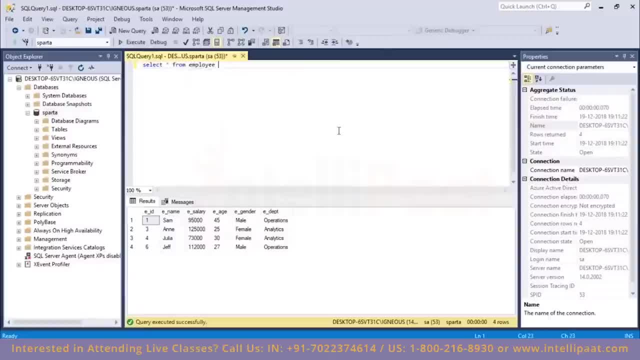 this would be the command: select star from employee. where salary is greater than hundred thousand dollars, I'll have to use the or operator and then give the second condition. so the second condition is: age needs to be greater than 30 execute. so again, we have four records over. 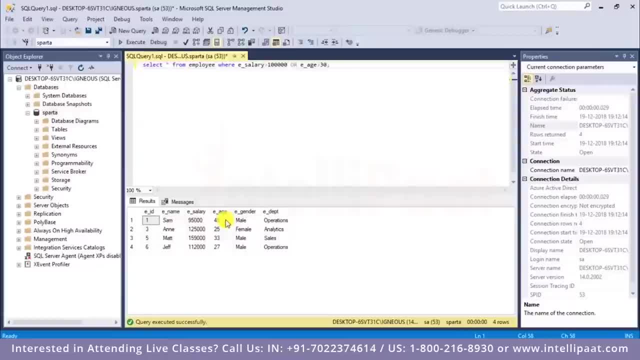 here. so the first record, sm, whose age is greater than 45. then we have an whose salary is greater than hundred thousand dollars. then we have met which satisfy both the conditions, actually you. His salary is greater than $100,000 and his age is also greater than 30.. 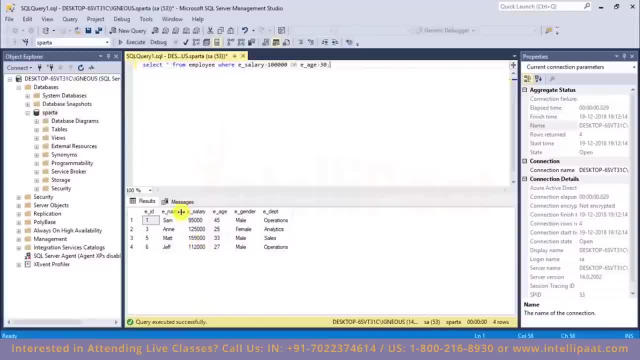 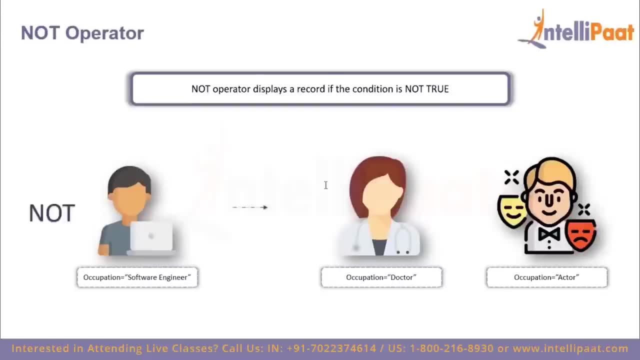 Then we have Jeff, whose salary is greater than $100,000.. So these four records. we see that at least one of these conditions is being satisfied. And finally we have the not operator. So with the not operator we can extract those records where the condition is not true. 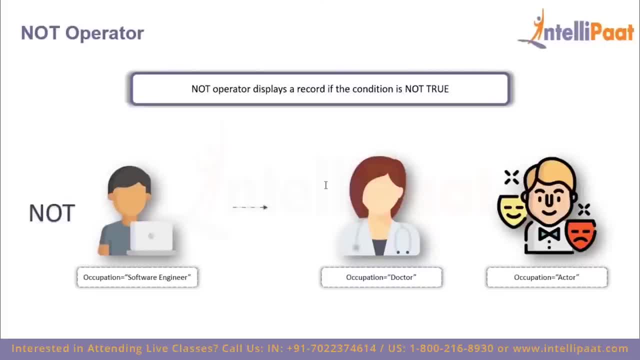 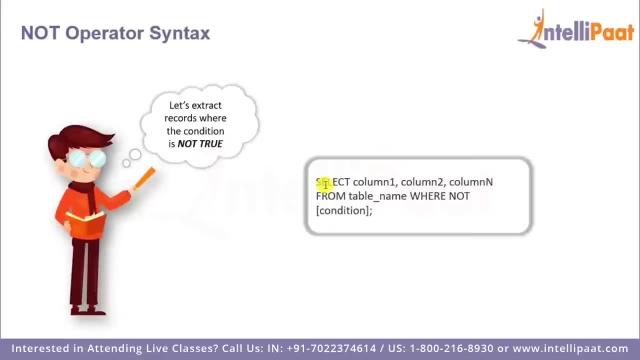 For example, if I wanted to extract all those records where the occupation of the person is not equal to software engineer, then I'll use the not operator. So let's have a look at the syntax of not operator. So here we follow up the var clause with the not operator and then give the condition. 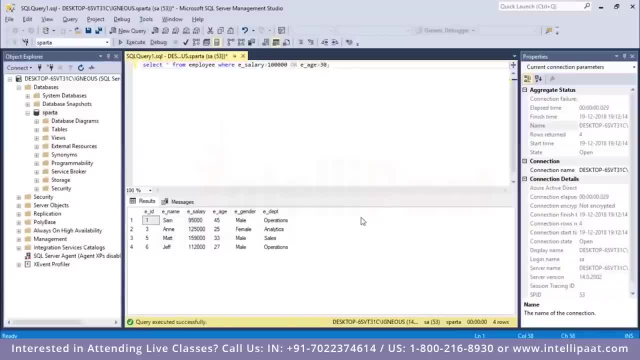 Now let's work with this not operator. So I want to extract all of those records where the gender is not equal to female. So the command would be: select star from employee var. After var clause I need to use the not operator and then give the condition. 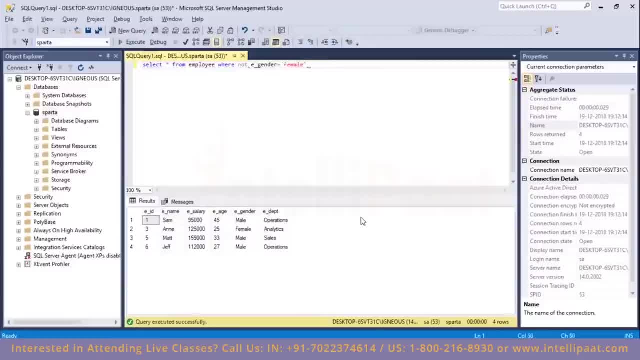 So gender is equal to female right. So before the condition I use the not operator. So this would basically give me all of the records where gender is not equal to female. So I'll hit execute. So you see that I get four records in total, and all of those four records the gender value is male. 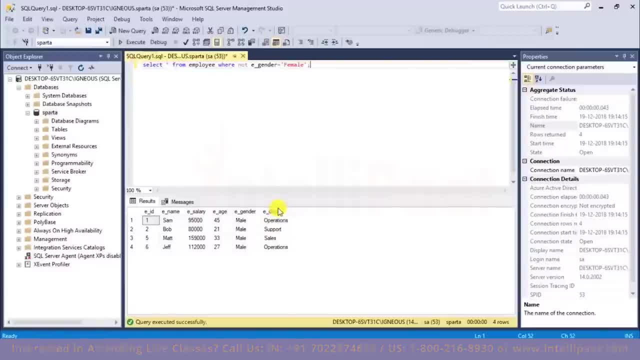 Now, similarly, I'll extract all of those records. Well, here the age is not less than 30, right, So select star from employee var. I need to follow it up with the not operator and then give the condition, which would be E of age is less than 30.. 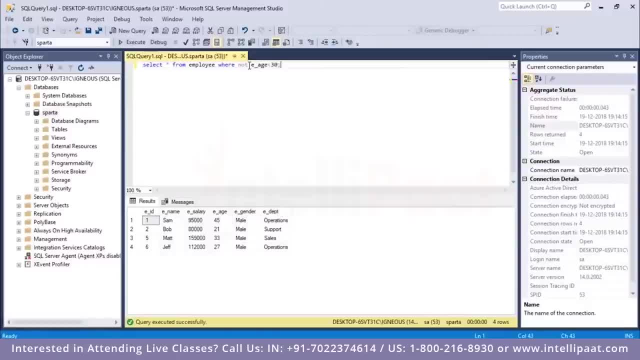 So this is the actual condition E of age is less than 30. And since I preceded with the not operator, I will get all of the records where age is actually not less than 30. I'll hit execute. So these are the three employees whose age is not less than 30.. 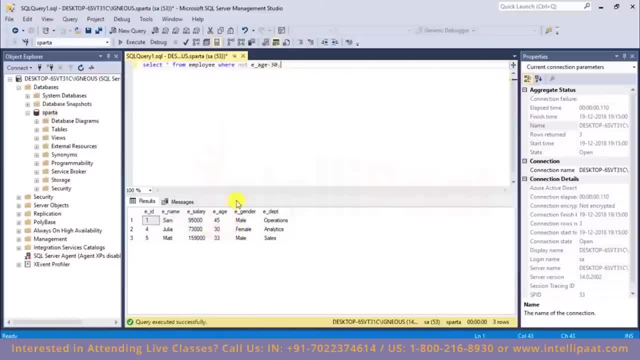 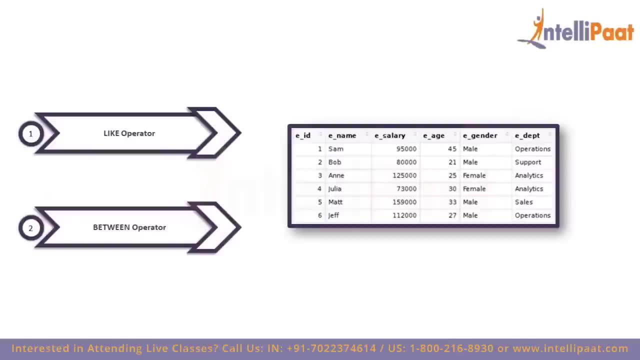 We have Sam, whose age is 45. We have Julia, whose age is exactly 30. And then we have Matt, whose age is 33.. So, guys, this is how we can work with and or and not operators, How to extract records with a like and between operators. 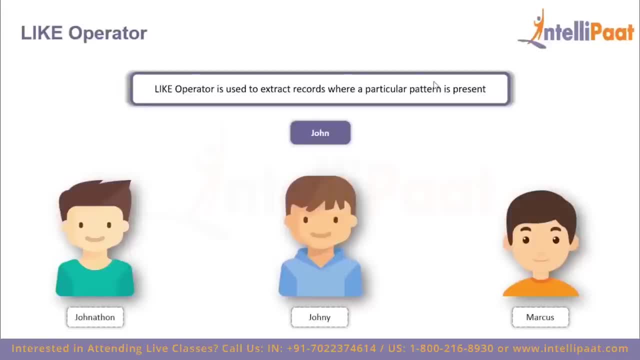 We'll start with the like operator, For the like operator is used to extract those records from a table where a particular pattern is present. For example, we'd want to extract all those records where the person's name includes John. So if we have records of three people in our table with the names Jonathan, Johnny and Marcus, 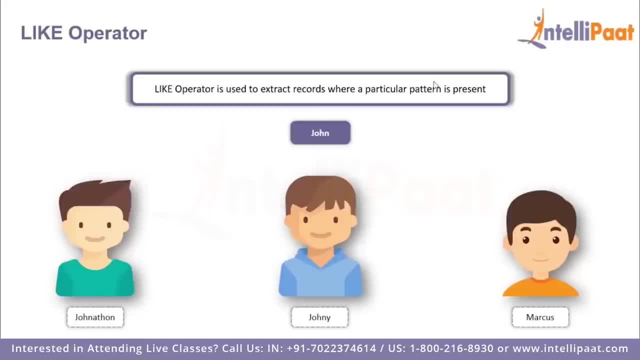 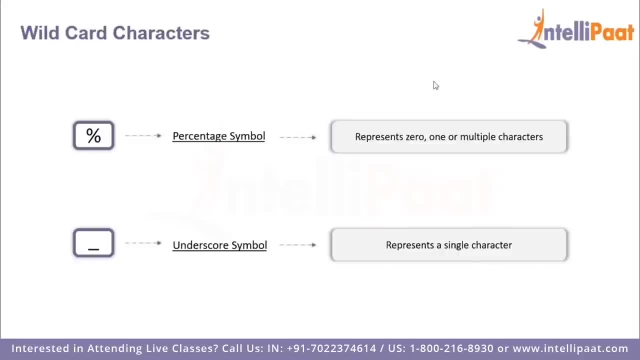 then, with the help of like operator, we can extract records where the names are Jonathan and Johnny, since they have the required pattern present in them. Now, the like operator is used in conjunction with the wildcard characters, And there are two wildcard characters. First one is the percentage symbol. 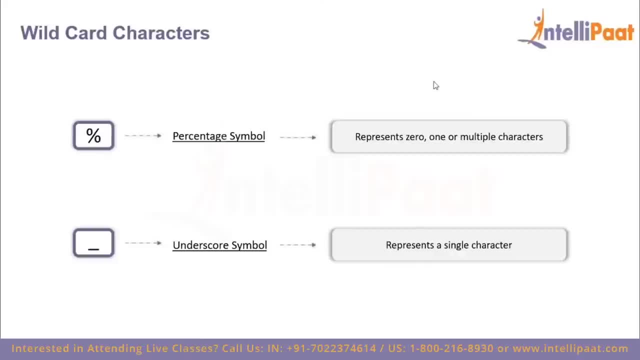 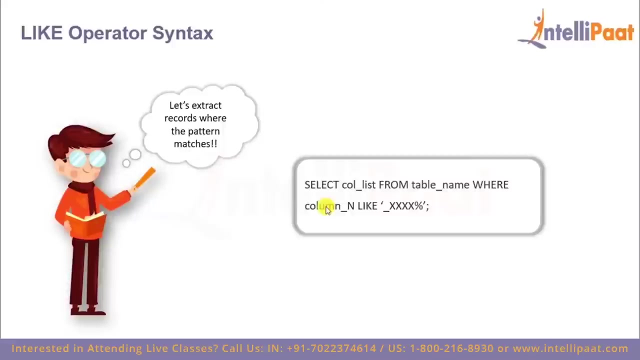 And the second one is the underscore character. So the percentage symbol is substitution for zero, one or more characters, While the percentage symbol is substitution for a single character. And this is the syntax for the like operator. After giving the where clause, be given the column name, followed by the like operator and then the pattern which you want to extract. 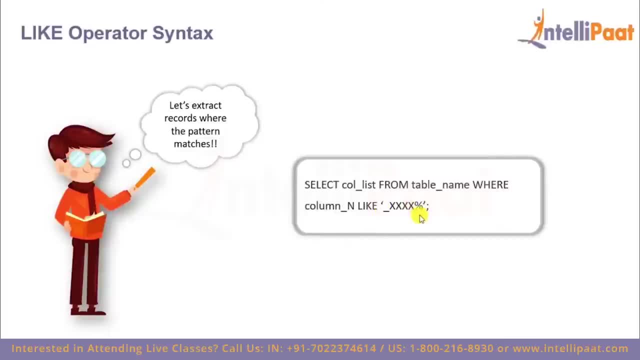 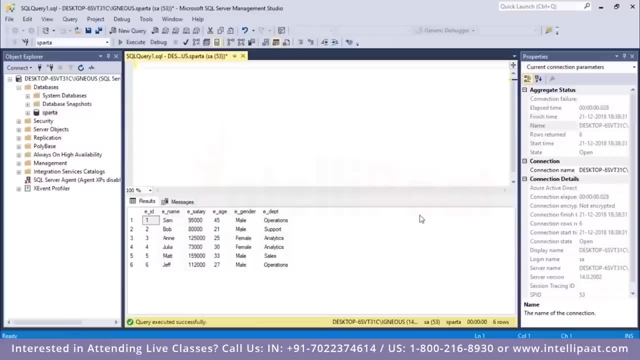 And keep this in mind, guys. the pattern should be inside single quotes. Now let's do some operations with the like operator. First, I'd want to extract all of those records where the employee's name starts with the letter J. So the command would be select star from employee, where I will give him the condition, which would be ename. 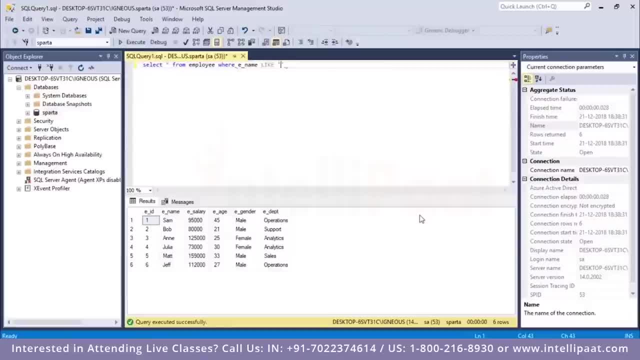 following which I will give him the like operator and inside single quotes, since the name should start with J, I will type J, after which I will use the percentage wildcard, So all of those names which start with J would be extracted. So let me hit execute. 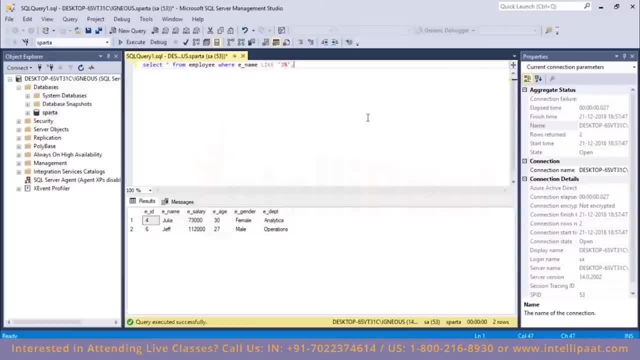 So Julia and Jeff are the two employees whose name starts with J. Now, similarly, I'd want to extract all of those employees whose age is in the 30s. Right Select star from employee where I need to give the condition. so eh, following which I'll give the like operator. 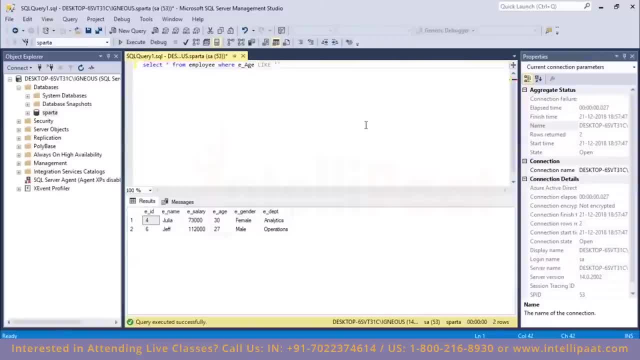 and then inside single quotes, age needs to be in 30s. So after 3, I will use the underscore wildcard character and then put in the semicolon. let me hit execute. So we have Julia and Matt over here. So Julia's age is 30, and Matt's age is 33.. 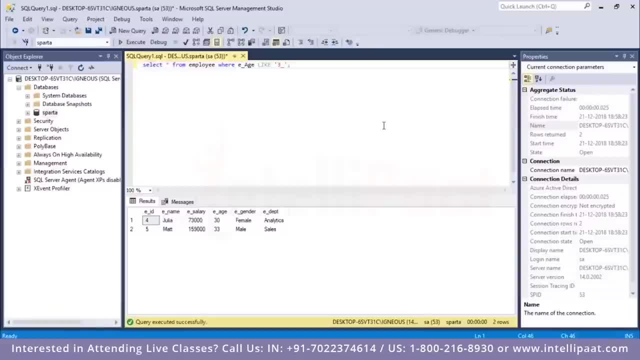 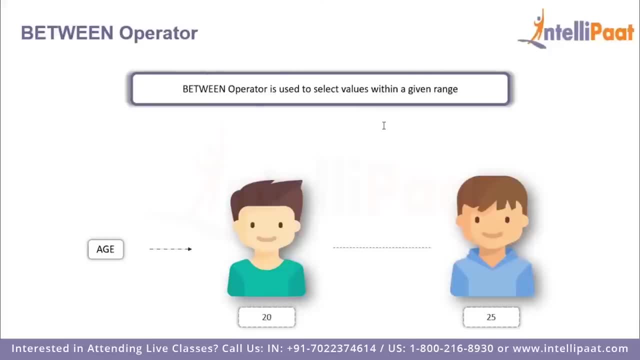 So they are the two employees whose age is in the 30s. Now let's look at the between operator. So the between operator is used to select values between a given range. For example, we can extract only those records where the age of the person is between 20 and 30.. 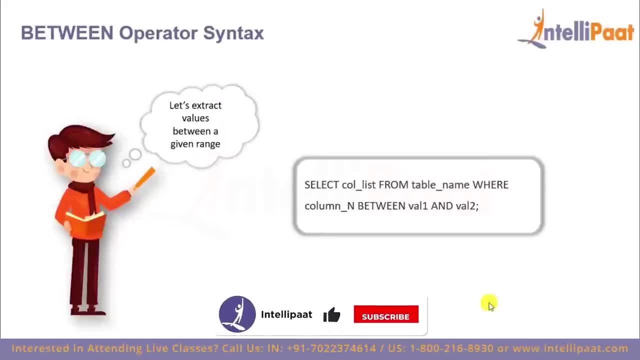 So we can extract only those records where the age of the person is between 20 and 30. So we can extract only those records where the age of the person is between 20 and 30. And 25.. And this is the syntax. 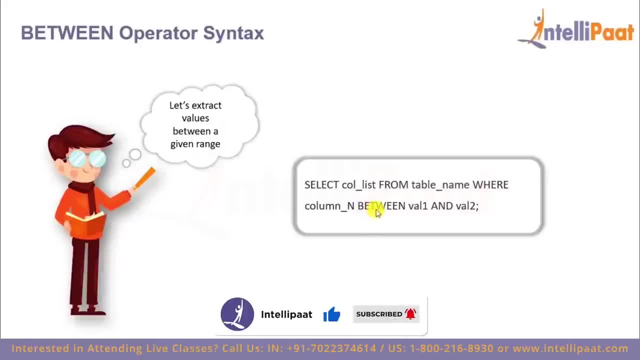 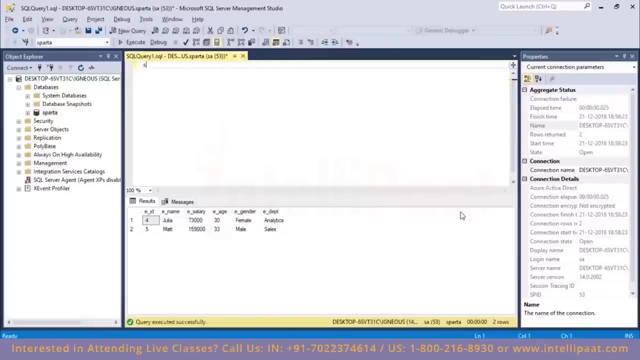 After where clause, we give in the name of the column, then we give the between keyword, after which we give in the lower value of the range, then use the and operator and then give the maximum value of the range. So I don't extract all of those employees whose age is between 25 and 35.. 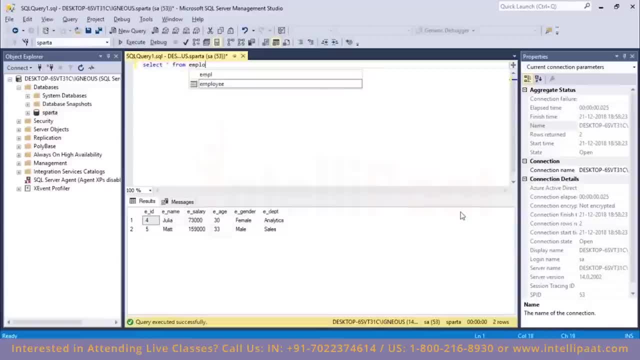 So the command would be: select star from employee, where the condition would be: eh should be between 25 and 35.. Execute. So Ann, Julia, Matt and Jeff are the four employees whose age is between 25 and 35. So, as you see over here, this value is inclusive, right, 25. 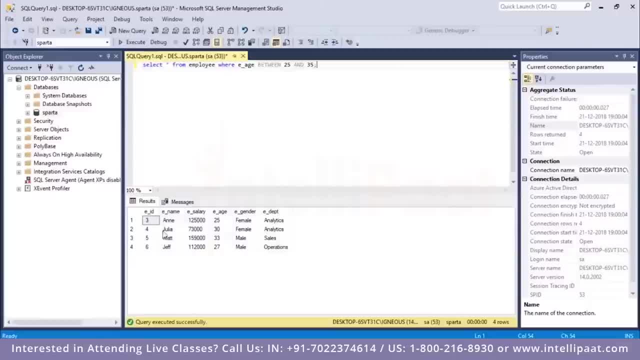 is inclusive. So Ann's age is 25, Julia's age is 30, Matt's age is 33, and Jeff's age is 27.. And these are the four employees whose age is between 25 and 35.. Now, similarly, I'd want. 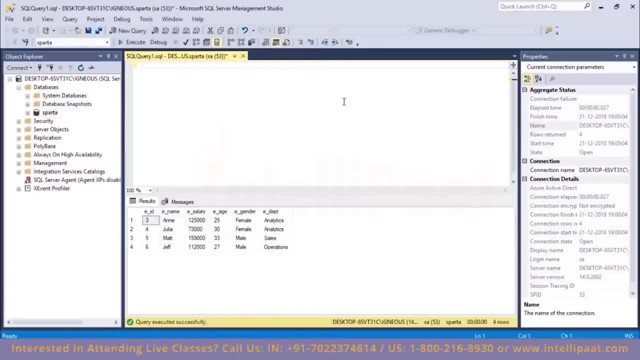 to extract all of those employees whose salary is between $90,000 and $120,000.. So the command would be select. start from. I need to give in the name of the table which is employee, Then I'll use the where clause and then give the condition. So the condition would be: 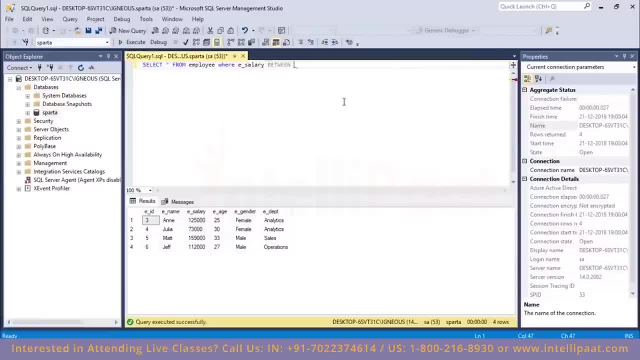 the salary between. So the salary needs to be between $90,000 and $120,000.. I'll put a semicolon. Let me hit, execute. So Sam and Jeff are the two employees whose salary is between $90,000 and $120,000.. So Sam's salary is $95,000 and Jeff's salary is $112,000. 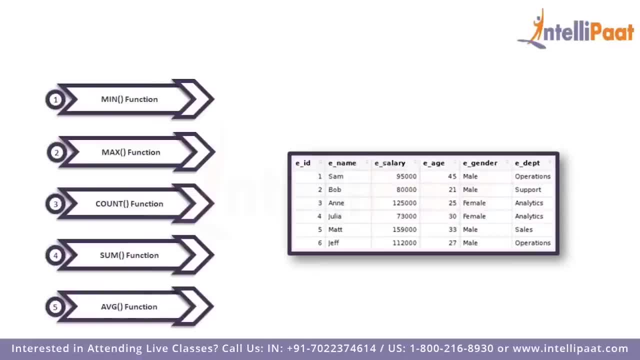 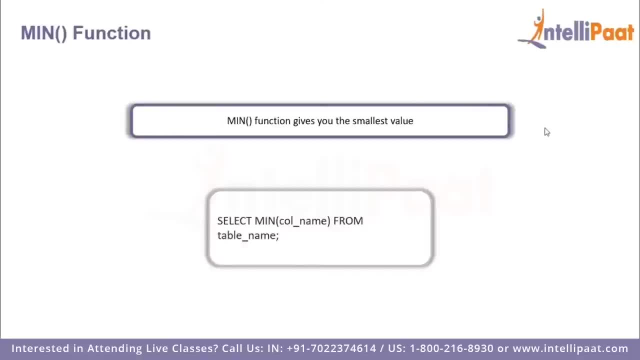 Some basic functions in SQL, So we'll look at the min function, max function, count function, sum function and average function. Let's start with the min function. The min function gives the smallest value in a column. Let's look at the syntax. 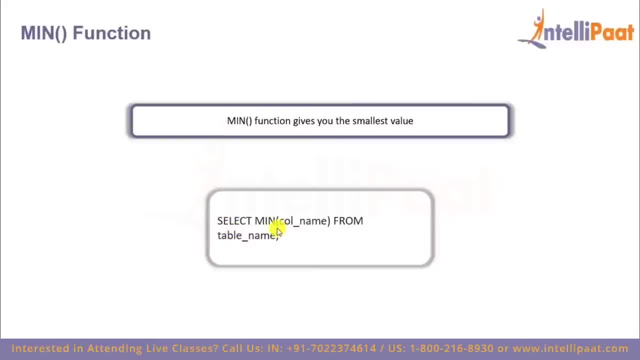 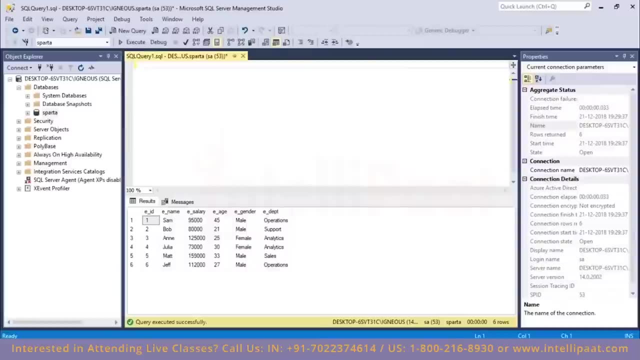 First we give in the select keyword, Then we give the min function And inside the parenthesis we specify the name of that column from which we're supposed to find the minimum value. So I'd want to extract the age of the youngest employee of the company. So this would be the 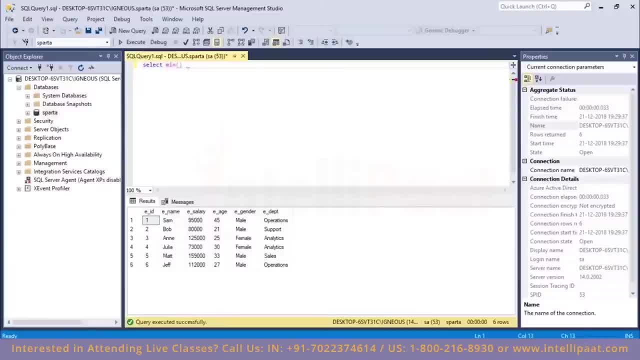 command start select, And then I'll use the min function and then pass in the column, which would be eh. I'll use the from keyword and then give in the name of the table, which would be employee. So the total command is select min. 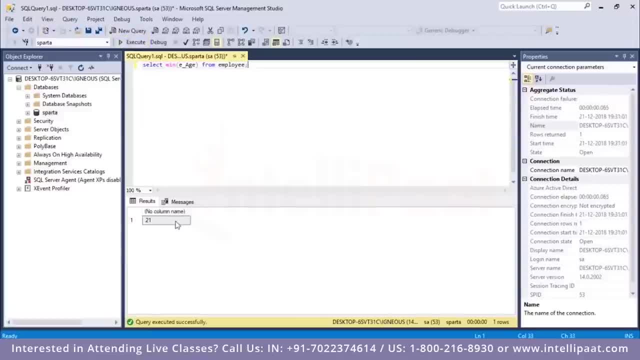 I'll hit execute. So we see that the minimum age in the table is 21.. Similarly, if I wanted to extract the salary of that employee who would get the least salary, So the command would be select min And instead of eh it would be esalary from employee, So the salary of the employee who 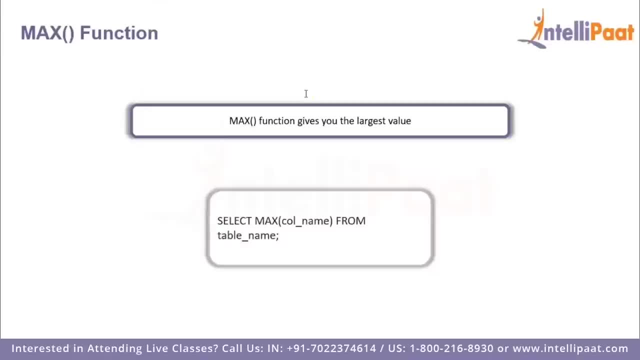 earns the least is $73,000.. Then we have the max function. The max function gives the largest value and we give in the select keyword, following which we give the max function, And inside the function we specify the name of the column from which we're supposed to get the maximum value. 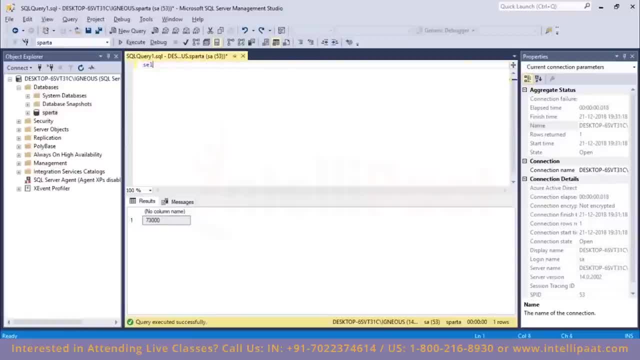 Now I'd want to extract the maximum age and maximum salary from this table. So this would be the command for that Select, And I will start off by extracting the maximum age Inside the max function. I will pass in the column which is eh, And then I'll use the from keyword and then give. 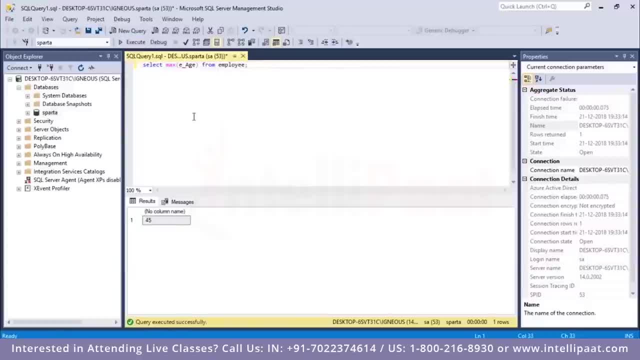 the maximum age. So the maximum age of an employee is 45.. Similarly, I want to find out the maximum salary- So that would be esalary- from employee Execute. So the maximum salary is $159,000.. Then there's a count function. So the count function returns the number of rows that 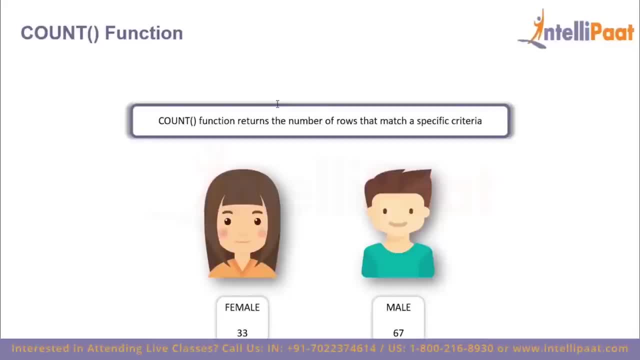 matches specified criteria. That is, if we wanted to find out the number of male and female employees in a company, Then we have the count function. So the count function returns the number of rows that match the. we can use the count function. Let's look at the syntax. So after the select keyword: 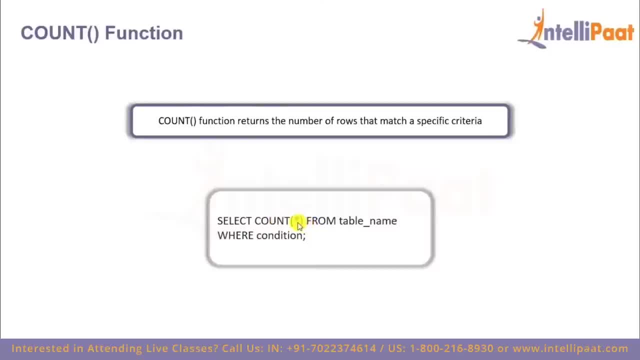 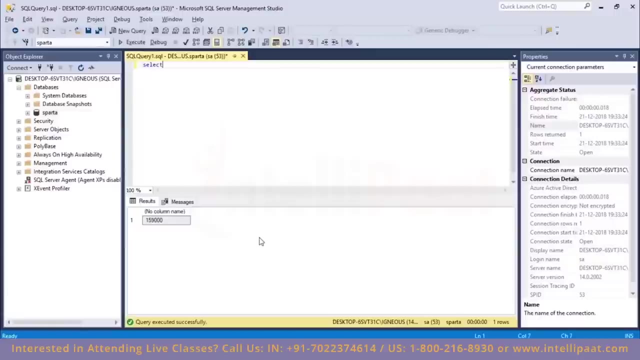 you will use the count function and give in an asterisk inside the parenthesis, Then you will give the table name and finally you will use the where clause to give the condition. So let's use this count function to get the count of number of male and female employees. So I'll start off by getting the count of. 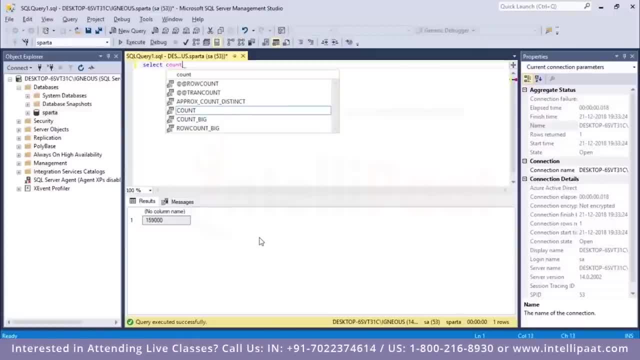 number of male employees, So select, I will use the count function and inside the count function I will pass in the asterisk symbol, After which I'll use the from keyword and then give in the name of the table, which would be employee. Then, using the where clause, I will give in the condition. So I do want the count. 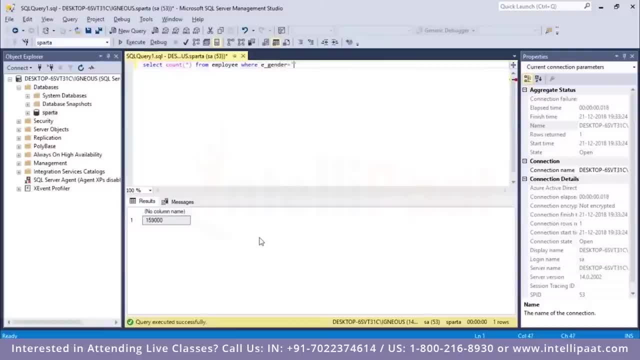 of all of the male employees. So E of gender should be equal to male. Let me see what do we get. So there are four male employees in total. Similarly, if I wanted to get the count of all the female employees, the command would be: 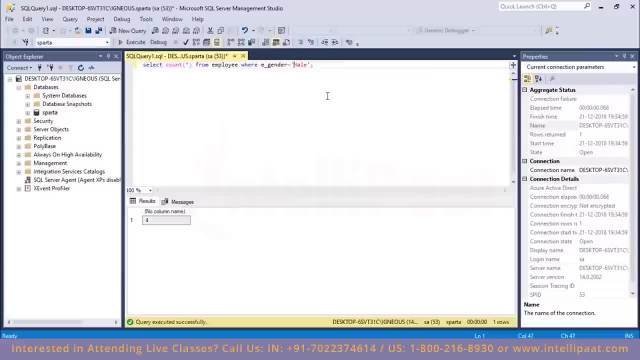 select the count of all the female employees. So if I wanted to get the count of all the female employees, the command would be: select count of star from employee where E gender equals female Right. so this would be the only difference. I'll hit execute. So I get two. So there are two. 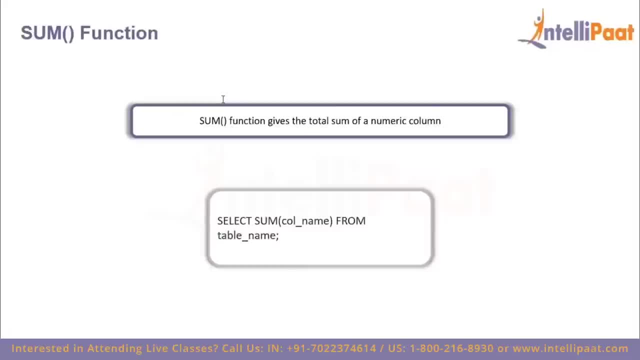 female employees in the entire organization. Then we have the sum function. So the sum function would give you the total sum of a numeric column, and this is the syntax. So here, similarly, we will give in the sum function after the select keyword and give the column name inside the parenthesis. So I want to 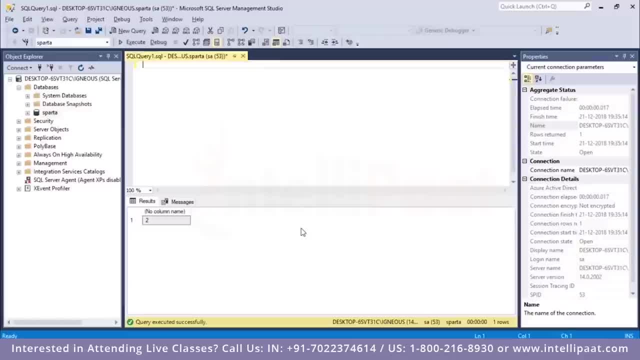 give the total sum of salaries of all of the employees, Right. so the sum of salaries of all of the employees Select, and then I'll use the sum function and then I'll pass in the column which would be E salary from the name of the table. 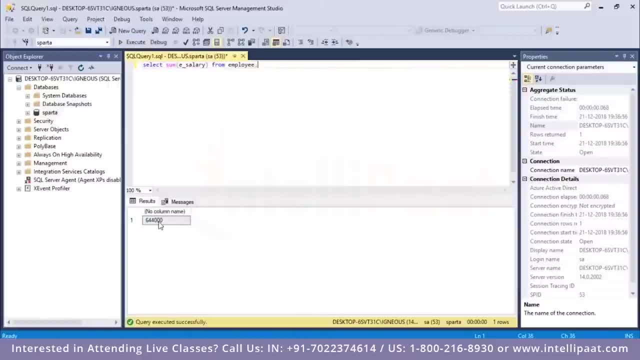 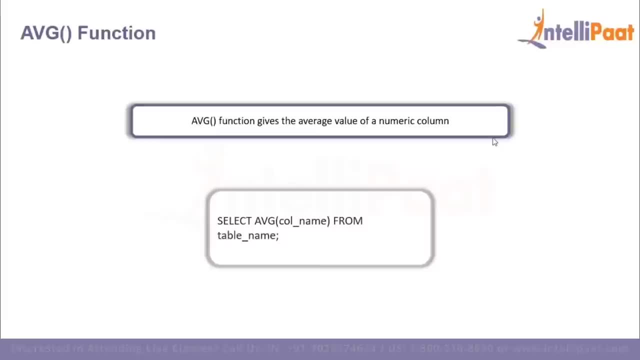 which is employee. So the total salary of all of the employees included is six hundred and forty four thousand dollars per annum. And finally, we have the average function. So the average function gives us the average value of a numeric column and the syntax is same as the rest. So we'll 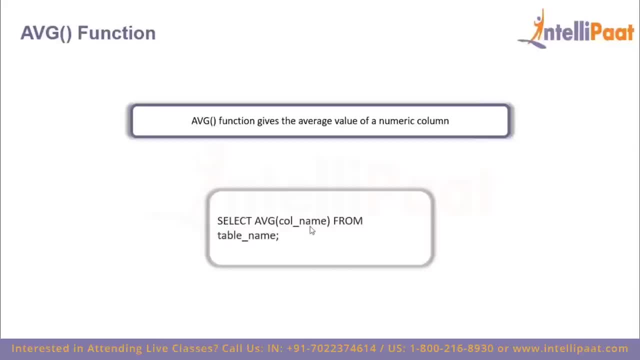 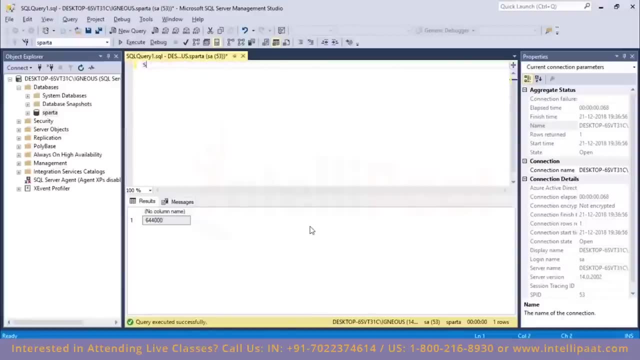 give in the average function after the select keyword and give the column name inside the parenthesis. So this time I want to get the average age of all of the employees, So select, and then I will use the AVG function and then give in the column, which would be E age, from the name of the table, which is employee, So the 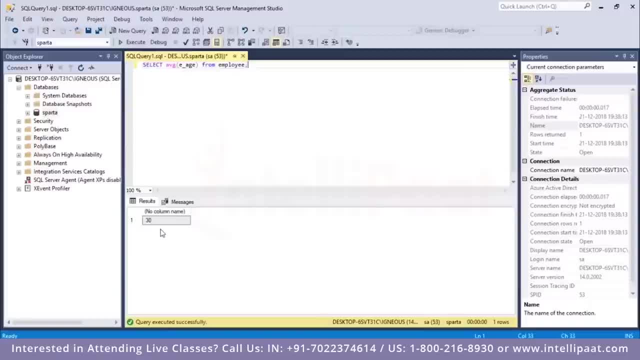 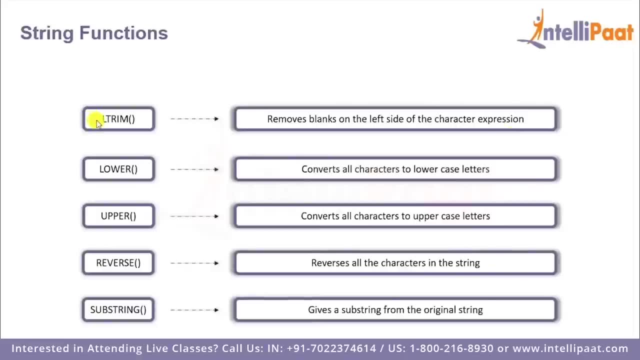 average age of all of the employees is 30.. So, guys, these were some of the aggregate functions in SQL, Some string functions. So first we have the L trim function, which helps in removing the blank spaces on the left side of the character expression. So let's implement this function in SQL server. So let me. 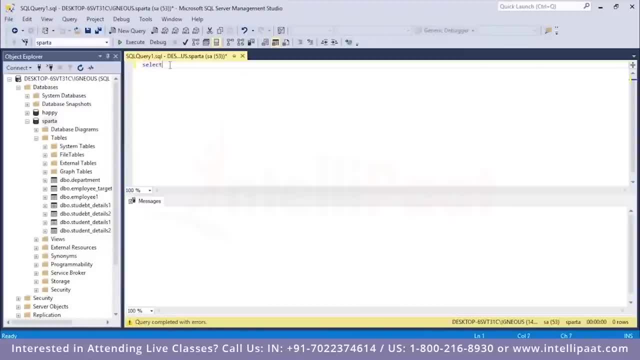 first create a string with some blank spaces on the left side. So I'll type select and then I will give some blank spaces on the left side. Now let me pass in the string and I'll name the string to be Sparta. I'll hit execute- Right. so 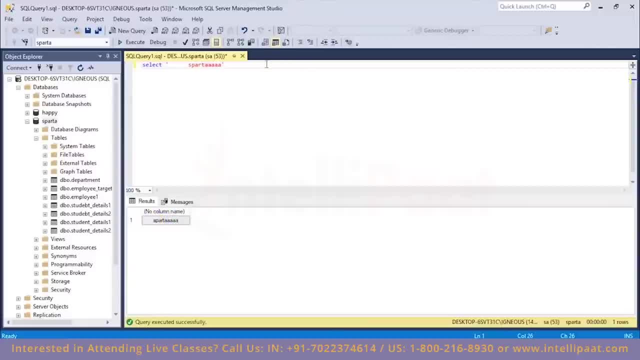 this is the string which has some leading spaces on the left side. Now if I want to remove all of these blank spaces on the left side, all I need to do is use the L trim function. So I will type select L trim and inside this I will. 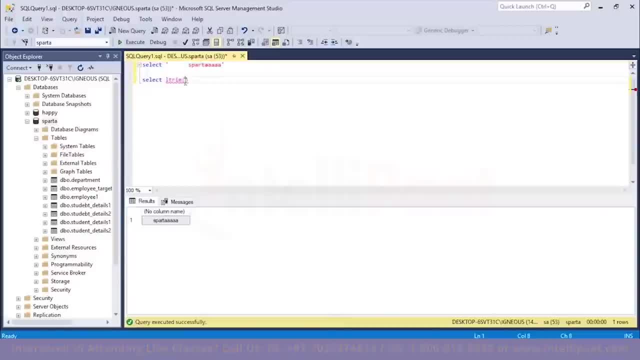 pass in the string with the leading spaces. So I'll copy this and I will paste it over here Now. let me copy this and paste it over here Now. let me copy this and I will paste it over here Now. let me execute both of this simultaneously. Right? so this is the string with the. 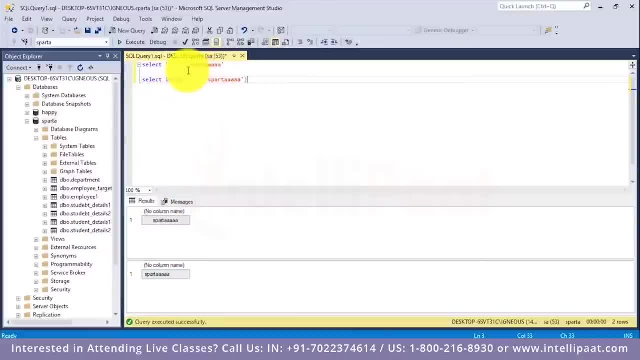 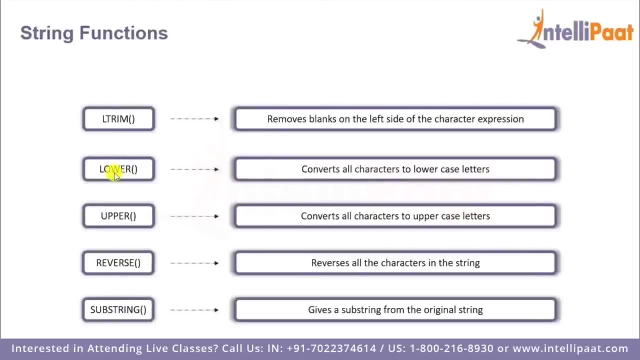 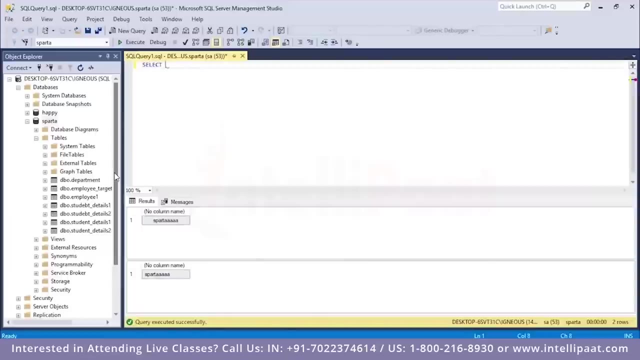 leading spaces, and when we use the L trim function, all of those blank spaces on the left side were removed. Then we have the lower function, which basically converts all the characters to the lower case. So let's look at an example. This time let me actually print a string which has all the characters and 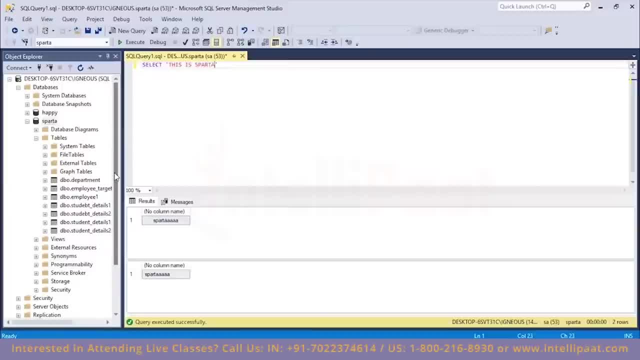 capitals. So this is Sparta. So here we see the lower function, which has all the characters and the string have capitals. I'll execute this and this is what we get. Now, if I want to convert all of the characters into lower case, I can just use a lower function. So I will type. 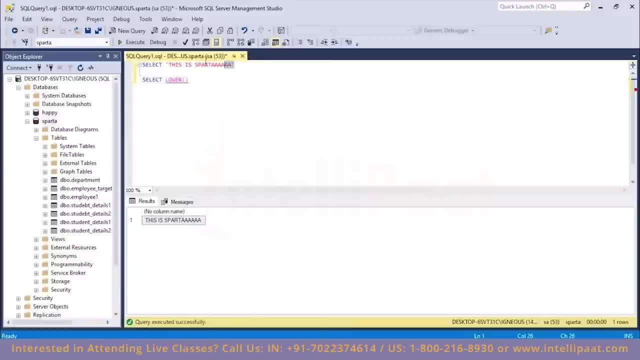 select lower and then pass in the string inside the function. I'll copy the string, I will paste it inside this, I'll hit execute. So this is the string where all the characters were in capitals and after using the lower function, this string where all the characters were in capitals have been. 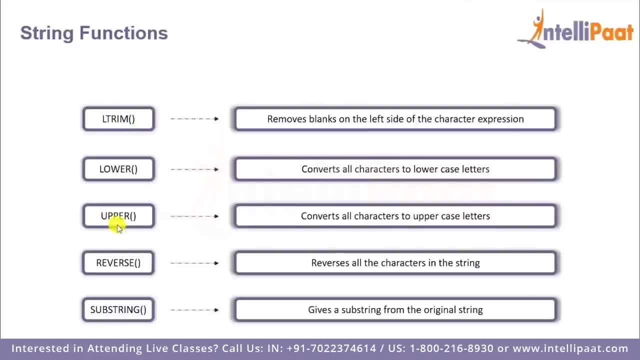 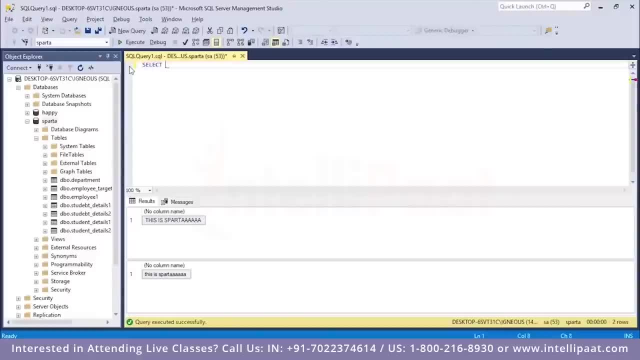 to lowercase. Similarly, we have the upper function which basically converts all the characters to uppercase. So this time I will take in a string which has all the characters in lowercase. So select, I will type hello world. let me print this right. so here we see that initially all of the characters are in lowercase. 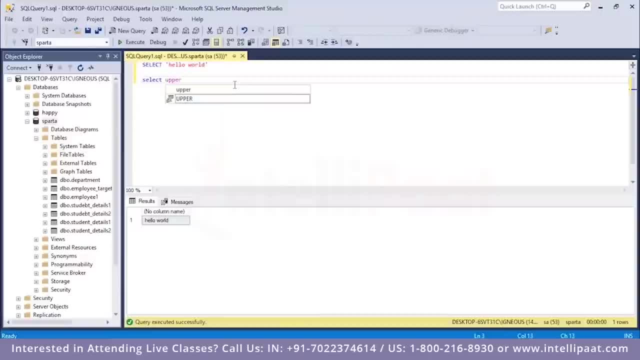 Now, after this, I will type select upper and then pass in the string inside the function. I'll copy this, I will paste it over here, I'll hit execute. So this was our initial string and after using the upper function, we have converted the string into capital case. After that we have the reverse function, which 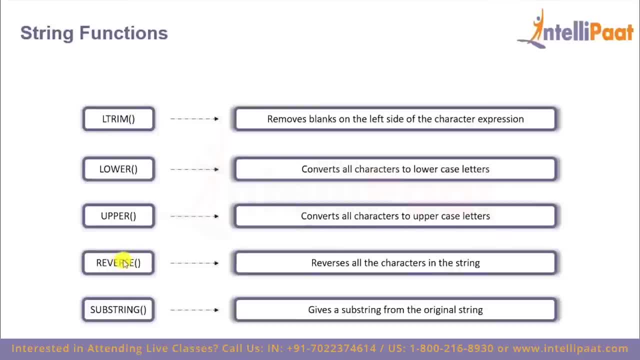 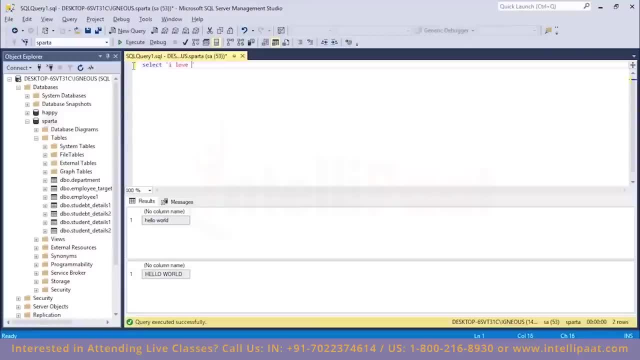 basically reverses all the characters in the string. So let's implement this too. So let me take in a random string again, select, and I will type: I love ice cream. I'll hit execute. So this is what we get initially Now. after this, I will use the reverse function: Select, reverse and I 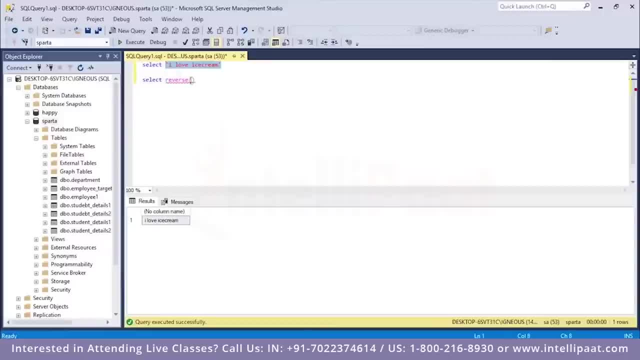 will pass in the string inside the reverse function. I'll copy it and I will paste it inside this function over here. Now let me execute. So this is the initial string and after using the reverse function, we have reversed all of the characters in the string, right? So you see that this is the starting and 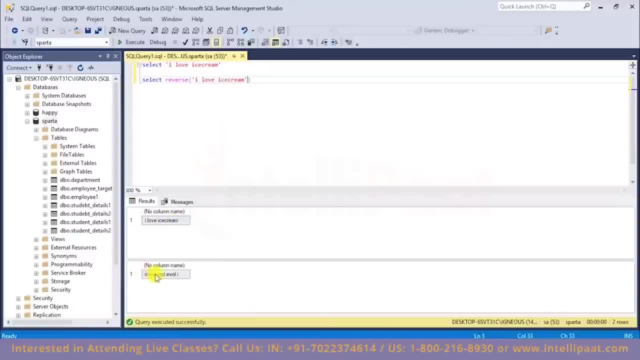 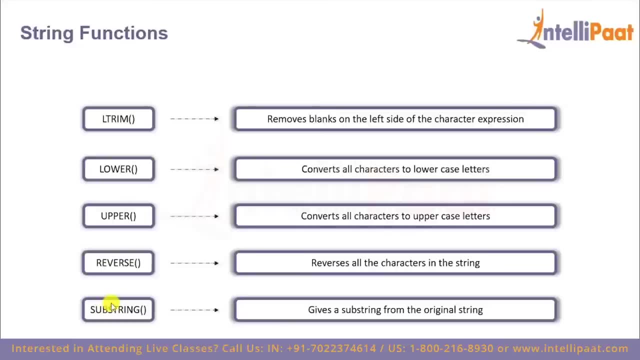 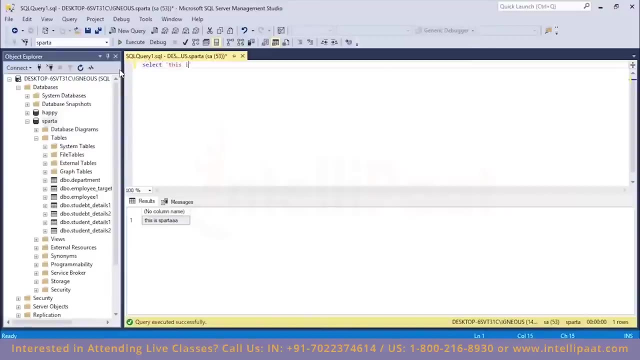 this is the ending over here, and after reversing it we get this final string And finally we have the substring function, which gives us a substring or part of the string from the original string. Now let me give in the original string first. So I will type select, and then the string would be this: sparta. 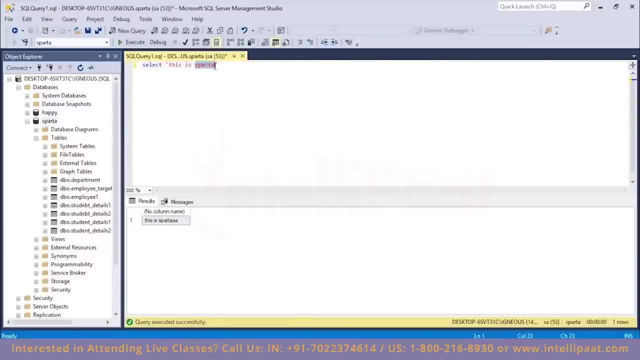 Now let's say I would want the substring sparta from this entire string. So this is where we can use the substring function. So I will type select substring. Now the substring function in three parameters. first, as the original string. so I will copy the: 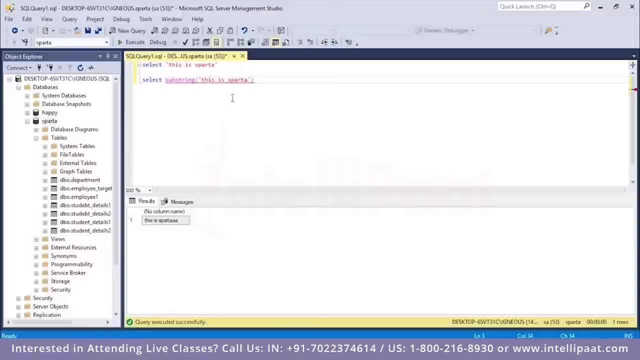 original string and I will pass it into this as the first parameter, and now after that I need to give in the index value from where the substring starts. so this is the first character of the substring which I want. so the index value would be 1, 2, 3, 4, 5, 6, 7, 8 and 9. so I'll type 9 over here and then the third. 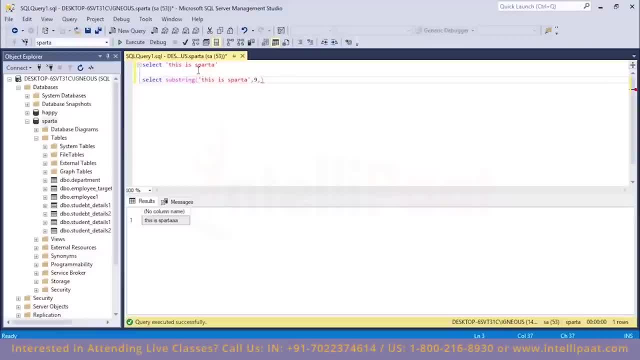 parameter would be the length of the substring. so the length of the substring is 1, 2, 3, 4, 5 and 6, so I will pass in 6 over here. now let me execute all of this and let's see what do we get. so this is the original string. this is: 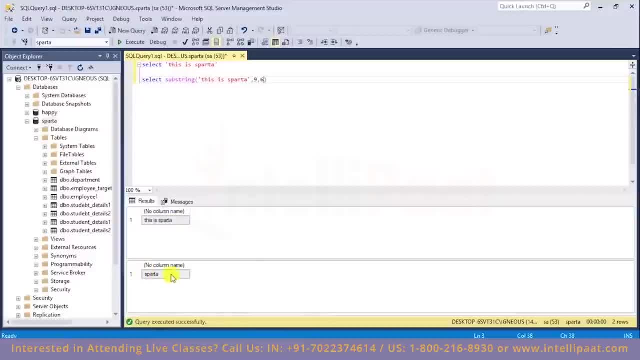 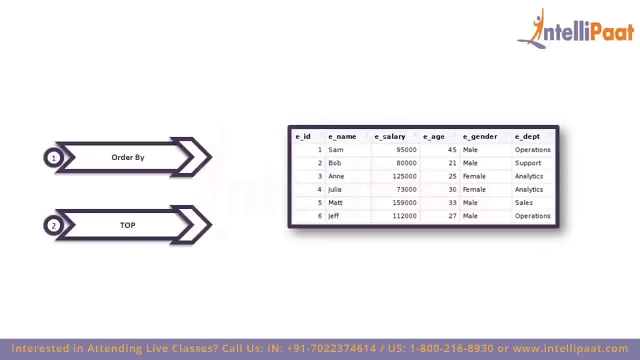 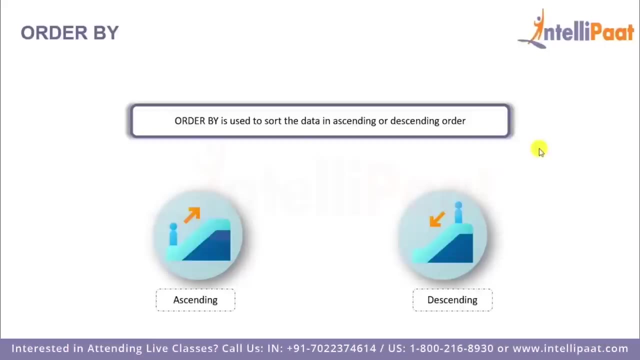 pada and after using the substring function, we have extracted only this part from the entire string. so these were some of the string functions in SQL. order by and the top clause. so order by is used to sort the data in ascending or descending order and by default, order by sorts the records in ascending order. so let's have. 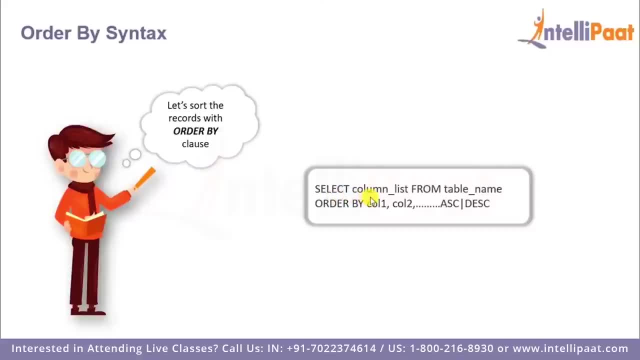 a look at the syntax. we'll start with select keyword and then, given the column list, then we'll use the from keyword and give the table name, following which will type the keywords, order by and give the columns with respect to which you are to sort the data and finally we'll state whether the ordering should be in. 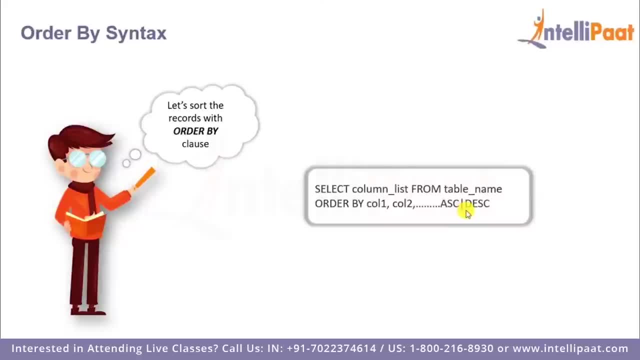 ascending or descending, and I've already told you guys that by default the sorting is done in ascending order and if you want the sorting to be done in descending order, we will use the DESC keyword. so I want to sort the table, with respect to the salary column, in ascending order. so this would be the 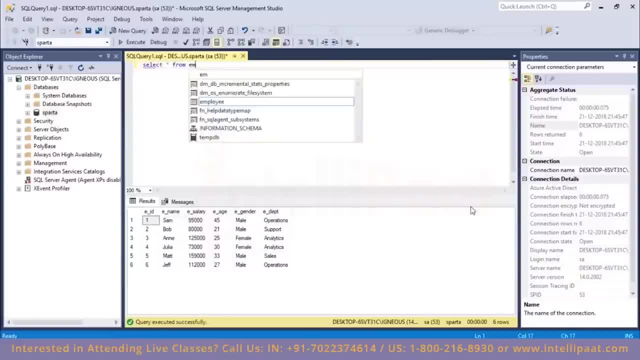 command for that select start from the name of the table is employee, after which I will use the keywords order by and then given the name of the column, which would be salary, and since I want it with respect to ascending order, so I don't need to add anything else. so let me hit execute right, so we have. 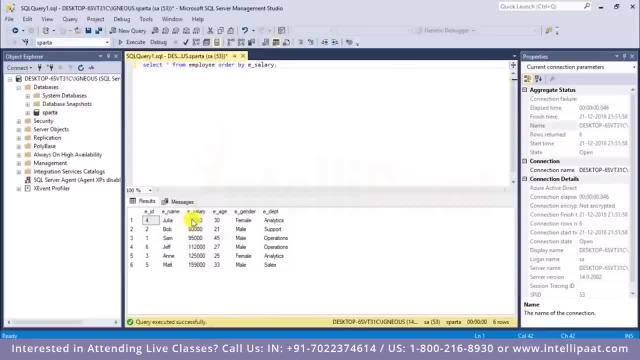 successfully sorted this table in ascending order, right. so Julia has the lowest salary and Matt over here has the highest salary. so this is an ascending order: 73,000, eighty thousand ninety five thousand and goes on till 159,000. now let's say I want to sort this table in descending order of the salary, so for 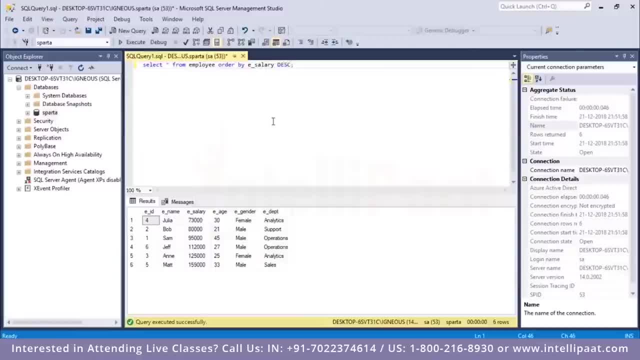 that all I need to do is add in the keyword DESC. let me hit execute. right. so this time the table is sorted in descending order. So over here, at the top we have the maximum salary, which is 159,000, and at the bottom we have the lowest salary, which is 73,000. 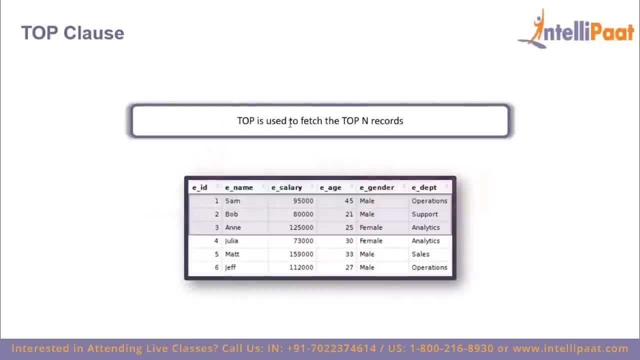 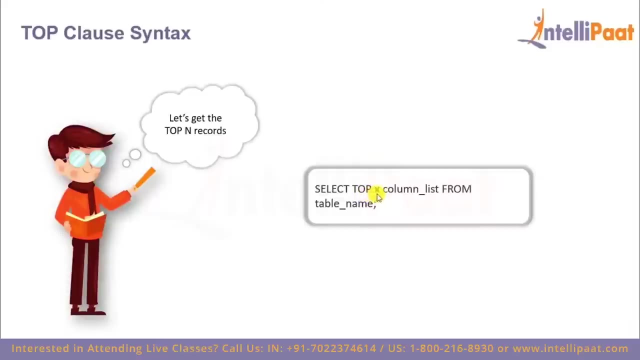 Now let's look at the top clause. The top clause is used to fetch the top end records from a table. So top clause is useful on large tables with thousands of records. and this is the syntax. We've got the select keyword first, then we type in top and then the number of records. 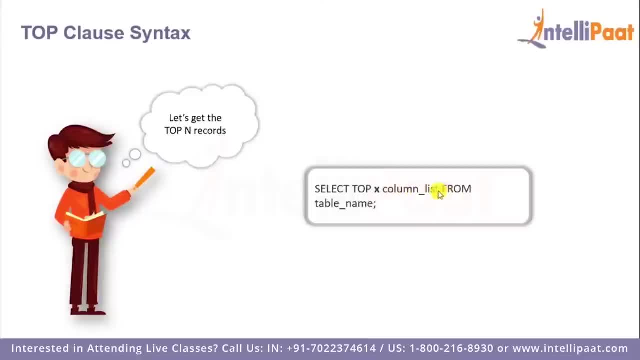 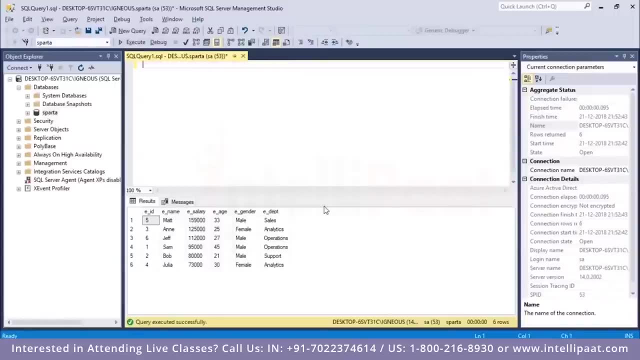 we want to see in our result, followed by the column list, And then we use the from keyword and given the name of the table. So I want to see only the top three records from the entire employee table. So this would be the command for that. 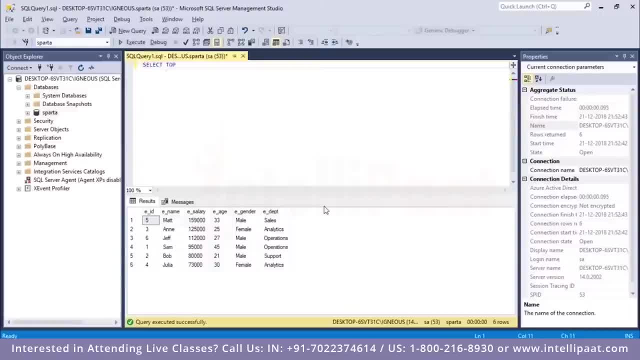 Select, and then I will use the top keyword and since I want three records, the number would be three, And since I want to see all of the columns, I will put in star over here. Then I want all of these records from the employee table. 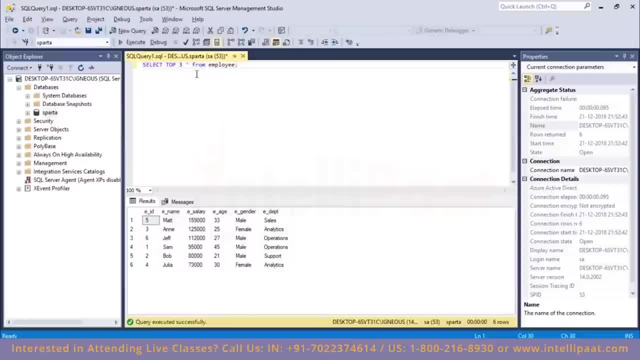 So this is the entire command: select top three stars. So I've got the top three records from the table. Now I will use the top clause and the order by clause and fetch the three oldest employees of this company. So let me write the command for that. 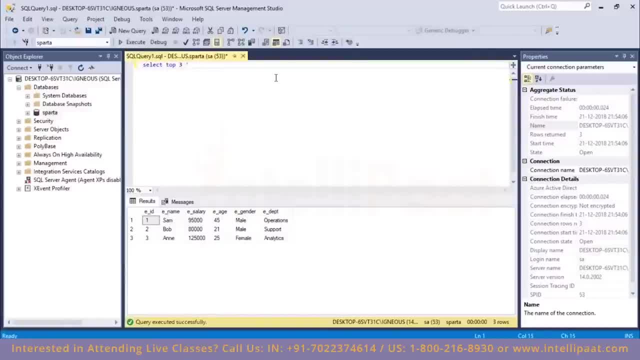 Select top three star. So I've used the top clause to fetch the top three records. Now this would be from the employee table and then I will use the order by clause. So I want to order it with respect to the age of the employee and I want it in descending order. 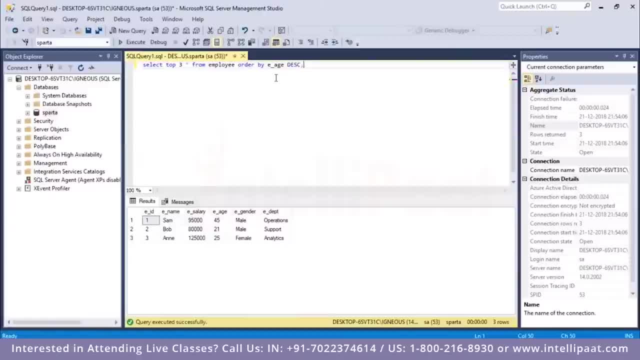 That is, the employee who has the maximum age should be at the top. Now let me hit execute. So I've got three records over here and the records are arranged in descending order of their age. So Sam has the highest age, 45, and Julia over here has the lowest age- 30, right. 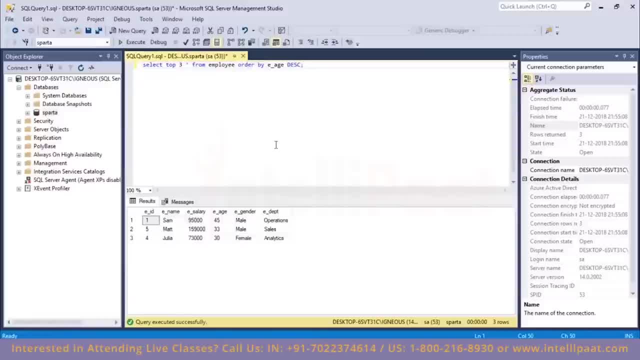 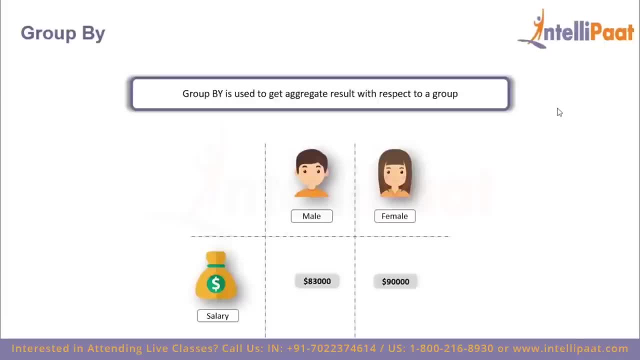 So Sam, Matt and Julia are the three senior, most employees of this company And this is how we can work with the order by clause and the top clause, The group by statement. the group by statement does used to get aggregate result with respect to a group. 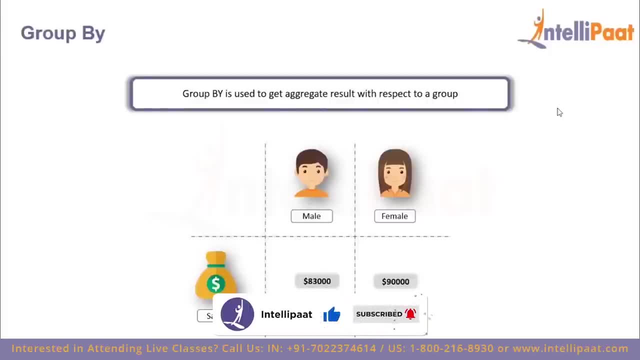 For example, let's say we wanted to find out the average salary where, with respect to gender, That is, average salary of male employees separately and average salary of female employees separately. This is where we can use group by to divide the data into two groups, male and female, and find out the average salary of each group separately. 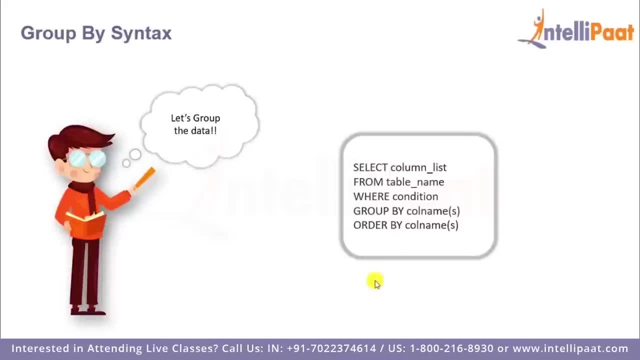 an average salary of each group separately. Now let's have a look at the syntax. So here you'd have to be careful of the sequence. So the group by clause follows the where clause and precedes the order by clause. So if you mix up the sequence then you may not get the right result. 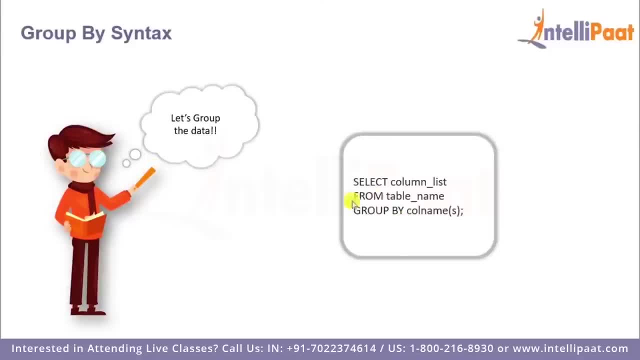 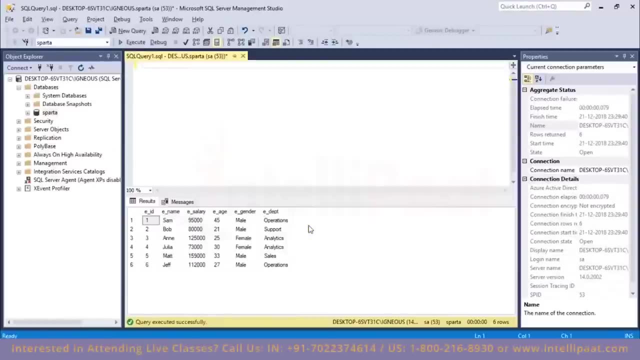 And if you're not using the where clause and the order by clause, you can directly follow up the group by statement after the table name. So I would want the average salary with respect to the gender. So this would be the syntax for that. 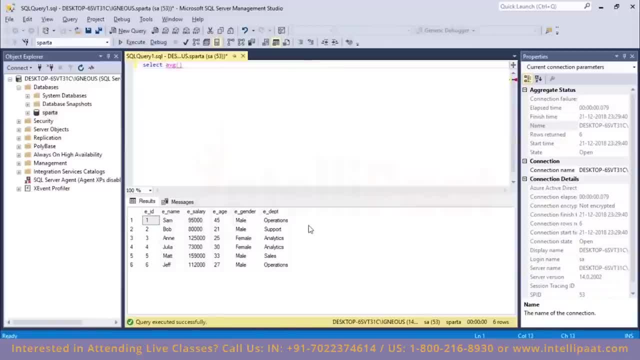 Okay, And since I want average salary, I will use the AVG aggregate function and then, given the name of the column, which would be E salary, And since I also want to see the gender column, I will give an E gender over here. 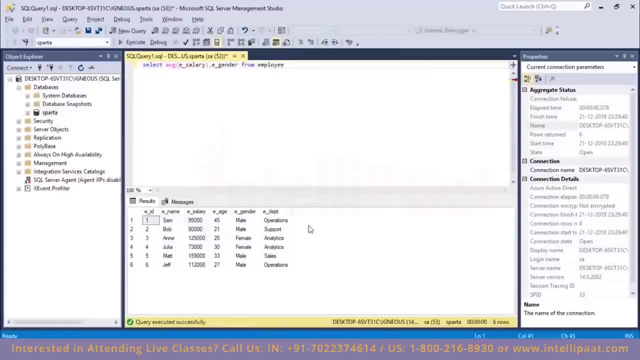 And this is from the employee table And since I have already given the name of the table, I can use the group by statement over here And after the group by statement, I need to give in the column with respect to which I have to group the data. 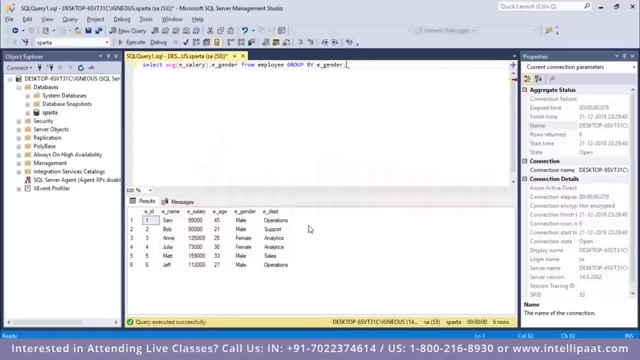 And I want to group the data with respect to the gender column. So this would be my total command: select average of E salary and E gender from employee group by E gender. So let me hit, execute Right. So this is the average salary with respect to the female employees and this is the average. 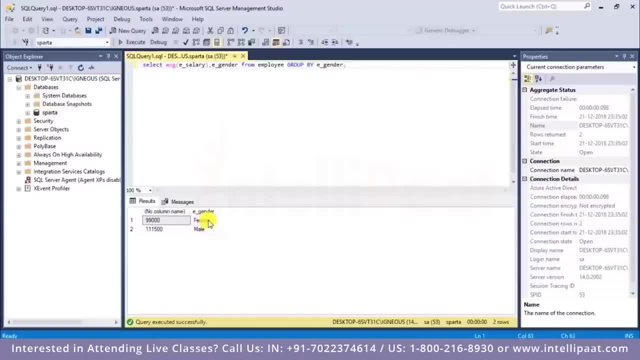 salary with respect to the male employees. So the average salary of female employees is around $99,000 per annum and average salary of male employees is around $111,000 per annum. Okay, want the average age with respect to the department and I'll also use the order. 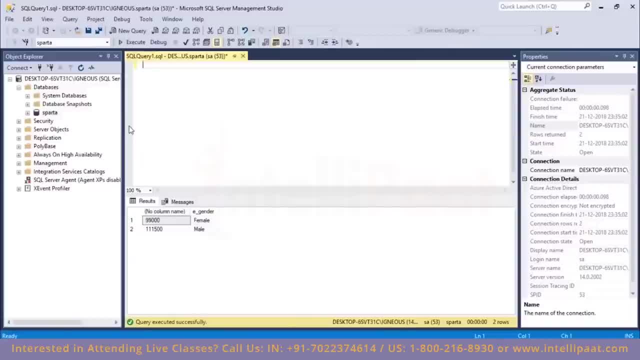 by keyword to sort the data in descending order with respect to the average age. so this is the syntax select. since I want average age, I will use the average aggregate function and then pass in the column which would be e age. and I would also want to have a glance at the departments e, d, e, p, t. I will, given the 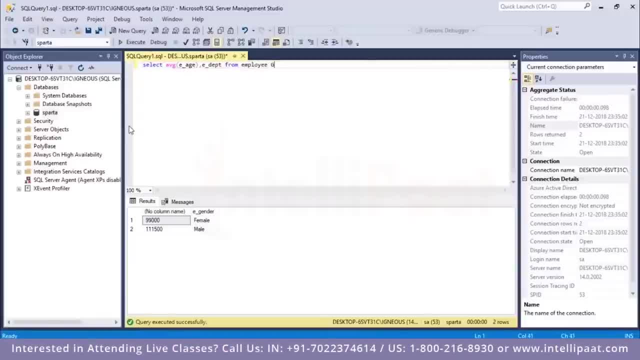 name of the table which would be employee. after which I will given the group by statement and I want to group this with respect to the department. so group by: e, d, e, p, t. and after the group by statement, I need to give the order by statement. so order by, and I want to order the result with respect to the 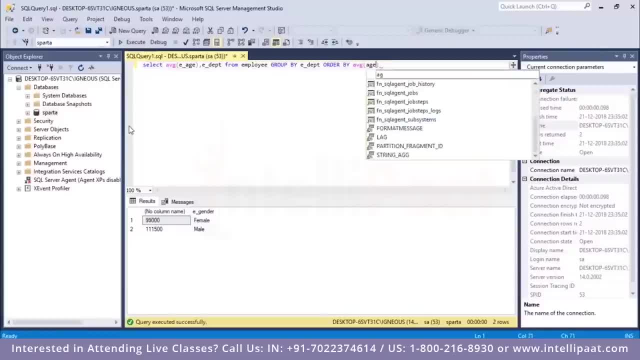 average age. so again, this would be average age and I want the sorting to be in descending order. so D, E, S, C. so this is the table: total command, select average, e age and e department. so I'll be getting the average age and the department column from the employee table and I'm grouping 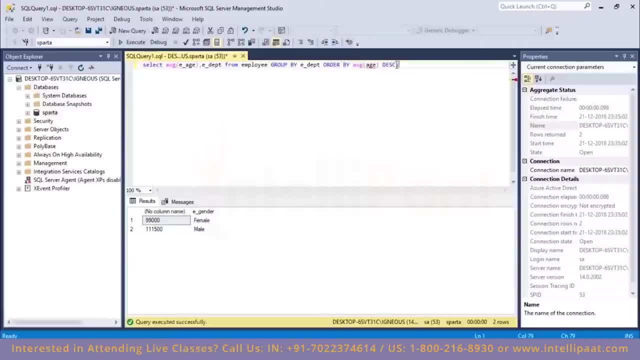 it with respect to the department column and I'm sorting it in descending order of the age. so this would be e age over here, so let me hit execute. so we have the average age with respect to each department, ordered in descending order. so operations department has the maximum average age of 36. 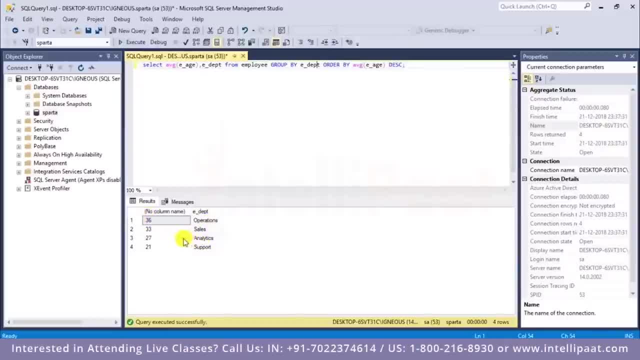 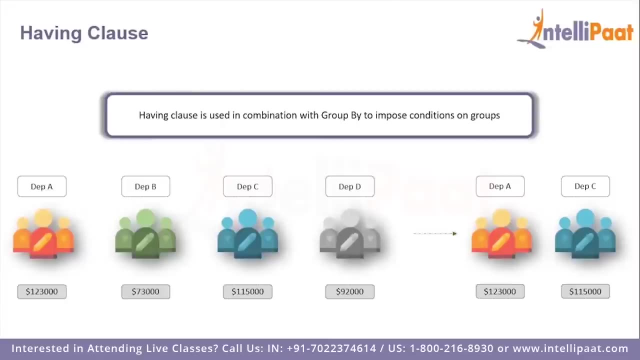 then sales has an average of 33, analytics department has an average age of 27 and support has the youngest staff of age 21. and this is how we can use a group by Clause. they having Clause is used in conjunction with the group by statement to impose certain conditions on the groups which are to be displayed. 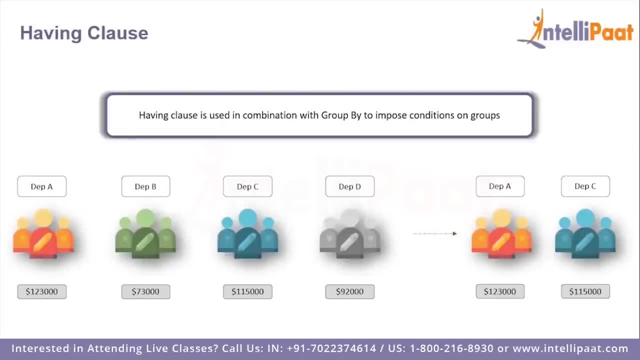 so they having Clause was added to SQL because the WHERE keyword could not be used with aggregate functions, for example, over here we have four departments- A, B, C, D and B, C and D- And we also have the corresponding average salary of the employees belonging. 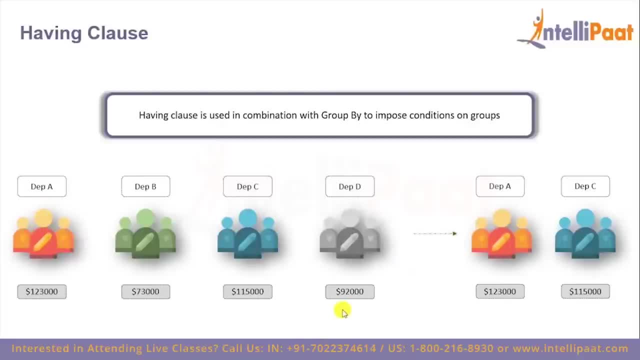 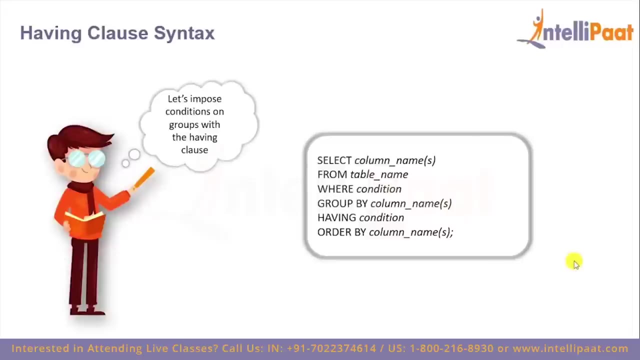 to each department. Now let's say we wanted to see only those departments where the average salary is greater than $100,000.. So this is where halving clause can be used to impose the condition and get only those departments where the average salary is greater than $100,000.. 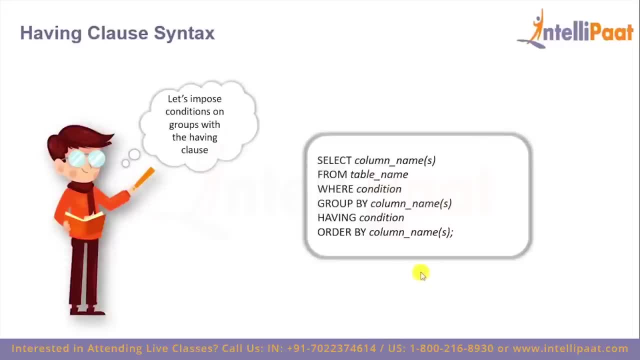 And this is the syntax for the halving clause. Here you need to keep in mind that the halving clause must follow the group by clause and must also precede the order by clause, if used. So let's go to SQL Server and implement the halving clause, So we'll group this table. 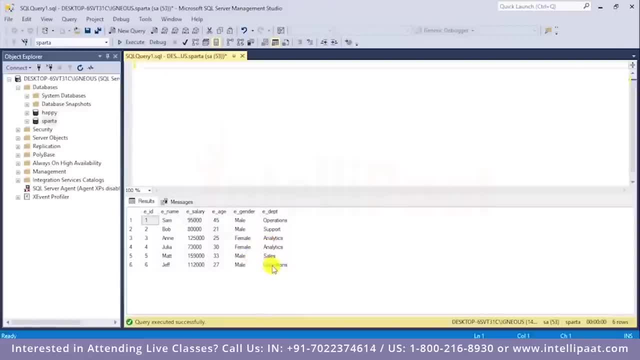 with respect to the department column and then use the halving clause to display only those departments where the average salary is greater than $100,000.. So let me go ahead and write the syntax For that. I will type in the select keyword and: 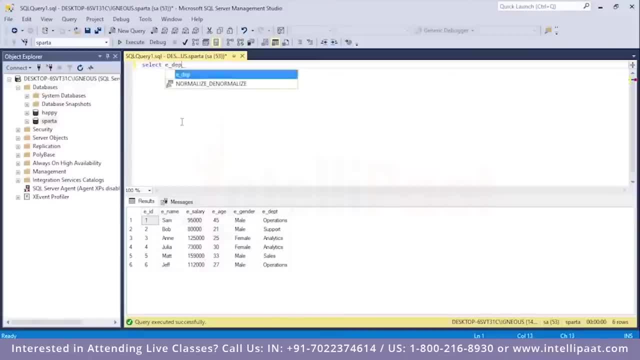 then list on all of the columns which I want from this employee table. So I need to do this. I can click on the close button here and then on the close button, the department column. I would also need the average salary, so I'll use the 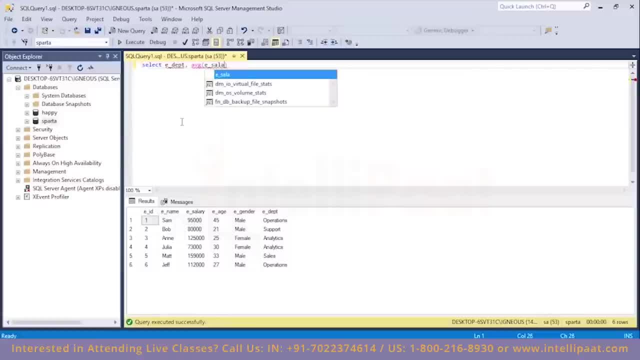 aggregate function AVG and then pass in the column which is e salary and I will name this column as average salary. now I would want this from the employee table, so I'll use the from keyword and then give the name of the table which is employee. after this I will give the group by keyword to group this table. 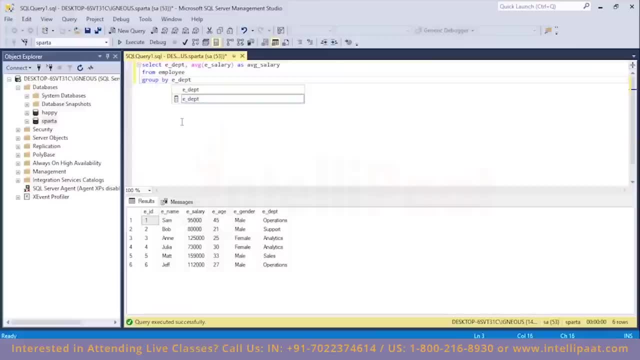 with respect to the department column. so I will give in the name of the column, which is e, te, PT. now, before I go ahead and use the halving clause, let me actually execute just these three lines of code, right? so what I've basically done is I have grouped this employee table with respect to the department. 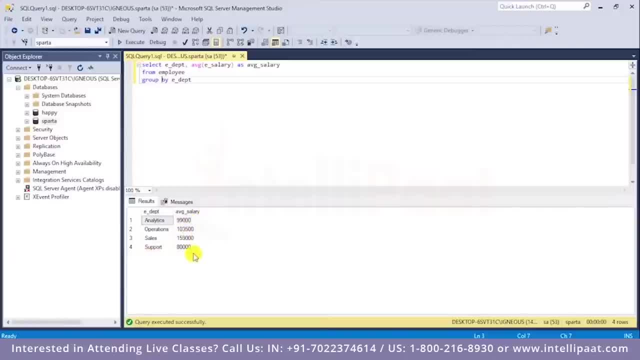 column and we have the average salary with respect to each of these departments, right? so this is the average salary of analytics department, average salary of operations department and average salary of sales and support. now I will use the halving clause to display only those records where the average salary is greater than $100,000. so the average. 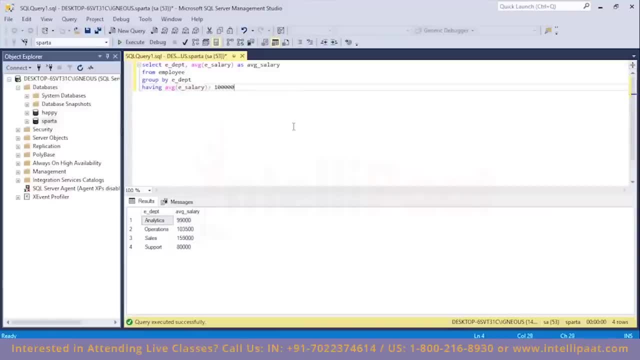 salary needs to be greater than $100,000. now I'll select all of this. I'll hit execute right. so we see that out of the four departments, only operations and sales department have the average salary of the employees to be greater than hundred thousand dollars. so the average salary of employees in operations 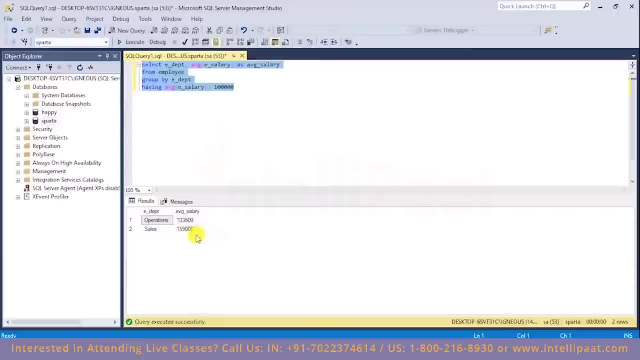 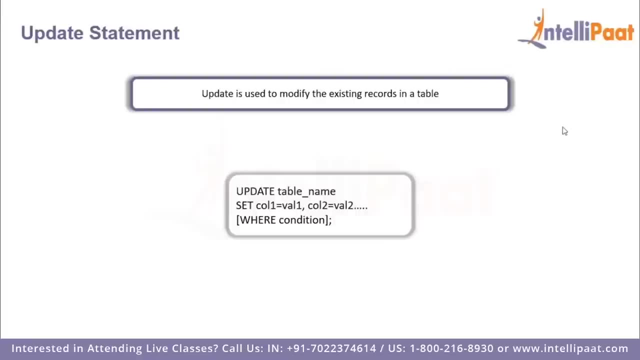 department as hundred and three thousand dollars, and the average salary of in the sales department is $159,000.. This is how we can work with a halving clause in SQL. So the update statement is used to modify or change the existing records in a table. 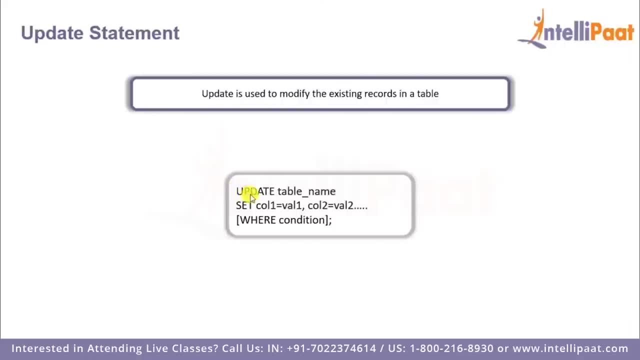 And this is the syntax for the update statement. So we'll start with the update keyword and then, given the name of the table, Then we'll use the set keyword and assign new values to the columns which you want to update And finally we'll use the where clause. 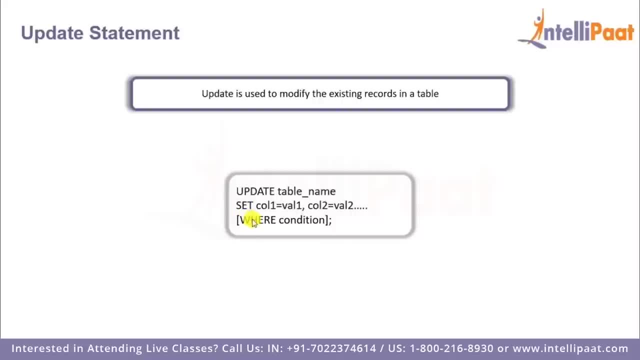 to give in the condition which should determine where the columns are to be updated. So I'm putting the where clause over here in square brackets, because it is optional. Now let's update some records of our employee table. So this is our employee table. 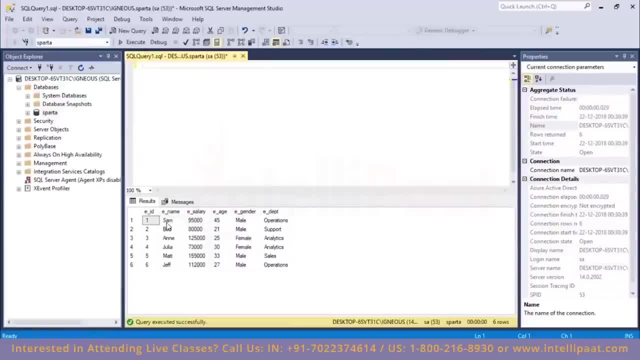 And I want to set this age value to 42, where the name equals Sam. So this would be the command for that. So I will give in the update keyword and then, given the name of the table, which would be employee, and then use the set keyword. 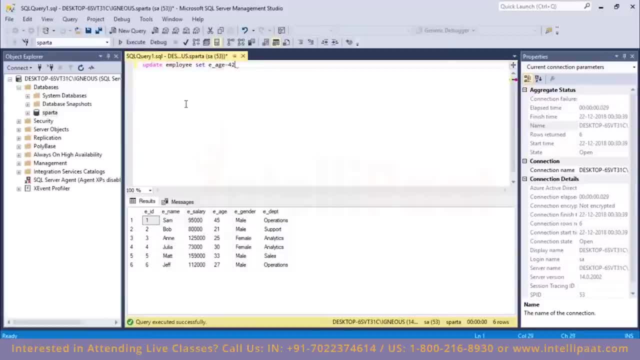 and then set the age value to be equal to 42. Then use the where clause and then set the condition. So the condition is the name should be equal to Sam. So where the name is equal to Sam, I am updating the value of age from 45 to 42.. 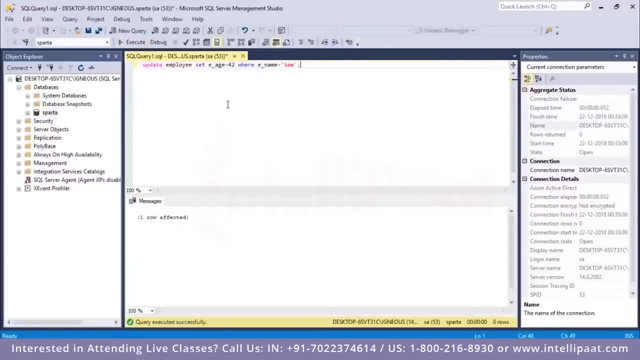 Let me put a semicolon, Let me hit execute So you see that one row has been affected. So now let me have a glance at the change table. Select start from employee. So we see that initially the age value was 45, where the name was Sam. 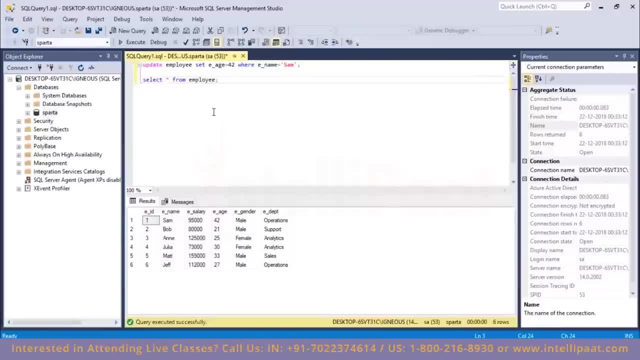 So the age value has been changed from 45 to 42.. Now, similarly, I don't want to change the department to tech, wherever the gender value is female, That is, I want to change the department of all of the female employees, from analytics to tech. 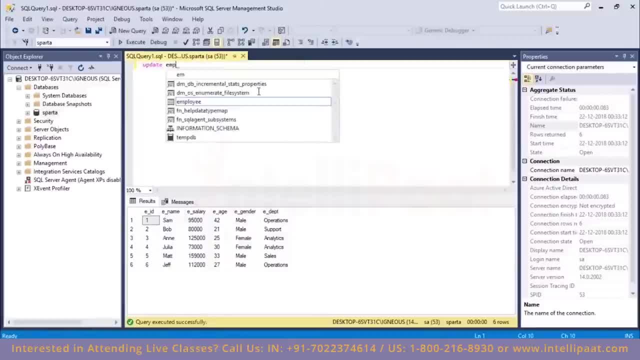 So this is how I can do it Again: update keyword, and then I'll give in the name of the table and then the set keyword. So over here I want to set the department to be equal to tech, where the gender is equal to female. 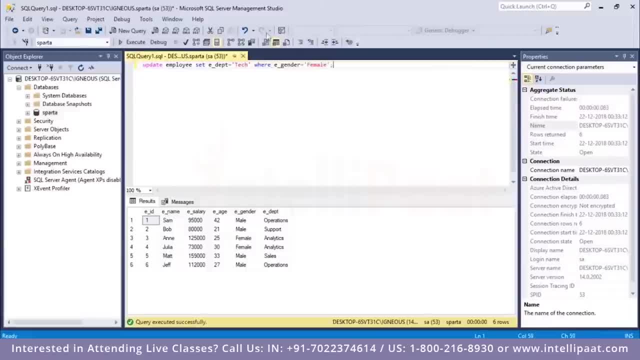 So let me put in female over here. So let me hit execute now and let's see what happens. So we see that two rows have been affected. Now again, let me have a glance at the modified table. Select- start from name of the table- is employee. 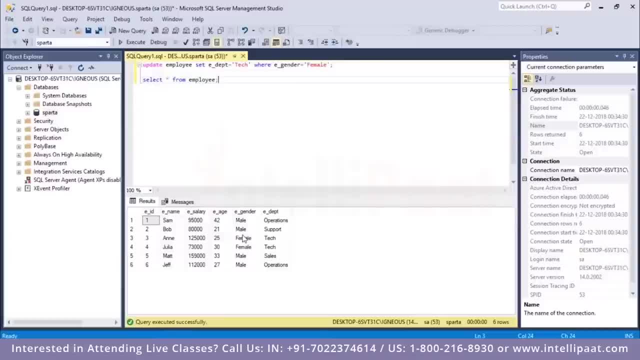 Right, You can see that initially, the department of both of the female employees was analytics, So that department has been changed from analytics to tech. Now I want all of the employees to have the same salary, So I will update this entire column to have the same value, which is $50,000.. 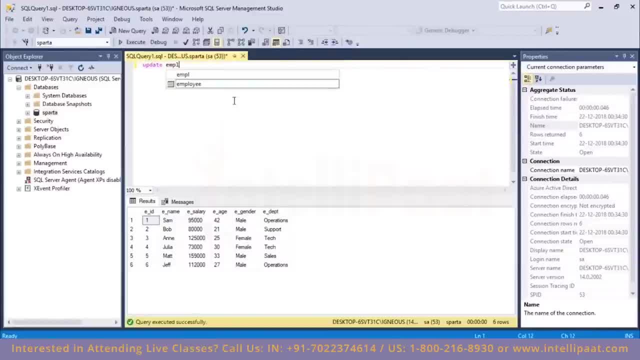 So this command would be quite simple: Update and then the name of the table which is employee, And then I'd have to set the salary to be equal to 50,000.. That's it. Let me hit execute. So we see that six rows have been affected. 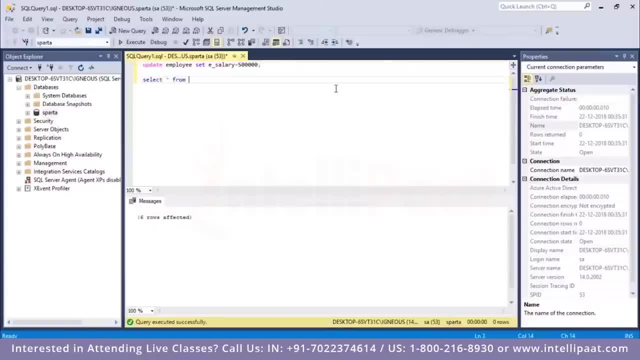 Again, let me have a glance at the modified table. Select start from the name of the table. is employee Execute- again Right. so we see that the salary has been right. so we see that the salary has been updated. So every employee's salary is same. 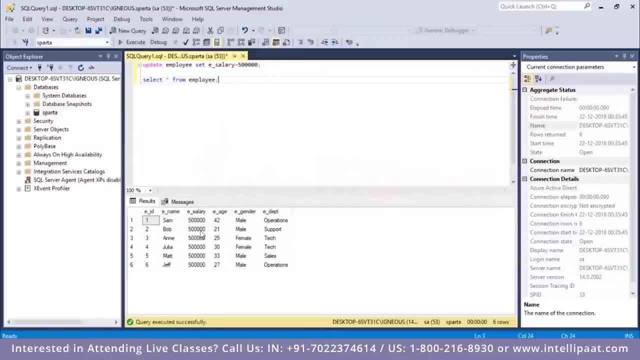 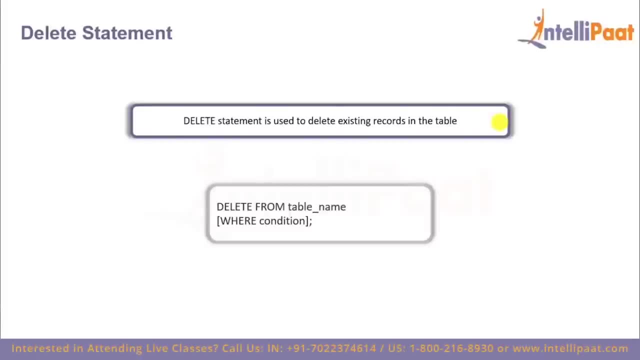 It is $50,000 per annum And this is how we can work with the update. So the delete query is basically used to delete or remove one or more existing records in the table. So let's have a look at the syntax. We'll start with the delete keyword. 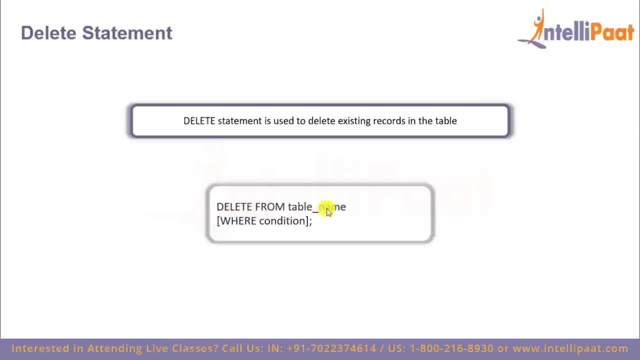 and then put in the keyword. from Then we specify the name of a table. After that we'll specify the var condition, But that's optional. Now let's delete some records from our employee table. So we have our employee table right here. 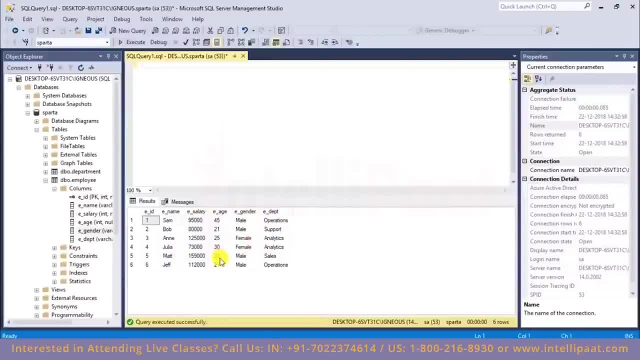 And I'd want to delete that record where the age of the employee is equal to 33.. So this would be the command for that. I will give in the delete keyword and then I'll type from and give in the name of the table. 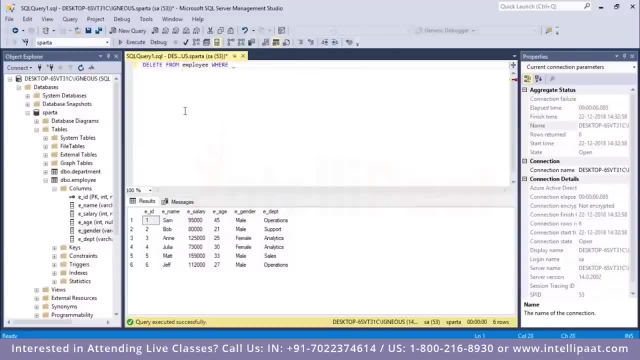 which would be employee. After that I'll use the var clause and give the condition. So the condition would be: eh is equal to 33.. I'll put in a semicolon over here and I'll hit execute. So you see that one row has been affected. 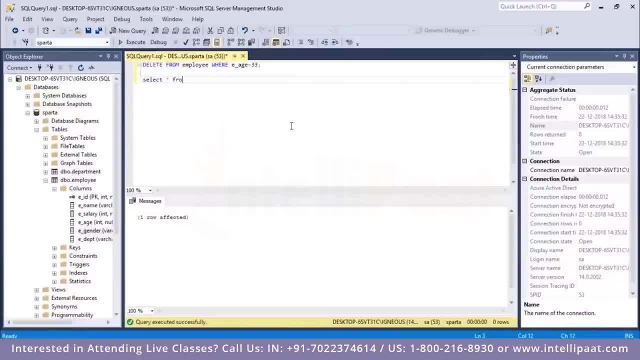 Now let me have a glance at the modified table. So I will type in select star from employee Execute- Execute again. So you see that that record where the age was equal to 33 has been removed. So initially we had six records. 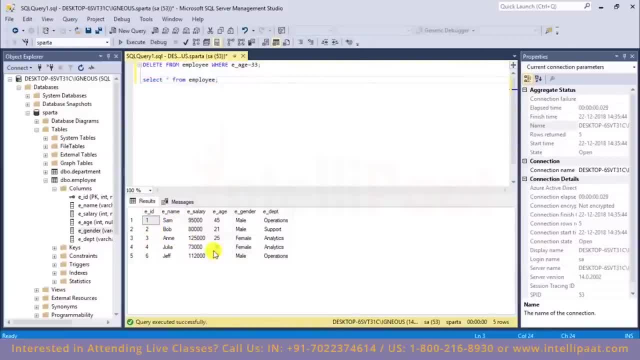 Now we only have five records in our table Now. similarly, I'd want to delete that record where the employee name is equal to Sam. So let me write the command for that. So I will give in the delete keyword first and then I'll give in the from keyword. 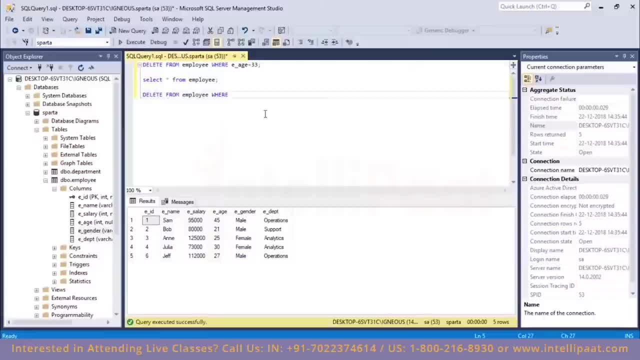 After that I'll give the name of the table employee, then use the var clause and then give the condition. So this time the condition would be eName. So eName is equal to Sam Right Execute. Again, we have one row which has been affected. 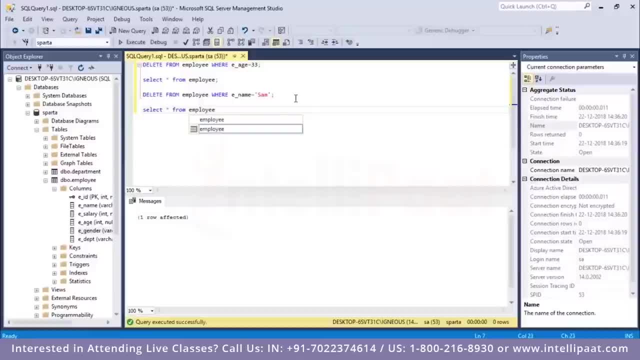 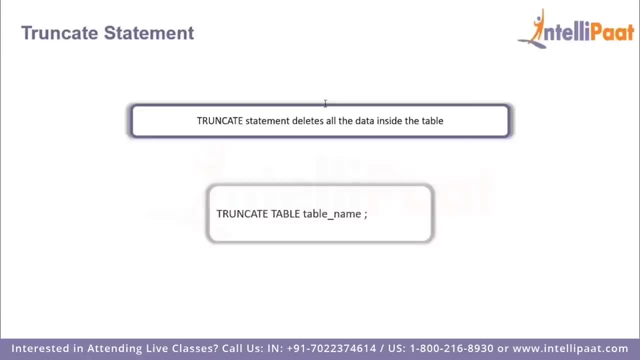 Select star from employee. And let's see the modified table now. So see that another record has been deleted And that record where the name was equal to Sam is the record which has been deleted. Then we have the truncate statement. So the truncate statement deletes all. 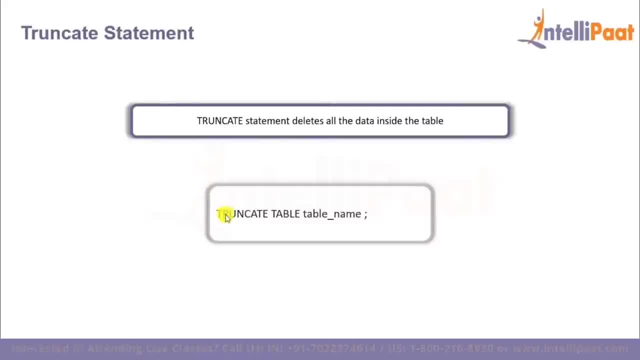 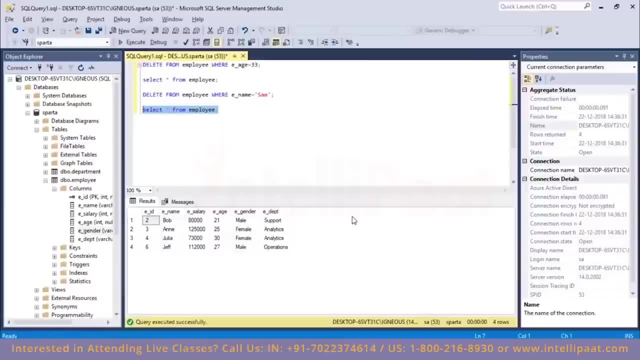 of the data inside the table. So here we'll give in the keywords truncate table and then give the name of the table. So let me go ahead and remove all of the records from this employee table using the truncate command. So I'll type truncate table and then I'll 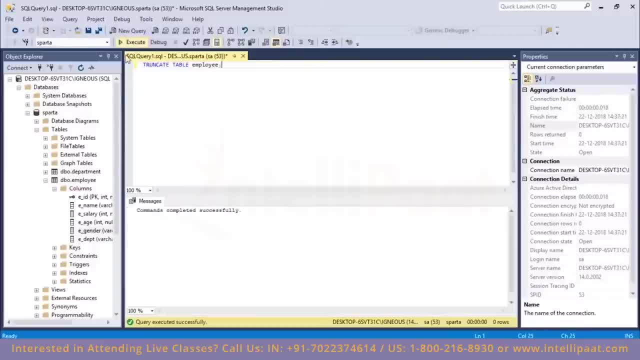 give in the name of the table, which is employee: Execute. So see that Commands completed successfully. Now I will type select Start from employee. Now let's see what do we get. So we see that all of the records are empty. 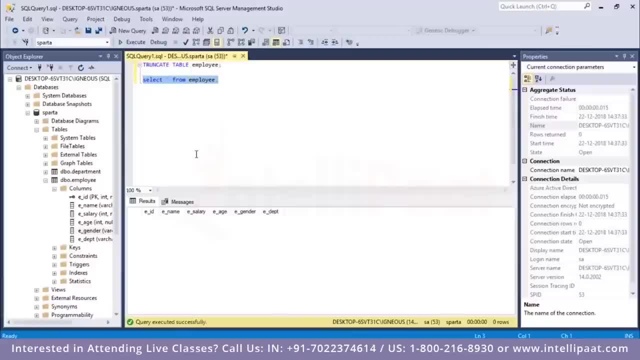 This is because the truncate table command basically removes all of the data from the table. And the specialty of the truncate command is, even though it removes all of the records from the table, the structure of the table remains intact. So we see that the structure of this table over here. 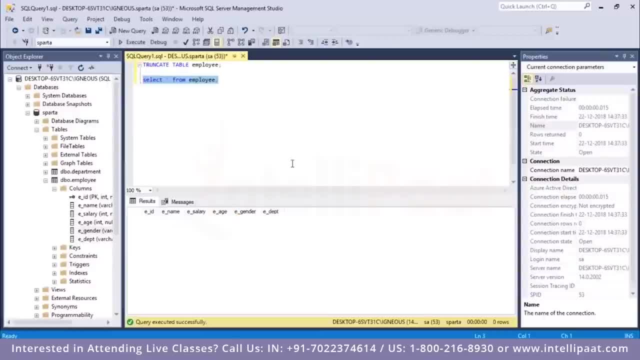 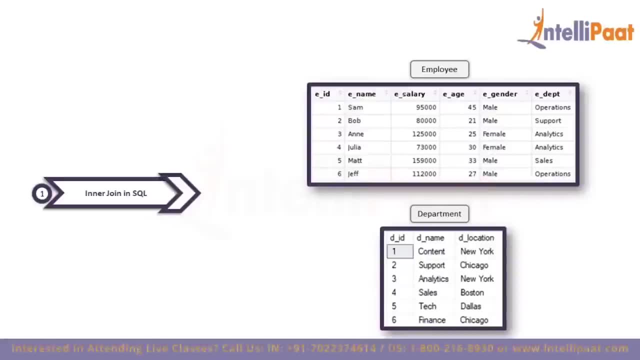 employee table. it is still intact. So this is how we can work with the delete and truncate statements, How to implement the inner join. We'll be implementing the inner join on these two tables. First is the employee table, which comprises of employee ID, employee name, employee salary. 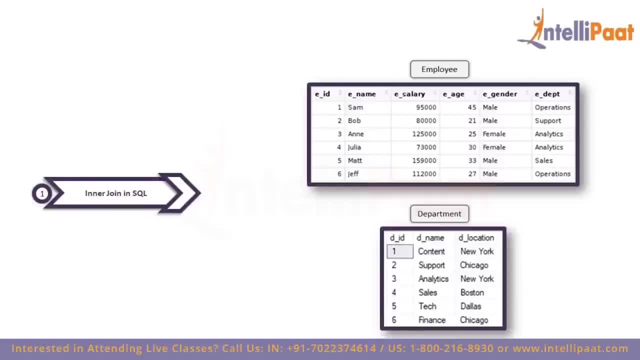 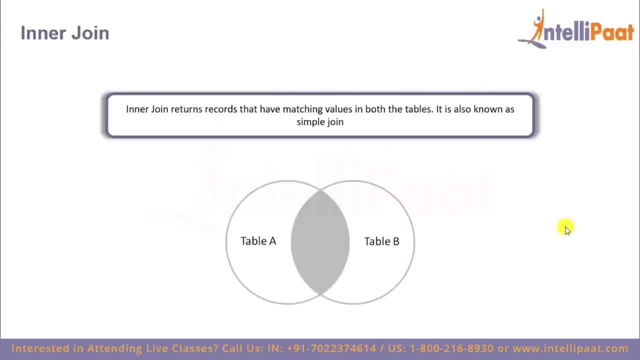 age and gender and the department in which the employee works. Then we have the department table, which comprises of department ID, department name and the location where the department is present. So the inner join basically gives us those records that have matching values in both the tables. 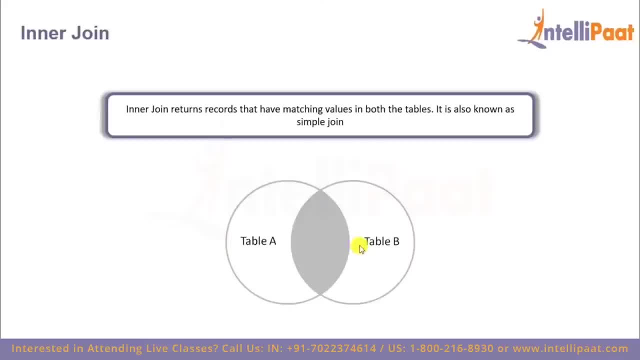 So let's say we have two tables, table A and table B, And when we apply inner join on these two tables we'll get only those records which are common to both table A and table B. So let's have a look at the syntax. 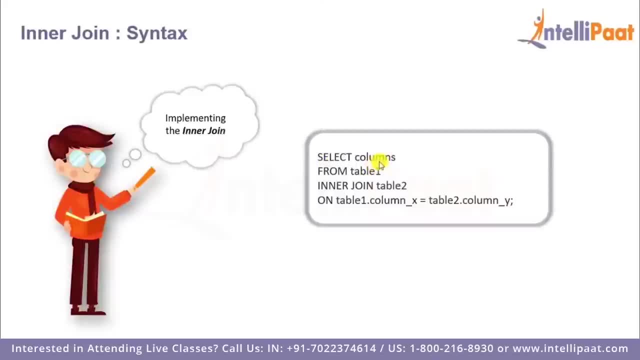 We'll give the select keyword first and then the list of the columns, following which we'll give the from keyword and give the name of the first table. Then we'll use the keywords inner, join and give the name of the second table. 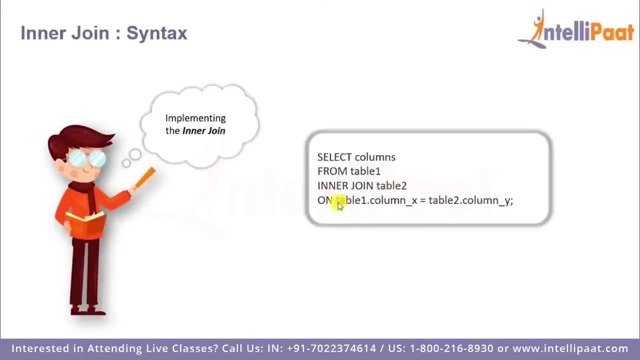 After which we'll use the on keyword. So this on keyword tells SQL that this inner join needs to be done on some condition, And that condition will be: values from column X of table 1 should be equal to the values of column Y from the table 2.. 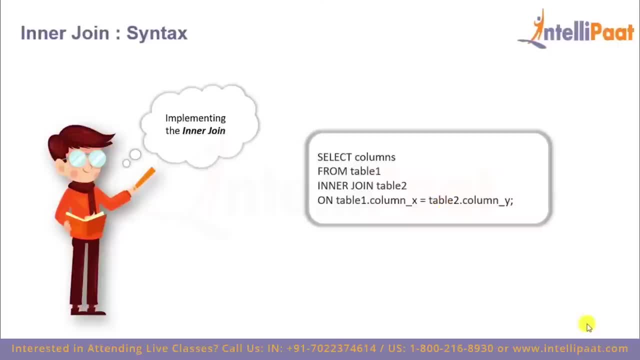 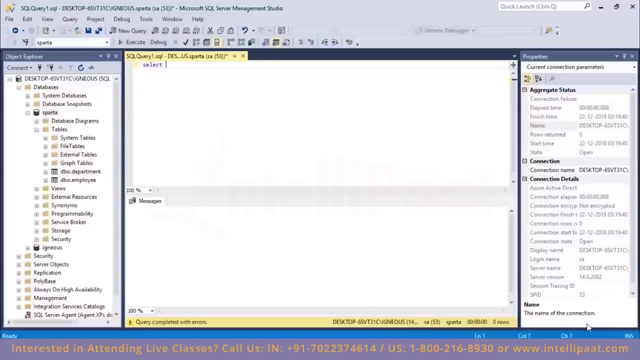 Now this might sound complicated, so let's just implement this inner join on the employee table and the department table. So before I go ahead and implement the inner join, let me have a glance at both of the tables. So I'll start with the employee table. 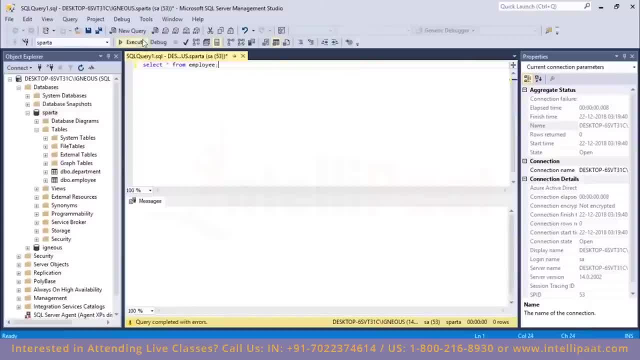 Select start from employee. So this is our employee table. So we see that we have this department column over here which tells us about all the departments in which the employees work in. Now, similarly, let me have a glance at the department table. 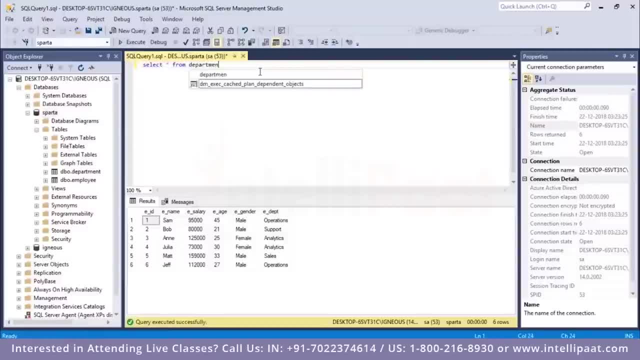 Select. start from. I will give them the name of the table, which would be department. So we have three columns over here And I have this D name column over here which gives me all of the names of the departments. So this is the common column between the employee table. 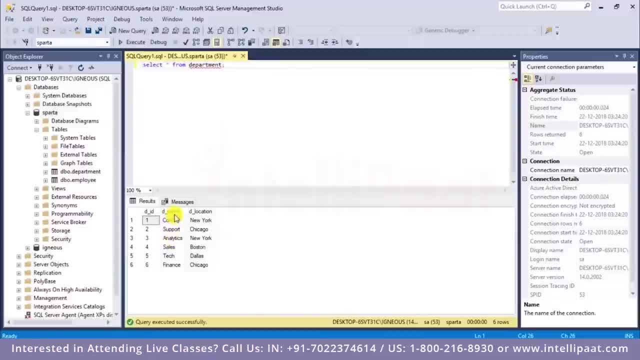 and the department table. We'll be applying the inner join condition on the D name column of the department table and the E, D, E, P, D column of the employee table. So let me go ahead with the syntax of inner join I will give in the select keyword. 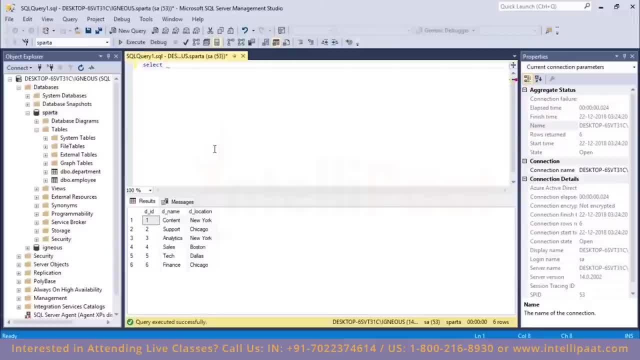 and then give in all of the columns which I do want to select. So I want to select the E name column and E, D, E, P, D column from the employee table. So first I would have to give in the name of the table. 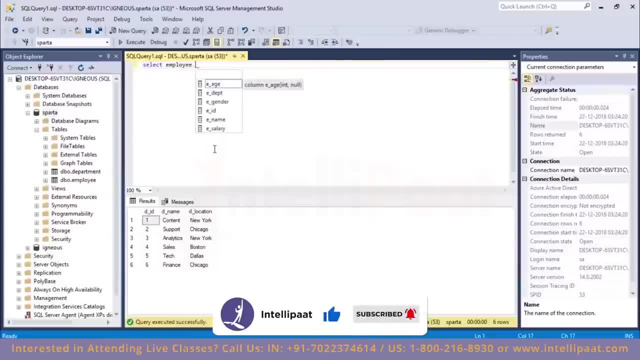 which is employee, Then I'll put dot over here and then give in the name of the column. So I want the name column from the employee table And similarly I'd also want the department column from the employee table. First I will give in the name of the table. 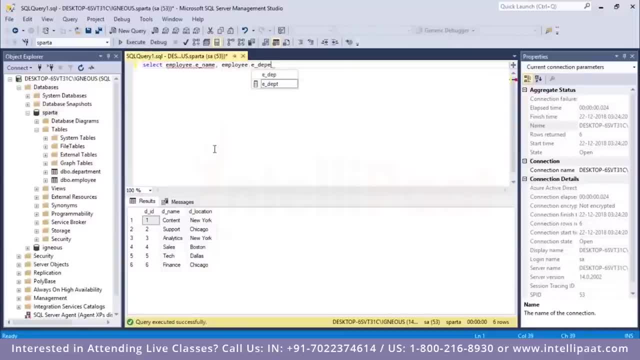 I'll put in dot over here and then give in the name of the column, which is E, D, E, P D. Right Now I'd also want the department name column and the department location column from the department table. So first I will give in the name of the table. 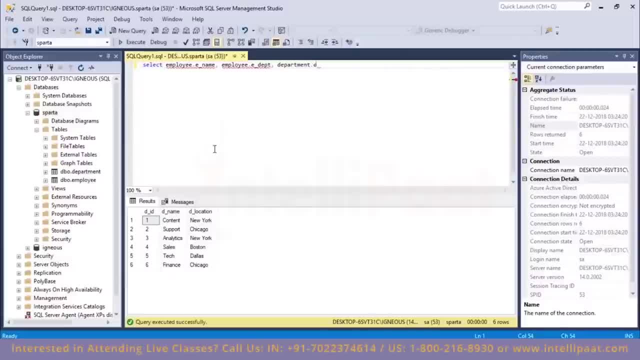 which is department, I'll put in dot over here and then give the name of the column which is D name. Similarly, I'd want to extract the department location column from the department table First. I will give in department over here. 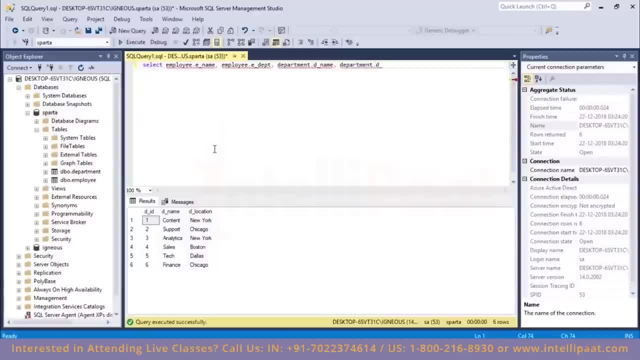 which is the name of the table. I'll put in dot And then I will give in the name of the column, which is D underscore location. After this, I will give in the from keyword and then give in the name of the first table. 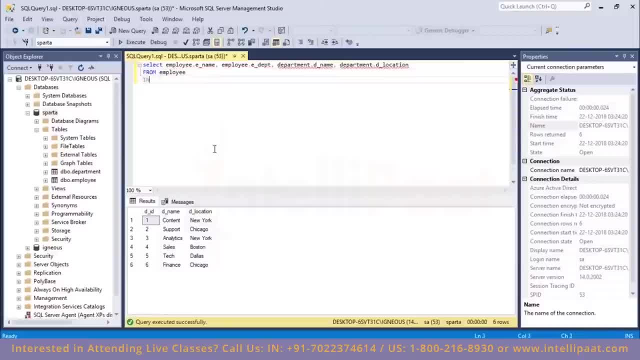 which would be employee. Then I will give in the keywords inner join, given the name of the second table, which would be department right. So I am selecting these four columns and the inner join would be on the employee table and the department table right. 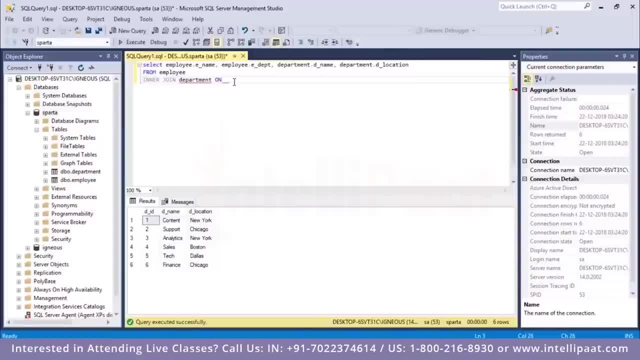 Now I will use the on keyword and give the condition. So the condition would be: the values of the E, D, E, P, D column of the employee table and the values of the D name column of the department table should be equal. So employee dot. 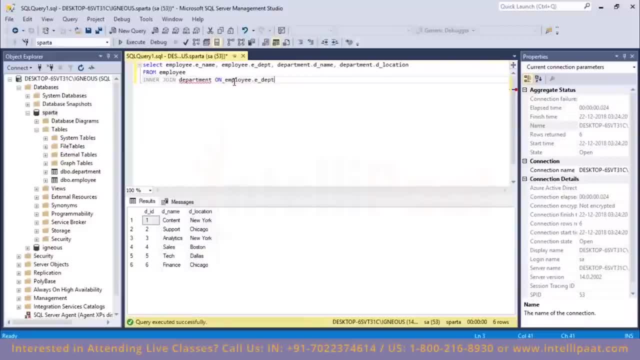 E D E P D column of the employee table should be equal. So employee dot E D E P D should be equal to department dot D name. Right guys? so this is the complete syntax to implement inner join on these two columns of the employee table and the department table. 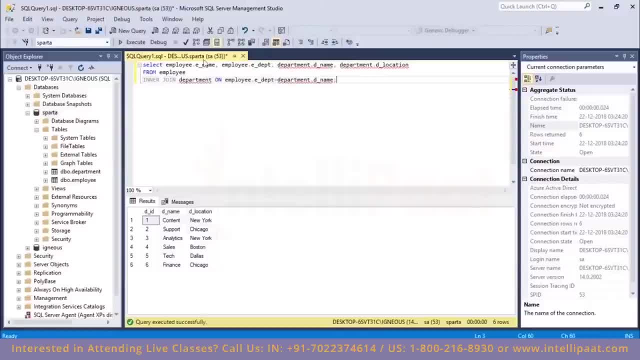 And I'm selecting the E name and E department columns from the employee table and D name and D location columns to the department table. Let me hit, execute, right And this is what we get. We have these four columns over here: employee name, employee department. 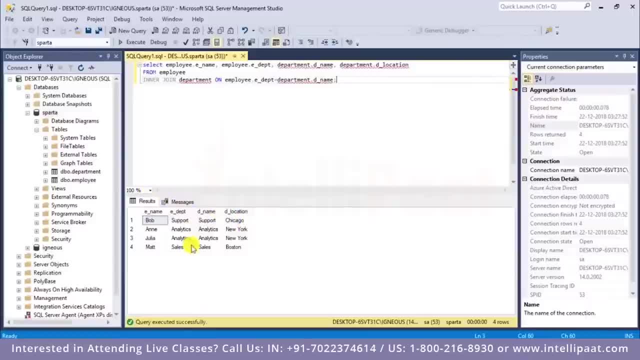 department name and department location. And since this is inner join, we have only those records where the values from E, D, E, P, D have matched to those values of D name, And this is how we can implement inner join. So the left join basically returns all the records. 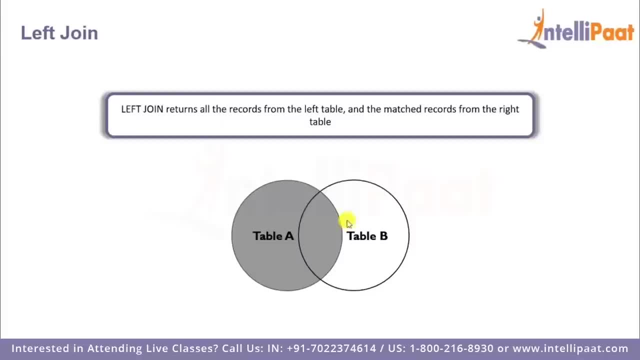 on the left table and the match records from the right table. So if we take table A and table B, then applying left join on these two tables would give us all the records from table A and only the matched records from the table B. So let's have a look at the syntax. 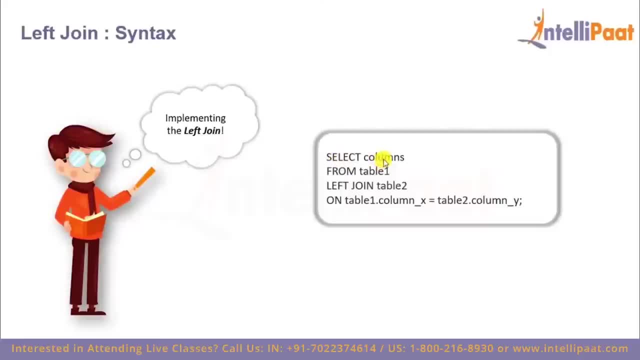 We'll start with the select keyword and then get the list of the columns, following which we'll give the from keyword and give the name of the first table. Then we'll use the keywords left- join- and then give the name of the second table. 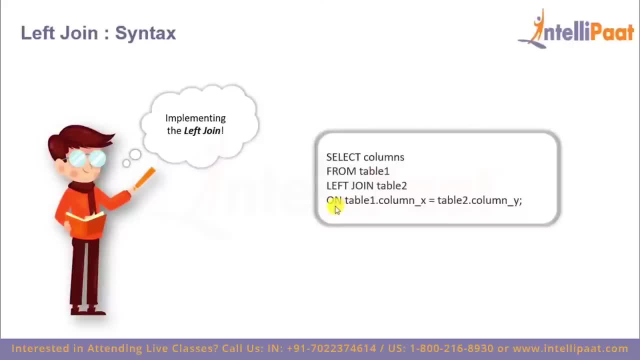 After which we'll use the keyword on. So this on keyword tells SQL that this left join needs to be done on some condition, And that condition would be: values from column X of table one should be equal to values from column Y of table two. 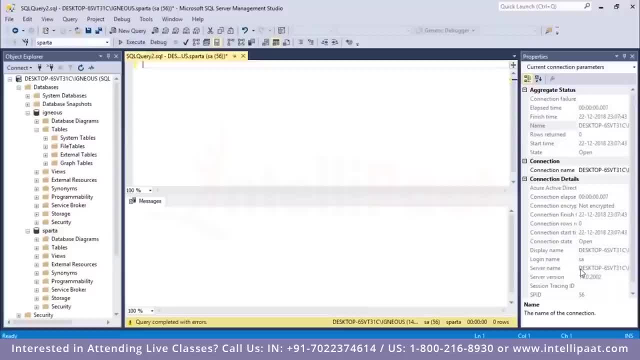 So let's implement this left join on the employee table and the department table. So before I implement the left join, let me actually have a glance at both of the tables. So I'll start with the employee table. Select star from employee And these are the columns present in the employee table. 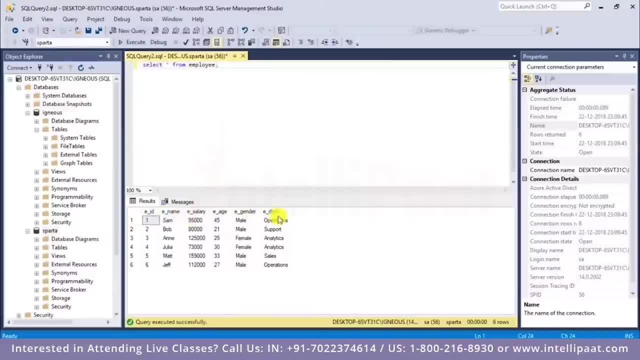 Employee ID, employee name, employee salary, employee age, employee gender and employee department. So I'll be taking this employee department column from the employee table Now. similarly, let me have a glance at the department table. Select star from The name of the table is department. 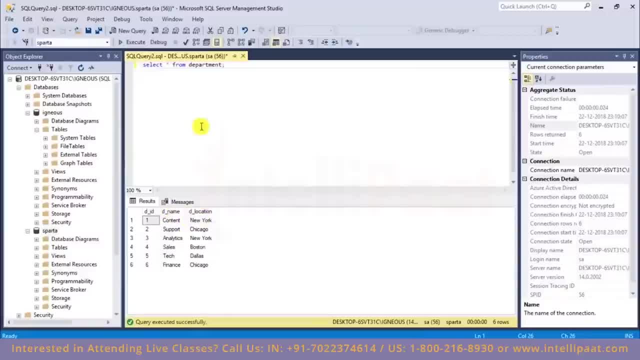 So we have the department ID, department name and the department location And from this department table we'll be selecting this D name column. So we'll be applying the left join on the E-D-E-P-T column of the employee table and the D name column from the department table. 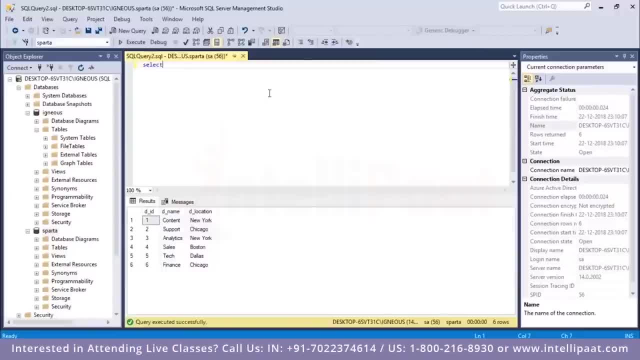 So let me start. Let's start with the syntax to implement the left join. So I will give in the select keyword first and then I will give all of the columns which I want to select. So I want to select the employee name column from the employee table. 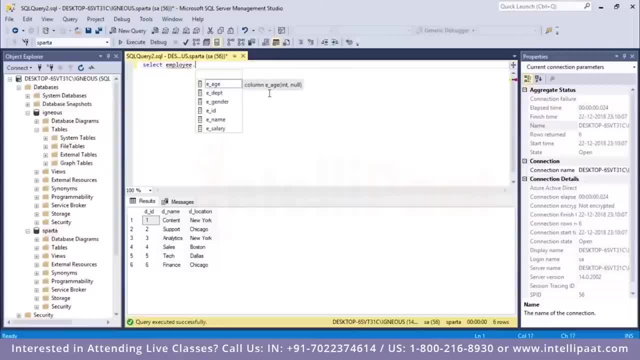 So first I will give in on the name of the table which is employee, Then I'll put dot over here and then I will type employee name. Now I'd also want the employee department column, So first I will give in the name. 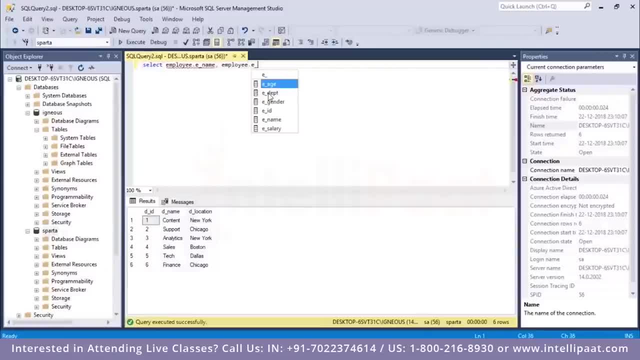 of the table which is employee, I'll put dot over here And then I will give in E-D-E-P-T over here. Then I'd want the department name name column and the department location column from the department table. so I will given the name of the table first which is department, I'll put a dot over. 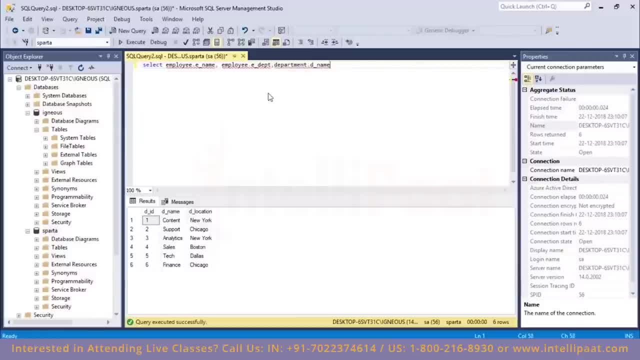 here and I will select the department name column from the department table. similarly, again, I will type in the table name, which is department, and I'll put a dot over here and then I'll also select the department location column. so now that I've selected all of the columns, let me give in the keyword from and then 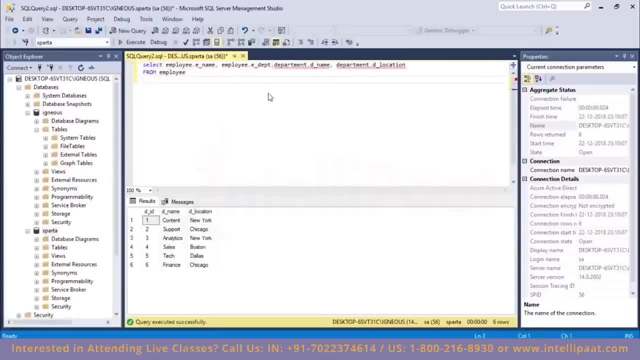 give the name of the first table, which is employee. then I'll give the keywords left- join- and then give the name of the second table, which is department. now I will give the on keyword and then give the condition, and the condition would be the values from the employee department. column from the employee table should be: 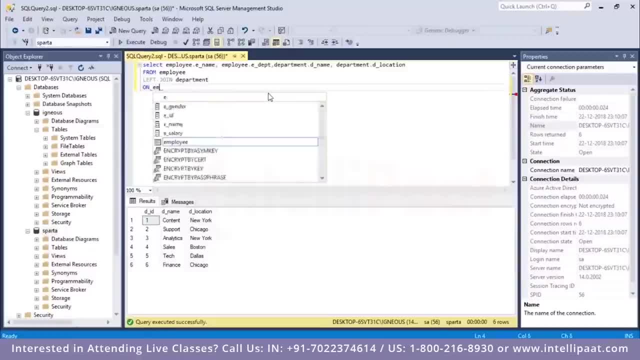 equal to the values of the department name column from the department table. so employee dot e, the EPT, these values should be equal to department dot T name. I'll put a semicolon over here now. let me hit execute. right. so this is the result when we apply the left join operation on the: 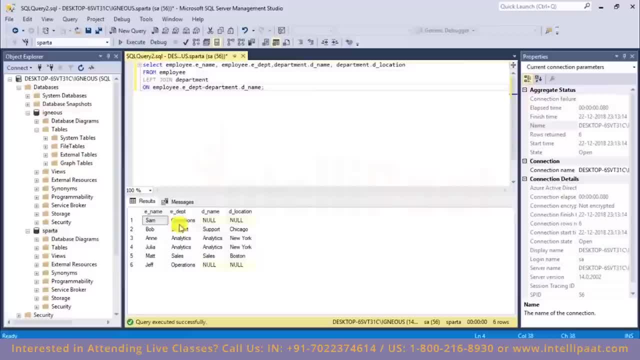 employee table and the department table. so we've got all of the records from the left table, which is the employee table, and we see that we get only the match records from the department table, which is the right table. over here and wherever the records haven't matched, we get null values. so you see that the 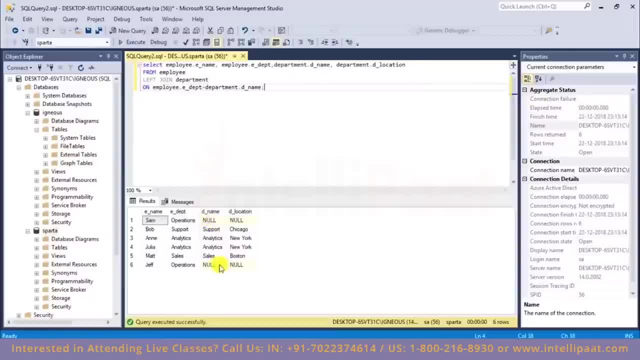 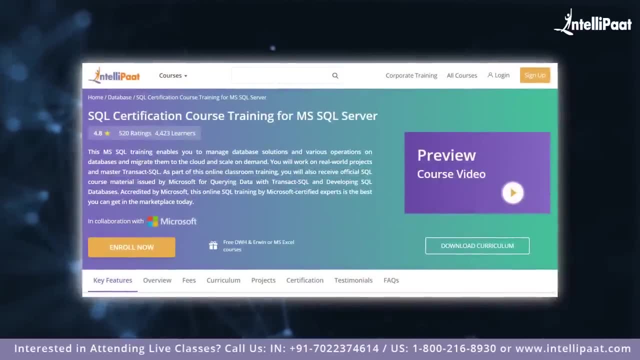 operations department is not present in the department table, so that is why we have null values over here, and this is how we can implement a left join. just a second for guys. Intellipaat provides SQL online training in partnership with Microsoft and mentored by industry experts. the course link is given in the 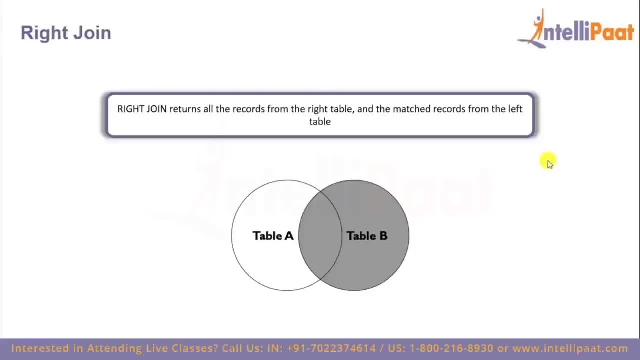 description below. now let's continue with the session. so the right join basically returns all the records from the right table and only the match records from the left table. so if we take table A and table B, then applying right join on these two tables would give us all the records from table B and 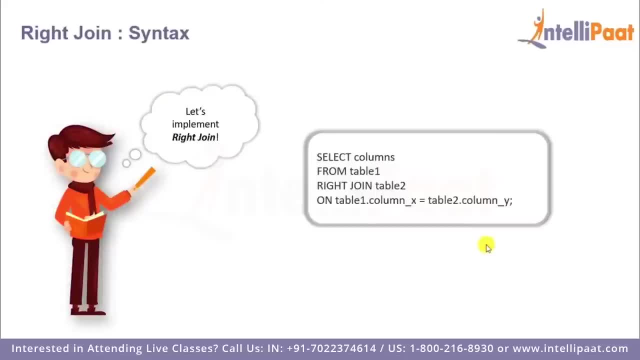 only the match records from table A. so let's have a look at the syntax. we'll start with the select keyword first and then given the list of the columns, following which we will give the from keyword and then give the name of the first table. then we'll use the keywords right, join and then give the 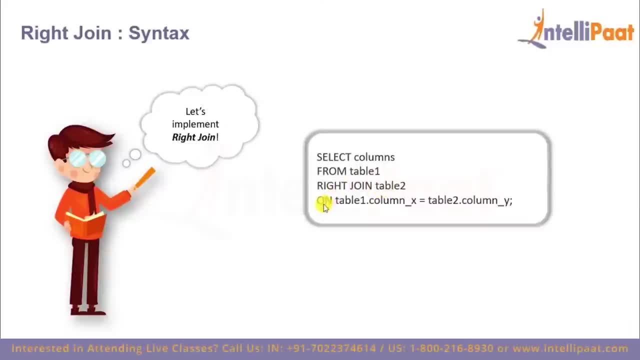 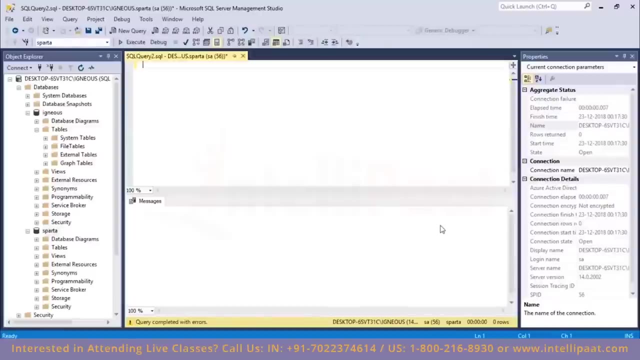 name of the second table, after which we'll use the keyword on. so this on keyword tells SQL that this right join needs to be done on some condition, and that condition would be: values from column X of table one should be equal to values from column Y of table two. so before I go ahead and implement the 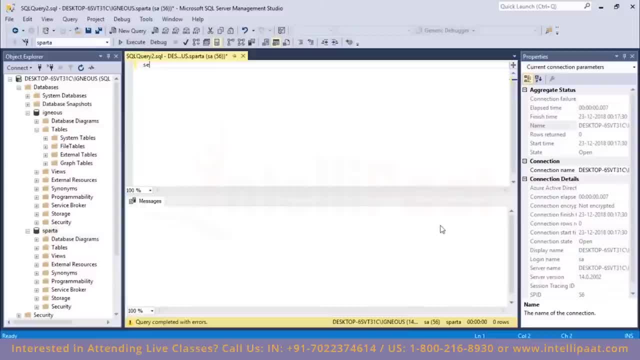 right join. let me actually have a glance at the employee table and the department table. so I'll start with the employee table. select star from employee. so this is our employee table, which comprises of these columns: employee ID, employee name, employee salary, employee age, employee gender and employee. 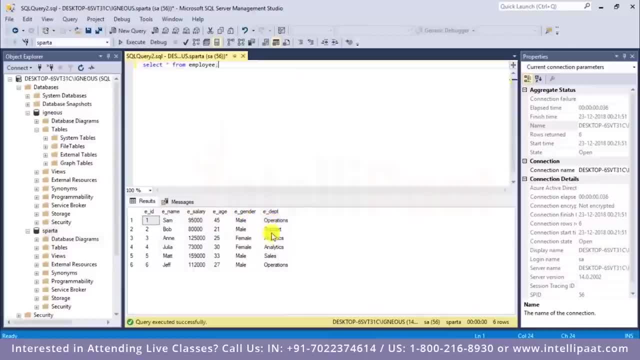 department and will be implementing the right join with respect to this column employee department. now let me also have a glance at the department table. select star from the name of the table as department. I'll hit execute. so the department table comprises these three columns: department ID, department name and department location. 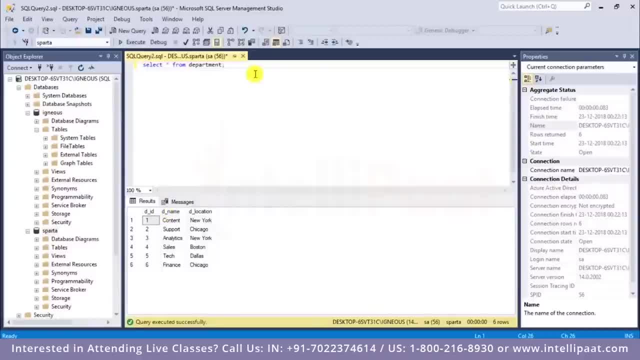 and we'll be implementing the write join with respect to this D name column. so now let me go ahead and write the syntax for the write join. so I will put in the select keyword first and then I'll give in all of the columns which I want to. 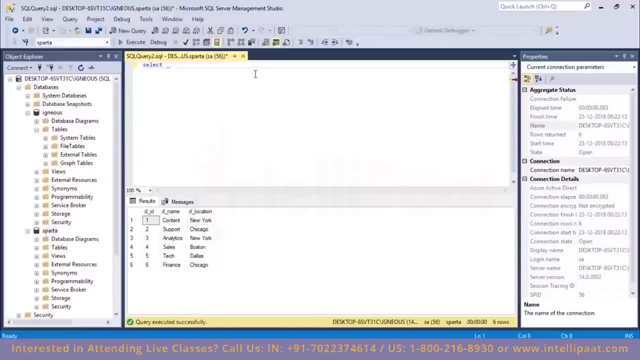 select, so from the employee table. I want to select the employee name and the employee department columns, so for that I'd have to give in the name of the table first, then I'll put dot and then I will give in the name of the column which I want to select, so employee name. similarly I also want the employee. 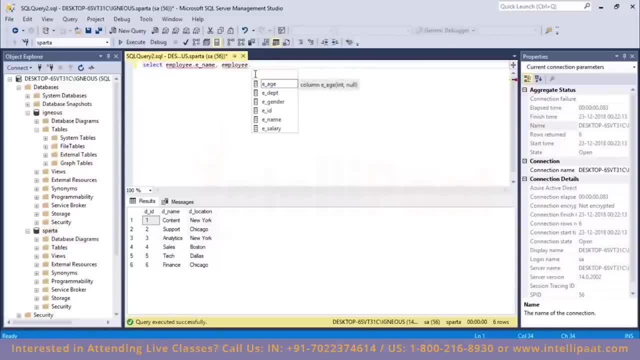 department column. so first I will give in the name of the table which is employee, dot. and then I'll select the EDPT column and then I want the department name and department location columns in the department table. so I'd have to give in the name of the table which is department. I'll put in dot over. 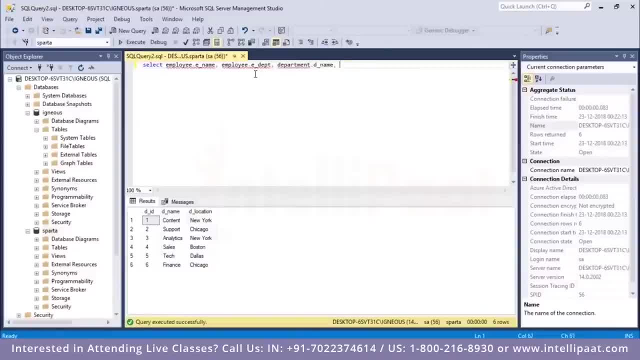 here and then given the name of the column, which is D name. similarly, I'd also want the department location, so I'll put dot and then select department location. now I will given the from keyword and then given the name of the first table, which would be employee. after that I will type the keywords right- join- and then give the. 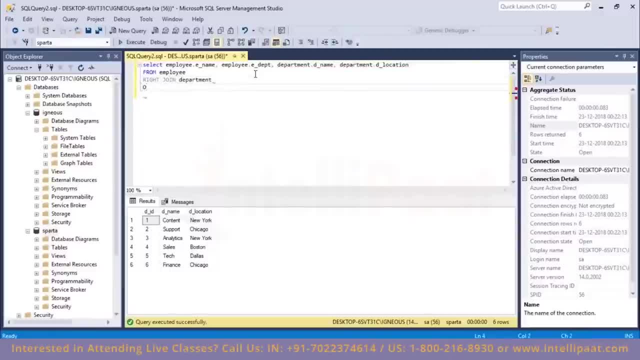 name of the second table, which is department, then I'll use the on keyword and then give the condition. so the condition would be: values of EDPT column from employee should be equal to values of D name column from the department table. so employee dot E DEPT should be equal to department dot D name. I'll put. 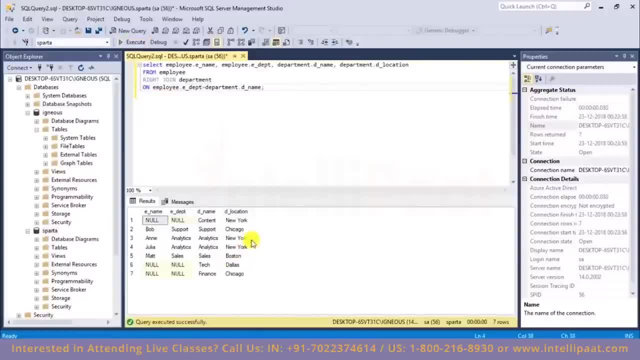 semicolon over here. let me hit execute. and this is the result which we get when we apply right join on the employee table and the department table. and since this is the right join, we see that we have all the records from the department table and we have only the match records from the employee table. so we see that. 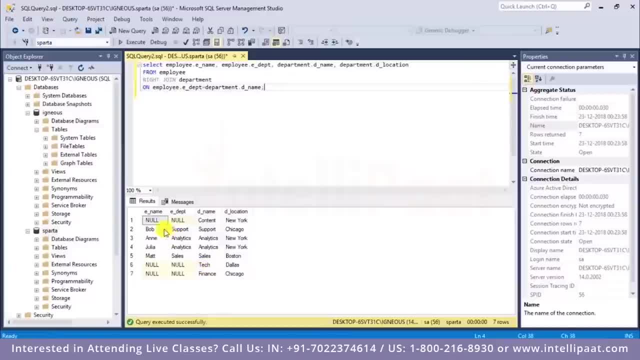 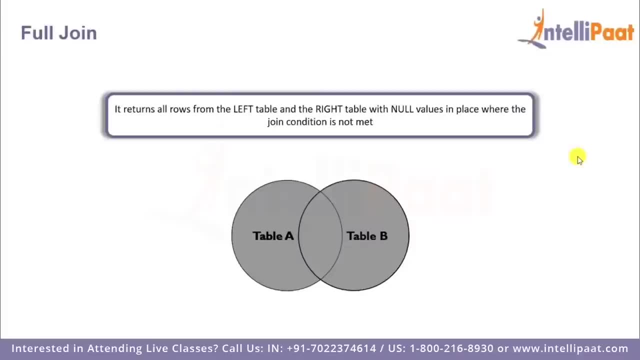 there is no content. tech and finance department is required to execute employee Departments in the employee table. So that is why we have null values over there and this is how we can implement the right join. So the full join basically returns all the records from the left table and also all the records from the right table. 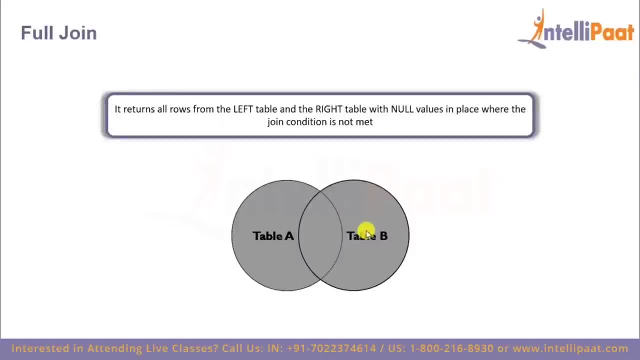 So if we take table A and table B, then applying full join on these two tables would give us all the records from table A and also all the records from table B, And wherever the join condition is not met, we'll get null values in that place. So let's have a look at the syntax. 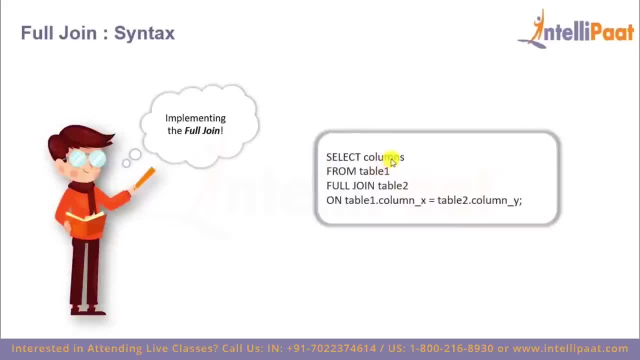 We'll start with the select keyword first and then given the list of the columns, Following which we'll give the from keyword and then give the name of the first table. Then we'll use the keywords full join and then give the name of the second table, after which we'll use the keyword on. 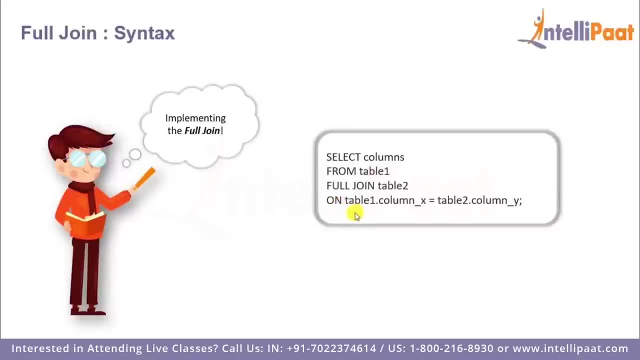 So this on keyword tells SQL that this full join needs to be done on some condition, and that condition would be: values from column X of table 1 should be equal to values of column Y from table 2. So before I go ahead and implement the full join, 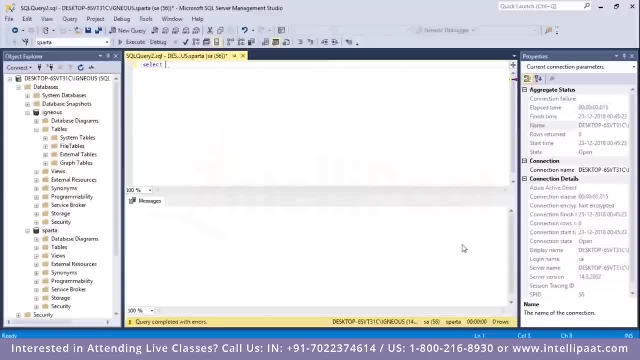 Let me actually have a glance at the employee table and the department table. So I'll start with the employee table first. So select start from the name of the table is employee. So we have these columns in the employee table: employee ID, employee name, employee salary, employee age, employee gender and employee department. and 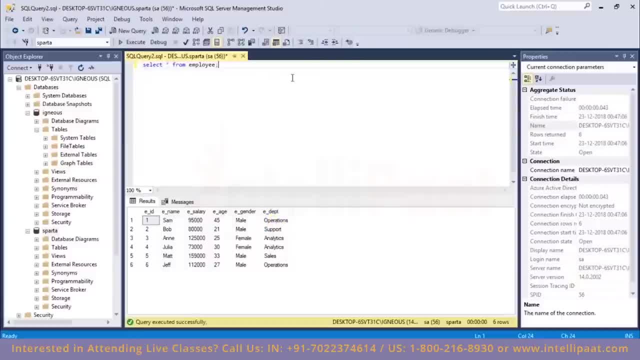 We'll be applying the full join on the employee department column. now let me also have a glance at the department table. select star from the name of the table as department. I'll hit execute. So the department table has these three columns: department ID, department name and department location, and we'll be applying the full join condition on this. 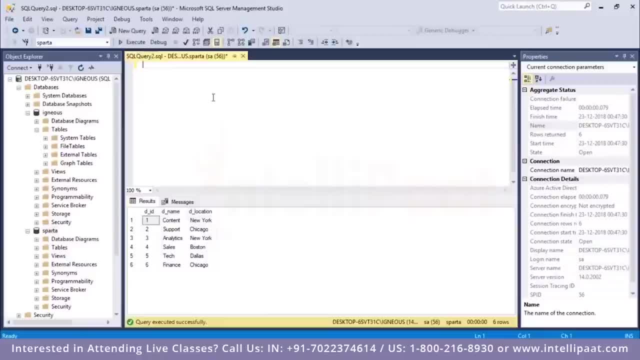 department name column. So let me start with the syntax for the full join. So I will give in the select keyword first and then I'll give in the list of all of the columns which I want to Select. so I want to select the employee name and the employee department. 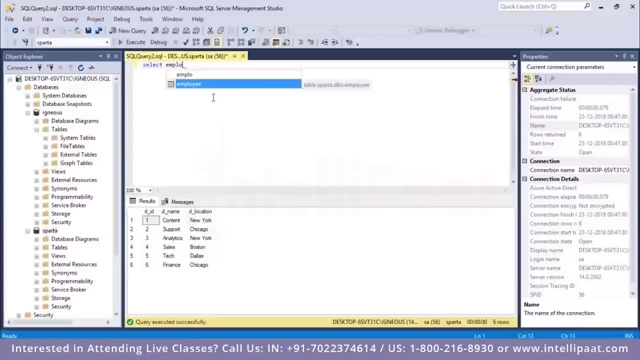 columns from the employee table. so So first I've given the name of the table, Which is employee, and then I'll give in the name of the column, which would be employee name. Similarly, I'd also want the employee department column, So I'll give in the name of the table: employee, I'll put dot over here and then I'll select the E, D, E, P, D column. 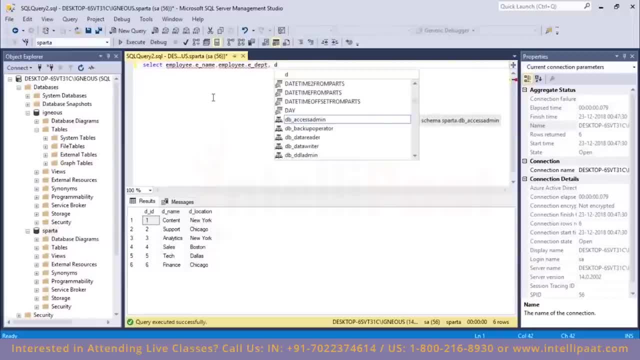 After that tied up, also want the department name and department location column for the department table. so I'll give in the name of the table: department, I'll put dot over here and then I'll select department department name. Similarly, I'll also select the department location column, So I will give in the 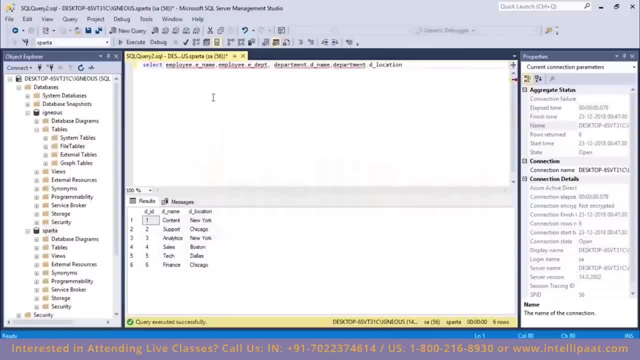 name of the table I'll put dot and then I'll select the department location column. After this, I will use the from keyword and then give in the name of the first table, which is employee. Then I will use the keywords full, join and then give in the name of the second table, which is department. 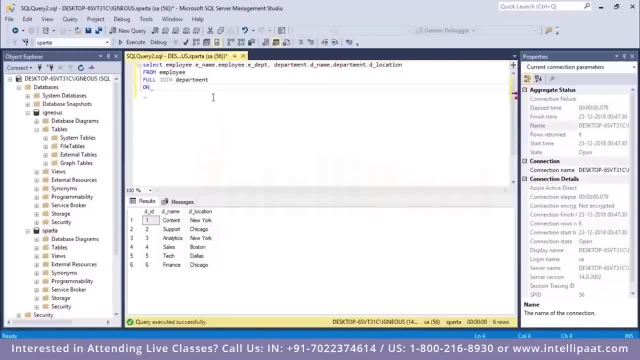 After that I will give the keyword on and then specify the condition on the basis of which the full join needs to be done. So the condition is the values of e dept column from the employee table should match with the values of the dname column from the department table. So that could be. 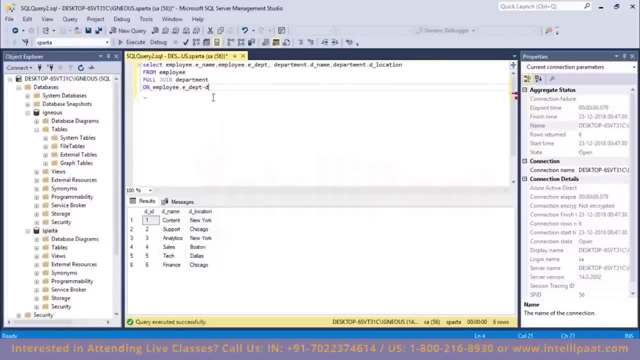 employee dot e dept is equal to department dot d name. I'll put semicolon over here. let me hit execute. So this is the result of the full join on the employee table and the department table. So wherever we see null values, that means that the records have not. 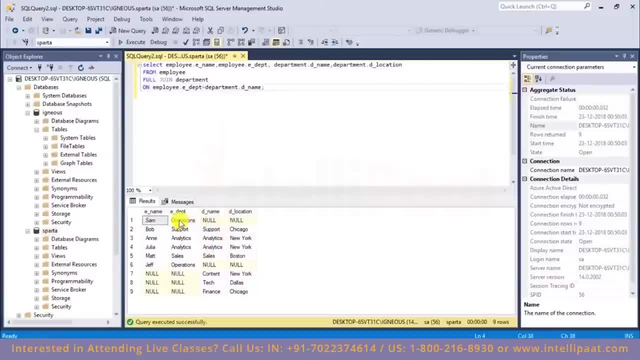 been assigned, matched over here. So operations is present in the employee table but it is not present in the department table. So that is why we have null values in the columns extracted from the department table. Similarly, we have content tech and finance departments only in the department table And that 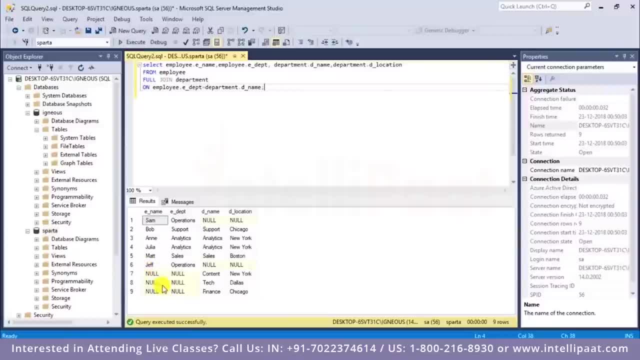 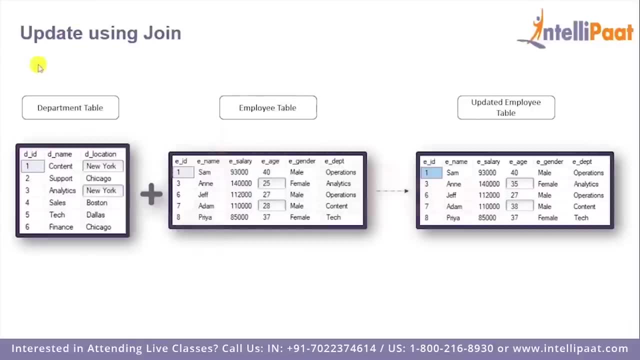 is why we have null values in the columns extracted from the employee table, And this is how we can implement the full join. So let's understand how can we use update with join Here we have two tables: the department table and the employee table. Now I'd want to update the each value in: 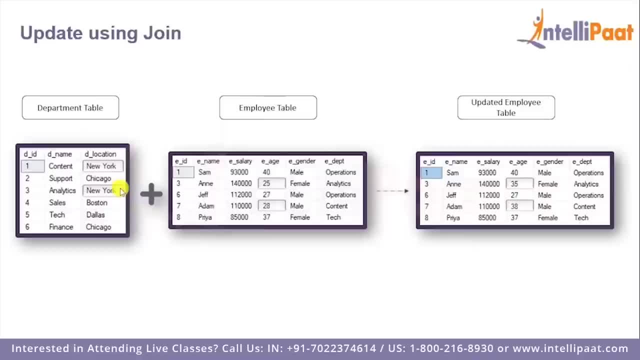 the employee table wherever the department location is New York. So for the department table we can find out that content and analytics departments are based in New York, So in the employee table we'll update those each values where the department is either analytics or 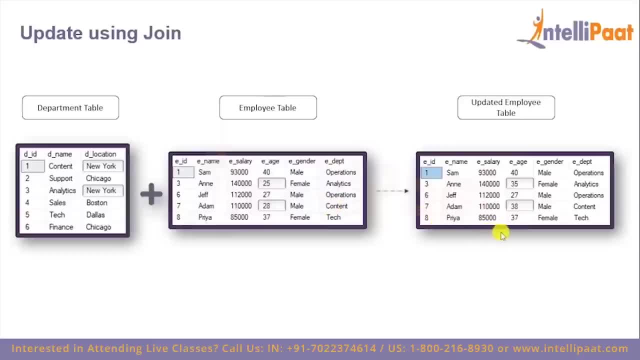 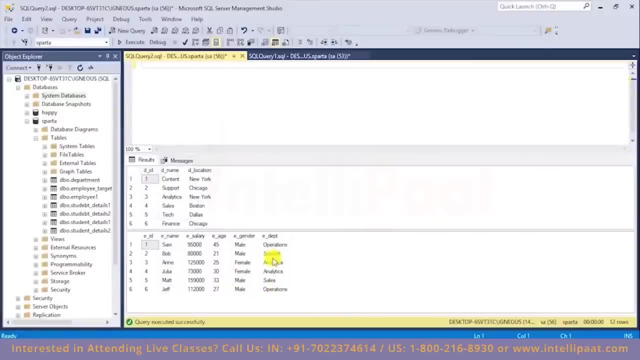 content And after updating the table using the join statement, we see that these two values have been modified. So we have the department and employee table write in front of us and we'll be implementing the same task. so from this employee table we'll add 10 more to the age values wherever the department 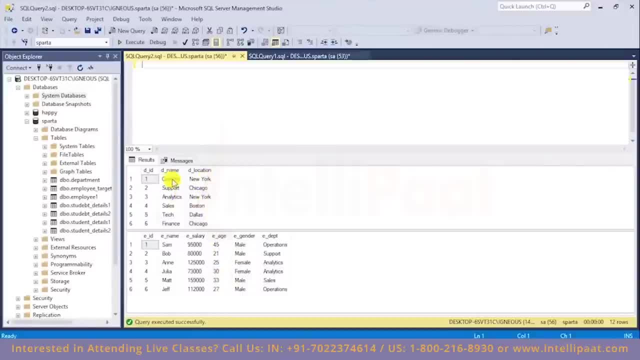 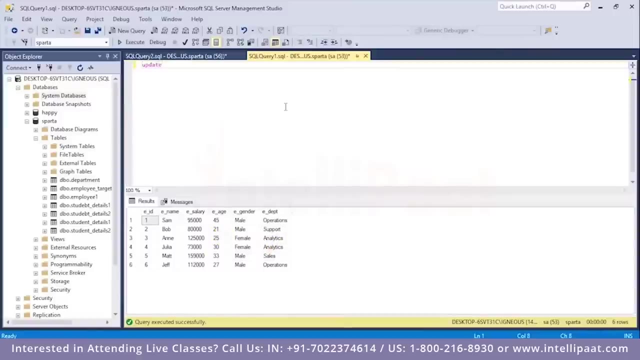 location is equal to New York and since we've already seen that content and analytics are based in New York- so basically these two records where the EDPT value is equal to analytics- we'll be adding 10 more to these two age values. so let me write the syntax for that: I'll type update and then give the. 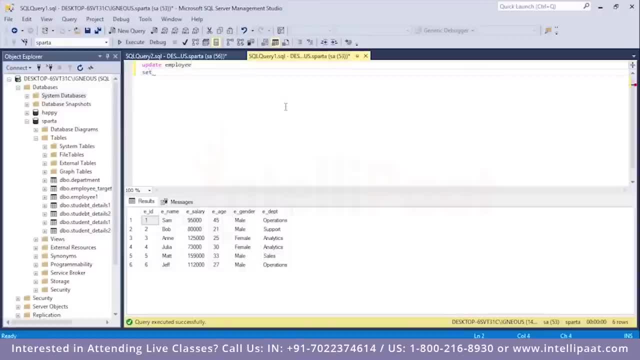 name of the table which I want to update. so that would be employee. after that I'll use the set keyword and then update the age value. so eh, and I'm adding 10 more to the eh value. after that I'll use the from keyword and give. 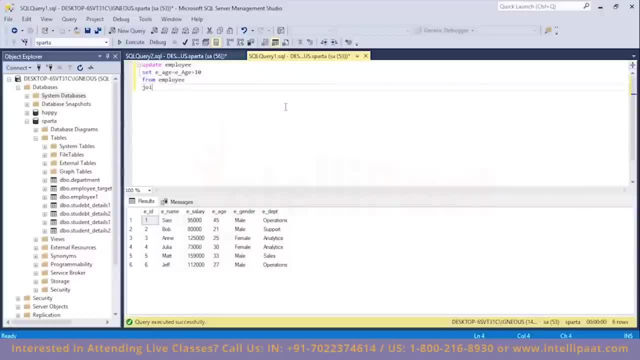 the name of the first table, which would be employee, then I'll type join and then give the name of the second table, which would be department. then I'll type on and then state the join condition. so the join condition is you. the values of the EDPT column from the employee table should be equal to the 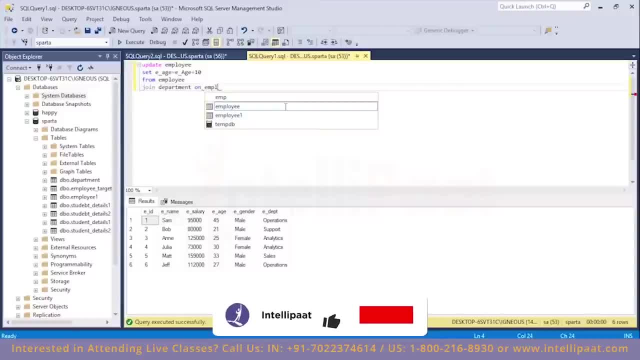 values of D name column from the department table. so employee dot EDPT should be equal to department dot D name. and finally, we'll specify the wire condition, which would be the location should be equal to New York. so while select all of this, I'll click on execute. so you see that two rows have. 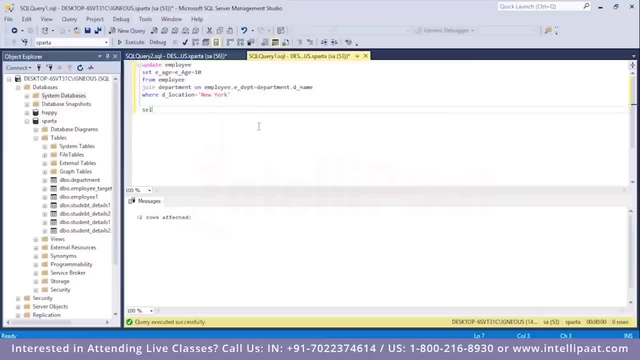 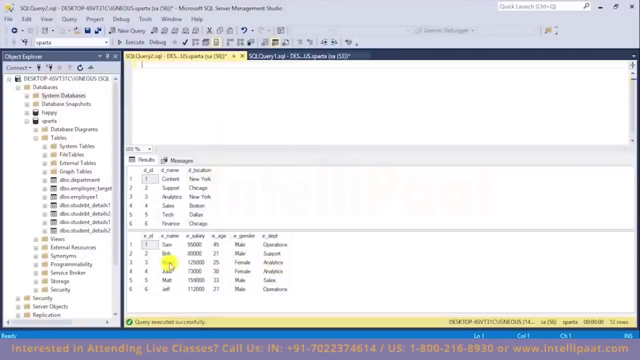 been affected. now let me have a glance at the modified employee table. select. start from. I'll type the name of the table which should be employee. now I'll execute this. so let me see the original age values. so over here the department is analytics and we see that the initial age of Ann and Julia is 25. 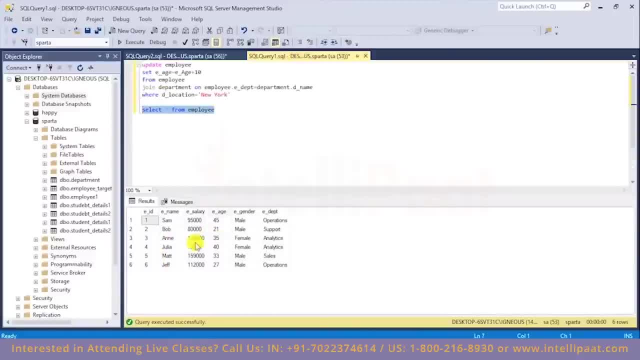 and 30, and after applying the update command, we see that the age has been been modified to 35 and 40. So Ann's initial age was 25.. After updating, it became 35. Similarly, Julia's initial age was 30. After updating, it became 40. So this is how we can use update with. 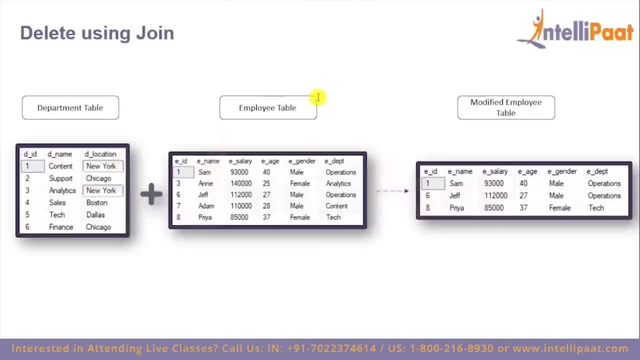 a join condition. Now let's understand how can we use delete with join? So this time, from the employee table, I'll be deleting those records where the department location is equal to New York, And since content and analytics are based in New York, we'll go ahead and delete those two. 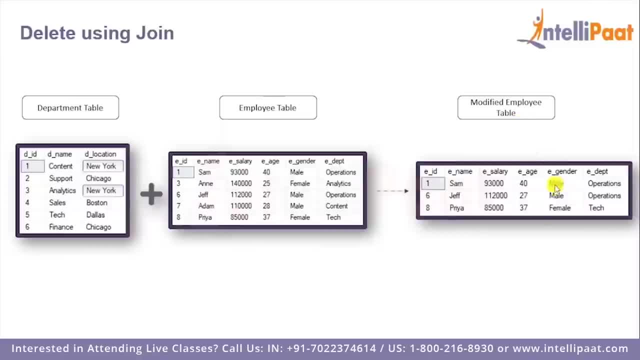 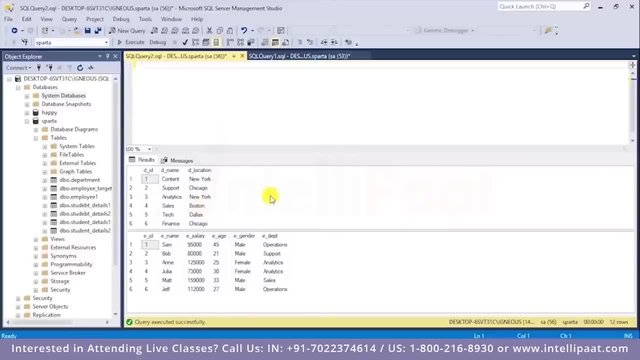 records from the employee table. So in the final modified employee table we see that there are no records for the department is either content or analytics. So again, we'll be implementing the same task From this employee table. I'll be deleting those records where the department 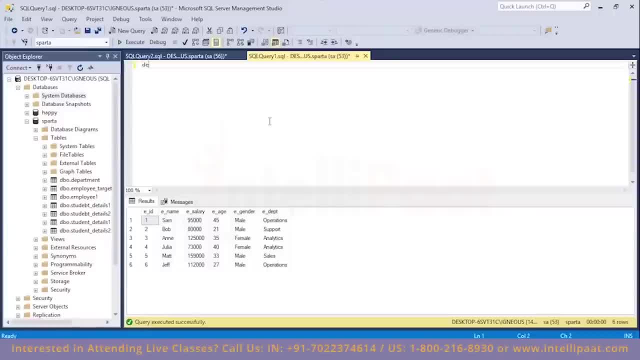 location is in New York. So let me write the syntax for that. So I'll type delete and then give the name of the table from which I'd want to delete the records. So that's would be employee. After that I will give the from keyword and then give the name of the first. 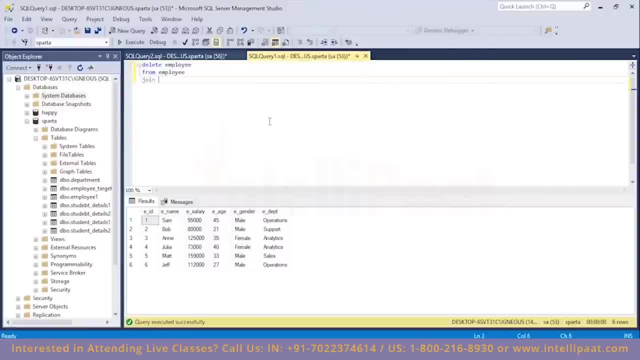 table, which would be employee. again. Then I'll type join and then give the name of the second table, which would be department. Now I will give on and give the join condition, which is same again. So the values of EDPT column from the employee table should be equal to the values of D name. 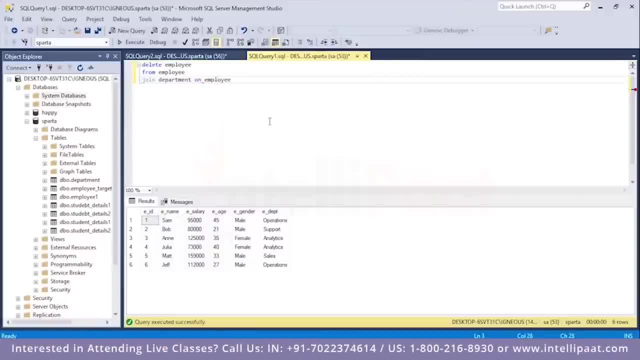 column from the department table. So employee dot EDPT should be equal to department dot D name. And finally I'll use the where condition, which would be D location should be equal to New York. So I'll select all of this, I'll click on execute. 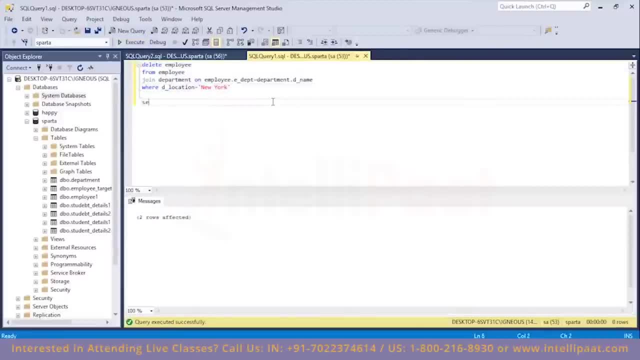 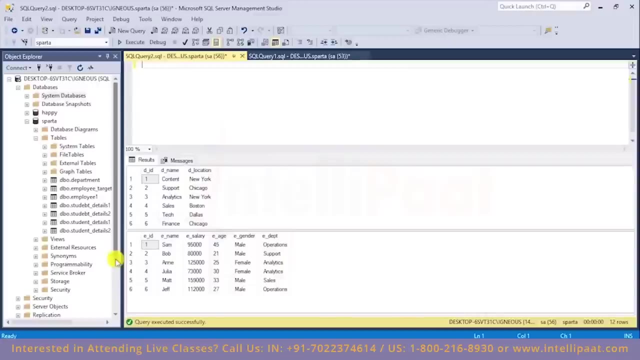 So again we see that two rows have been affected. Now let me have a glance at the modified table. Select start from employee. So see that there are no records for the department is analytics. So if you have a look at the original table, we see that there are two records. 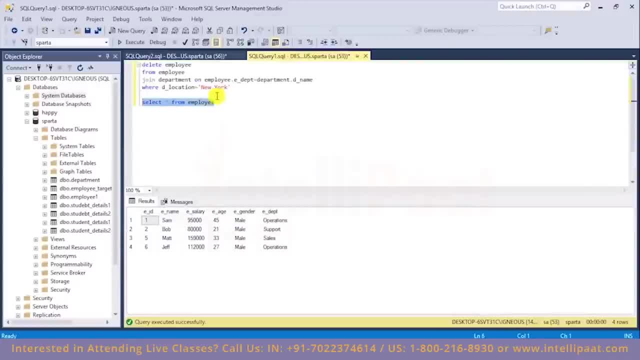 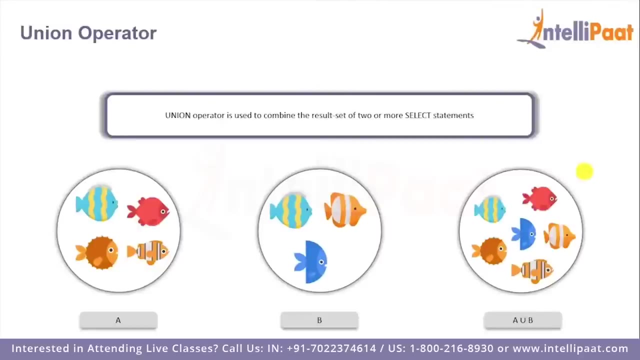 where the employees were present in the analytics department And after deleting those two records, we just have four records present in the employee table. And this is how we can work with: update and delete statements using join, So the union operator is used to combine the results of two almost select statements, For example: 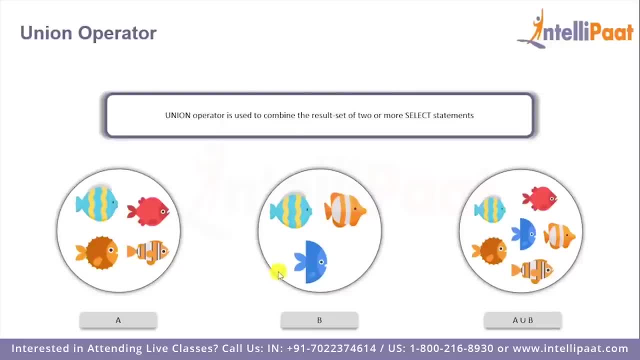 the first select statement returns these four fish and the second select statement returns these three fish, then the union operator would return the result set of these two select statements And there's a record which is present in both the tables. we'll get only one of them in the 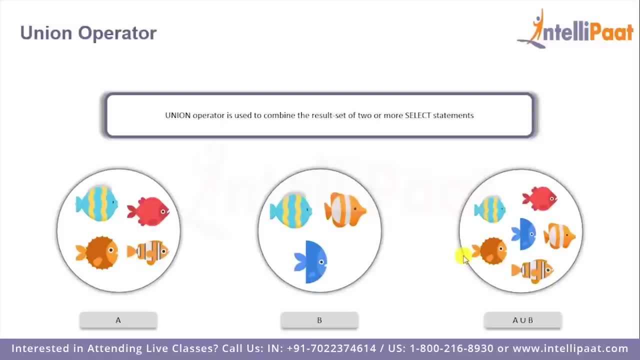 final result, That is, there will be no duplicates in the final result. So here we see that this blue fish, as present in both the tables A and B, but in the final result of a union B, they'll get only one of the value, And this is the syntax for the union operator. This is the syntax for the union. 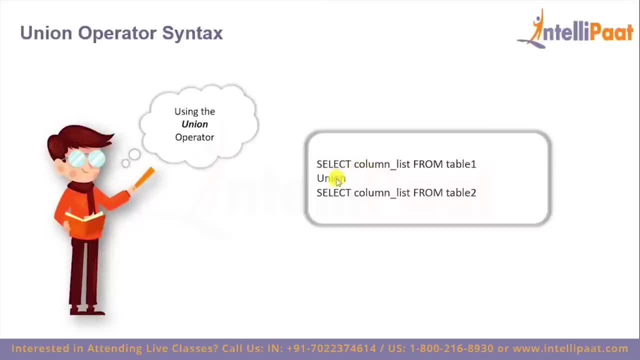 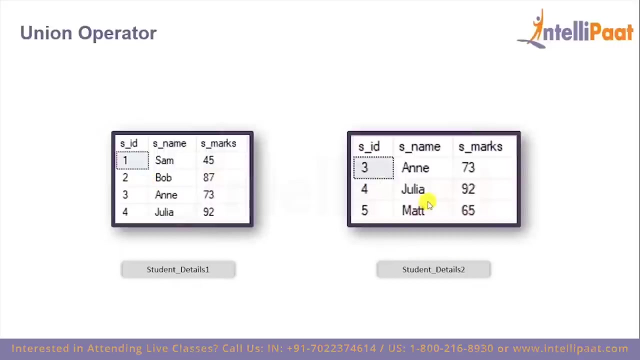 operator, we'll give the first select statement. after that, we'll give the union operator following, which will give a second select statement. now you also need to keep in mind that the number and order of columns must be same in both the select queries, and we'll be implementing the union operator on these. 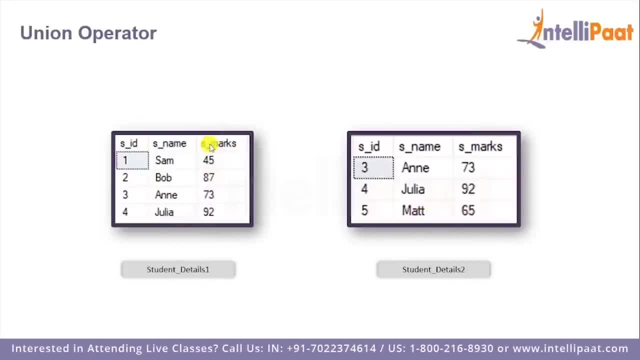 two tables. so we have the student details: one table which has the columns s ID s name and s marks and has these four records. the other table is student details two, which has the same columns and comprises of these three records. so let's go to SQL server and work with a union operator, right? so we have our two. 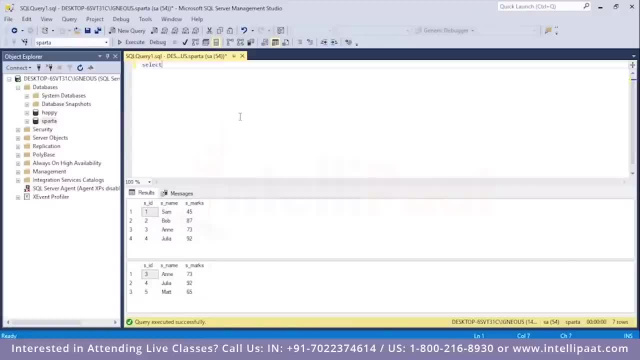 tables right in front of us. so let me start with the syntax. I'll get the first select query- select start from- and then I'll give the name of the table, which is student details one. after that I'll give the union operator and then give the next select statement- select start from, and then the name of the table is: 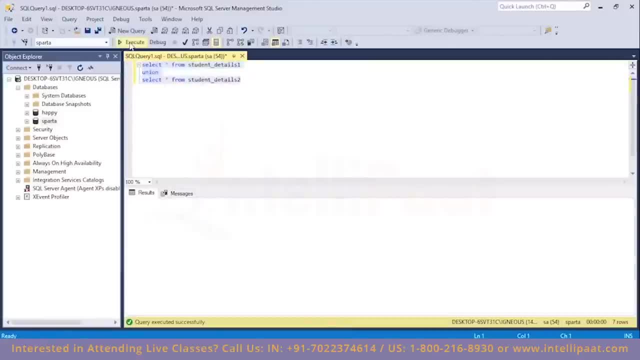 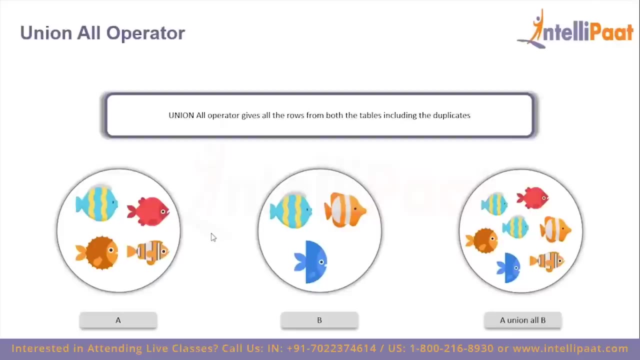 student details. two: I'll select all of this. I'll hit execute. so the union operator has given us the result set of both of the select statements. then we have the union all operator. the union all operator gives all the rows from both the tables, including the duplicates as well. so here, since the blue fish is present in both, 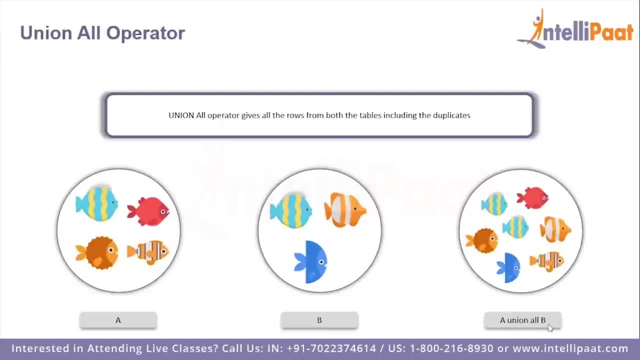 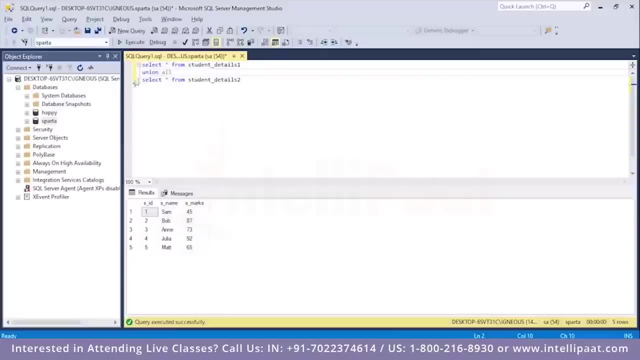 the tables a and B. the final result of a union: all B will also have the duplicate value. so now let me just add the all keyword over here. so I am using the union all operator between these two tables. now I'll hit execute so we see that we also have the duplicate values. so here these records. 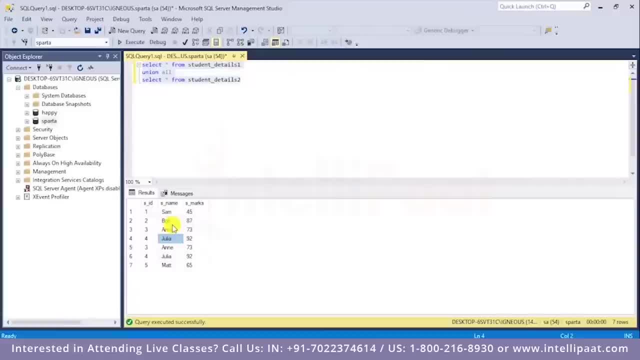 were an and Julia are present. these are from the first table and again here and in Julia. so these two cards are from the second table. so we have also got the duplicate record this time because we've used the union all operator. now again, let me remove this all keyword. let me hit execute so see that there are no. 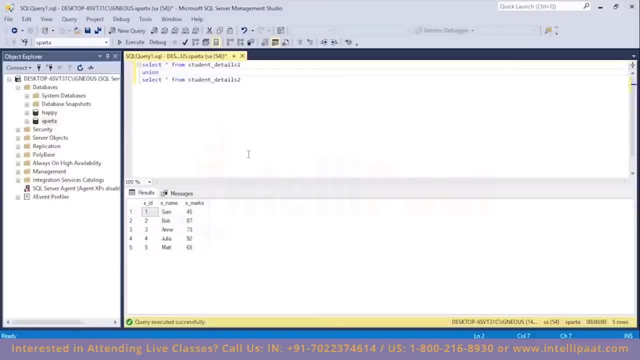 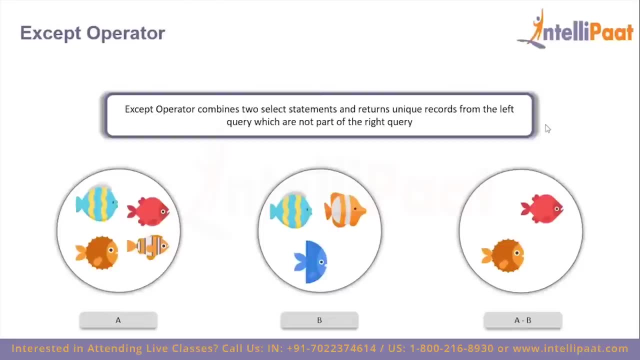 duplicates time. So this is a difference between union and union all operators. So this is how we can work with the union and union all operators. So the except operator combines two select statements and returns unique records from the left query which are not part of the right query. For example, 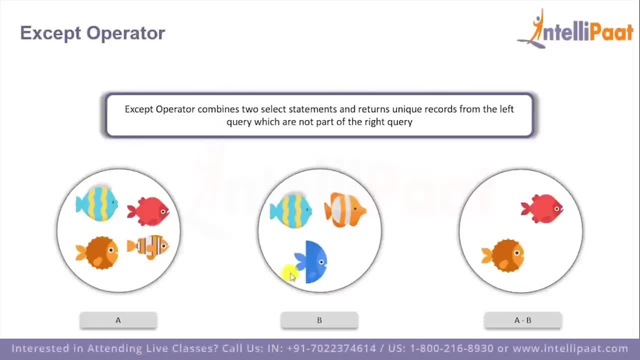 if the first select statement returns these four fish and the second select statement returns these three fish, then the except operator would return us these two fish, which were part of the first select statement, but not the second select statement. And this is the syntax of the except. 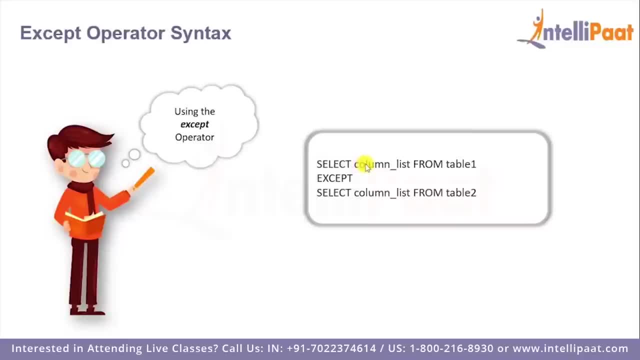 operator, We'll give the first select statement. after that, we'll give the except operator, following which we'll give the second select statement. Now you also need to keep in mind that the number and order of columns must be same in both the select queries, And we'll be implementing the except. 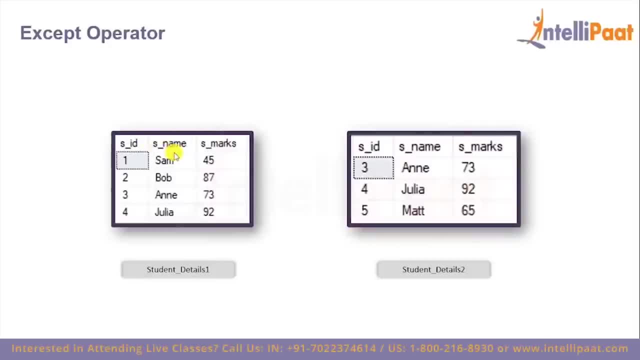 operator on these two tables. So we have the student details, one table which has the columns s id, s name and s marks and has these four records, and the other table is student details 2, which has the same columns and comprises of these three records. So let's go to SQL server and work with the except operator, Right, so we? 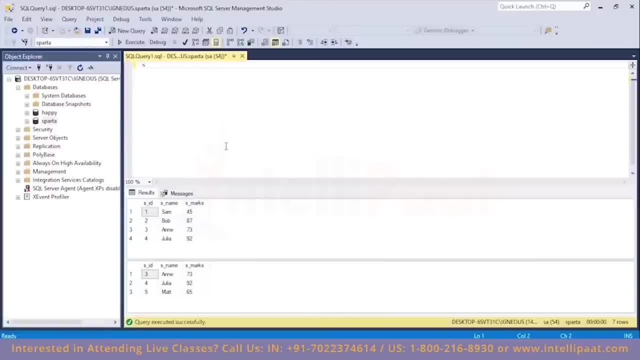 have our two tables right in front of us. So let me type in the syntax. I will give the first select query, which is select, start from, and then I'll give in the name of the table, which is student details one. After that I will use the except operator and then give in the second. 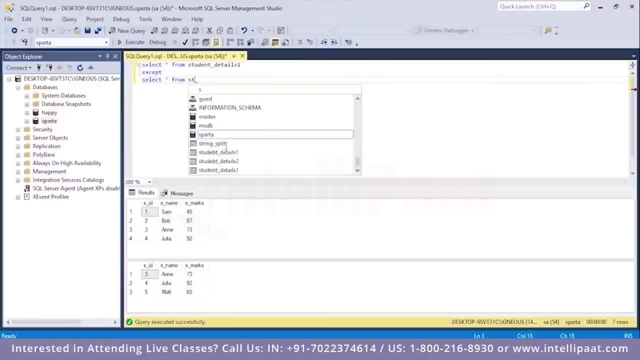 select statement which is student details one. And then I'll give in the second select statement, Select start from the name of the table as student details two. I'll select all of this again, I'll hit execute. So this is the result of the except operator. So these are the two. 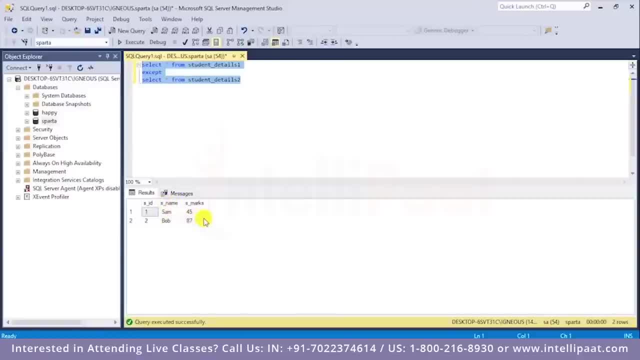 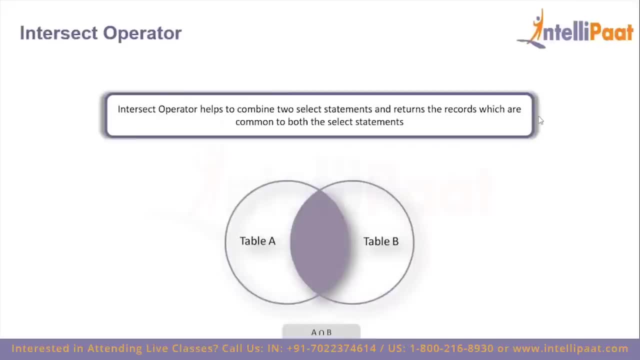 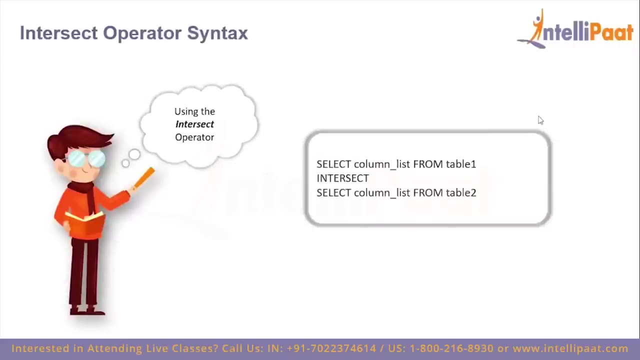 records which were part of the first select statement but not the second select statement, And this is how we can work with the except operator. So the intersect operator helps to combine two select statements and returns only those records which are common to both the select statements. And this is the syntax for the intersect operator. We'll give the first select. 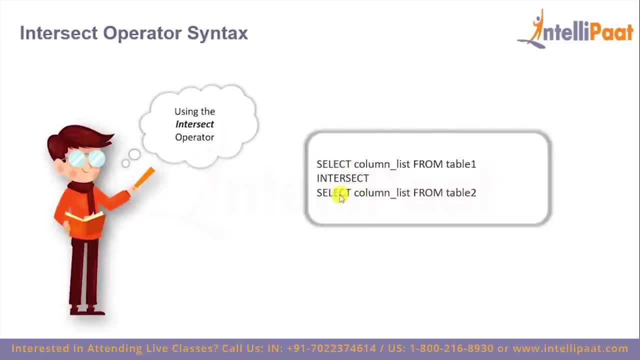 statement, After which we'll give the intersect operator, Following which we'll give the second select statement. So this intersect operator basically retrieves the common records from both the left and right side of the intersect operator. Now you also need to keep in mind that the number 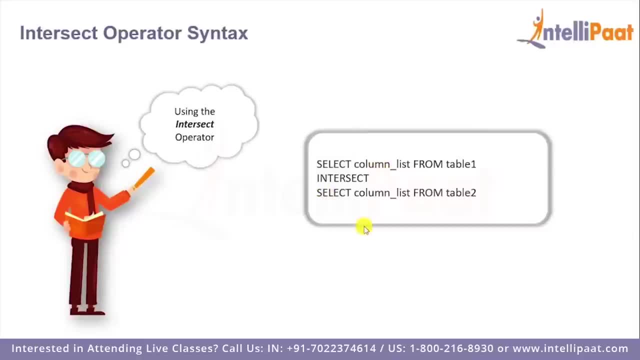 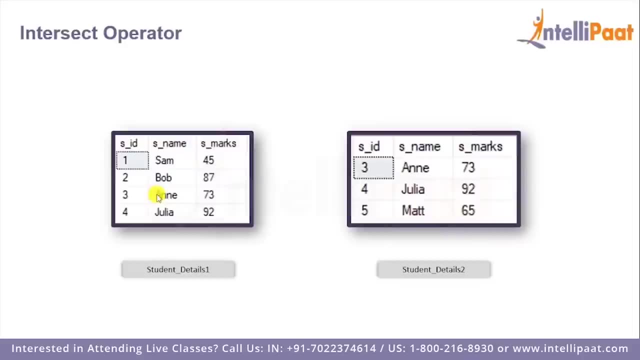 and the order of the columns must be same in both the select queries And we'll be implementing the intersect operator on these two tables. So we have the student details, one table which has the columns s ID s name and s marks and has 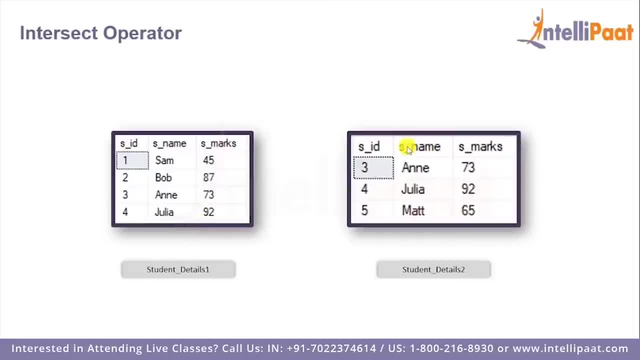 four records. The other table is student details two, which has the same columns and comprises of three records. So let's go to SQL Server and work with intersect operator. So these are our two tables over here. This is the student details one table and this is the student details two. 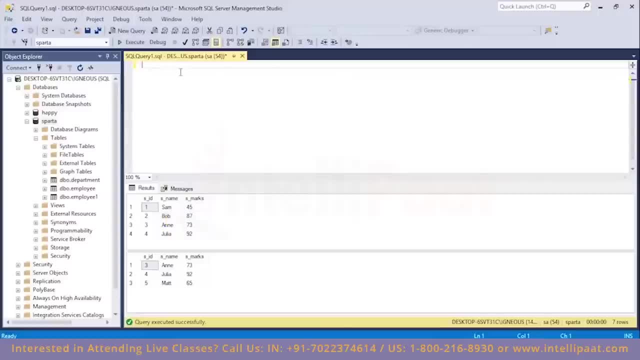 table. Now let me implement the intersect operator on these two tables. So I will give the keyword select, star from, and then give the name of the table, which would be student details one. After that I will give the intersect operator Intersect, and then give the second select. 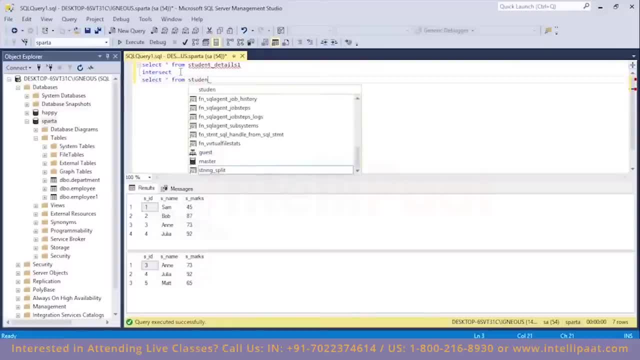 statement: Select star from student details. two Right guys. so this is pretty much the syntax. So we'll give the first select statement, After that we'll give the intersect operator and then we'll give the second select statement. Now let me select. 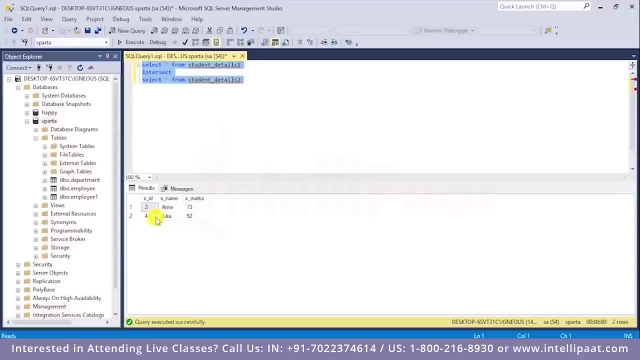 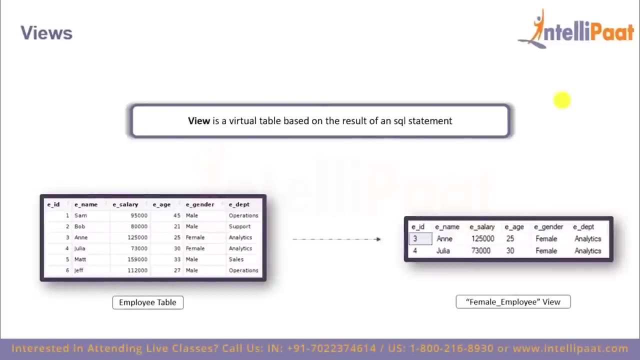 all of this, Let me hit execute. So these are the two records which are common to both the student details- one table- and also the student details- two table. And this is how we can work with the intersect operator. So views are virtual tables which are used to limit the information that you 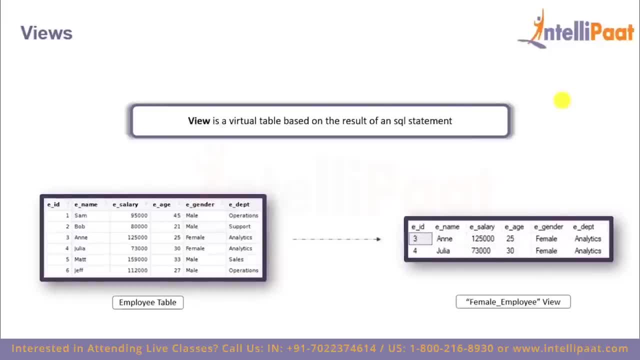 want to display- And these are actually nothing but the result of an SQL statement- which have a name associated with it, For example, from this employee table. let's say we wanted to perform multiple operations on the records where the gender is female, So we can create a view for only the female employees from. 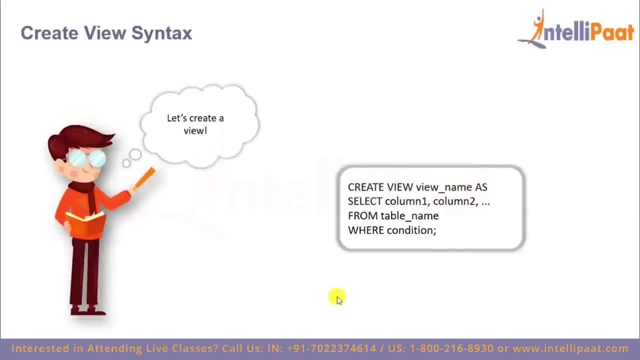 the entire employee table. So let's have a look at the syntax to create a view. We'll start off by using the keywords create view, then give the name of the view, After which we'll give the keyword as and then give the list of the columns which you want to select from the table. So let's 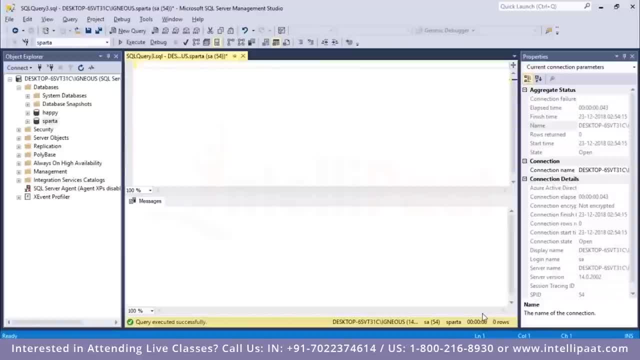 see create a view from our employee table. So I don't create a view which would comprise of only the female employees from the entire employee table. So this would be the command for that Create view. then I'll give the name of the view, which would be female employees. After that I will. 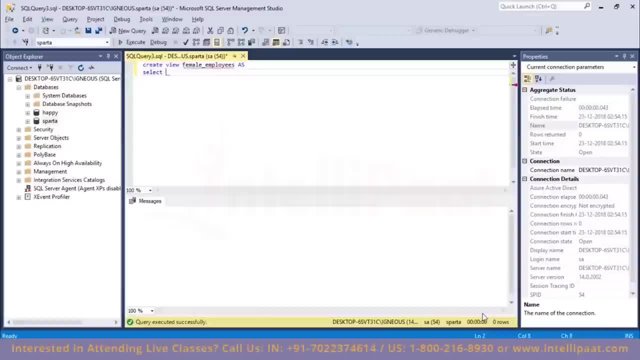 give in the keyword as and I will select all of the columns from the employee table. So select star from employee using the where clause. I will give in the condition. So the condition would be: e gender is equal to female. So I'll put a semicolon over here. I'll hit execute. So you see that commands have. 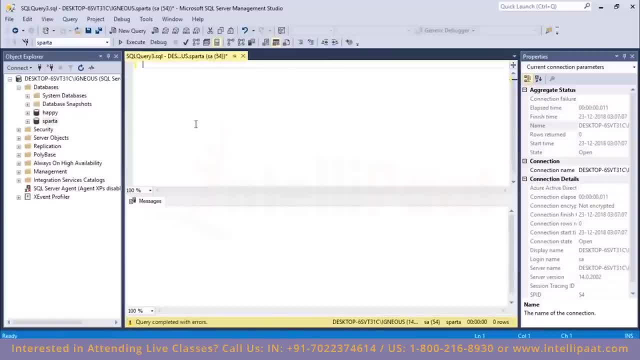 been completed successfully. So now let me have a glance at the female employees view. Select star from, I'll give the name of the view, which would be female employees. I'll put a semicolon, hit execute Right. So we see that we have successfully created a view from the employee table And in this view, 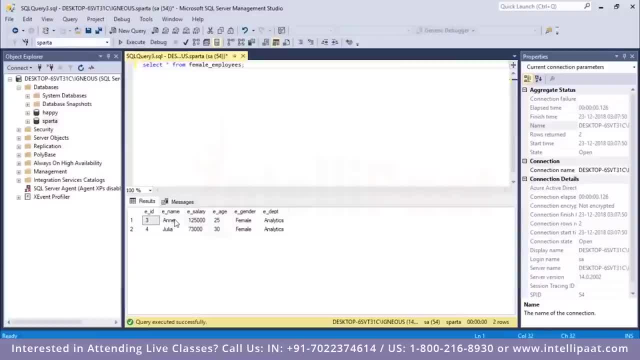 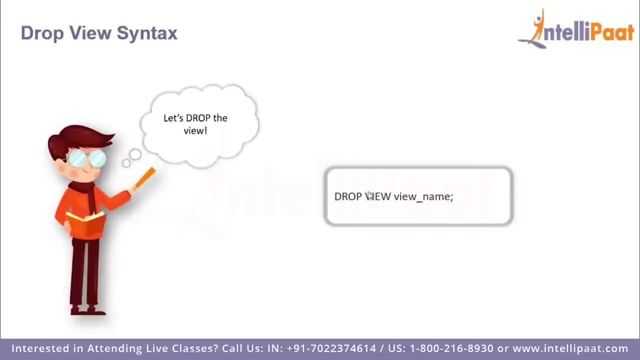 we have only two records, which comprise of the employees, and and Julia, and both of them are obviously female. Now let's see how can we drop a view. So the syntax for dropping a view is pretty simple. All we have to do is give the keywords drop view and then give the name of the view. 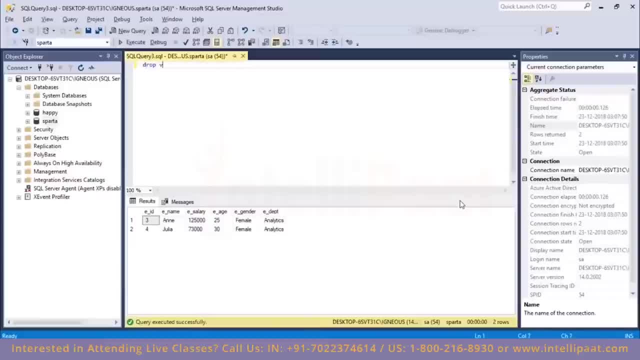 So let me drop this female employees view. I will type in drop view And then I will give in the name of the view, which is female employees. I'll put a semicolon: execute. So again, commands have been completed successfully. So now let me see if the view exists or not. Select star from female. 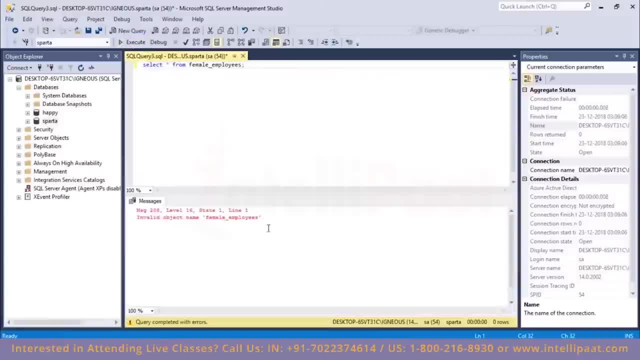 employees execute And this is the result which we get: invalid object named female employees And we get this. the view female employees has been dropped, so this is how we can work with views. so the alter table statement is used to add, delete and modify columns in. an existing table. now let's have a look at the syntax to add column to an existing table. so we'll start off by giving the keywords alter table, then we'll give the name of the table. after that we'll give the add keyword and the name of the column which you want to add to our table and finally we have to. 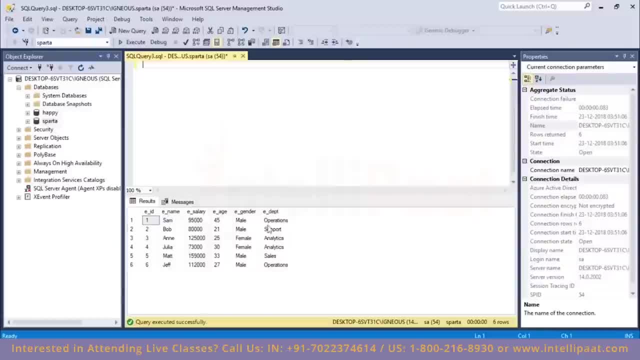 assign a data type to this new column. so to our existing employee table I'll add a new column, date of birth, using the alter table statement. so let me start with the syntax alter table. then I'll give the name of the table, which would be employee. after that I will give in the add keyword and then given the name. 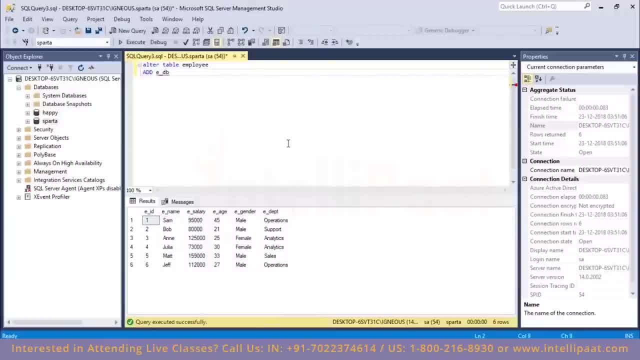 of the column. so I'll name the new column to be E, DOB, which would stand for employee date of birth, and then I'll finally give the data type of the new column. so the data type would be date. so I'll put a semicolon, I'll hit. 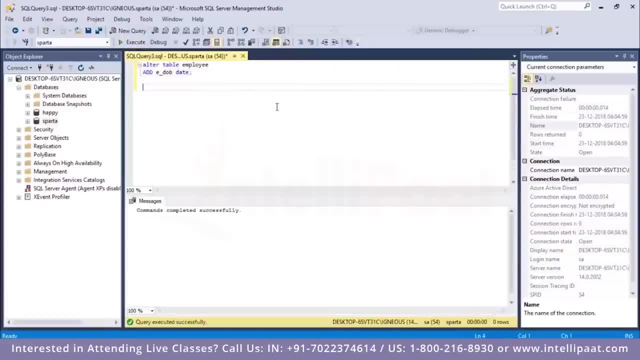 execute. so commands have been completed successfully. now let me have a glance at the modified table. select star from employee right. right, so we see that this new column employee date of birth has been added. so you see that this new column employee date of birth has been added to. 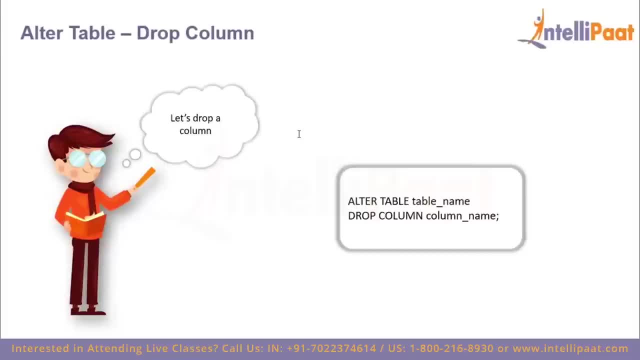 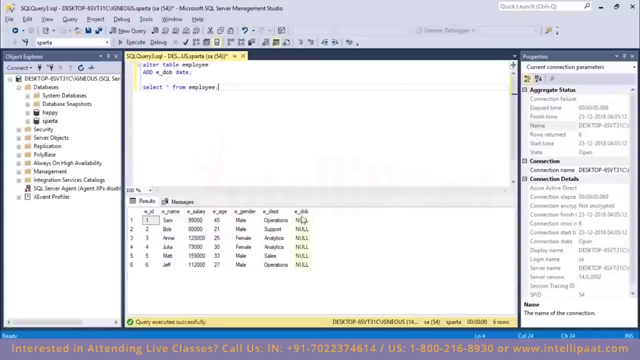 our employee table. now let's see how can we drop a column from a table. again, we'll start by giving the keywords alter table and then we'll give the table name. after that we'll give the keywords drop column and specify the name of the column which is to be dropped. so I want to drop this new column which I have. 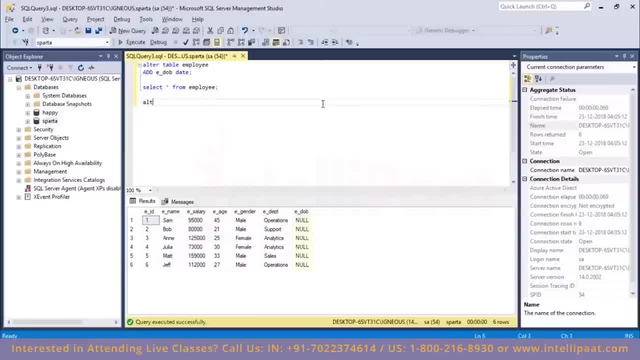 just added to this employee table, so let me write the command for that. so I want to drop this new column, E DOB, which I've just added to this employee table, so let me write the command for that: alter, alter table, and then the name of the table is employee- alter table, and then the name of the table is employee. 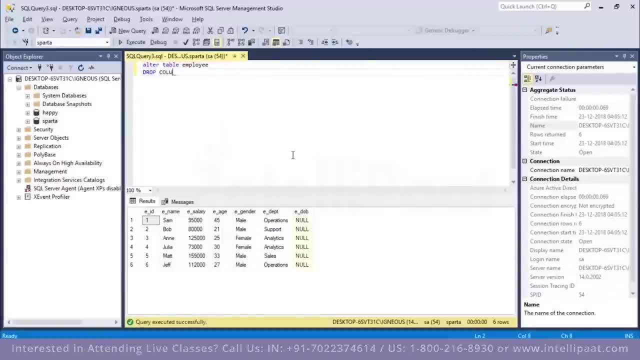 after that I will give in the keywords: drop column and I want to drop the E DOB from this employee database. I'll put a semicolon, hit execute. so again. the commands have been successfully executed. now let me have a glance at the modified table. select star from employee. I'll put a semicolon execute. so again the new. 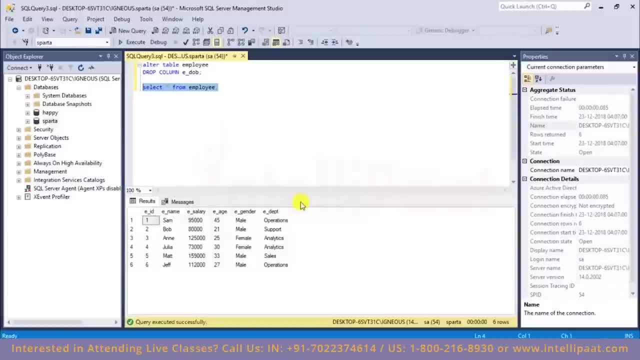 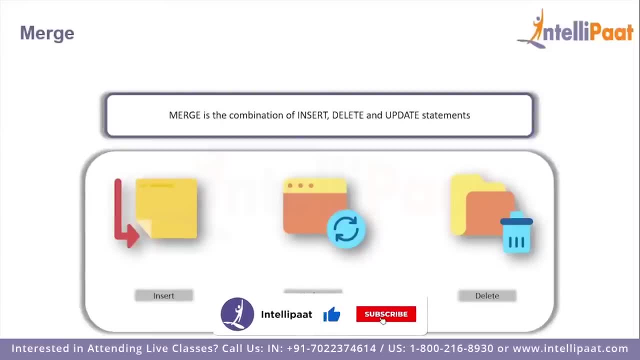 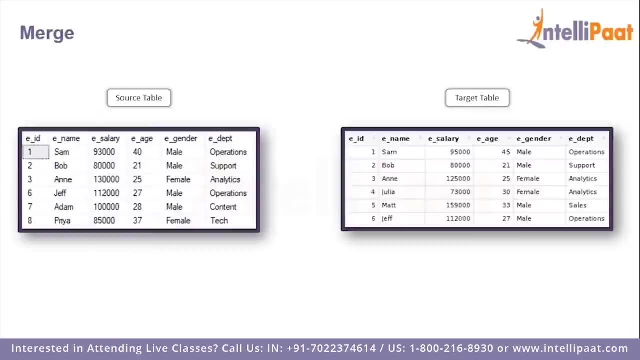 column which you had just added has been dropped, so this is how we can work with the alter table statement. so the merge statement helps us to perform insert, update and delete in just one statement. this means we no longer require multiple statements to perform insert, update and delete, and for the March statement we 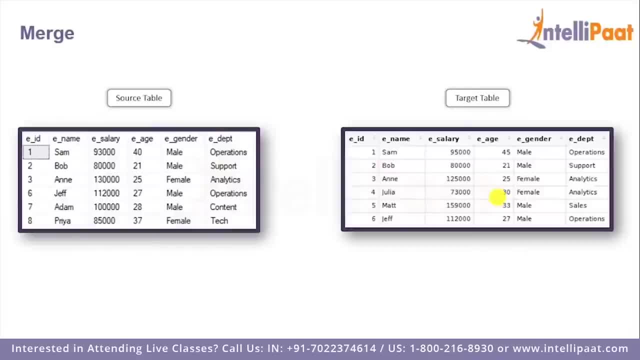 require two tables: a source table and a target table. so the source table basically contains all the changes which are to be applied to the target table and the target table as that table upon which will be implementing all the changes. now, the mode statement basically joins the target table to the source. 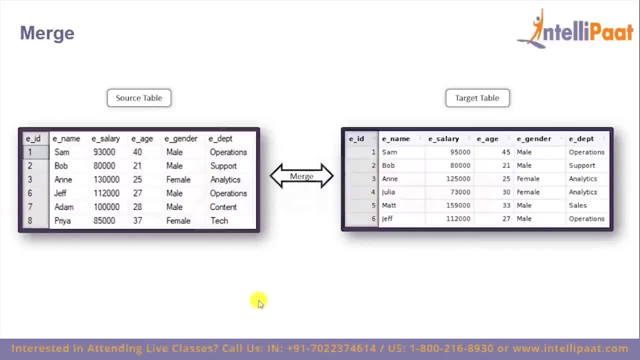 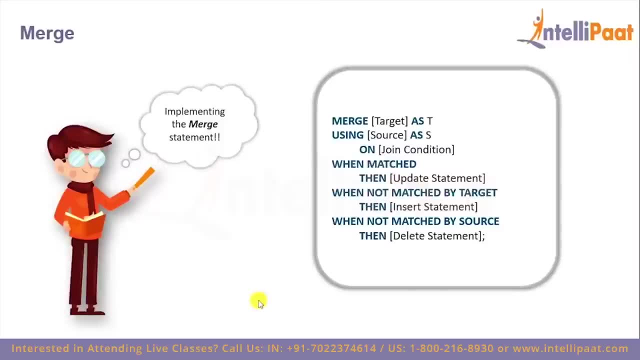 table. using a common common course in both the tables and based on how the rows match up, we can perform insert, delete and update operations on the target table. Now let's have a look at the syntax of the merge statement. So we'll start with the merge keyword and 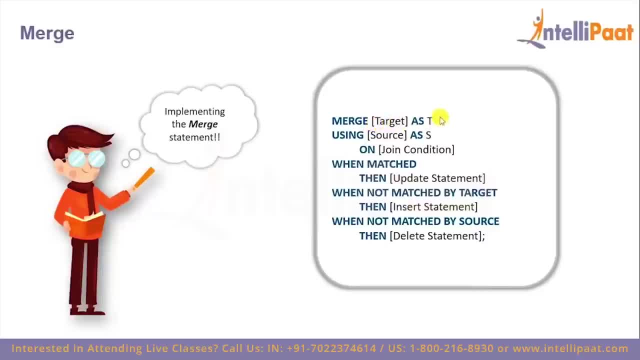 then give the name of the target table and assign it an alias using the as keyword. Then we'll type using and give the name of the source table and also assign it an alias using the as keyword. again After that we'll type on and then 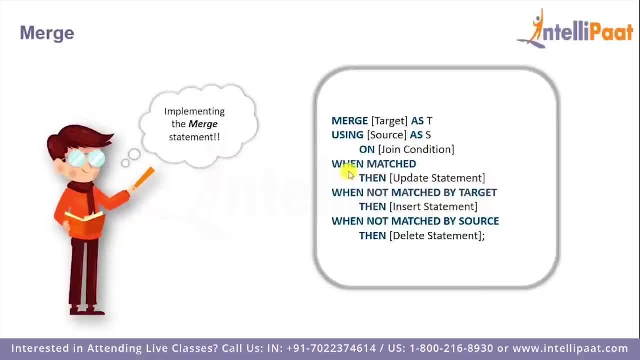 set the join condition, Then we'll type when matched. So if the rows match up based on the join condition, then we'll go ahead and update the target table. After that we check when not matched by target. So this basically means that if there are some rows which are present in the source table but not in the target, 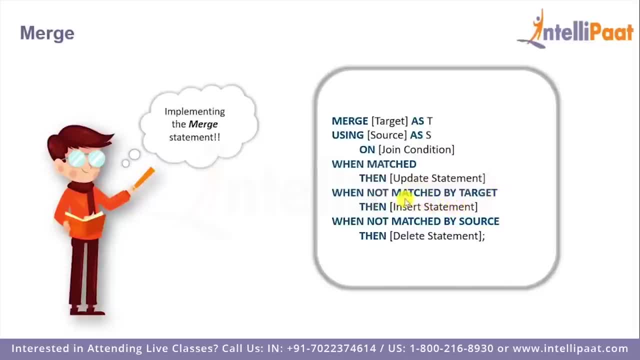 table, then we'll go ahead and insert those rows from the source table into the target table And finally we'll type when matched. So if the rows match up based on the, finally we check when not matched by source. So here we are checking if there. 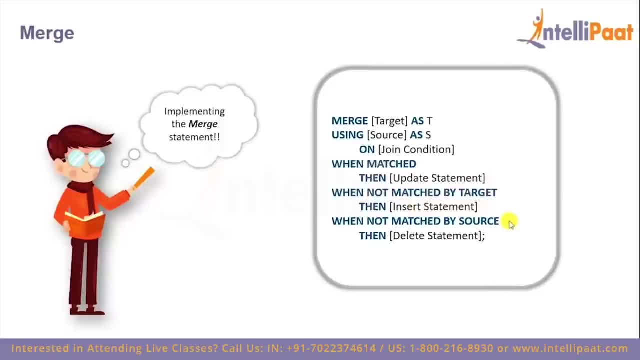 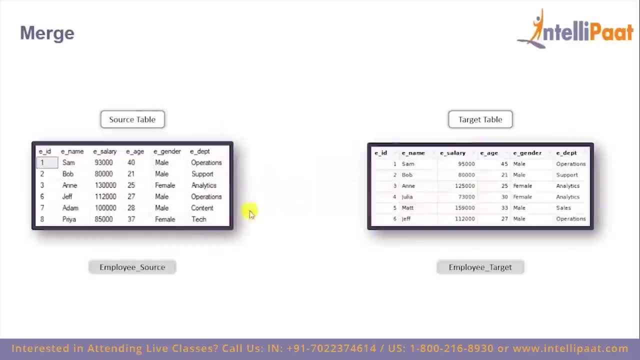 are some rows which are present in the target table but not in the source table, Then we'll go ahead and delete those rows from the target table And for the practical purpose we'll be using these two tables. So this is our source table with the name employee source and this is our target table with the name. 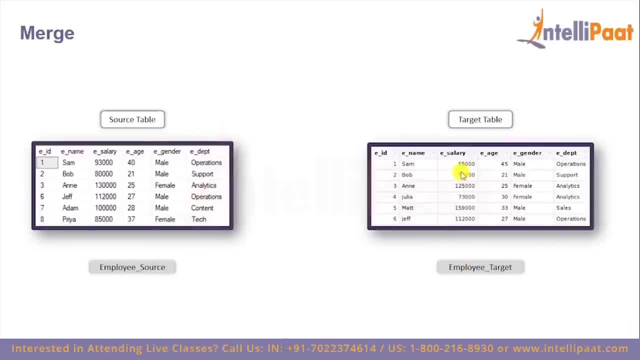 employee target. So, using the merge statement, we'll be updating the e salary and eh columns in the target table wherever there's a match. Also, insert the records with employee ID 7 and employee ID 8 into the target table from the source table and delete the records with. 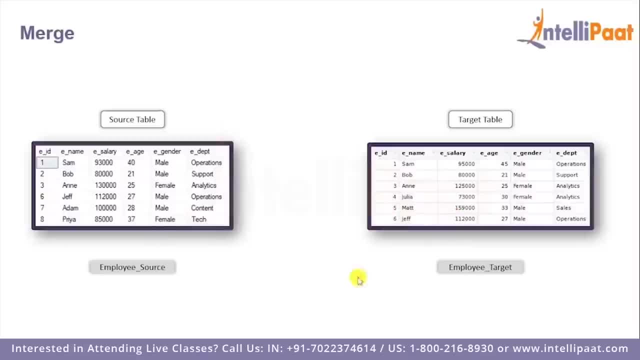 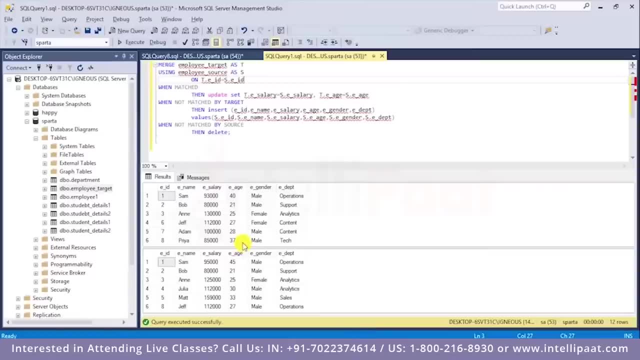 employee ID 4 and employee ID 5 from the target table, because they're not present in the source table. So let's go to SQL server and work with a merge statement, Right? so we have our two tables right in front of us. This is the 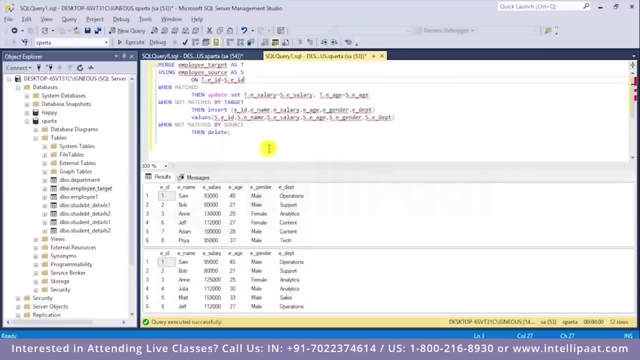 employee source table and this is the employee target table, and we also have the merge syntax to apply on these two tables. So we'll type merge and then give the name of the target table- employee target. we'll assign it an alias t. Similarly, we'll give the employee source table and. 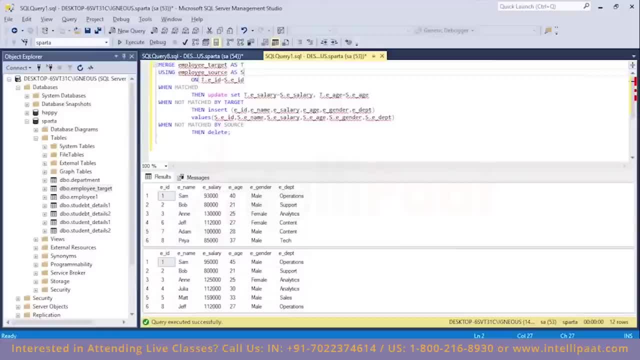 then assign it an alias s. After that we'll type on and then set the join condition. So the join condition is: teid is equal to seid. So we basically set the join condition on the employee ID columns of the source table and the target table. 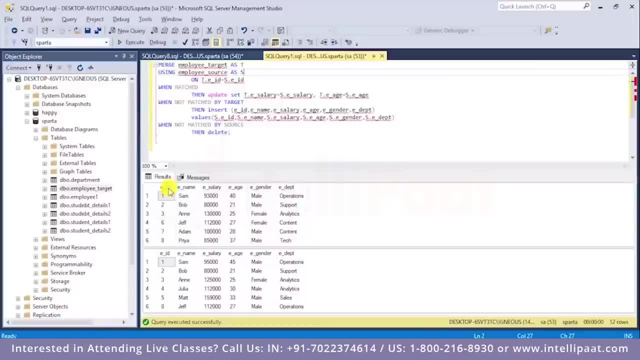 malfield, Then we have when matched, so there is a match between the rows of these two tables, then we'll go ahead and update the target table. So here in the update statement we have: te salary equals se salary and teh is equal to S dot. eh, so if the records match, then I'll be setting the values of: 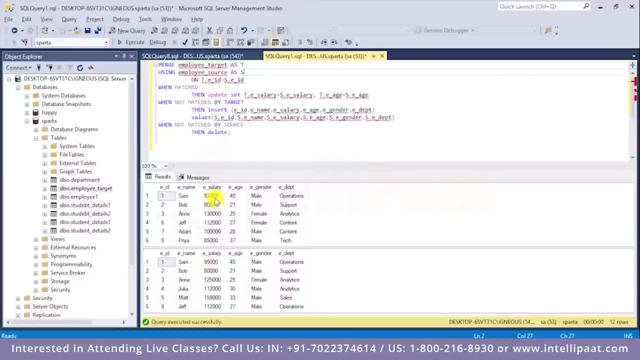 the salary column of the target table to be T & E values of the salary column of the source table. Similarly, I'll also set the values of the age column of the target table to be equal to the values of the age column of the source table. and then we have when not matched by target. So here we. 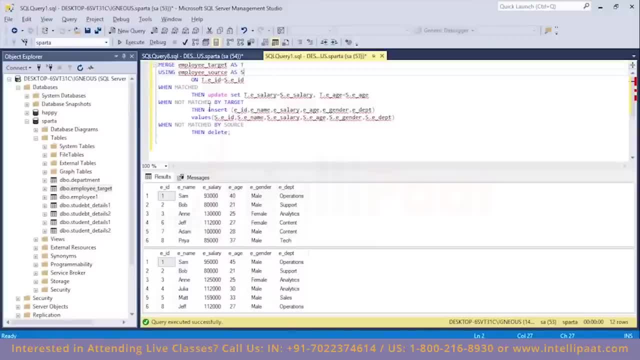 are checking if there are some rows which are present in the source table but not in the target table, and if that is the case, we'll go ahead and insert all of those into these columns of the target table and the values would be coming from the source table. So this employee ID column from the target table. 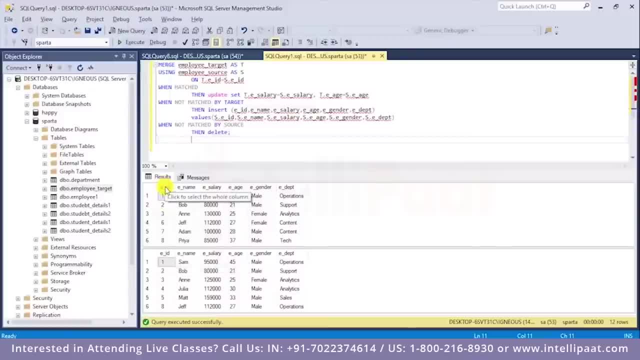 would be getting the values from the employee ID column of this source table. Similarly, this employee name column of the target table would be getting its values from the employee name column of this source table. and finally, we'll check when not matched by source. So if there are some rows which 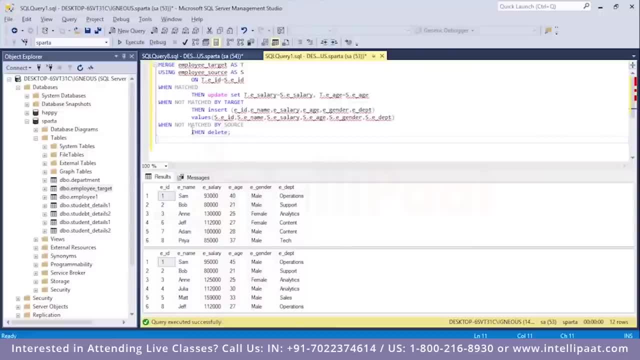 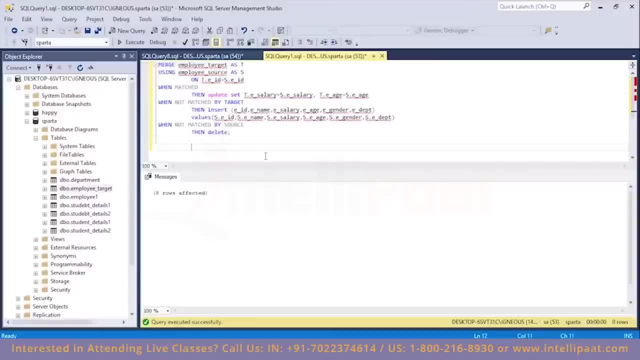 are present in the target table. we can even strengthen them to this one to make it present in the target table but not present in the source table. then we'll just delete all of those rows. So I'll select all of this and I'll click on execute. So you see that eight rows have. 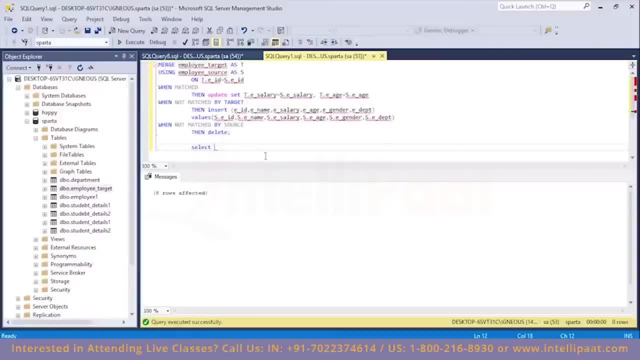 been affected. Now let me type the select statement and have a glance at the modified employee target table. Select star from employee target. I'll select this. I'll click on execute Right. so this is our modified employee target table. So we also have our original employee target table over here. 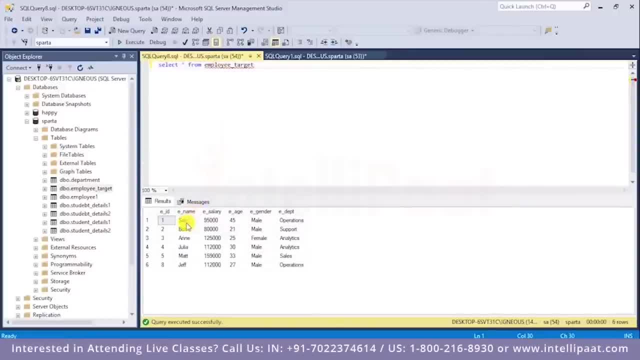 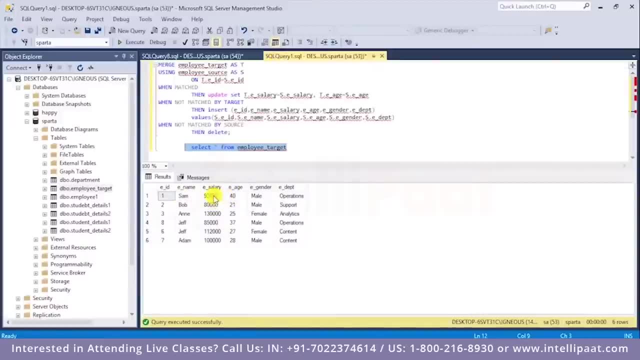 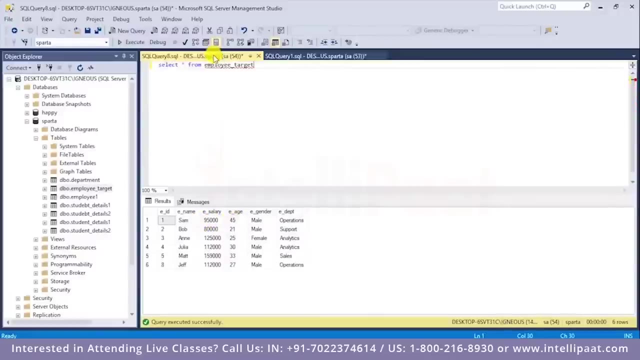 So let me compare these two tables. So we see that initially, Sam's salary was $95,000 and his age was 45, and after applying the merge statement, his salary changed to $93,000 and his age changed from 45 to 40.. Similarly, Ann's initial salary was $125,000 and after applying the merge, 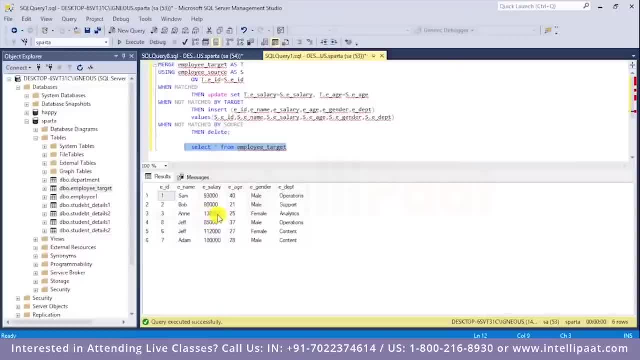 statement his salary changed to $195,000 and his age changed from 45 to 40. So we see that statement. her salary changed to $130,000.. And then, with the merge statement, we have also inserted the records with employee ID 7 and employee ID 8 and deleted these two records. 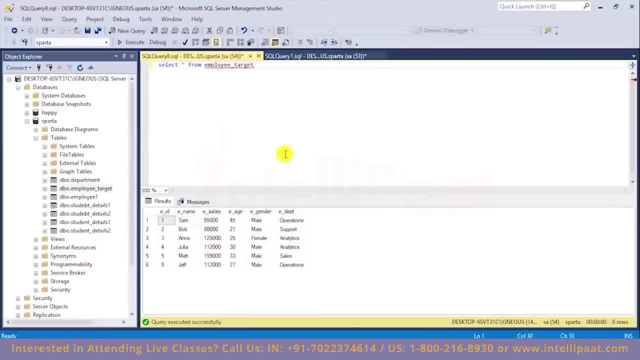 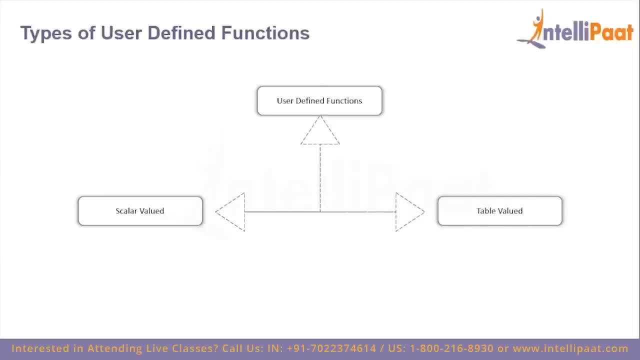 from the employee target table. So this is how we can work with a merge statement. So these are the two types of user defined functions. in SQL We have scalar valued functions and table valued functions. We'll start with the scalar valued functions. So, as the name states, a scalar. 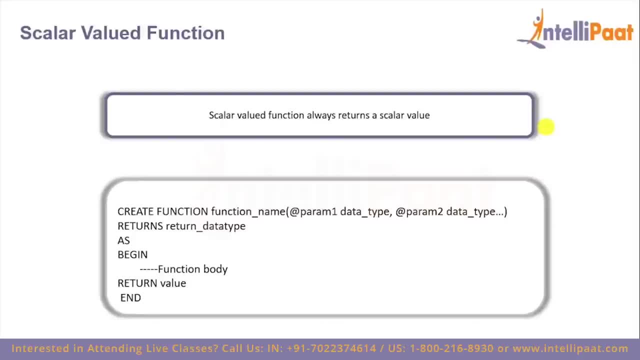 valued function always returns a scalar value. So a scalar value could be int, varcat, date and so on, And this is the syntax for a scalar valued function. So we'll type create function and then we'll give the function name And inside the parenthesis we'll specify the names of the. 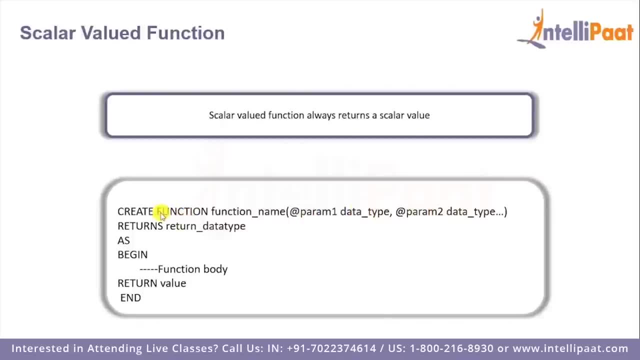 parameters and their data types. And since the function is going to return a value, we'll give it a name. And since the function is going to return a value, we'll give it a name. We'll type the returns keyword and specify the type of data which will be returned After that. 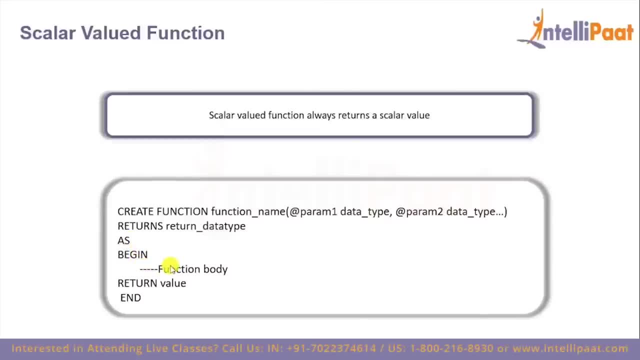 we'll type as begin and then give the function body and then return the final scalar value. Finally, we'll use the end keyword to end the function. So let's go to SQL server and create our first scalar valued function. So I'm going to create a scalar valued function which will take 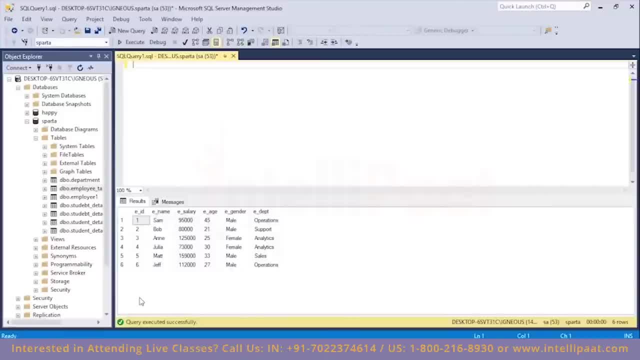 one integer value, add five more to the original value and return the updated value. So let me type the syntax for that Create function and then I'll give the function name, which would be add five, And inside the parenthesis I'll pass the first parameter. So I'll name the parameter to. 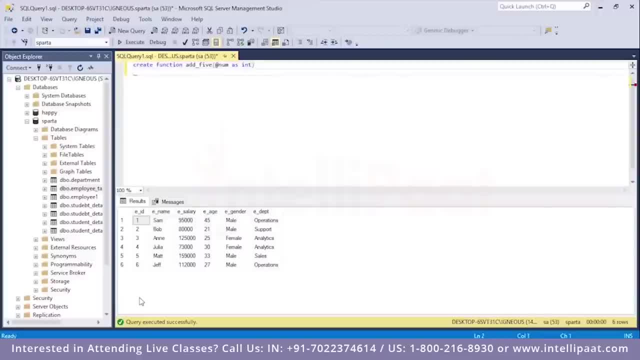 be num, And this would be of integer type. After that, I'll type the returns keyword, And then the type of data which will be returning is also of integer type. After that, I'll type as begin, and since all we have to do is add five more to the original value, so I'll not write anything. 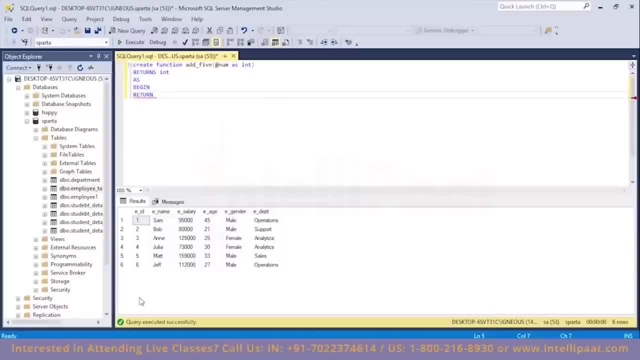 inside this. So I'll directly type the return keyword And inside this return keyword I will add five more to the parameter value. So that would be at the rate num plus five. So what we are basically doing over here is the value which is sent as parameter inside this function. we'll. 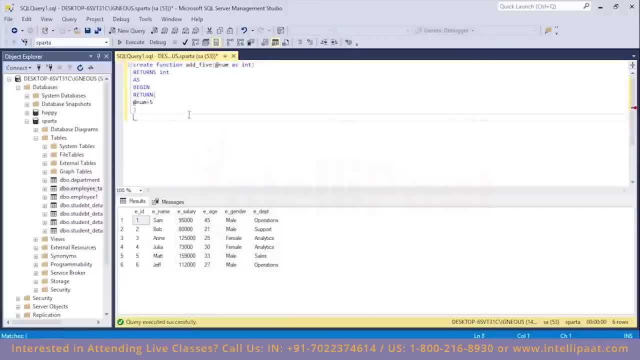 add five more to that value and then return it, And finally I'll type the n keyword to end this function. So let me hit execute. Right, so we have successfully created this add five function. Now let me go ahead and call this function. So to call the function, I'll type select And then I'll have 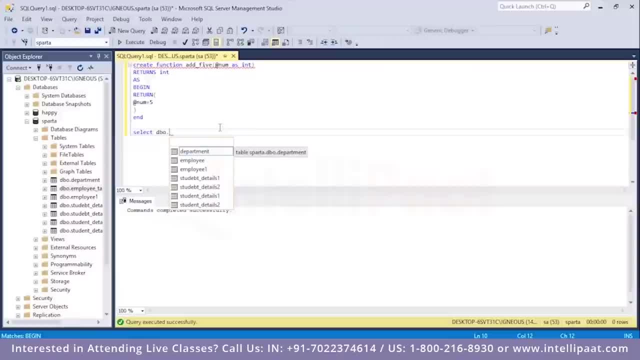 to type dbo dot, And then I'd have to give the function name, which is add five. Now let's say I'll hit execute Right, so we see that this function works properly. So I've sent 10.. And the 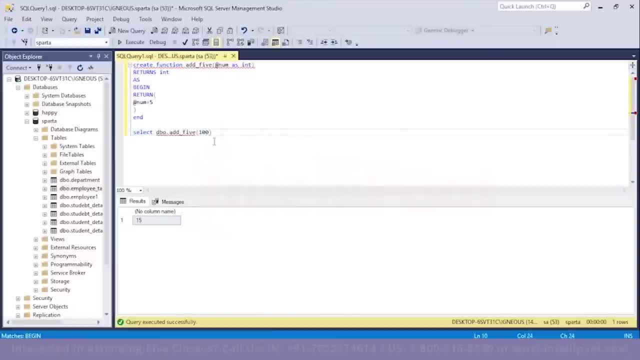 result which you've got is 15.. Similarly, let me send 100 as the parameter. Now I'll select, I'll hit execute Right. so the value which is returned is 105.. So this is how we can create a scalar valued function. Then we have table valued functions. So these table valued functions, 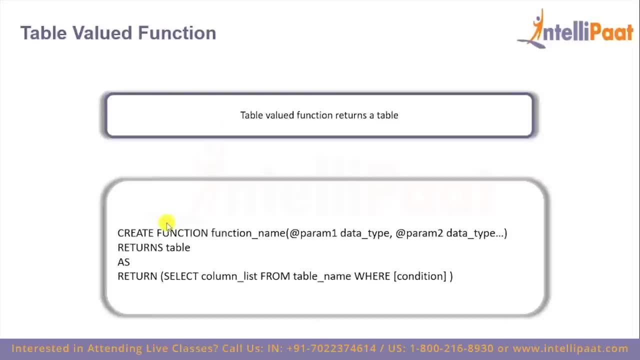 return a table instead of a scalar, And this is the syntax for a table valued function. So here the return type is stable. So after the returns keyword we'll type in table, because we're supposed to return a table. After that we'll give the keywords as return and then given the SELECT statement. Now you need to keep. 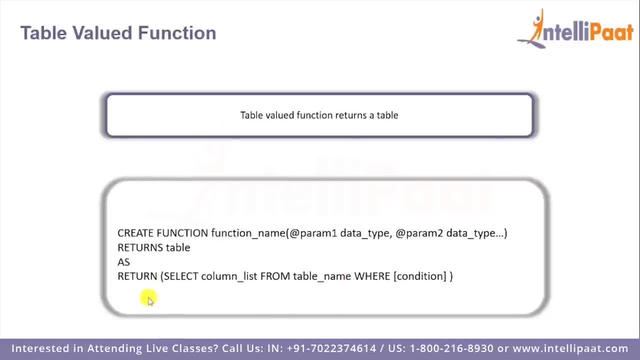 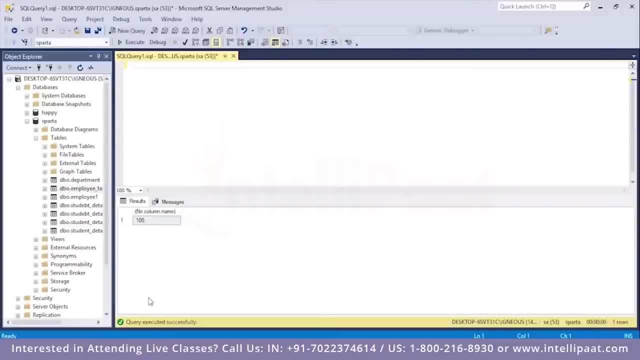 in mind that there are no begin and end keywords for a table valued function, So let's go to SQL server and create our first table valued function. Now I'll be creating a function which would help me to individually extract the male employees and the female employees from the employee table. So 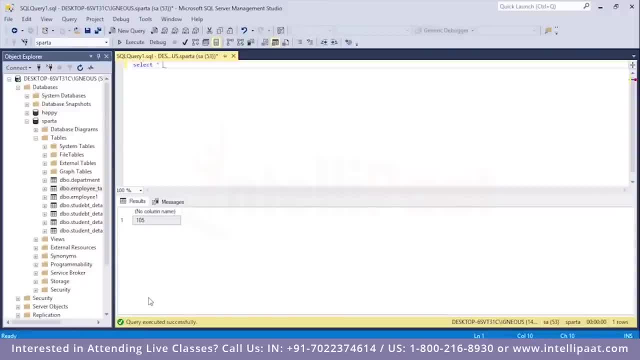 before I do that, let me actually have a good at the employee table first. so I'll type select star from employee right. so we have this employee table right in front of us. now let me go ahead and create the command. so again, I'll type create function and then I'll give the name of. 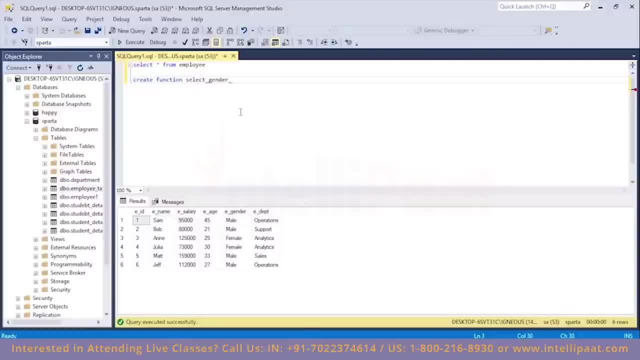 the function, which would be select gender. now, inside the parenthesis, I will pass in the parameter. so I'll name the parameter to be gender and this would be of varchar type, so as varchar, and the length would be 20. after that I'll give the returns keyword and, since this is a table valued function, the return type. 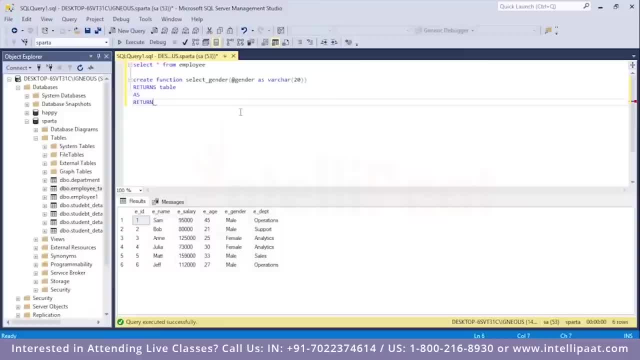 would be table. so I'll type as return and then given parenthesis, and inside the parenthesis I will give my select statement. so the select statement would go something like this: select star from employee where e gender is equal to, at the rate gender. so this e gender is basically the e gender. 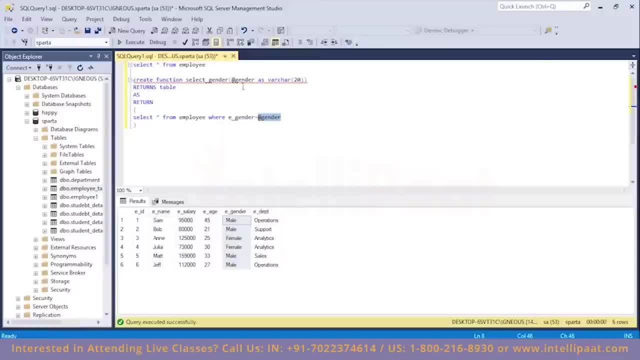 column from the employee table and this at the rate, gender is the parameter which will be passing inside this function. so let's say, if the user passes the value male inside this function, then we'll be extracting all of the records where the gender value is male. similarly, if the user passes the value female, 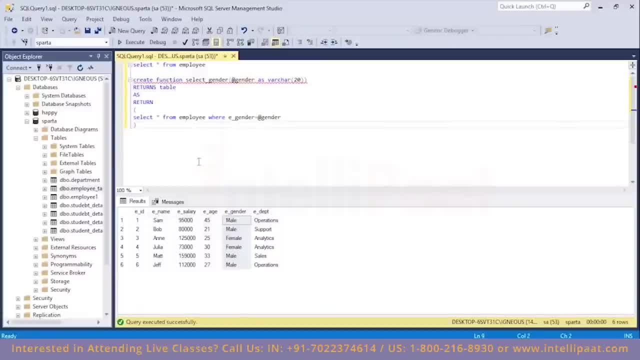 scale does a similar mistake. if the number of records of arandy is now being entered, we'll create the sement. let's now delete this. now we'll be extracting all the female employees from this table. so let me select this, let me hit execute right, so we have also created. 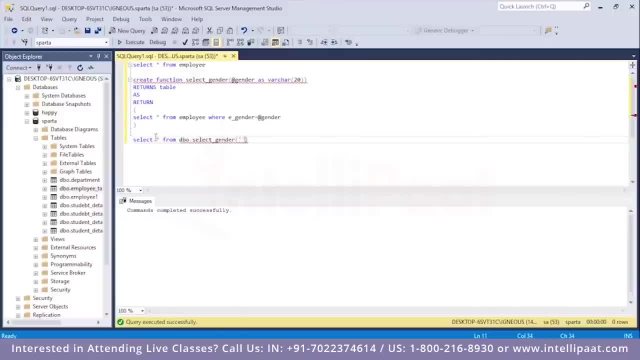 this select, dejend or dot, and then give the name of the function, which would be: And inside the parenthesis I will pass in the value And since I want all of the male employees, I'll type male over here, Right? So I'm typing select star from this, because this will basically return a table. 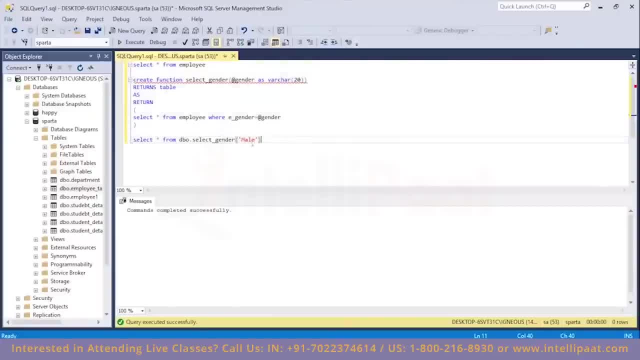 And from the table which is returned. I would want all of the records, So let me select this. I'll hit execute Right. So we have successfully extracted all of the male employees from the employee table. Similarly, if I'd have to extract all of the female employees, the syntax would be similar. 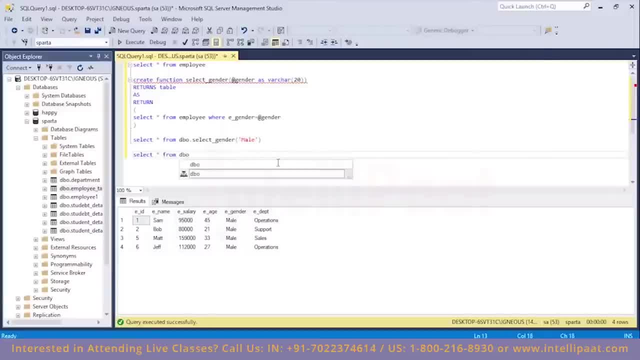 So I'll type select star from and then I'll type dbo dot select gender And then I will pass in the value female, I will select this, I'll hit execute. So again, we have successfully extracted the female employees from the employee table. 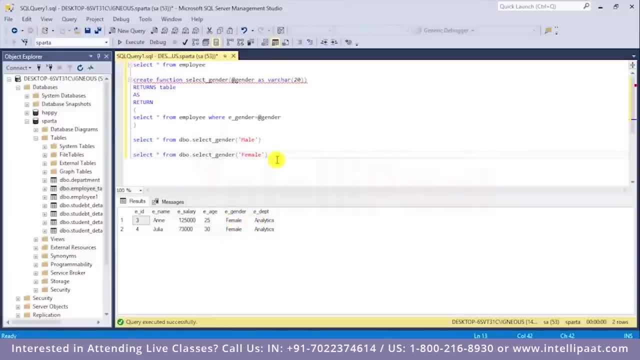 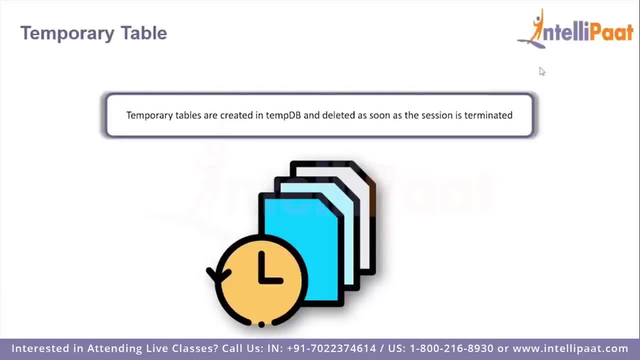 So this is how we can create table valued functions in SQL. So temporary tables basically help us to store and process intermediate results. Now these temporary tables are Created in the temp DB and are automatically deleted when they're no longer used. So the temporary tables could be very useful in cases wherever we need to store temporary data. 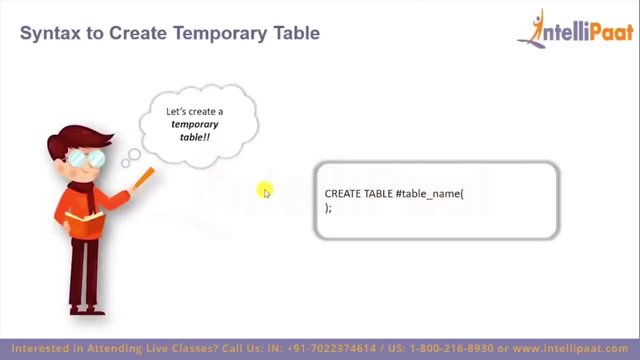 And this is the syntax to create a temporary table. So first we'll give the keywords create table And before we give the name of the temporary table we'll precede it with a hash. So this hash symbol basically signifies the table which we are creating is temporary. 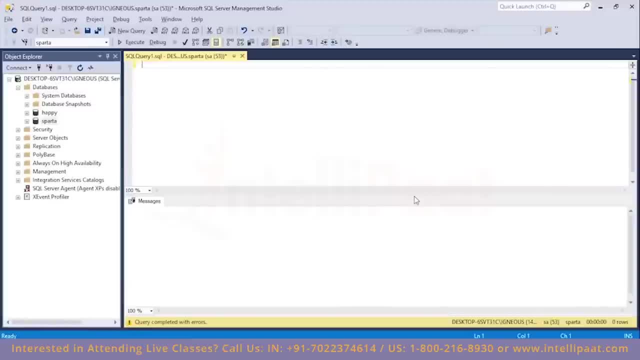 So let's work with some temporary tables Now. So let me create a temporary table with the name student, which has two columns: One is student ID, Another is a student name. So I'll type create table, I'll put in the hash symbol and then give the name of the temporary table, which would be student. 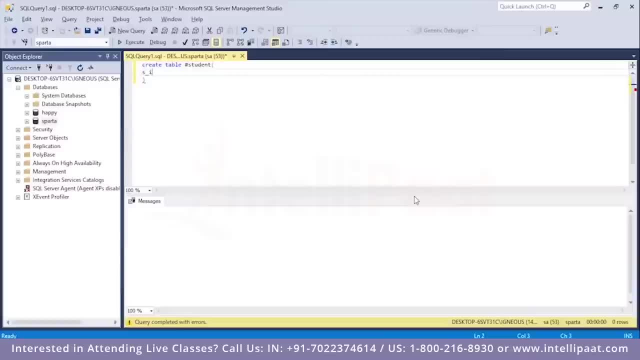 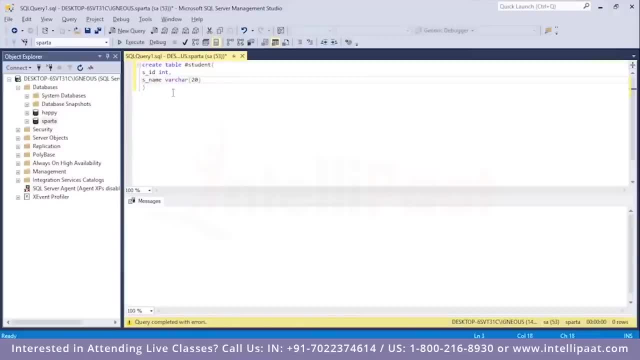 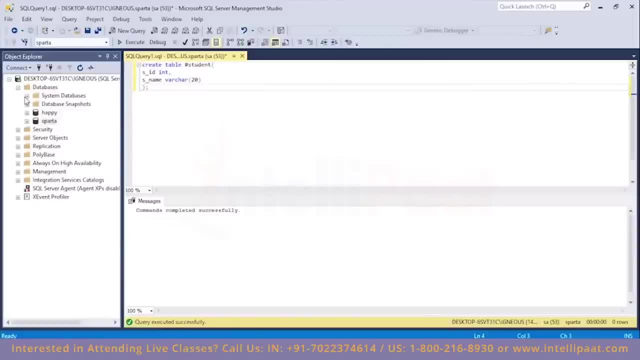 So let me show you guys where the temp DB is actually. So you'd have to click on the system databases And over here you'll see the temp DB, And inside temp DB you have all of the temporary tables. So let me refresh this. 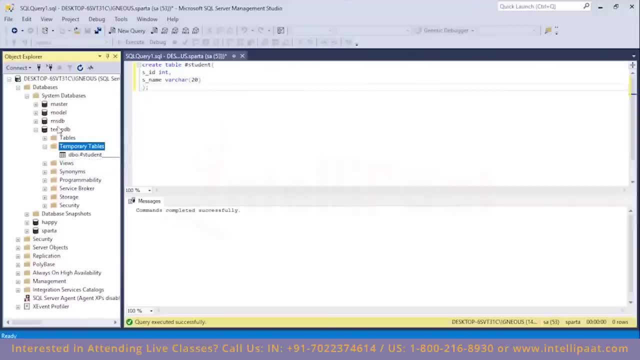 Right, So we see that we have this temporary. So we see that we have this temporary table- student- inside our temp DB database. Now, similarly, I can also use the select statement with this temporary table which I've created. So I'll type select, start from, and before giving the name of the table, I need to give the hash symbol and then give the table name, which would be student. 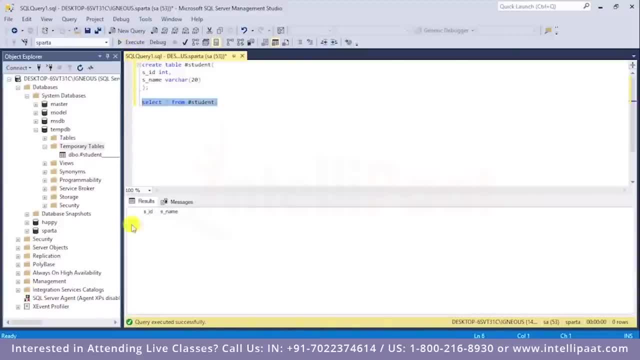 Right. So let me select this and I'll click on execute Right. So this is our table and we don't see any values because we haven't inserted any into this table. So, similarly, we can also use the insert command and insert some values into this temporary table. 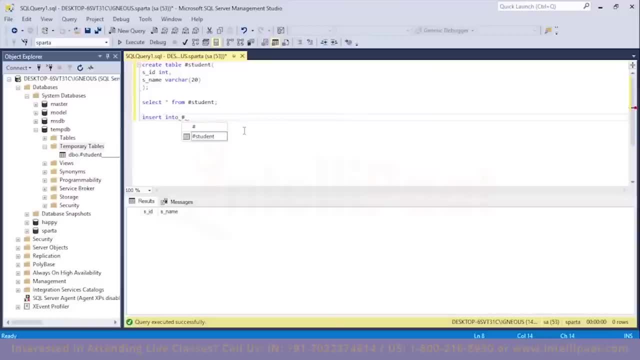 So I'll type insert into. after that, I'll give the hash symbol and then give the name of the temporary table, which would be student. I'll follow it up with the values keyword and then give the values which are to be inserted inside this. 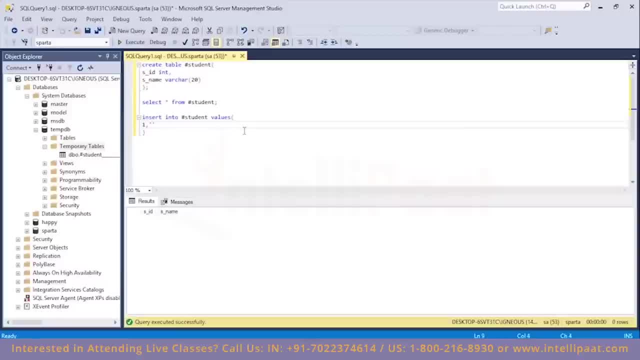 So first is student ID, which will be one, Then I'll give the name of the student. So name of the student is Sam. So again I will select this and I'll click on execute. So one row has been effected. Now I'll select this line again and I'll hit execute. 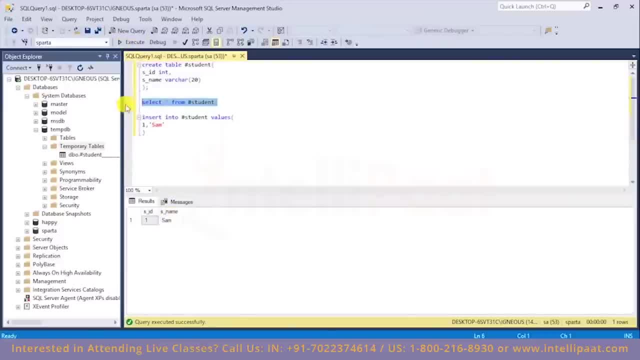 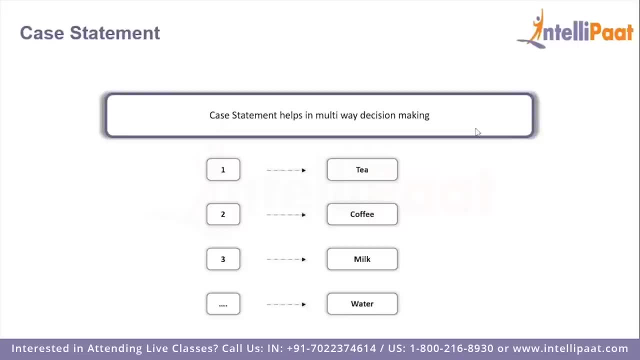 Right. So we have successfully inserted this record inside our temporary table student. So this is how we can work with temporary tables in SQL. So the SQL key statement helps us in multi-way decision making. So let's take this example to understand key statement properly. 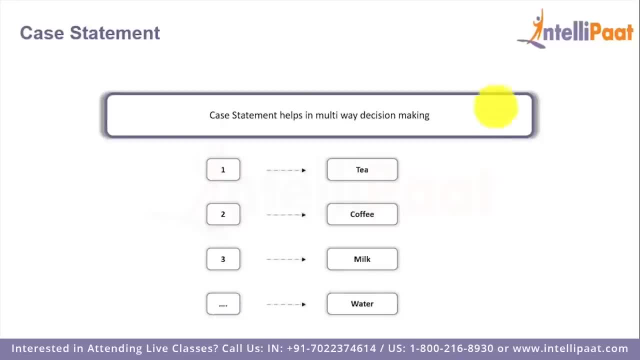 Let's say there are 10 buttons, starting from 1 to 10.. So if the person selects 1,, then he wants 2.. If he selects 2,, then he wants 3.. If he selects 4,, then he wants 5.. 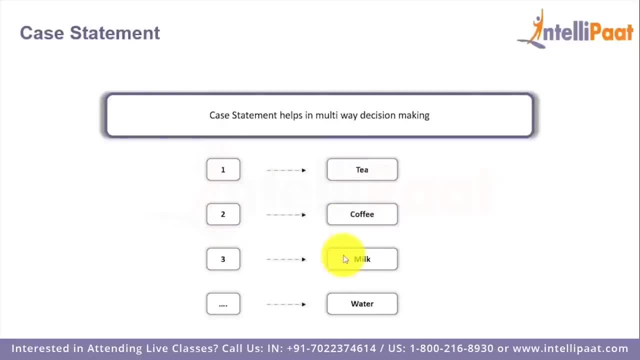 If he wants to order coffee. Similarly, if he selects 3, then he wants milk, And for any other case the person will order water. So this is basically how the key statement works. So the key statement goes through conditions and returns a value when the first condition is met. 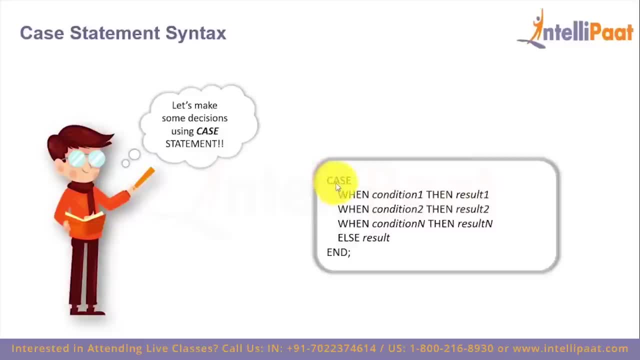 And this is the syntax for the key statement. So we'll type in case, following which we'll give the when keyword and give the first condition. After that we'll type then and specify what will happen if this condition is satisfied, And we'll do the same for the rest of the conditions. 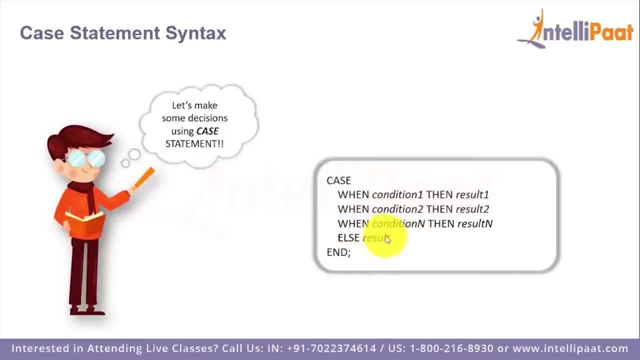 After that we'll type else and state what will happen if none of the above conditions are satisfied. Finally, we'll give the end keyword. So now let's go to SQL server and start working with the case statement. Just a quick info, guys. 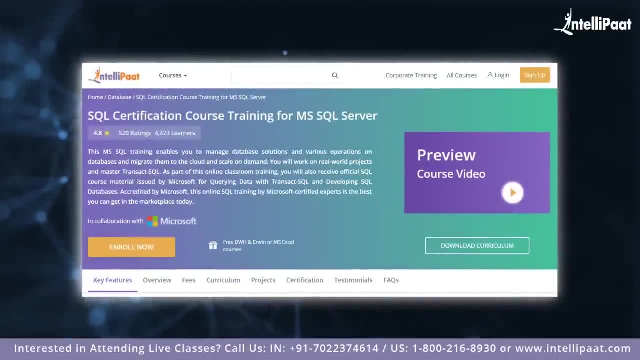 Intellipaat provides SQL online training in partnership with Microsoft and mentored by industry experts. The course link is given in the description below. Now let's continue with the session. So I'll check some conditions using the case statement. So first I'll check if 10 is greater than 20.. 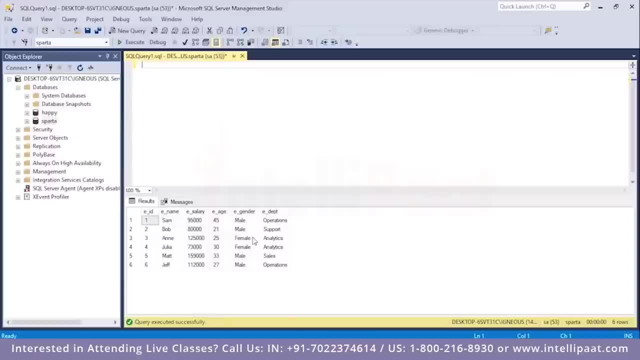 And if this evaluates to true, I'll just print 10 is greater than 20.. After that, I'll check if 10 is less than 20.. And if this condition evaluates to true, I'll print 10 is less than 20.. 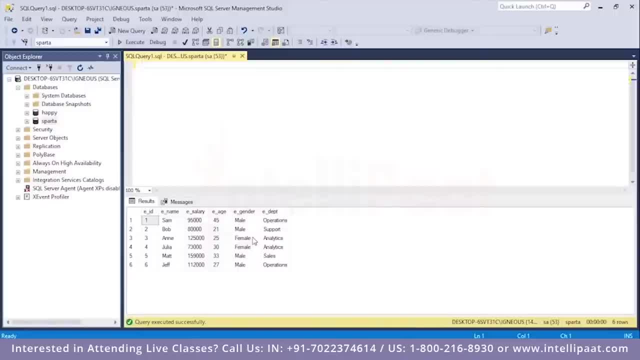 And if none of these two conditions evaluate to true, I'll just print: 10 is equal to 20.. So let me write the syntax for that Select, I'll give the case statement, Then type when and give the first condition, which would be 10 is greater than 20.. 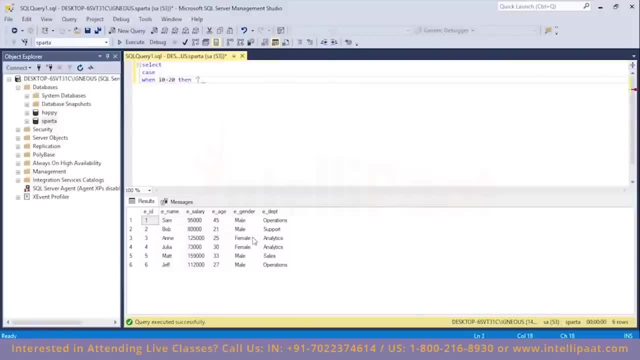 I'll type then And state what will happen if this condition is evaluated to true. So I'll just print 10 is greater than 20.. Then I'll type when And then state the second condition, which would be 10 is less than 20.. 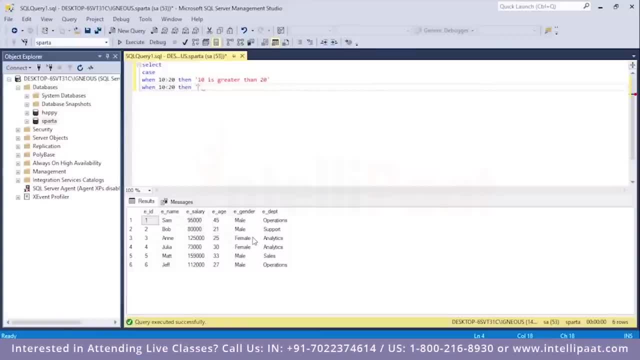 I'll type then. And if this condition evaluates to true, I have to print 10 is less than 20.. And if none of these conditions evaluate to true, I'll type else And just state 10 is equal to 20.. 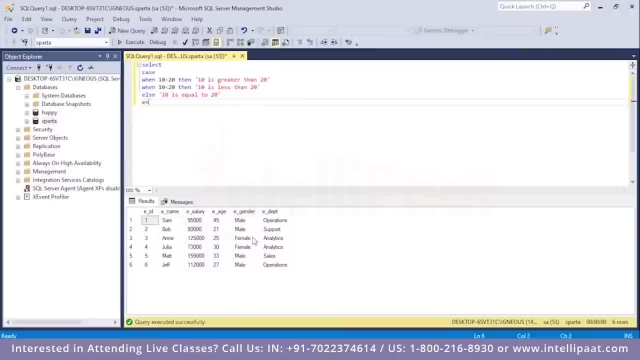 And I'll finish off the case statement with the end keyword. So let me hit execute So we get the result: 10 is less than 20.. So we get this result because the first condition has been evaluated to false, Because obviously 10 is not greater than 20.. 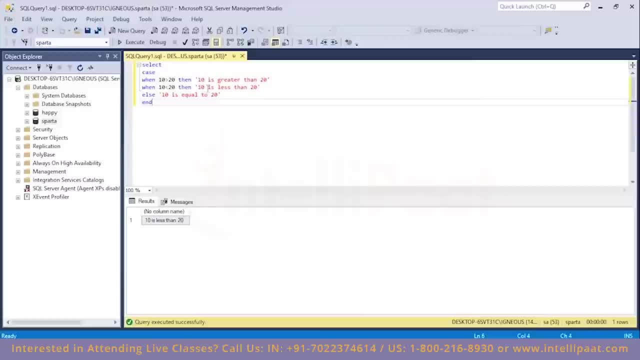 And since 10 is less than 20, this has been evaluated to true And we print: 10 is less than 20.. So now let's also implement this case statement on top of our employee table. So before we do that, let us actually have a glance at the employee table. 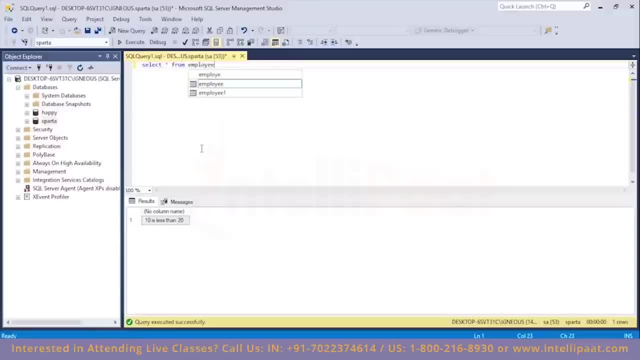 So I'll type select: start from employee Right. so this is our employee table. Now, using the case statement, I would want to add a new column grade which would be dependent on the salary column. So if the salary is less than $90,000, the grade would be C. 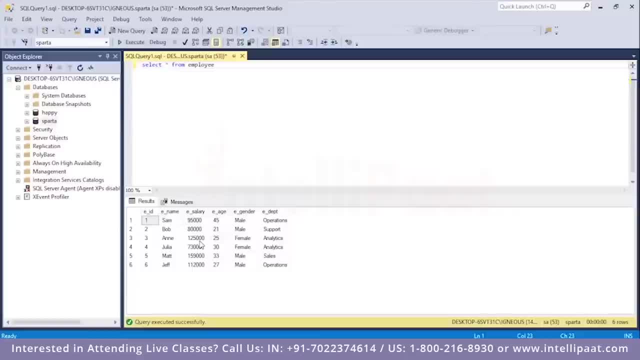 If the salary is between $90,000 and $100,000.. $120,000, the grade would be B, And if the salary is greater than $120,000, the grade would be A. So let me write the syntax for that. 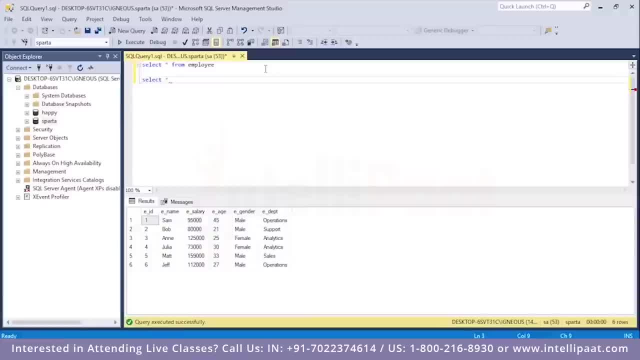 So I'll type select And I want all of the columns from the employee table. I'll type start And I'll add a new column, grade, And I'll be getting the values in this column with the help of the case statement. 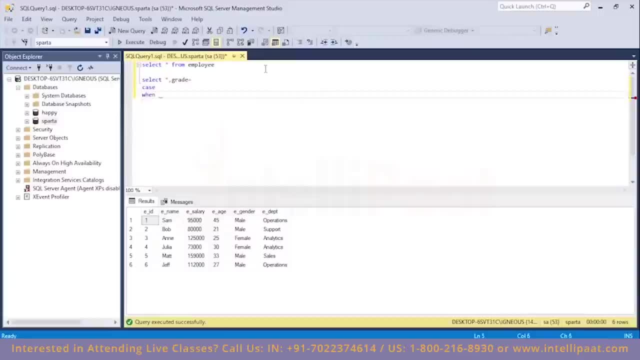 So I'll type case And then type the when keyword and give the first condition. So the first condition would be E- salary is less than $90,000. And if this evaluates to true, the grade would be C. I'll type when and say the second condition. 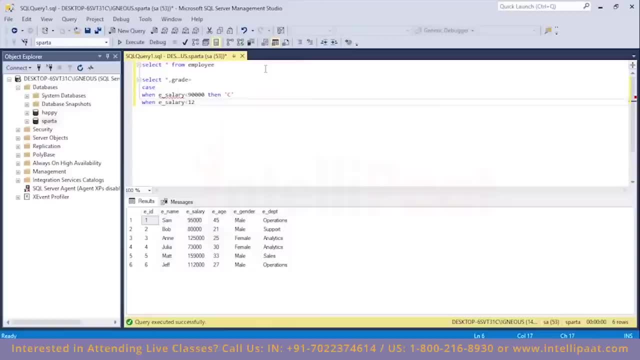 So the second condition would be: if E salary is less than $120,000.. So here, if the first condition is evaluated to false, then it would mean the salary is greater than $90,000.. And after that we'll check if the salary is between $90,000 and $120,000. 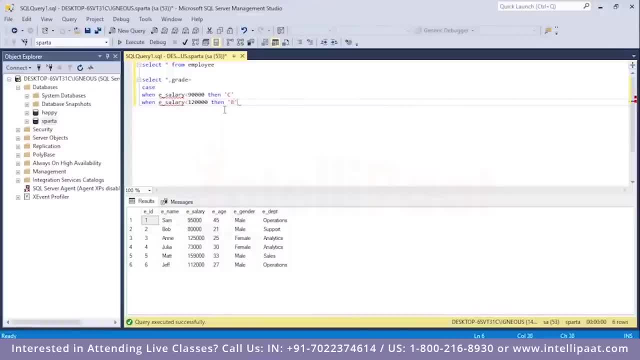 And if that evaluates to true, the grade would be B, And if none of these conditions evaluate to true, that would mean the salary is greater than $120,000.. So I'll type else, And then the grade which I want is A. 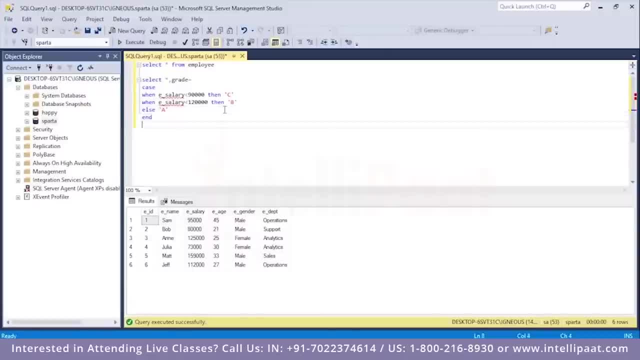 And I'll finish off this case statement with the end keyword: And I want all of this from the employee table. So I'll type from And then give the name of the table which would be employee. I'll type go, I'll select all of this. 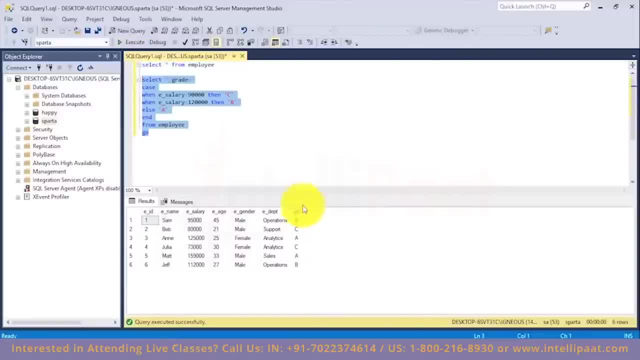 And I'll hit execute Right. So here we see that this new column grade has been added to the employee table And this grade column is dependent on the salary column. So here we see that the salary is between $90,000 and $120,000. 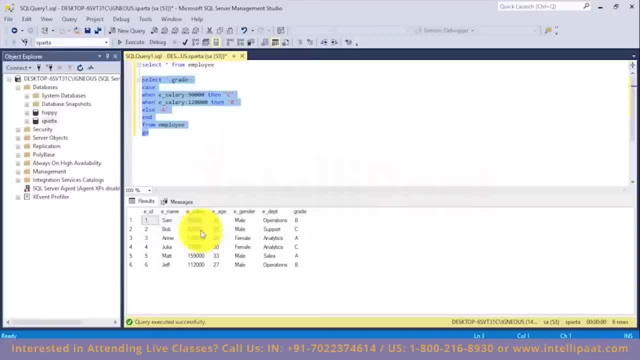 That is why the grade is B. Here the salary is less than $90,000.. The grade is C And over. here the salary is greater than $120,000.. That is why the grade is A. So this is how we can work with a case statement in SQL Server. 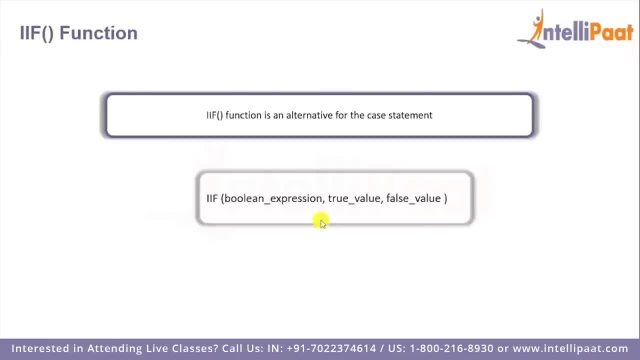 So the if function is an alternative to the case expression. This if function takes in a Boolean expression as the first parameter And returns the true value if the Boolean expression is evaluated to true. Similarly, returns the false value if the Boolean expression is evaluated to false. 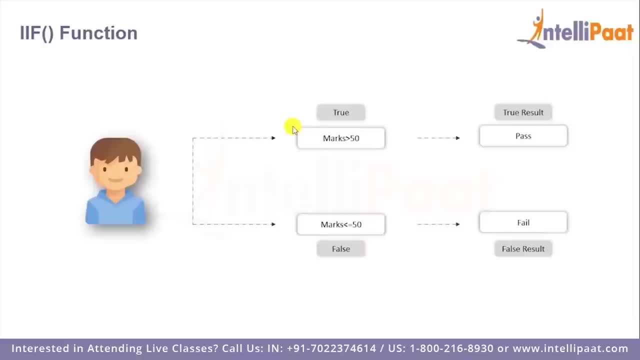 For example, let's say in the Boolean expression we are checking if the marks scored by a student are greater than 50. And if it evaluates to true, we'll return pass, And if the Boolean expression evaluates to false we'll return fail. 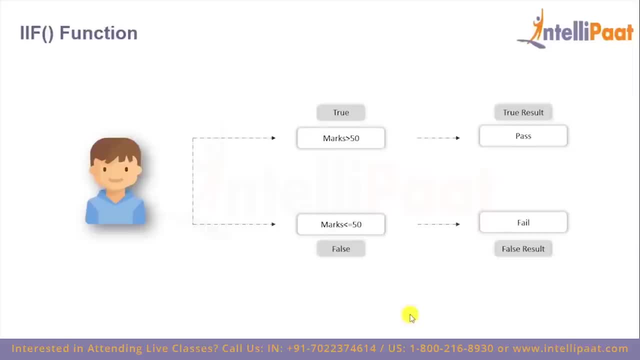 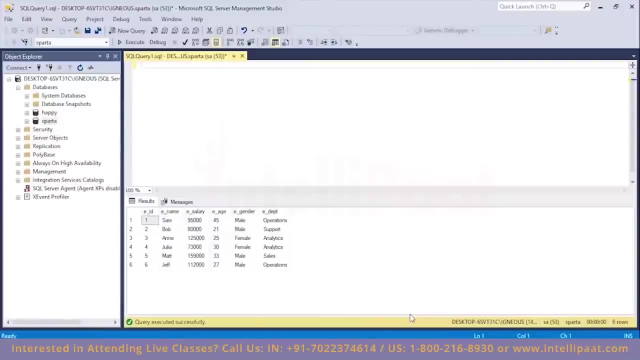 So this is how the if function works. Now let's implement this if function in SQL Server. So, using the if function, I'd want to check if 10 is greater than 20.. And if it evaluates to true, I'll print: 10 is greater than 20.. 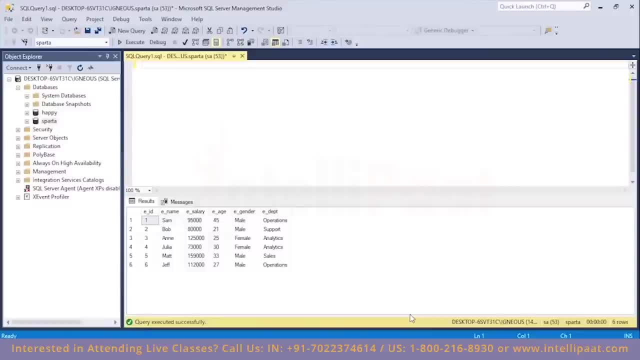 On the other hand, if it evaluates to false, I'll print: 10 is less than 20.. So let me write the syntax for that I'll type select. After that I'll use the if function and pass in the first parameter, which is the Boolean expression. 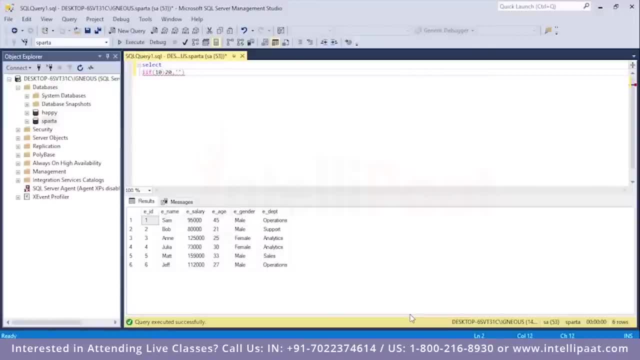 So 10 is greater than 20.. And if it evaluates to true, I would want to print 10 is greater than 20.. On the other hand, if it evaluates to false, I would want to print 10 is less than 20.. 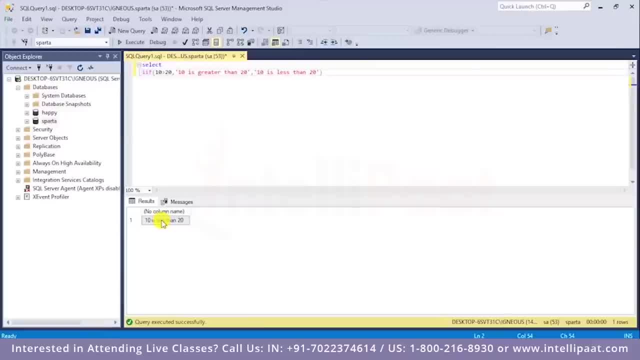 I'll hit execute. So what we get is 10 is less than 20.. So we get this result because this Boolean expression has been evaluated to false And it is redirected over here, And we get the false result, which is 10 is less than 20.. 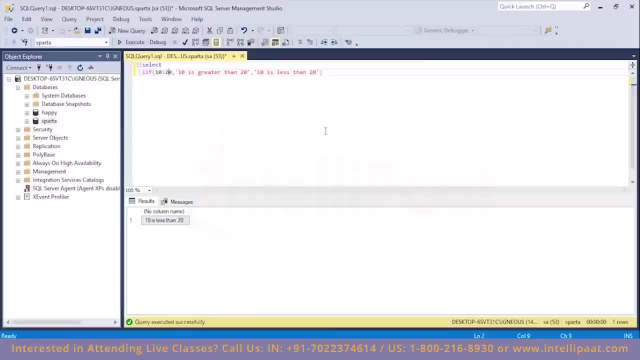 Now I'll go ahead And also implement this, if function, on top of the employee table. So before I do that, let me actually have a glance at the employee table first. So I will type select star from employee. So we have our employee table right in front of us. 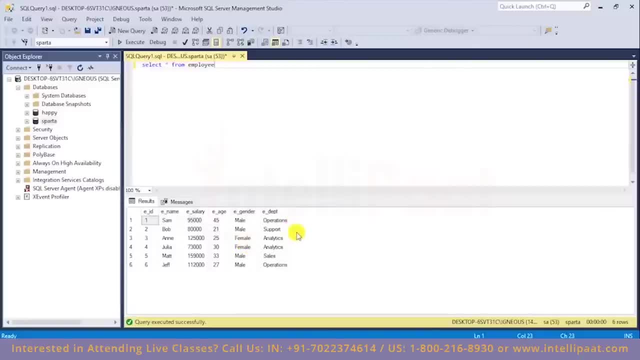 Now, using the if function, I'd want to add a new column- employee generation- And that new column would be dependent on this age column. So if the age of the employee is greater than 30, then the new column would have a value: old employee. 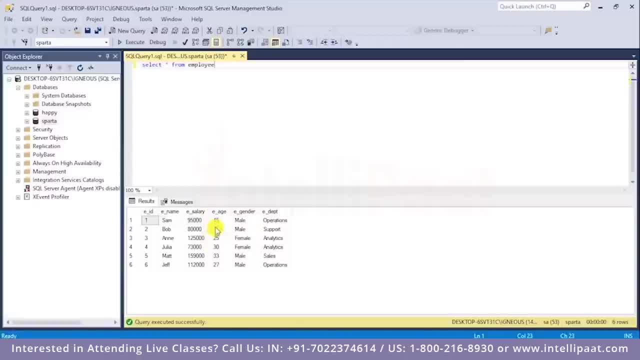 Similarly, if the age of the employee is less than 30, then the value in the new column would be young employee. So let me write the syntax for this. I will type, select and list down all of the columns which I want from the employee table. 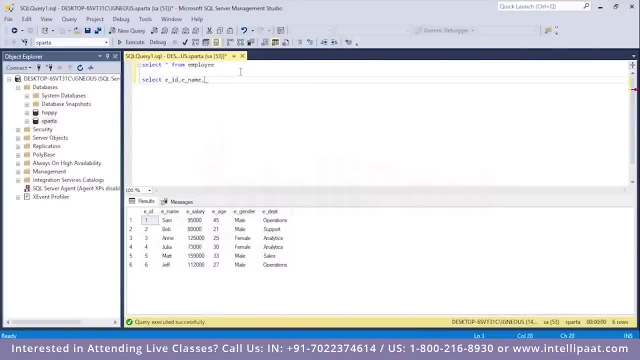 So I want the employee ID column, employee name column, employee age column. Now, after this I will use the if function to add the new column, So I'll get the first parameter, which would be the Boolean expression. So here I will check if e of age is greater than 30.. 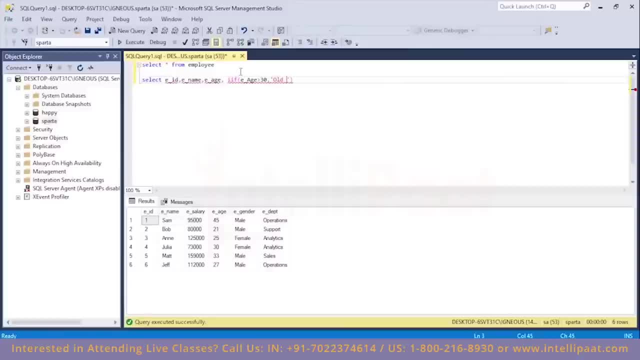 And if the age is greater than 30, I would want the value to be old employee. On the other hand, if the age is less than 30, I would want the value to be young employee. Now, I will name this new column as employee generation. 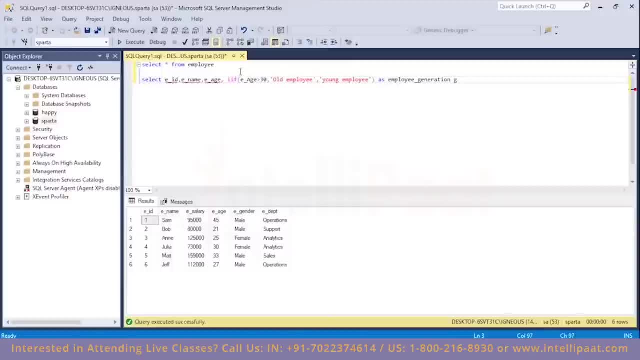 So let me just type the name of the column: employee generation over here, And I would want all of this from the table Employee. Now I will select this. I will hit execute Right. So we see that a new column has been added to this. 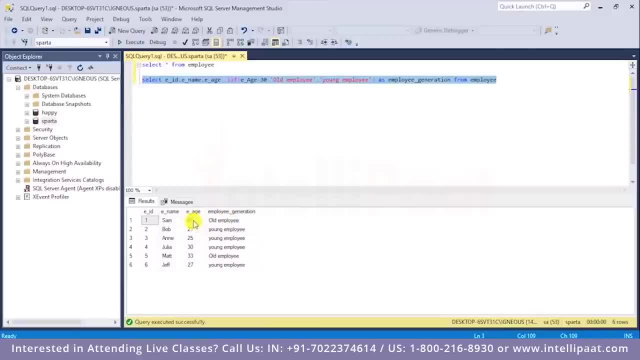 And the name of this column is employee generation. So here, if we have a glance at this age value, it is 45. And the corresponding value in employee generation is old employee. Similarly, here it is 21.. And since the value is less than 30, we get young employee. 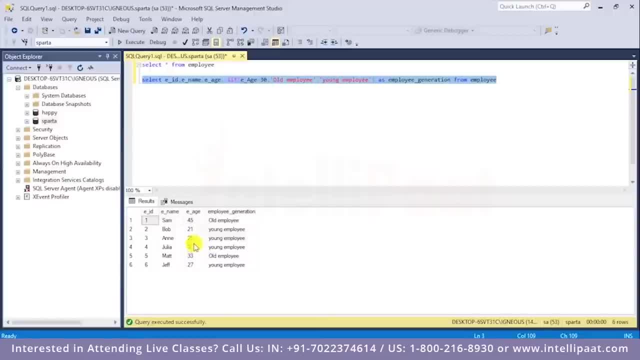 And these two. it is 25 and 30. And since these two values are also not greater than 30,, we have young employee over here And Matt whose age is 33,. we have the value old employee And we have Jeff whose age is 27,. he is a young employee too. 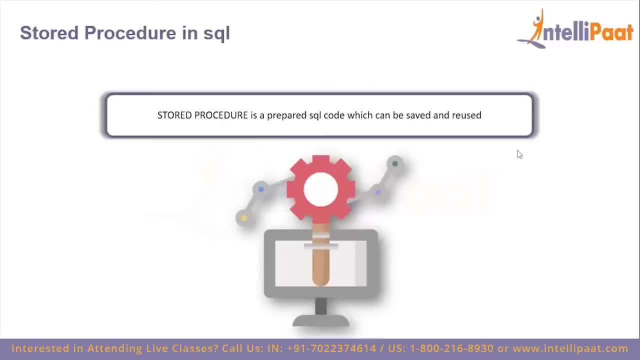 So this is how we can work with the if function in SQL. So a stored procedure is basically a prepared SQL code which we can save so that the code can be reused again. So if we have an SQL query that we write over and over again, 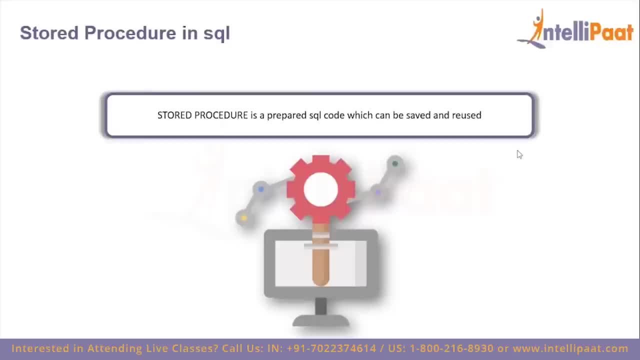 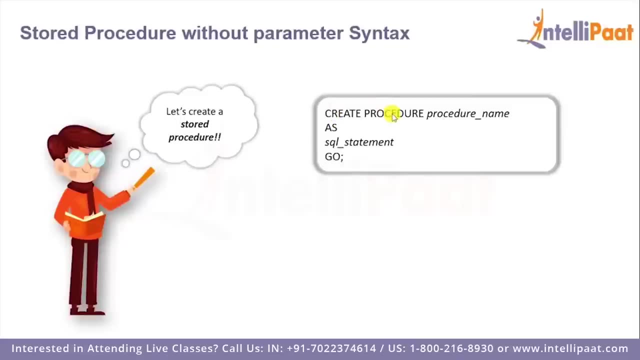 we can save it as a stored procedure and then just call it whenever we want. Now let's have a look at the syntax of the stored procedure. So we'll give the keywords create procedure and then give the procedure name. After that we'll give the keyword as and then give the SQL statement. 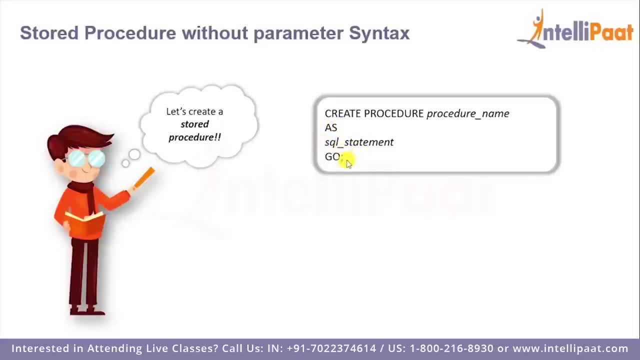 for which we need to create the procedure, And we'll end the procedure with the go keyword. Now, after we create a procedure, we need to execute it. So this is the syntax to execute the procedure: We'll type exec and then give the name of the procedure which is to be executed. 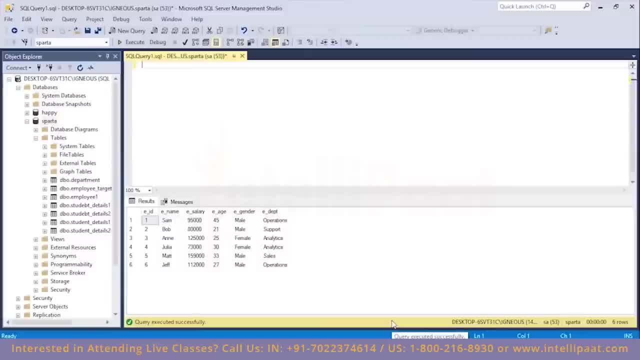 So let's go to SQL Server and work with some procedures. So now I want to create a procedure which would help me to easily access this eh column from the employee table. So I'll type create procedure and then I'll give the name of the procedure, which would be employee age. 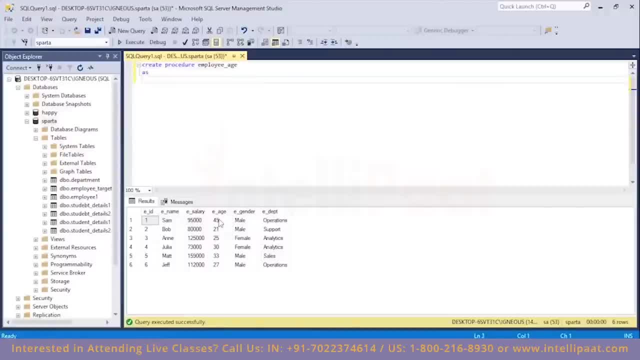 I'll type as and then give the SQL statement which would help me to access this eh column. That would be: select eh from the name of the table is employee, and then I'll give the go keyword. Now I'll hit execute. So we see that we have successfully created the employee age procedure. 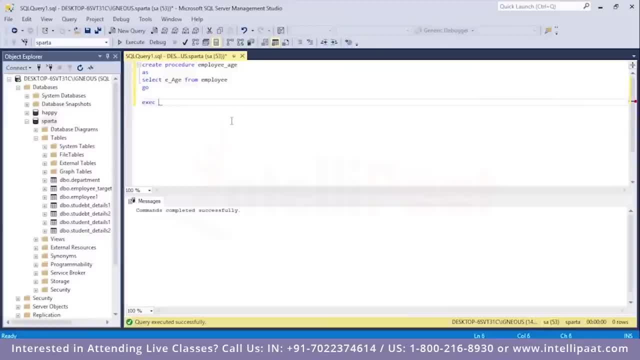 Now I will use the exec keyword and then call this procedure. So the name of the procedure is employee age. I'll select this line, I'll hit execute. So with this employee age procedure, we can easily access the eh column from the employee table. 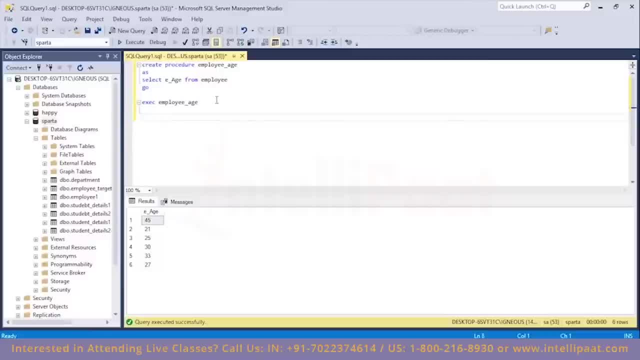 Now, similarly, I'll create another procedure which would help me to access all of the records from the employee table: Create procedure and I'll name this procedure as employee details. I'll follow it up with the as keyword and then give the SQL statement which would help me to access all of the records from the employee table. 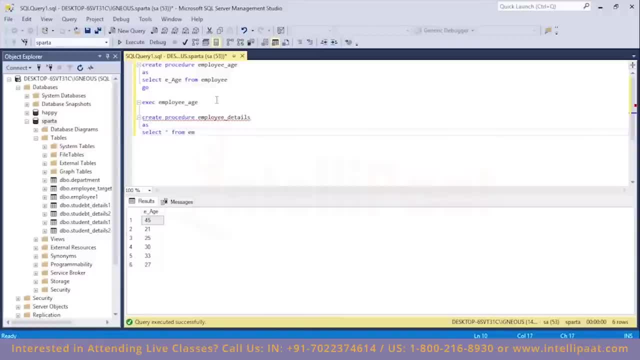 Select start from employee. and again I'll finish this procedure off with the go keyword. I'll select all of this, I'll hit execute. So again, we have successfully created the employee details procedure. Now to call this procedure, I'll use the exec command and then pass in the name of the procedure, which is employee details. 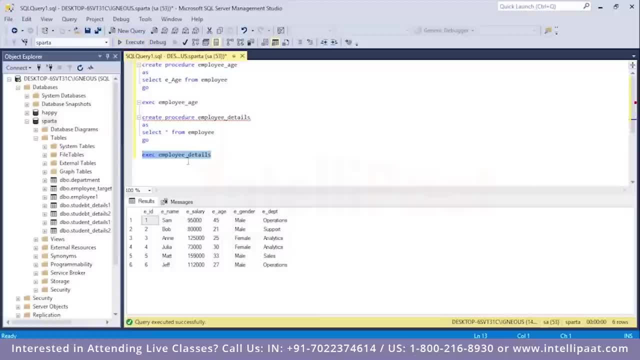 So I'll select this, I'll hit execute. So, with the help of employee details procedure, we can easily access all of the columns and all of the records from this employee table. Now we can also pass parameters to the procedure, So the syntax for this is just slightly different. 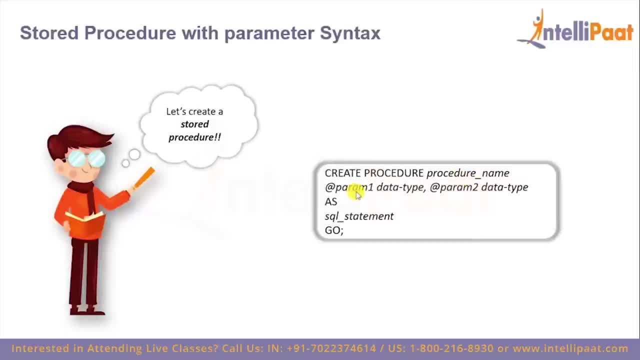 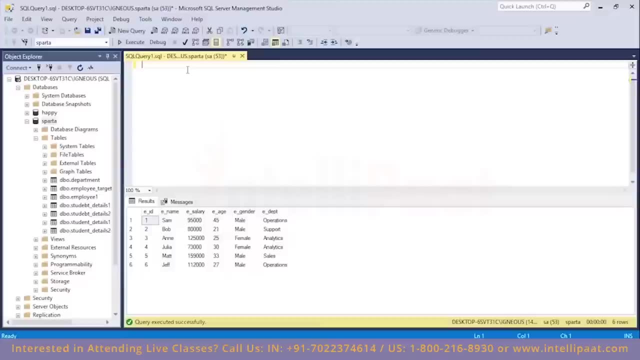 Here, after giving the procedure name, we follow it up with the list of parameters and their corresponding data types. So let's create a procedure with a parameter now. So now I'll create a procedure which would help me to access the male employees and the female employees separately from this employee table. 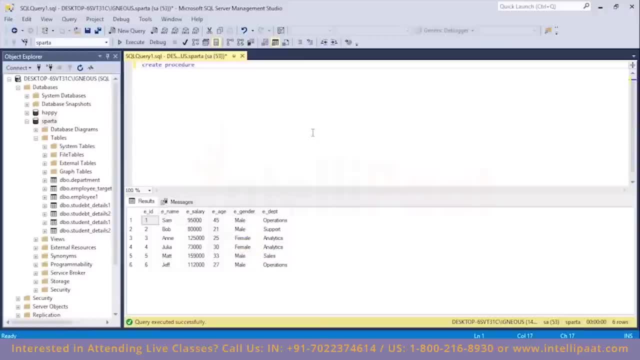 Create procedure and I'll name this procedure to be employee gender. After this, I will pass in the parameter. So the name of the parameter would be gender And it is of variable length character with a maximum length of 20.. I will give the as keyword after this. 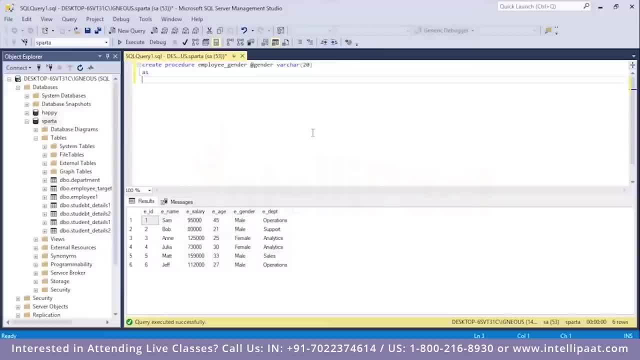 And then pass in the statements which would help me to individually access the male employees and the female employees Select. start from the name of the table. as employee, I'll follow it up with the where clause and give the condition. So this time the condition would be: e. gender is equal to. 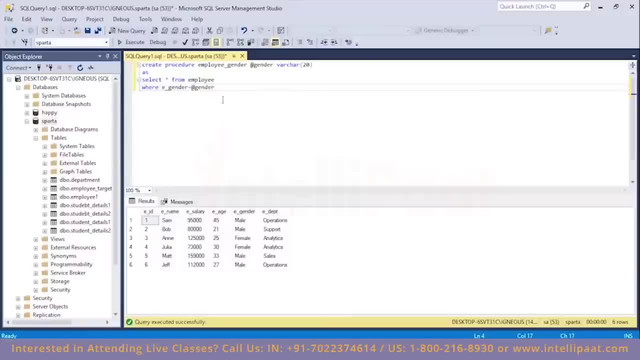 At the rate, gender. Let's understand this properly. So here e gender is basically this column And we are passing in the value of this parameter to this column. So let's say, when we call this procedure and the value is female, then we'll get all of the female employees. 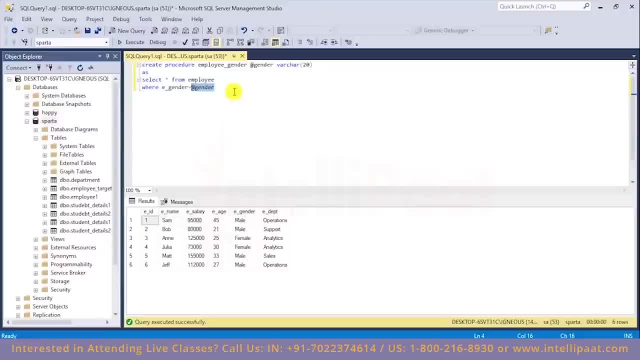 And similarly, if the value is male, then we'll get all of the male employees. Now let me finish off this procedure with the go keyword Right. So I have successfully created this employee gender procedure. Now let me go ahead and execute this procedure. 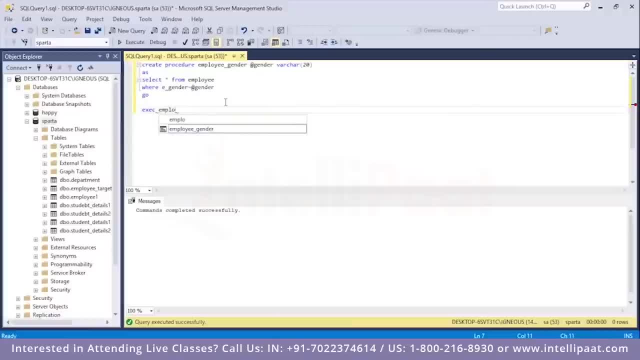 So I'll type exec and then give the name of the procedure, which would be employee gender. And now let's say I want all of the male employees, So I will give in the parameter name at the rate gender, And I will give in the value which would be equal to male. 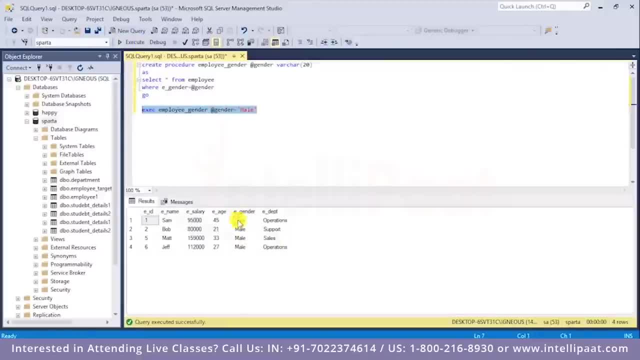 So let me execute this now. Right? So I've got all of the male employees from the employee table. Similarly, if I wanted all of the female employees from the employee table, this would be the command for that Execute I will give in the name of the procedure, which would be employee gender. 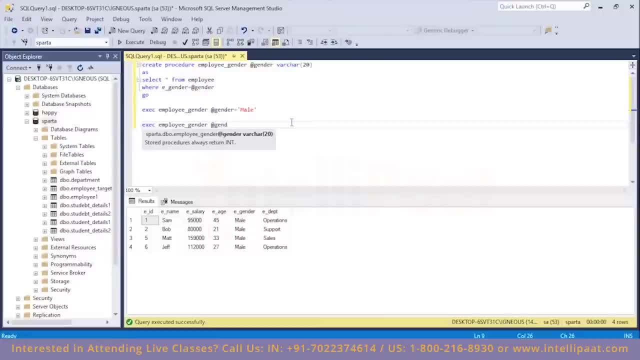 I will give the name of the parameter which would be at the rate- gender- And then pass in the value. So this time I would want all of the female employees, So the value would be female. I'll select this, I'll hit, execute. 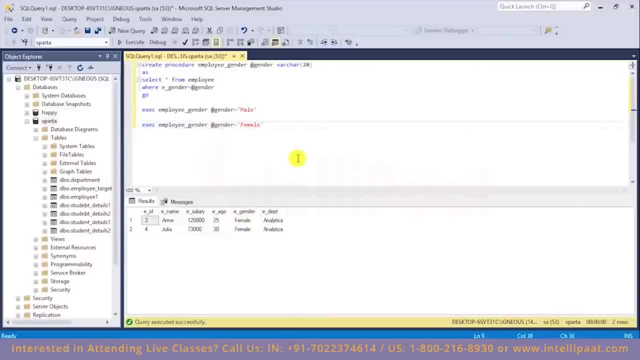 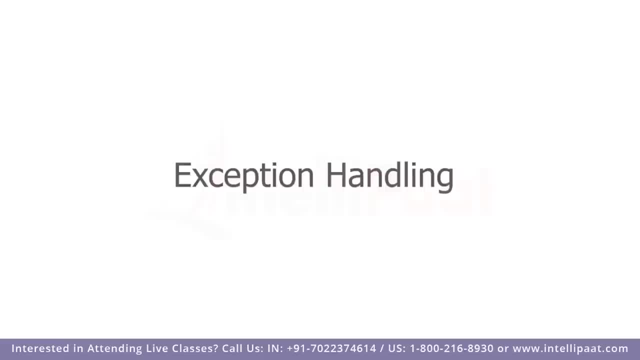 Right. So this time we've got all of the female employees from the employee table. So this is how we can work with stored procedures, Either with parameters or without parameters in SQL. So an error condition during a program execution is called as an exception. 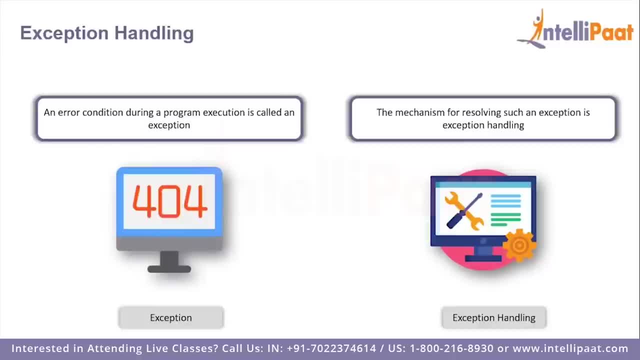 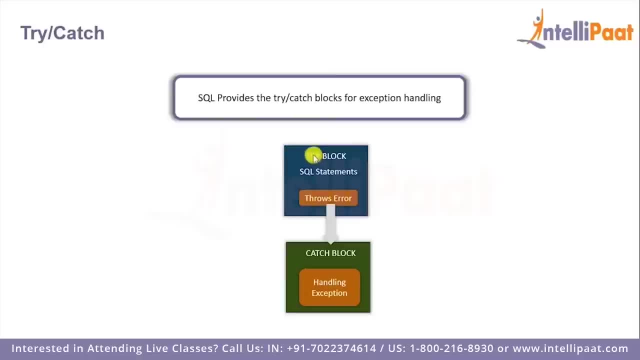 And the mechanism for resolving such an exception is known as exception handling, And we can do exception handling in SQL with the help of try-catch blocks. So the try statement allows us to test a block of statements while they're being executed And the catch block allows us to handle any exception which occurs in the try block. 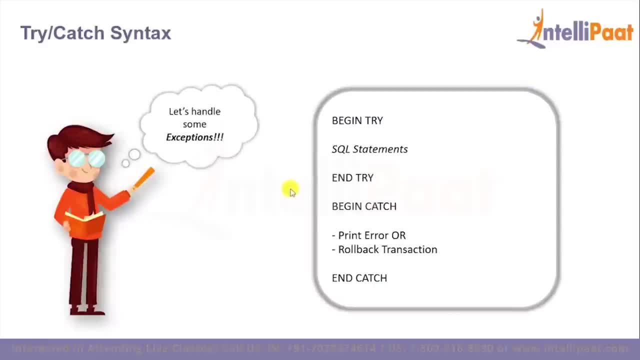 Now let's have a look at the syntax, The syntax of the try-catch block. So we'll give the keywords begin, try And then give the statements which are to be tested. After that we'll end the try block And begin the catch block. 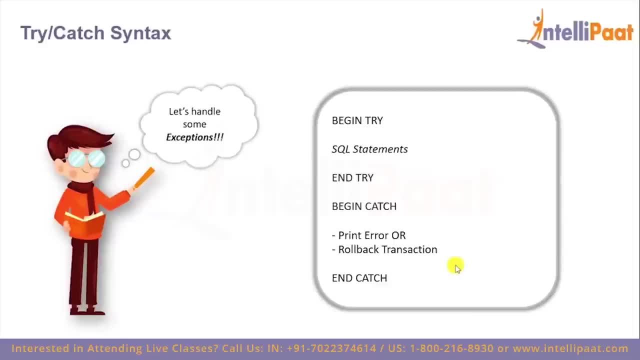 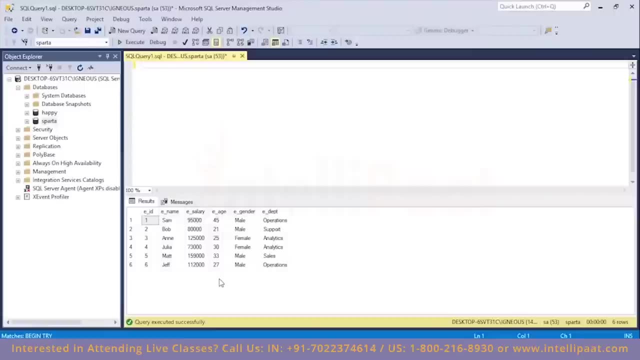 And inside the catch block we'll either print the error or roll back the transaction And we'll end the catch block as well. So let's go to SQL server and do some exception handling. So I'll be declaring two variables and divide one of the variables with zero. 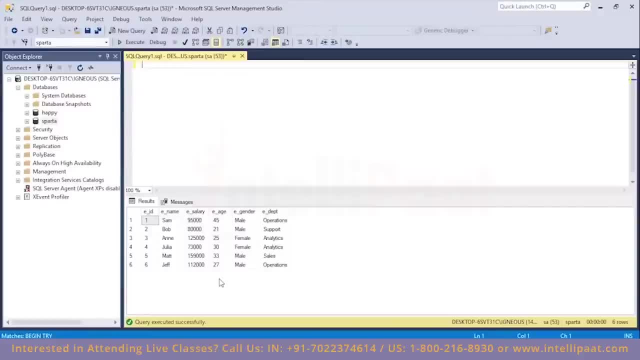 So this needs to give us divided by zero exception. So let's go ahead and handle this exception now So we can declare a variable in SQL by using the declare statement. So I'll type declare And then use the at the rate symbol to declare a value. 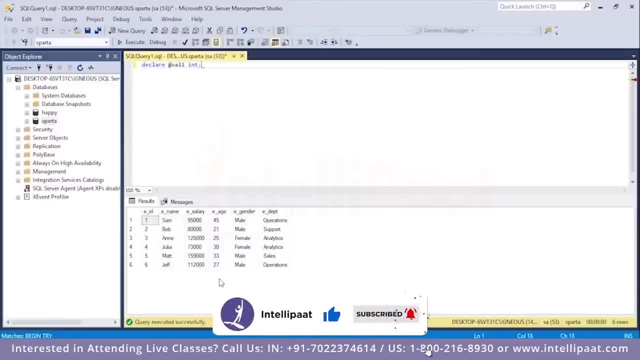 And I'll name this variable as val1.. And this is of integer type. Similarly, let me go ahead and declare the second variable. I'll type declare at the rate, And the name of this variable is val2.. And the data type is integer again. 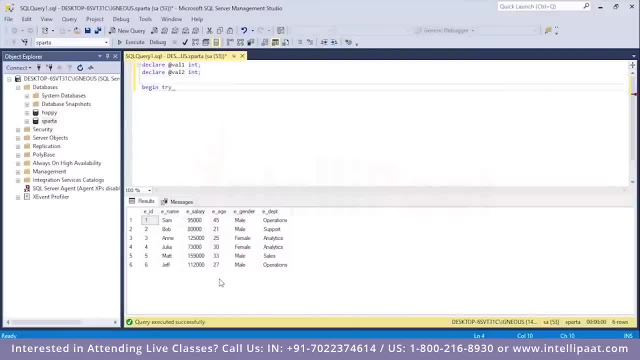 Now I'll begin the try block. I'll type begin try And then inside this I will set the values for both value 1 and value 2.. So I'll use the set keyword And then the value which I'll be assigning to val1 is 8.. 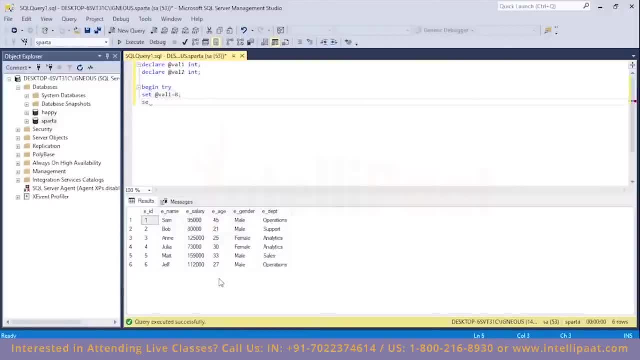 I'll put semicolon. Similarly, let me assign something to val2 as well. So set at the rate val2.. Now, inside val2, what I'll basically do is divide val1 with zero. So now this statement should basically give us the error. 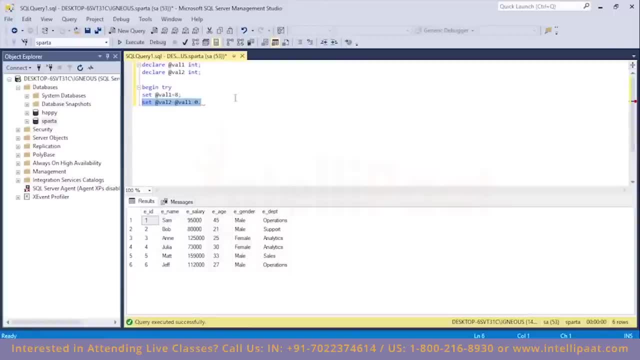 When we divide any integer value with a zero, we'll get an indefinite value. So this is the statement which will be giving the error. Now I will end the try block And try Right Now. after this, we'll begin the catch block. 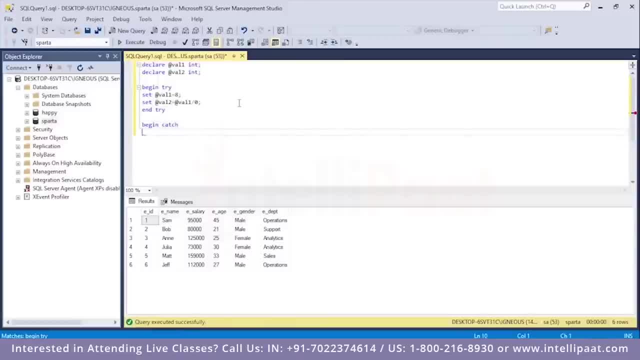 Begin Catch And inside the catch block I will just print out the error which occurred in the try block And I will display the default error message And I will end the catch block as well. So let me hit execute now. So the default error message which you get is: 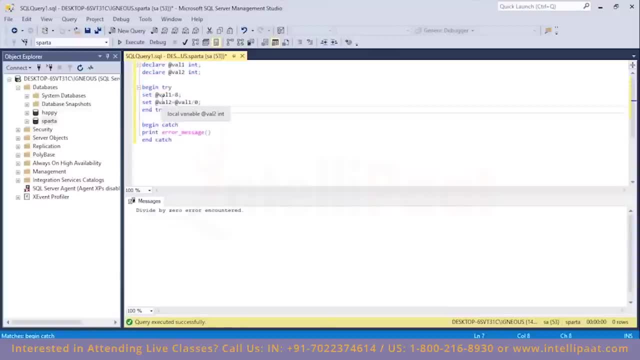 divide by zero error encountered. So what we basically did with this set of statements was we encountered an error within the try block and we handled that error inside the catch block. So inside the catch block we sent a default error message and that default error message. 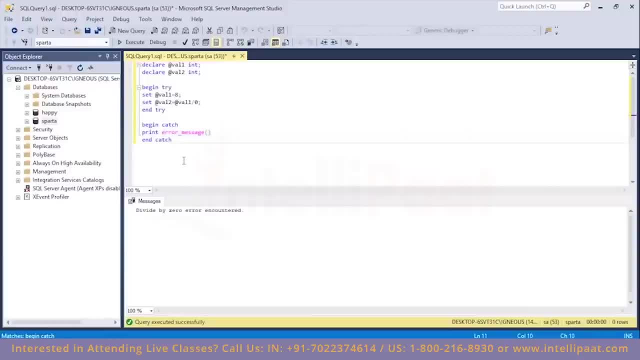 was divide by zero error encountered. Now we can also create user defined messages. So let's go ahead and create some user defined messages And for that purpose I'll be doing exception handling on top of the employee table. So let me actually have a glance at the employee table first. 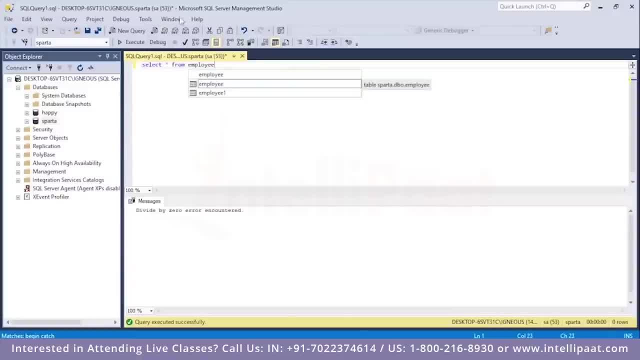 Select start run. The name of the table is employee Right. so we have this employee table right in front of us. So now what I'll do is I'll try to add the salary column and the name column. Now, the problem with this is: 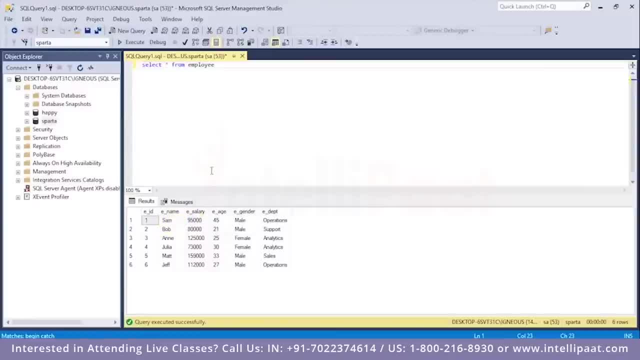 we cannot add a numerical column with a string value, So let's handle this exception. So I'll type begin, try And then I will give the select keyword and I will try to add e salary column with the e name column, And I want this from the employee table. 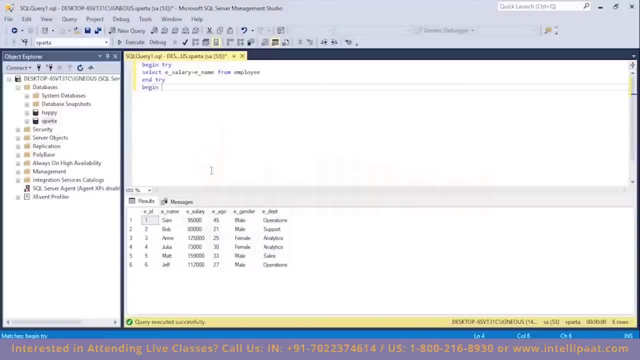 I will end the try block. After this I need to begin the catch block. So begin catch Now. inside this I will print the user defined message. So print And I would want to print. cannot add a numerical value with the string value. 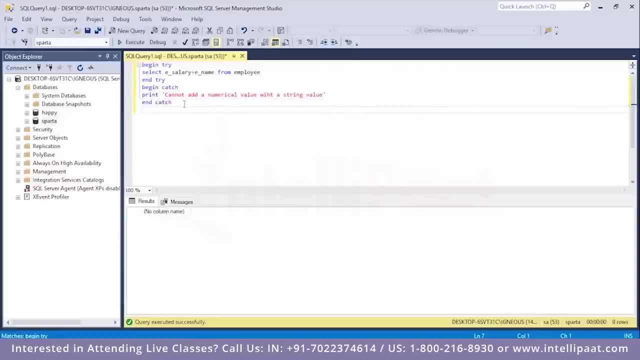 I will end the catch block as well. After this, I will give the go statement. Let me hit execute. So this is the message that the user defined And I want to add a numerical value with the string value. And we got this user defined message. 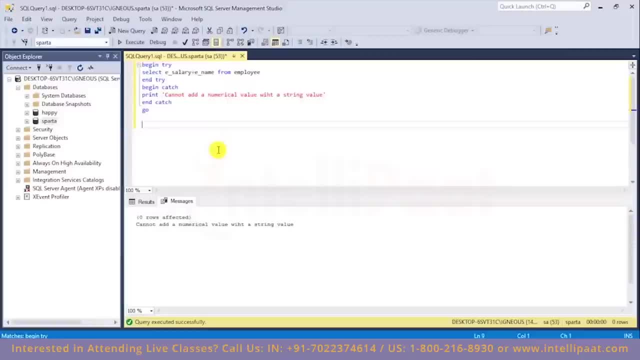 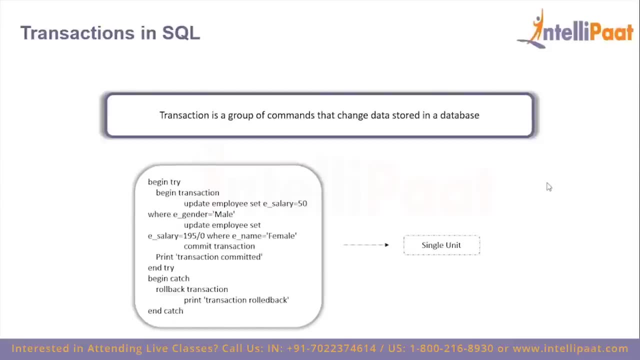 because we had encountered an error inside the try block. So this is how we can do exception handling in SQL. So a transaction is basically a group of commands which change data stored in a database And the transaction is treated as one single unit. So this transaction basically ensures that either. 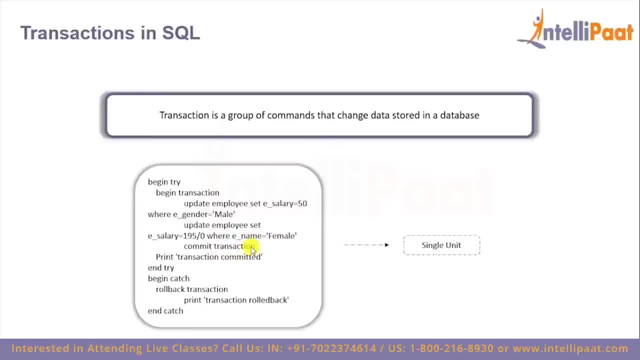 all of these commands are executed successfully or none of them is So. let's say, if one of the commands in the transaction fails, then all the commands will fail and any data which was modified in the database will be rolled back. Similarly, if all the commands inside the transaction execute successfully, 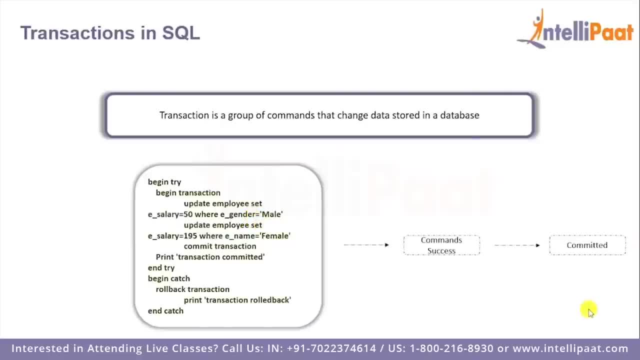 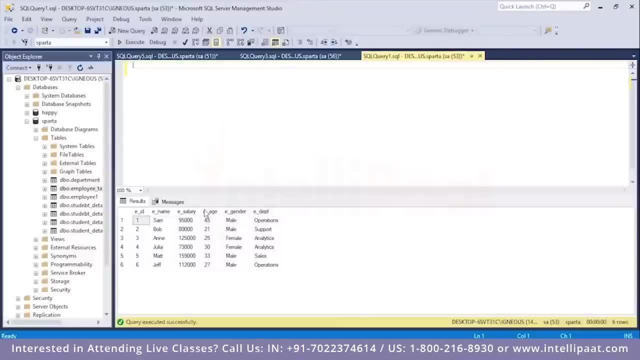 only then the transaction will be committed. So this is how transactions ensure integrity of data. So now I'll begin a transaction And inside the transaction I'll try to update this age value from 45 to 30.. So let me write the syntax to begin a transaction. 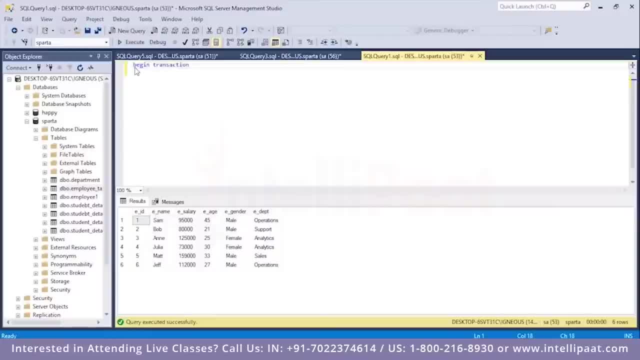 So I'll type begin and then type transaction And inside this I'll give all of those SQL statements which either have to be committed or rolled back. So over here I'll give the update statement, I'll type update and then give the name of the table which would be employee. 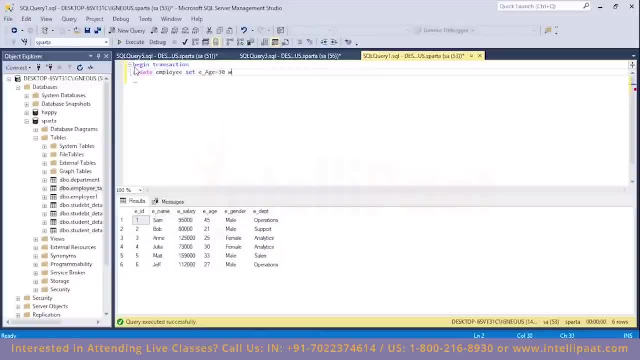 Set, eh, to be equal to 30, where ename is equal to Sam. So I'll select these two statements and I'll execute them. So you see that one row has been affected. So now let me have a glance at the modified table. 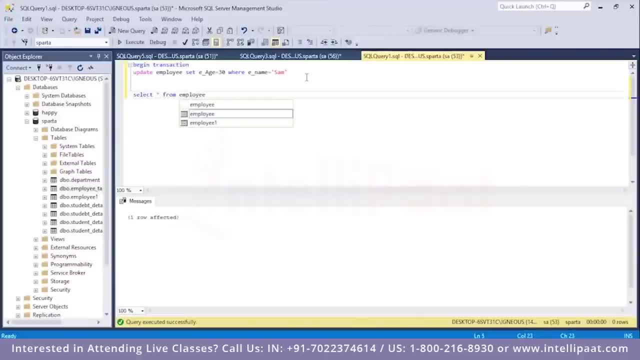 So I'll type select star from employee. I will select this command over here. I'll execute this Right. so you see that initially the age value was 45 and after we applied this update command, the age has been changed from 45 to 30.. 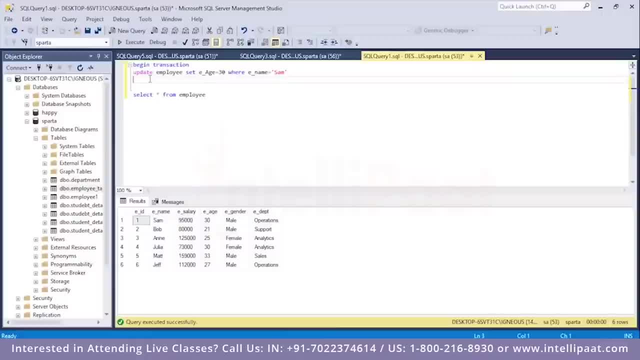 Now, since this command is inside a transaction, we have the option to either roll back this command or commit this command. So now let me go ahead and actually roll back this transaction. So to do that, I'll type rollback transaction. So now let me select this. 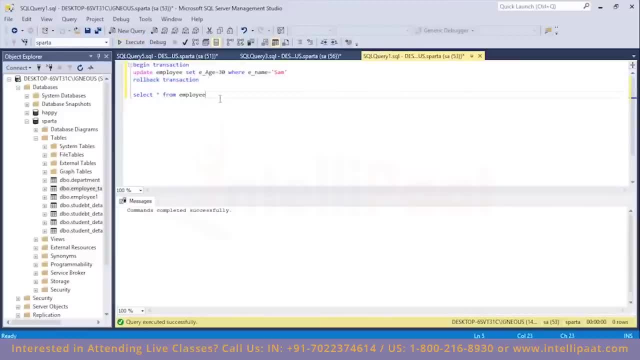 I'll click on execute. So you see that the commands have been completed successfully. Now let me again have a glance at the employee table Right. so since we have rolled back the transaction, we see that the age value has gone back to the original value. 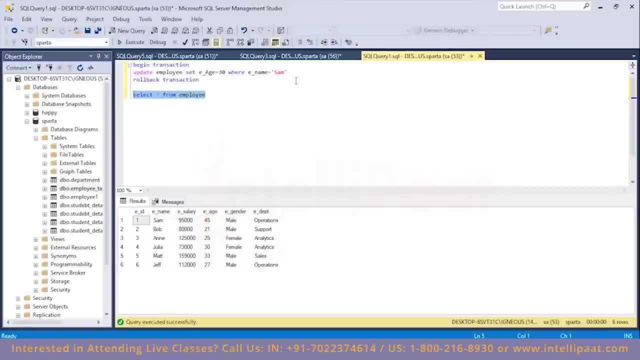 Which is 45. So initially, using the update command, we had changed the age value from 45 to 30. And after that we had rolled back the transaction. Now what I'll do is I'll execute these two statements again And let me have a glance at the table. 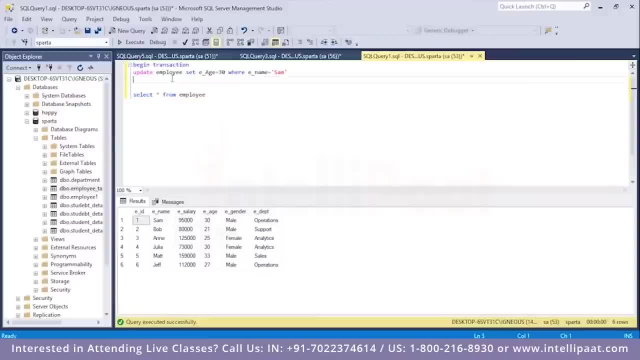 Right. so again we see that the age has been changed to 30. So this time, instead of rolling back the transaction, I will commit the transaction. So I'll type commit transaction, So I'll select this, I'll click execute. Now let me have a glance at the table. 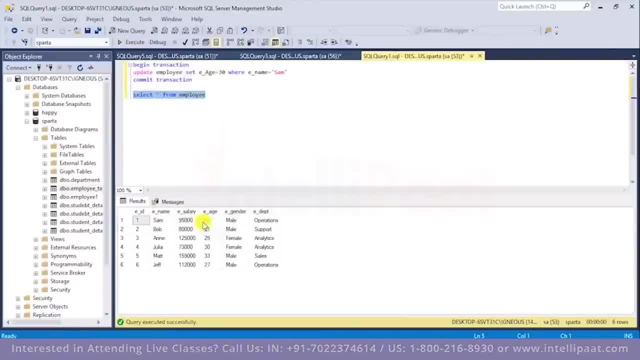 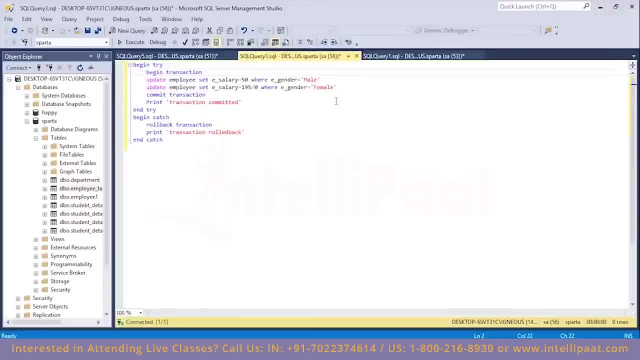 So this time the transaction has been committed and the change is permanent. So this is how we can either commit or roll back the commands using a transaction. Now let's look at another example. So in this example we are using transactions inside the try-catch block. 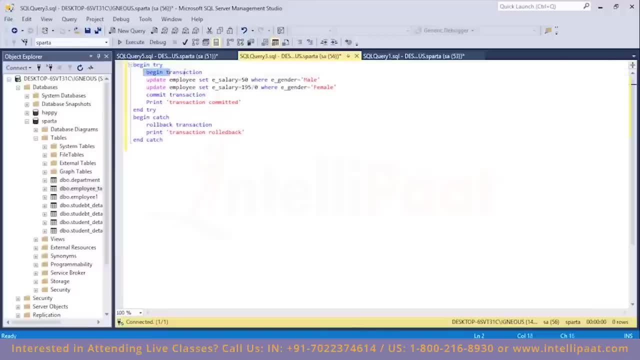 So over here we are beginning the try block and inside this we are beginning the transaction. And inside the transaction we are trying to update the salary value to be equal to 50 where the gender value is equal to male, So wherever the gender is equal to male. 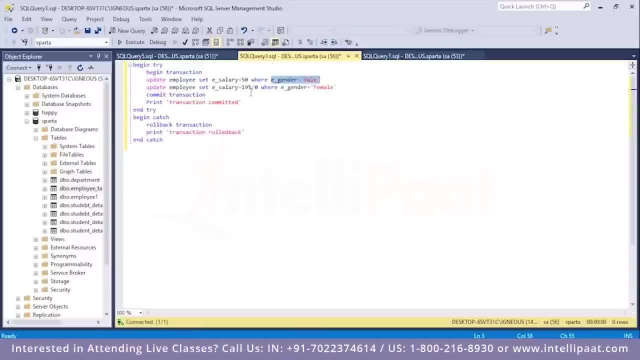 we'll update that salary value to be equal to 50.. Similarly, wherever the gender value is equal to female, I will change that salary value to be 195 divided by 0, which would give us an undefined value, And after that we'll commit this transaction. 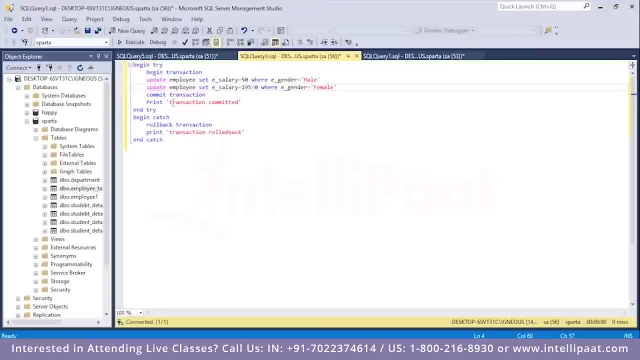 and print transaction committed. Now, since we have put this transaction inside the try block, if any error occurs, that will be sent to the catch block and we will roll back the transaction. So over here we see that we are dividing 195 with 0.. 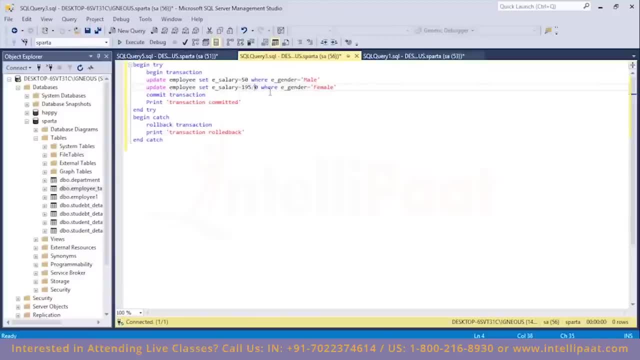 And since this gives us an undefined value, we will get an error And that error will be handled in this catch block and we will roll back the transaction. So let me execute this, So you see that the transaction has been rolled back because we get an error inside the try block. 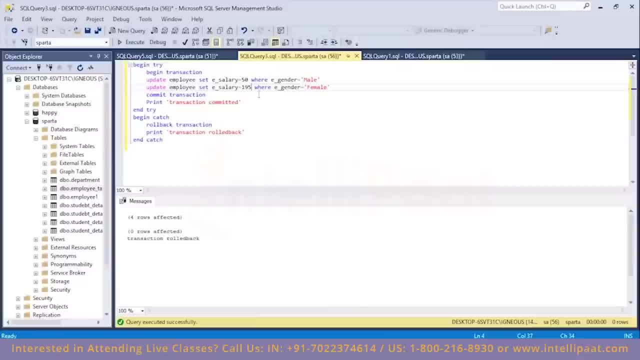 Now what I'll do is I will remove this divided by 0 and run this command again. So this time we see that the transaction has been committed because there was no error inside the try block. So now let me have a glance at the modified employee table. 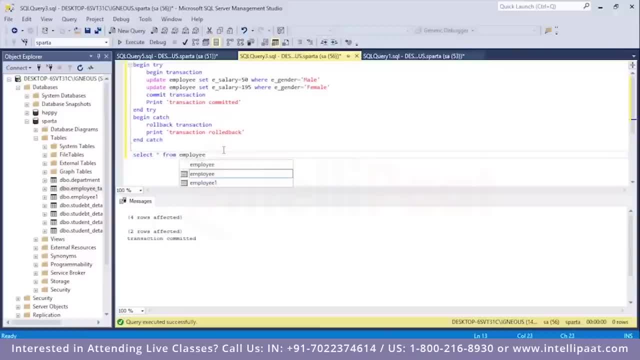 So I'll type select start from employee, I'll select this, I'll click on execute. So we see that we have changed the salary value to be 50, where gender is equal to male. Similarly, I have changed the salary value to be equal to 195. 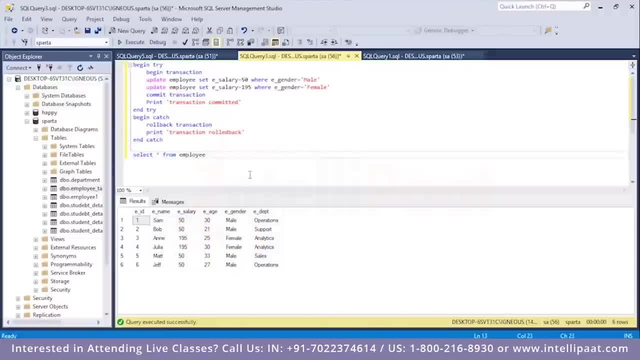 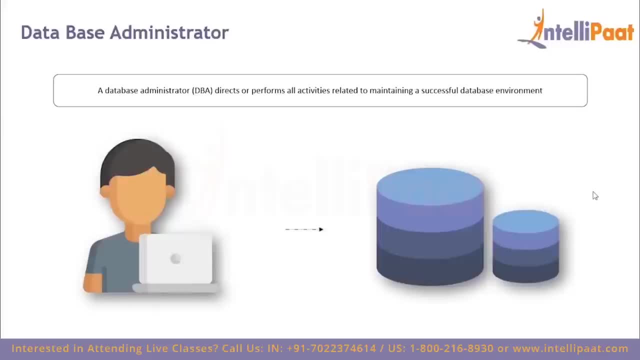 where the gender is equal to female. This is how we can work with transactions in SQL. So who is a database administrator? Well, a database administrator is someone who directs or performs all activities related to maintaining a successful database environment. So now that we know who is a DBA, 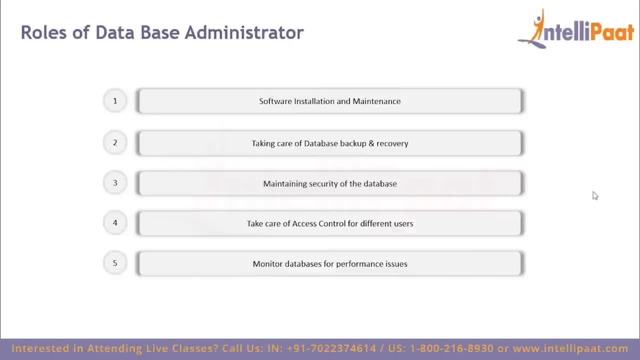 let's look at some of the roles of database administrator. So a DBA has to take care of the initial installation and configuration of a new Oracle or SQL server database. The system administrator sets up hardware and deploys the operating system for the database server. 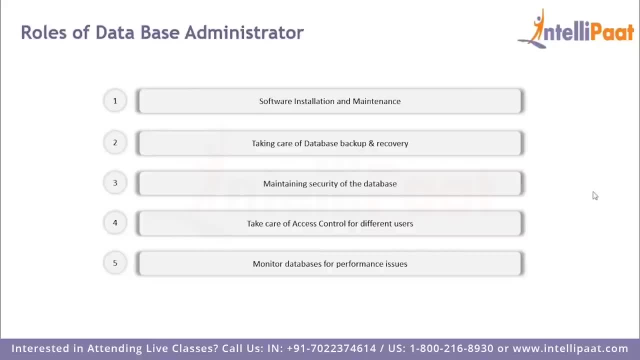 Then the DBA installs the database software and configures it for use As updates and patches are required. the DBA has to handle this ongoing maintenance. A DBA has to also take care of backup and recovery of databases. So a DBA has to take care of backup and recovery of databases. 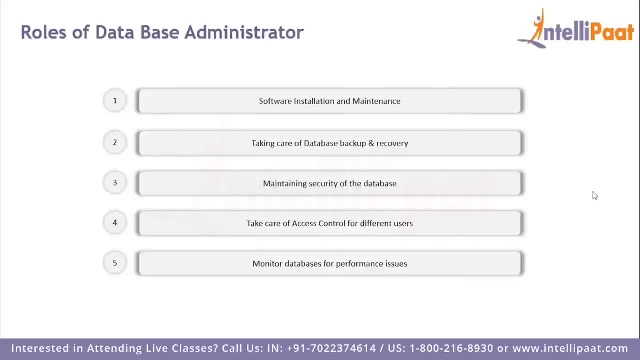 So DBAs have to create backup and recovery plans and procedures, based on industry best practices, that make sure the necessary steps are followed. Another role of DBA is to maintain security of the database, So a DBA needs to know potential weaknesses of the database software. 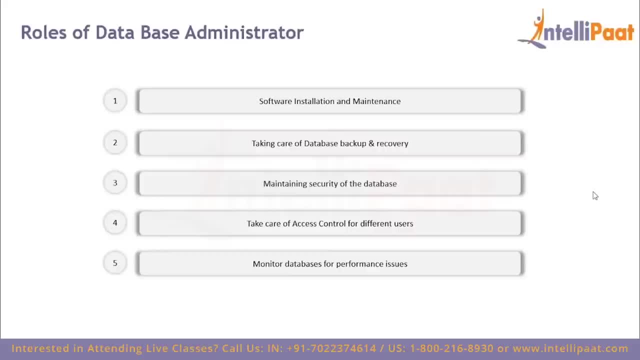 and the company's overall system and work to minimize risks. In case of a security breach or irregularity, the DBA can consult audit logs to see who has done what to the data. The DBA has to also take care of access control. 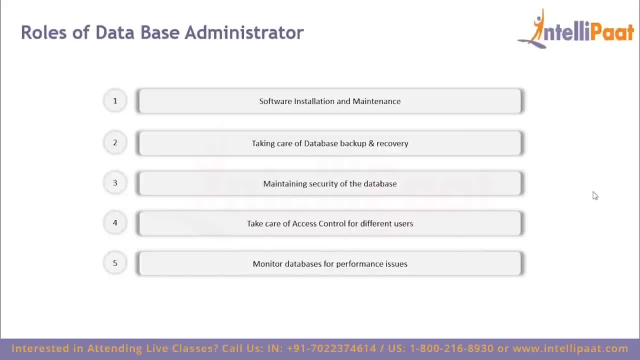 That is, it has to verify which users can be granted access to the system and which users should be denied. Then a DBA has to also monitor databases for performance issues. So if some part of the system is slowing down the processing, the DBA may need to make configuration changes to the software. 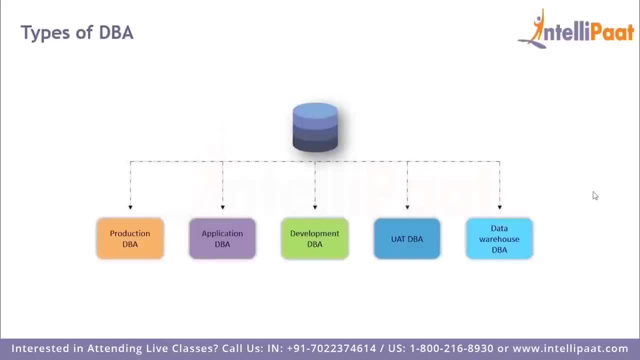 or add additional hardware capacity. So now that we know what are the roles of a DBA, let's look at the types of DBA. Let's start with production DBA. So a production DBA is responsible for maintaining databases within an organization. 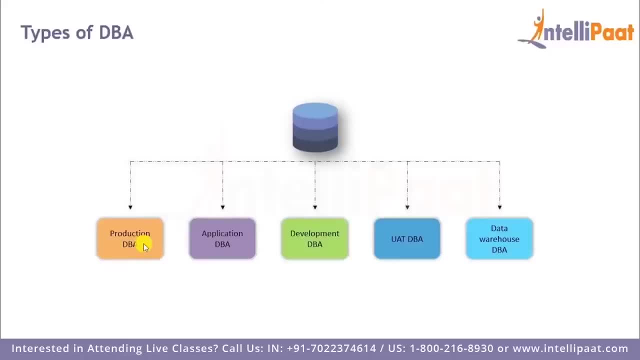 The production DBA often gets involved when all the design decisions have been made and he or she has to keep things up and running. So the production DBAs basically take over after applications have been created and they would have to keep the server running smoothly. 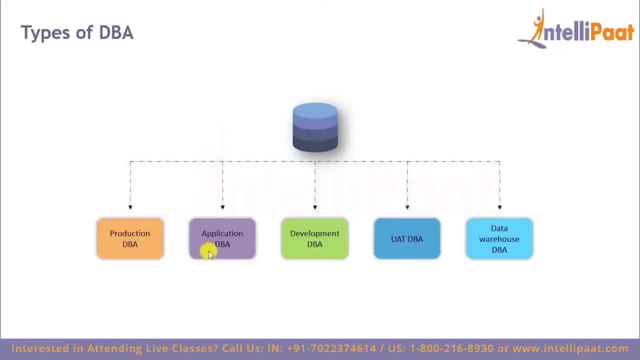 back it up and plan for future capacity needs. Then we have application DBA. So an application DBA focuses on a specific business application. He or she would be an expert in SQL and would implement the application business logic using SQL or any other query language. 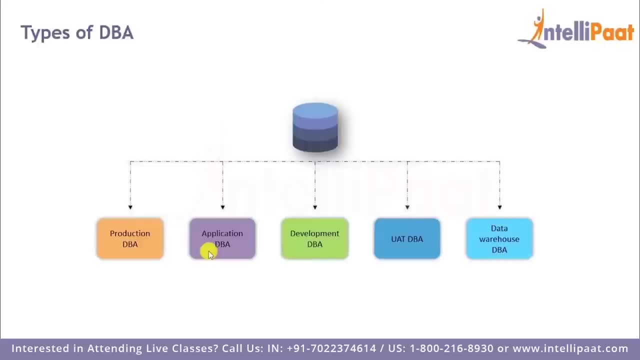 They would be also responsible for performance tuning of the database application. Next, we have development DBA. So the development DBA focuses on tasks related to building an effective, usable database environment to support the creation and maintenance of applications. Development DBAs need to be skilled in the process of data modeling and normalization. 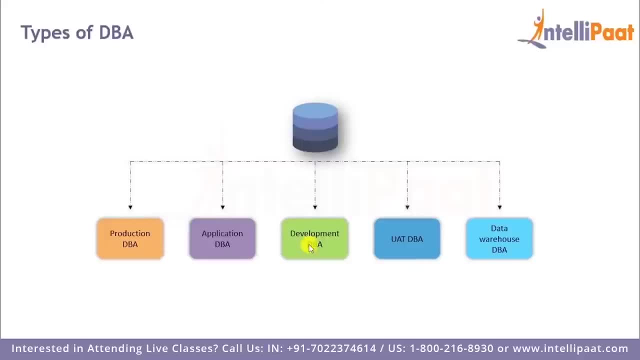 to ensure that databases are designed to promote data integrity. Then there's UAT DBA. So a UAT database actually stands for Under Application Testing Database And the UAT DBA is completely responsible for the testing and development of UAT database. 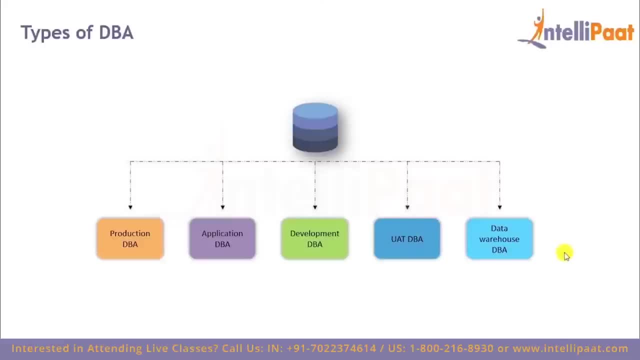 And finally, we have development DBA- Data Warehouse DBA. So a warehouse DBA is responsible for analyzing and understanding the data provided. It is his responsibility to study and track patterns for analytics and business intelligence. Hence, a warehouse DBA handles a more significant amount of data for a more critical function. 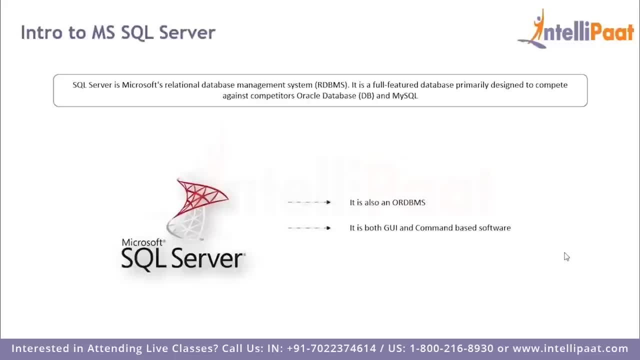 Now let's understand what is MS SQL Server. So Microsoft SQL Server is a relational database management system, or RDBMS, that supports a wide variety of transaction processing, business intelligence and analytics applications. So Microsoft SQL Server is built on top of SQL that is tied to TransactSQL or TSQL. 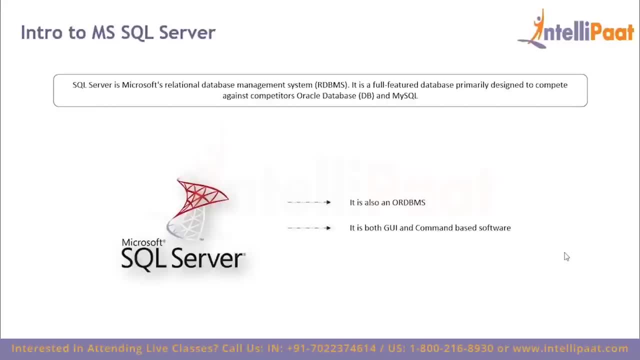 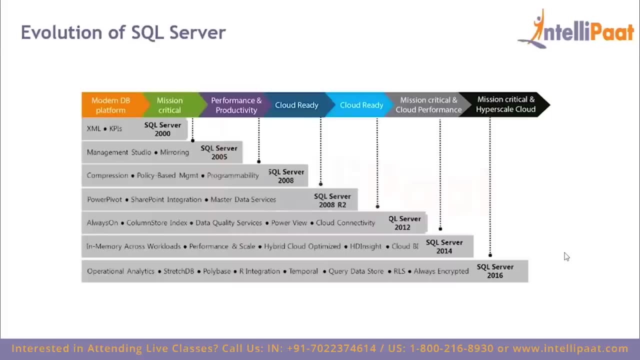 which is an implementation of SQL from Microsoft that adds a set of proprietary programming extensions to the standard language. Now let's look at the evolution of SQL Server. So the SQL Server database platform that we know today began with the SQL Server 7.0 release. 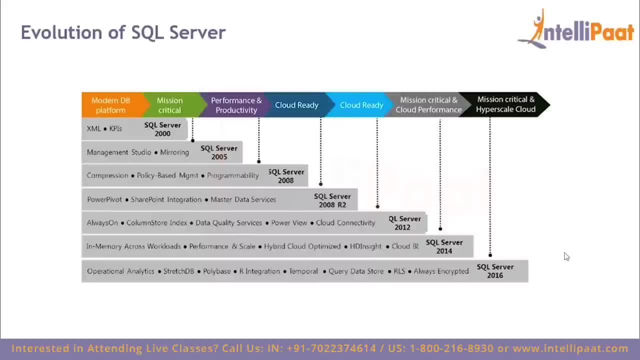 in 1998.. So Microsoft re-architected the core database engine code in SQL Server 7.0 to address the database's scalability issues, transforming it from a departmental database into a true enterprise-level database. Perhaps even more important, Microsoft added OLAP services, which would eventually become 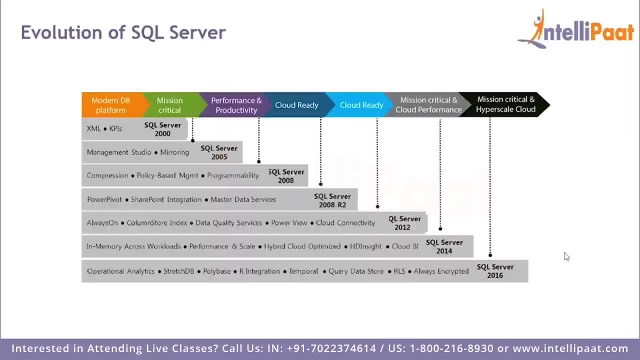 SQL Server analysis services. Then the SQL Server 2000 release saw Microsoft continuing to push the process of the platform into enterprise. This release boosted scalability through large memory and address windowing extension support. The company also expanded SQL Server's data handling capabilities with the new XML data type. 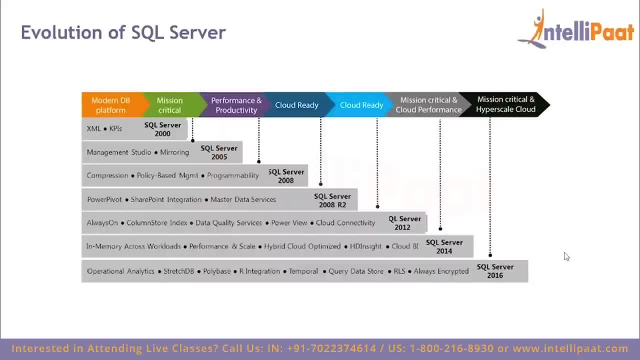 And then came SQL Server 2005,, which was a major milestone. Microsoft added CLR integration Plus. this was the first release to include the popular SQL Server reporting services subsystem out of the box. Microsoft also had replaced data transformation services with the new SQL Server integration. 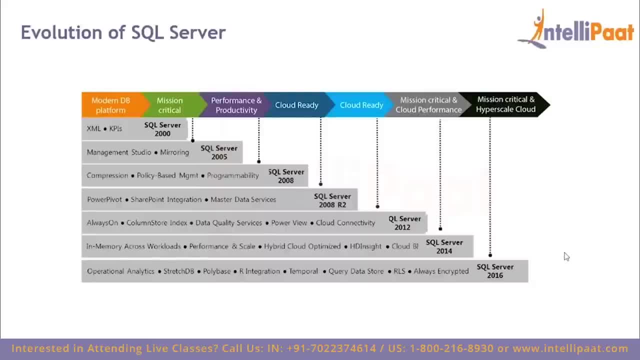 services in this release, And then SQL Server 2008,. Microsoft refined SQL Server's enterprise capabilities, adding transparent data encryption as well as the file stream and geospatial data types. SQL Server 2008 was also the first release with built-in row and page compression for 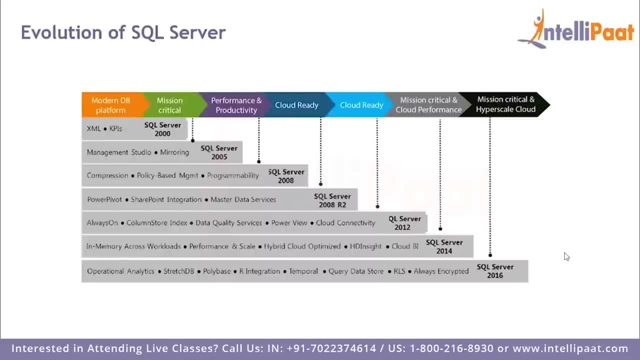 tables and indexes. Then came SQL Server 2012,, which expanded SQL Server's BI capabilities, with the addition of PowerView, which is a graphical data navigation and visualization tool. In this release, Microsoft also added always-on availability groups, which extended SQL Server's 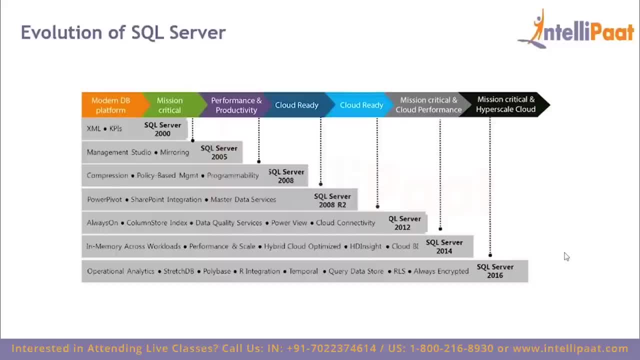 high availability and disaster recovery options. The next release was SQL Server 2014,, which provided a new in-memory capability for tables that could fit entirely in memory. It also provided a new hybrid disaster recovery and backup solutions with Microsoft Azure, enabling customers to use existing skills with the on-premise version of SQL Server. 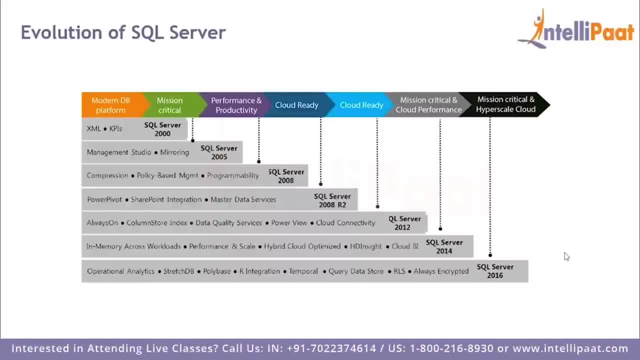 to take advantage of Microsoft's global data centers. Then SQL Server 2016 released, which added new built-in JSON support in SQL Server for JSON imports, exports, parsing and storing. A new poly-based query engine was also added to integrate SQL Server with external data. 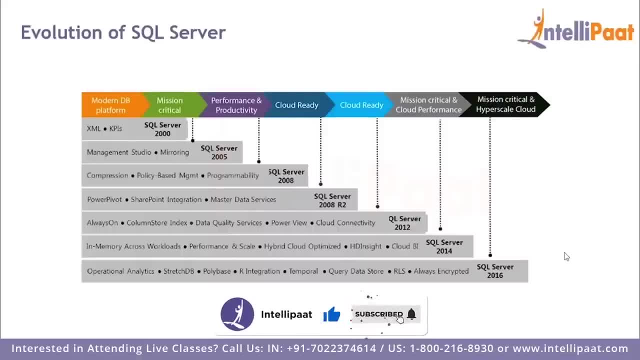 in Hadoop or Azure Blob storage, And the latest release is SQL Server 2017.. And with this release, SQL Server is no longer just a Windows-based RDBMS. We can now develop applications with SQL Server on Linux, Windows, Ubuntu or Docker and deploy. 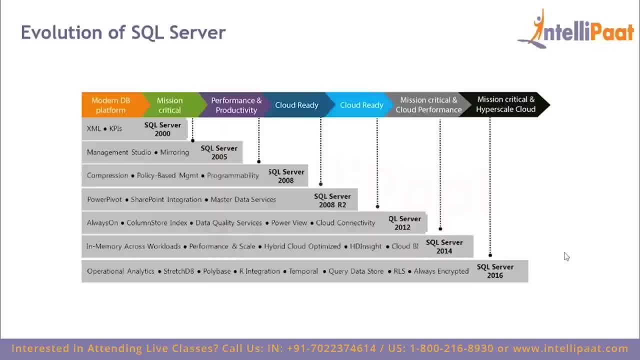 them on these platforms. This release also has support for Python, So our data scientists can now more easily perform machine learning right inside of SQL Server. Now let's look at the different editions of SQL Server. So first we have the Enterprise Edition. 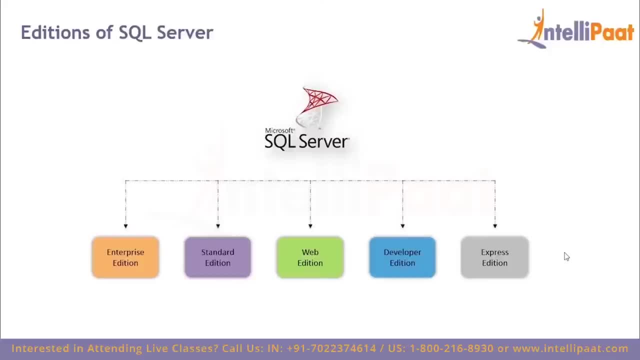 So SQL Server Enterprise Edition includes both the core database engine and add-on services, and with a range of tools for creating and managing a SQL Server cluster, So it can manage databases as large as 524 petabytes And it supports 640 logical processors. 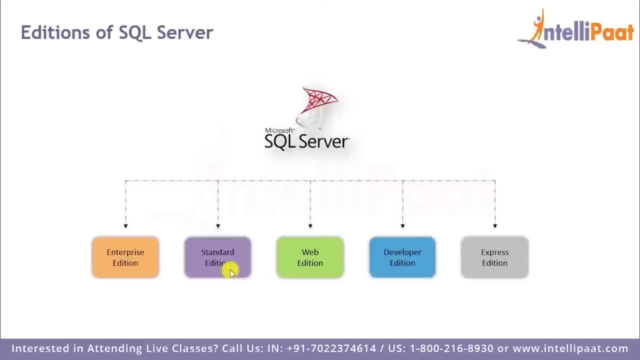 Then we have the Standard Edition. The SQL Server Standard Edition includes the core database engine along with the standalone services, So it differs from the Enterprise Edition in that it supports fewer active instances, that is, fewer number of nodes in a cluster. 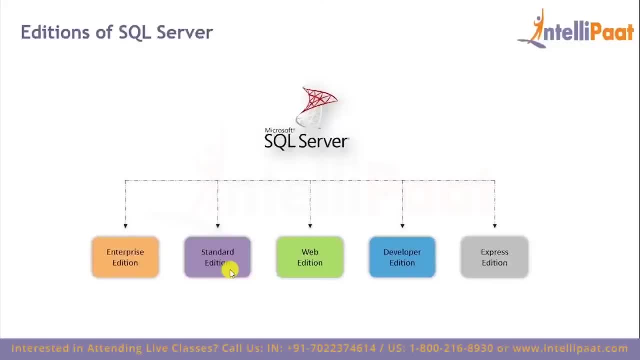 And it also does not include some high-availability functions such as hot-add memory and parallel indexes. Then we have the Web Edition, Which is just a little bit more advanced. So let's take a look at the Web Edition. It's a low-TCO option for web hosting. 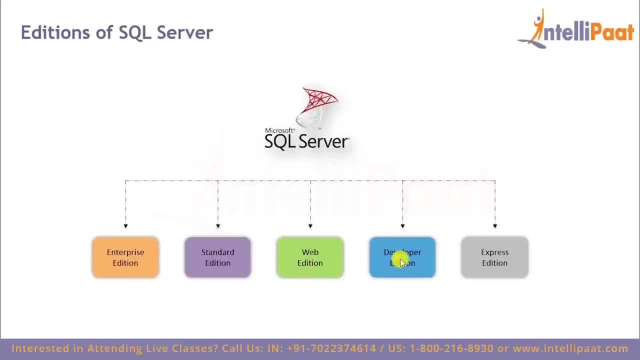 And then we have the Developer Edition. So this edition includes the same features as Enterprise Edition, but it is limited by the license to be only used as a development and test system and not as a production server. And finally we have the Express Edition. 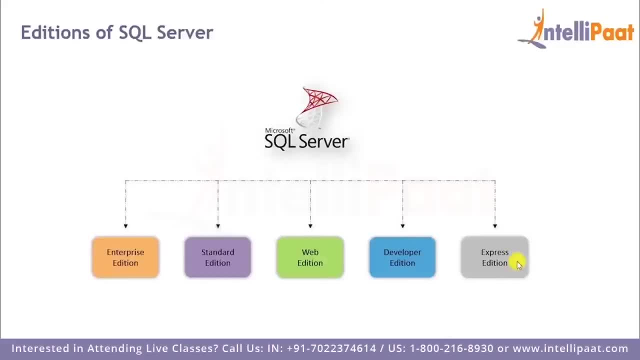 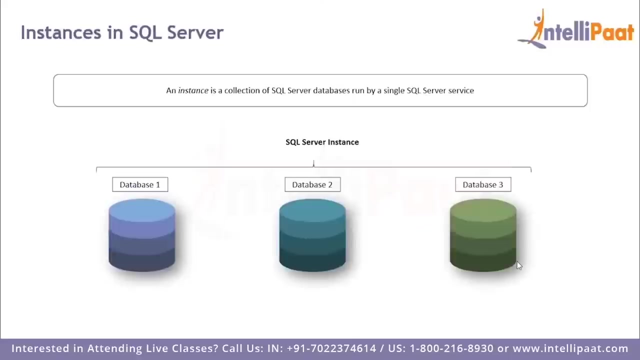 So it is basically a scaled-down free edition of SQL Server, which includes the core database engine. While there are no limitations on the number of databases or users supported, it is limited to using 1 processor, 1 GB memory and 10 GB database files. 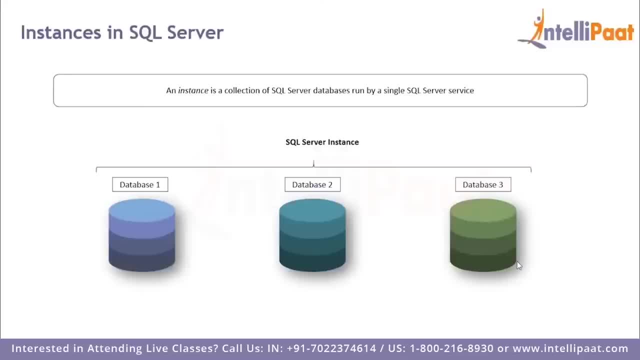 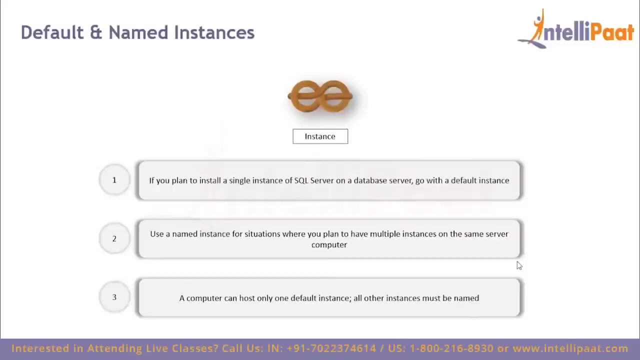 Now let's learn about instances. So you can consider an instance to be one complete installation of SQL Server, And each instance manages several system databases and one or more user databases. So an instance is either the default named instance or it is a named instance. 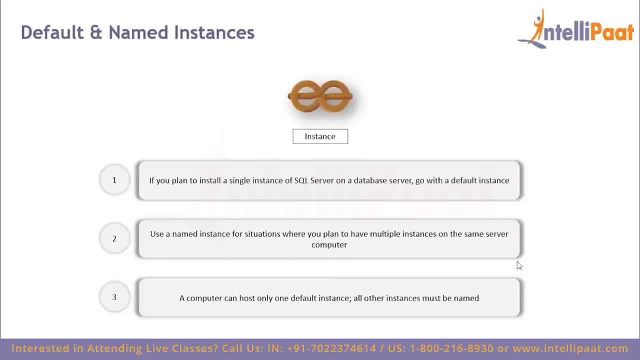 A default instance does not require a client. It does not require a client to specify the name of the instance to make a connection. But a named instance is identified by the network name of the computer plus the instance name that you specify during installation. So the client must specify both the server name and the instance name when connecting. 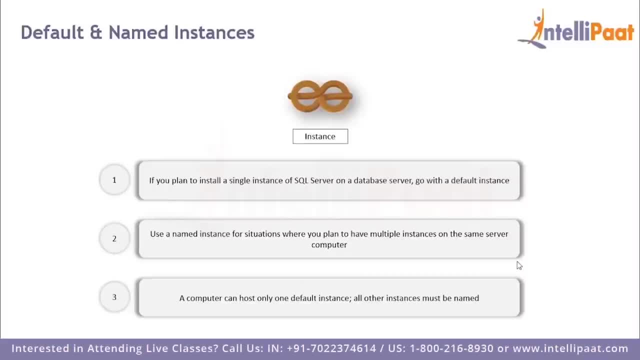 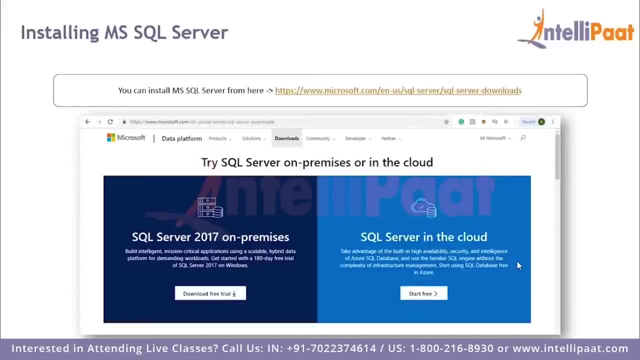 And a computer can have only one default instance and all the others must be named. Now let's go ahead and install SQL Server into our systems. So we can install SQL Server from this Over here: Microsoft SQL Server- SQL Server downloads. So I'll click on this link. 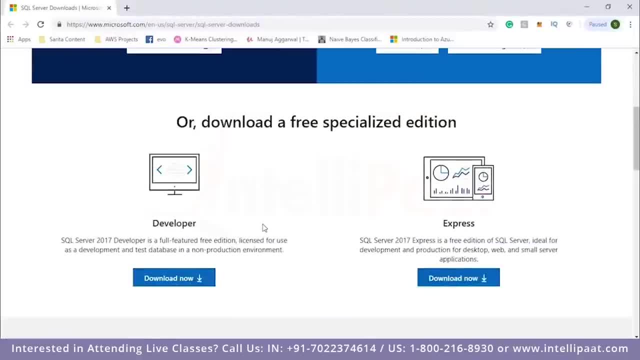 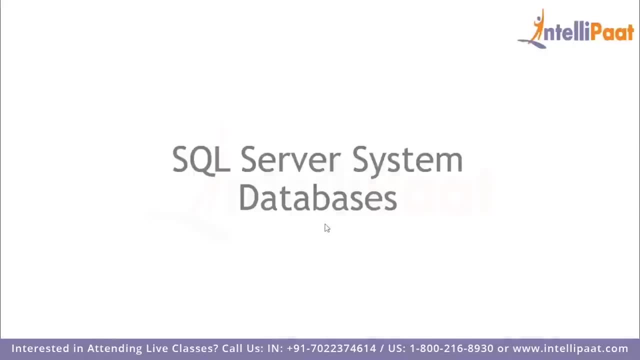 So this is the website, And for this course I'll be using the developer edition, So all I have to do is click on download now and it'll be downloaded. Now let's look at the different system databases in SQL Server. So when we install Microsoft SQL Server, the system databases are automatically created. 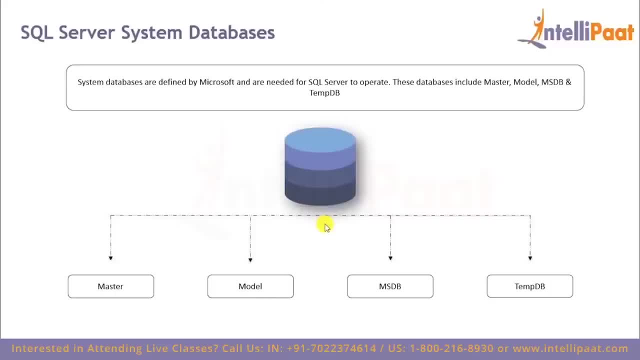 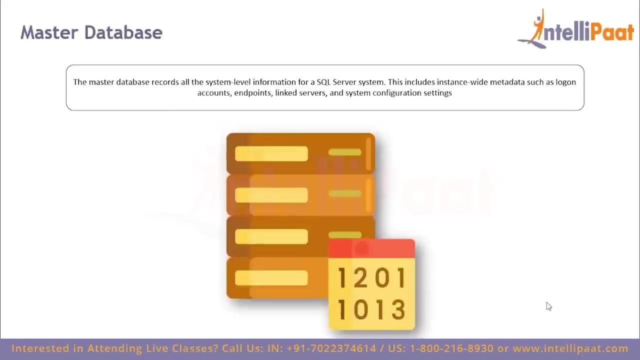 on every SQL Server instance. These system databases allow the database engine and administrative applications to properly manage the system. And these are the available system databases: Master Model, MSDB and TempDB. So let's start with Master Database. The Master Database contains all of the system level information for SQL Server. 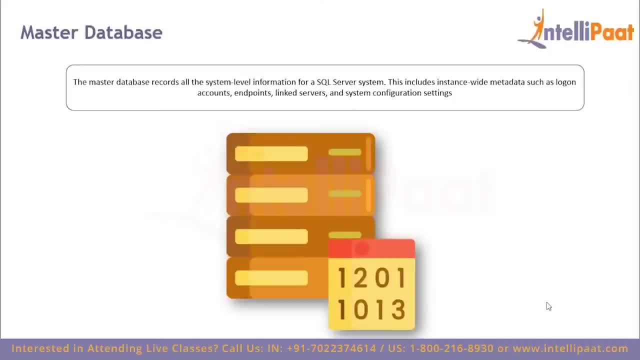 All of the logins, linked servers, endpoints and other system-wide configuration settings. The Master Database is also where SQL Server stores information about the other databases on this instance and the location of their files. So if the Master Database is not present, SQL Server cannot start. 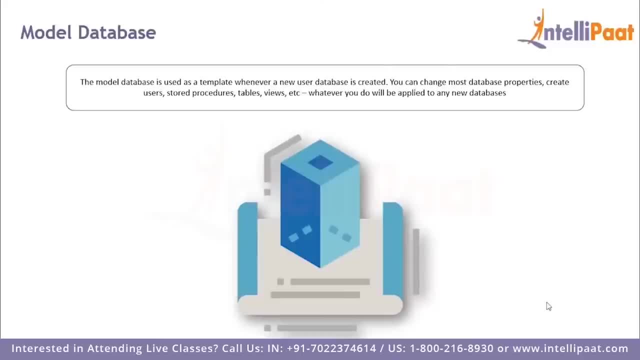 Then we have the Model Database. So the Model Database is used as a template whenever a new user database is created. So modifications made to the Model Database, such as database size, collation, recovery model and other database options, are applied to any databases created afterward. 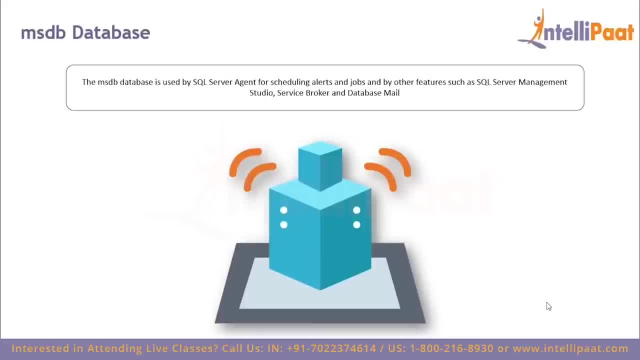 Then we have MSDB, which is used by SQL Server. It is used by SQL Server agent for scheduling, alerts and jobs, So MSDB also holds backup history. So using the MSDB tables it's possible to determine when each database and file group 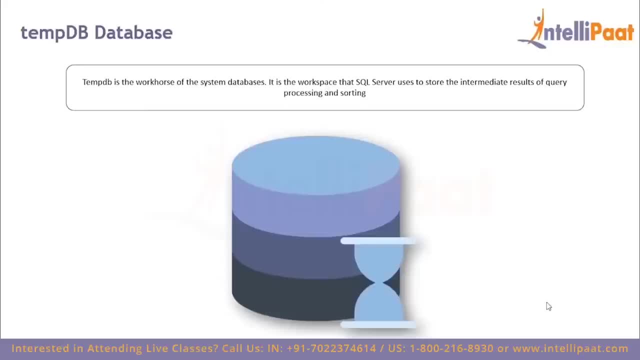 was last backed up. Then we have TempDB, which is basically a workspace for holding temporary objects or intermediate result sets. One interesting thing about TempDB is that it is recreated every time the SQL Server service is started. Any objects that we've created in TempDB will be gone once the server restarts. 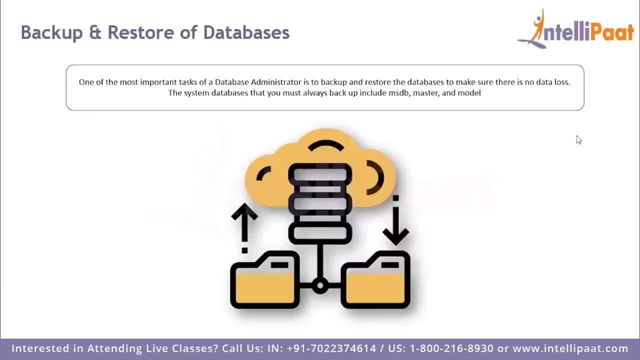 So one of the most important tasks of a database administrator is to backup and restore the databases to ensure that there is no data loss, And for this purpose, the SQL Server backup and restore component provides an essential safeguard for protecting critical data stored in our SQL Server databases. 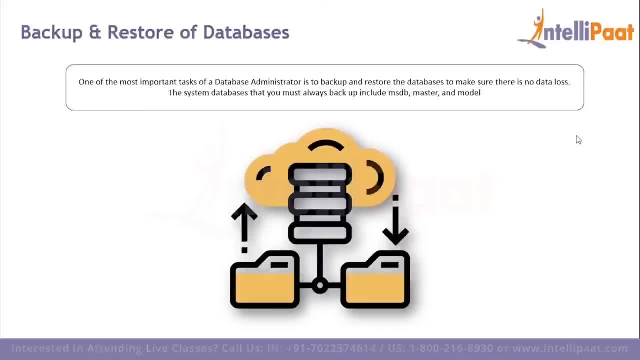 So, to minimize the risk of catastrophic data loss, we need to backup our databases to preserve modifications to our data on a regular basis, And this is where a well-planned backup and restore strategy helps in protecting our databases against data loss caused by a variety of failures. 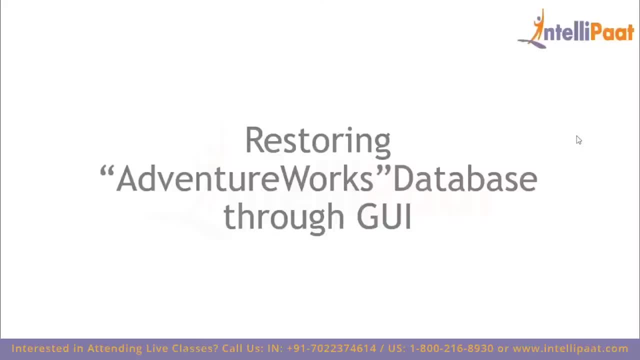 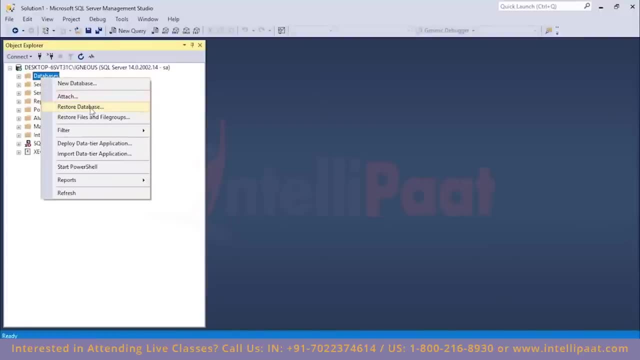 Now it's time to restore and backup the AdventureWorks database. So I will right click on this databases folder over here And, since I want to restore the AdventureWorks database, I will select this option- restore database- and I will set the source to be device and I will add a device. 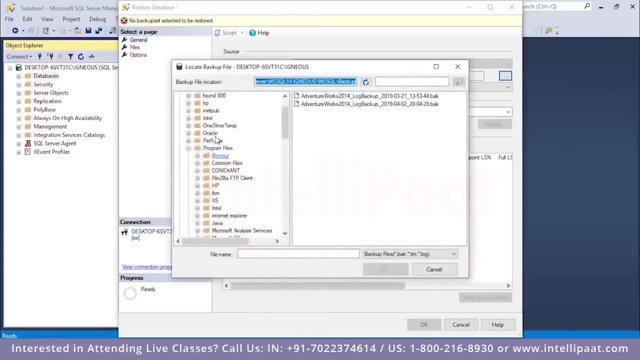 And that would basically be the file which I have to add. So I will go to the D drive. So inside D drive I have this AdventureWorks folder And this is my database over here: AdventureWorks 2014.. I'll click on, OK. 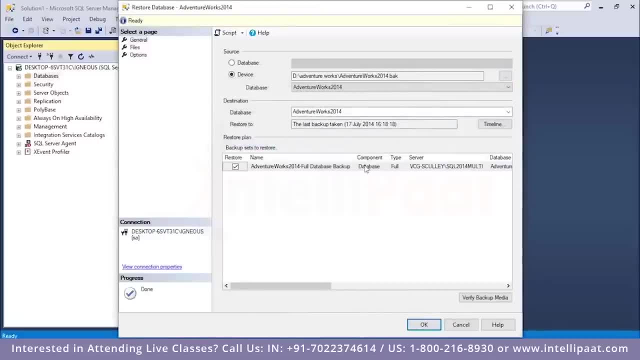 Again. I'll select this and I'll click on OK. So I have successfully added this AdventureWorks 2014 database. Now I'll click on OK And I'll just wait for the database to be restored. Right, so we get this message: that database AdventureWorks 2014 has been restored successfully. 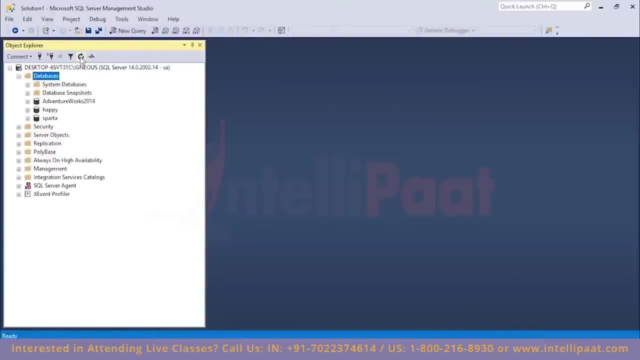 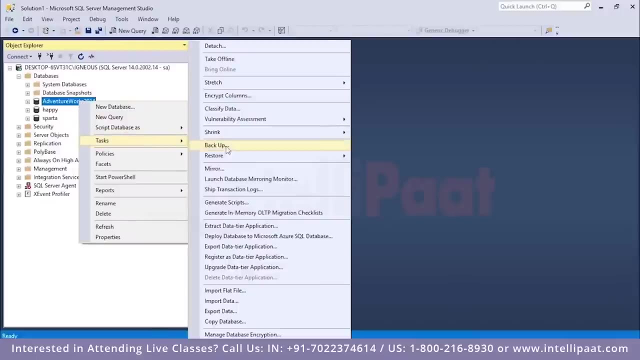 Now, if I open this databases folder, I will refresh this and we see that we have this AdventureWorks 2014 database over here. Now my next task would be to make a backup of this database. So for that purpose, I will right click on this and then select tasks, and I have this. 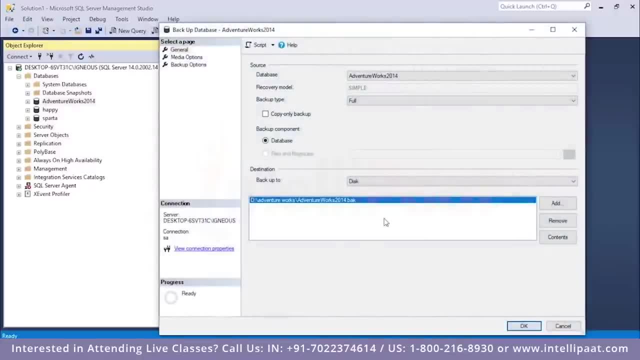 option of backup. I'll select this Now I will remove all of the previous backup models which I had created, So I will select this. I'll click on remove Now. I will click add and add a new backup. Let me name that to be new backup. 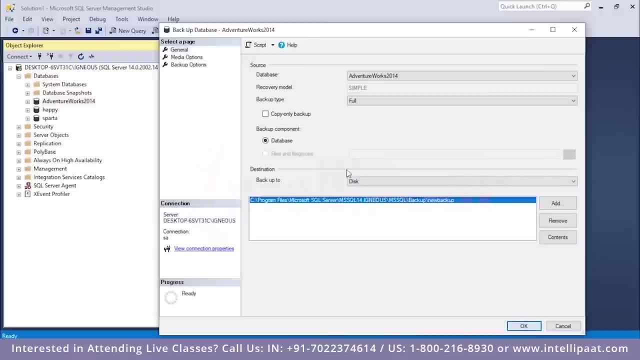 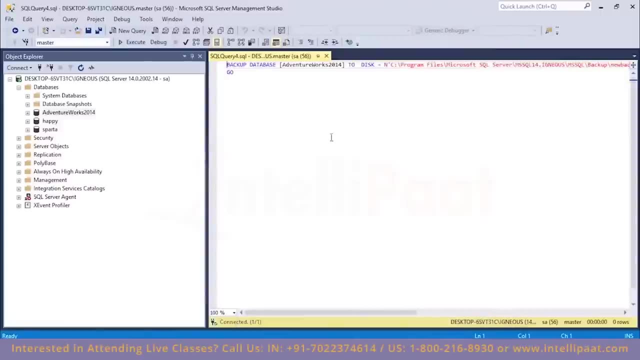 I'll click on OK. Now again, if I want the TSQL code for this, all I have to do is select the script And this would be the TSQL code to get a full backup of this AdventureWorks database. So now I'll select OK. 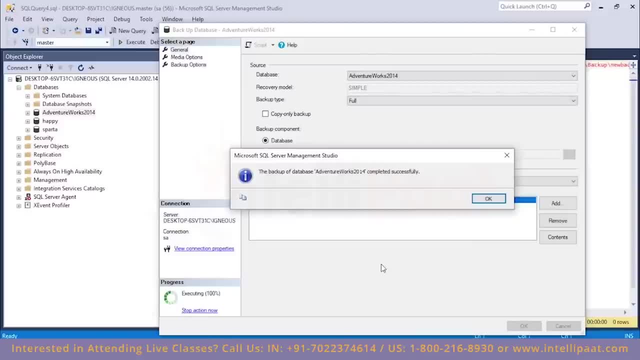 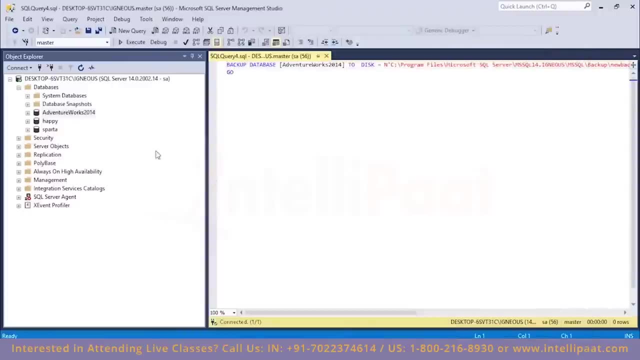 Again, let me wait till the backup is completed. So we get this message that the backup of database AdventureWorks 2014 has been completed successfully, Right, So first we went ahead and restored this AdventureWorks 2014 database And after that I made a full backup of this database. 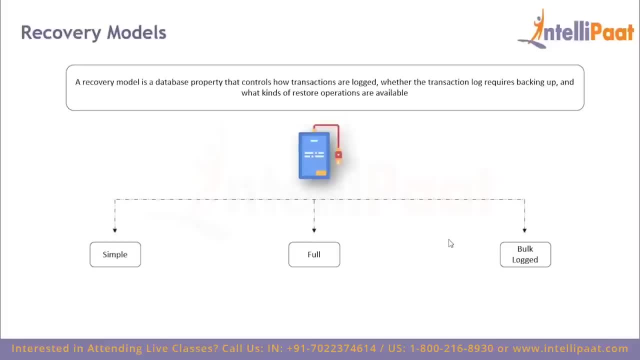 Now let's look at recovery models. So recovery model is basically a database property that controls how transactions are logged, whether the transaction log requires or not The transaction log requires backing up and what kinds of restore operations are available, And all of the backup, restore and recovery operations are based on one of these three. 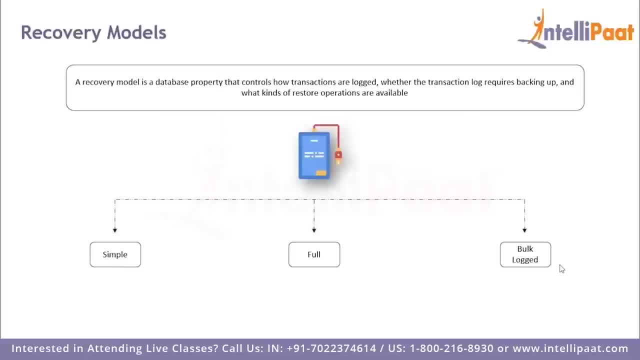 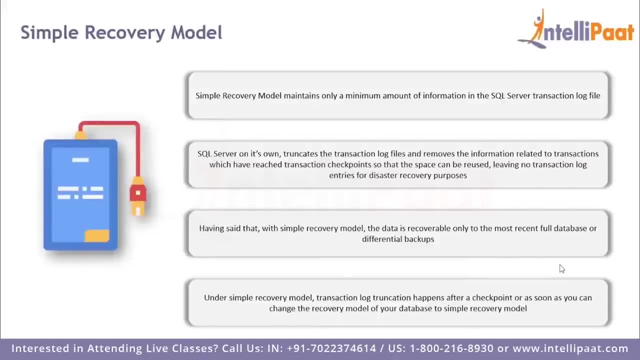 available recovery models which are simple, full and bulk logged recovery models. So let's start with simple recovery model. Well, as the name suggests, it is the simplest among the available models. So when we choose the simple recovery model, SQL Server maintains only a minimum amount. 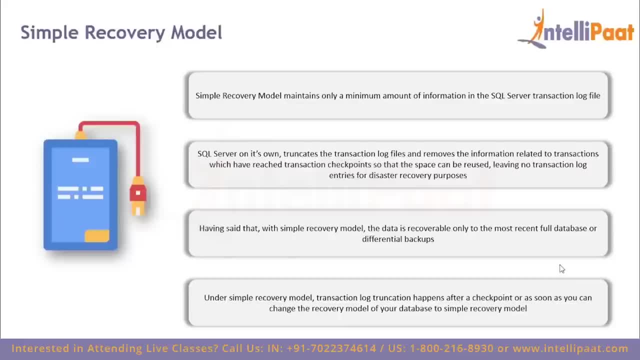 of information in the transaction log And while using the simple recovery model, we may restore full or differential backups only. So it is not possible to restore such a database to a given point in time, And we may only restore it to the time when a full or differential backup occurred. 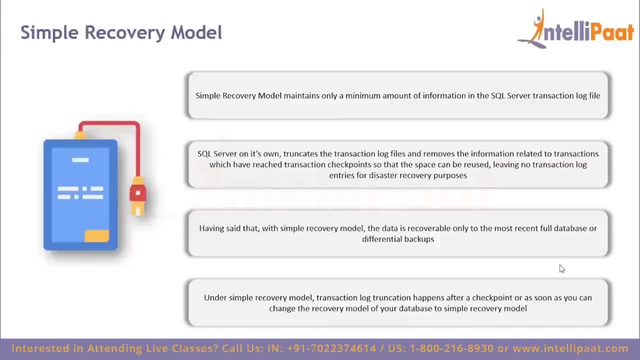 Therefore it will automatically lose any data modifications made between the time of the most recent full or differential backup and the time of the failure. So the simple recovery model requires very less administration And it is easier to manage in the full or bulk log models. 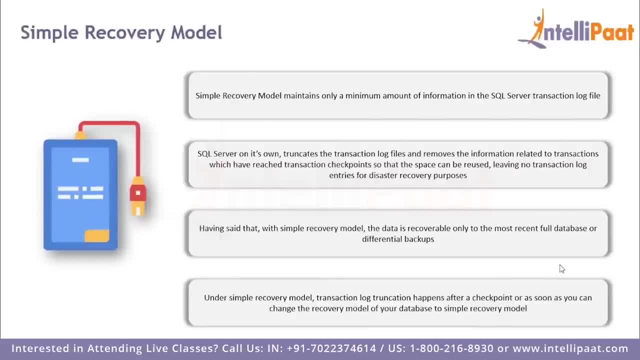 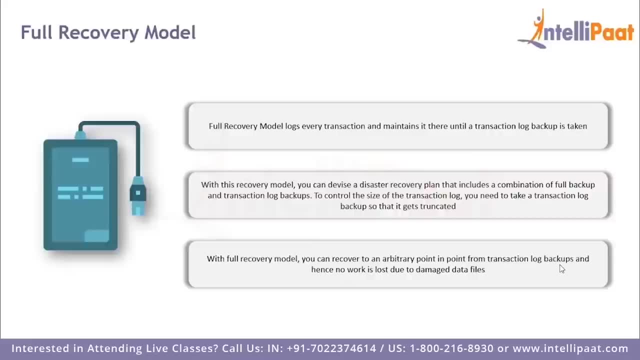 But there would be higher data loss if a data file is damaged. So next we have full recovery model. So with the full recovery model all the transactions are fully recorded in the transaction log file And this allows us to design a disaster recovery plan that includes a combination of full and 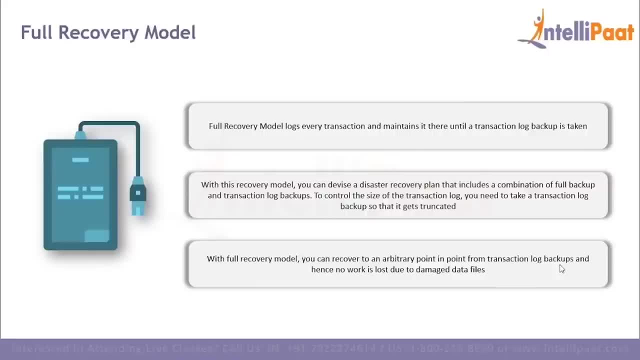 differential database backups in conjunction with transaction log backups, And, in addition to preserving data modifications stored in the transaction log, the full recovery model also allows us to restore a database to a specific point in time, And hence no work is lost due to a damaged file. 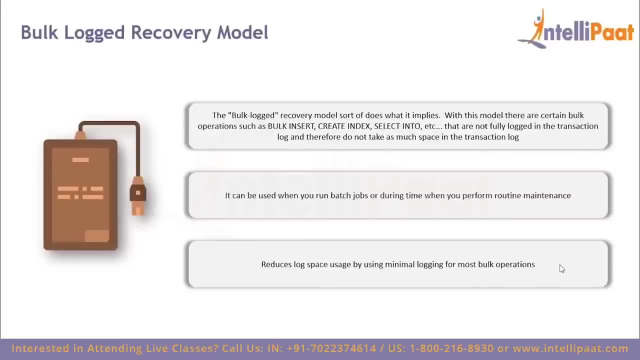 Next we have bulk log model. The bulk log recovery model is a special purpose model that works in a similar manner to the full recovery model. The only difference is in the way it handles bulk data modification operations. So the bulk log model records data. 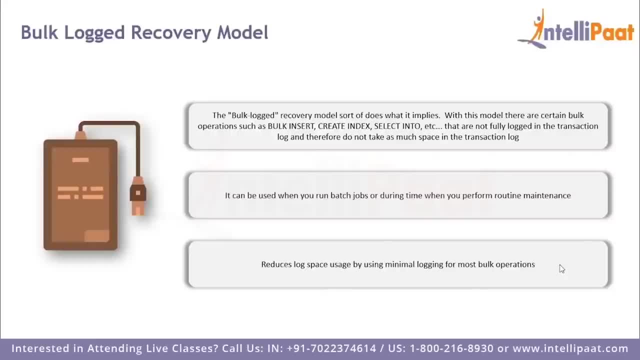 And the full recovery model records these operations in the transaction log using the technique known as minimal logging. So this saves significantly on processing time, but prevents us from using the point in time restore option. So now let's change these recovery models in SSMS. 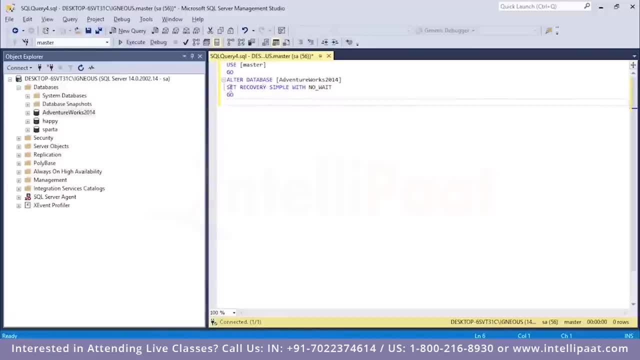 So this would be the command to set the recovery model to be simple. So set recovery simple with no wait. go, Let me just execute it So see that commands have been completed successfully. Now, if I want to change this recovery model from simple, 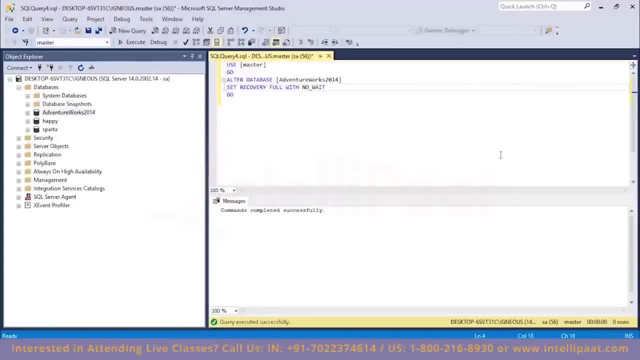 To full. All I have to do is write full over here. Now I'll click on execute. So this time we have changed the recovery model from simple to full. Now again, if I want to change this recovery model from full to bulk log, 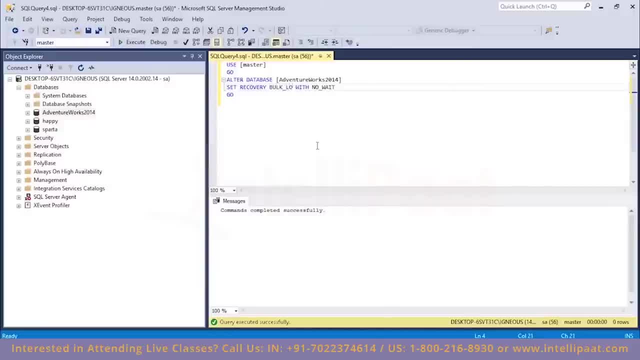 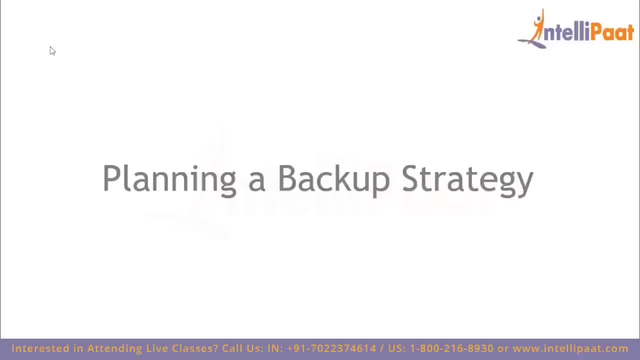 All I have to do is type in bulk underscore logged over here. I'll click on execute Right. so this time the recovery model which we are using is bulk logged. Now let's see how can we plan our backup strategy. So, after we have selected a recovery model, 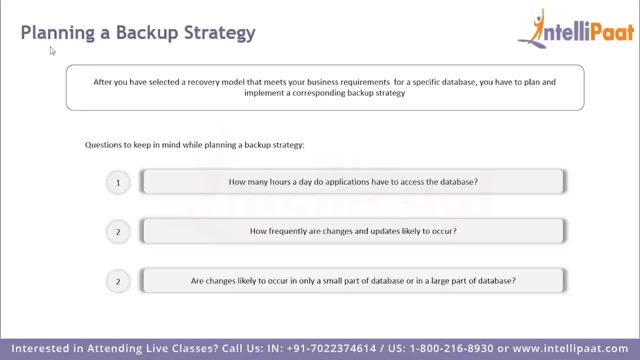 That meets our business requirements for a specific database, We'd have to plan and implement a corresponding backup strategy. So these are some of the questions which we'd have to keep in mind While planning a backup strategy. How many hours a day do applications have to access the database? 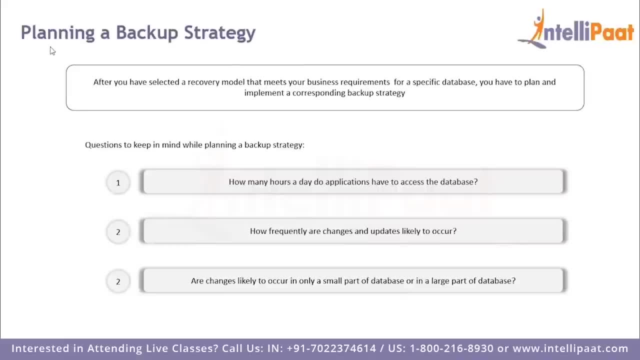 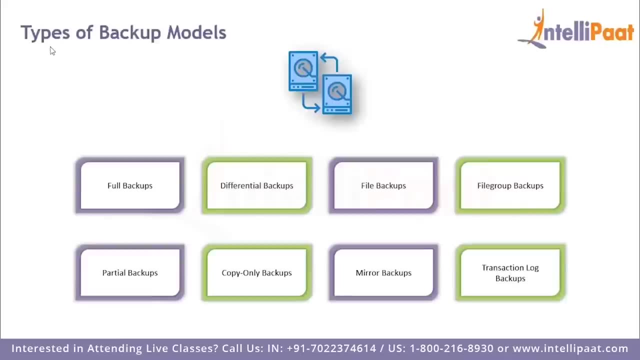 And how frequently are changes and updates likely to occur, And are these changes likely to occur in only a small part of the database Or in a large part of the database? And these are the different types of backup models Which we can use. 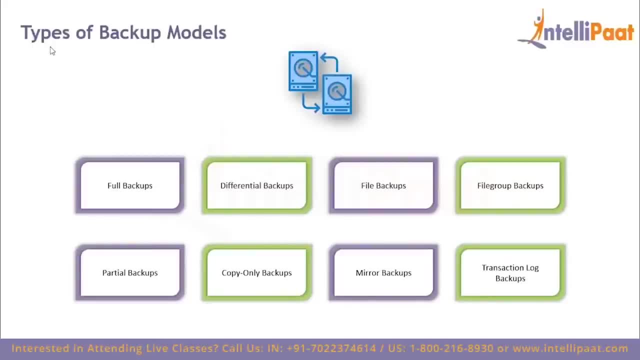 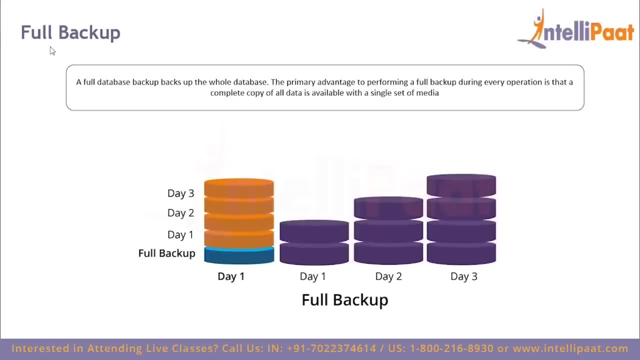 So we have full backups, Differential backups, File and file group backups, Partial backups, Copy only backups, Mirror backups And transaction log backups. So a full backup, as the name implies, Backs up everything. It is the foundation of any kind of backup. 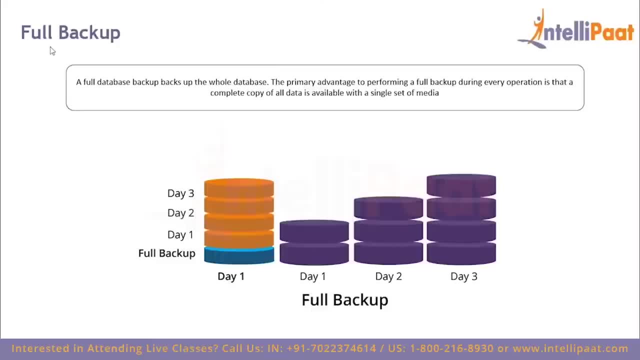 So this is a complete copy Which stores all the objects of the database, That is, tables, procedures, functions, views, indexes, So basically everything. So the full backup will be able to easily restore a database in exactly the same form as it was at the time of the backup. 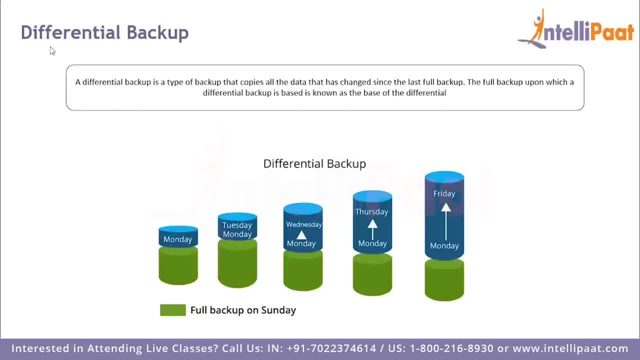 Then we have differential backup, So you can consider a differential database backup to be the superset of the last full backup And it contains all changes that have been made since the last full backup. So if there are very few transactions that have happened recently, 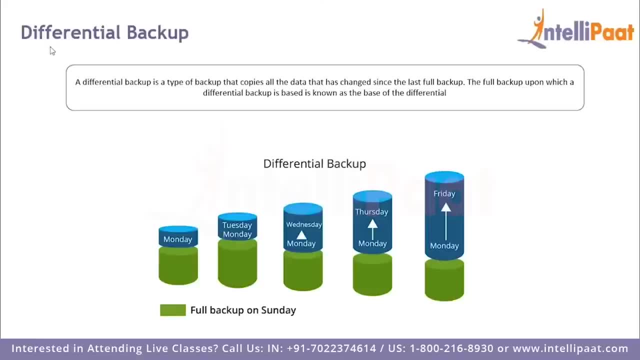 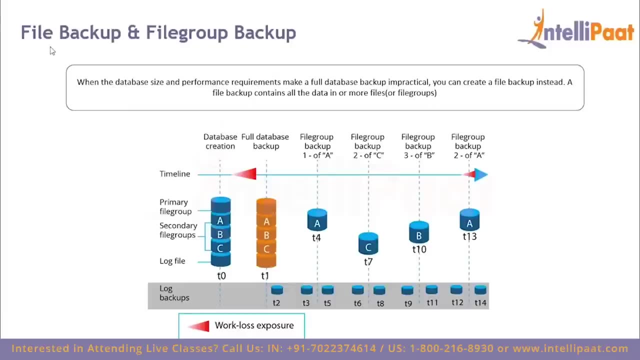 A differential backup might be small in size, But if you made a large number of transactions The differential backup could be very large in size. Then we have file and file group backup. So whenever the database size and performance requirements make a full database backup impractical, 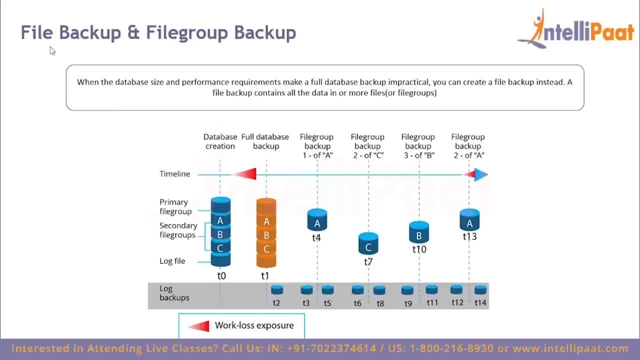 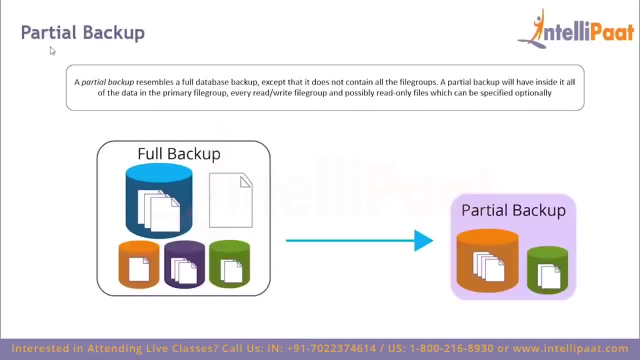 We can create a file backup instead. So a file backup contains all the data in one or more files, which are known as file groups. Then we have partial backup. So partial backups allow us to backup only a subset of the data files. So these partial backups, 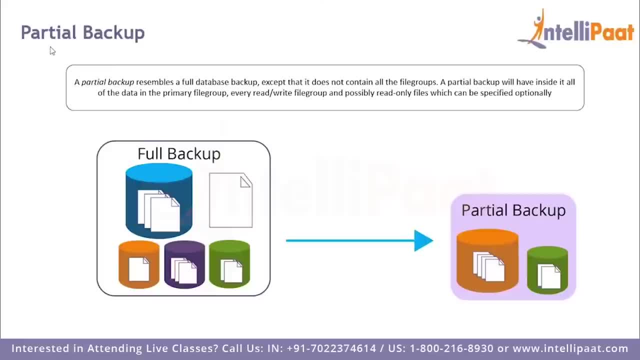 Will make a backup copy of the primary file group And all read write file groups And by default, they will omit any file groups designated as read only. This means that partial backups are only relevant for databases that contain read only file groups. Otherwise, a partial backup will capture exactly the same data and objects as an equivalent full database backup. 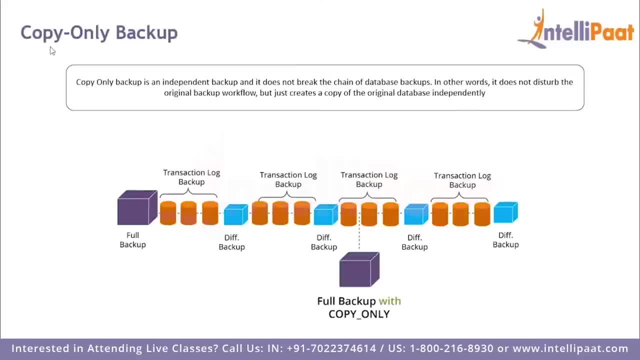 So next we have copy only backup. So a copy only backup is a SQL Server backup That is independent of the sequence of conventional SQL Server backups. Usually, taking a backup changes the database and affects how later backups are restored. However, occasionally it is useful to take a backup for a special purpose. 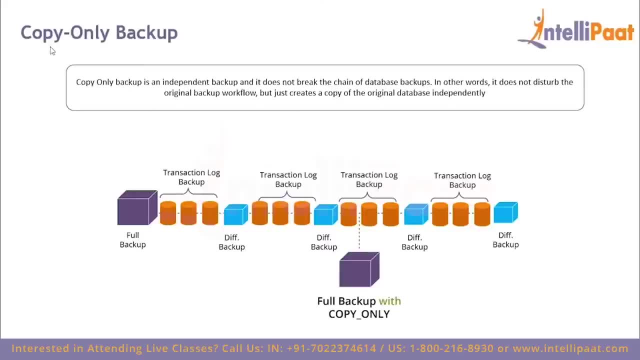 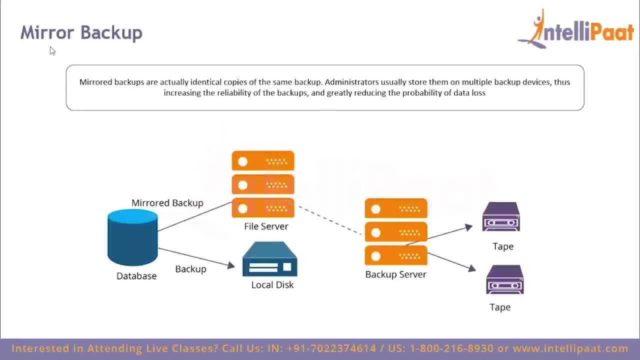 Without affecting the overall backup and restore procedures for the database, And this is exactly where a copy only backup can be used. Then we have mirror backup, So mirror backups are Actually identical copies of the same backup, And these identical copies are stored on multiple locations. 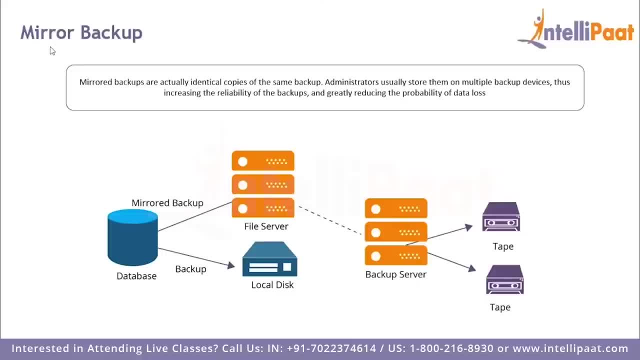 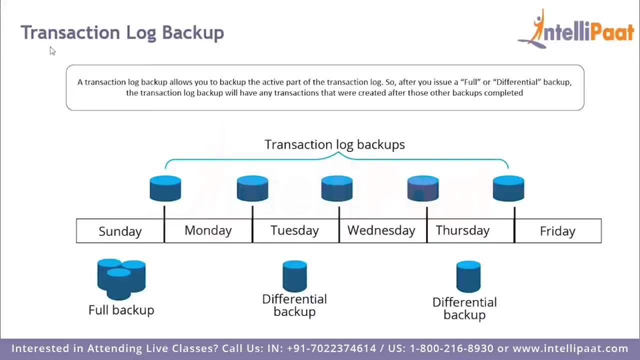 So this increases the protection level By having additional copies of the backup set And in case one of the copies gets lost or is corrupted, We can use the mirrored copy to perform a restore. So, finally, we have the transaction log backup. So a transaction log backup allows us to backup the active part of the transaction log. 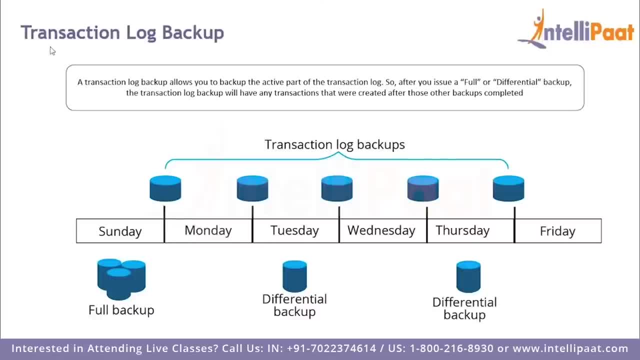 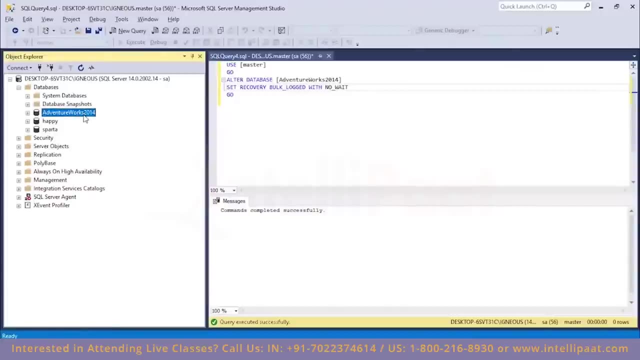 So after we issue a full or differential backup, The transaction log backup will have only those transactions That were created after those other backups had completed. So now let's implement backup models in SSMS. So now again, I will select this AdventureWorks database. 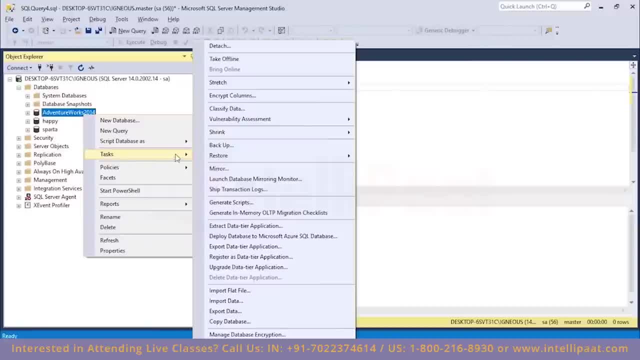 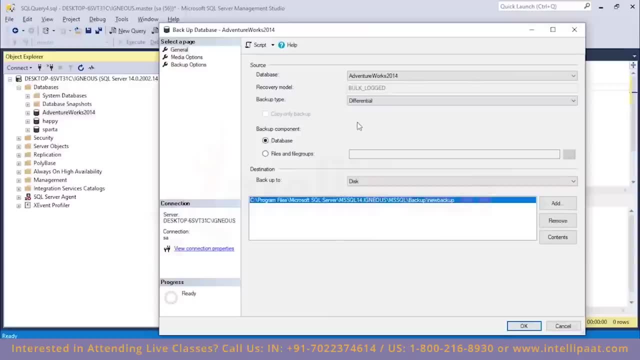 Right click on it, I will select tasks And since I want a backup, I'll click on backup. So this time I want a differential backup, So I'll select differential And all I have to do is Click on OK. And before that, if I also want the TSQL code for this. 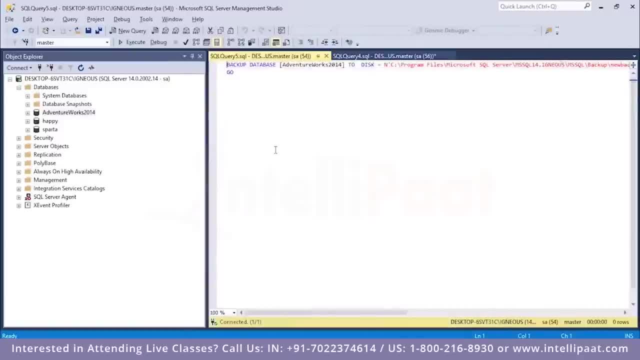 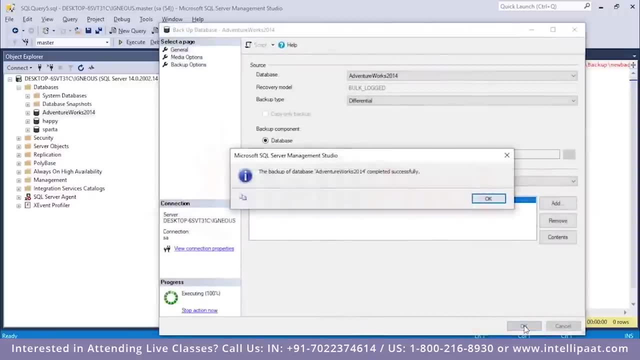 All I have to do is click on script, And this is the TSQL code, to get the differential backup of this database. I will click on OK. So you see that the backup of the database has been completed successfully. Now, similarly, if I want to get a transaction log backup, 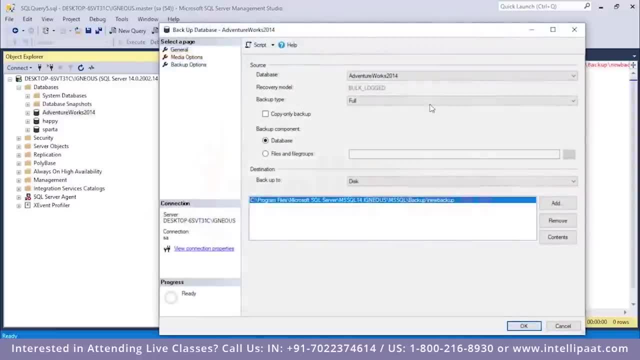 I'll right click this Tasks Backup And this time, instead of choosing full, I'll select transaction log And again, if I want the TSQL code, I'll click on script. So I'll just click on OK over here. So this time we have a transaction log backup of the AdventureWorks 2014 database. 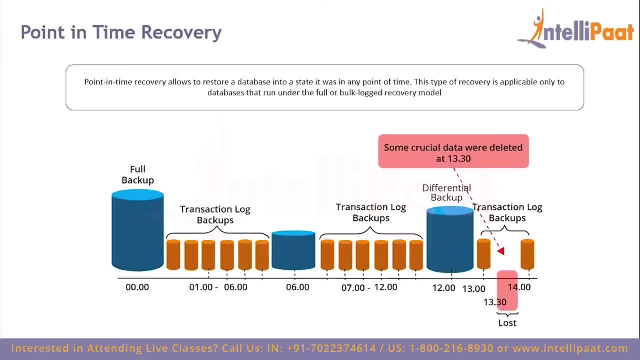 So now let's understand what is point in time recovery. So point in time recovery allows us to restore a database into a state it was in at any point of time. This type of recovery is applicable only to databases that run under the full or bulk logged recovery model. 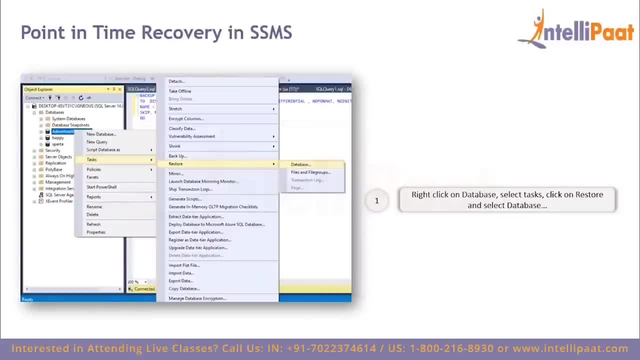 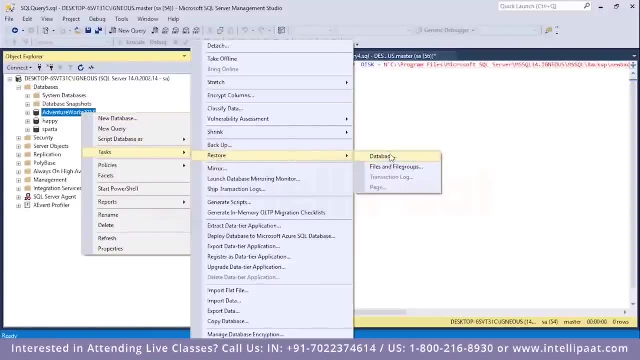 So now let's implement point in time recovery in SSMS. So I have this AdventureWorks 2014 database over here. I'll right click this, Select tasks, I'll click on restore Database And I have this timeline option over here. 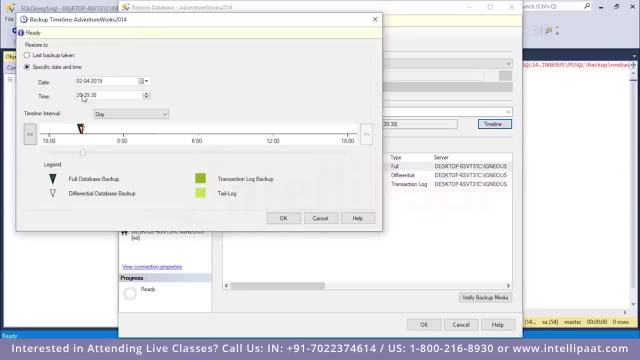 So I'll select timeline And I will set a specific date and time. So I want to recover this database from 2 hours back, So I'll set this to be 18. And I will click on OK Right. So this is how we can do point in time recovery. 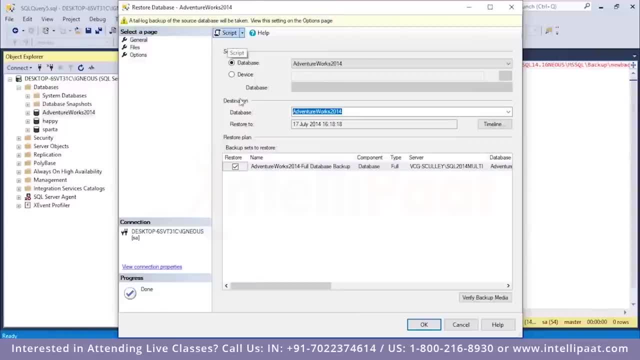 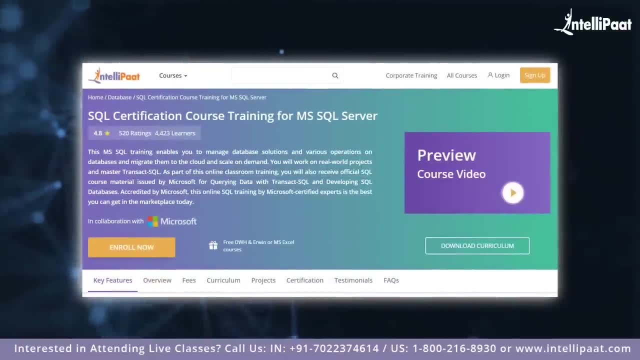 So again, if I want the TSQL code for this, all I have to do is click on script, But for now I'll click on OK. Just a quick info, guys. Intellipaat provides SQL online training in partnership with Microsoft and mentored by industry experts. 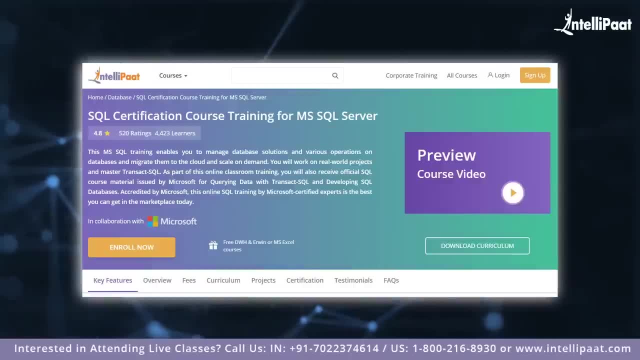 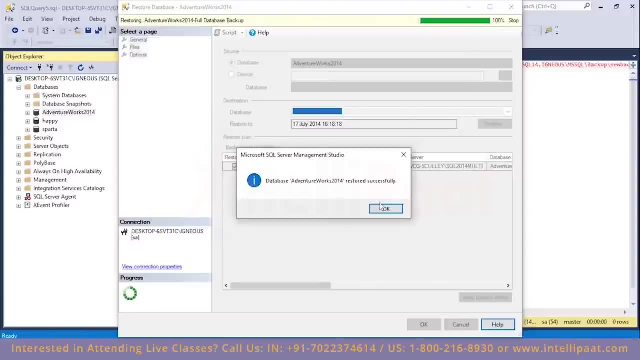 The course link is given in the description below. Now let's continue with the session. So we've successfully got the point in time recovery of this database for 2 hours back. Now we'll see how to import and export data in SSMS. 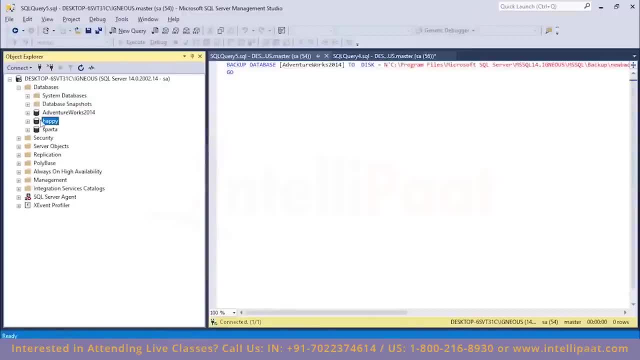 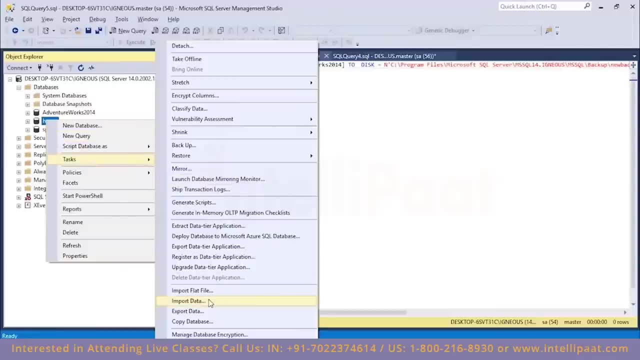 So I have this happy database over here And I want to import a flat file into this database. So for that I'll right click this. I have the option of tasks And over here I have to select import data. I have to set the data source. 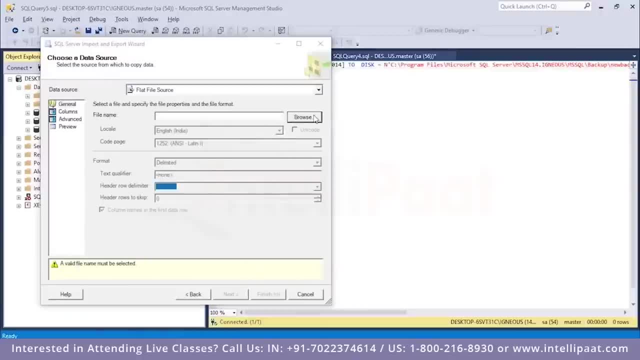 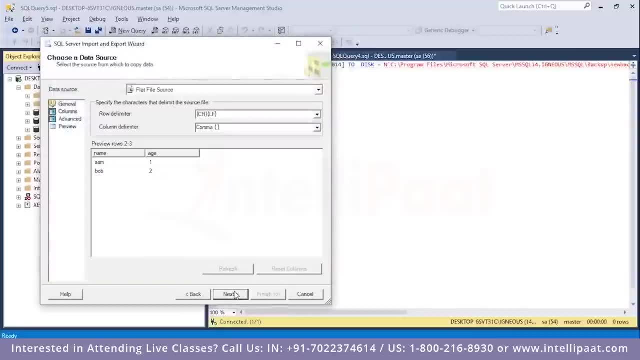 So the data source would be a flat file- Flat file source. Now let me browse that flat file. So I have this new file over here. I'll open this Now. all I have to do is keep clicking on next. So this is the data which is present in this flat file. 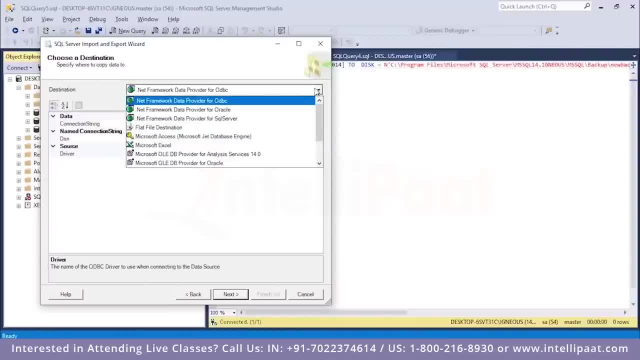 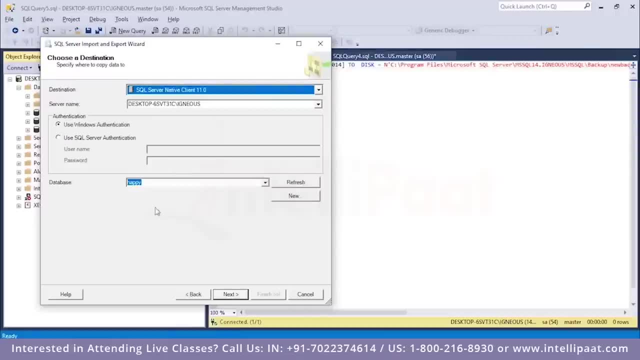 Click on next And then I'd have to set the destination. So I want to store this into my database. So the database would be SQL server native client. Now, this will be stored in this happy database. I'll click on next Next. 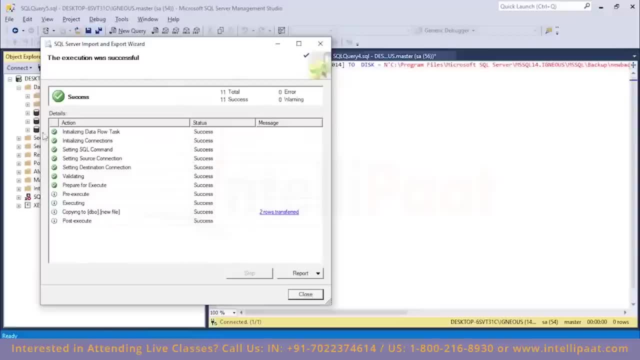 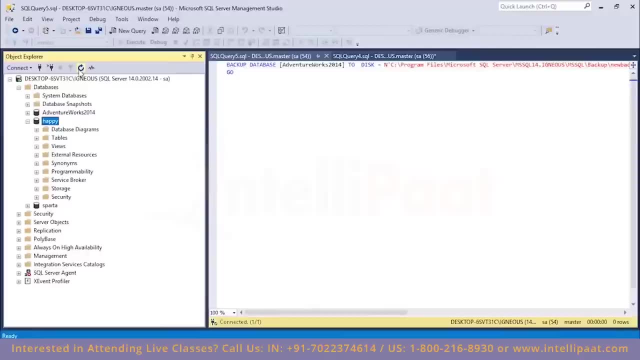 And I'll have to click on finish over here. So you see that we have successfully imported this flat file into our database. Now let me refresh this. Let me have a look at the tables over here. So we have imported this new file into this database. 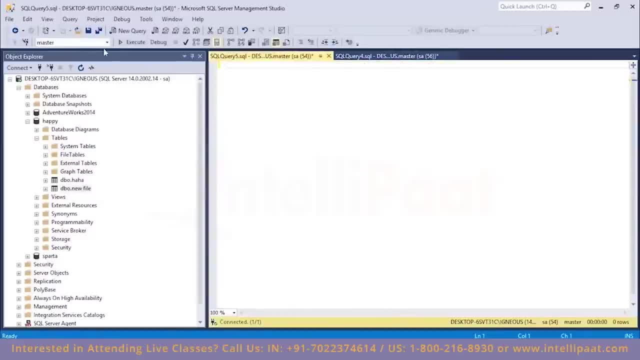 Now let me go to this database first, which would be happy over here. So select: start from new file. I'll execute. Right, So we have successfully imported the data set. Now what I'll do is add a new row to this file and export this into a new file. 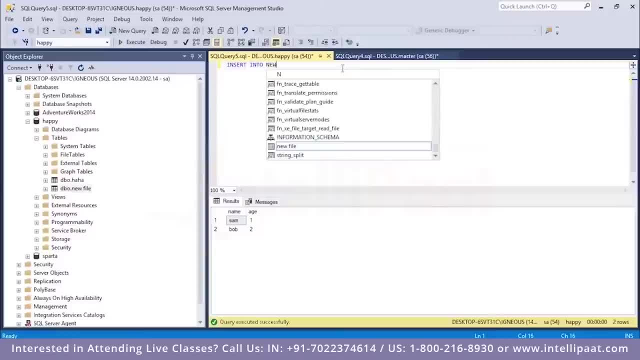 So insert Into New file. It will be values And then let's see the name is Ann And her age is three. I'll execute this. Now let me look at the modified data. So that will be: select star from new file. 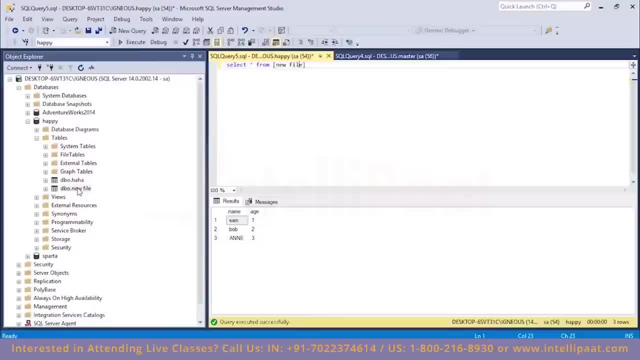 So we have successfully added this new record. Now I would want to export this data. So this time again, I will right click this database And I will select tasks over here. I have the option of exporting data Now. the source would be: 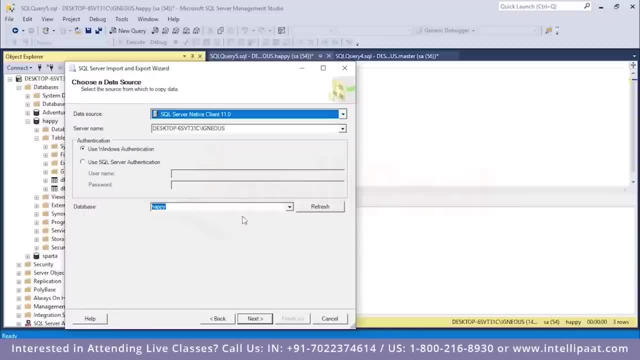 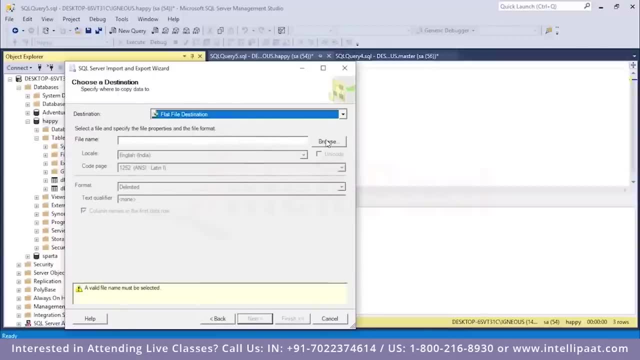 Sequel server native client. Now, this time the database is again happy. I'll click on next. I'd have to choose a destination, So the destination would be a flat file. I'd have to choose a file name over here, So I want to store this into a new file too. 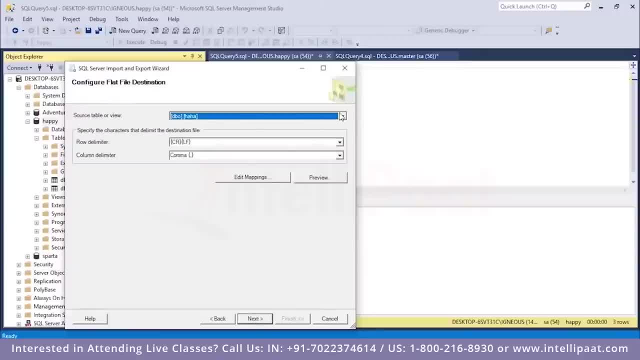 And I'll click on next, Next. So over here I'd have to choose the table which I want to export. So I want to export this new file. I'll click on next Now, next again, And I'll click on finish. 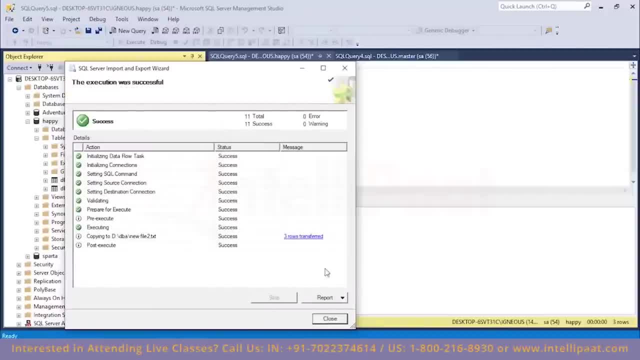 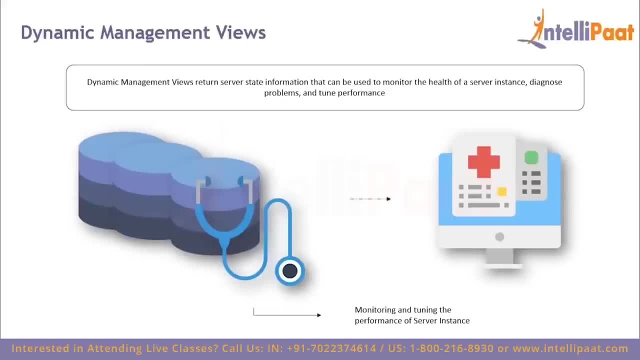 So this time we have successfully exported this data from SSMS. So dynamic management views and dynamic management functions are system views and system functions That return metadata of the system state On querying the related system objects. Database administrators can understand the internals of SQL. 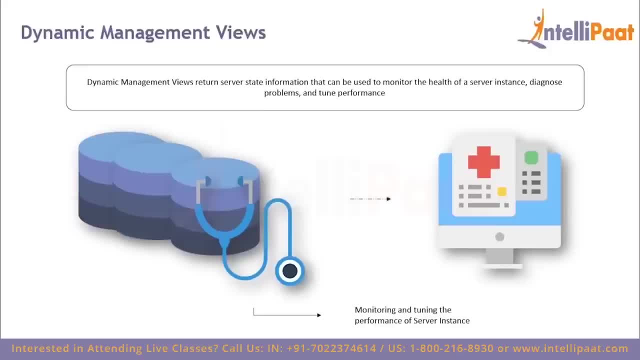 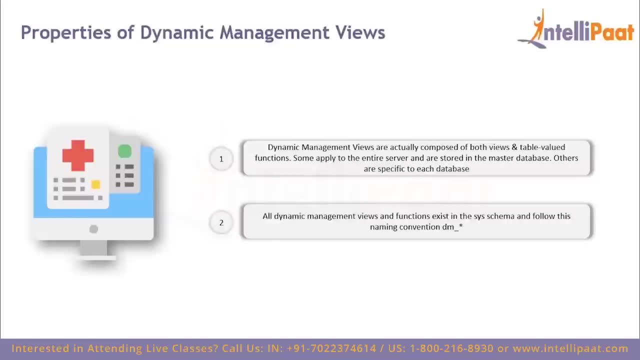 So these dynamic management views allow us to monitor the performance of SQL server instance and diagnose issues with it. Now let's look at some of the properties of dynamic management views. So dynamic management views are composed of both views and table valued functions. Some of them apply to the entire server and are stored in the master database. 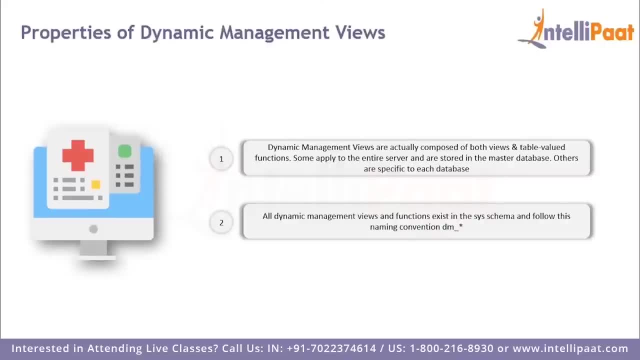 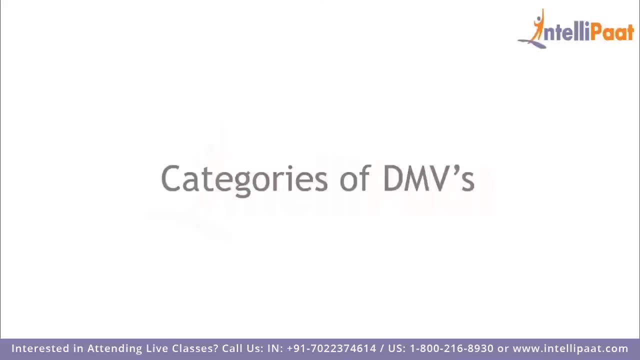 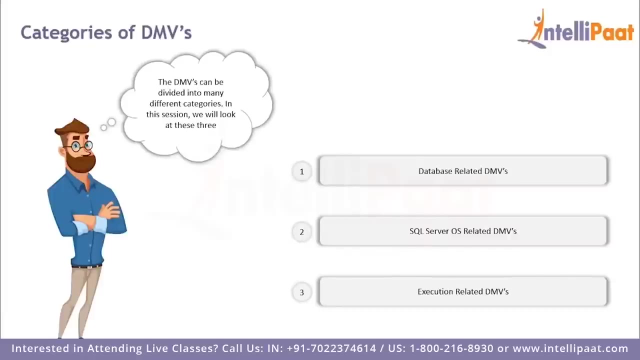 Others are specific to each individual database, And all of these DMVs start with the prefix DM underscore. Now let's look at some categories of DMVs. So DMVs can be divided into many different categories, And in the session we'll be looking at three of those. 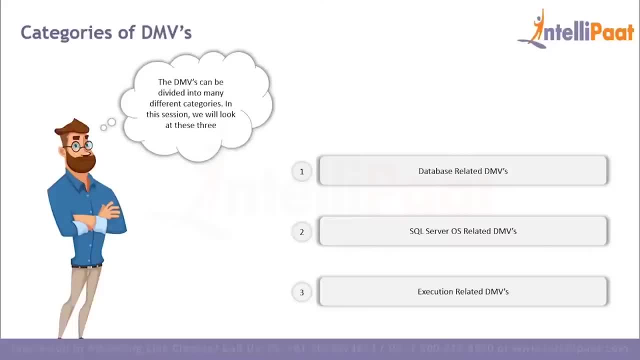 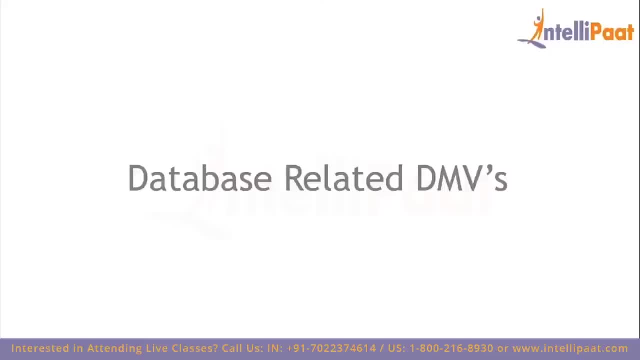 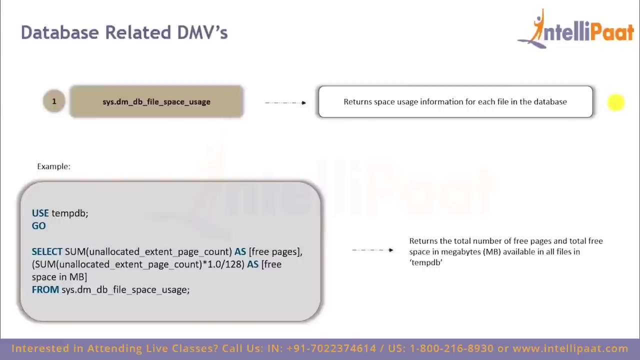 So we'll be looking at database related DMVs, SQL server, OS related DMVs And execution related DMVs. So let's start with database related DMVs First. we have DM, underscore, DB, underscore, file, underscore space usage, Which returns the space usage information. 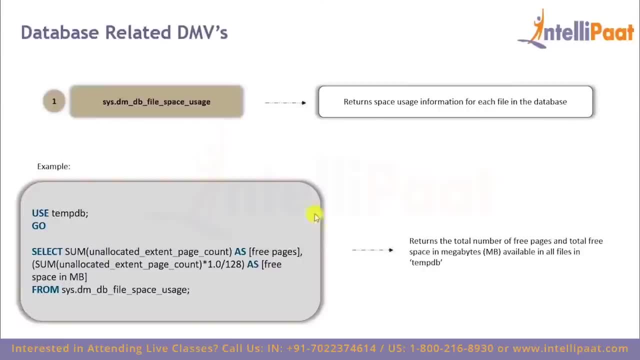 For each file in the database. Now we will use this DMV To get the total number of free pages And total free space in megabytes Available in all files in tempdb. So let me just run this command over here. I will click on execute. 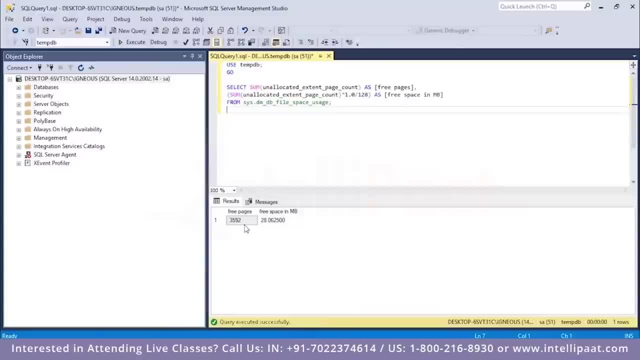 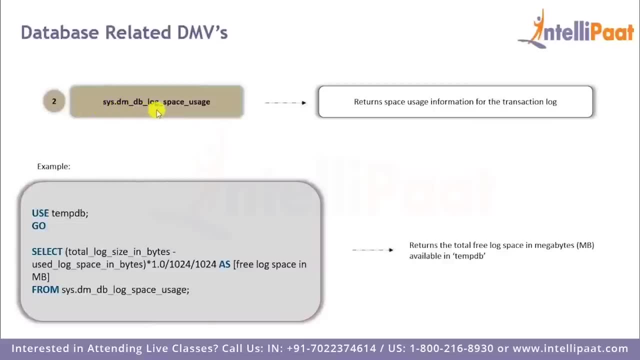 So the total number of free pages available in tempdb are 3592. And the total free space is 28 MB. Next, we have DM underscore, DB, underscore log, space usage, Which returns space usage information for the transaction log, And we will use this DMV to get the total free log space in megabytes. 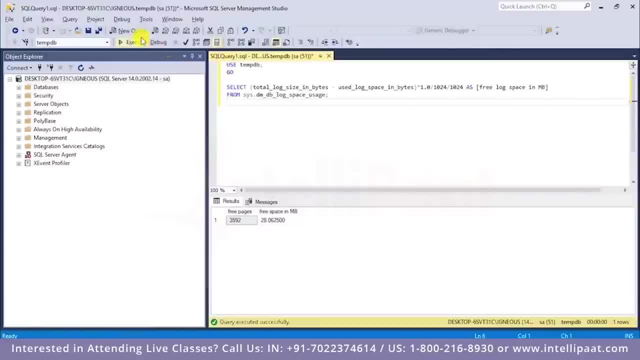 Available in tempdb. Now again, I will run this command in SSMS. I will click on execute So you see that the total free log space is 5.74 MB. So this is the total free log space in tempdb. Next we have DB underscore partition stats. 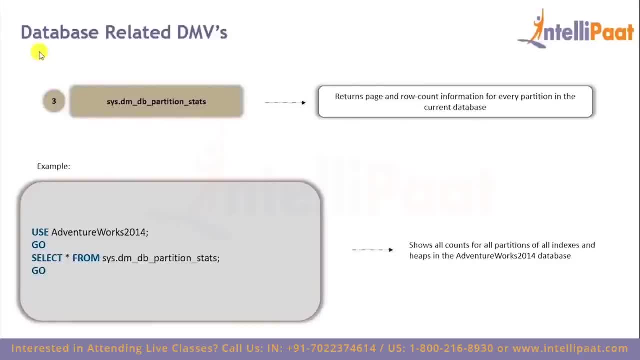 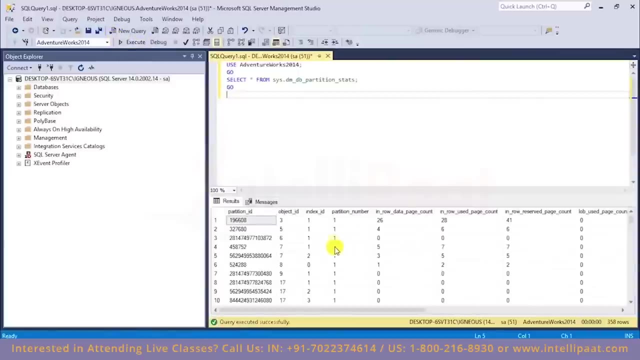 Which returns page and row count information for every partition In the current database. And this time we will get the counts for all partitions of all indexes And heaps in the AdventureWorks 2014 database. Let me click on execute. So these are all of the partition stats for all of the indexes. 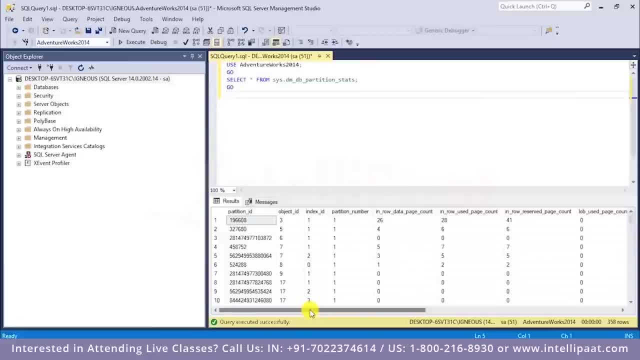 And heaps in the AdventureWorks 2014 database. So here we have different statistics, such as Index ID, partition number, the data page count and so on, And over here we have the reserved page count, the used page count, The row count. 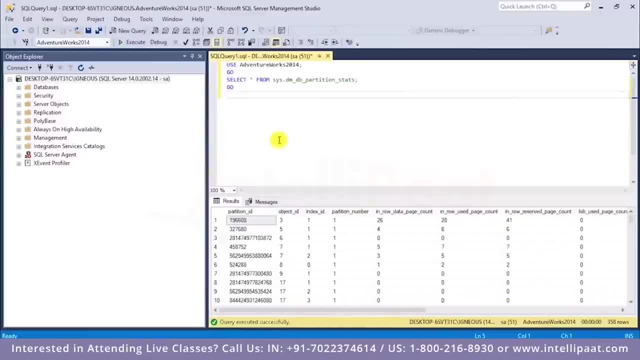 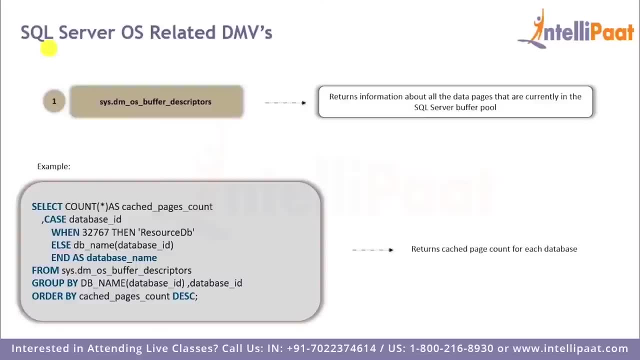 So these are all of the partition stats which we can get from this DMV. Next we will head on to SQL Server OS related DMVs. So first we have the DM underscore OS buffer descriptors, Which returns information about all the data pages That are currently in the SQL Server buffer pool. 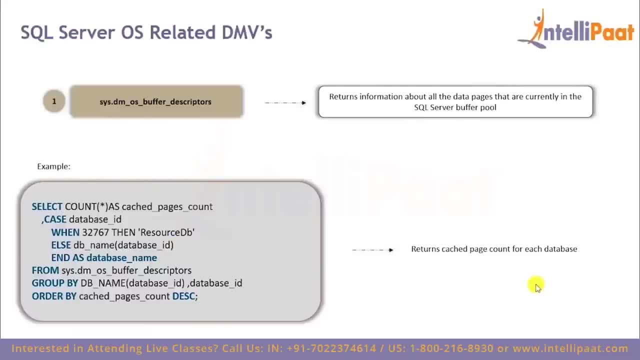 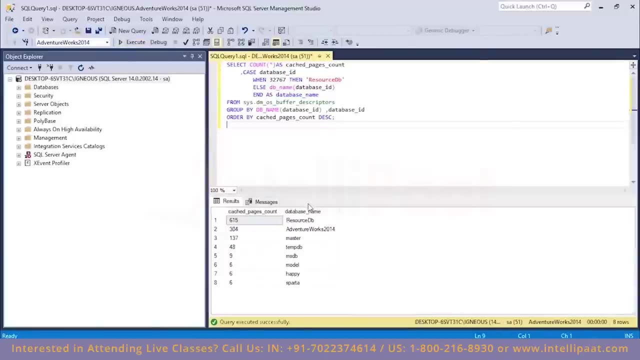 So with this command over here We will get the cached page count for each database. Again, I will run this command in SSMS. I will click on execute. So these are the different databases which I have in SQL Server And this is the cached page count. 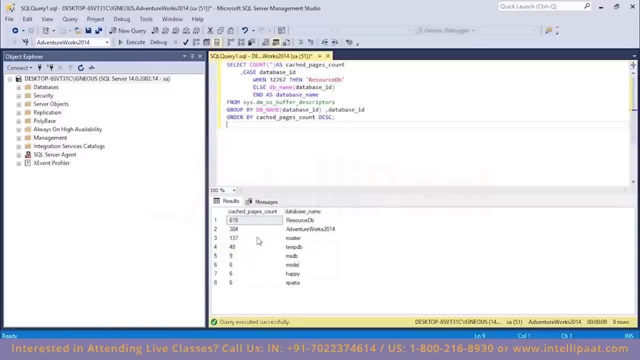 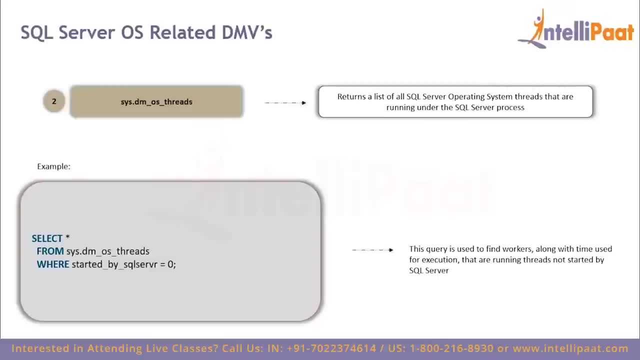 So in MasterDB I see that there are 137 cached pages, In MSDB there are 9.. In Spada there are 6. And in AdventureWorks there are 304.. Next we have DM underscore OS threads, Which returns a list of all SQL Server operating system threads. 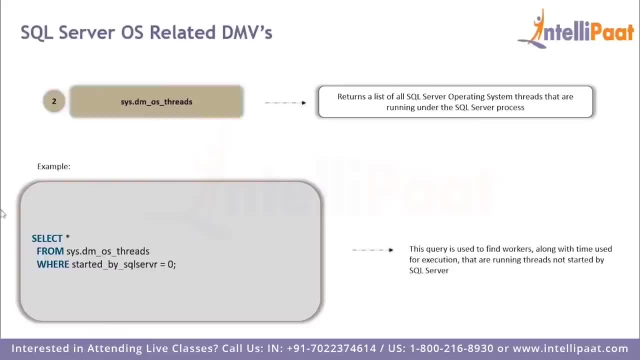 That are running under the SQL Server process. So this query over here is used to find workers, Along with time used for execution, And are running threads Which are actually not started by SQL Server. So this is all of the information about the threads. 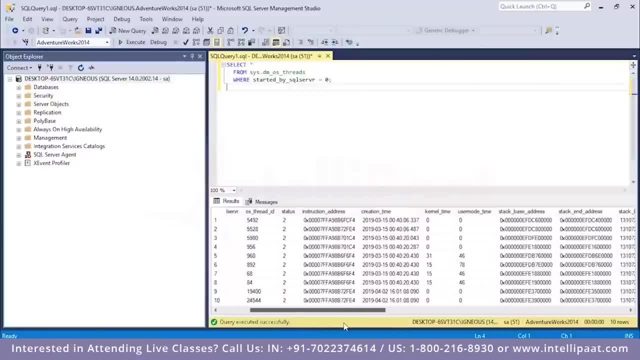 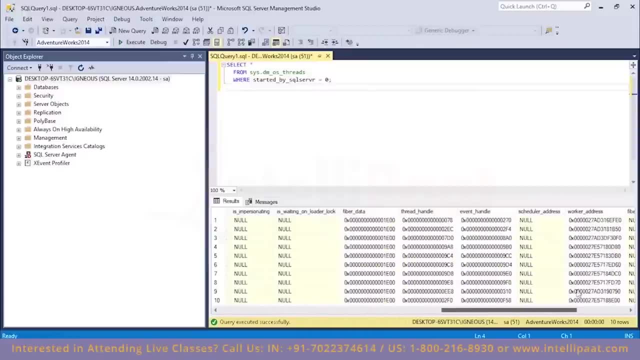 Which are not yet started by SQL Server. So we have different columns. We have the OS thread ID, The creation time over here, The kernel time, User mode time And over here at the back end of it We have got the address associated with each of these threads over here. 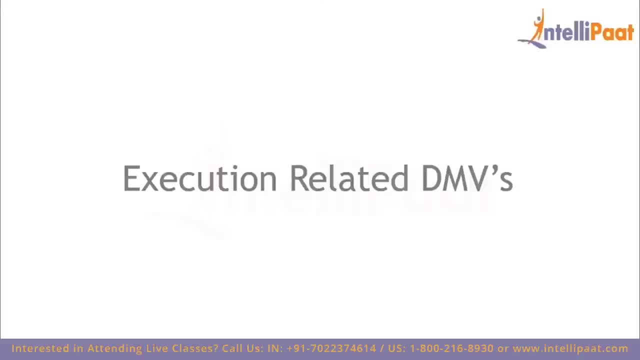 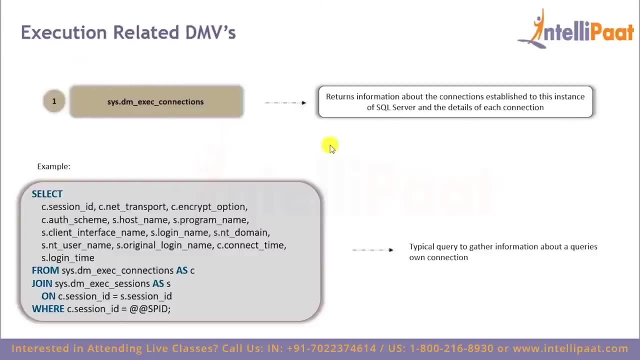 Now it's time for the third category of DMVs, Which is execution related. So first we have DM underscore EXEC connections, Which returns information about the connections established To this instance of SQL Server And the details of each connection, And this command over here is used to gather information. 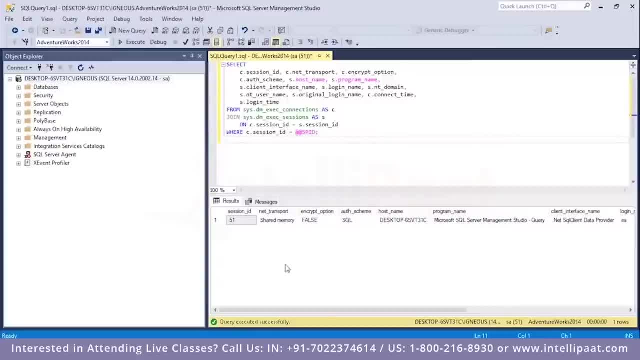 About a query's own connection. So for this query we see that the session ID is 51. And we have other columns as well, So we have the host name over here. This is the host name. We have the program name over here. 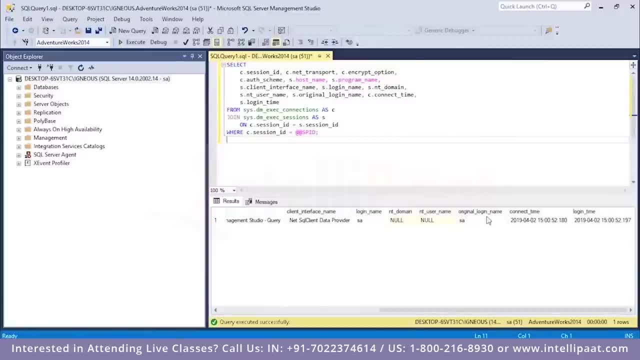 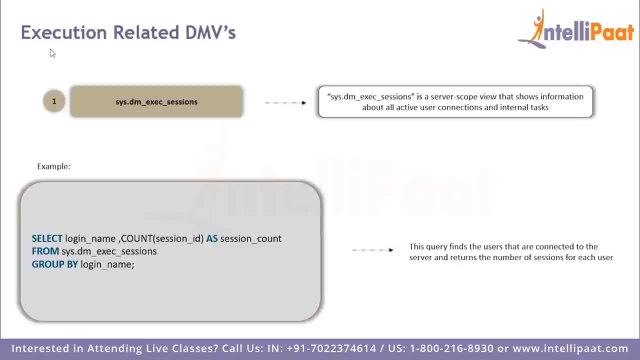 We have the login name And we have the original login name, The connection time And the login time. So next we have DM underscore, EXEC sessions, Which shows information about all active user connections And internal tasks, And this command over here. 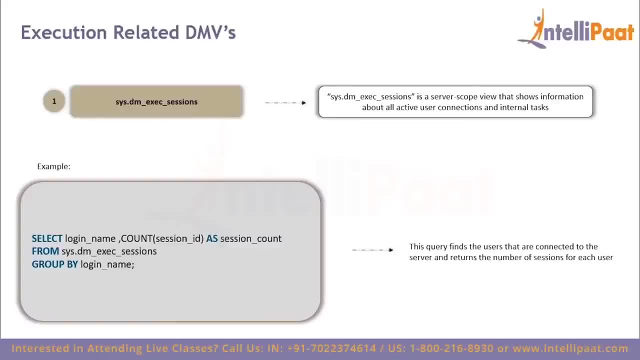 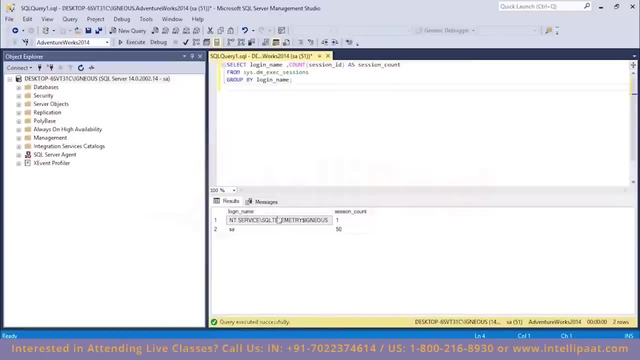 It finds the users that are connected to the server And returns the number of sessions For each such user. So we see that there are two users currently. One is anti-service igneous, Another is SA, And for the first user The session count is 1.. 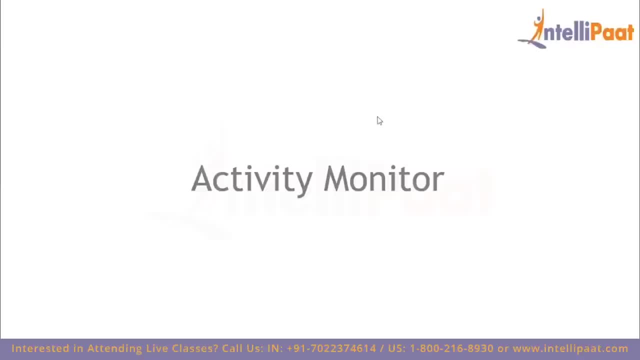 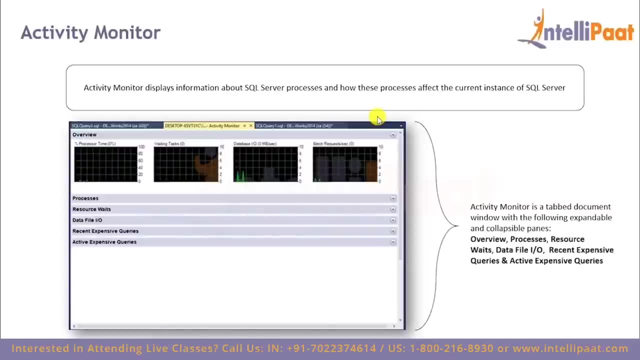 And for the second user The session count is 50.. So those were some of the dynamic management views. Now we will work with Activity Monitor. So SQL Server Activity Monitor is a feature in SQL Server Management Studio That displays information about the SQL Server processes. 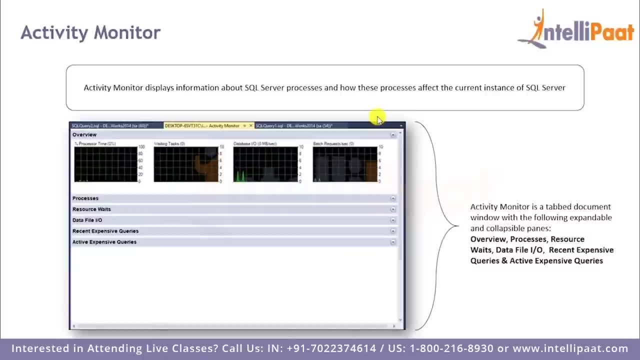 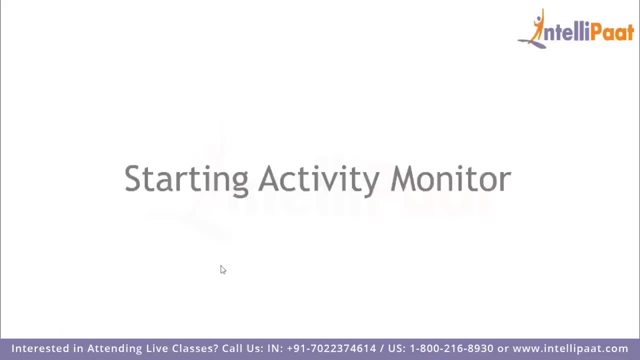 And their effect on SQL Server performance. So the Activity Monitor consists of these expandable panes. So we have overview, We have processes, Resource weights, Data, file IO, Recent expensive queries And active expensive queries. Now let's go ahead and start Activity Monitor in SSMS. 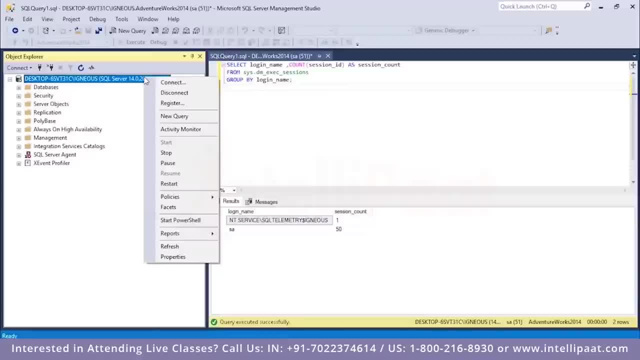 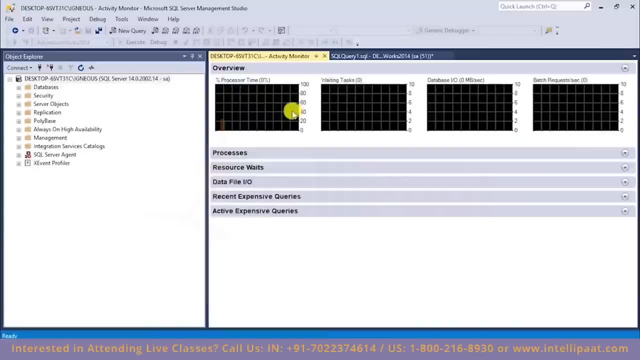 So over here I would have to right click on this And then select Activity Monitor. So we have opened up Activity Monitor. So this overview pane over here It contains the graphs for the most important SQL Server instance information. So this percent processor time. 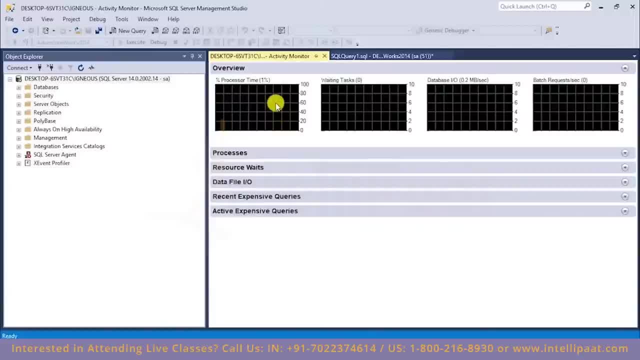 It tells us the percentage of files, Of time The processors spent to execute threads that are not idle, And then we have waiting tasks. So this over here gives us the number of tasks That are waiting for processor IO Or memory to be released. 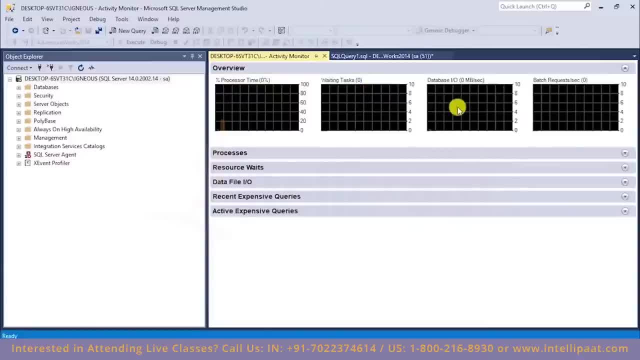 So that tasks can be processed. Then we have database IO, So this gives us the data transfer rate in megabytes per second, And it could be either from memory to disk, Disk to memory Or disk to disk. And finally we have batch requests per second. 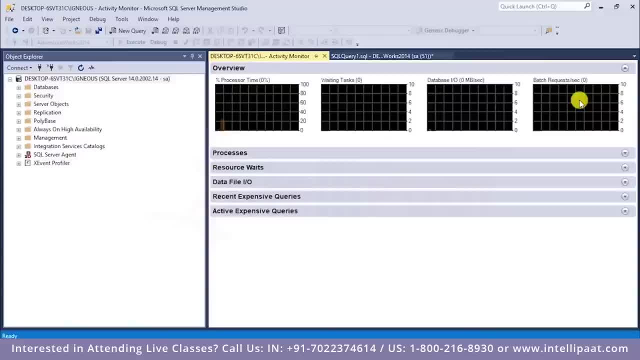 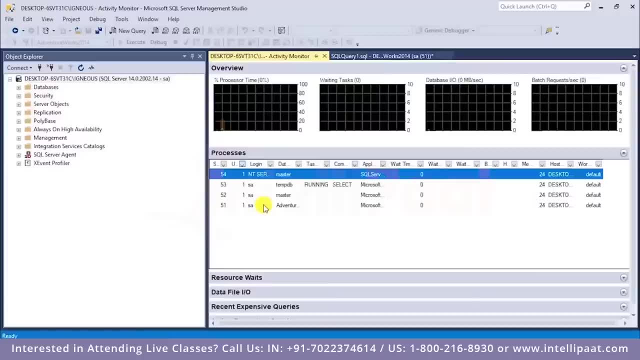 Which gives us the number of tasks Or the number of SQL Server batches received by the instance in a second. Now let's look at the processes pane. So this processes pane shows us the information about the currently running processes On the SQL Server databases. 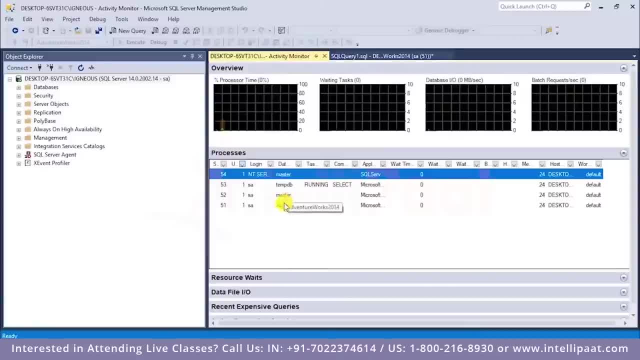 And who are running those processes. So we have information for session ID, We have user process, We have login name And so on. Right? So we see that these are the users over here And these are the databases which the users are currently working on. 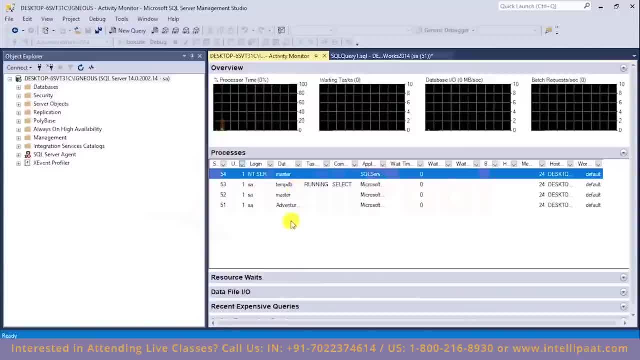 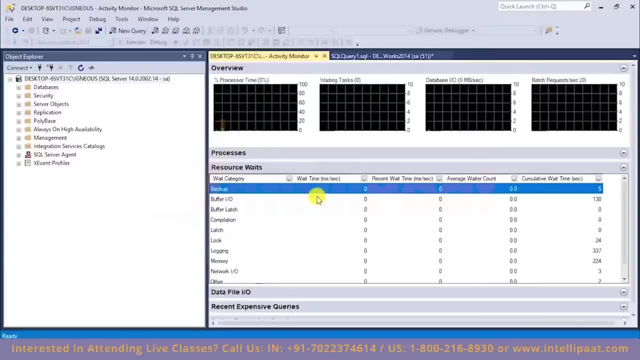 We see that the user SA has worked on TempDB, MasterDB And this AdventureWorksDB. After that we have the resource weights pane And this provides information with respect to a thread Which is waiting for a key resource Such as memory. 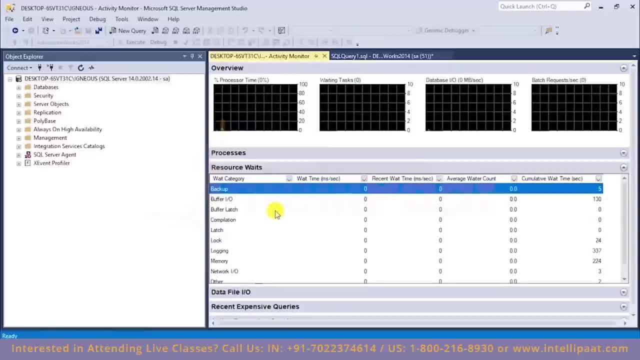 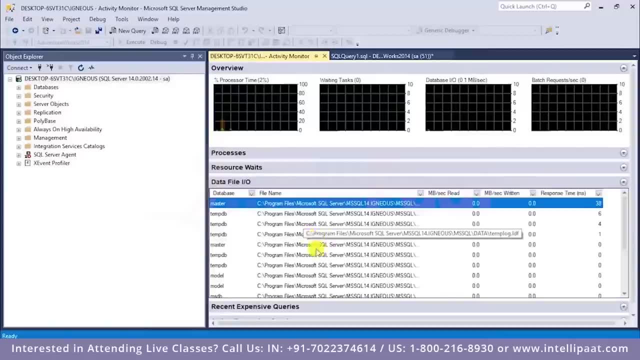 CPU Or network. So these are all of the threads which are waiting for something. And then we have the next pane, which is data file IO. So this pane shows information about the database files on the SQL Server instance. So for each database, 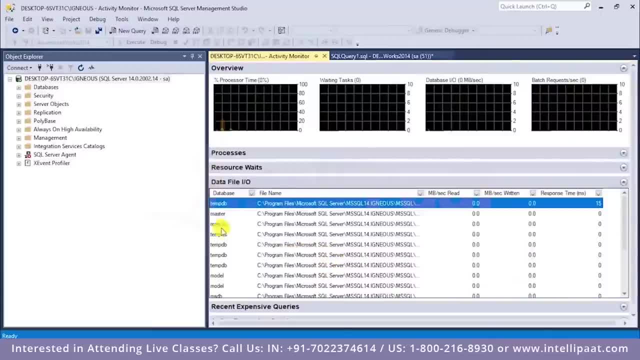 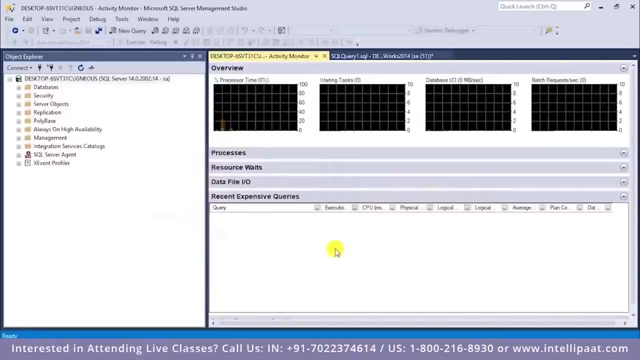 All the database files are listed. So we have all of the different databases over here- TempDB, Master Model And so on- And these are different files which are part of this database. And then, following on, we have the recent expensive queries pane. 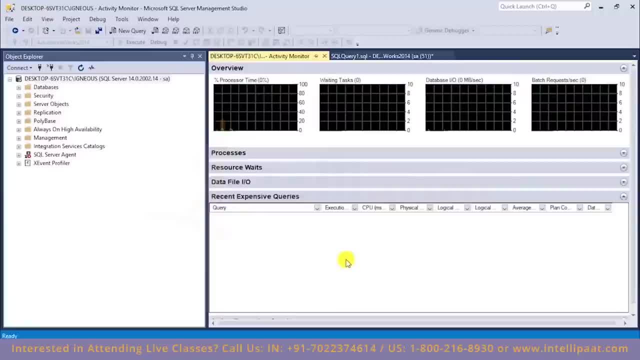 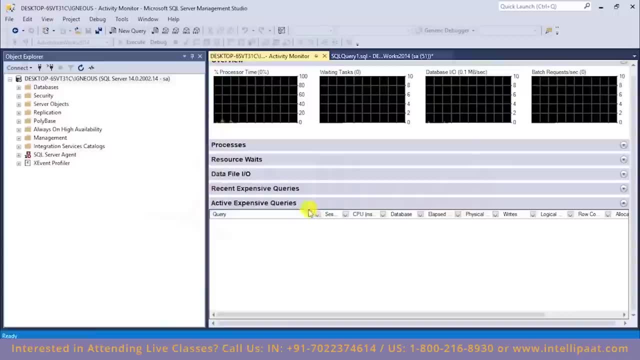 So this pane shows all the expensive queries in the last 30 seconds Which use up a lot of resources, Whether it is memory, Disk Or network. And finally We have the active expensive queries, Which shows all the currently active expensive queries running. 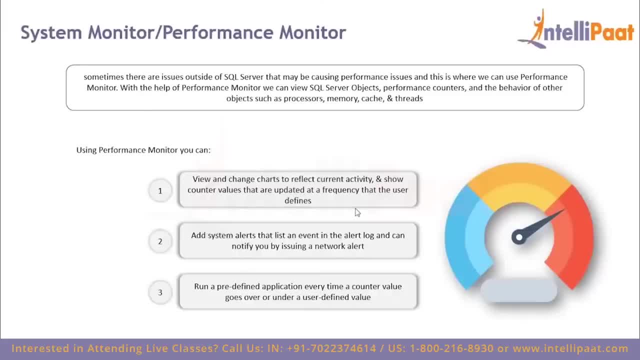 Now we will work with the performance monitor. Now, sometimes there might be issues which occur outside of SQL Server That may cause performance problems in SQL Server, So this is where we can use performance monitor. So performance monitor is a monitoring tool Which is shipped with Windows. 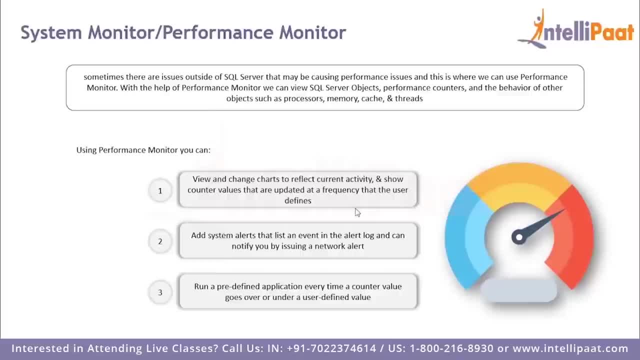 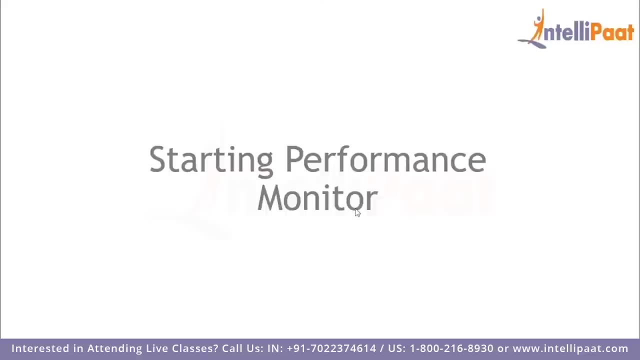 And it helps in tracking various performance counters And monitors overall system And application performance, And these counter values are shown in real time graphs Which can be saved in log files And used for analysis. Now let's work with performance monitor in SSMS. 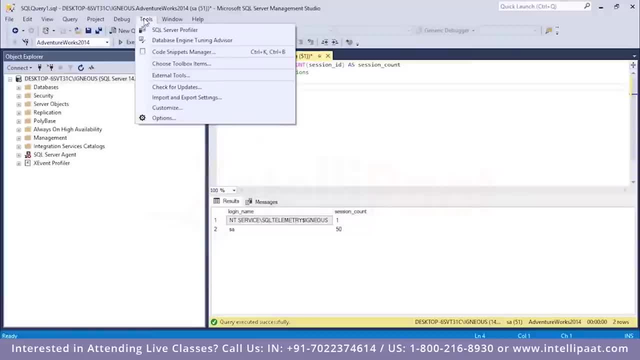 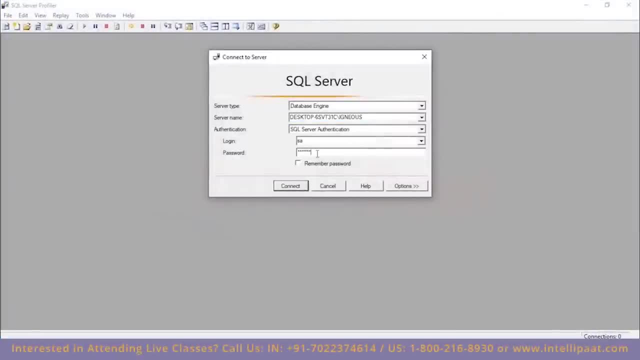 So to open performance monitor I'd have to click on tools And then select SQL Server Profiler. I will just give the connection name and the password over here. I will connect Now. again inside the SQL Server Profiler I have this tools tab. 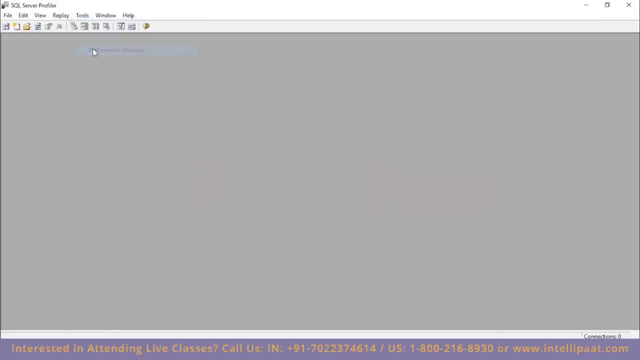 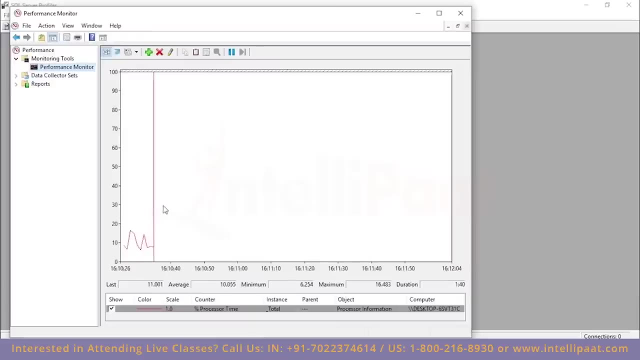 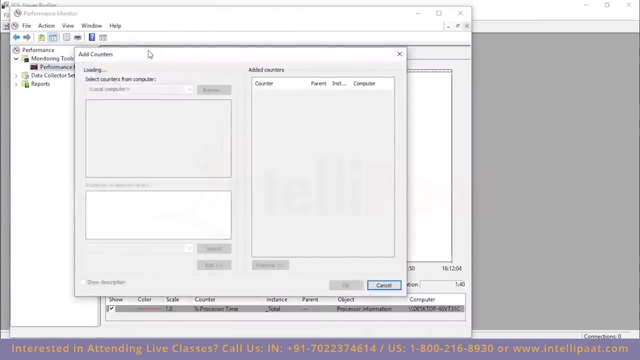 So I'll select this And then select performance monitor. Over here. I will select performance monitor And we see that there is a graph which tells me about performance of the system. Now, if I want to add some counters, I would have to click on this plus symbol over here. 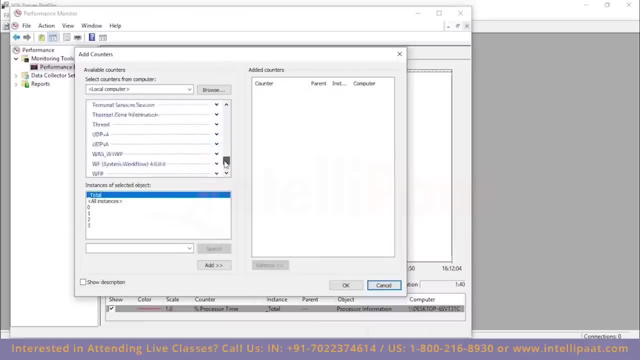 And I can add all of the performance counters. So let's say I want performance counters related to memory. So let me go to the memory section over here And inside memory Maybe I want to add available megabytes. I will add this: 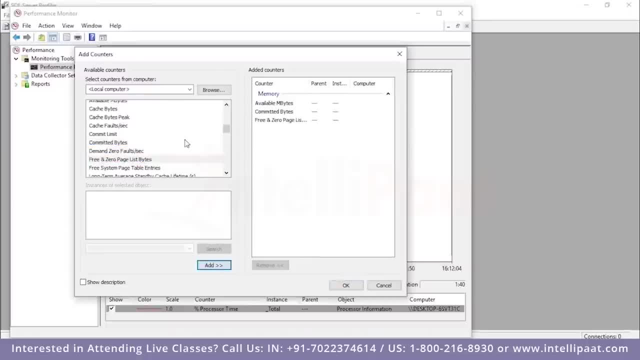 I will add committed bytes, Free and zero pageless bytes. So this is memory Again in logical disk Maybe. I want the cache bytes. I would also want the commit limit Now similarly under physical disk. I would want the disk read time. 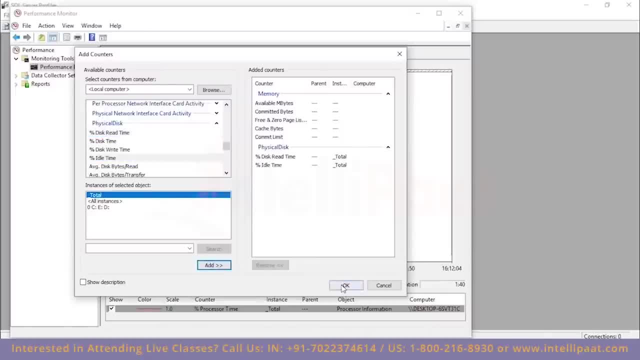 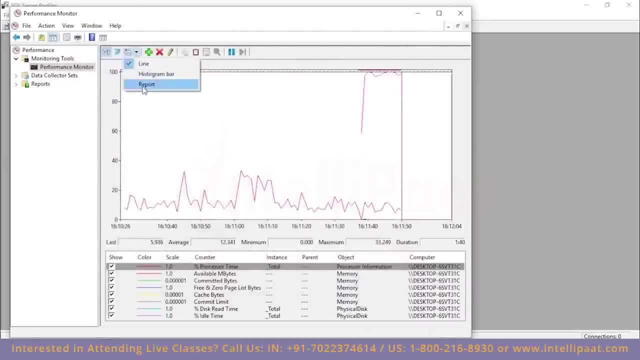 And the idle time over here. Now all I have to do is click on OK. Now, if I want to get a report of this, We see this change graph type And I will click on report. So this is the report which I have. 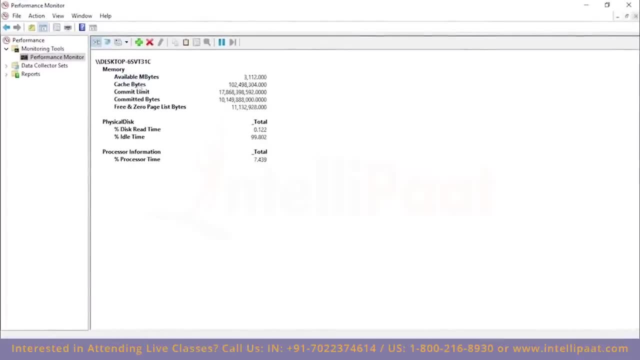 So we see that available megabytes. This is the available megabytes, Cache bytes, Committed limit Committed bytes And the free and zero pageless bytes over here And we have the percent disk read time under physical disk. Percent idle time under physical disk. 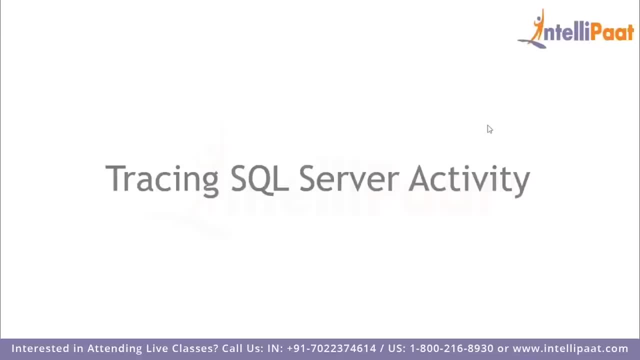 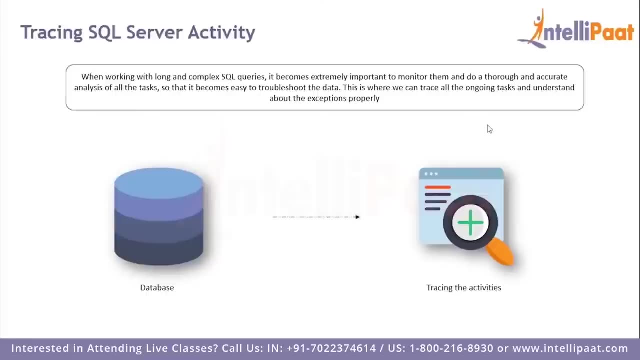 And we also have the processor time over here. Now let's see how can we trace SQL Server activity using SQL Server profiler. So whenever we are working with really long and complex SQL queries, We have to make sure that all of those tasks are performed accurately. 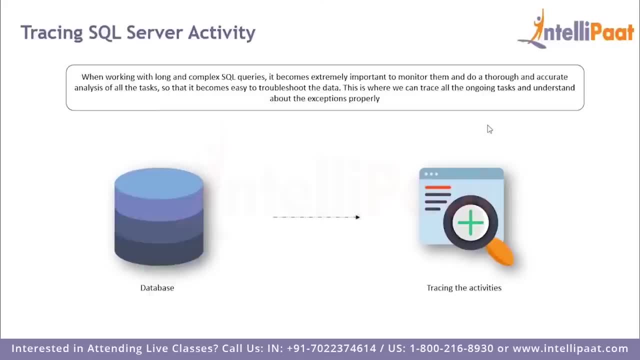 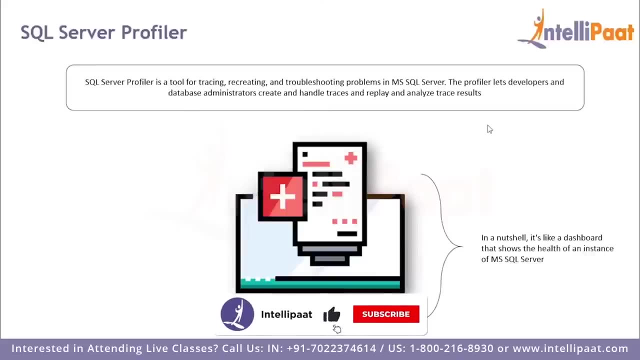 This is where tracing all these tasks becomes important. So SQL Server provides a tool called as SQL Server profiler For exactly this purpose. So profiler is a tool for tracing, recreating and troubleshooting problems in MS SQL Server, And it lets developers and database administrators to create and handle traces. 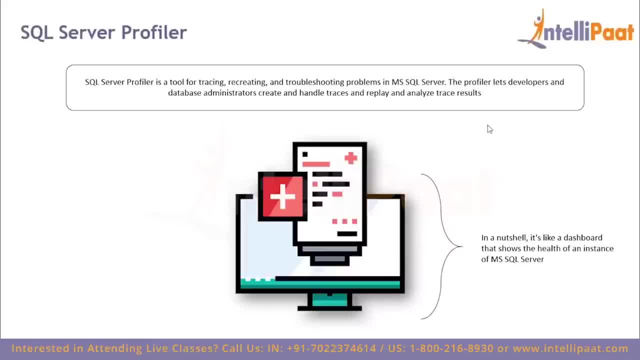 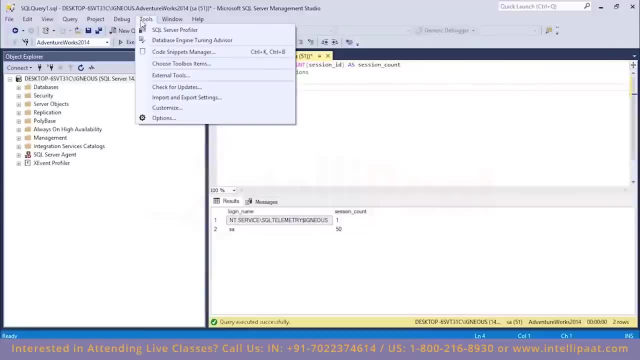 And replay and analyze these trace results. Now let's go ahead and work with SQL Server profiler in SSMS. So we are back to SSMS. Now I'd have to click on tools And then select SQL Server profiler. Again, I will give in the password. 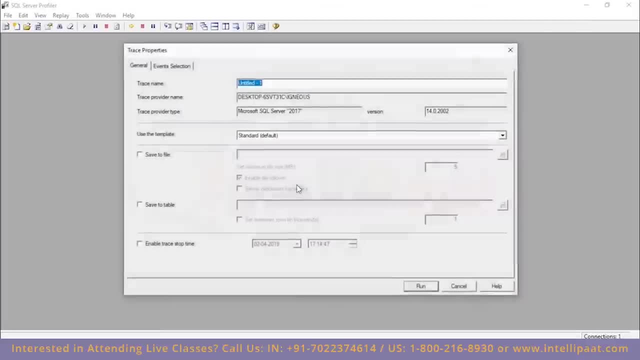 And then establish the connection. Let me click on connect. Now I'd have to give a new name to this trace, So I will name this as New trace And then maybe I will also save this to a file. So let me give in the destination. 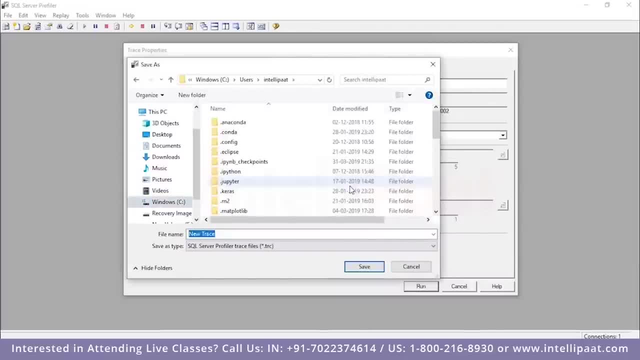 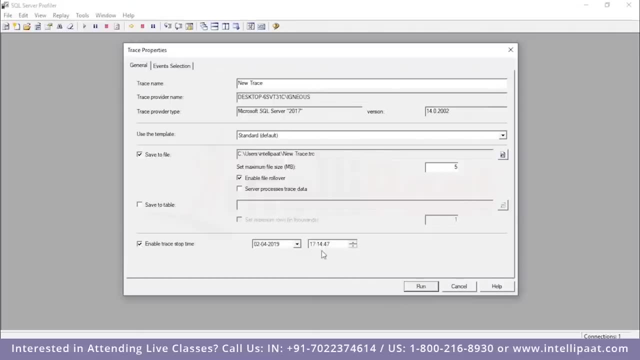 So I'll save this in my C drive. I'll click on save over here. Now I can also set the trace time, So let me schedule it. So I want this SQL Server profiler to run for at least one hour And again over here. event selection. 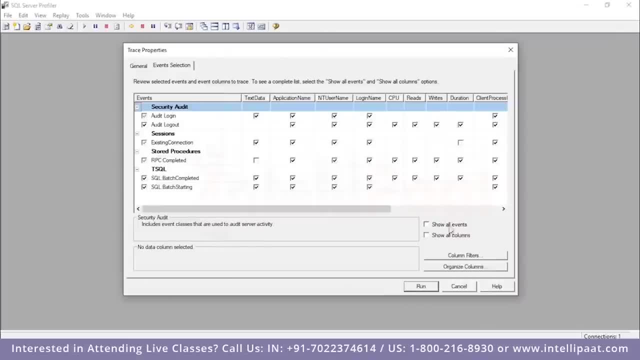 So this is where I can set all of those events which I want to be traced. So I'll click on this show all events And let me add some events over here. So I want to trace the cursor- prepare Cursor- unprepared option. 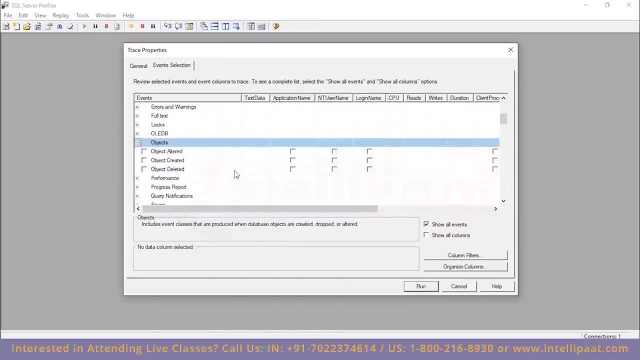 And let me go to the objects tab over here And I want to know whenever an object is altered, created or deleted. Similarly, let me go to this performance tab And I want to know about order stats. And now all I have to do is click on run. 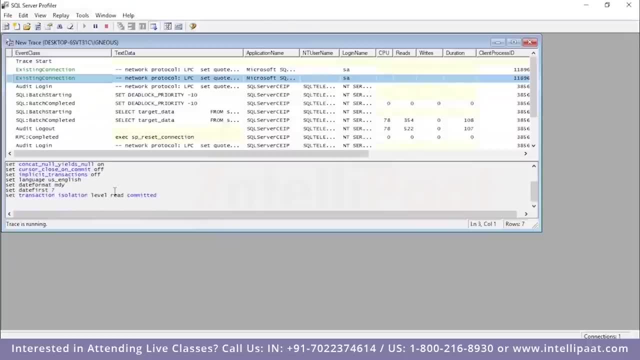 So we see that the trace has started And we get all of the information over here. So we have the detailed information of whatever is happening. So we have the event class text, data, application name, NT username, login name and so on. 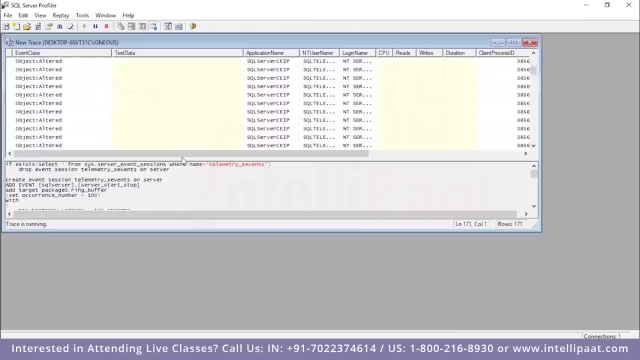 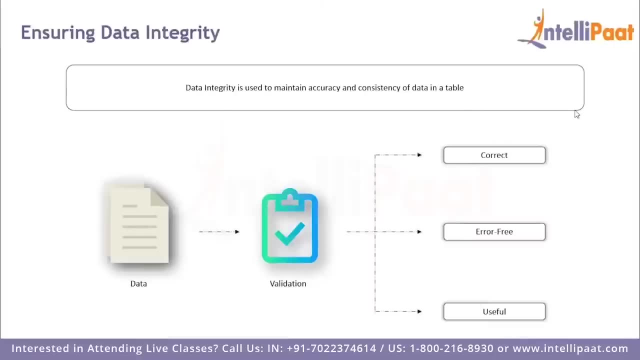 And we also have the reads- writes and the duration for the reads and writes over here. So this is how we can work with SQL Server profiler. So why do we need data integrity? Well, data integrity is used to maintain accuracy and consistency of data in a table. 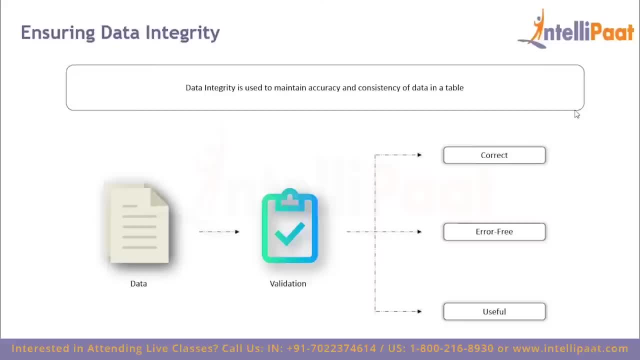 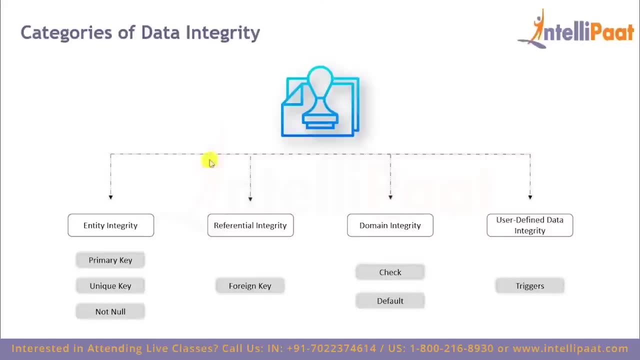 So, whatever data we have with us, we need to make sure that it is correct, error free and useful, And data integrity can be grouped into these categories, So we have entity integrity, referential integrity, domain integrity and user defined data integrity. 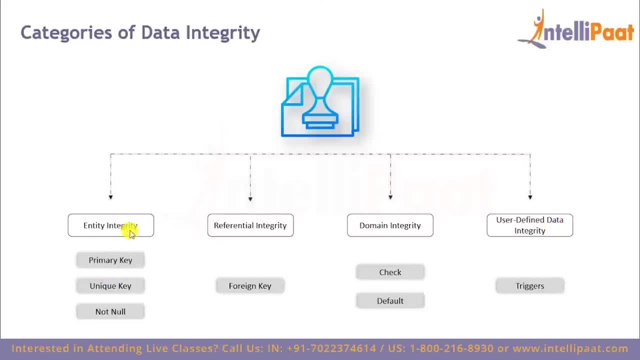 So entity integrity ensures that each row in a table is a uniquely identifiable entity And we can apply entity integrity to the table by specifying a pattern. So we have primary key, unique key and not null. Then we have referential integrity, which ensures the relationship between two tables is proper. 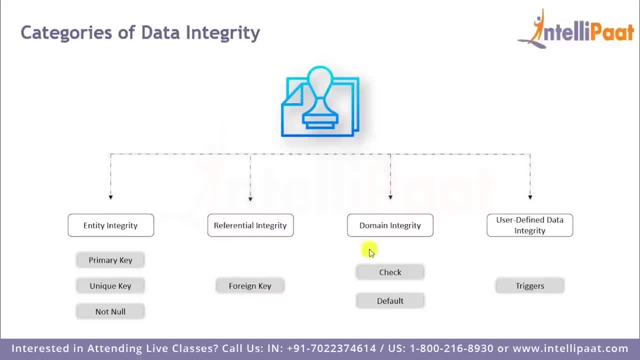 And we can apply this using a foreign key constraint. And then we have domain integrity, which ensures the data values in a database follow defined rules for values, range and format, And we can enforce these rules using check and default constraints. And finally, we have user defined data integrity. 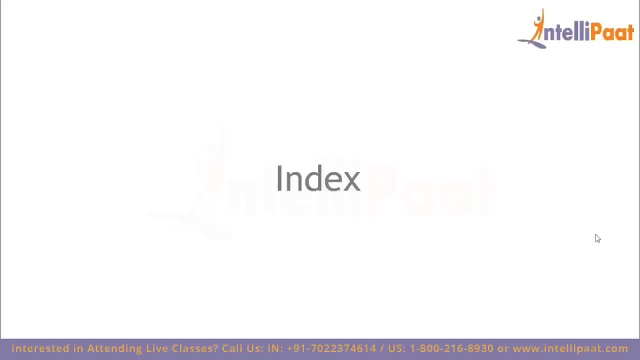 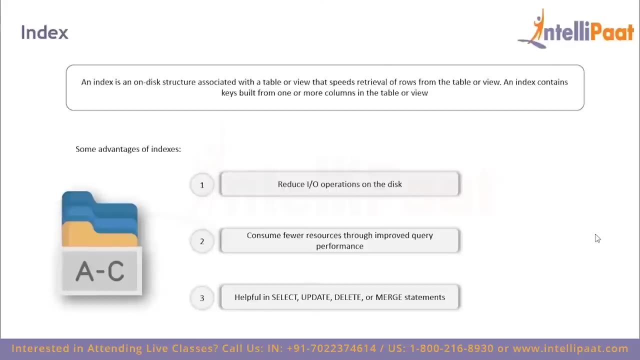 which can be enforced. So now that we know about data integrity, let's learn about indexes in SQL Server. So indexes are special lookup tables that the database search engine can use to speed up data retrieval. Simply put, an index is a pointer to data in a table. 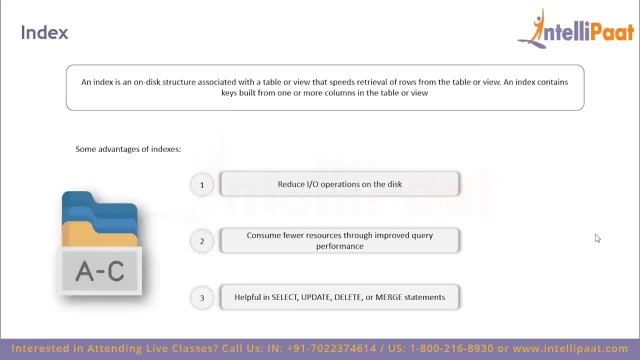 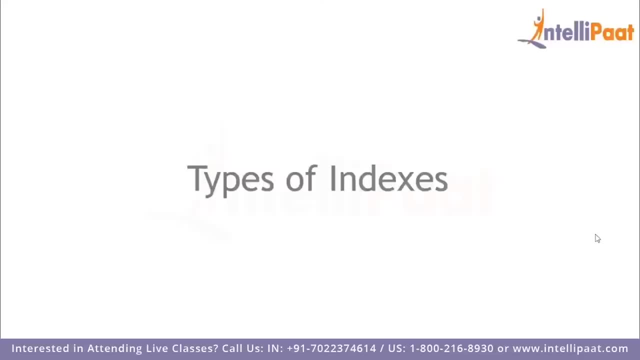 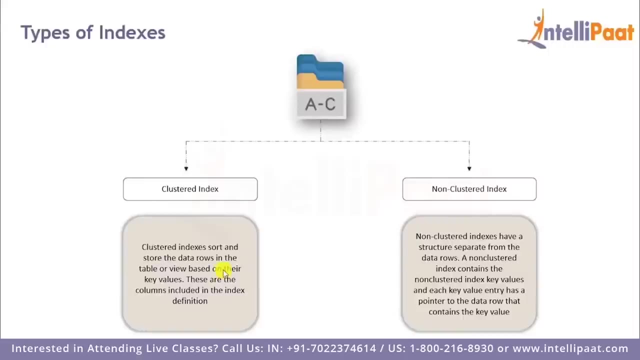 So these indexes in a database are very similar to indexes at the end of the books, whose purpose is to find a topic quickly. Now, again that we know what exactly is an index, let's look at the types of indexes. So in SQL Server, indexes can be grouped into clustered and non-clustered. 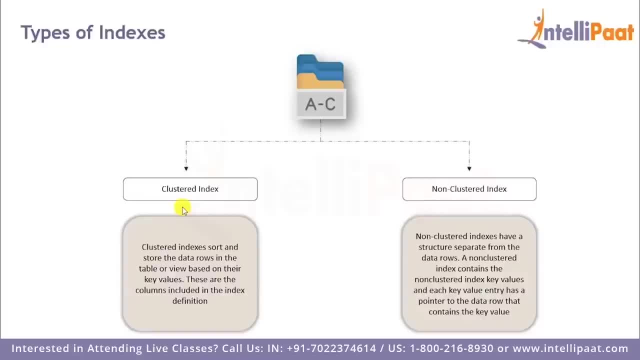 So a clustered index defines the order in which data is physically stored in a table And since table data can be sorted in only one way, therefore there can be only one clustered index per table. So in SQL Server the primary key constraint automatically creates a clustered index on that particular column. 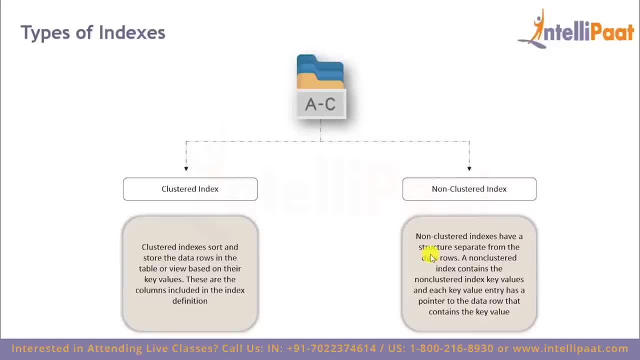 But when it comes to non-clustered index, it doesn't sort the physical data inside the table. In fact, a non-clustered index is stored at one place and table data is stored in another place, And this is actually similar to a textbook, where the book content is located in one place and the index is located in another. 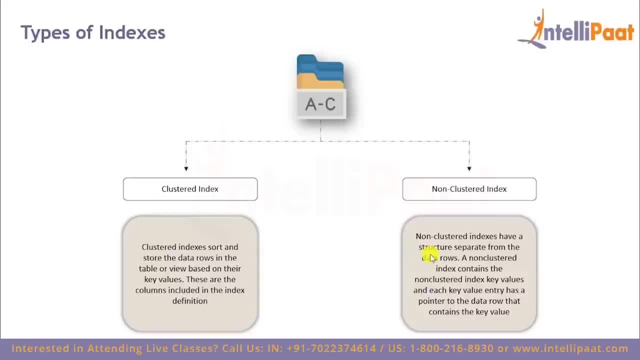 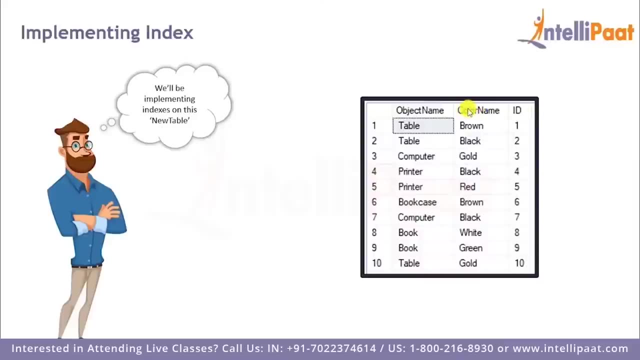 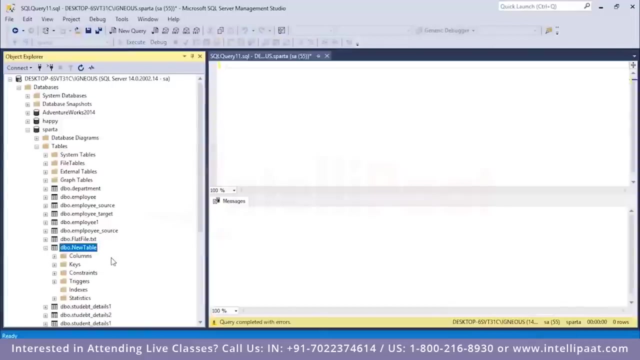 And this allows for more than one non-clustered index per table, And we'll be implementing indexes on this new table, which comprises of these columns: object name, color name and ID. So we have this new table over here Now, if I have to create an index on top of this, 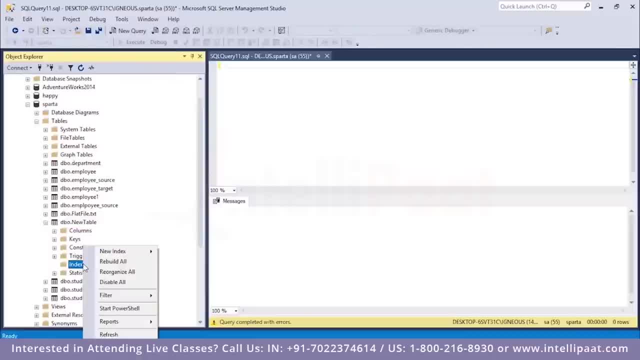 we have this index folder inside this table, So I would have to right click on this, select on new index, And if I want to create a clustered index, I will select this option- clustered index- and then give a name to this clustered index. 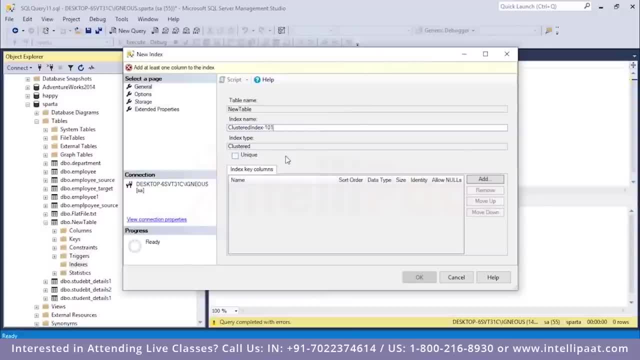 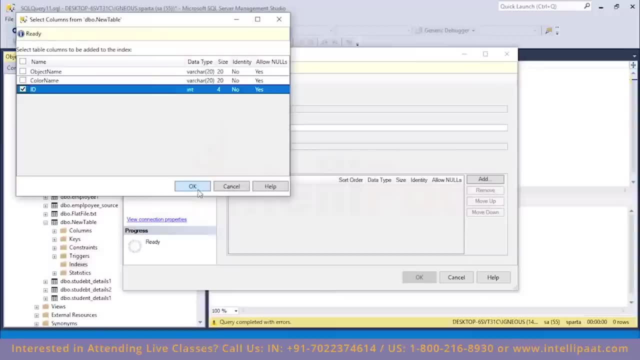 So I will name this as clustered index 101. And I will go ahead and add this new table And I will create this clustered index on top of the ID column of this table. I'll click on OK. Now again, if I want the TSQL code for it, all I have to do is click on script. 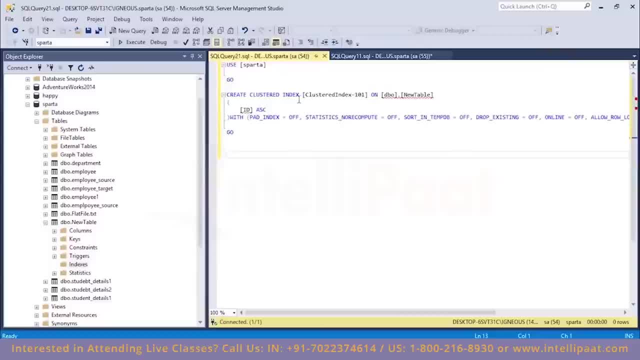 So this is the TSQL code to create a clustered index with the name clustered index 101.. And it is built on top of the ID column. So now again, I will go to this dialog box and click on OK. So you see that we have successfully created a clustered index with the name clustered index 101. 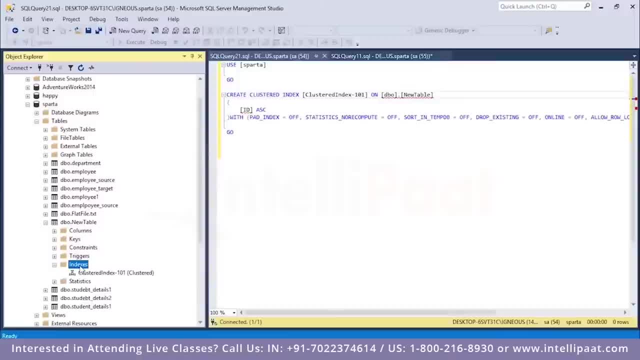 Which is on top of the ID column. Now, similarly, if I want to create a non clustered index, I will right click on this folder, select new index And this time I will choose non clustered index And again, I will give a name to this. 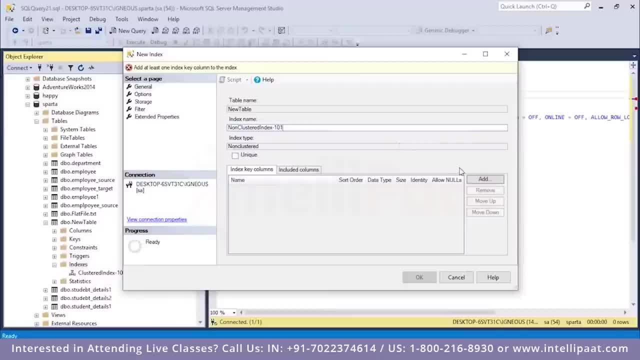 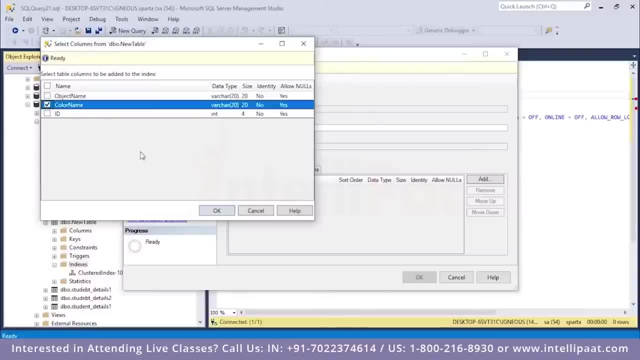 So this will be non clustered index 101.. I will go ahead and add a column on top of which this non clustered index is supposed to be, So I'll choose the color name column. I'll click on OK Again if I need the code for this. 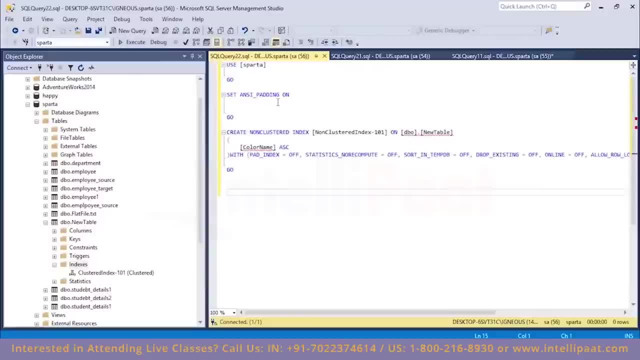 I'll click on script. So this is the code to create a non clustered index with the name non clustered index 101.. And this is on top of the color name column. So again, I will finally click on OK. And we have also successfully created the non clustered index with the name non clustered index 101.. 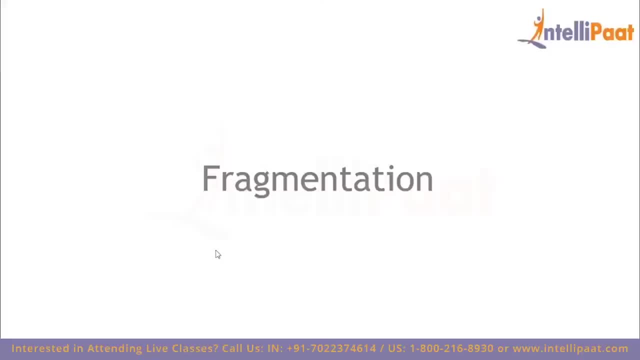 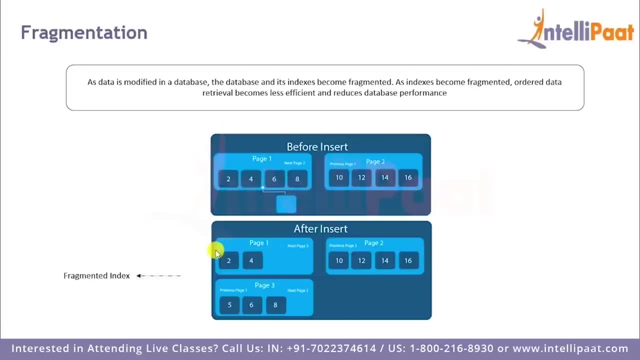 Now let's talk about one of the problem which is associated with indexing And that is known as fragmentation. So index fragmentation happens when the indexes are scattered all over the database. Well, whenever SQL Server performs IO operation, it initially reads the data from the disk, which is known as physical read. 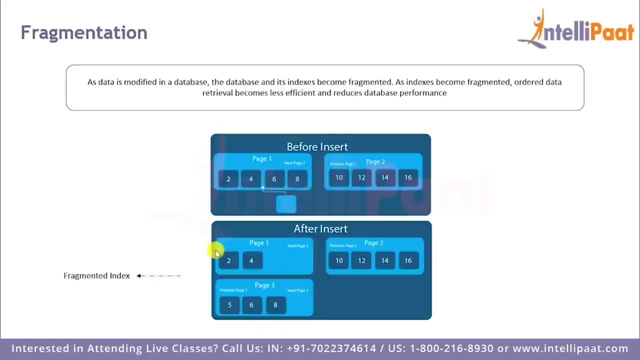 So it pulls everything into the SQL Server buffer. So there is a logical order in this buffer And whenever the query runs again, instead of doing physical read, SQL Server would look into the buffer And if it can't find the requisite data in the buffer, that is when it will do physical read from the disk. 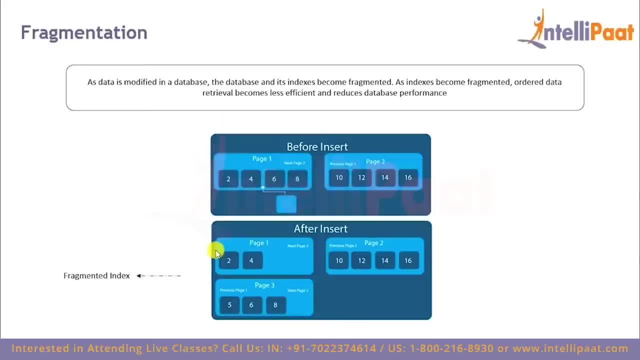 Now there might be a case where the logical order of the indexes is not equal to the physical order of the indexes, And this is called as index fragmentation. Now, why does it happen? Well, whenever we insert or update data, the indexes become fragmented. 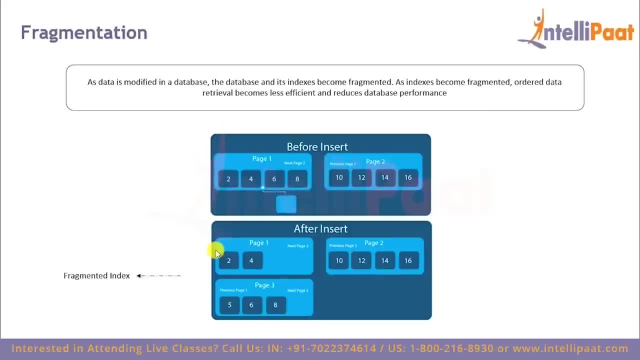 And as indexes become fragmented, order data retrieval becomes less efficient and reduces database performance. So let's actually take this example. So initially we have two data pages for a table with a clustered index. Now a new row with the primary key phi needs to be inserted. 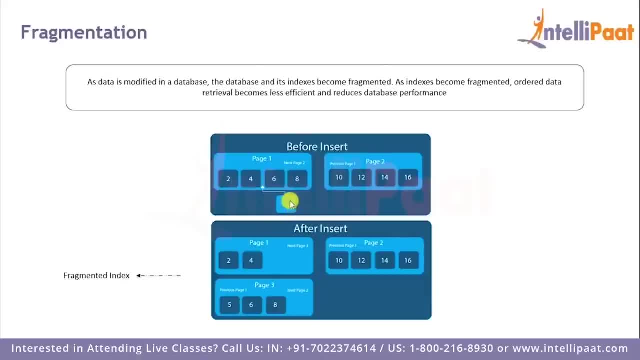 And since it is a clustered index, new row is inserted in order And because the target page is full over here, the new row does not fit And SQL Server splits the page roughly into two halves and inserts the data into this new page. 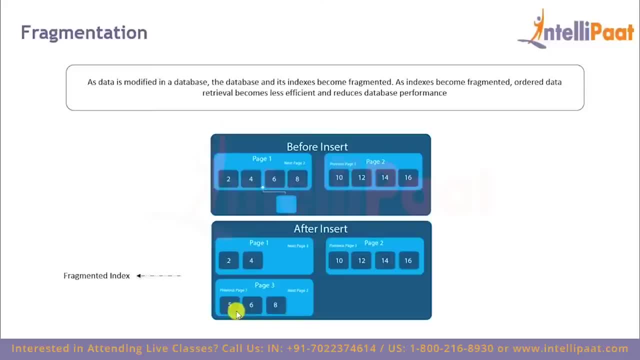 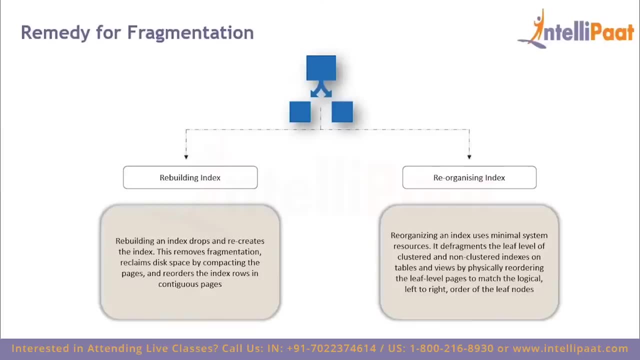 Now what happens is the logical order of the index does not match with the physical order, And this is when we say that the index has become fragmented. Now, to deal with fragmentation, we have two solutions. We can either rebuild the index or reorganize the index. 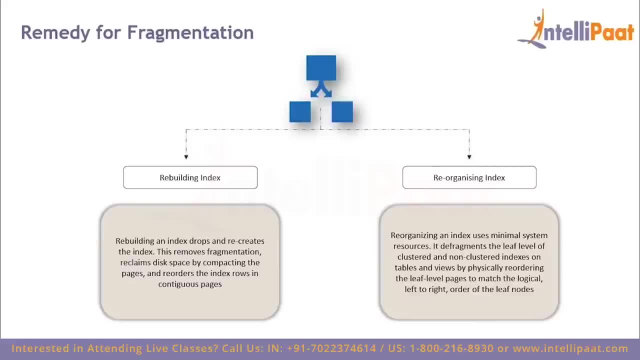 So rebuilding is the process of changing the whole p-tree, That is all. the existing indexes are dropped and new indexes are recreated, While reorganizing index is the process of cleaning, organizing and defragmenting the leaf level of the p-tree. 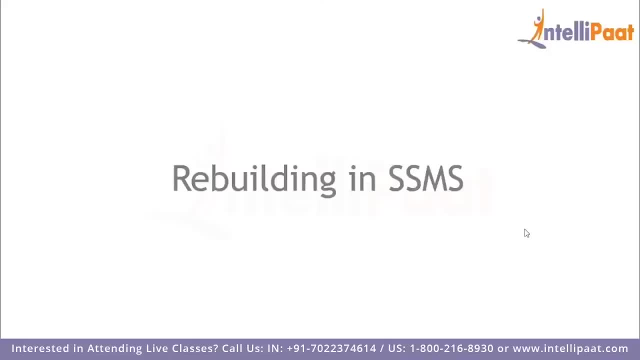 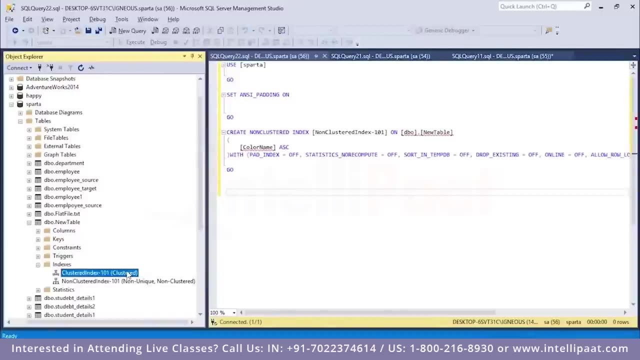 Now we'll go ahead and implement these concepts in SSMS. So I will take these clustered index and I want to rebuild this clustered index. So if I want to do that, I will right click on this and I have this option to rebuild. 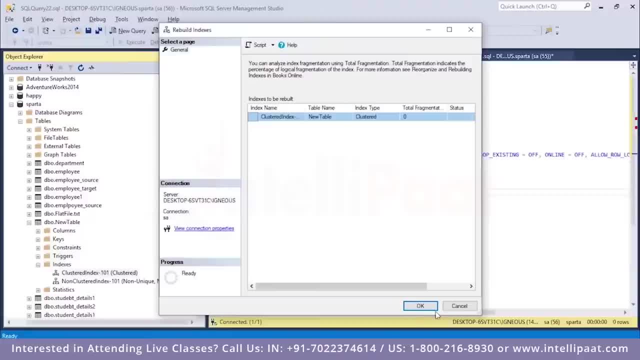 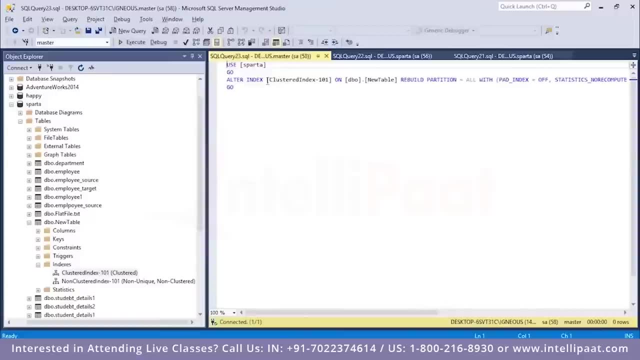 I'll click on this. Now all I have to do is click on OK. And again, if I need the TSQL code for this, I'll click on OK. All I have to do is click on script And this is the TSQL code to rebuild this clustered index 101. 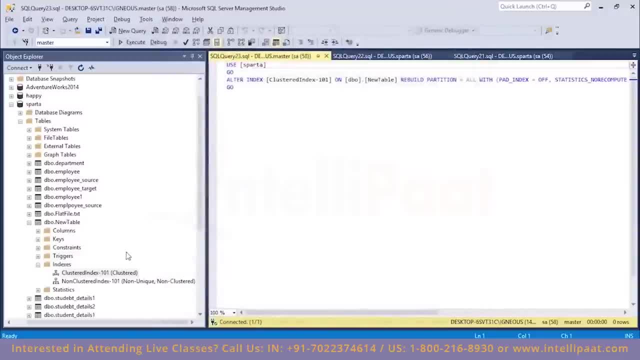 So I will go ahead, click on OK. And I have successfully rebuilt this clustered index. Now I want to reorganize this non-clustered index. So this time I will right click on this, select Reorganize, And again select this and click on OK. 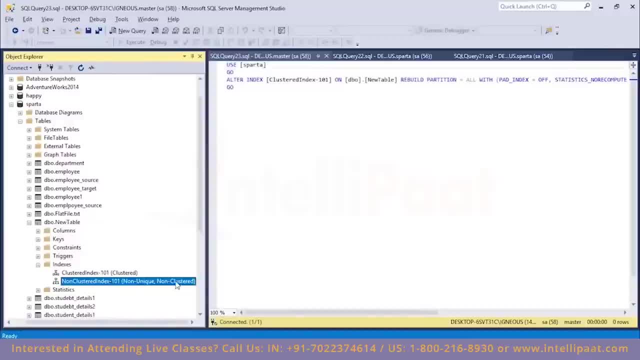 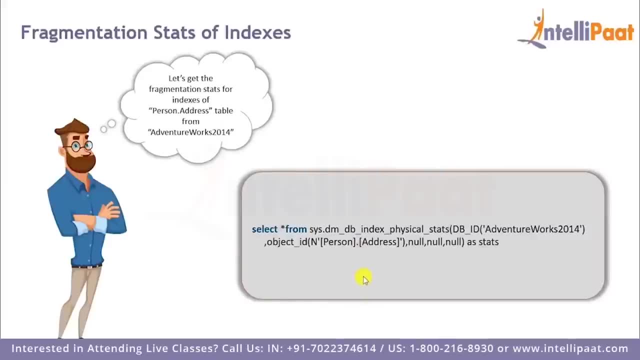 So this time I have successfully reorganized this non-clustered index. Now let's see how can we get the fragmentation stats of indexes. So we can use this dynamic management function, sysdm__db__index__physicalstats to get the fragmentation stats. 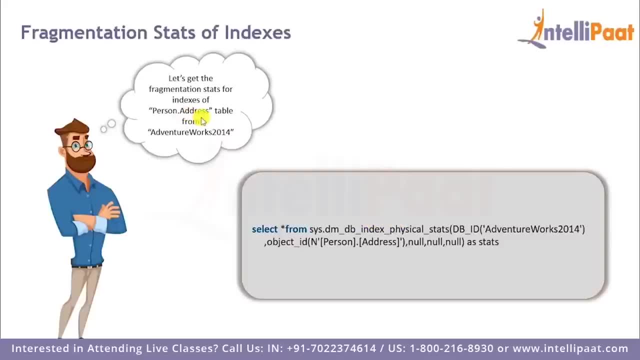 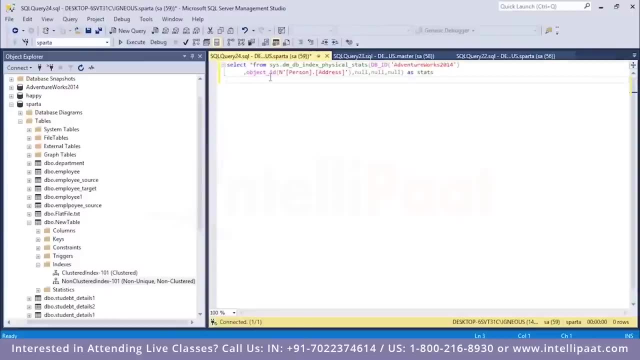 And we'll be applying this on top of this personaddress table from the AdventureWorks 2014 database. So I'll just paste the code over here And I want these index stats For this table over here: personaddress. I'll click on Execute. 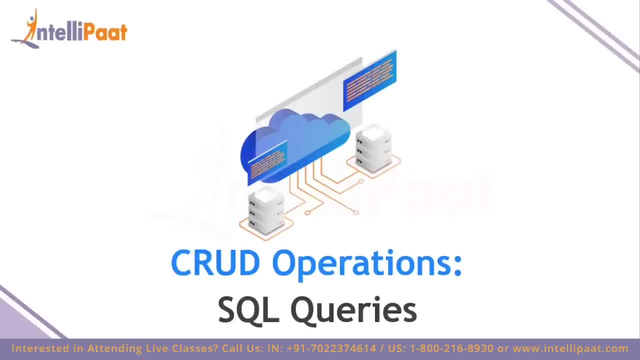 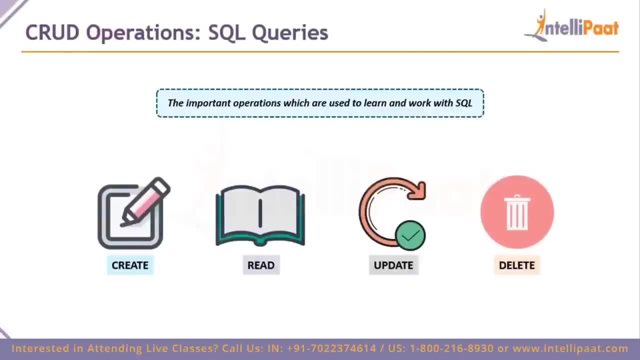 And these are the fragmentation stats for this table: CRUD operations. CRUD operations is where we'll actually check out some quick SQL queries, But first you need to know what CRUD stands for, guys. So every time you begin to learn SQL, or you're revising SQL, or you need to understand what SQL is. 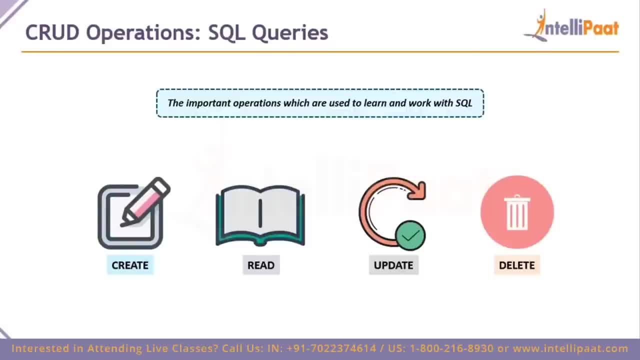 you will begin with CRUD operations as your first practical hands-on guys, And that's the reason I have chosen this, The reason I have chosen this particular thing to show it to you guys. C in CRUD stands for create, R stands for read. 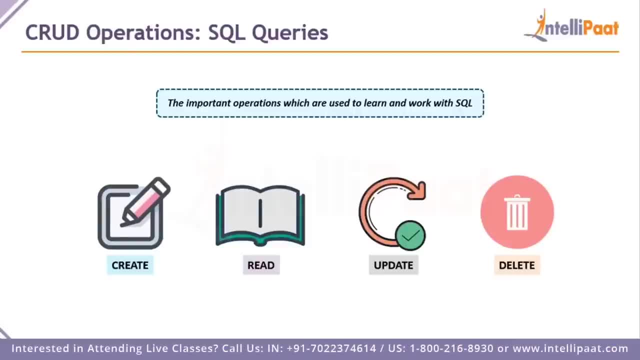 U stands for update And D stands for delete, guys. So these are some of the operations we can perform on a database. So we can perform a create operation, We can create something on the database, We can read stuff from the database, We can update the database and eventually delete the database as well, guys. 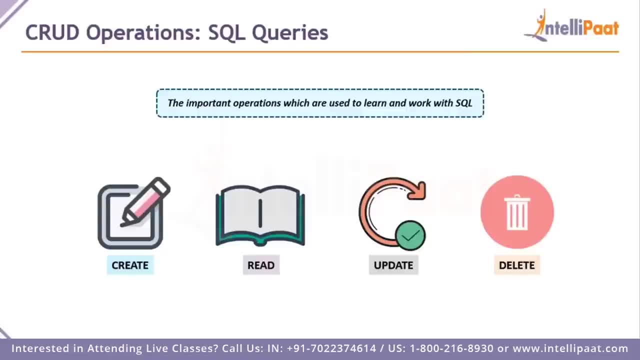 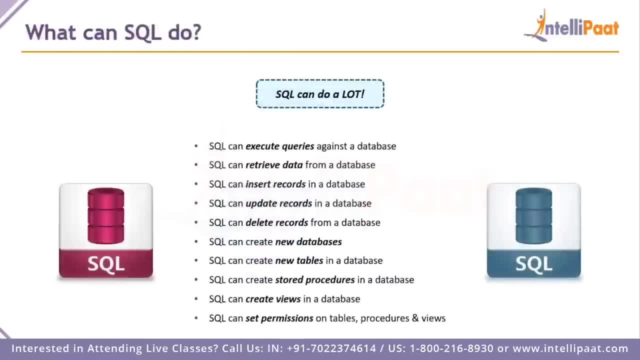 You can eventually, you know, not just the database. You can create tables, delete tables, read tables, update tables And so much more as well, guys. So on that note, what can SQL do? We're talking a lot about, you know, SQL can do this, SQL can do that. 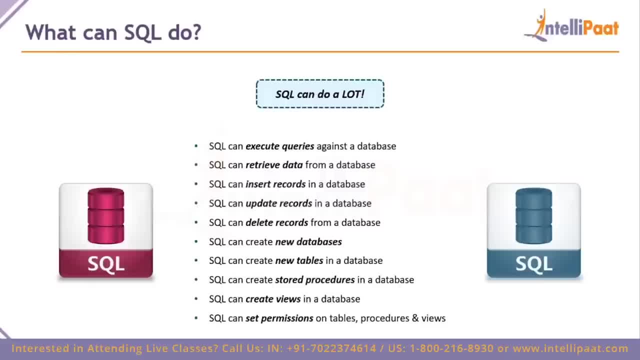 But then if you have to put everything under one header, this is what I would say, guys. SQL can execute queries in a database, It can retrieve data, It can insert the record into a database, update the records, delete- basically the CRUD operations. 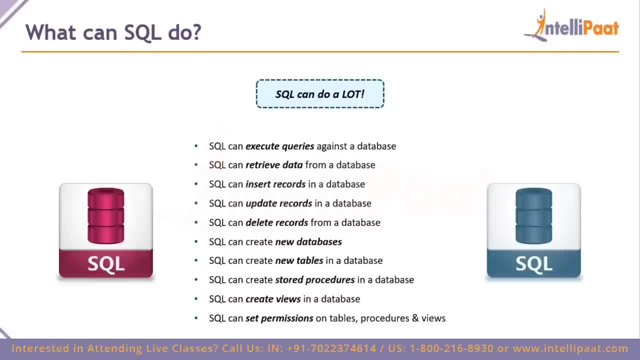 It can create new databases, create new tables, And then you have something called a stored procedure, which is basically like a ready set of commands. All you have to do is, you know pretty much, just run that stored procedure and it will run lots and lots of commands for you at once. 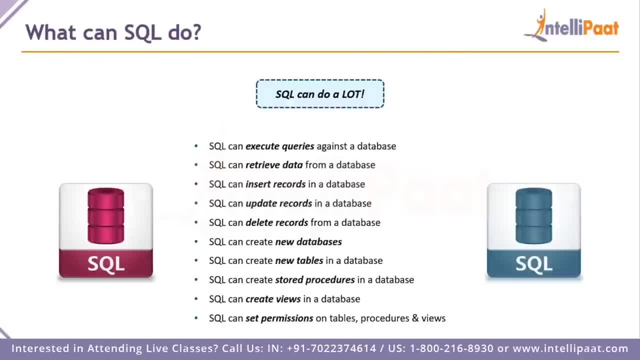 And you know, let's say, let's say you're a huge organization, You do not want to type queries every single time And there are thousands and thousands of lines of queries. So stored procedure is basically a saved file where you just run it and it runs all of these thousands of lines of queries for you to pick whatever data you're looking for in a database. 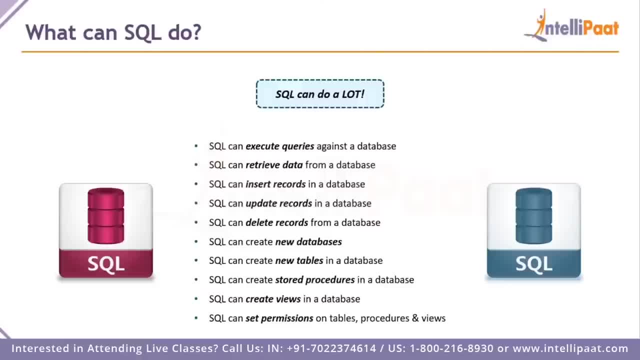 So it's basically like a shortcut And then SQL can create views as well. Views are these temporary entities Where you know, let's say, our data, our table contains thousand rows, where we don't want to see thousand rows or thousand columns. 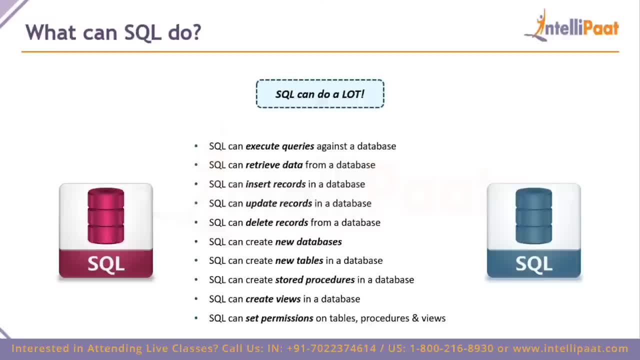 In fact. so we just want to see three columns and three entries. So in that case we create something called as a view, where we only pick these stuff that we want to see And then we show it on the screen. It's as simple as that, guys. 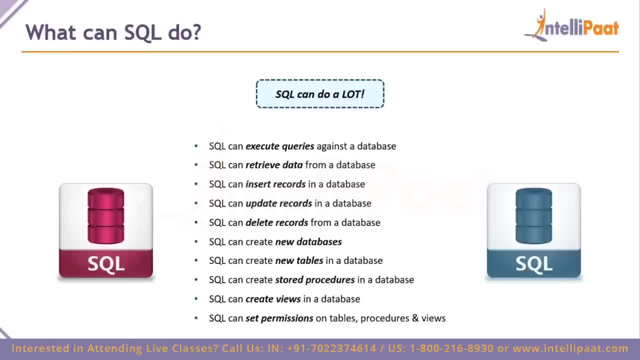 And then, coming to permissions, as we already told you, it offers very good security measures And we can set any permission for any person accessing, you know, any client accessing the database on tables, procedures, views and so much more, Guys. 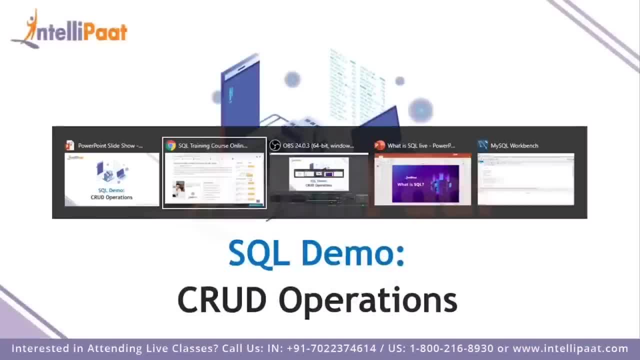 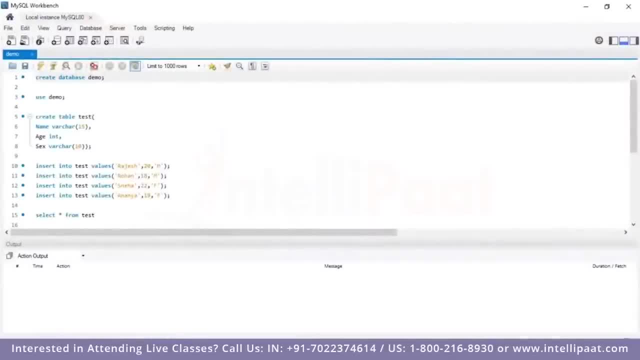 So this quickly brings us to our operations demo. Well, let me quickly jump into my SQL workbench. So my SQL workbench: again, this comes completely with the SQL Server installed. It gives you a workbench, It gives you a platform to basically write your queries, guys. 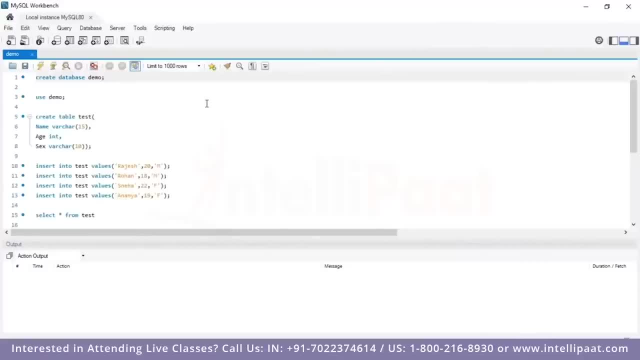 So I have pretty much written down a couple of sample queries for you guys to just take a look at and work with, And let me work with you on every single line of query that we've pretty much written. So the first query says: create database demo. 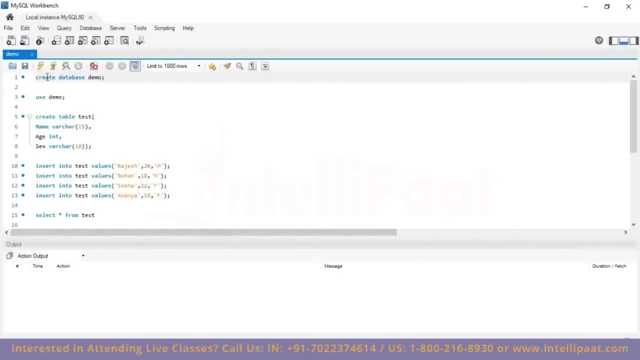 This line is fairly simple because you can pretty much it's a very high level language, right? So we're creating a database entity and we are calling our database as demo. This particular name is extremely important because you're going to be using it a lot, guys. 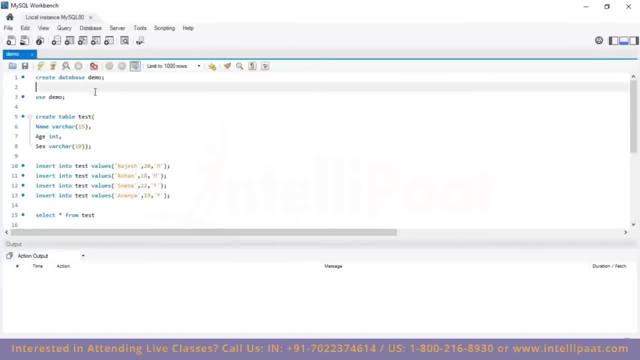 So the first step is to create a database, And let me quickly run this query. As you can see, our database has been created now, So we just created it. We created one database and we left it there. So think of it as a box, where you just close something in a box and put it next to you. 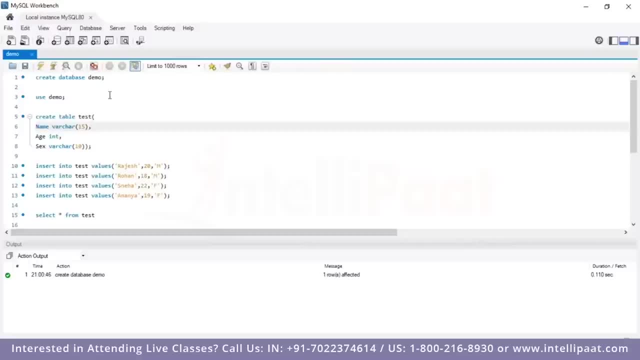 So unless you actually open that box and, you know, start using stuff, it won't make sense, right? So then we actually use the query, which is use demo. Demo is again it's basically use, followed by the name of the database. 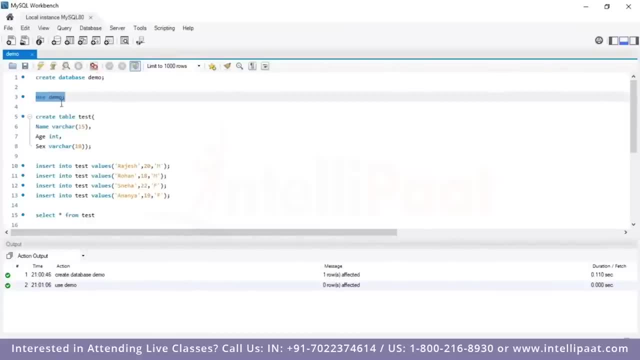 So use demo will pretty much open that database box for us where we can work with it on the inside guys. And the next query is something very simple, where you know our database is again a plain entity, So we need to create some tables there. 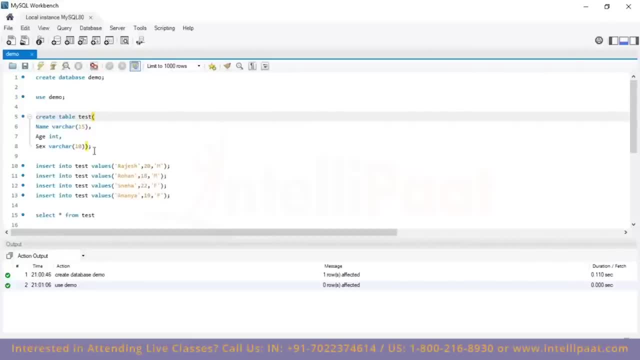 So in this particular demo, I'm going to create one table for you guys using this very simple syntax. So the actual syntax to begin with creating a table is create table. The table name in my particular case is test. Well, you can have it anything that you want. 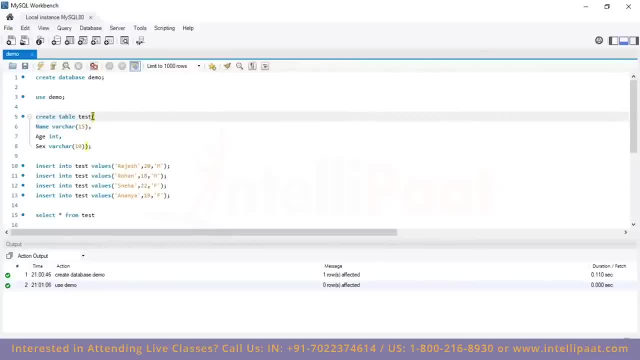 And we're going to open a bracket where whatever command we put in this particular, you know, as a parameter, needs to be under this parentheses, guys. So, as you can see, we have highlighted one and it highlights the other one for me. 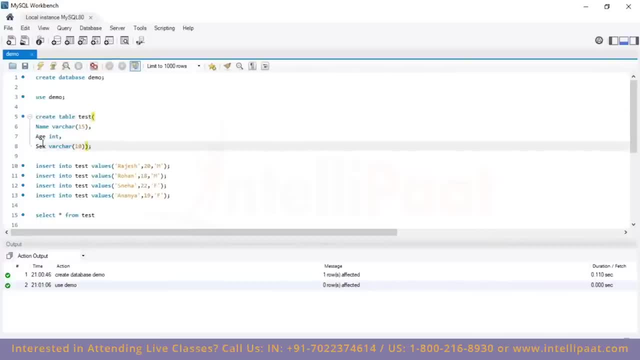 So whatever, from here till here, Pretty much goes on. It goes on under the create table header, guys. So I've created three columns for my database. One is the name. It's a varchar, It means it's a character. Name is a character, right. 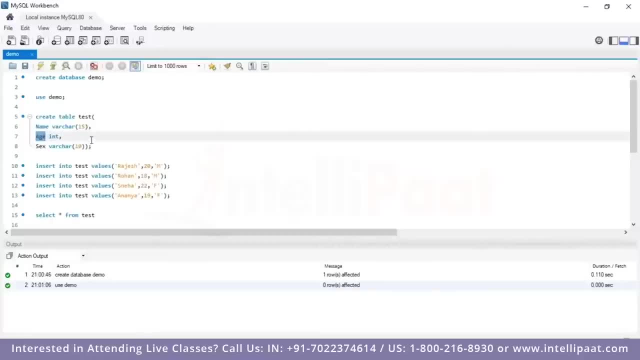 I cannot have name as two and three and whatnot. And then we have age. Age is pretty much the integer as we pretty much can go on using. We don't have to use short int, long int, you know, tiny int and all of that because, again, we know pretty much if you're going to work with a human age. 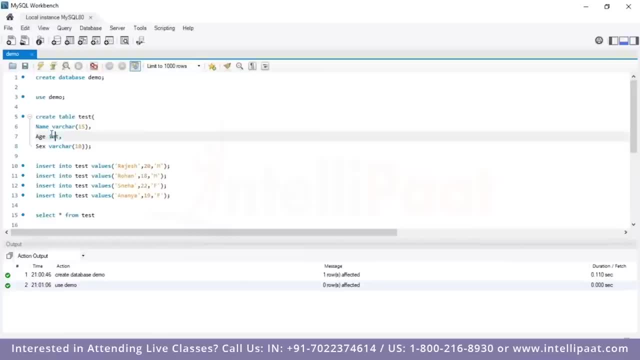 it's going to be somewhere between zero and maximum Hundred or something Right, So int will suffice. And then we have the pretty much of the person is the male or a female, and more So pretty much that that again is a single character. 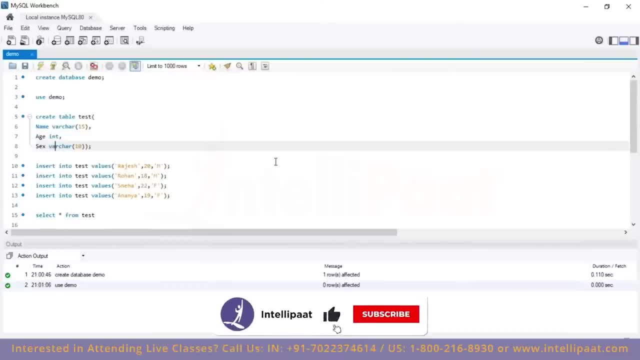 So we're going to use care varchar and we can go on using text as well if you want, But then that's a waste of memory, guys. So as soon as I run this particular query, I'm going to select this query. I'm going to run it as soon as I run this. 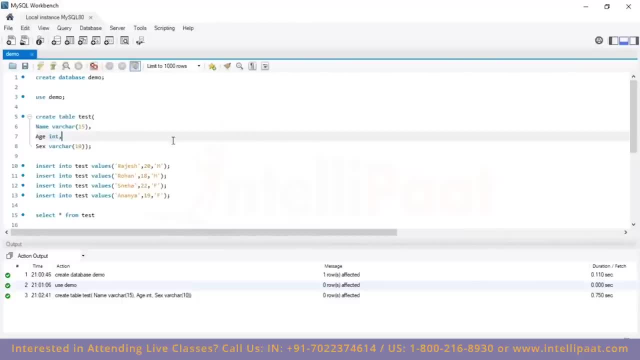 What it does is: our database is now created, Our table is now created, But then we just created an empty table, So we do not have any data in our table as of now. So to quickly change that, we're going to put in some data into the table. 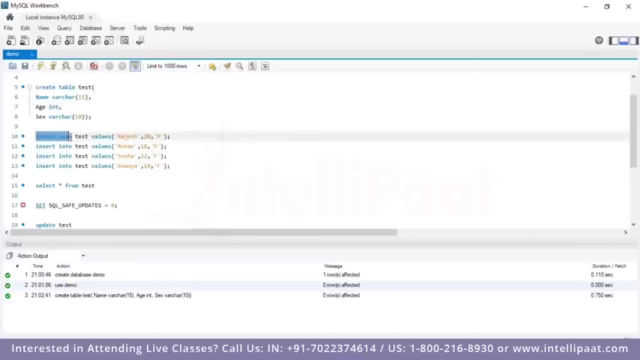 So the command we use to put data into the table is insert into, followed by table name and values, And this is the most simple way you can go on to insert a value to your table, guys. So we're going to have to map it in the way that we have created. 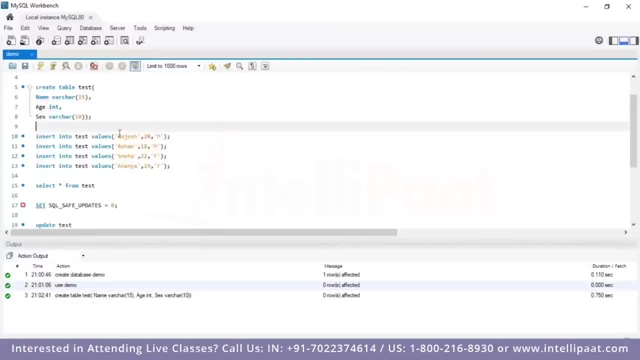 So I've created it as name, age and sex. So basically I need to go on to define name, define age and define the sex guys. So the name of this particular entry is Rajesh. His age is 20 and Rajesh is male. 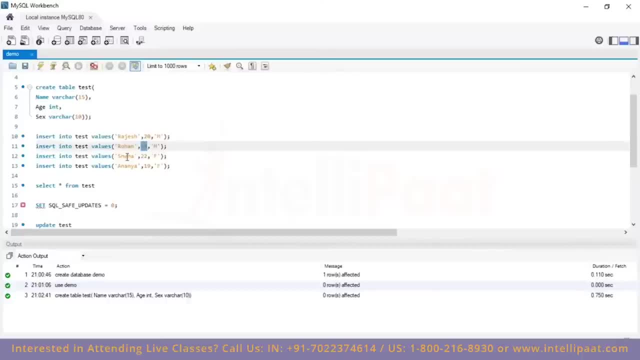 And then we have Rohan, who's 18 years old- He's a male as well. Then we have Sneha, who's 22 years old, and she's a female, And we have Ananyam, who's 19 years old, and she's a female as well. guys, 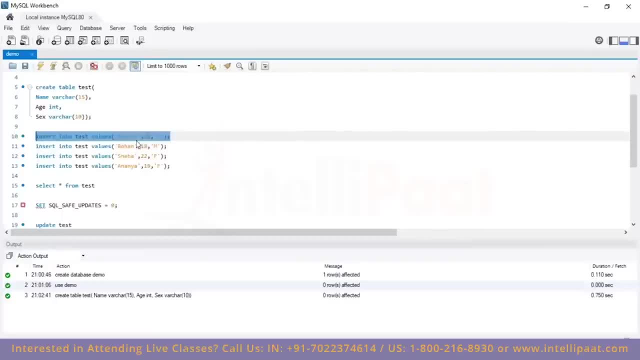 So we can run this query individually, where we go on adding one by one, one by one, In fact. I'm going to show you that right now. So let's run this query. It says that you know, one row has been affected. 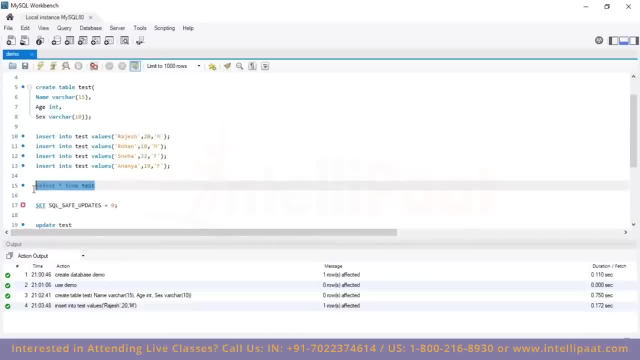 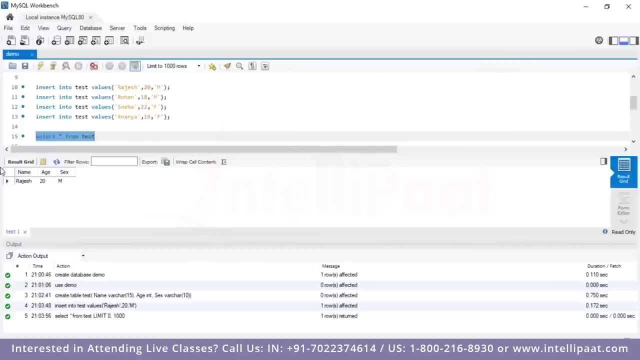 It means that you've changed something in one row of your database. So give me one second, Let me run this for you guys. You can see here, Right, So this is the output. Basically, this is what we call, as a result, grid, guys. 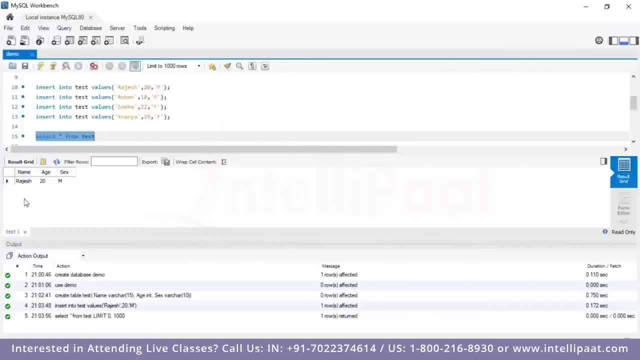 So here we can see that there is a date table created. Basically, there's a database created. There's a table inside the database where the name is Rajesh. He's 20 years old and he's male, So we just used one of these. 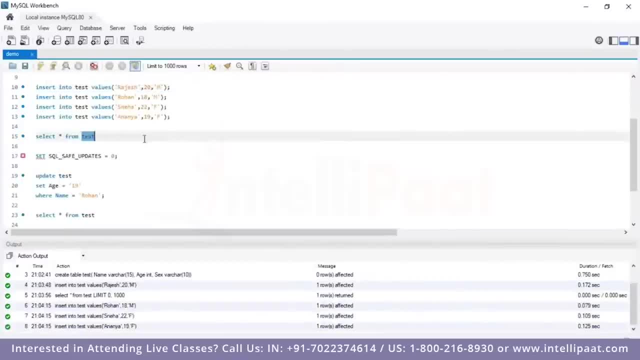 Right, So let me run all of these And then we're going to run this command: Select star from test. You might have seen the. you know pretty much the basic SQL query command that I showed you at the start of the session, where we had something more like a where clause and whatnot. 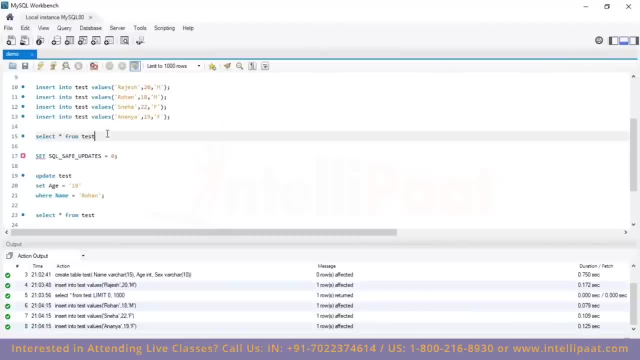 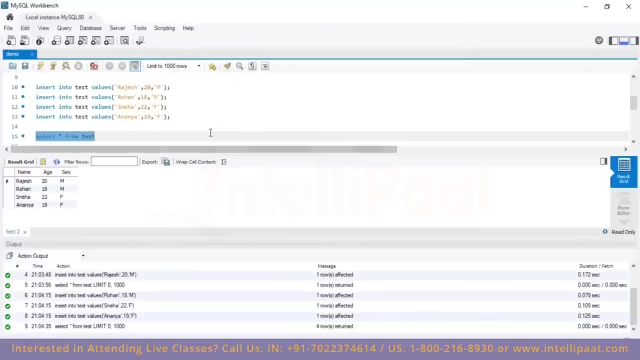 Right, So we can use that as well, But then this will give us the entire entry, present in our date, present in our table. So as soon as I run this instead of just Rajesh, all of the all, the four entities are: 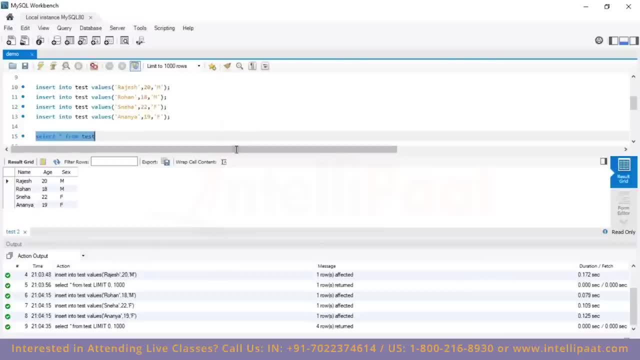 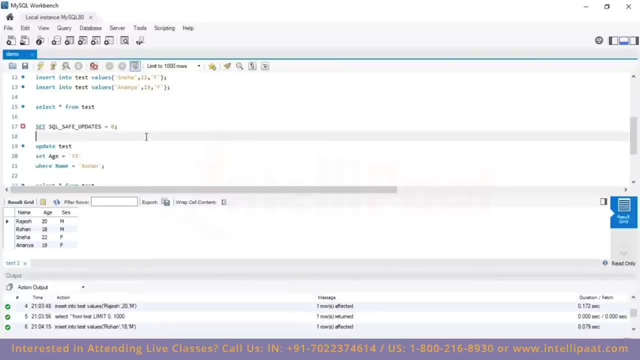 present for us: Rajesh, Rohan, Sneha, Ananya and more guys. So it is pretty much, you know, as simple as. Let me quickly Bring this down a little. Let me bring this down a little. Yeah, perfect. 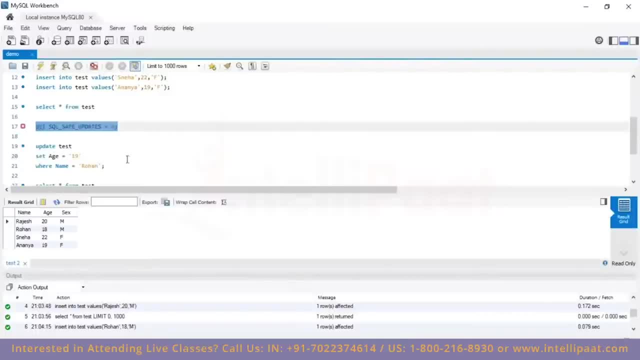 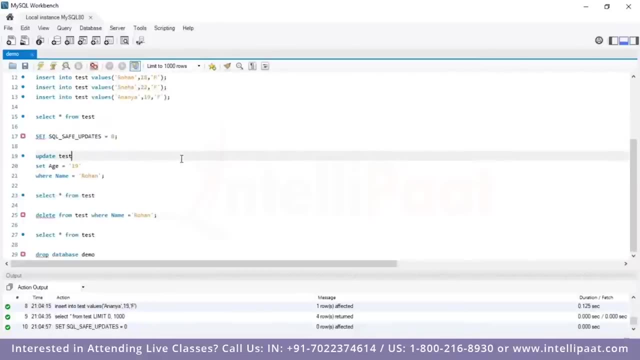 So, then, this command is particularly for MySQL workbench, where we have something called as a safe mode, And we, you know, take away the safe mode to work with the data without having to worry too much about keys, guys. So this is something that you might not have to use all the time. 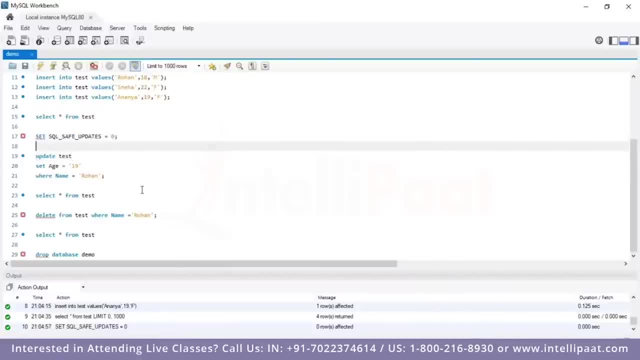 And I just quickly run it to make sure I do not get any warnings or errors: upfront guys. So the next command is: so we've created, since we're doing the CRUD demo, So we're done with the C part, where you have created the database, created the table. 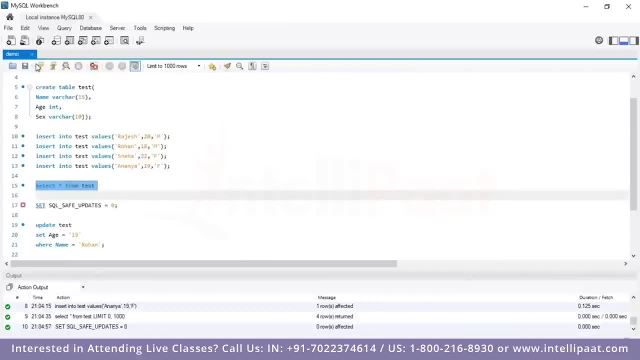 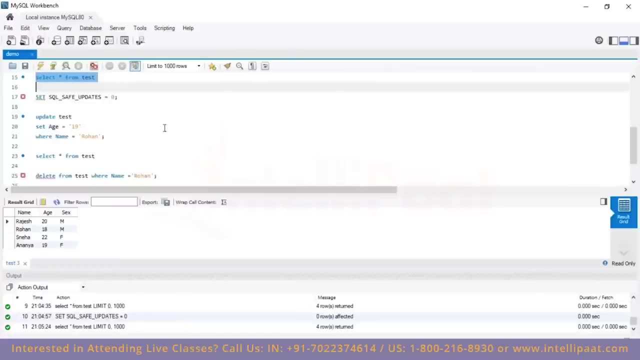 We have read the data, where we use this particular command to pretty much read all the data present in our database. And then we pretty much now are left with U and D, where U is for update, D is for delete, right. So now we're going to update some entry in this table. 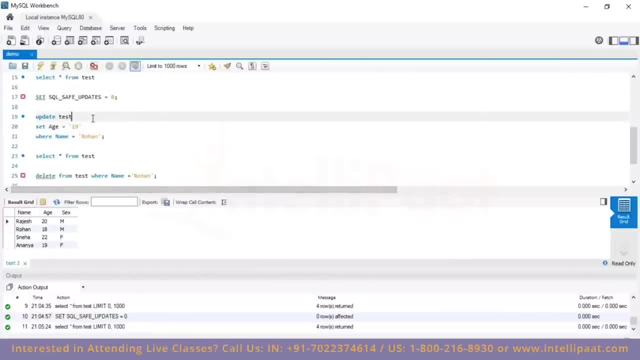 It's not as easy as double clicking and editing guys, So you need to put in queries- and that's why we call it a structured query language- And then, as you guys can see, it is extremely simple. So let me quickly zoom in a little. 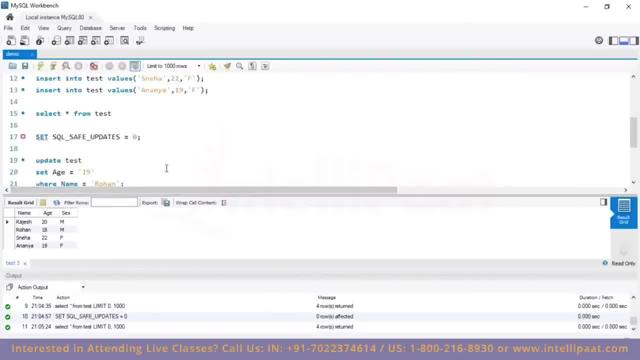 In case you guys are watching this on your mobile or something. So here is the query for updating it. So update the table name. So it's basically: test is our table name, if you can see here, right. So test is our table name. 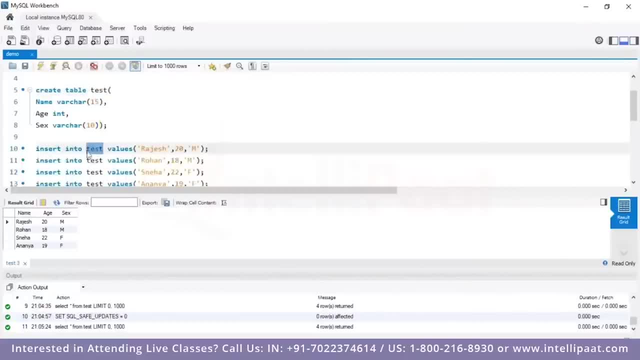 This is the creation command Test again, where we are inserting the data to which we're already done with. We're printing all of the things that we've already done And now we're going to update this particular table and we're going to set age equal to 19.. 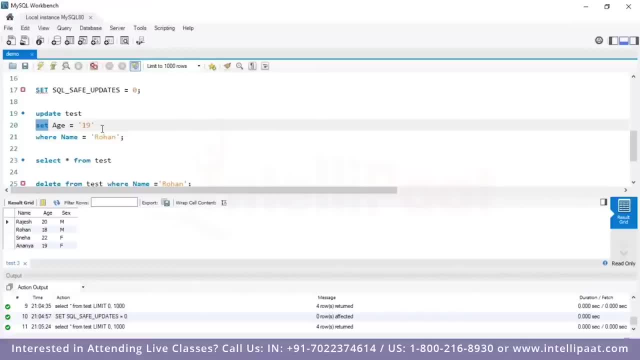 Okay, But whose age are we going to set to 19?? Right, So there are four people right now. We need to tell our database whose age I want to change to 19.. So, basically, that is where the where clause comes into case. 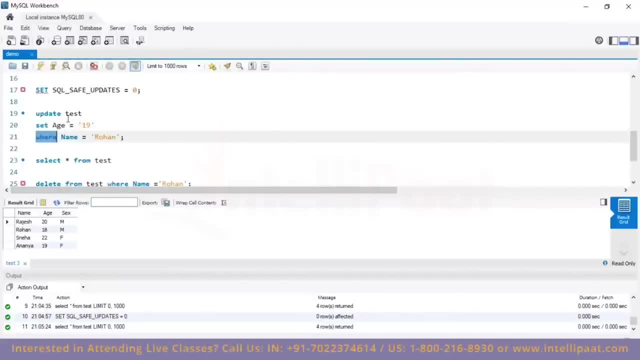 So the where clause says: hey, hey, database, update my date. I know, update my table. set age equal to 19 where name equal to Rohan. So it says: find this person called Rohan under the under the name column and change his particular. 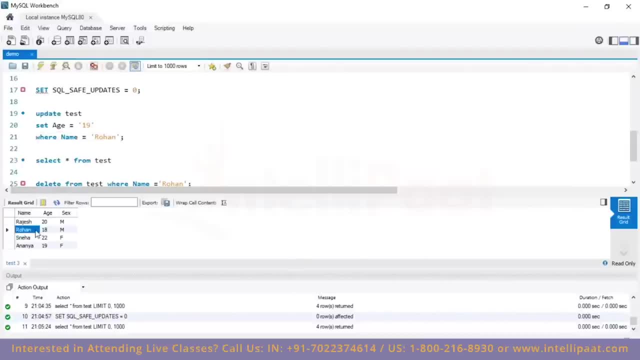 age, whatever it is, to 19.. So Rohan, as you can see in this particular mouse highlight that I've done for you guys, currently is 18 years old. So let's say manually, you might have to change ages at the end of the year or for his birthday. 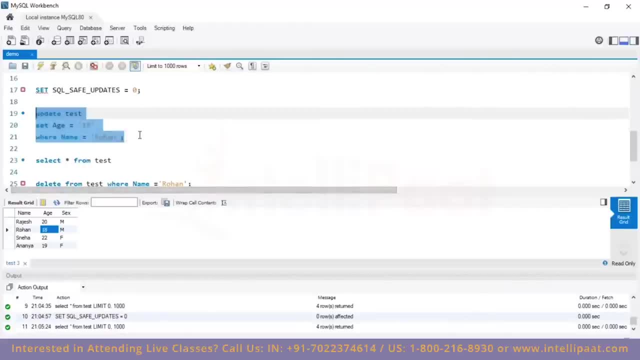 or whatnot. So as soon as I go ahead and run this command, Rohan will not be 18 years anymore. Rohan will be 19 years old. So let me use the select start from test to print the database out And as you can see right. so Rohan is not 18,, he's 19.. 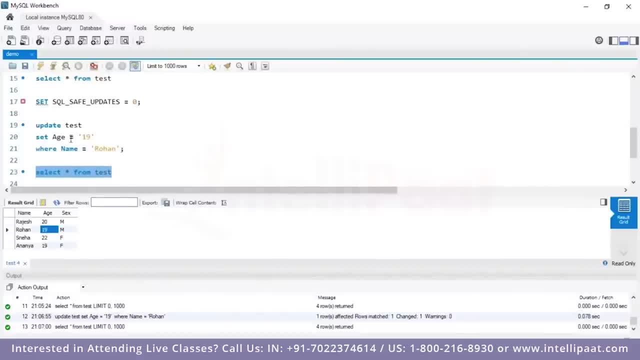 So you can change all as well. So you can change Rohan's name, You can change his sex if you want, And you can have a lot more. This is a very simple database. example, guys: You can have a lot more columns, a lot thousands of entries where you can run complex queries. 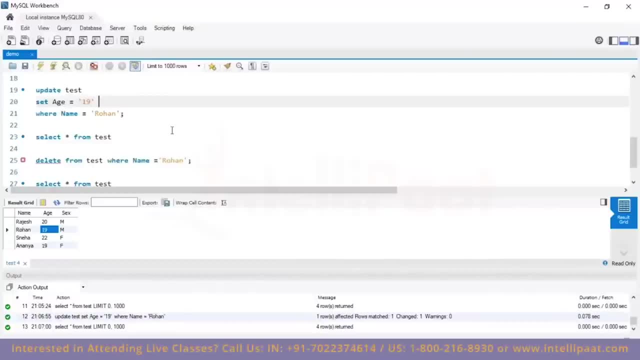 once you are trained to work with SQL as well, guys. So again, as I've said, pretty much my intention here is to just show you the basics and make you guys clear with the fundamentals of the CRUD operations. So now we have updated Rohan's age. 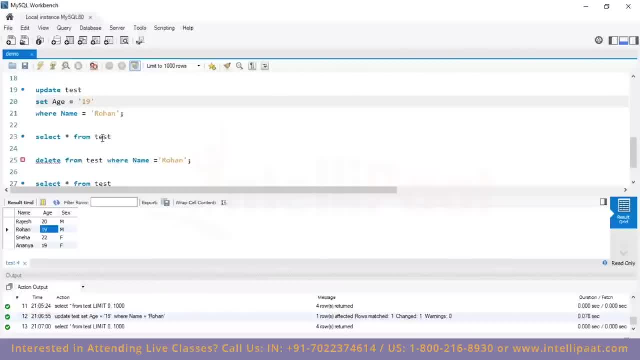 Rohan is not 18 anymore, Rohan is 19.. And pretty much this brings us to the D operation, which is the delete operation Again. so let's say you know, probably Rohan, just you know, cleared out of college and 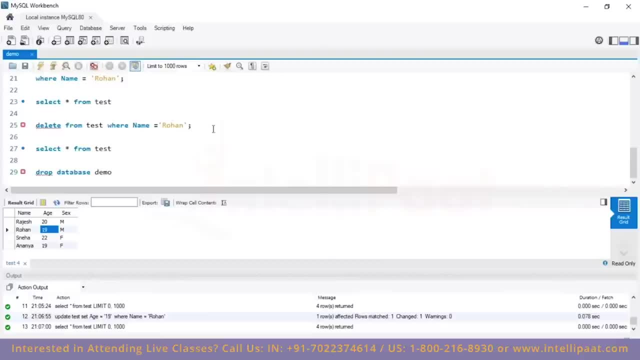 they decided to drop his name from the database and they do not want his name anymore. So delete from the table name or table name is test, where name equal to Rohan. So basically, I am telling you to wipe this So as you can see the mouse highlight and the blue color. I'm just telling my database. 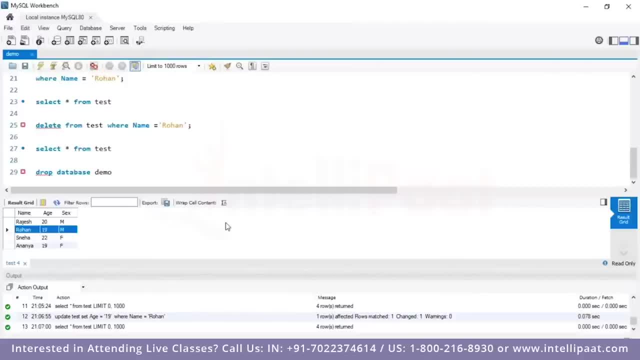 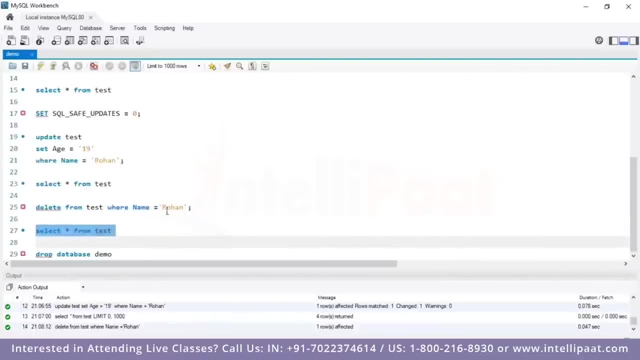 you know what? I don't want Rohan or any particular thing associated with Rohan anymore. So as soon as I run this command, you can pretty much see it. You can pretty much see that every time you run the command, you have to view it. 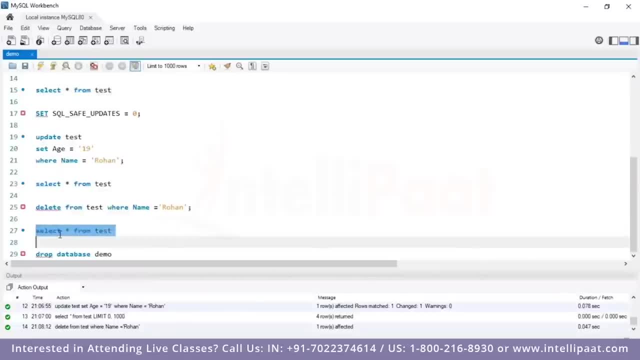 Right. So again, as you can see, I have a lot of select star from tests everywhere present. So as soon as I run this, as you can see, Rohan is not there anymore. We just have Rajesh, Sneha and Ananya guys. 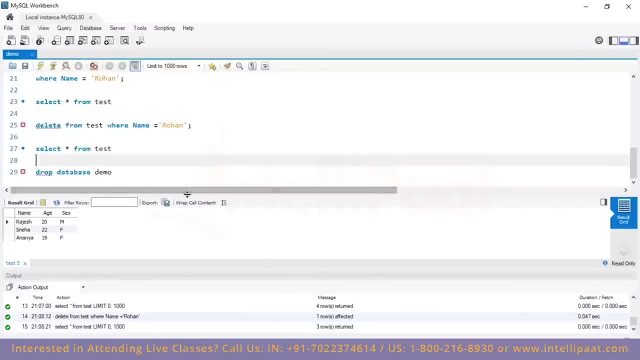 So this, pretty much, is the most simple way you can go on to performing CRUD operations, in my particular opinion, guys. But then if you have to reuse the same thing, you will come up with one particular error case, which I'll just show you right now. 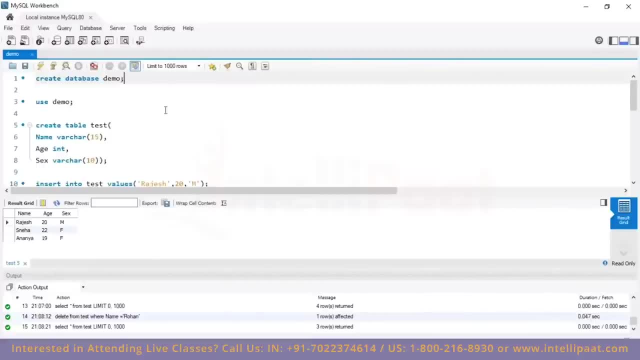 So this is a server architecture, right? So our database, which is called demo, and our table, called test, inside this demo is already present. So if I go out and just run this query again to see what happens, it's going to give me. 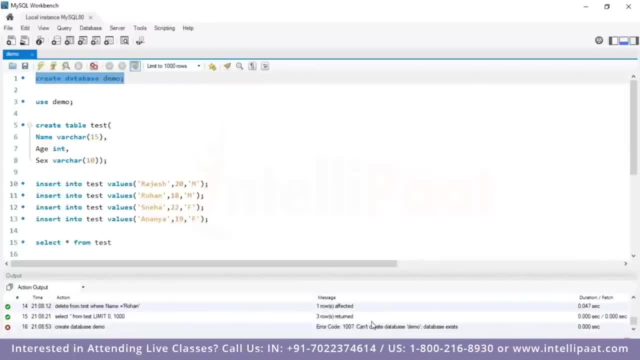 an error. It says: Hey, I cannot create another database with the name demo, because something called as demo already exists. So you're going to have to, you know, change this to demo one, demo one or two. whatever you're going to have to get into that database demo one or two, and then you can use the. 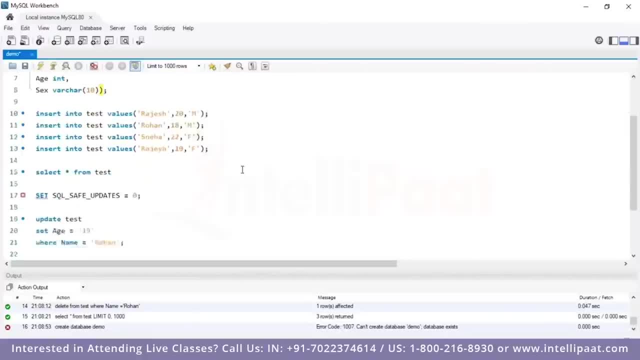 same table name because you're using a different database. Now, guys. so it's as simple as that. So and after you have done everything, if you want to delete an entire database, you know our database can have N number of tables. 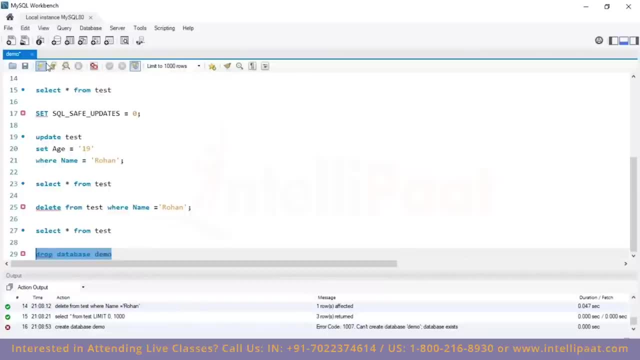 So if you choose to delete all of them, you can pretty much hit drop a database and, followed by the database name and done, It says one row affected, your database has been dropped. So whatever we have done until line 26 from now, pretty much is deleted guys. 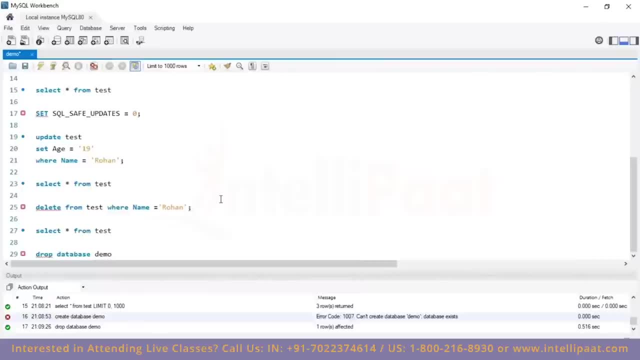 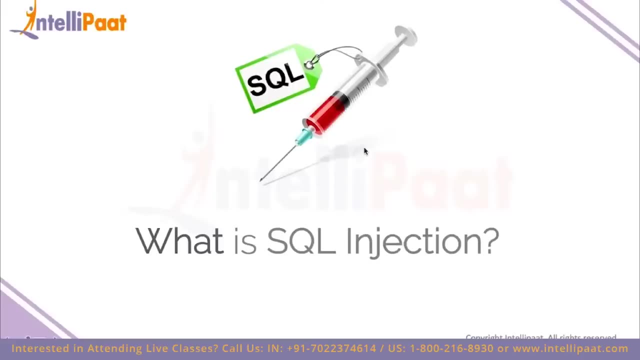 You know it is as simple as this and you can understand the query because it is in such a high level query, It is in such a high level syntax that it makes it very simple for beginners to learn. guys, What is SQL injection? So, guys, SQL injection is basically a method using which you are able to run commands on 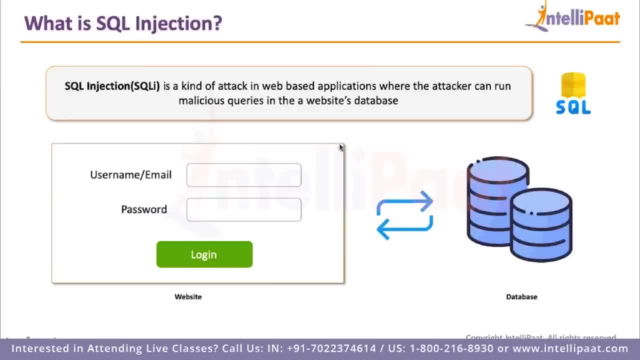 an SQL server or on an SQL database through the user interface of a website, And then you are able to do malicious tasks, such as logging into the website without even knowing the username password of an account, or getting or retrieving the details of a particular database. 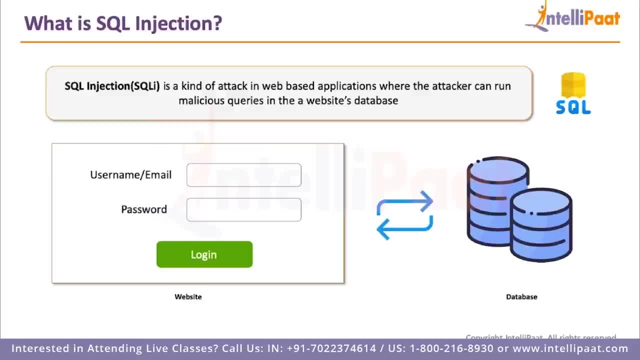 So what we are going to do is we are going to run some SQL commands from the user interface, Right, For example, in this session today. what we are going to do is we are going to have a look at a website like this, which is basically going to have the username, name and password. 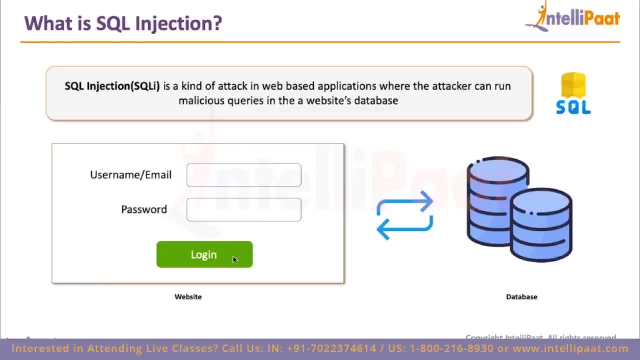 fields And we are basically going to check. when we basically enter the username, We basically enter the password, Then we are able to log into the website. But what happens when you do not know the username or when you do not know the password? 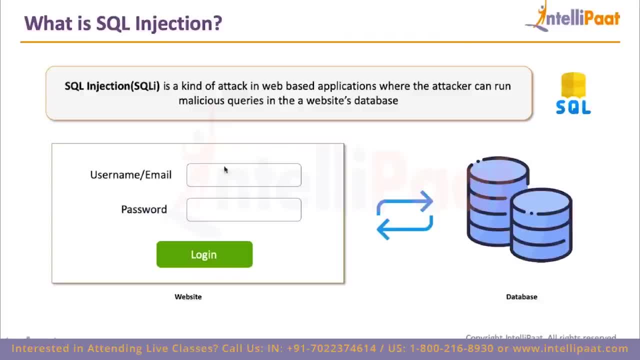 How can you inject an SQL query from this user interface and log into the website without even knowing any username and password Right? So that is something that we are going to understand, And the method of passing SQL queries from a website into the database directly is basically. 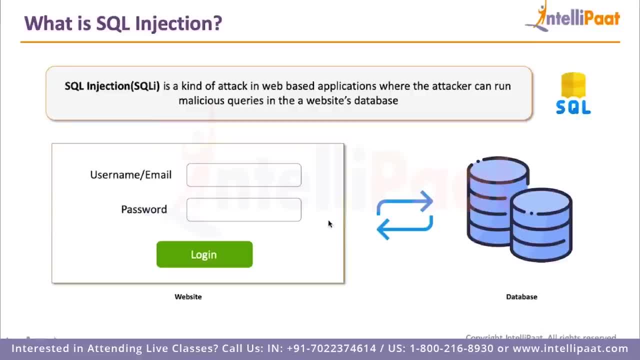 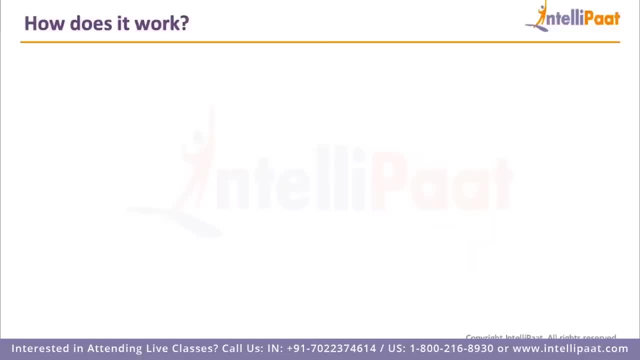 called SQL injection. Okay, So now you might be wondering: how does it basically work? All right guys, So let's go ahead and first understand how does a site work. How does a site basically work? So first thing that you have is a database. 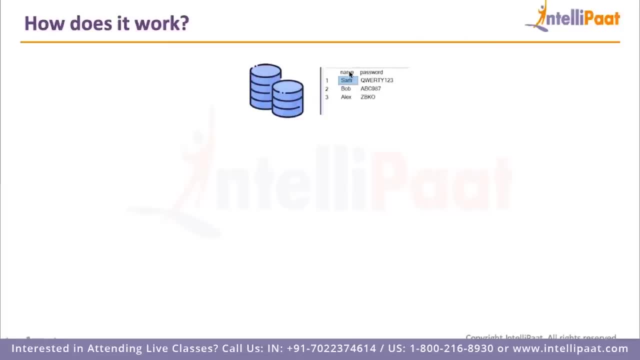 Right, And inside the database, you will have a table which will have all the usernames, which will have all the passwords, And these usernames and passwords will then be basically fetched by a website like this, Right. So, whatever username and whatever password you will be entering, 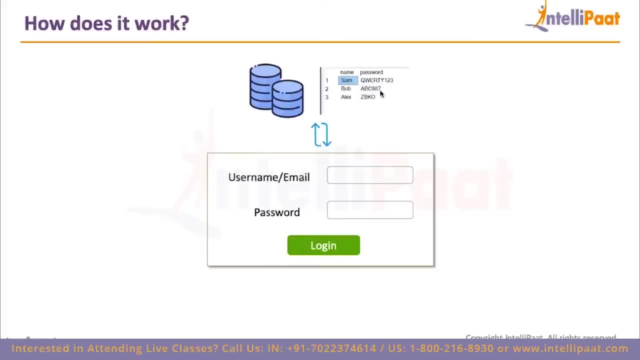 Right, It will be checked against the names and the passwords which are entered over here, Right, If they are an exact match. That is that if the email, Let's say if the username is Sam and if the password is QWERTY123. 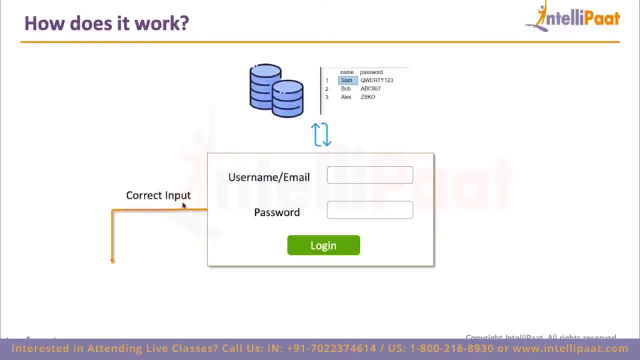 If this matches exactly, that means it's a correct input, And then in that case you will get a success message. In case the username is Sam but the password is something else, Let's say the password is not matching what is there in the database. 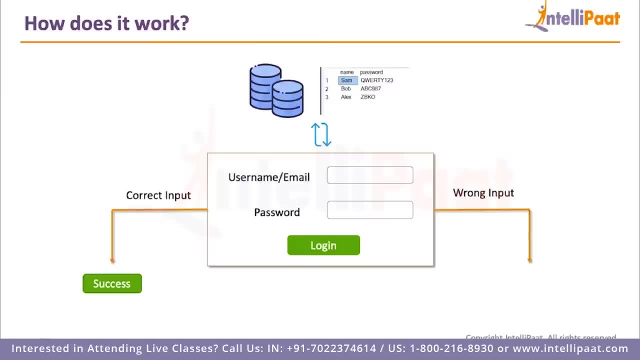 In that case, the output, or the sorry, the input- will be wrong, And with that, even the output will be failed, Right? So first of all, we will need an application which is going to work like this, And what I've done is I've created a sample application which works exactly like this. 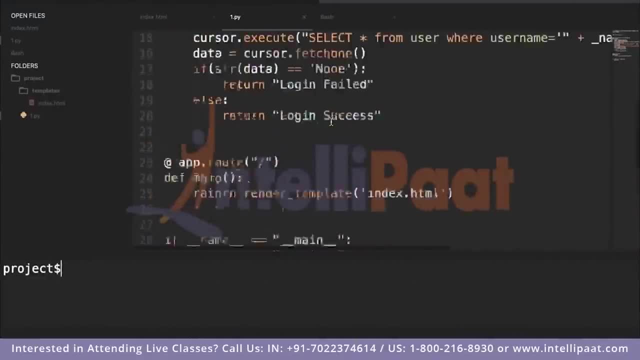 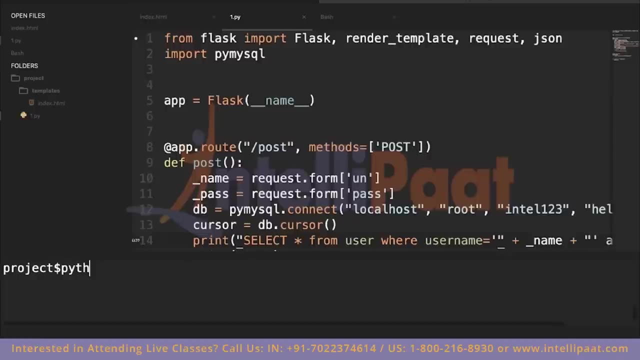 So what I have is basically a website. So basically, I have written some code in Python which is basically going to help us have a web page, Right? So let's run this code. So let me just run it quickly: Python 3.1.py. 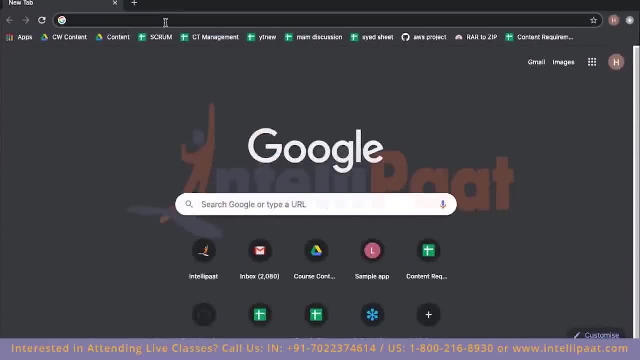 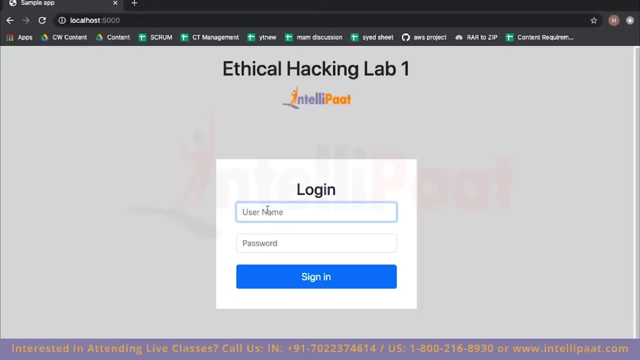 And with this, my code is now running. So if I go to my browser and if I go to localhost- 5000, this is the website which I created. Now in this website, What I can do is I can enter some username. 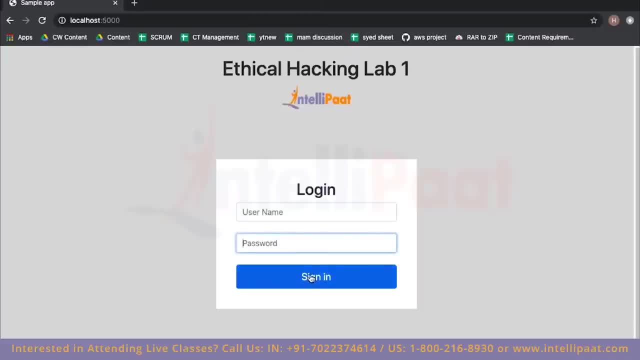 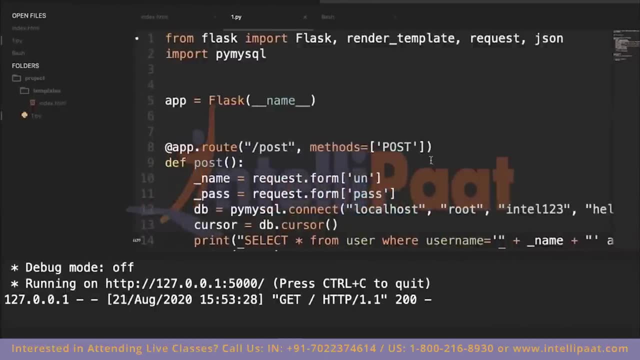 I can enter some password and then I can sign in. I can check whether that username and password is correct or not. Okay, So what is the username and what is the password? It will be basically be picked up from MySQL. So this is: this is the username. 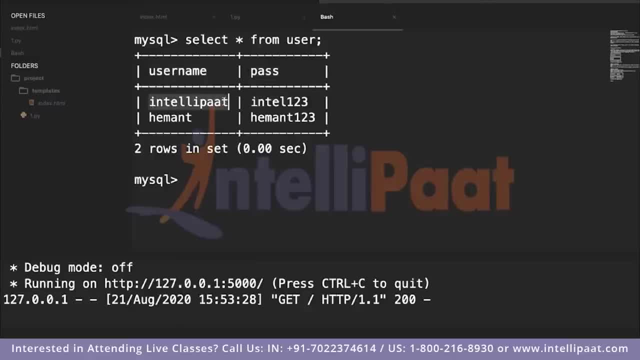 This is the password which I have in the database as of now. So if I enter a username which is Intel apart and if its password is Intel123. In that case, you know, I will get a success message over here. So let us try that. 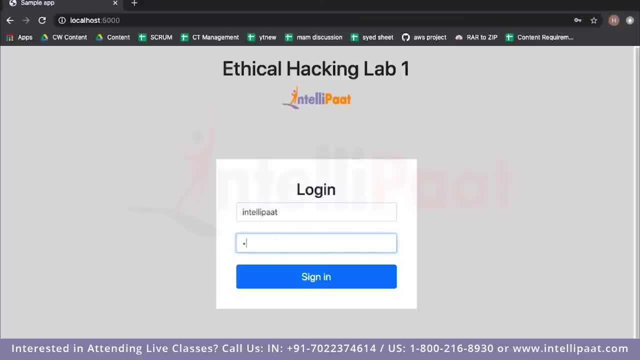 Let us enter Intel apart and let us enter the password as Intel123.. Let me click on sign in and you can see the messages. login is successful. Similarly, if let's say I enter the username as Intel apart and now let's say I enter a wrong password, 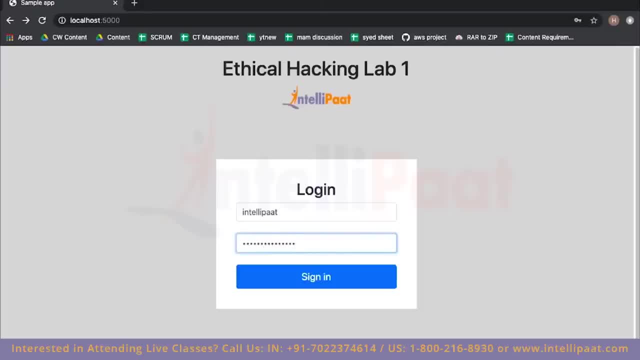 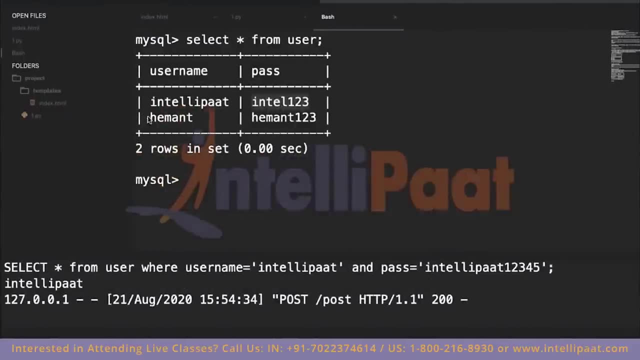 Let's say I enter Intel, part 123.. Let's say 4.. So if I click on sign in, in that case it is going to tell me login failed Why? Because in my database for the username Intel apart, the password is Intel123. 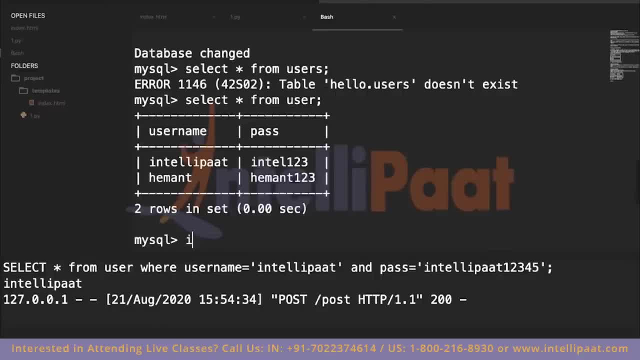 So I can add more usernames over here. So let's say, if I add a username, let's say insert into user, Let me enter a username. Let's say the username is sample and the password for the same is going to be sample123. 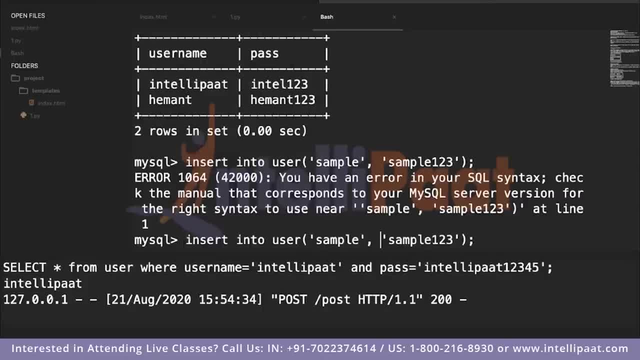 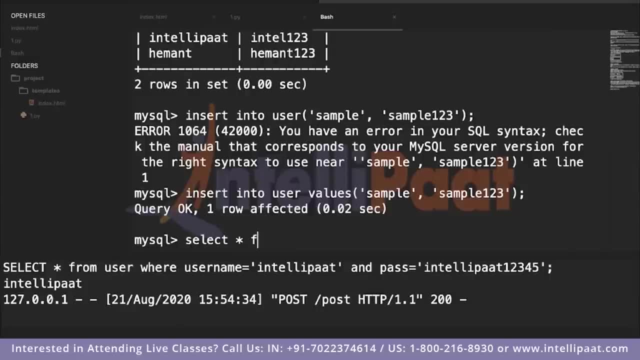 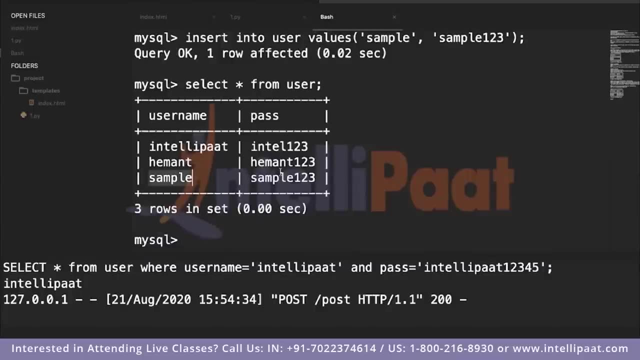 Let's say this is a query that I pass and I missed out on values over here, So let me enter that, Okay. So now, if I check my database, So these are the three records that I have. So my username is sample and my password is sample123. 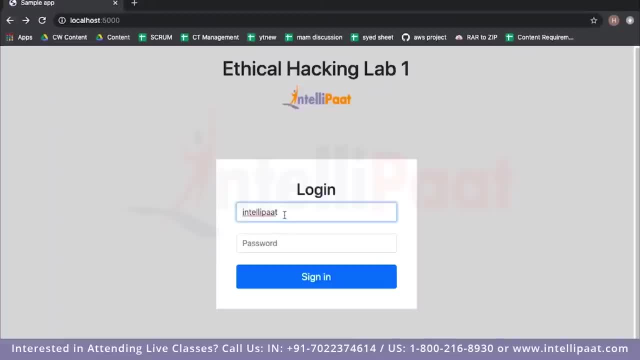 So now, if I go ahead and if I try this out, So if I enter the login name as sample and if the password is sample123., If I click on sign in, you can see the password is login is success Or the output is: login is success. 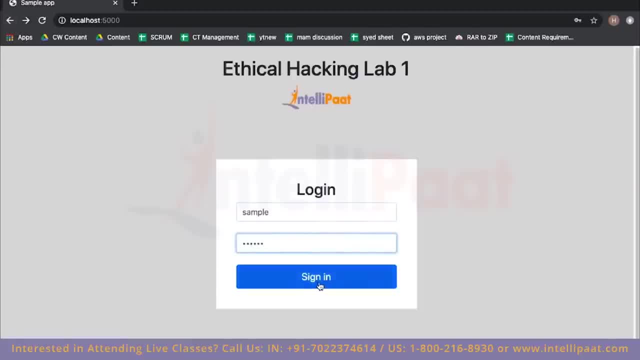 If I, let's say, enter some wrong password And if I click on sign in, it will say login has failed. So, guys, with this, you will now get to know that the website is working right, And this is the prerequisite that you need in order to understand how SQL injection will work. 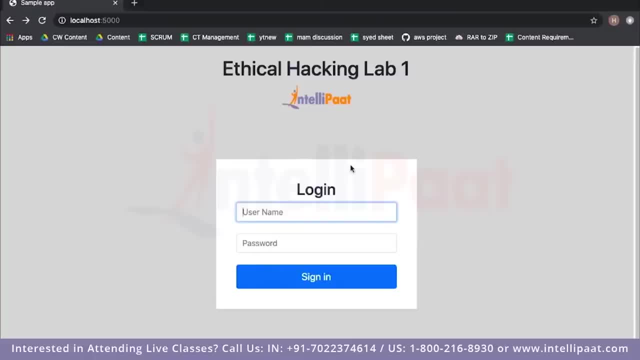 Now what we are going to do is we are going to spoof this website into believing that I am a correct username, Or the username that I am entering and the password that I am entering is correct. Let's see how we can go ahead And understand that, or how to do that. 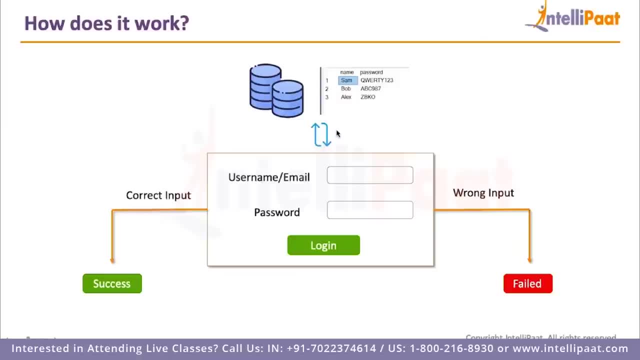 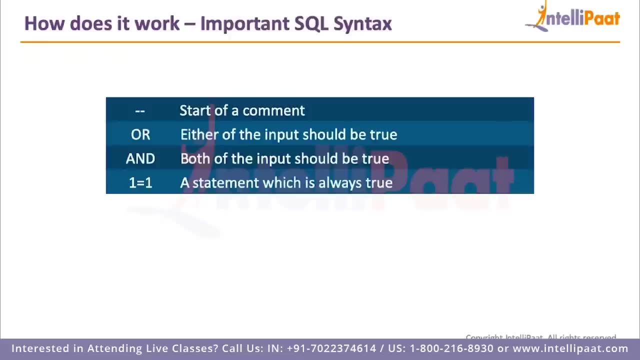 Let's go ahead and understand, But before doing that, you will have to know some basics about SQL injection. So let's understand those basics. So, guys, these are some commands or these are some syntax that you need to know in order to perform this attack. 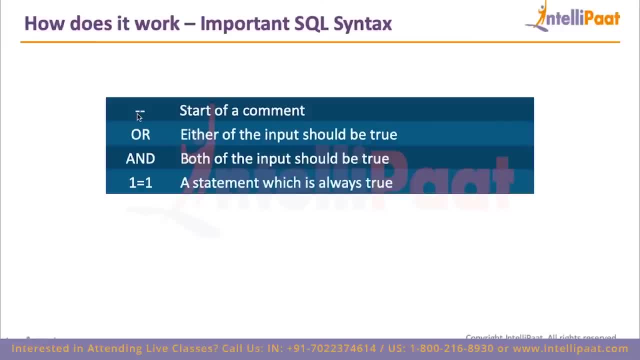 Right. So first of all, what you need to understand is what is the meaning of hyphen- hyphen. So whenever you enter hyphen- hyphen in an SQL query, that basically means it's a start of a comment. What is a comment? 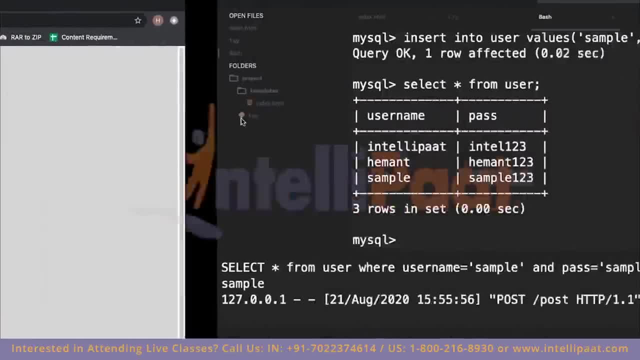 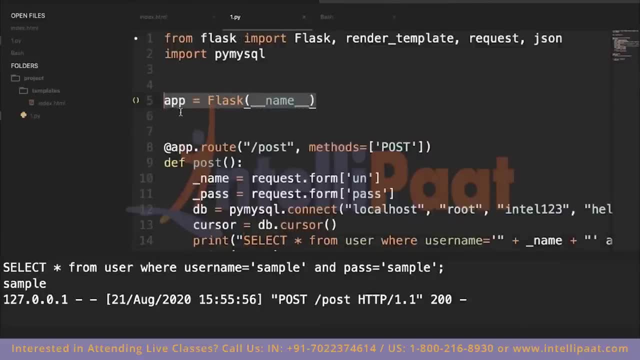 A comment basically means that let's say, in this code, in this Python code, If I want to make this line a comment, which when basically a comment is made, then basically that line is not processed or that code is ignored, Right? So if I wanted to make this line a comment, what I can simply do is I can add a hash in front of it. 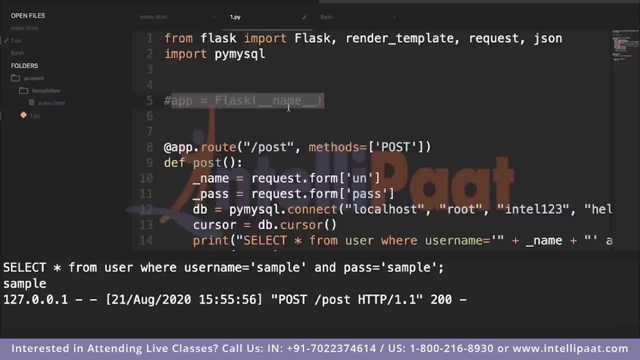 And now you can see this code has now become gray, which basically means, when I will be running this code now, This line will be ignored. So in SQL, if you want to add a comment, the line or the command for that is hyphen, hyphen. 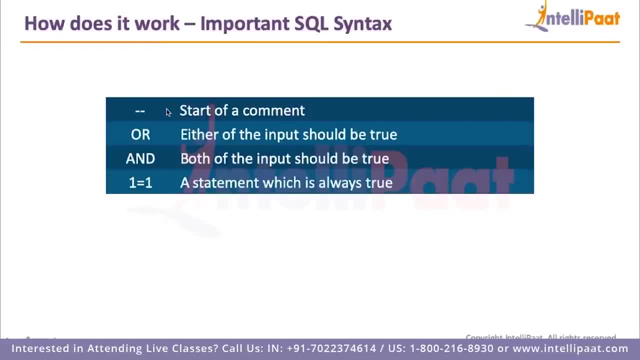 So wherever you will write hyphen hyphen, all the commands after hyphen hyphen will be ignored. All right, Then you have something called as OR. Now what is the OR operator? OR operator basically means either of the input, should be true. 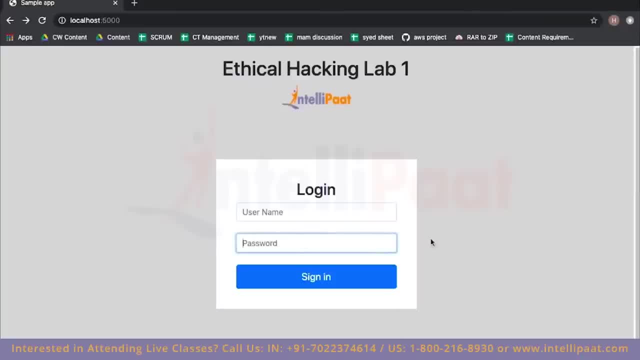 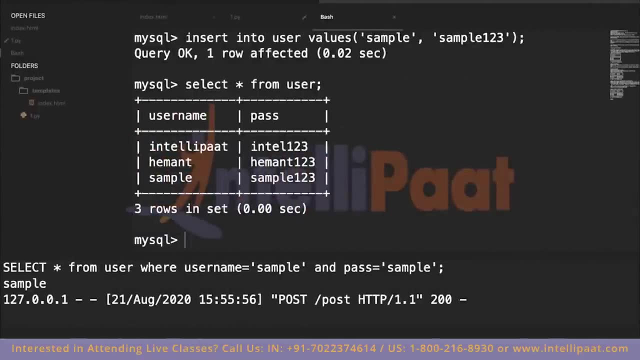 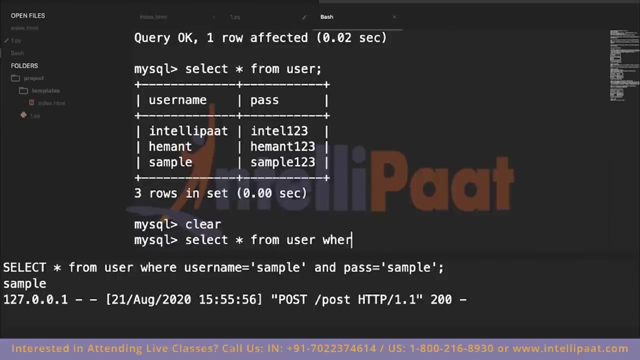 So if I'm using this website, either the username or the password should be correct. All right, To simulate this, let me just go to my database. So let's say I enter something like this: So if I enter select star from user where username is equal to hyphen, 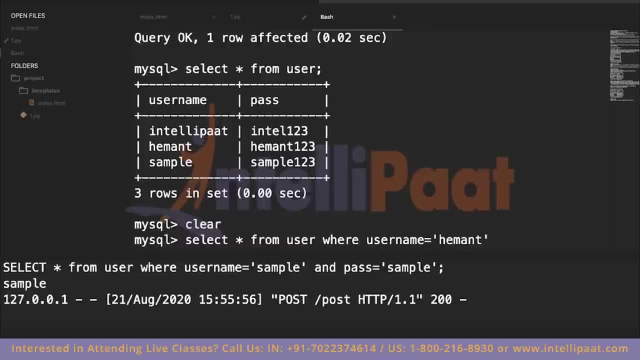 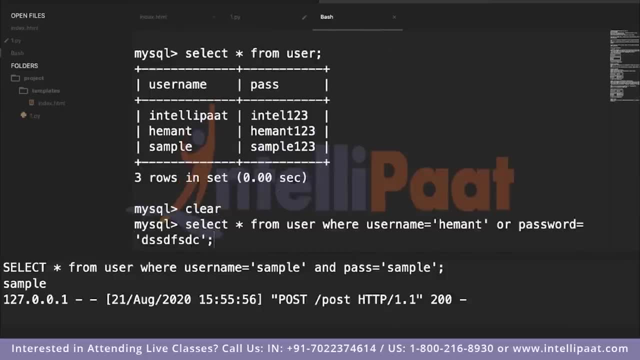 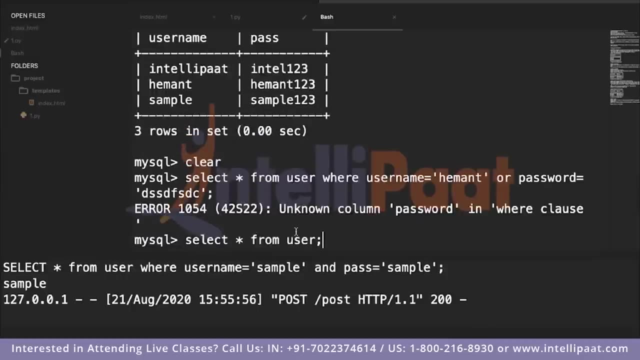 Right, This is correct. The username is there or password is equal to. let's enter something random, Then it should tell us whether this username is correct or not. This is a query. Let it enter. It says password in where clause Okay, So not password. 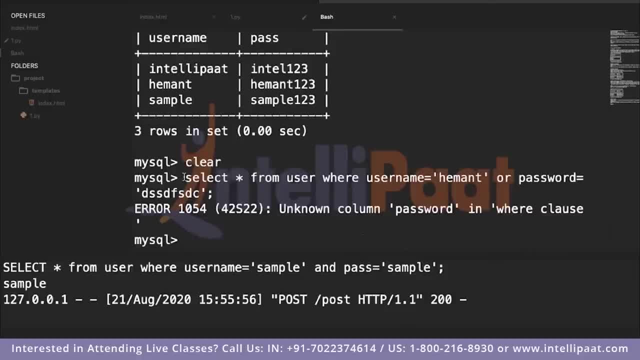 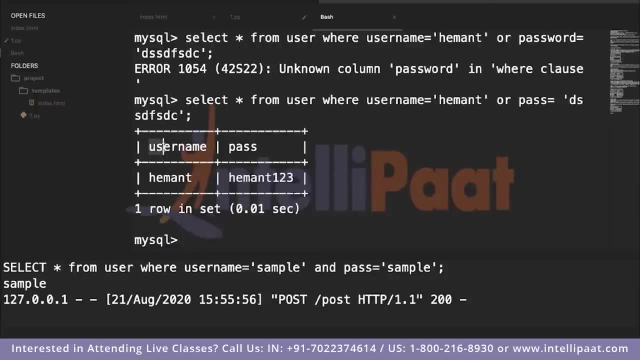 Sorry, It will be pass. The column name is pass. So can you see. it is still returning me the username and password, saying that these exist. Why? Because I've used the OR operator, But this is not the correct output. This is not the output that I want when I'm trying to log in. 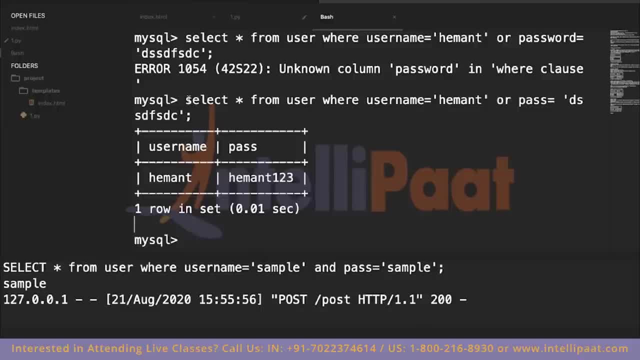 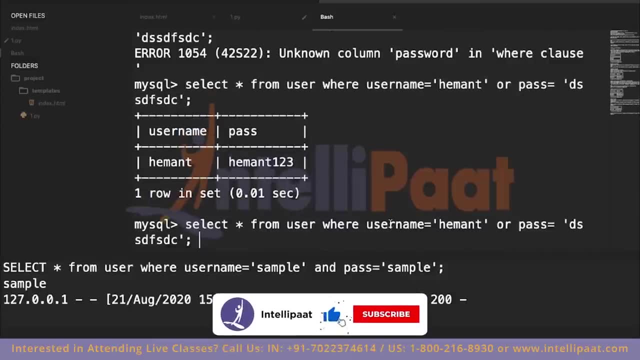 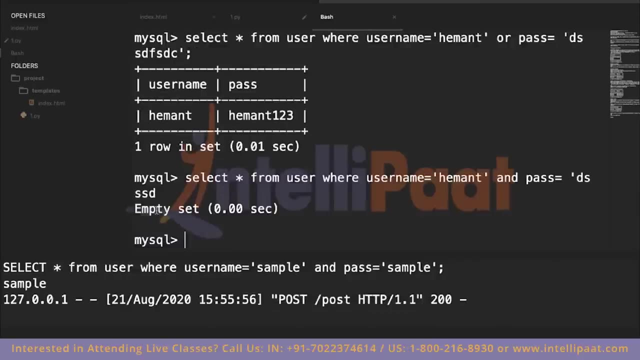 When I'm trying to log in. what I want to do is I want to see whether the username and the password are correct or not. Right, So taking the same statement again. If I change this OR to be, AND, Then it will not give me any output, which means empty set. 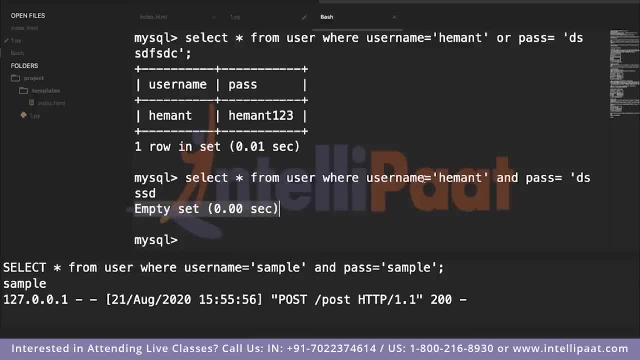 Which basically means that there is no username with the name Hemant and the password this, And hence it will give me a wrong, or it will give me a empty set, which basically means the user does not exist, And hence I will get a login fail. 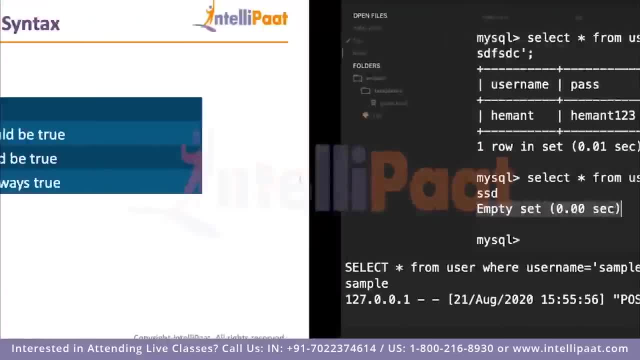 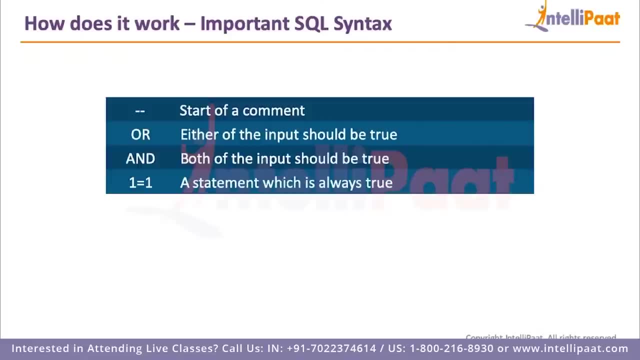 On my website, Right? So this is the difference between OR and AND. So in OR, either of the input should be there in the database, And in AND, both the input should be present correctly in the database. Only then it will give us a successful message. 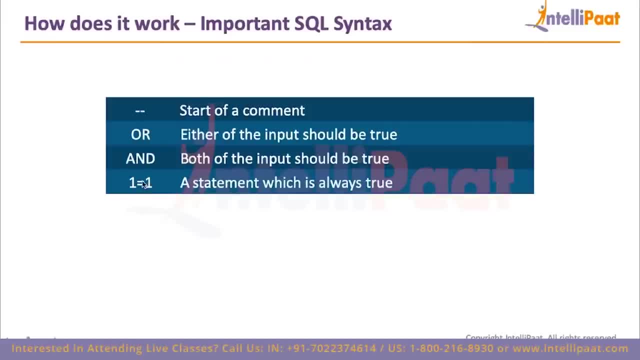 What is one is equal to one. One is equal to one is a statement which is always true, Right, And what does that mean? Whenever I will write, Let's say, if I write when username is equal to Hemant and one equal to one. 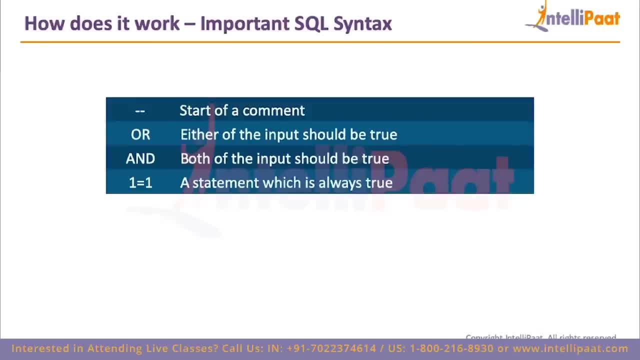 Which basically means that this statement is always going to be true, in case the username is Hemant, Because the second condition is always going to be true, which is one equal to one Right. So this syntax basically means that this statement or the condition is true. 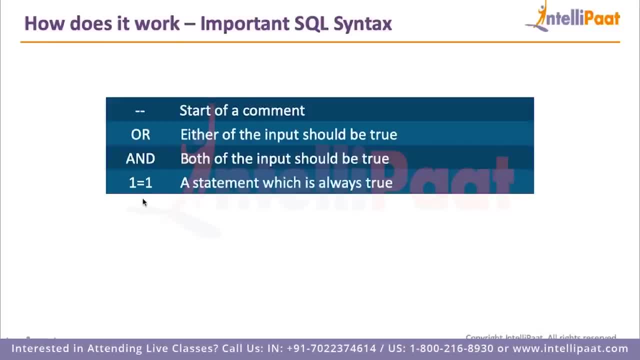 And you can use it anywhere. You can use it while you are, you know, working with an SQL query or when you basically want to go ahead and execute a statement. So now, let's go ahead and try these out And understand how You know will this work when you are working with an SQL query using these syntaxes? 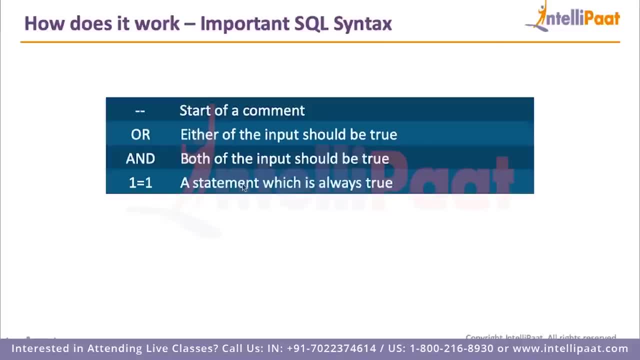 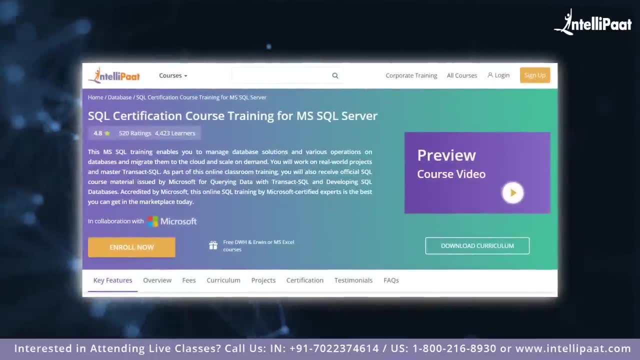 Okay, So let's go ahead and write an SQL query and let's see what the output would be according to what we have just learned. Okay, Just a quick info, guys. Intellipaat provides SQL online training in partnership with Microsoft and mentored by industry experts. 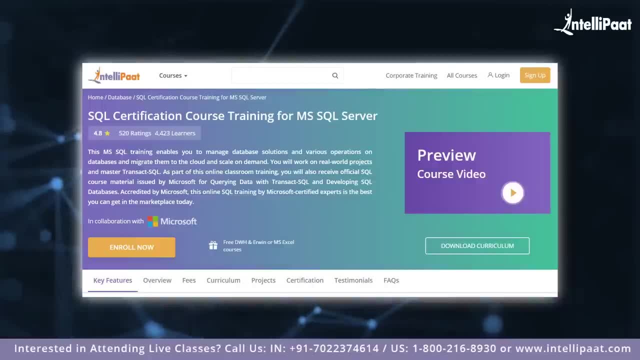 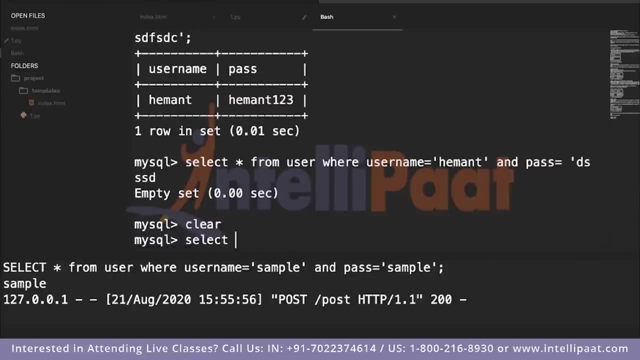 The course link is given in the description below. Now let's continue with the session. So, coming back to my MySQL shell, So let's say I have, Let's say I go ahead and first show you all the records again which I have in the table. 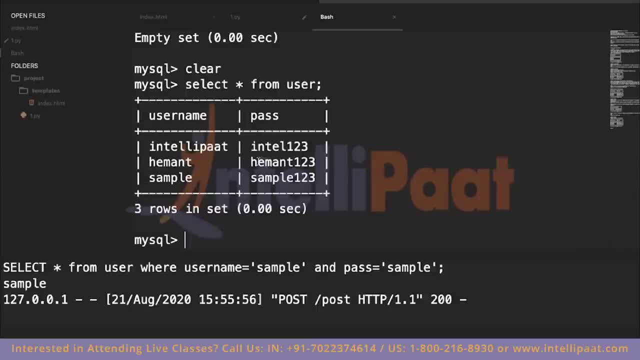 So these are all the records that I have in the table Right Now. what I'll be doing is, let's say, I type in select star from user where username is equal to Hemant and one is equal to one. Now what do you think will be the output of this? 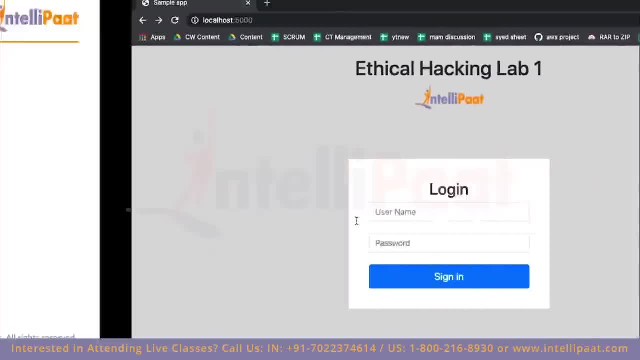 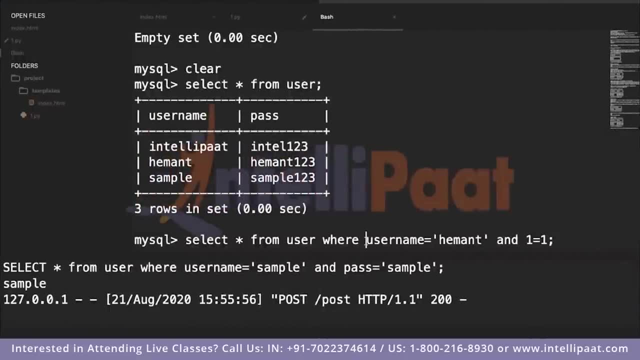 So let's try and analyze. So what did we learn in this slide? We learned that when we use and then both of the input should be true. So do we have username equal to Hemant in the user table? Yes, we do, And this is the condition which we are using. 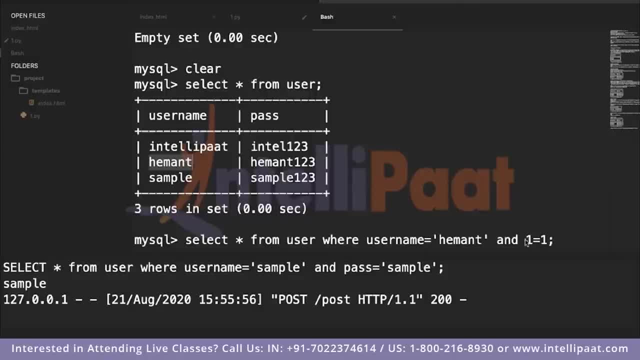 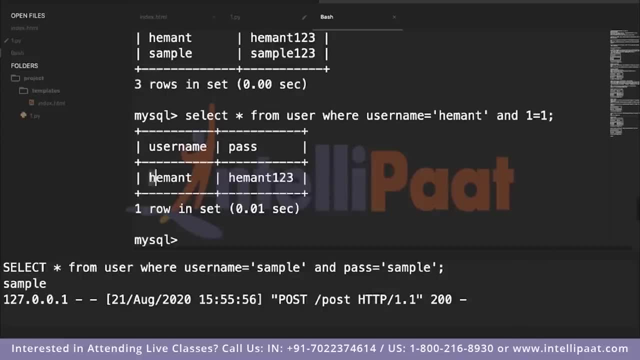 So this is true. Now let's see if this is true or not, And according to what we have learned, this condition is always true. Right Now, if you try and execute this, you will get the username Hemant and the password Hemant123.. 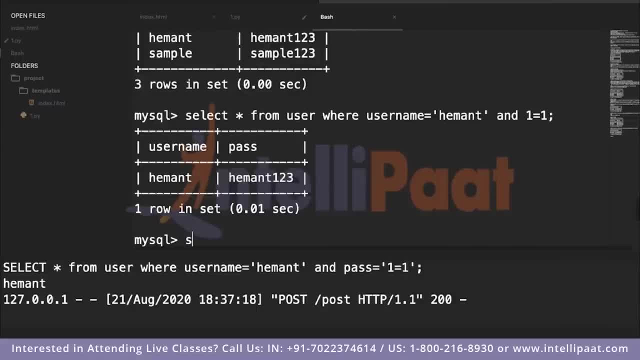 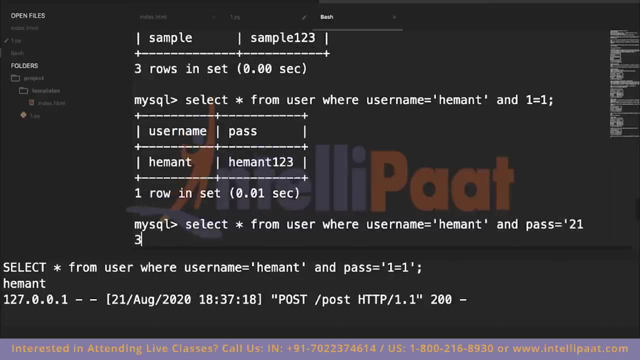 And then if we type in, Let's say, let's say I type in a query like select star from user, where username equal to Hemant and password is equal to, let's say, a wrong password, Let's say it's 12345.. Right, 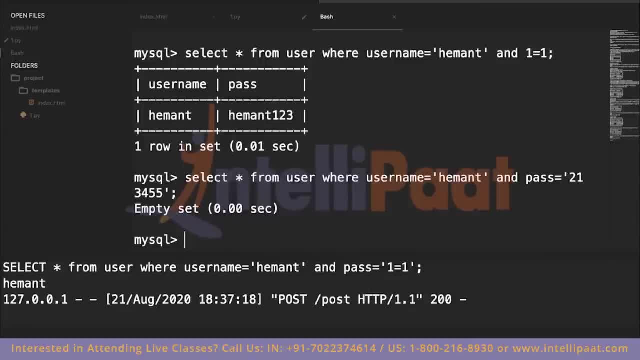 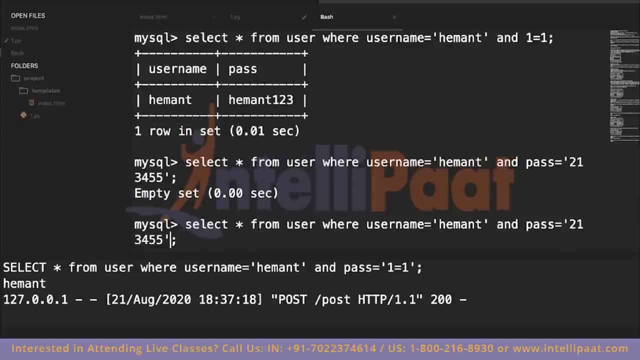 So in this case, it will not return anything. Now let's try to edit this query and let's try to apply the syntax that we have just learned Right. So what we'll do is: First, let's comment out the part which we don't need. 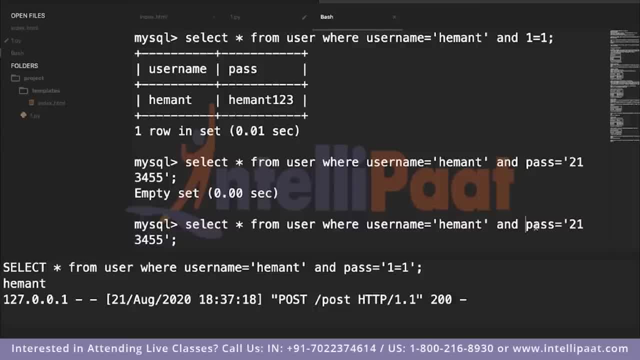 So we don't need the pass the part over here. This is correct, But this part part is wrong, Right? Because of this, the SQL query is not running, So let's comment this part out. So we'll add hyphen- hyphen space. 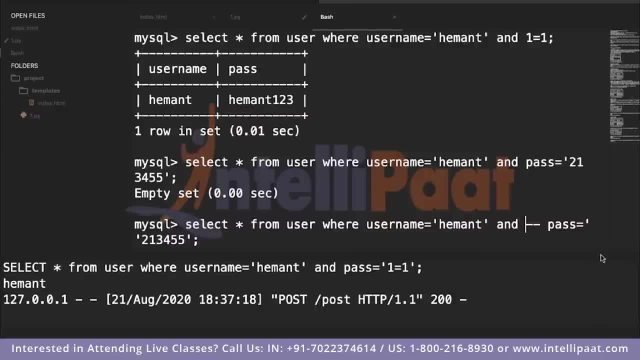 So this part is now commented. And now, if we just enter one equal to one over here and give a semicolon, Let's see what is the output that we get. And now, as you can see, You were able to bypass what you just wrote. 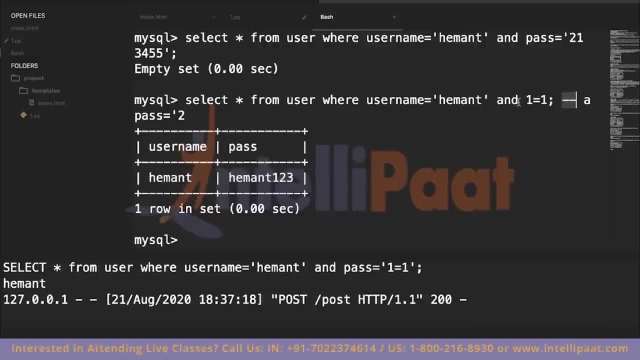 Right. So you commented out whatever was there later And you added one equal to one before that comment- And because of this, this query is just executing up till here- And whatever was there after and you have commented it by adding hyphen, hyphen. 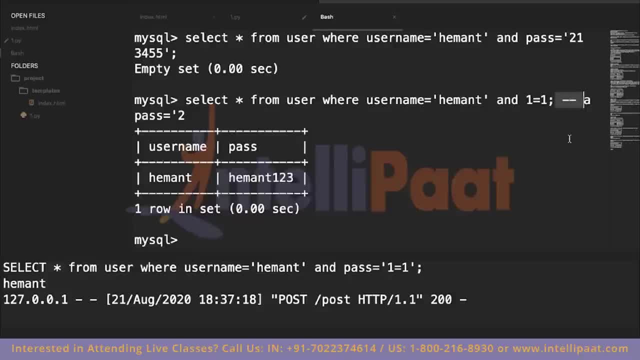 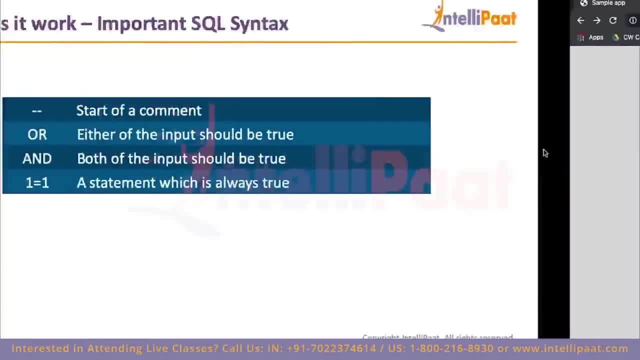 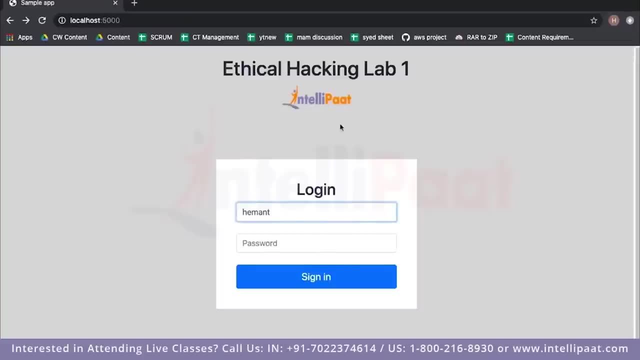 Right, So this is the basics of an SQL injection. If you understand this now, it will be very easy for you to gauge what I'll be telling you later. Right? So now let's go ahead, guys. And now let's try and understand how we can do SQL injection using a website like this. 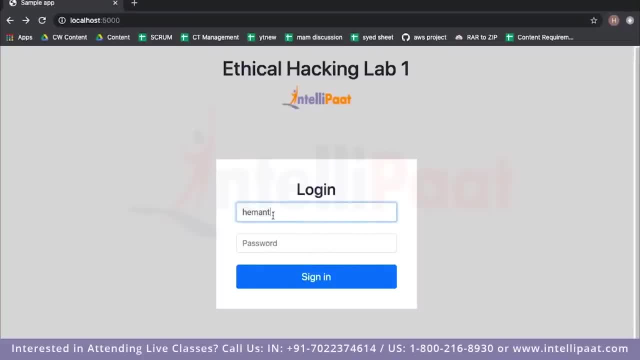 Alright, guys. So what we know of this website right now is that if I enter the username- And let's say this is the correct username, as I know- Let me enter the wrong password over here. So what happens? let's see. So if I enter the wrong password and if I click on sign in, 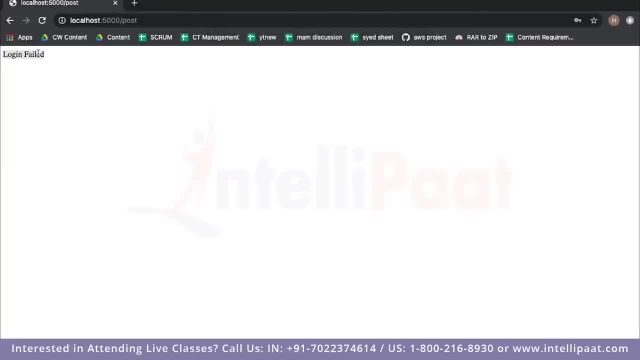 I get login failed. So I want to change this, or I want to achieve that I should get login successfully, So let's see how we can bypass this feature. So, as we know right now that the syntax of the current website is running in the background, 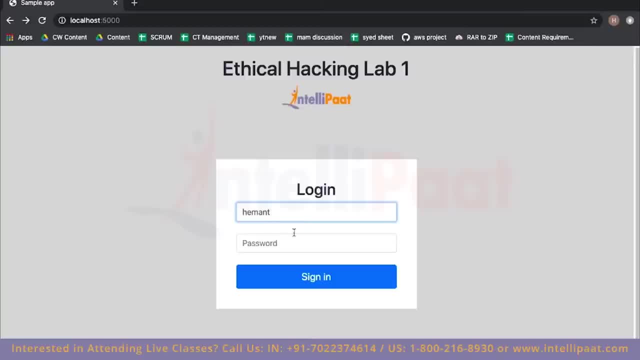 Select star from user, where username is this and password is this. So this is how most of the login websites basically work. Now, in order to achieve an SQL injection query or an SQL injection use case, What I will have to do is I will have to change the SQL query, or I will have to try to change the SQL query. 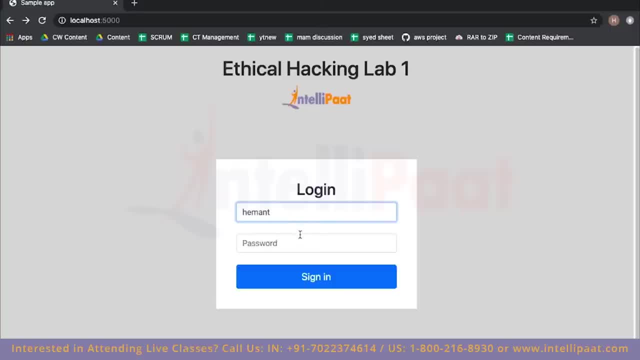 From this user interface, so that I can basically bypass into the system. So how can we do that? So that can be achieved by using the syntax that we learnt earlier, And let me first show you how we can do it, and then I will explain you what would have happened. 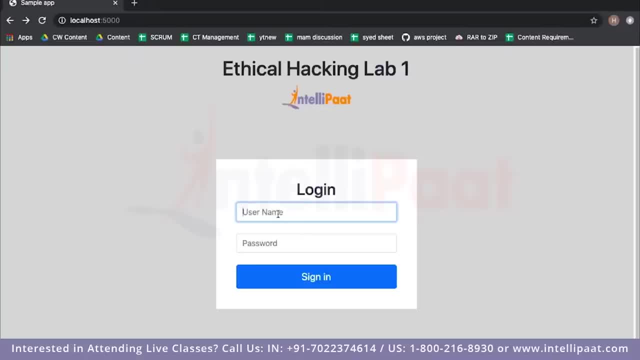 So, before whatever string that I am entering over here, that will have a semi, that will have an apostrophe starting before it, Or that will have an inverted comma starting before it. So let me close the inverted commas first, And then what I will type in is: I will type in: OR: 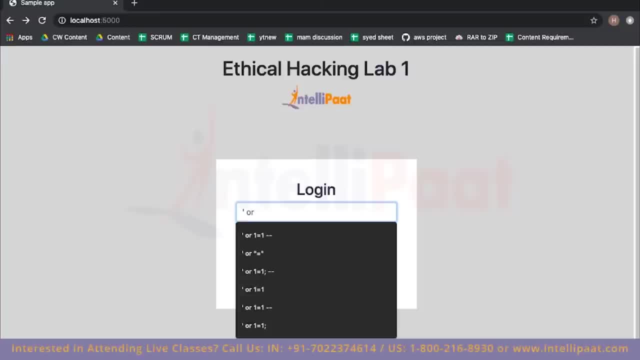 And then I will type in the query which is always going to be true, which is: 1 equal to 1.. Right, and then I am going to close this statement And after this, whatever is there, I am going to comment it out by typing in hyphen, hyphen and then space. 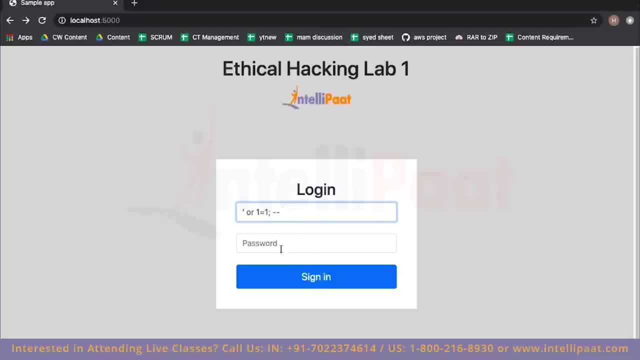 Okay, so this is, you know, the argument that I am going to pass over here, And now let's click on sign in. So it says: this field is required. No issues, you can fill this field. And now let's click on sign in. 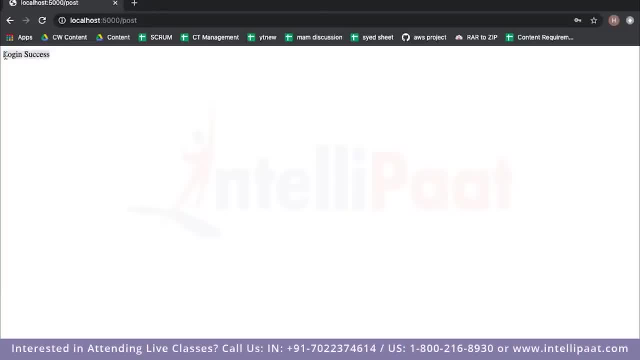 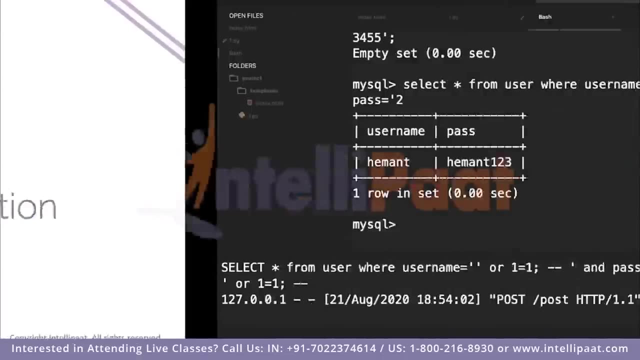 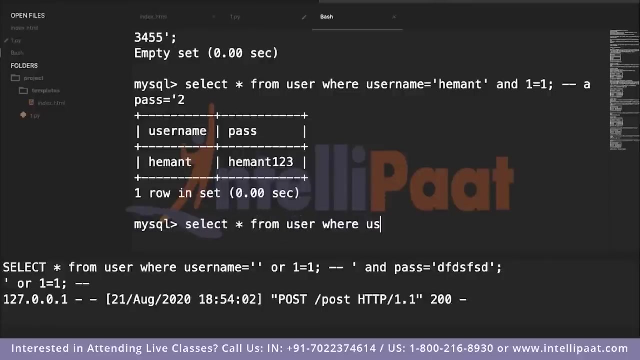 So now, as you can see, it says login success. Now, how do you think this would have happened? Let me go ahead and show you. So the query that we have in the code is: select star from user where username is equal to Hemant. 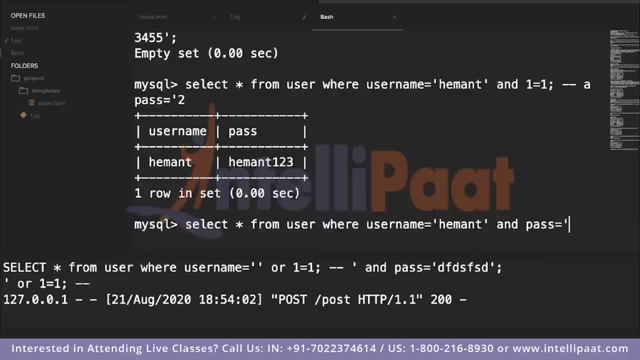 And pass is equal to Some password. Okay, this is the query which is executing in the background. Now what I have done is I have replaced Hemant with a string which goes something like this: So I first entered inverted comma, Then I entered a space. 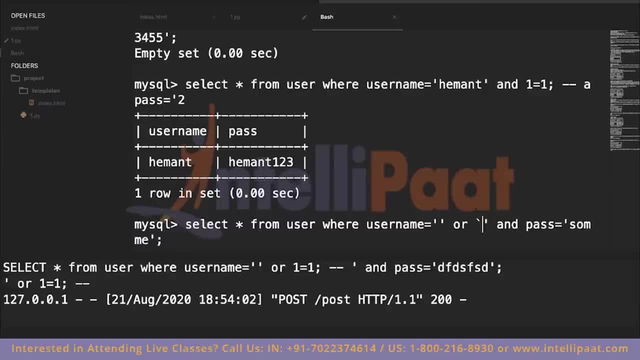 And then I said: OR 1 is equal to 1 semicolon space, comment sign and then space. Now see what has happened. This query Has now changed to this query And I have commented the rest of the part out. Now, if you execute this query, what will you get? 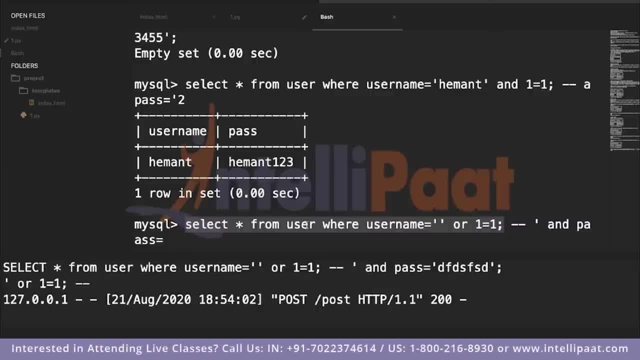 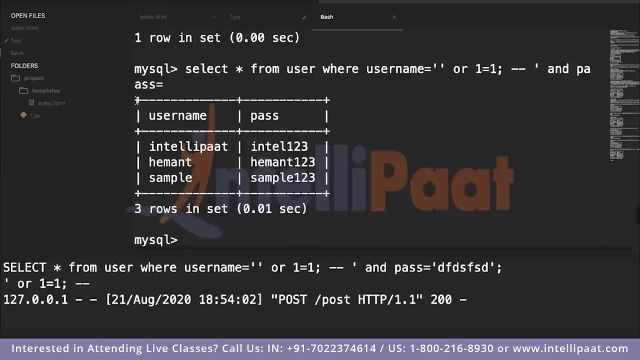 You will get all the usernames and you will get all the password. Let me hit enter. Can you see? I have got all the usernames and I have got all the password. And because this is something which is not an empty set, The website is now telling me that the login is successful. 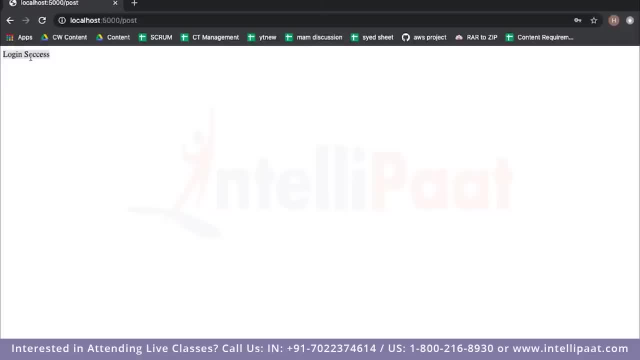 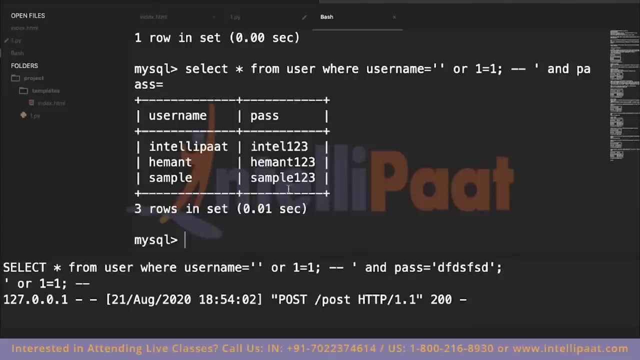 So, guys, this is a very simple and this is a very dangerous SQL Injection that we have just done, Because not only you have got access to the website, Not only you have spoofed the website, But in case you are able to get this result set out through some method. 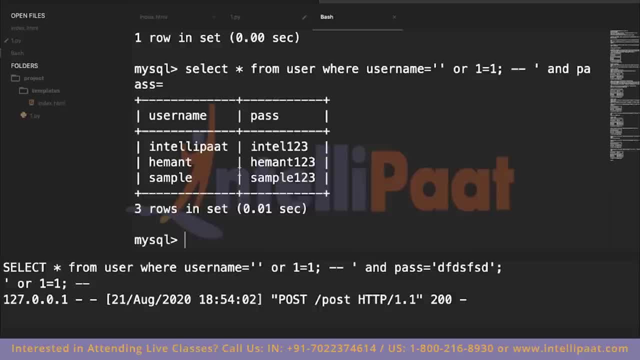 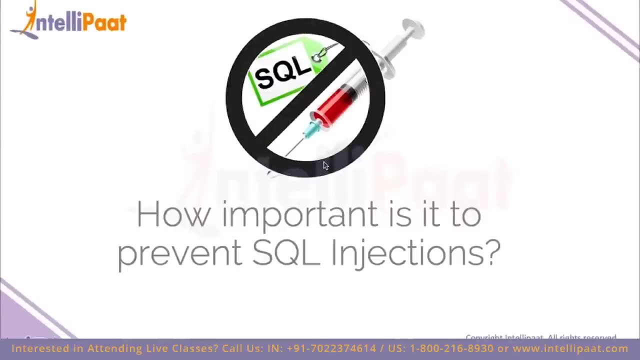 You will be able to get all the usernames and all the passwords that are there on the database of this website, Right? So, guys, this is how you do SQL injection. Now that we know how SQL injection works, How SQL injection is done, Let's go ahead and understand. 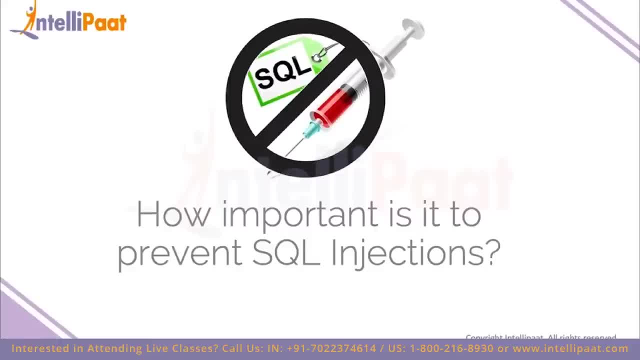 Is it really important to prevent SQL injection? So you might be wondering now, Whatever I have told you, Not a lot of people will be knowing about it, Right, And that is actually true. Not a lot of people know about how to hack websites. 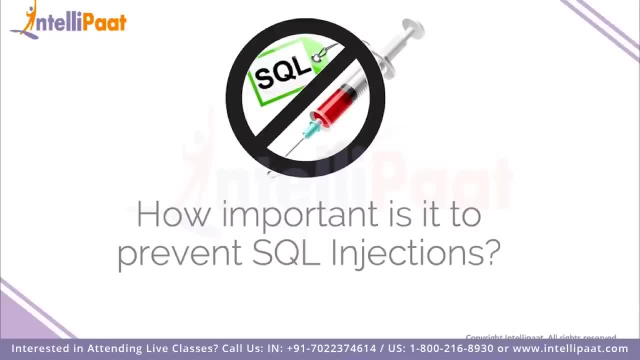 Or why would? What would be the purpose of someone hacking your website? So probably it just happens to big companies like Sony, Like LinkedIn, Like Twitter, Right, So why should you be worried about it? So that's a valid point. But imagine right now if you are doing a startup. 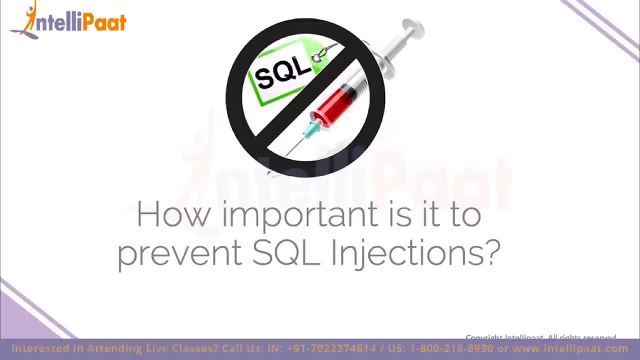 Right, Probably right now the need is not there, But if something like this happens to your website? Because, as we are growing towards a more technological world, A world which is more online, More and more people are getting the skill sets to work online or use the internet. 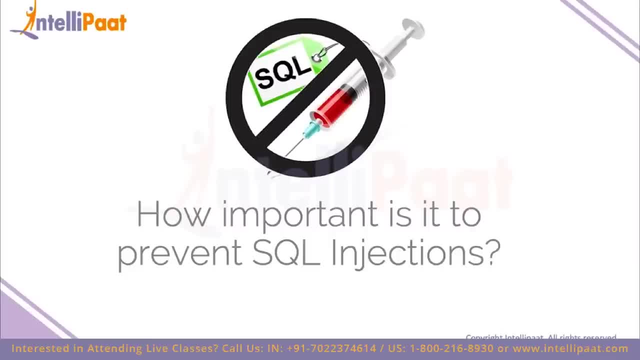 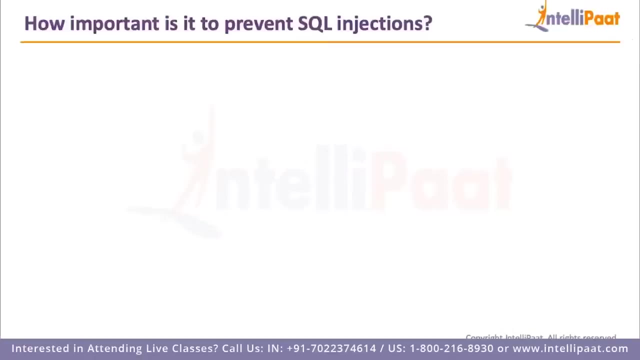 And with that, if, let's say, somehow somebody targets your website, It is going to be a huge loss to your business because the users which were using your website will not trust your website anymore. So to sum up, what is it important? to prevent SQL injections. 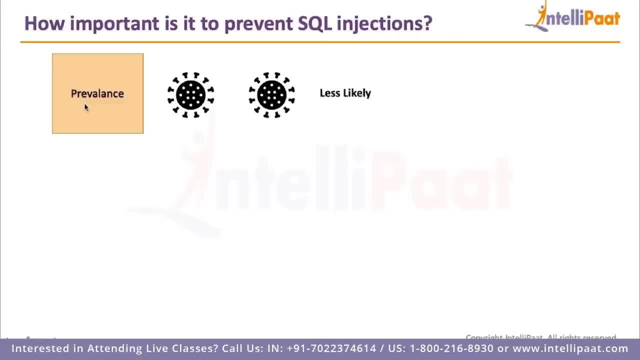 The point is that, yes, the prevalence is going to be very less. The attack might be happening to your website or it might not be. The chances of it happening is very less because there are very less individuals in the world out there who can do SQL injections. 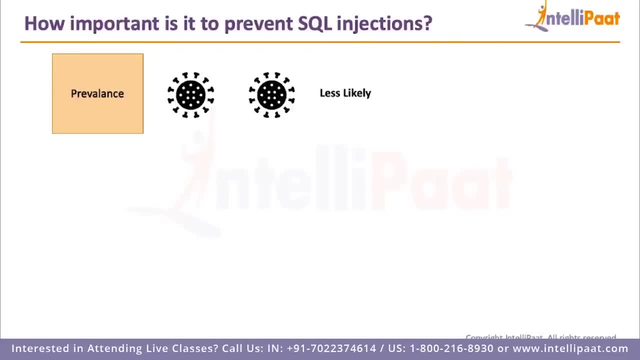 Right, And who would want to target a very small company that you have just started? But does this mean that you should ignore it? Well, no, Because the ease of exploitation for this particular subject that we just discussed is very easy. Right, And with that, in the future, as in when you know, we are going into the future more and 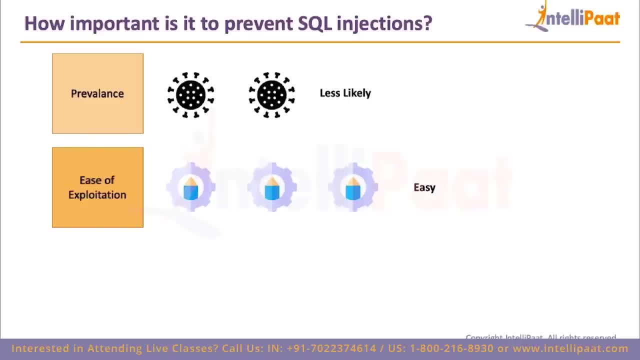 more people will get aware about this particular concept, this particular technology, And hence the chances of even somebody pointing out, Even somebody playing around with your website, is going to get you a huge business loss, Right, And that's why the impact of this is going to be devastating. 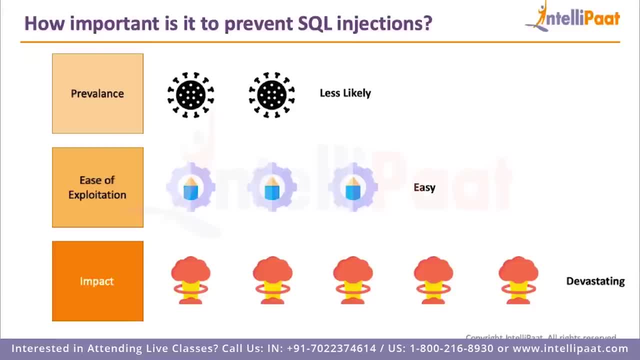 So that's why it is very important to prevent SQL injections, Be it a very small company, Be it a medium sized company, And it is important for large companies. obviously Right, And that's why you should learn all the best practices for development. 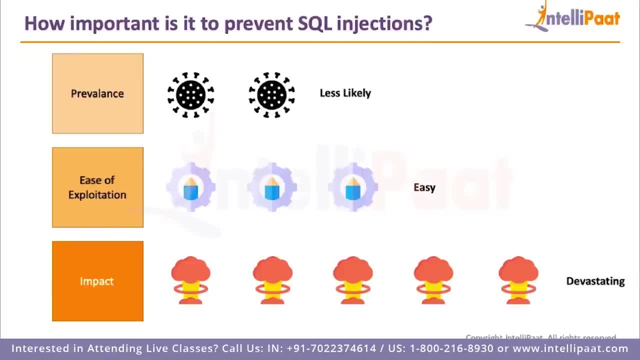 You should include people in the team who are cybersecurity experts. You should have test cases in your development team, which is basically going to go and help you out in understanding if your code is safe or not, Because it does not matter if your code is just working. 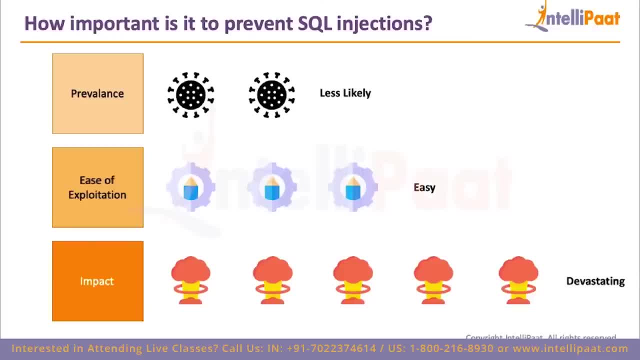 Your code has to be safe as well, And this is why you know the demand for ethical hackers, the demand for security specialists, is now increasing day by day, because companies have now started to recognize that, yes, this is a threat. Yes, this is something that needs to be addressed. 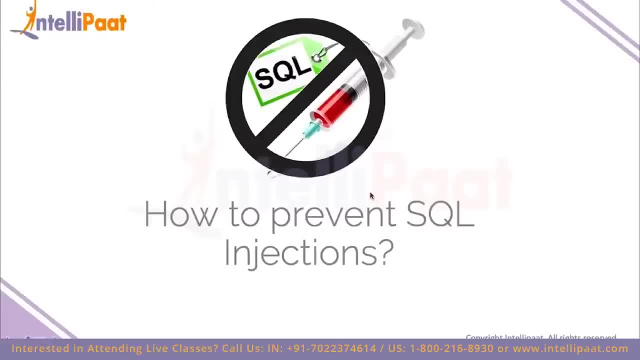 OK. So, with that said, how to prevent SQL injections, Now you will say, OK, So it's very important to prevent SQL injections, But how should you go ahead and advise a company so that they can prevent SQL injections? So let's understand that. 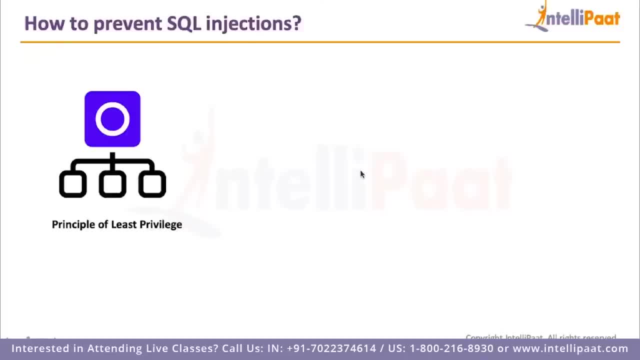 So first thing is you should use the principle of least privilege, which basically means, let's say, this website is able to, you know, insert or select data out of the database. So this website should have a username. which has a user name, This has the least privileges allotted to it, so that it can only do what it is supposed. 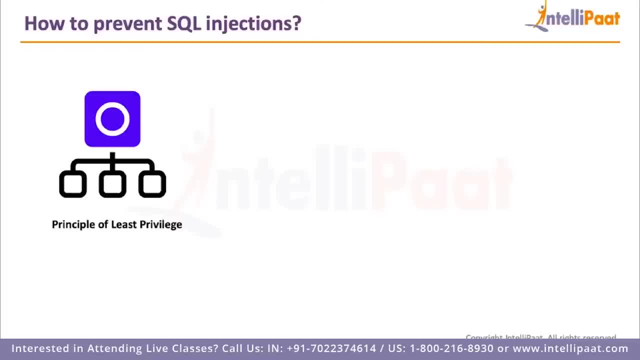 to do. For example, we just saw that if we use this website we are able to list all the usernames and all the passwords you know which are there in the table. So probably that should be a permission which should not be allowed, you know, to the user. 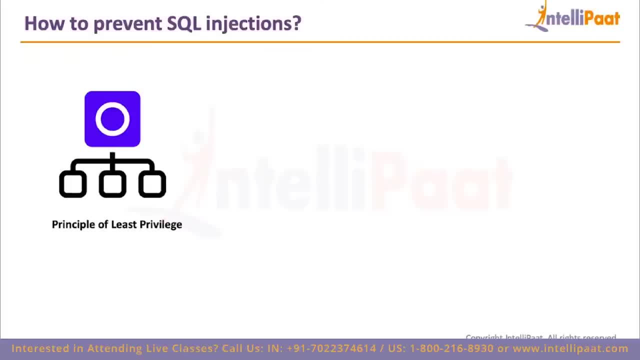 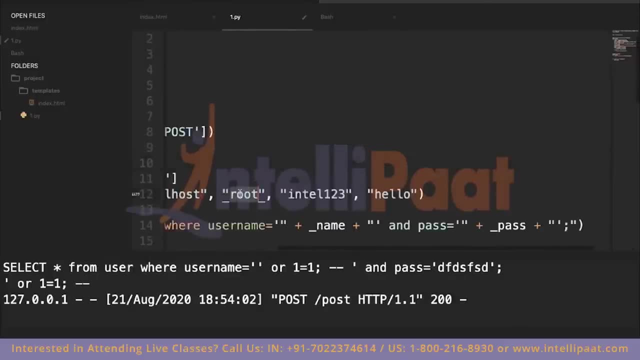 who is going to be, you know, assigned inside your code. For example, if you have a look at the code, the username that we have given over here is root, And that is absolutely wrong. You should never use root, or you should never use an admin user in your code. 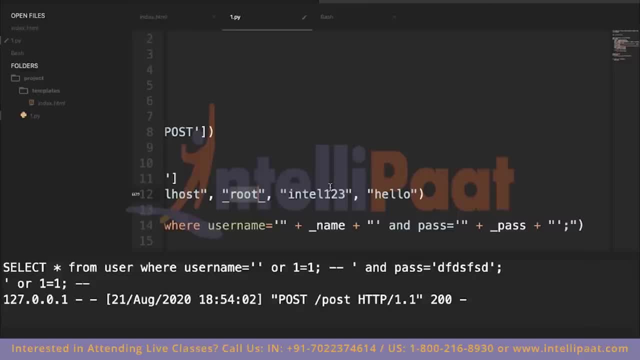 So it's very important to have a username which is going to have the least privileges, the privileges which will only help you to get the work done, and that should be assigned to your code. So that's point number one. Second point is that all the passwords, all the usernames, if they can be hashed in some 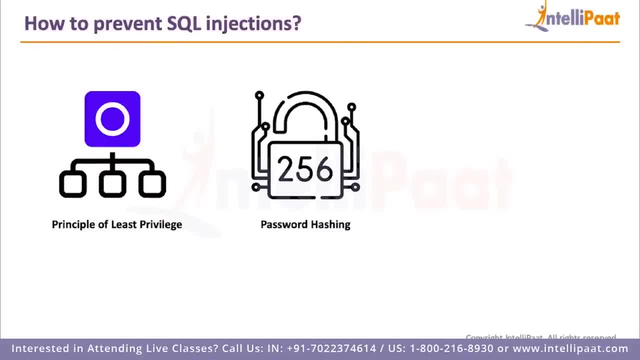 way, then also this attack can be. it can be basically avoided. How So? right now, we relied on the fact that whatever I'm entering, it is not being encrypted somehow, and then it is plainly being passed to SQL. But what if we put in a system in between which can basically encrypt all the data, or 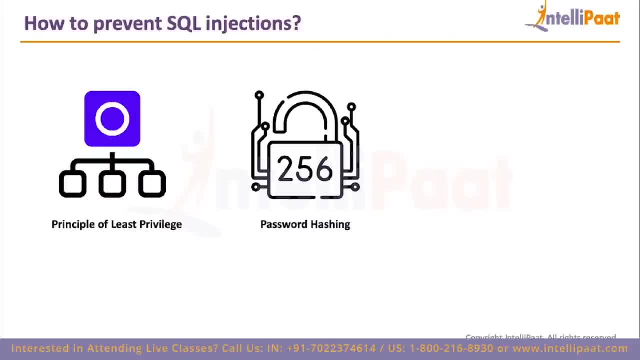 all the user inputs that you're giving and that encryption is basically tested out in. you know your, or it is passed to SQL as an argument. So in that case, what is going to happen is you will not be able to run any SQL query, Right. 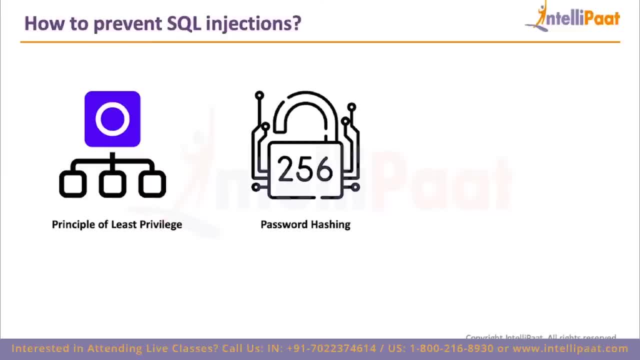 So that is also a possible- you know- preventive measure that you can take. And third thing that you can do is you can always employ third party authentication. So you would have seen that a lot of websites now have options like login with Facebook, login with Google. 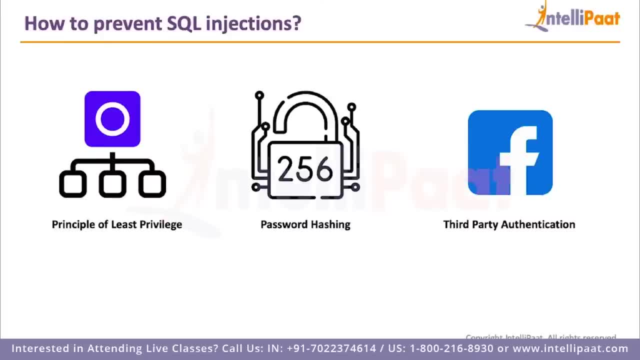 Right. So all these big companies, they have gone through a lot of you know work acts. they have been through a lot of situations. they have a lot of people who are working on the security aspect of their website and you can be rest assured that you, as a company owner or you- 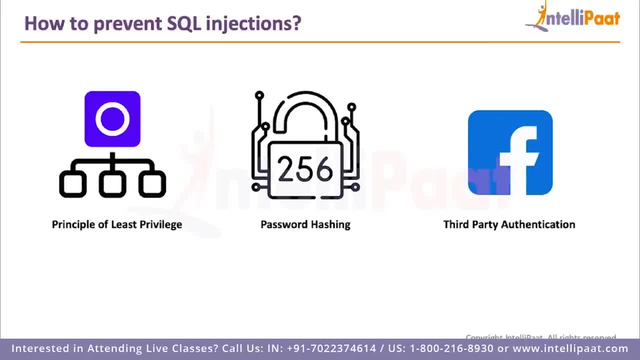 as a manager of a tech team, if you apply your brains and try to create a model which is cannot be spoofed, obviously that is not going to help you out, because the kind of feedback, which feedback which Facebook and Twitter as a company gets because they have, 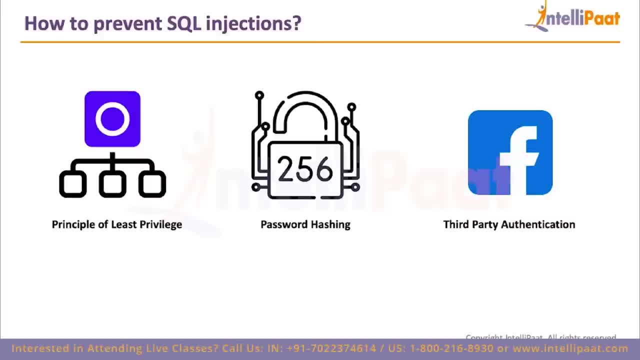 a lot of people like you, right, who probably would be able to, you know, test the application before it goes on to production, test out with different kind of scenarios, Right, And with that fact, their application obviously is more mature, Right? So it's always a good idea if let's say you do not want to go ahead and just make your. 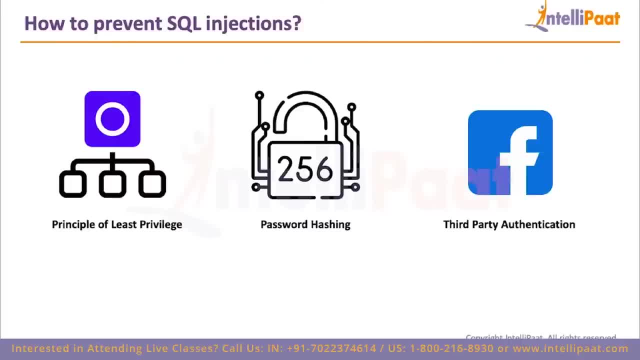 application secure, because otherwise, your thought would be just making your application secure, whereas your stakeholders would want more features in your application, Right? So if you have to balance both of them, why not use things which are already available? And, with that fact, why not use the third party authentication tools which are already available? 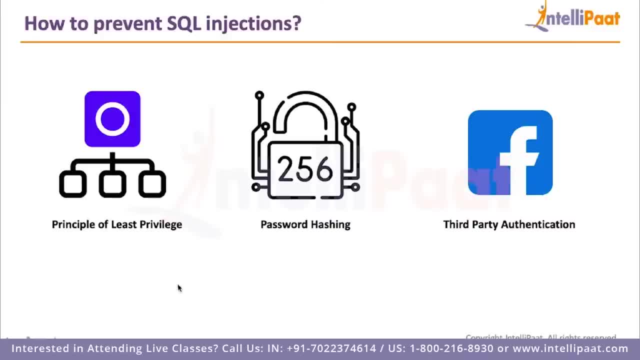 out there, Right? So this would be some of the methods that you can use to prevent SQL loss, To prevent SQL injections, and obviously there are more ways as well, So you can go ahead and practice the best practices of you know- coding, for example- instead. 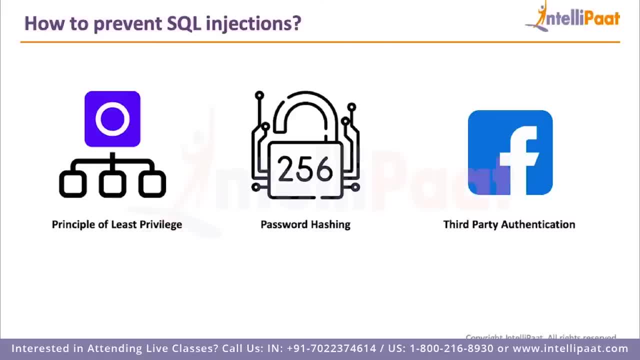 of concatenating the arguments, that, like we just did in the code, you can also pass them as arguments, and that is a topic for a separate discussion altogether. But majorly, if you follow all these three points, they should be enough to prevent a SQL injection. 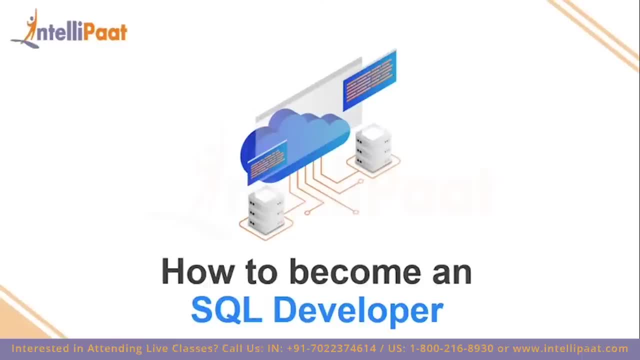 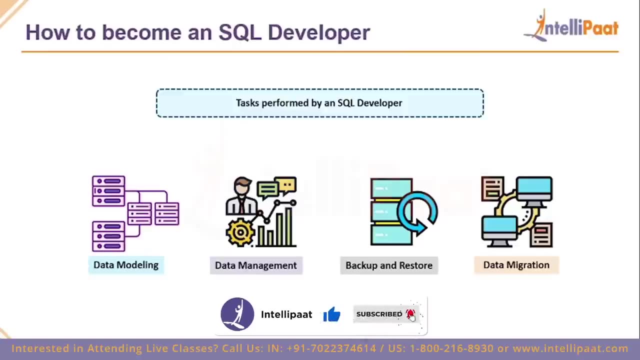 Now, how do you become an SQL developer? There are several tasks that are performed by an SQL developer, And if you wish to become an SQL developer, then you need to be comfortable performing these tasks. So let's take a look at them one by one. 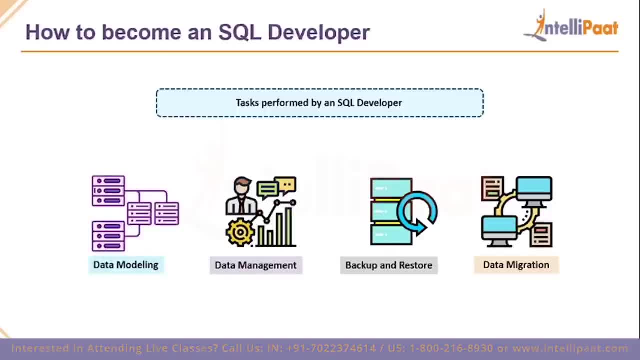 The first is data modeling. Data modeling basically means getting the entire business requirements that you need for a company to store data and then creating relational models with creating tables, creating identifying rules, identifying The columns, identifying the data types that those columns might hold and identifying the 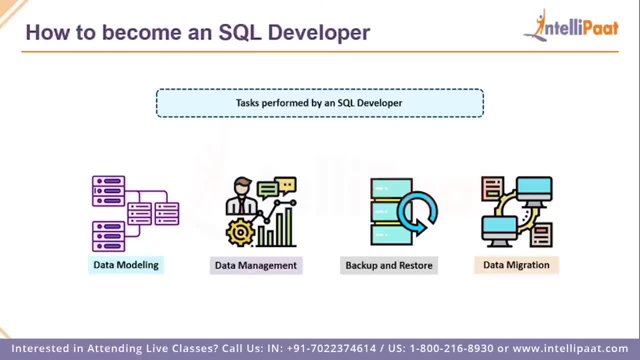 relationships between those tables and the constraints between those tables. Now it might sound very difficult, but don't worry. Stick with me till the end of the presentation and I'll show you how you can learn all of these things. These aren't as hard as they may sound. 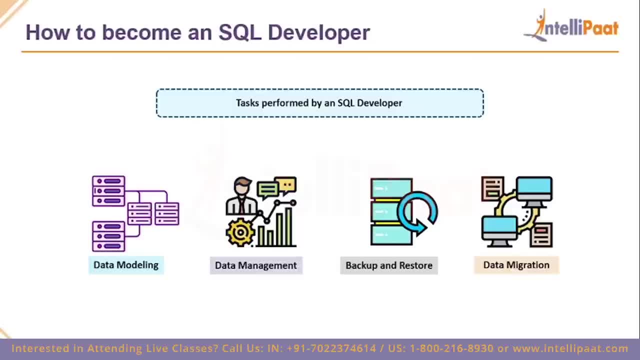 So data modeling is one of the most important tasks that an SQL developer performs. It allows him to transfer the business requirements into the SQL system. Then comes data management. Once the data modeling is done, the SQL developer then needs to get the data that the customer 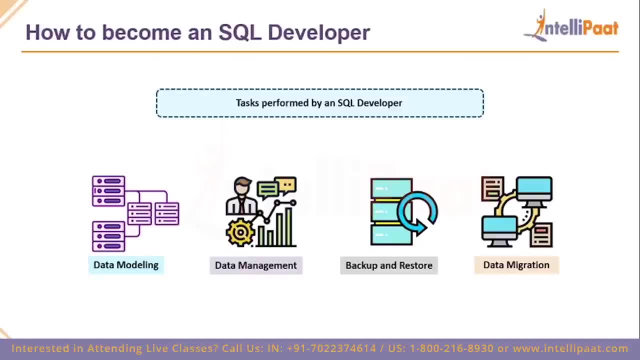 wants to insert, Insert them and keep the databases running in a consistent state and figure out how to keep the entire database in a consistent state. This is one of the tasks that are performed by SQL developer. Then comes backup and restore. This is more of a precautionary measure. 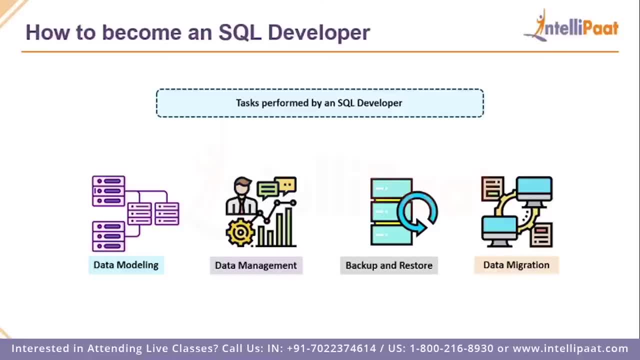 Because data is the most important part of an organization, they need to keep the backups of the databases that they have. Now, this could be decided by the company about how to go about it. It could be that they take hourly backups, could be that they take monthly backups, or 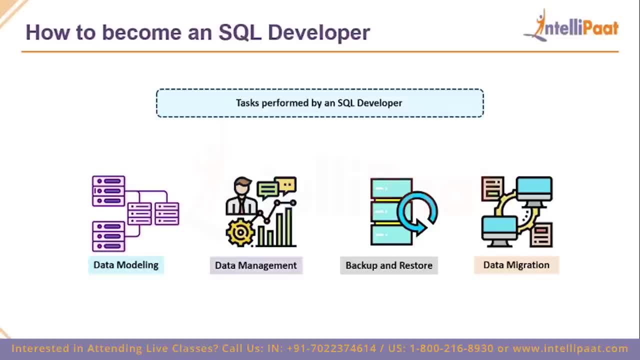 weekly backups. Whatever the company policy is, the SQL developer needs to implement those policies and many attempts they do it by automating these backups And then when the databases go out of network or something bad happens to the databases that we are working on, we can restore it using the latest copy of the backup that we made. 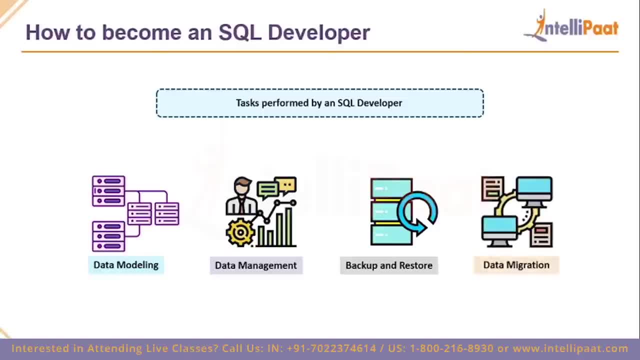 Then comes data migration. It does happen, more often than you might think, that you might need to change the database management system or you might need to migrate the data from one server to another server. This is where data migration comes into play, Supposing you are using a local SQL server and you are storing the data in that. 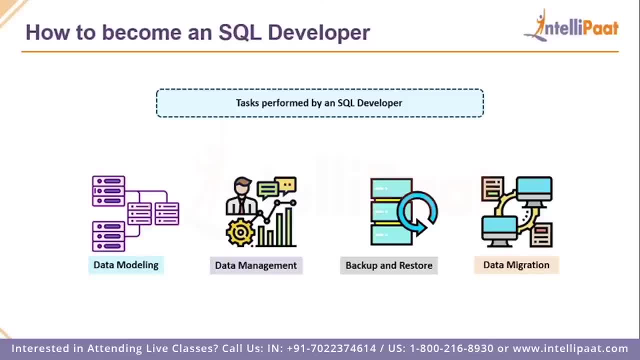 And your company decides that now it's time to move on cloud databases. Now you need to figure out a way to transfer all the data that you have on your local SQL server to the cloud SQL or cloud database, And that's part of data migration, which is one of the tasks performed by an SQL developer. 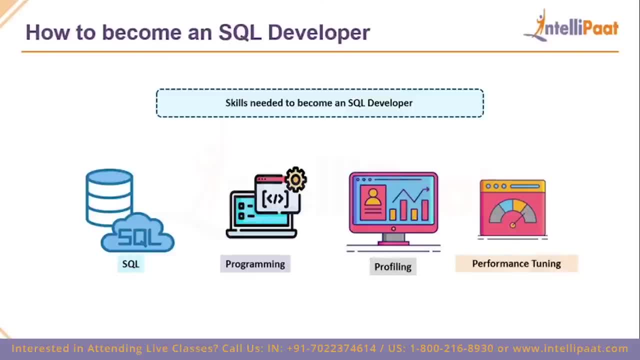 Now let's take a look at the skills that you need to become a SQL developer. You need to know SQL. I mean it's in the name: SQL developer. SQL stands for Structured Query Language. You basically need to know how to interact with the database management systems. how. 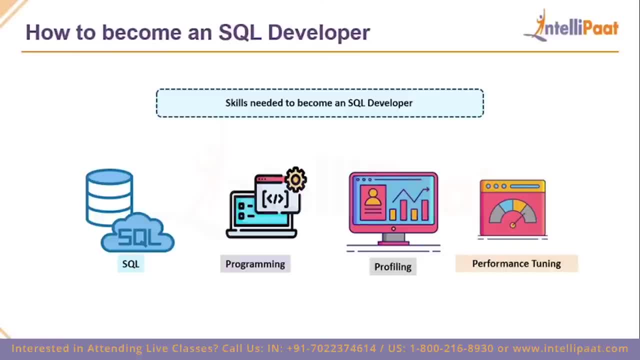 to issue queries and also how to understand how you could write queries that perform the tasks exactly as you need them. Then comes programming. Now you don't have to be an expert in programming, By no means you need to know the entirety of a program. 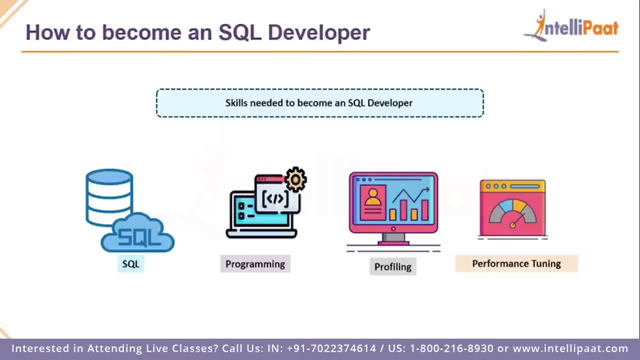 All you need to know is how to use a programming language to interface between your application and your database. So suppose you are building a web application and you are using MySQL and your web application is PHP, Then you need to understand how to connect that PHP application to your database and 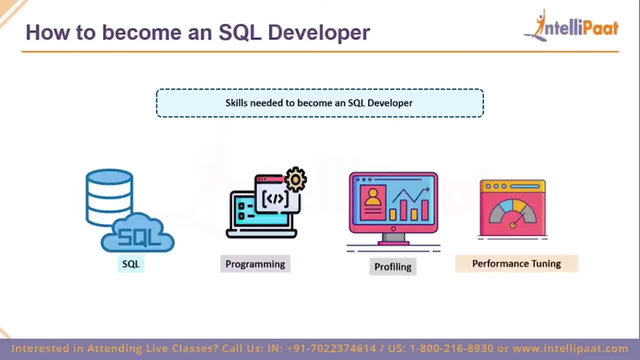 how to issue queries and how to fetch the results and display it to the user. Then comes profiling. Now, this is one of the most important tasks that a SQL developer does. Profiling basically means that once your database becomes of a considerable size, it might start. 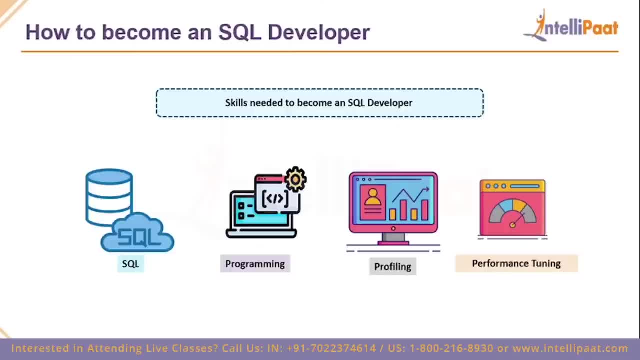 to slow down, It might perform poorly, And now your task becomes to profile it, which is to say to understand what parts of the database are causing this performance lag. You need to then take a look at the entire databases, issue some queries, profile them. 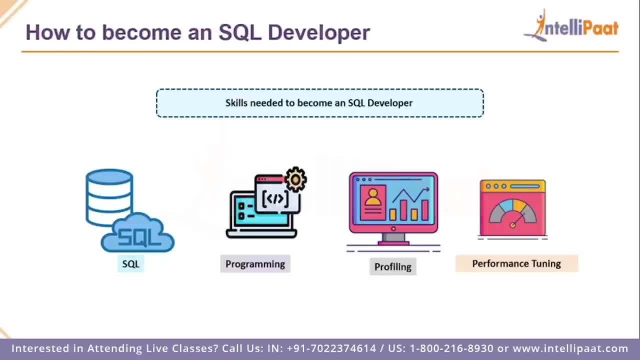 and figure out what are the performance bottlenecks and try and figure out how you can remove those bottlenecks and how you can improve the performance. Which brings us to the final point, which is performance tuning. As the name suggests, performance tuning is used to increase the performance of our database. 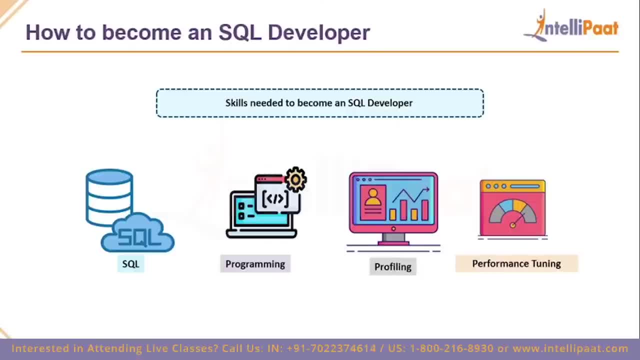 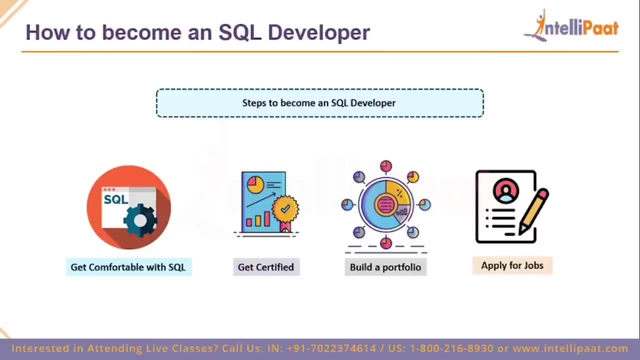 management systems. There are several ways to do it, and you need to understand what are the pros and cons of all those ways and then implement the one that fits best for your need. And now these are the steps to become an SQL developer. So the first thing that you need to understand is you need to be extremely comfortable with 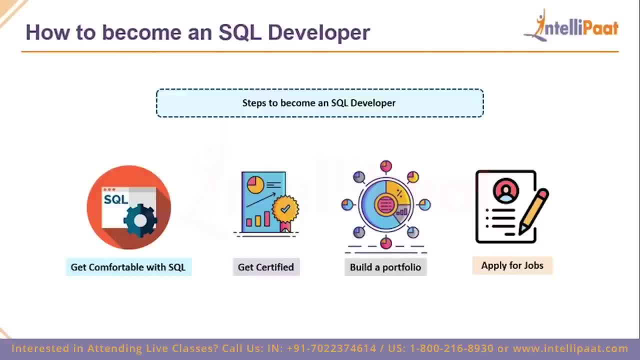 SQL. You need to understand how you can issue queries, how you can write SQL statements that translate a business requirement into an entire data query. This should allow you to write queries and get the data back from the database In the desired format and display it to the user or send it back to the client or the 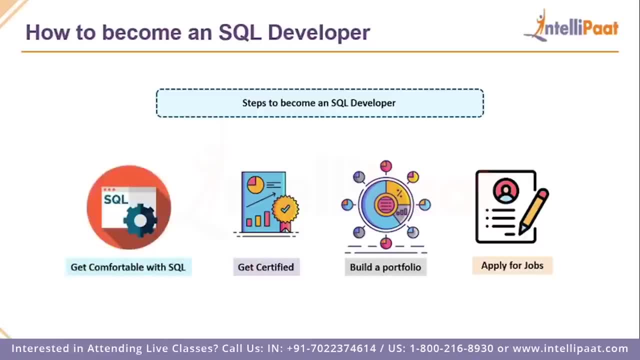 application. that's using the database. Then comes getting certified. Now, in today's day and age, certification is one of the most important things that allows recruiters to separate you from the crowd of all the resumes that they get For a given job. many people will be applying. 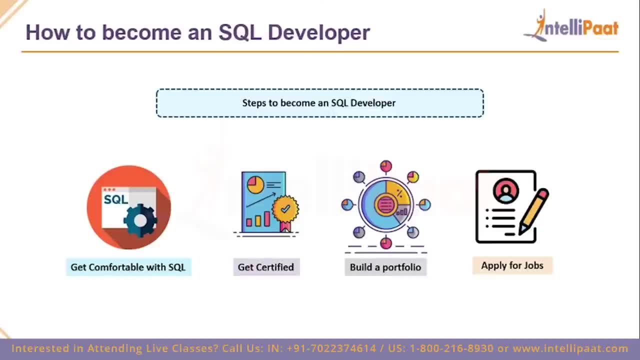 And if you are certified you definitely have an edge over the other uncertainties. So definitely keep in mind: getting certified does bring you ahead. Then build a portfolio. This sort of ties in with getting the certification. Building a portfolio basically means that you need to build things with the knowledge. 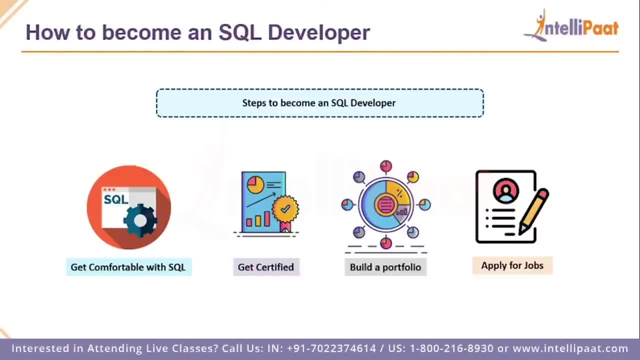 that you acquired while you are getting certified. Now, this sometimes as so happens, that you are asked to build projects when you are getting certified. So even after you do get certified, It's more than important to work with the skills that you have and try and build things. 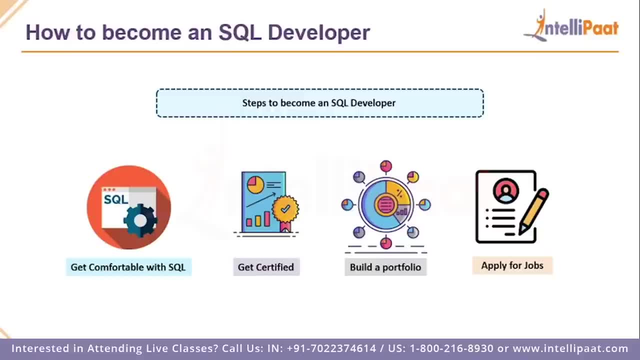 that could attract some of the recruiters. They look at your portfolio and they'll understand that you like doing these kinds of things and you might even get job offers because of those, And then finally, after building a reasonable portfolio, apply for the jobs, Start looking for jobs and apply for them, and you have a really good chance of getting. 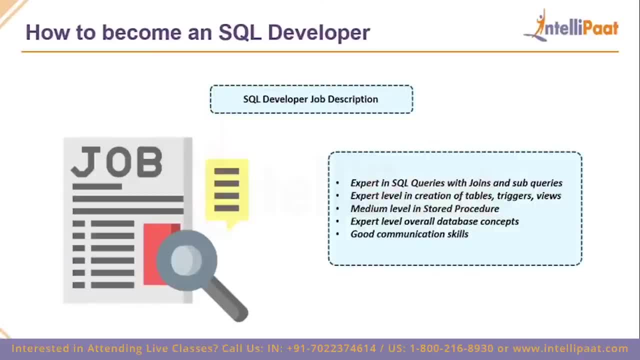 the jobs if you perform these tasks. To give you an example, Here's a job description, A job description of an SQL developer. So they need you to be an expert with the SQL queries. You need to understand how to do joins and subqueries. 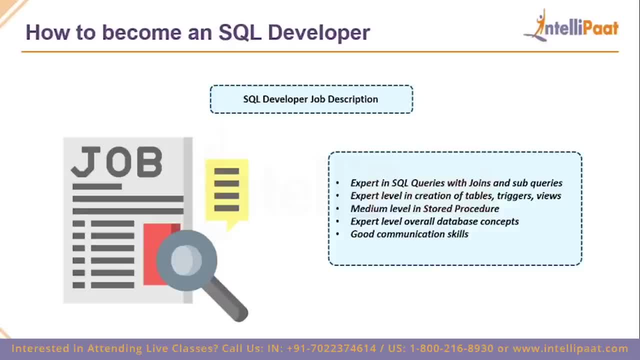 We'll take a look at them in the demo. You also need to be an expert in creating tables, triggers, views. Don't worry if you don't understand them. As I said, stick with me till the end of the slide and I'll show you how you can go about. 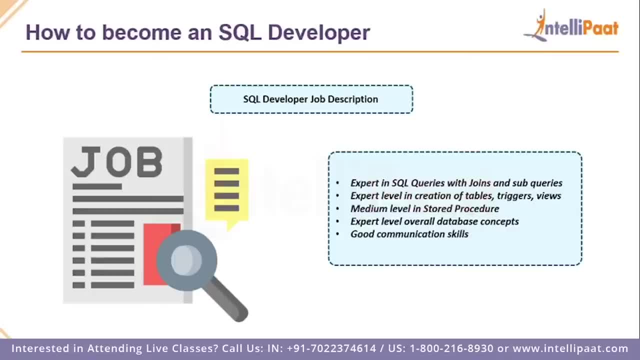 learning these things and getting a job as an SQL developer, You do need some medium level stored procedures. Think of stored procedures as basically functions that you can run by issuing just one command and they'll do an entire list of things for you. You also need to have a good grasp of the concepts of databases. 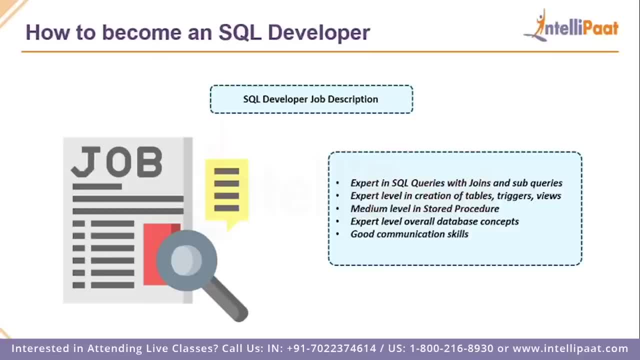 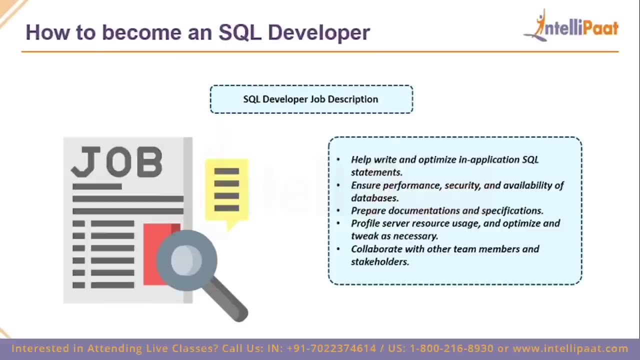 There are several fundamental theoretical concepts about database management systems that you need to understand in order to be very efficient with your database skills. Finally, good communication skills. Here's another job description And it's quite similar to the previous one, But you do need to understand that several companies might have different requirements. 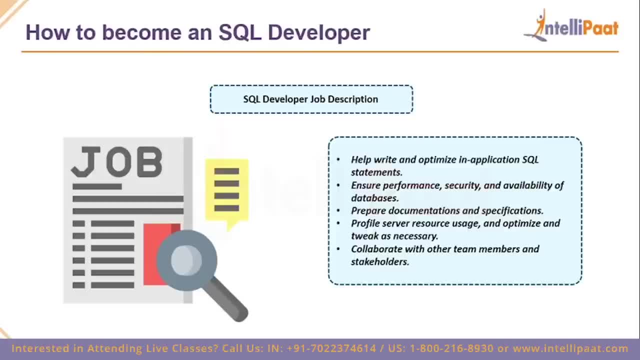 from their SQL developers, For instance, here, they want you to optimize in-application SQL statements. So this is where the programming part of your learning journey comes in. You need to ensure performance, security and availability of databases. You need to prepare documentations and specifications that tell the user of the database how the 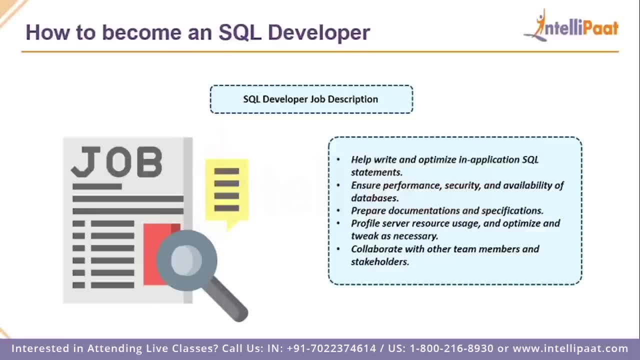 tables are structured and how you can go about doing them. Then there's profiling the server and resource users, and optimizing and tweaking as necessary. This is where it comes to optimizing the servers to perform better than they are And finally, collaborate with other team members and stakeholders. 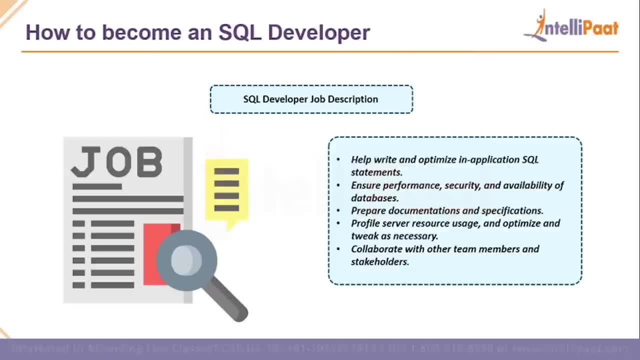 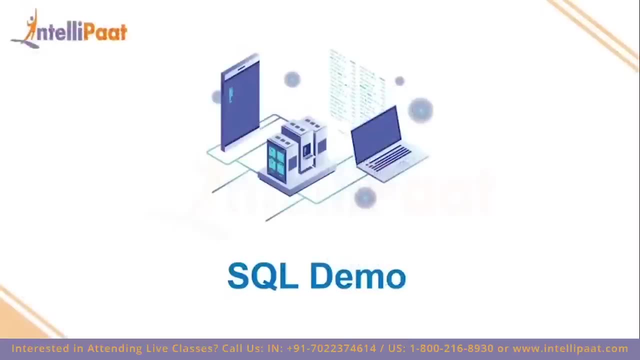 This is where you collaborate with other people, Try and figure out the value that the system should be bringing out, and then use the knowledge that you acquired in that collaboration and use your SQL skills to build databases and work with the team. And now, finally, we'll take a look at a demo. 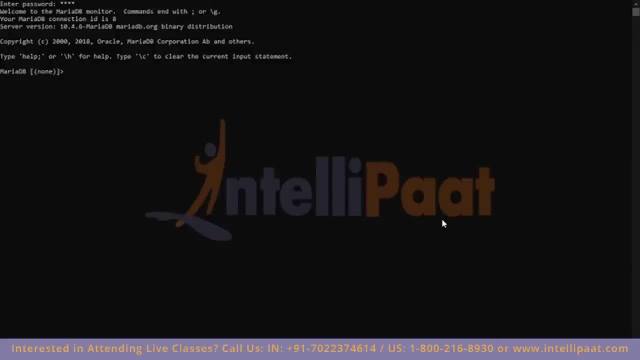 So I'm using MariaDB. You can use any database system that you want to use, If you can. you can use MySQL as well, or any other database system that you want. Everything is fine. So we'll be in this demo. I'll try and keep things simple so that everything doesn't go over your head, and I'll try and 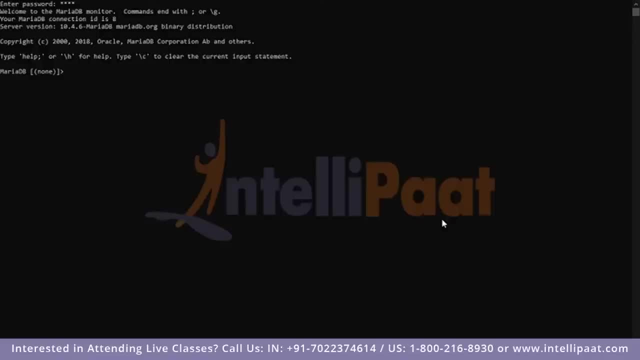 understand, Make you understand what I'm trying to do. So in this demo we'll be creating a database for a small car inventory database. So for a car inventory application, we'll be building a small database that will have two tables. Each table- first table- will contain the make of the car, such as Toyota, Hyundai or whatever. 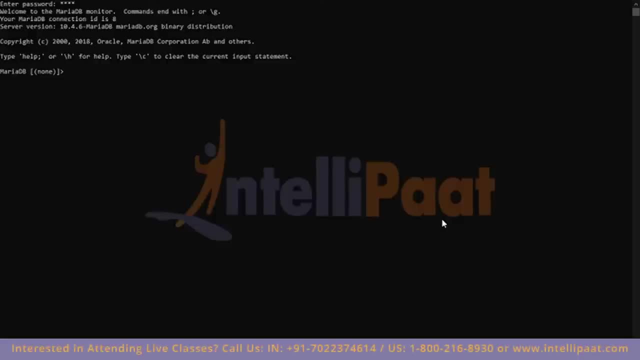 And the second table would contain the model information about the car: the name of the model, the make ID or the year And the price, and so on. So let's start. whenever you're working with a database management system, the first thing you need to see is: what are the databases that are already created? 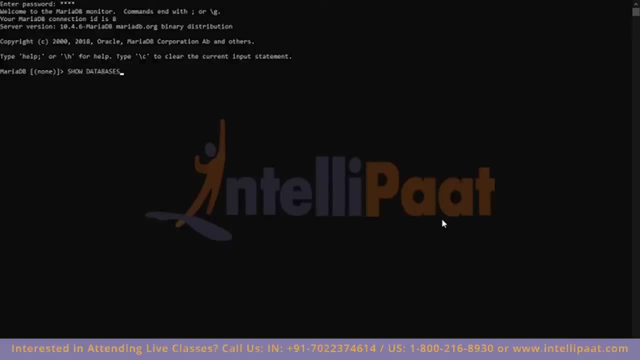 So the command showed databases. It's basis with an S. So, as you can see, by default our database management systems comes with four databases. These are used by the database management system internally, so you don't have to fiddle around with those databases. 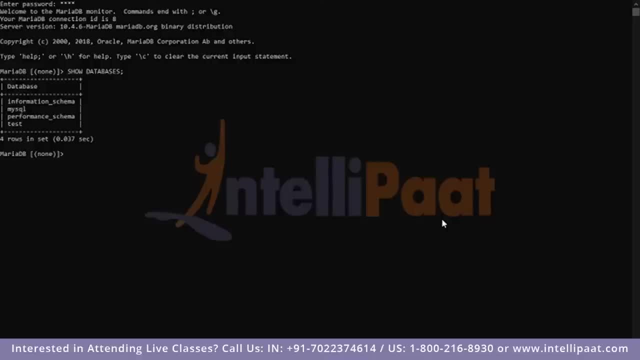 databases. now you can pick the name of your database that you want. make sure that it's not already existing in the existing databases. so just type the name. so to create a database, just type create database and, as you can see, i'm typing the queries in uppercase letters. 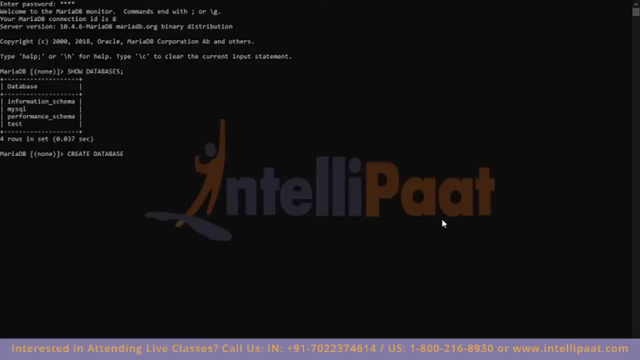 i'll show you why i'm doing that in a moment. and the name of the database would be car inventory. now you can name it anything you want, just make sure that you remember what you named it and end the sql statement with echo semicolon. press enter and our query ran. 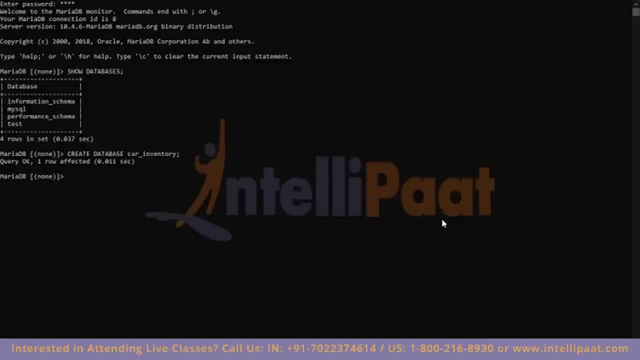 okay it. one robot was affected, which means our database is created perfectly. now, if we run the show databases command again, as you can see, we have a car inventory. we just run use car inventory. now, whatever commands we need to do is we need to create a table named make which will store the make of the car. now. 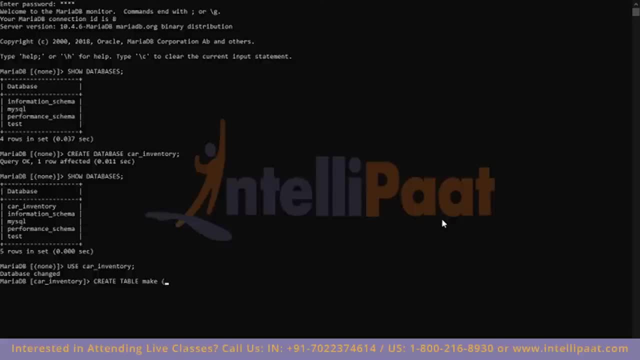 as you can see, i am typing the create and table words in the keywords in the sql statement as capitalized, and make is in small letter. this is mostly preferential, but i like to do this to separate the things that i can rename and separate the things that are the. 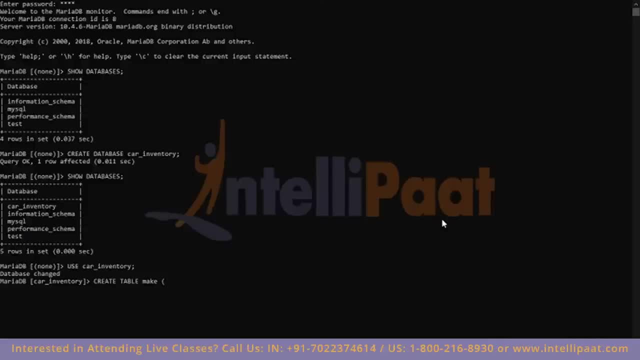 keywords. so i can't type any other keyword than create to create a table. but i can rename the table from make to make, car or car make or whatever. this is something that i can choose, so to differentiate between those, i like to do it this way: you can choose whatever syntax. 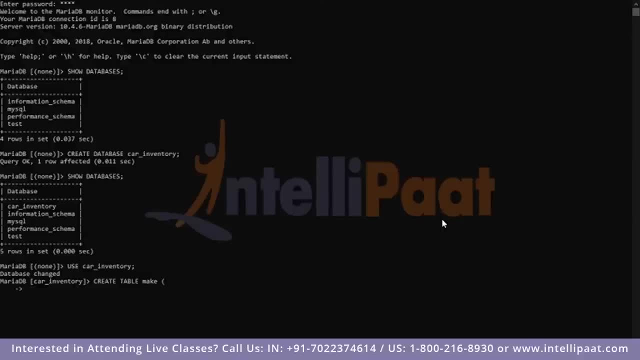 you like. now open the brace, press enter, and now we will begin defining the model of our database. so the first thing we need is an id. think of an id as a primary key. so if you have been a student, you know that you are assigned role numbers. those role numbers are: 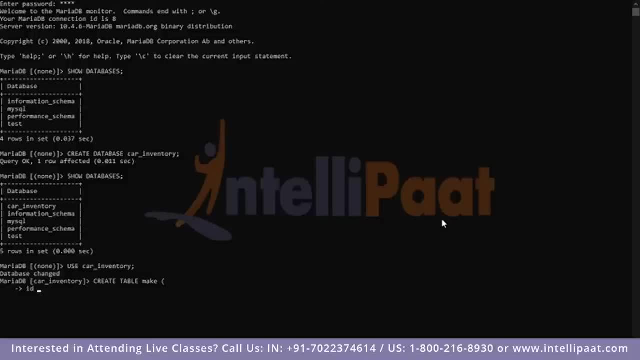 used to uniquely identify you, so even if another student in your class has the exact same name as you, you can still be differentiated using the rule number. this is what the id is for in any database or relational database table. it would be an integer. we do not want it to. 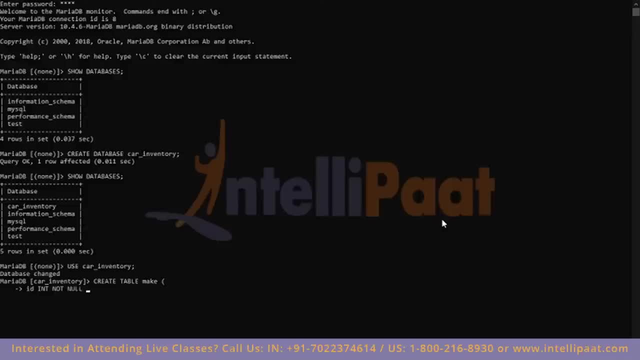 be null. null means absence of value. we do not want anyone, as we do not want any student, to not have a roll number. and finally, we want it to auto increment, which means, as we are entering the rows into our database tables, these ids are auto generated and they are automatically assigned in an increasing order from one. okay, now we need the. 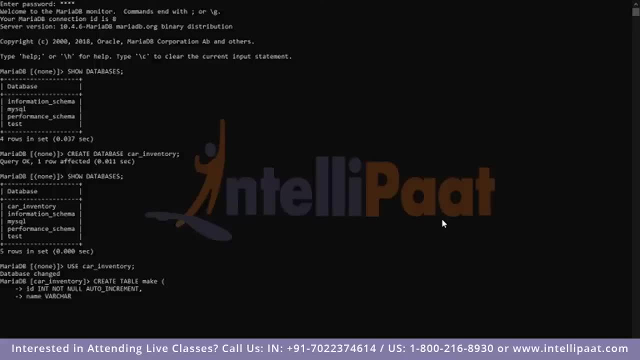 name of the make of the car. i'm going to store it as a variable character of length 30 and, finally, i will define the primary key to be id. don't worry if this syntax doesn't make sense. i'm just trying to get you to understand how to issue these queries and i'll guide you. 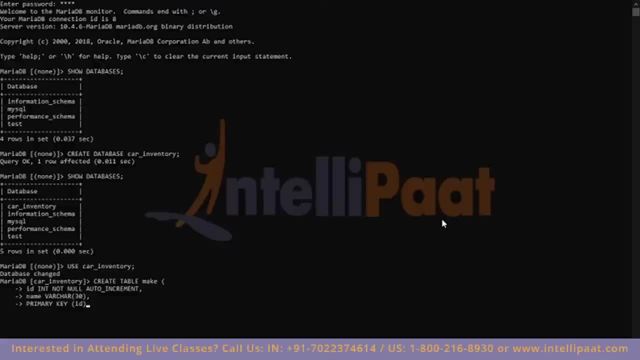 to the resources that you need to learn these syntaxes. finally, let's close our syntax. press enter and, as you can see, it worked fine. if it would have thrown some error, that would have been a problem. if it has not, let's move ahead. now we will create the table model, which is the. 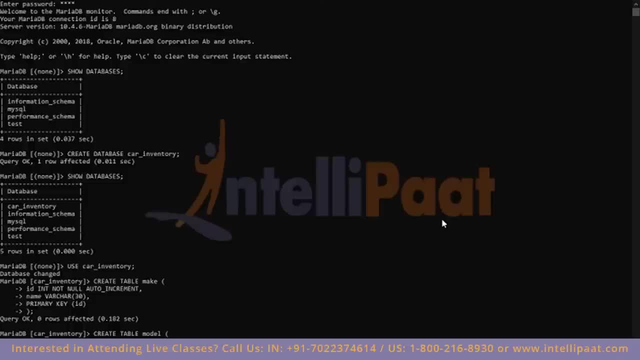 last table that we need to create for this demo. now again, i'll be assigning an id, which would be the similar thing. it would be integer, not null, and auto increment, press comma. and now we need to define the things that we need to store in this model table. the name of the model would be a variable character, variable character basically. 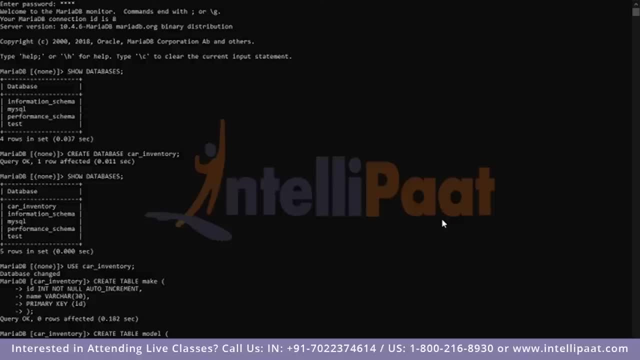 means it could be somewhere around 30 characters: the name of the car, name of the name of the model of the car, and we do not want it to be null, so it's not. then comes price, now price. i can store it, although you do need to spend more time with the customers and your business stakeholders. 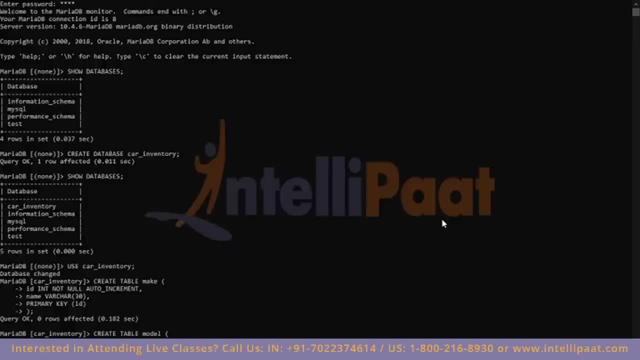 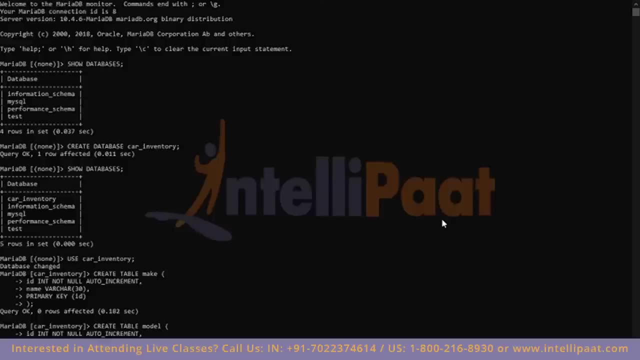 to understand whether you want to store it as null or a precision value like float or double. and then comes here: now you can store er as integer as well. i'll be storing it as variable character because i will not be performing any mathematical operations on it and variable characters allow you to use less memory. 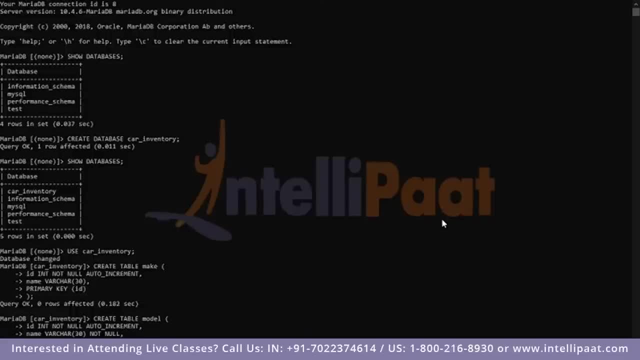 we do it not null, because we do not want to use it as a variable character. here we create our variable character and we, omdat the number character is equal to the Extreme And the ley is equal to less realization values, want it to be empty at any case, which is why it maintains the integrity of our data. and finally, 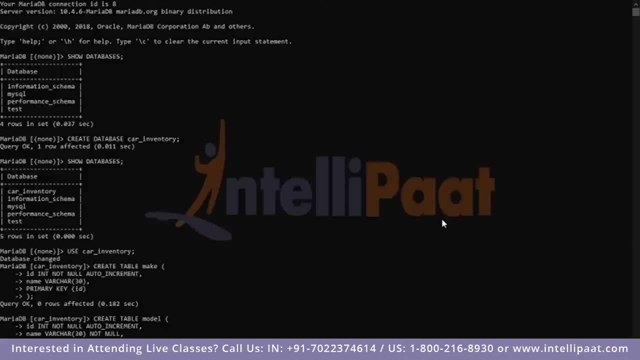 this is the foreign key. this make id will contain the information about the make of the car, which will be stored in the make table. i'll show you what that means in just a minute. it has to be int and it has to be not null. now, one thing to note is that this make id would have same properties as 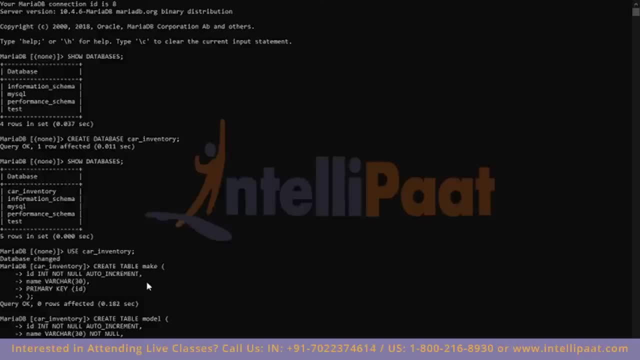 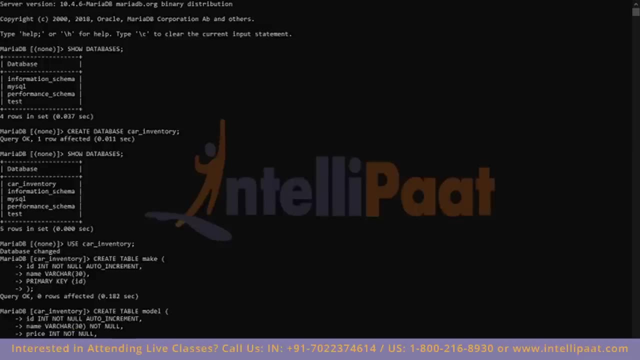 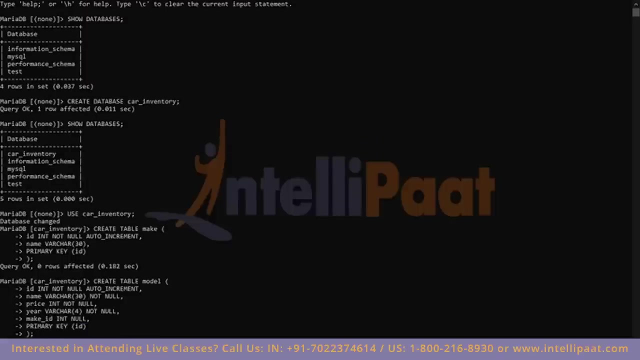 the id of the make table. you don't need to add the auto increments, just the integer. and it's not null. and finally, we will define the primary key. the primary key of the table would be the id, not the make id, the id of the table. and finally, and it's done now, the last part of the table is: 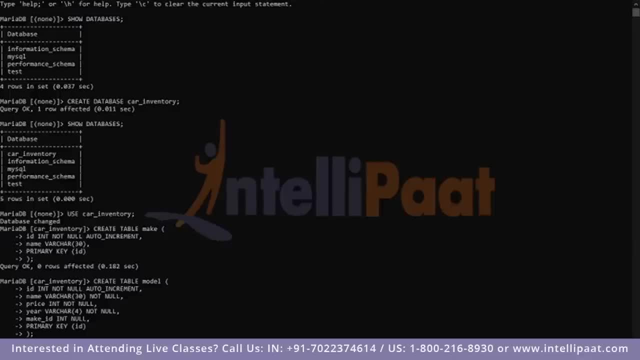 that we'll be adding a constraint. the constraint basically allows us to enforce some data integrity rules. so in this, what we're doing is we are adding a constraint by altering the table named model. we are adding the constraint and we are naming it car model. make fk. fk stands for foreign key, so we will be adding a foreign. 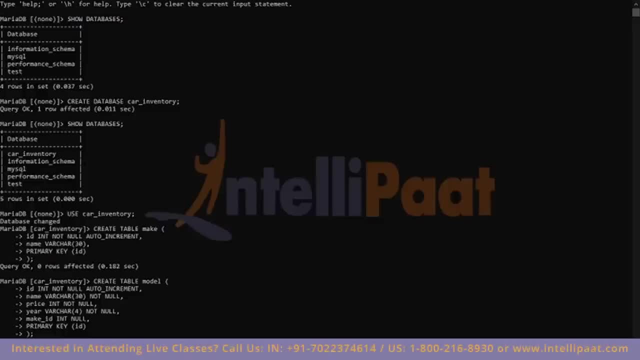 key on the make id of the table. make id, as you remember, is the that we created when we are creating the model table, and this will be referencing the make tables id column, and the final thing that we want to add is we want it to cascade on delete. i will show all of what all of this means in just a moment. 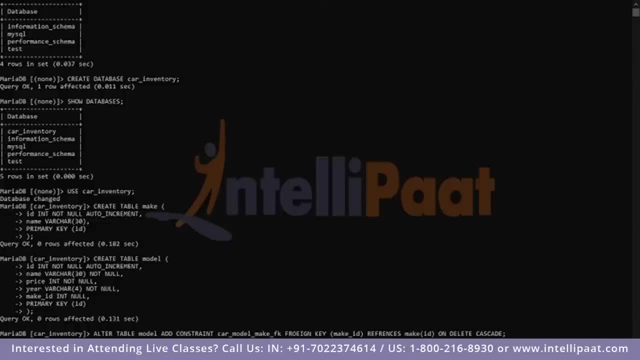 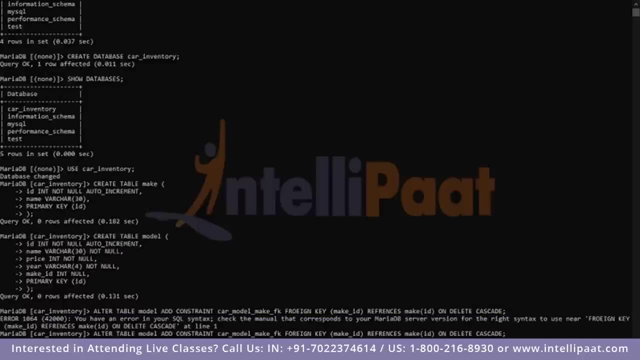 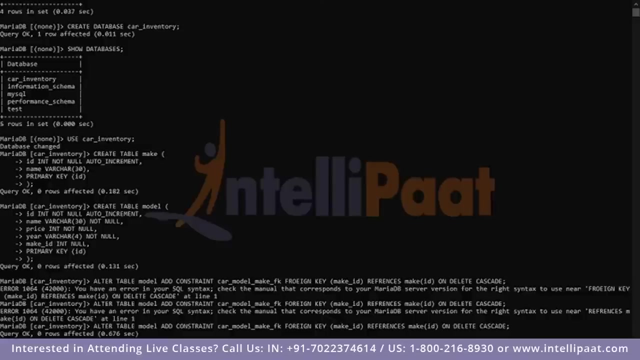 okay, i think that's in. oh, i misspelled the word foreign here. okay, and another thing that i it's been references, i think. yeah, as you can see, typing long queries could lead to issues. as you can see, it's done and our foreign key constraint are in place, so what this means basically is that inside 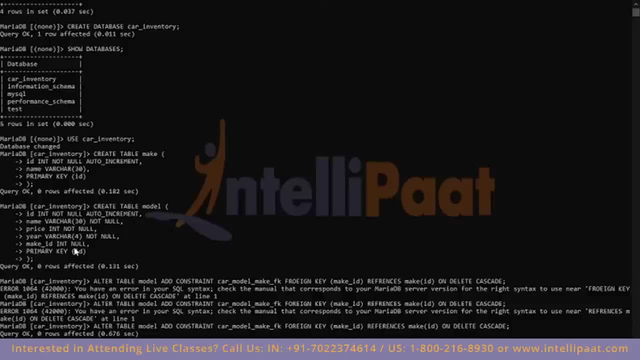 our model table, the make id will only contain the information that already exists in the make table. for instance, if i enter a car and i want to add its make, i cannot add the id four or five or whatever i want, arbitrarily. this would lead to data integrity violation, which we 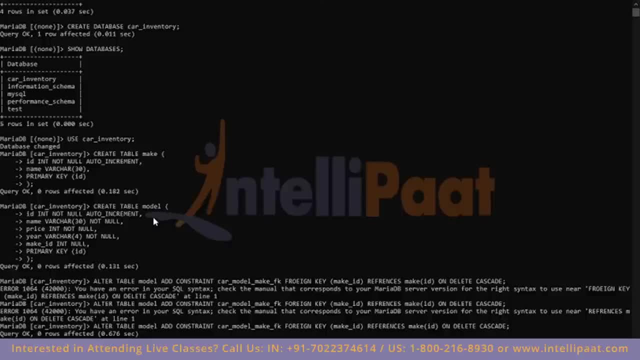 have prevented by by adding a foreign key constraint. and what all of these means i'll show you in a minute. let's start and insert into the make table in now. we will be inserting into make and the thing that we want to insert is the name. the id will be auto generated and auto. 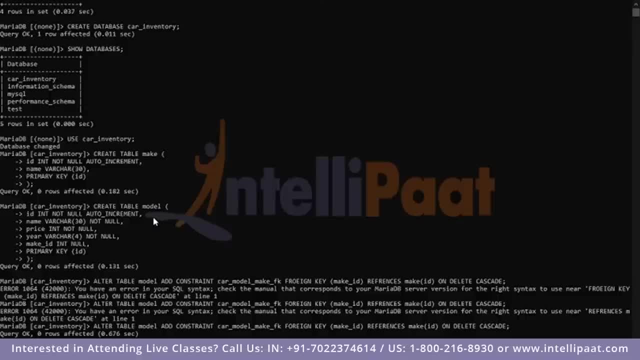 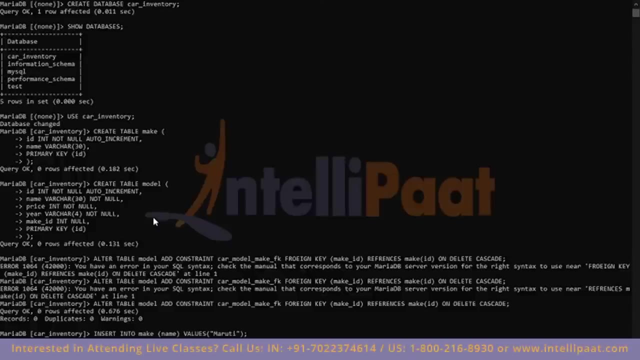 incremented, so we do not need to worry about it. and the values that i want to insert is, since it's a variable character, i need to store it as a string and i will store it as mark. so it's inserted, let's store. let's store toyota. 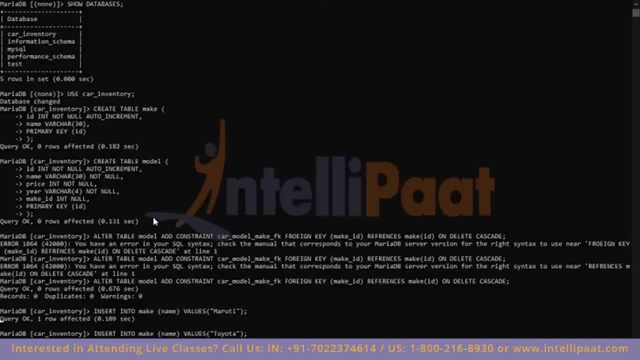 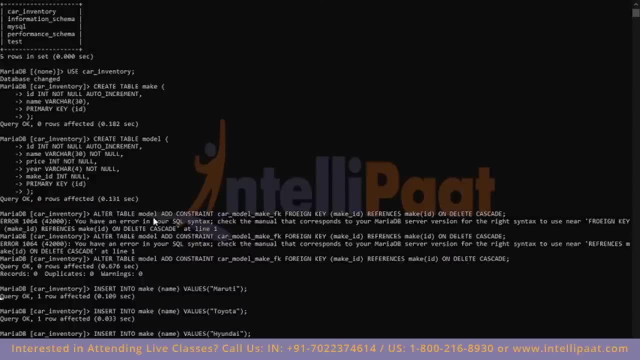 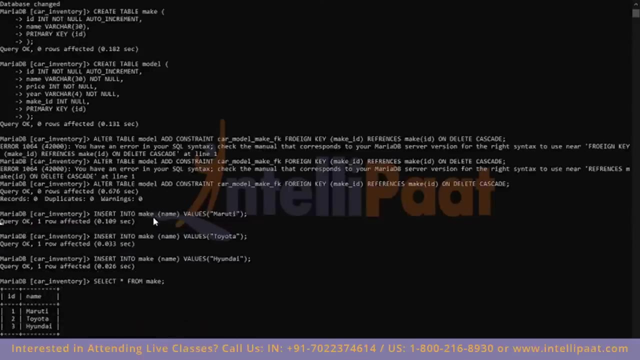 toyota. finally, let's store yu and hyundai. now that these three things are inserted, let's see select star from make. so we have three names for the makes of the card that we'll be storing and the ids are, as you can see, automatically generated and incremented. 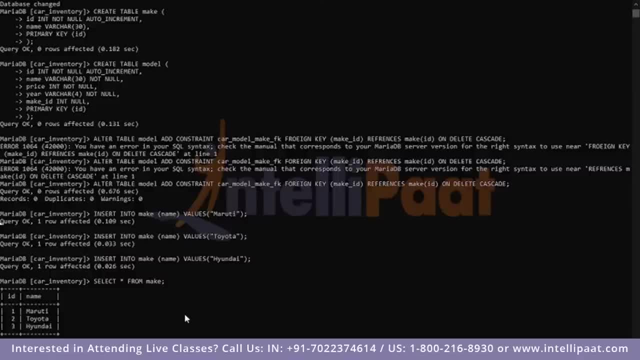 now what we need to do. we need to insert into the model. inside the model, we will insert the name of the model, the price of the model, year of the model and, finally, the make id. now, this is where our integrity constraints come into play. i'll show you what i mean in just a second. as you can see, there are only one, two and three ids. 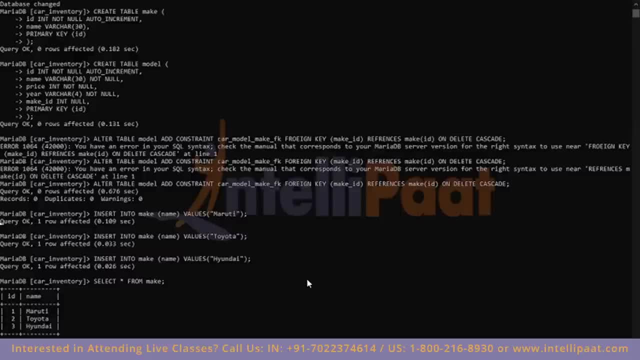 so if i try to add a car with id 4, it will. it should show me an error. let's see whether it does or not. so i'll be adding hyundai i10. so i'll be adding hyundai i10. so i'll be adding hyundai i10. 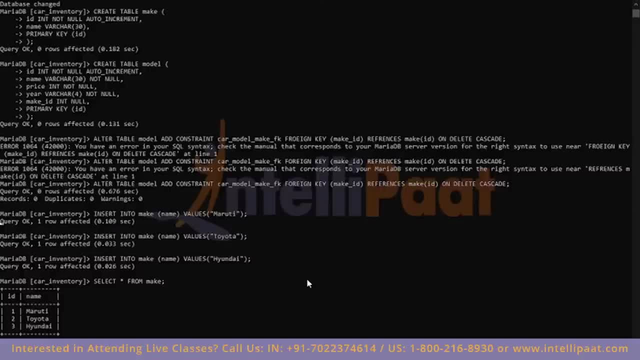 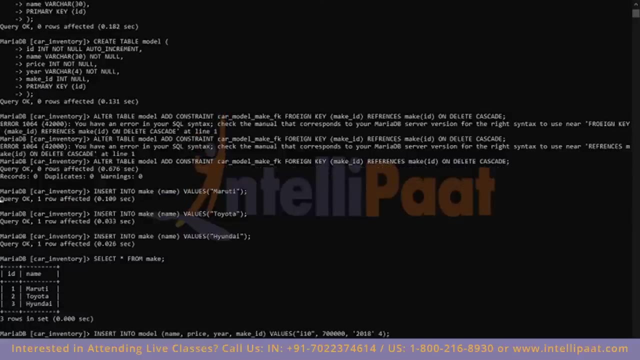 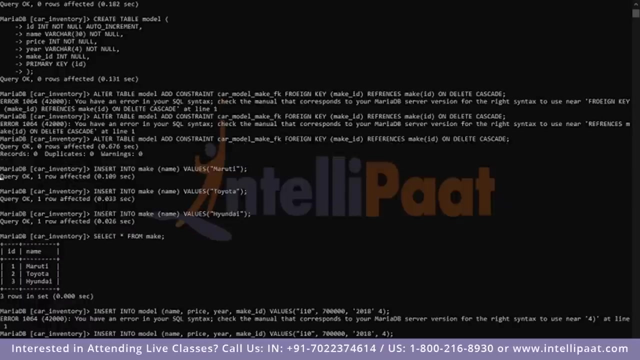 let's price it arbitrarily okay, and let's say the year is 2018. now finally comes time for the make id, so i enter 4 and, as you can see that we cannot insert using- oh sorry, there's a yeah, yeah, so the foreign key constraint fails and it disallows me from inserting invalid data now. 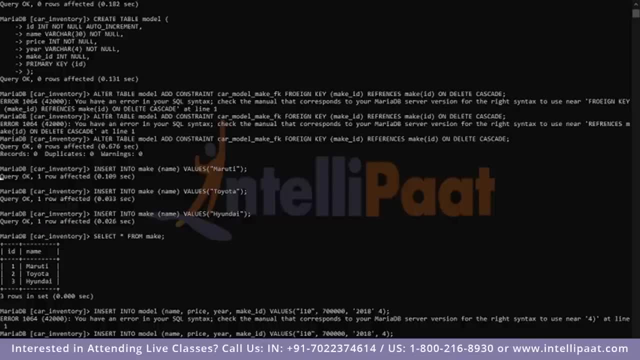 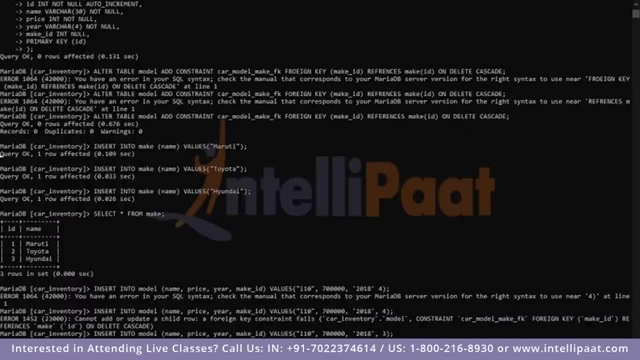 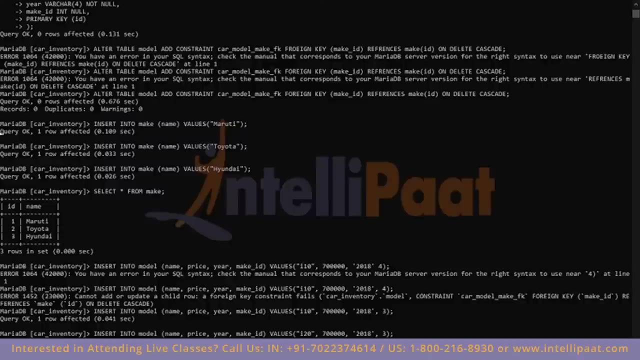 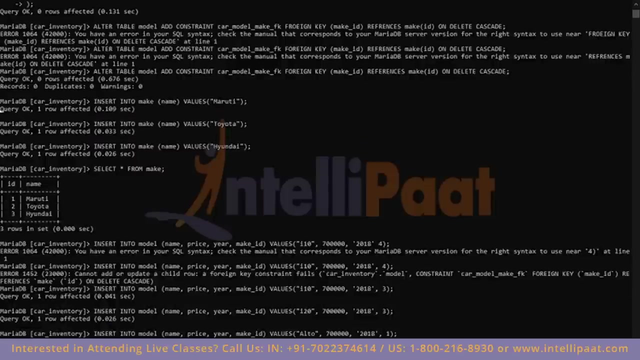 if i want to insert, insert the hyundai i10, i just need to make the make ids 3 and it does work. now let's store some other values so that we can run further queries. let's store i20. finally, let's store although- and let's do it this way so it works. let's see: select star from model. 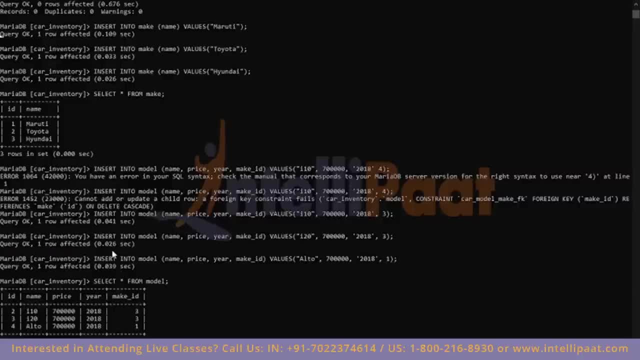 and we have inserted everything and we have disallowed from inserting an invalid data. as you can see, invalid data was disallowed. we got an error, so it works perfectly fine. now we will be looking at some advanced query. we'll be using something called a join, so suppose that i want to write a query that will show me the name of the model, the make of the model. 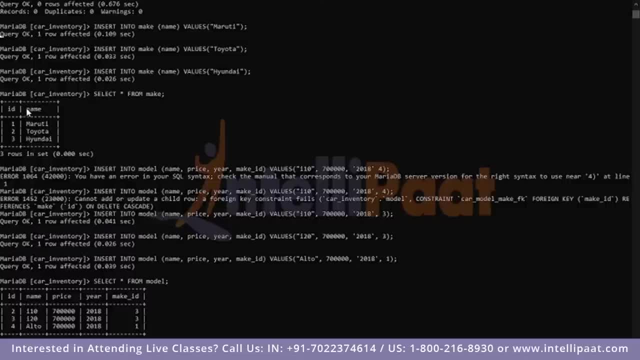 and the price of the car. so i want the make name, the model name and the price. i want maruti- uh sorry, hyundai i10 and price 7 lakh or whatever it is. so since these are stored in two tables for maintaining the integrity, we need to perform a slightly more advanced query. this is called a join query. 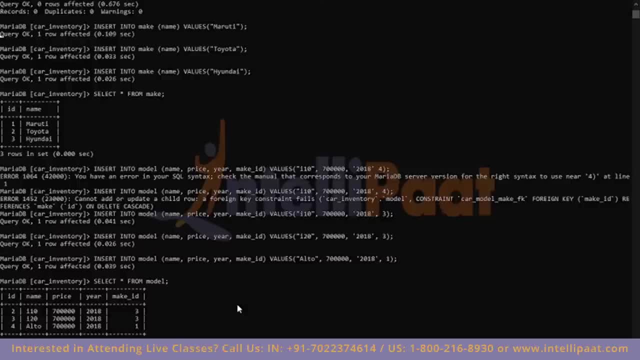 so let's do that. so i will show you how to do it. using the select keyword, i will be using the make tables name and i will be showing it as make underscore name. i'll show you what that does in just a moment. now that that's done, i will be doing the showing the model name and model dot. 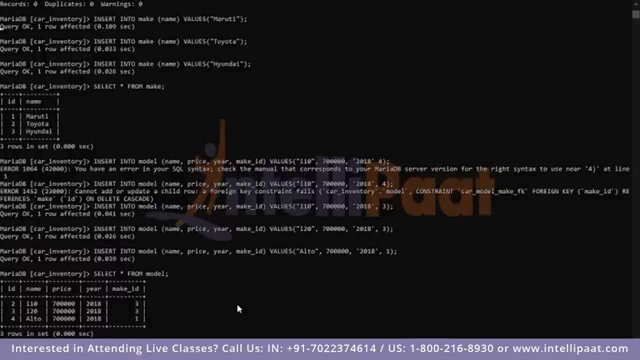 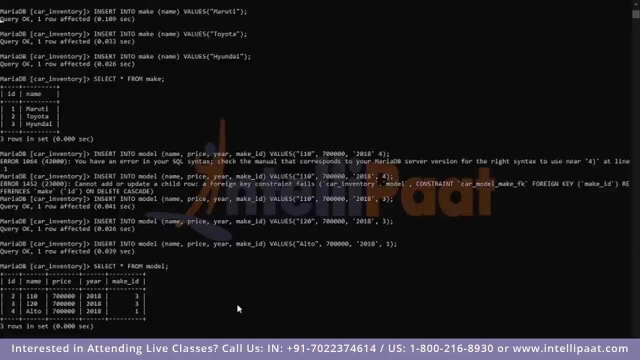 price. now that we have defined what we want to display, let's tell which table we're going to use. so i will be using the model table, press enter and now we will tell the sql database management system which is the table column that we want to join on. so to join on, we'll be using the foreign. 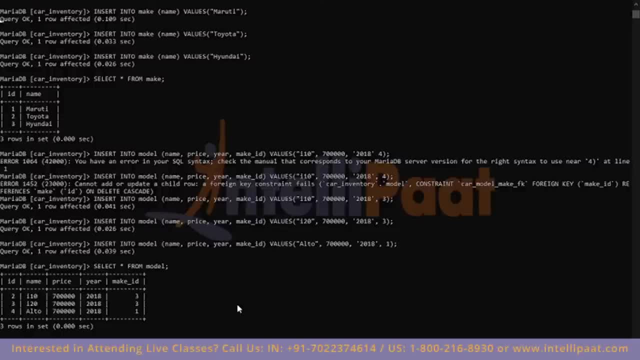 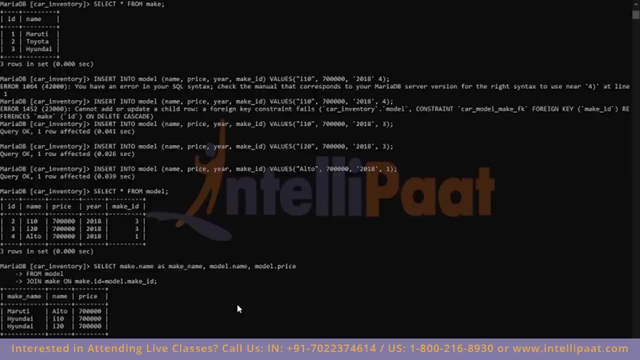 key constraint. basically, we tell it: okay, join on the table named make and on the column id on the make and make sure that it equals the model tables make id. and here we go. so we have maluti, alto, 7 lakh. hyundai i10, hyundai i20, so we have the 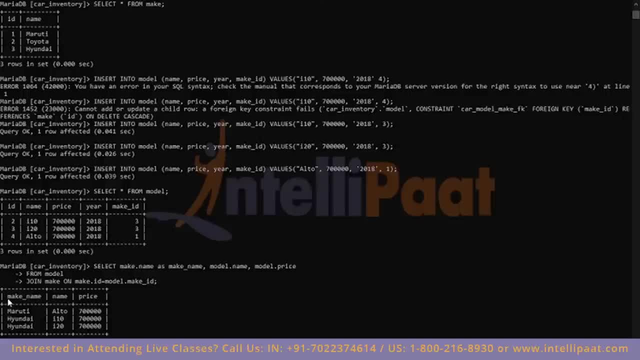 data that we want to use and we have it stored in different tables and just one query allowed us to write it entirely. this make dot name is make underscore name. i wrote it because the name attribute might have conflicted and having two names in the same attribute could be a little. 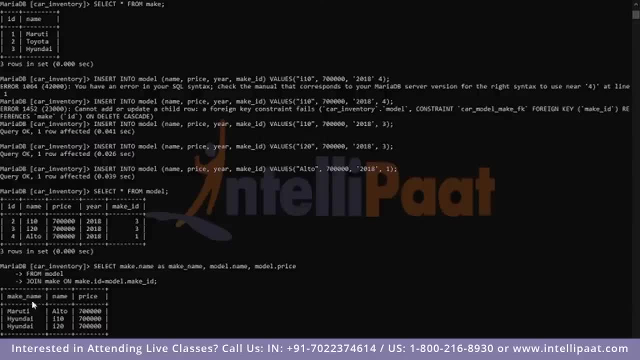 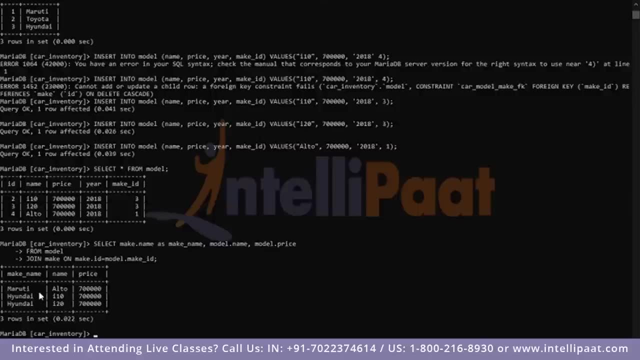 ambiguous to understand which we are talking about. so that's why i named the column. name is make underscore name and we can do it on the fly. so it's not actually done in the table, it's done right here now if you want to look at what are the constraints that you have laid on. 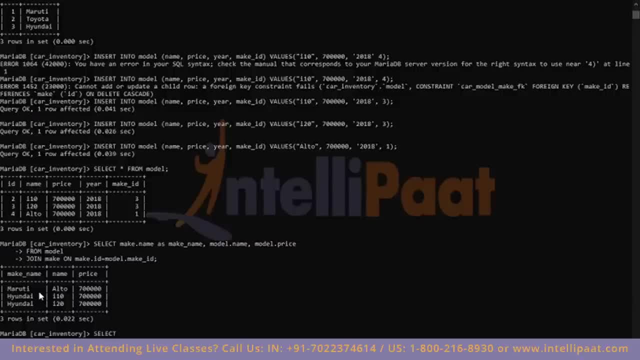 the table. basically write this command. we will see what are the constraints that are on our make table, so we will be selecting the column name and the constraints. constraint name from information underscore schema. this is a table that has been already created or this is the database that was already created and used by our database management system. it's called information. 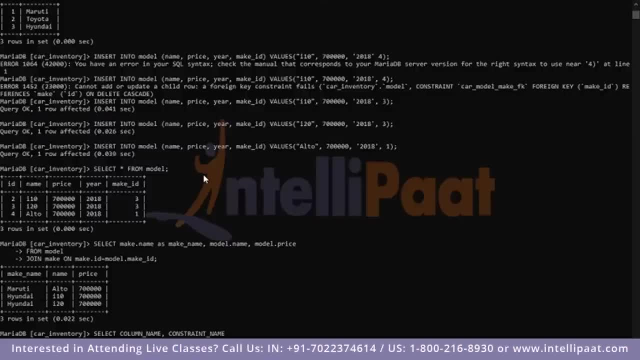 schema and we will be using the key column usage table these. this is maintained by the database management system, so we do not have to do anything. and finally, we tell it the name of the table that we want the data for. so we go where table name. let me write it: table name equals to: and the name of the table that we are using. 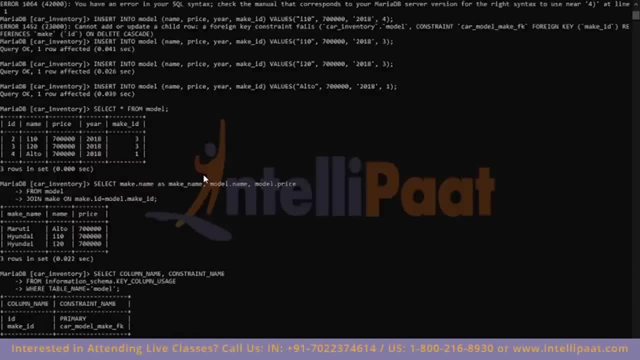 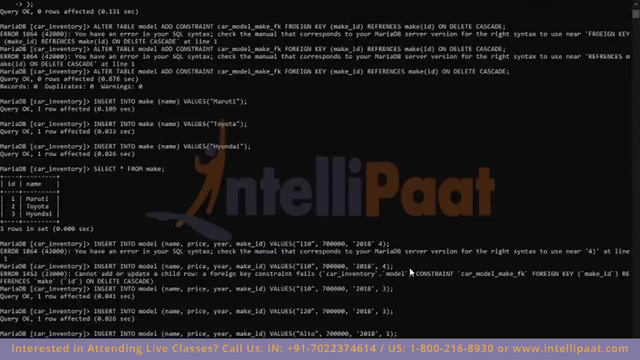 here is the model table and, as you can see, we have a primary key constraint on the id attribute and a foreign key constraint named car model fk, which is called make id. now i'd like to show you what we did when we applied the foreign key constraint and added the on delete. 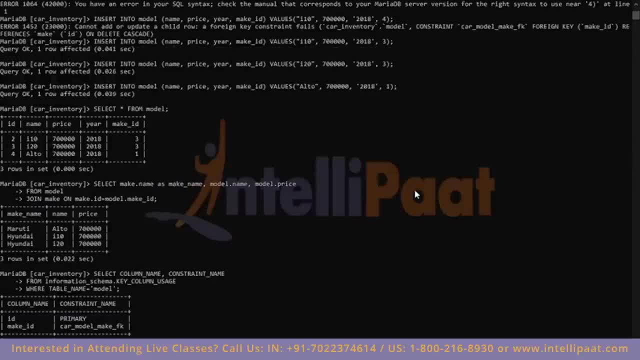 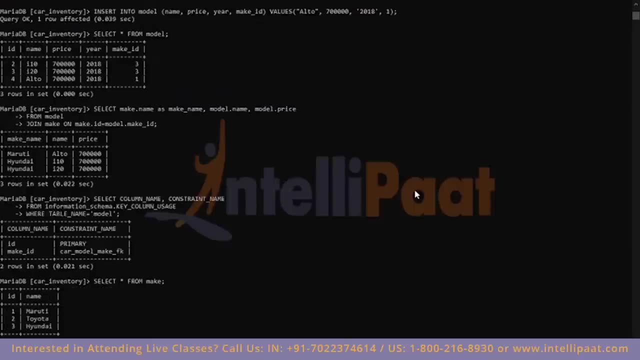 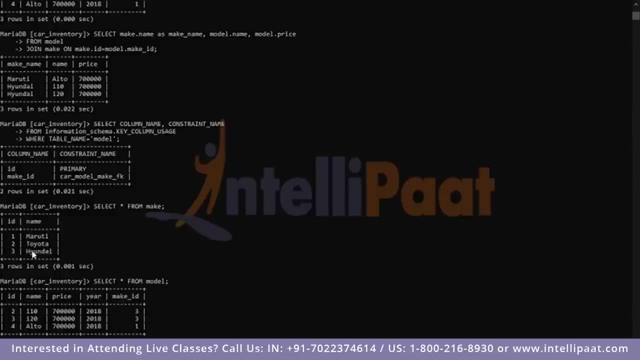 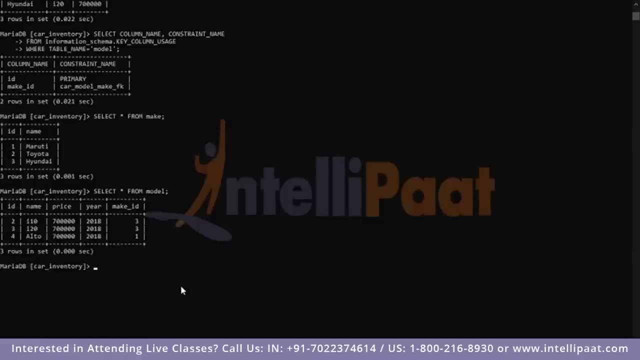 cascade. so what it actually means is that let me show you: we select everything from make, select everything from model. and now what I want to do is, when I delete the Hyundai row from our make table, the model table, every car related to Hyundai should be deleted automatically. so to do this, you 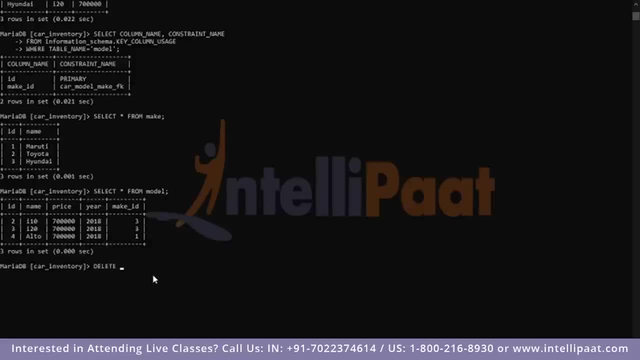 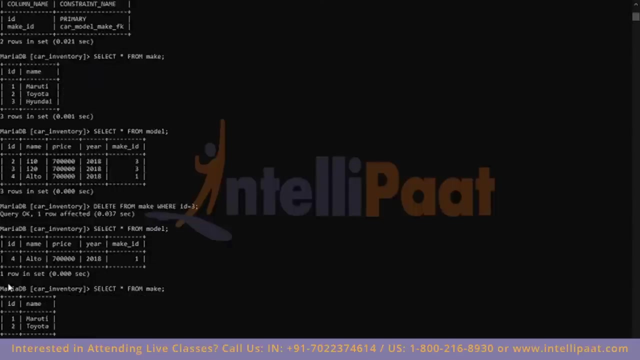 basically have to just issue a command like this: delete from make where ID equals 2 and the ID for the Hyundai is 3. I press ENTER. now let me see, and, as you can see, every car associated with the Hyundai make has been removed. this again enforces the integrity constraints and, as you can, 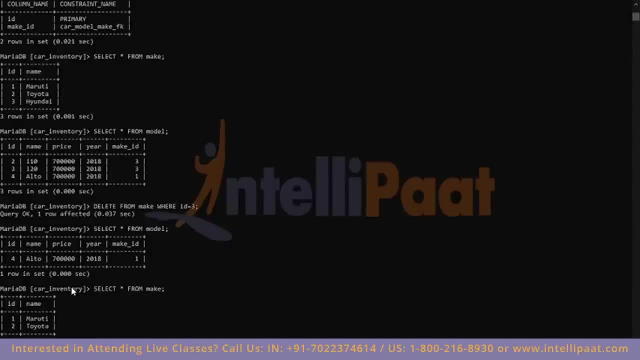 see, the Hyundai row is deleted from here as well. now, finally, I'd like to show you how you can remove a foreign key constraint. so, for instance, this: if you placed an incorrect constraint, how you can go about deleting it. so it's quite simple. all you have to do is type the query- alter table. the name of the. 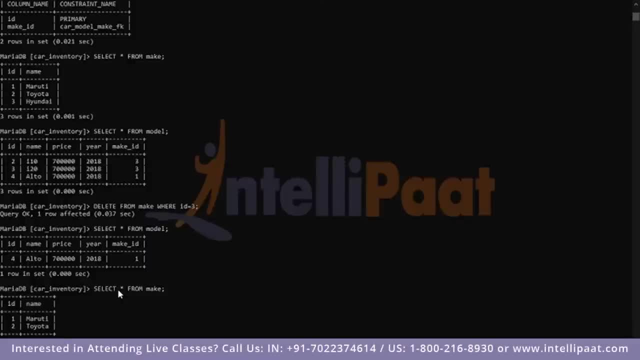 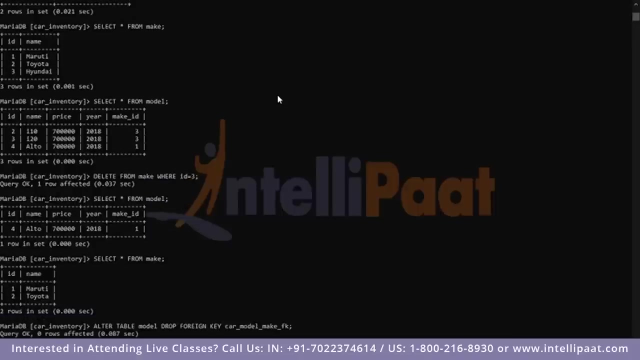 table on which we have placed the foreign key constraint was called model type- drop foreign key and the name of the foreign key, as we can see here, is car model: FK. car model make FK and I press ENTER and this is done. so now let me go up and see if the 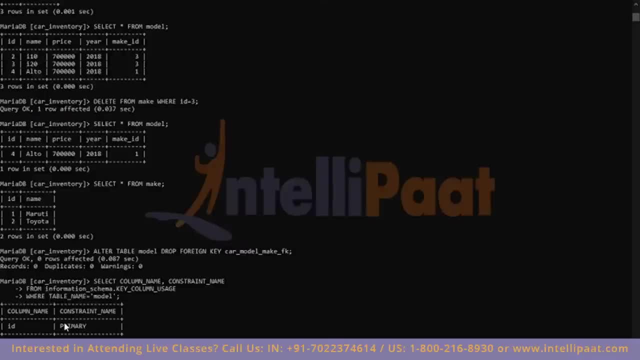 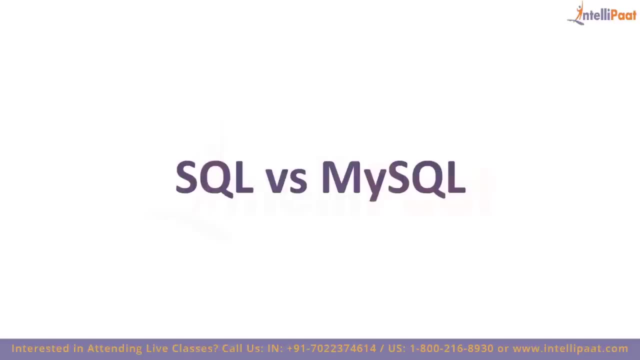 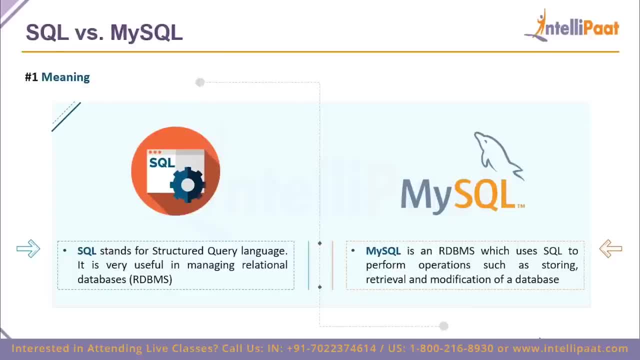 guys, as I told you, SQL stands for a structured query language and it is one of the most amazing language which is basically used to manage a relational database system. and what is mysql? mysql is the relational database system which is basically used alongside SQL to perform operations case. so any 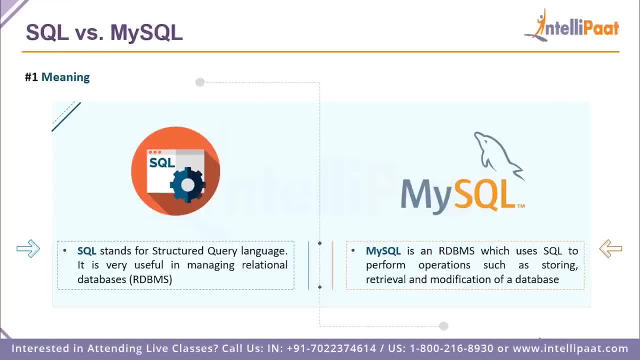 operations such as storing data, retrieval of data or modification of data in the database. and this brings us to the second point, which is basically complexity. when you have to talk about complexity, you know SQL as a language. it has to be learned on, it has to be worked on and practiced to ensure that you can make. 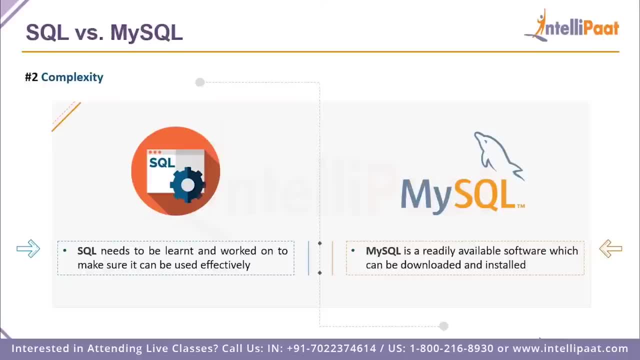 the most efficient use of your queries to work with your database. then, coming to mysql, you know, mysql is basically a readily available software, which is, you know, you can, which you can download it, install it and begin working with it without much of a prerequisite. and then coming to point number three, it is the. 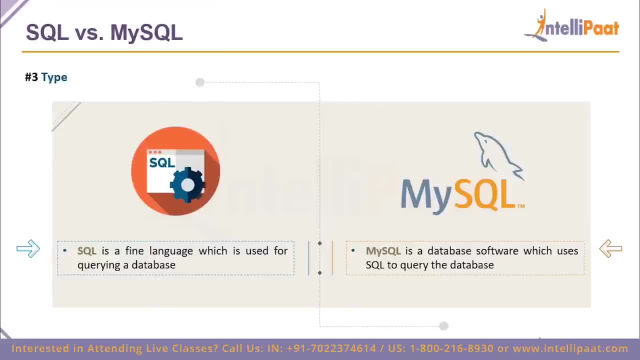 type of usage that we have to talk about, because SQL is a very fine language. it is a very well-tuned language which is put together to work with a database. but mysql is an entire database software, an entire platform, which is basically making use of SQL to query the database case. again, when you have to think about 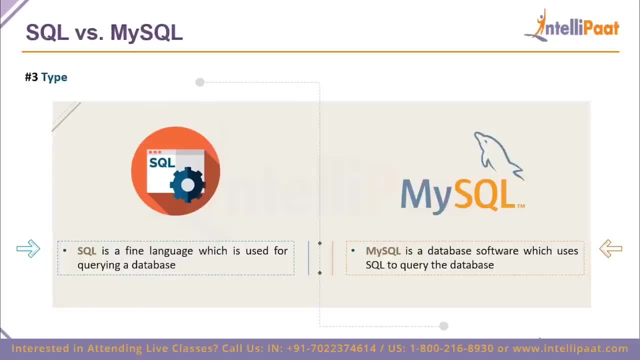 what to learn with. again, if you're using mysql, then obviously learning SQL is a prerequisite, but then if you're just learning SQL, then you might not have to work with a mysql database, because there are many other forms of relational database management systems where you can go on to use SQL as well. coming to 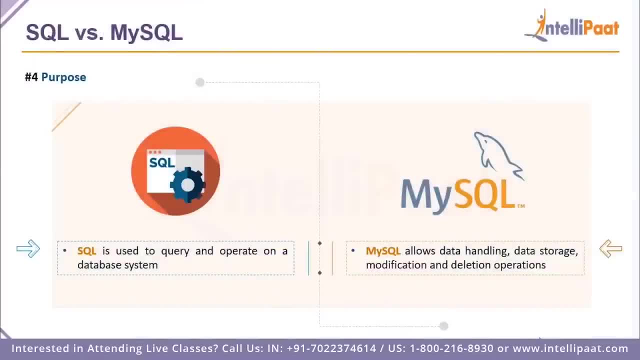 point number four. point number five. point number six. point number seven: point number four is the purpose. when you have to talk about purpose again, SQL is the language which is used to operate on the database, while mysql is the tool which allows SQL to perform operations such as data handling, data storage, data. 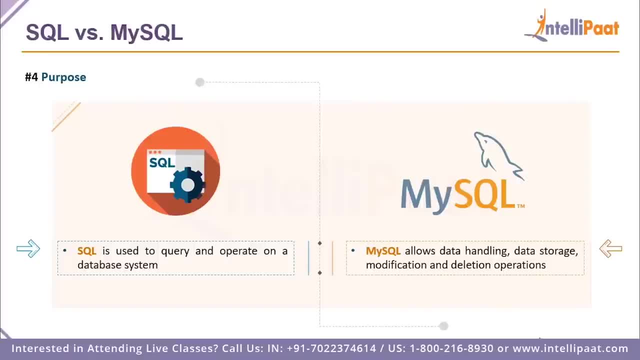 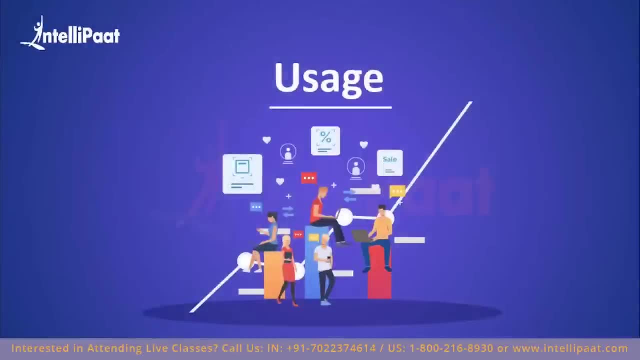 modification, deletion operations and much more. so I hope you guys are getting the general picture. your SQL is the language, while mysql is the database on which SQL works. with guys coming to point number five, point number five is the usage. when you have to talk about usage, again, there are various techniques. 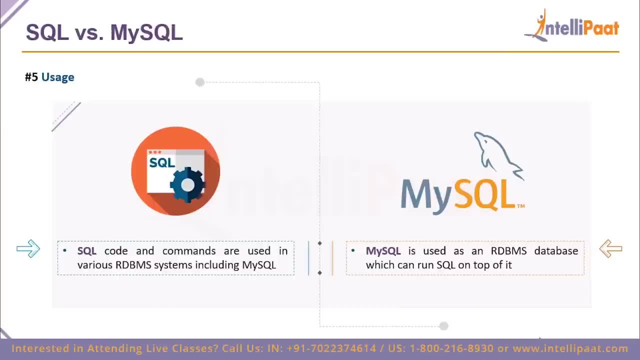 that mysql uses. you know there are multiple code segments, code snippets, multiple commands and pretty much everything else which you know is used to talk to various rdbms systems, and in fact mysql is one of them. but then we have to talk about mysql. mysql is the rdbms database, pretty much, which ensures 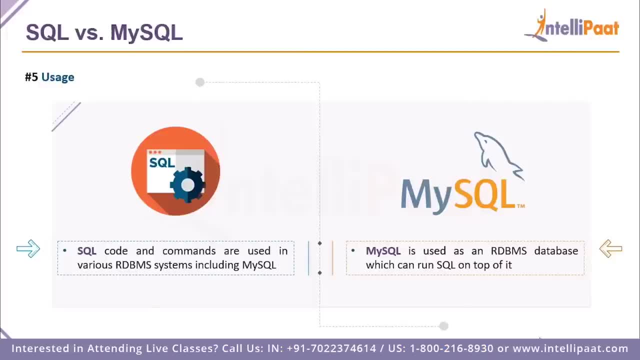 our languages, such as SQL, can run on top of it. but then if you're thinking, how well does SQL run on mysql guys? it is extremely efficient and even today SQL is a very old language and mysql is a pretty old open source software too. from mysql is a very old open source software too. from mysql is a pretty old open source software too. from. 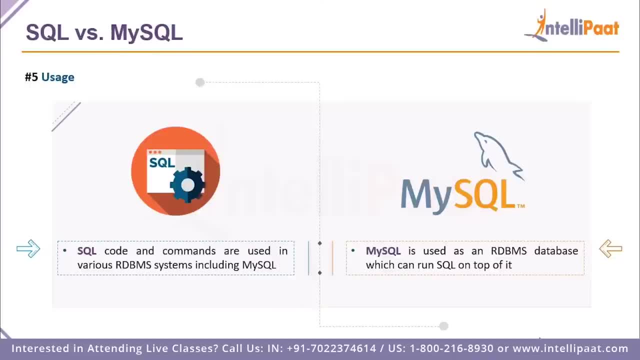 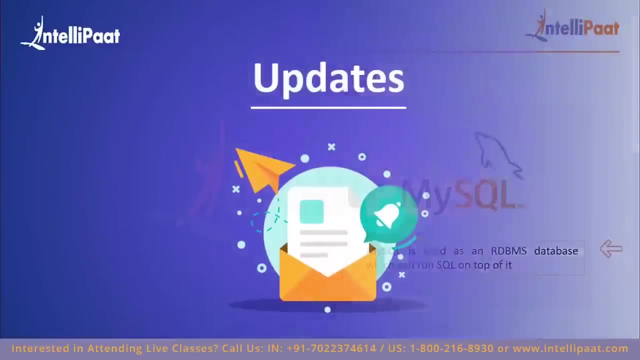 its day of the release pretty much all those years ago. it's still there and I would not consider calling SQL or any of the mysql rdbms as legacy because, as I told you, there are companies around the world- fortune 500 companies- who make use of these every single day, guys. and then, coming to point number six, it's updates. 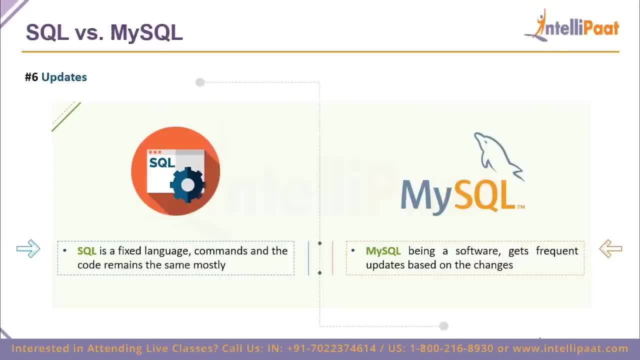 because SQL is a fixed language, right? so, no matter what, there are multiple flavors of SQL. of course. there's a Oracle SQL, there's some Microsoft SQL, multiple types of SQL, which is basically like a flavor of it you can run or pretty much, if you learn our SQL, right? so SQL is a fixed language, if you. 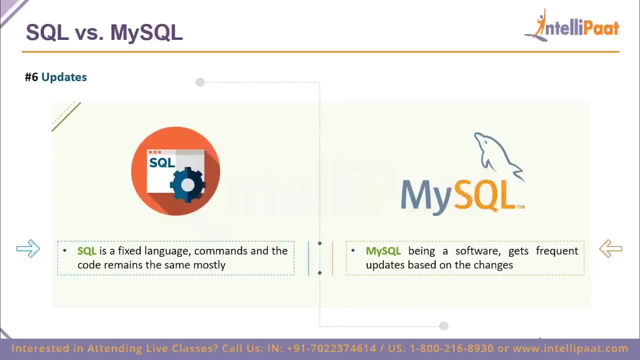 learn it, then pretty much you can all the code, all the commands, 99% of the code segments of the syntax pretty much remains the same. but then when we have to talk about mysql, are the updates are more frequent here because at the end of the day it's a software and it has to cater to various customer bases. but then 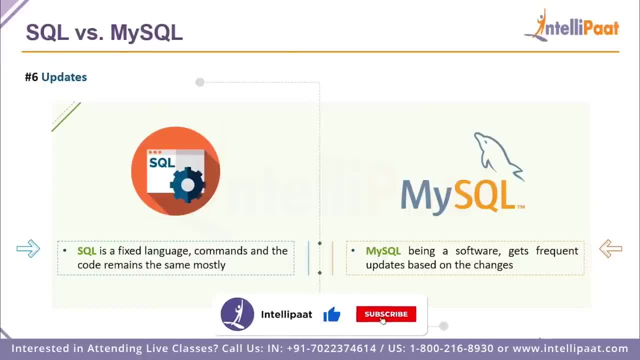 even, at the end of the day, solving bugs, making your software more efficient or helping you work with your database management system in a more efficient way. if that requires frequent updates, then yes, mysql provides that, guys. then coming to the quick summarization of this particular difference SQL. as I told you, it has been 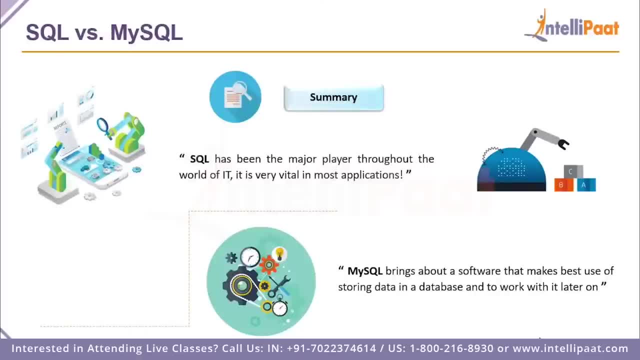 a big player. it has been a huge player in the world of IT and it is very, very vital when we have to talk about the applications and its usage in applications. guys, and coming to mysql, you know mysql brings about a software which pretty much makes the best possible way to store structured data. 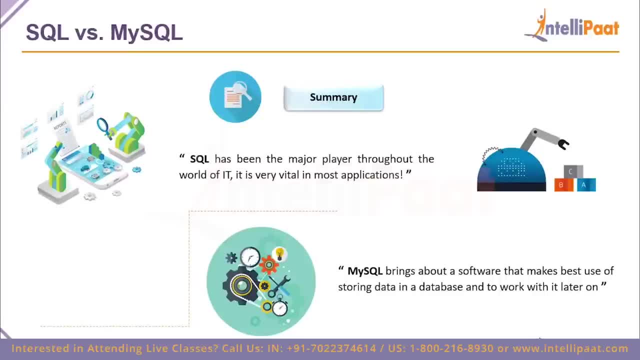 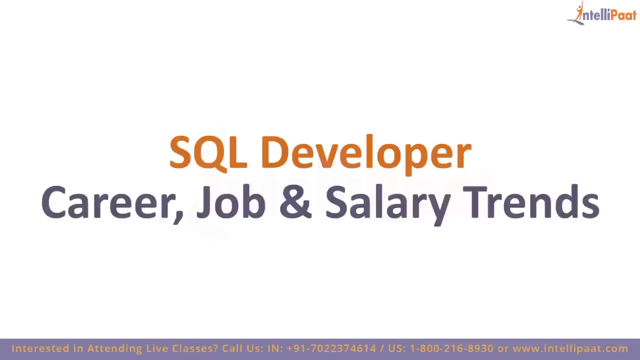 into it on the data database and eventually to work with it later on by making the developers or the coders life a lot easier. guys- and on that note you have reached the end of this quick comparison between SQL and mysql. okay, so we've seen that. next we look into the skills to have as a SQL developer. 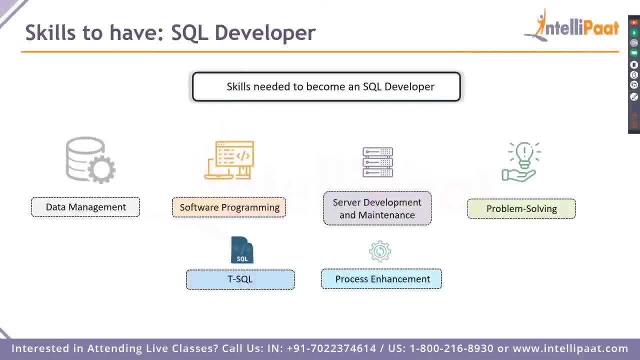 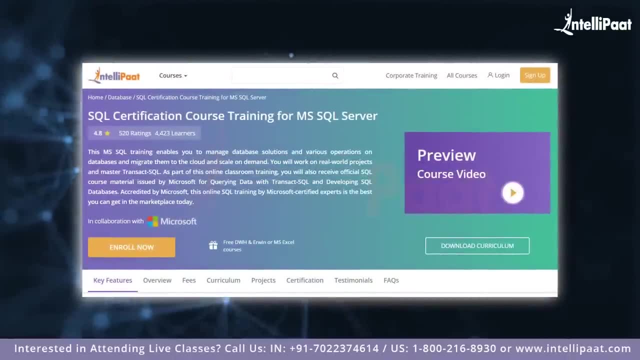 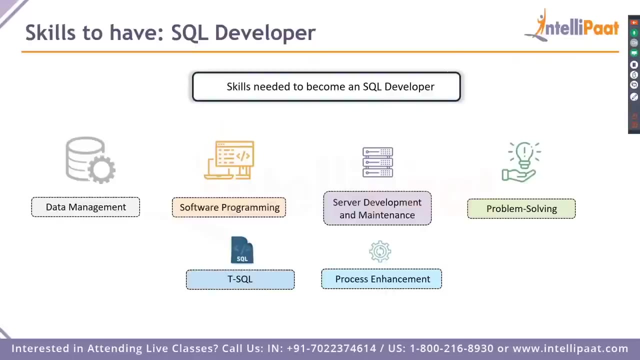 so we saw what are the requirements and the rules of an SQL developer. now the skills. just a quick info, guys, intellypad provides SQL online training in partnership with Microsoft and mentored by industry experts. the course link is given in the description below. now let's continue with the session. first of all, data management, obviously. 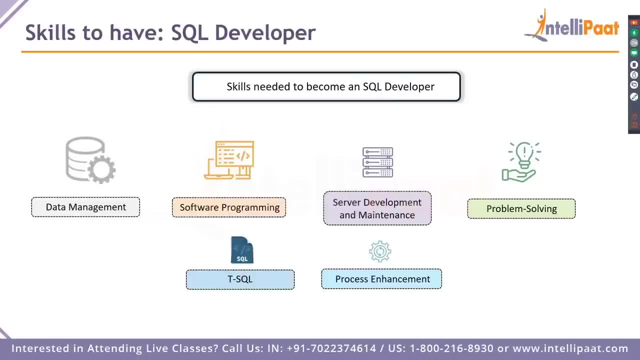 because database manages, so has data in it. so to manage that you will need to know a very good knowledge of SQL so that you will be able to manipulate it and also manage the data accordingly. software programming is recognizing an required. it is not mandatory that you can only become an sql developer having a very thorough. 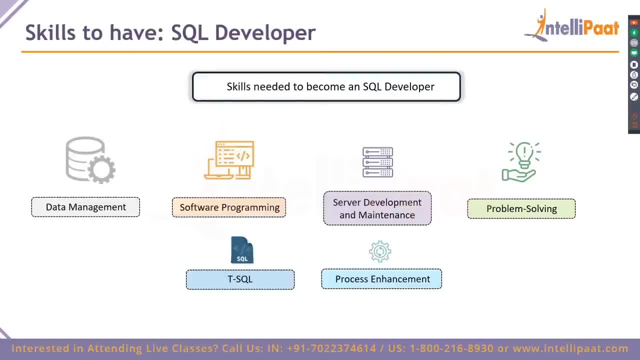 knowledge of a programming language, but having the basics or having the intermediate knowledge of software programming. so let's say your company uses java, then learning how java works will obviously help when you build a database for that company. so, because that database should be compatible with java and yes, so that's what you should also know. software programming server. 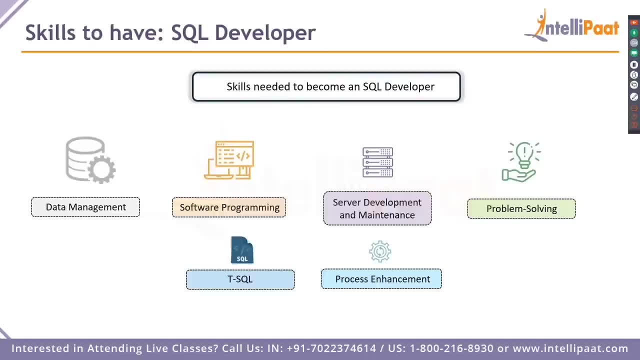 development and maintenance. so this again you can learn on the go. so server development in the sense to run virtual machines and to create databases on it and also maintain it. problem solving if there is a problem arise if there is a problem, so this particular person should be able to create a query. 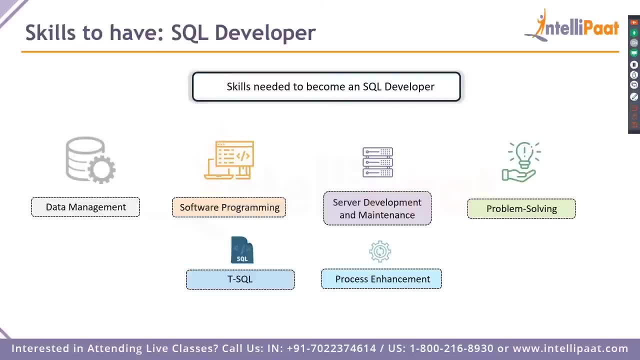 which solves that problem, or should be able to make the database more compatible. and then teamwork. so that's what you should also know. software programming, so this again. you can learn sql, which is basically related with transactions. so learning this is not compulsory at the beginning for an sql developer, but learning this will also improve their chances of getting a job. 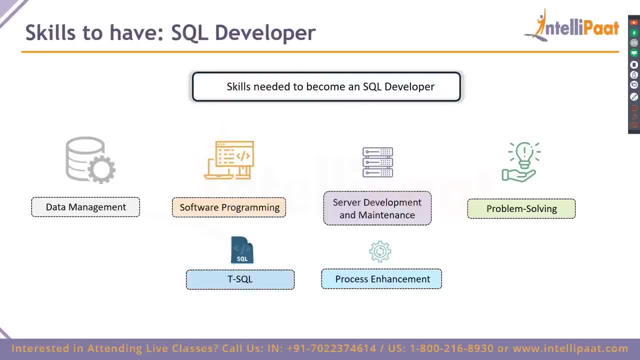 then process enhancement. this is to make better business decisions so you can be an sql developer and also be involved in process enhancement. that is, a company might go with a set of processes which is already organized and they go with that process and then they go with the process. 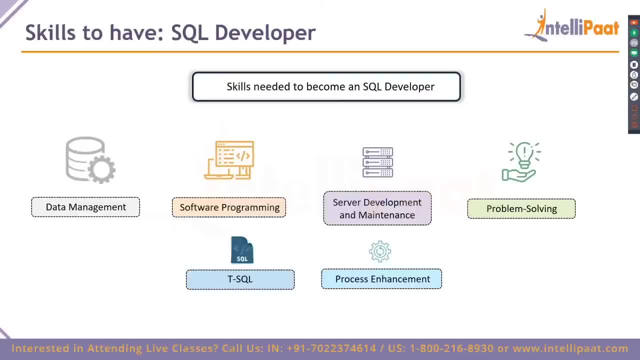 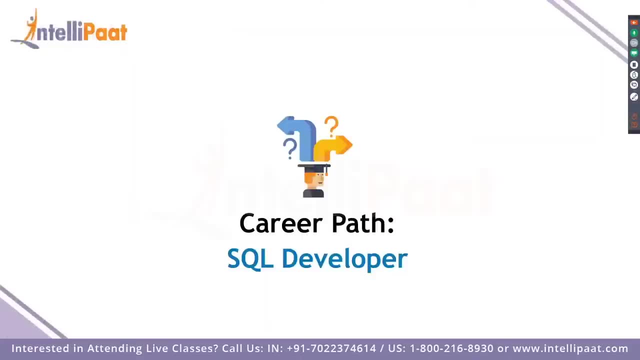 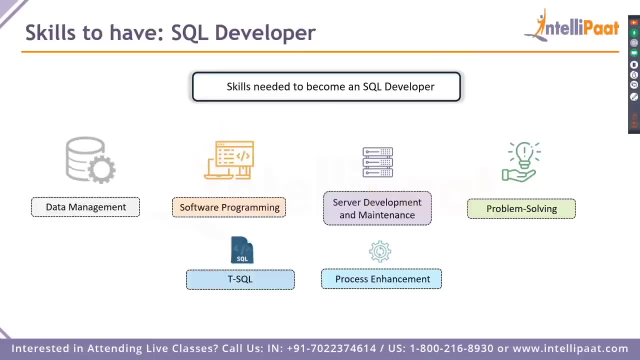 that flow. so, let's say, an sql developer can go ahead and change that process if that benefits the need. okay, so you've seen this, okay. so these are the basic skills which you need. first of all, learn sql. so that is the most basic thing. so if you learn sql, you will be able to manage data and 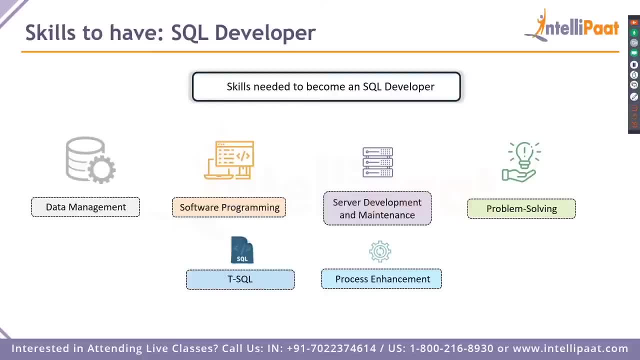 understand software programming, because without software programming, without knowing how an application works, you will not be able to build a compatible database with it. so you will be able to build a compatible database with it: development and maintenance, problem solving t sql and process enhancement. so make sure to go by the flow: start off with sql software programming and then move. 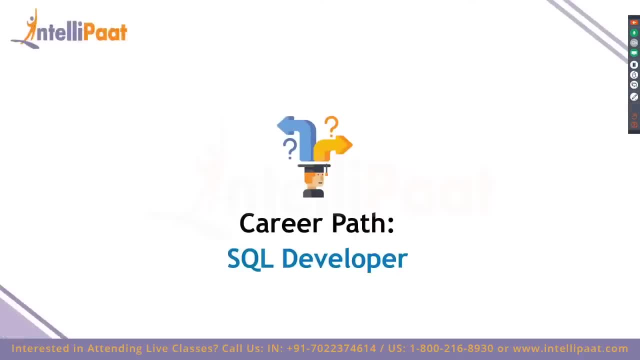 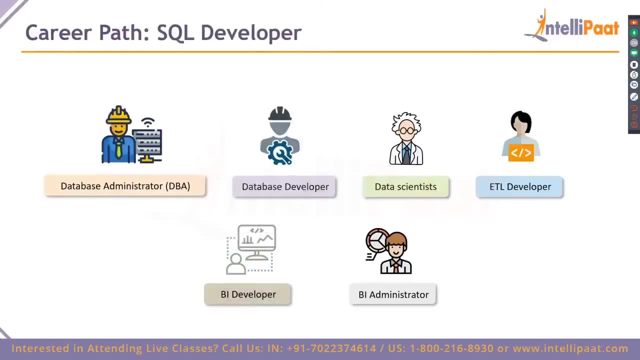 ahead with the other tools and then the career path. so once you have all these skills, you can obviously start applying for a job. then as an sql developer. there are various profiles, it is not just developer, there are so many different profiles within a company. so, as i told you, a 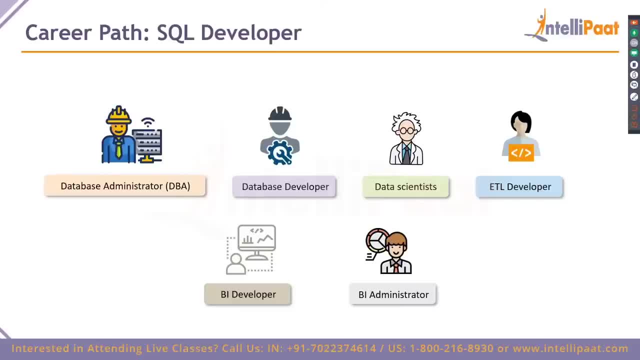 sql developer should be able to maintain, should be able to build, should be able to manipulate. so let's say, if you want to maintain a database, so you can become a database administrator. so the basic task of a database database administrator is to administer the usage of the database in. 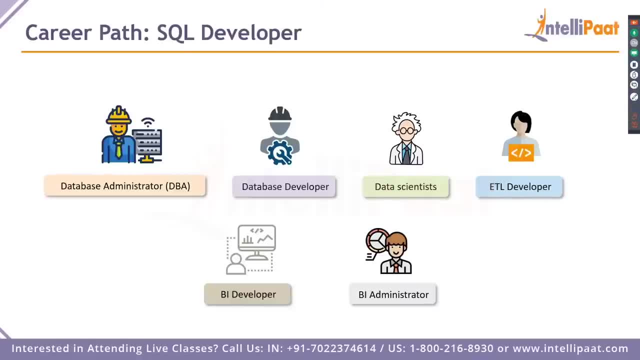 that particular company. so you will be the head of the entire database system. you will be able to administer every single transaction, so it's basically maintaining. and then a database developer is a person who builds and also manipulates databases. so you can also become a database developer by doing, by having the skills. so let's. 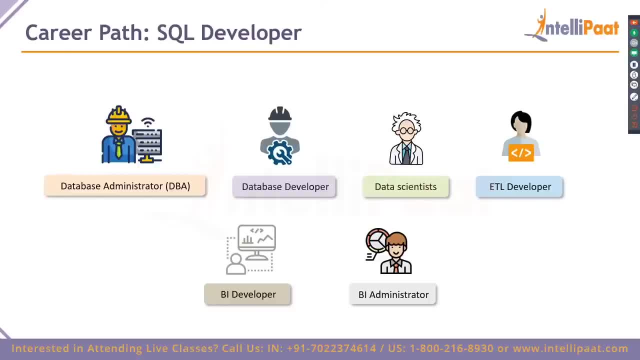 say for a database administrator, you should go with a more of a view that you will be able to manage any kinds of problems which are arising. you should be able to solve any kinds of problems which are arising. a database developer should go with. let's say, this person should be able to create 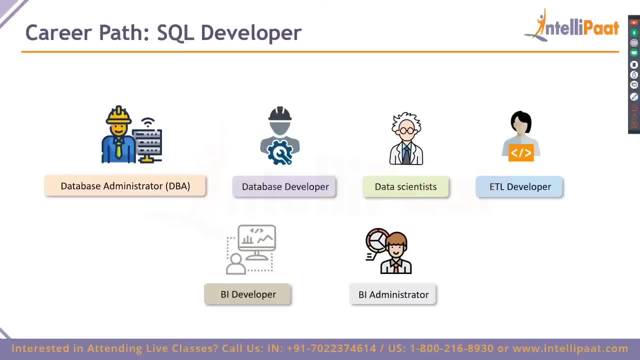 queries for any scenarios given in the company. okay, so next is data scientists. so obviously data scientists need sql. without sql it will be very hard for them. so sql is a need for data scientists as well. so learning any sql, that is, any sql engine, will help the data scientists. and then etl developer. 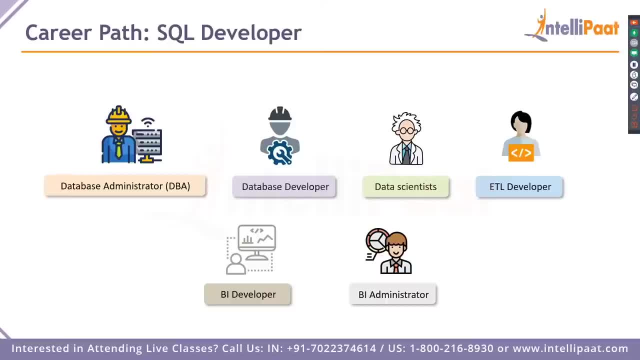 so this basically involves big data: extract, transform and load. and again you can also become an etl developer by learning sql and then you can also become an etl developer by learning sql and learning databases. then bi developer and administrator. so bi is business intelligence. so in business intelligence you obviously need to create visualizations and to create visualizations. 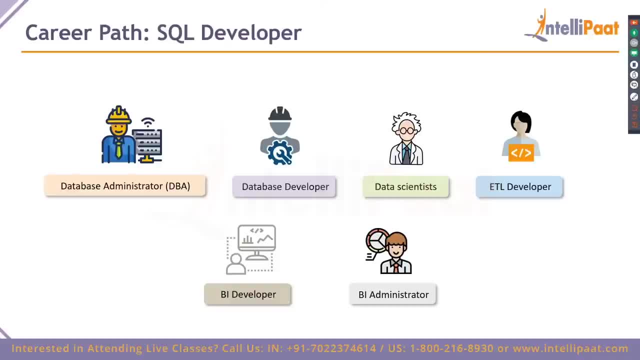 you need to manipulate or query data and to do that you should obviously know sql and it will help in becoming a bi developer. so to become a bi developer and an administrator, you should not just know these skills which i showed you for an sql developer, you should also learn bi tools. 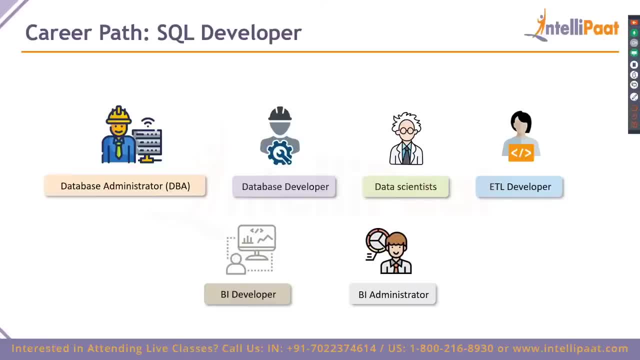 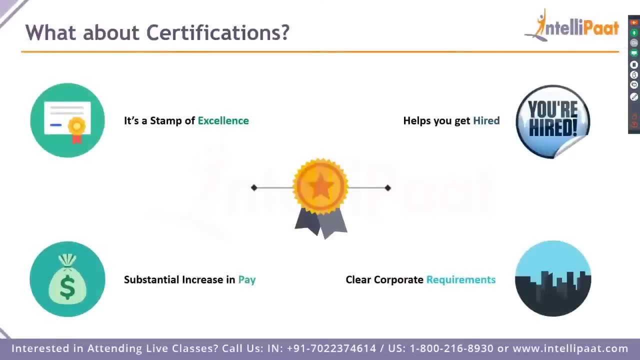 like tableau or power bi. so only then you can more head with bi. okay, so now we've seen that we look into the certification path for an sql developer. first of all, uh, what are certifications and why do you need it? first of all, it's a stamp of excellence, that is, if you have it on your resume. 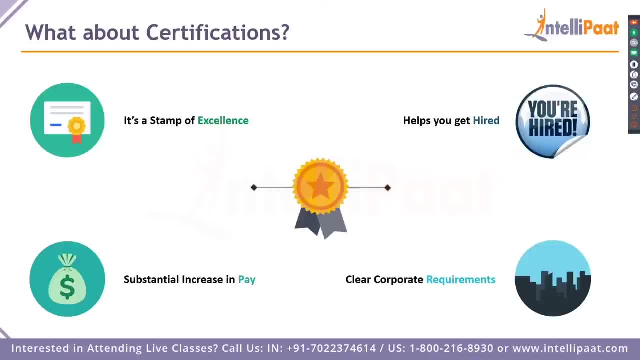 it adds value, so that you don't need to even explain that you know database. if they see that you have a certificate from oracle or, let's say, a certificate from microsoft, they're going to understand that you have prepared and cleared that exam and you know well enough. and then 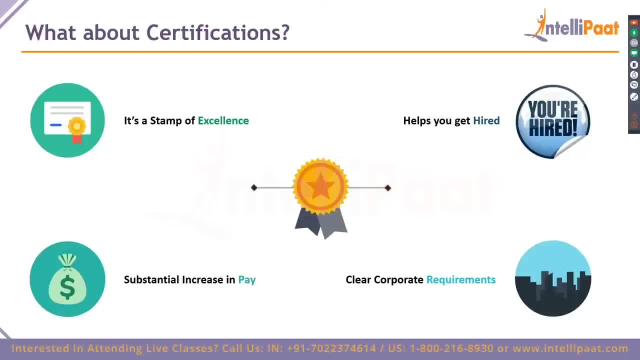 substantial increase in pay. so once you get earning certifications, obviously you are putting in time and effort to make yourself better in your career, so that will obviously give you a good hike. clear corporate requirements: so, as i told you, every single company needs a database developer. so for that, so for clear corporate requirements, that is. 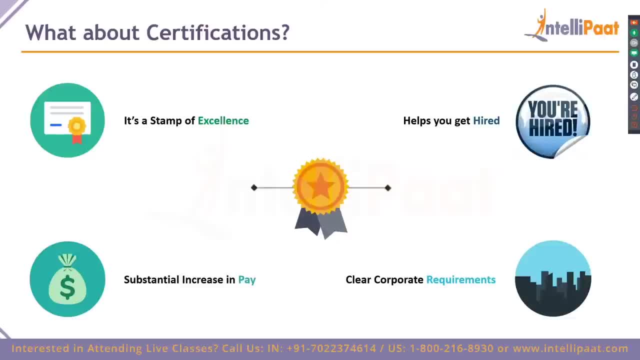 might have a requirement of having a particular certification and that will help if you're going to go for that particular job and helps get you hired. so obviously these everything goes back to that point. so these are certifications. why do you need a certification? and also, while you do, 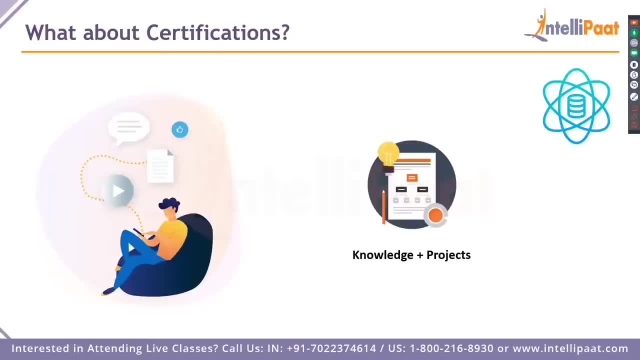 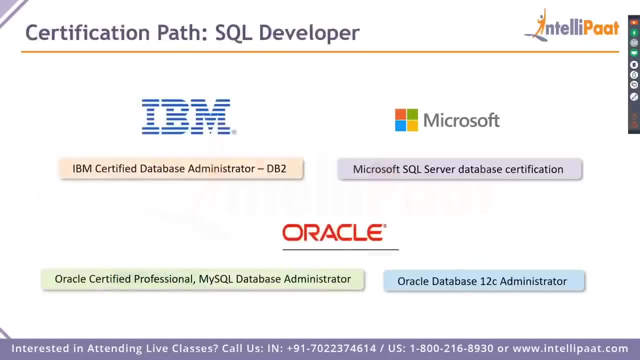 certifications, you'll be able to understand a lot and also will be able to experiment with a lot of projects before you enter enter the corporate career itself. okay, so these are some sql developer certifications. first one is the ibm certified database administrator, db2, so this involves the 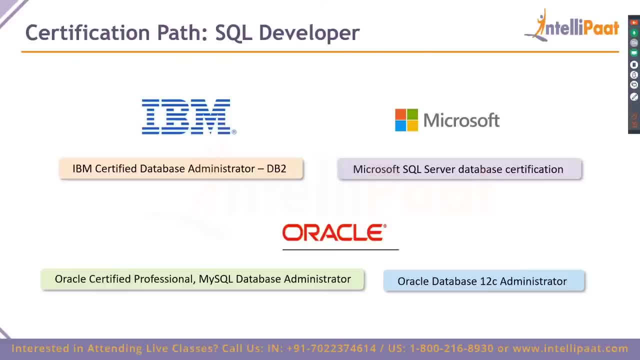 database called db2. then microsoft sql server database certification. this involves microsoft sql and then oracle. under oracle there are two. one is oracle certified professional or mysql database administrator. so mysql is one of the most popular databases in the world and you can go ahead with mysql database administrator without any hesitation. 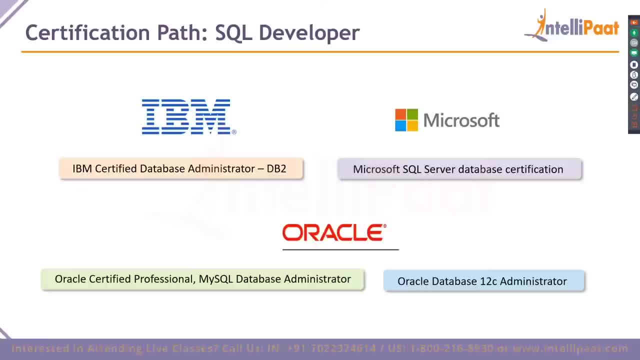 but the one more thing you'll have to remember is there are n number of mysql database administrators or oracle certified professionals also. oracle database 12c administrator is also one more certification which you take up to go for a particular role. so these are some of the most. 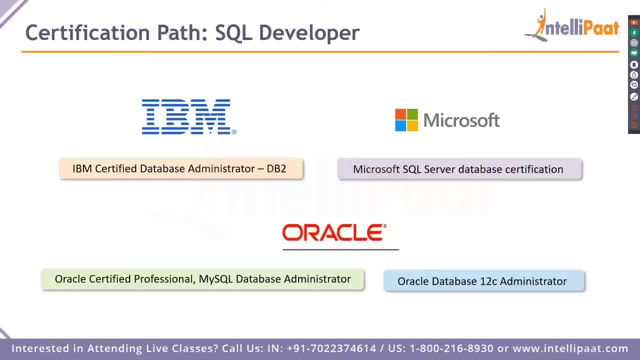 popular certification courses. so in s for sql developer. so if you want to- it is not just so- let's say, if you complete the ibm certification, it is not just you can go for ibm. the thing is you can go for any company which uses db2 or, if you do, the microsoft sql server. so 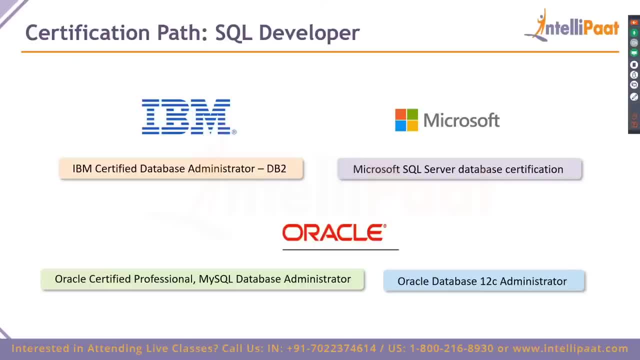 any company which uses microsoft sql server needs a database developer or an administrator with an apt certification, and you can be eligible for that, and same goes with oracle. so these are some of the popular certifications. you can check out more. if you want to check out other, uh, so let's say maria. 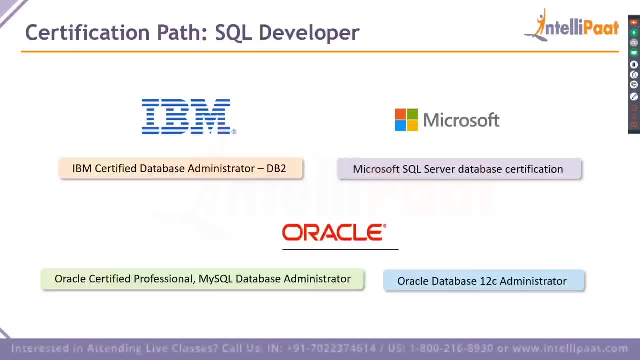 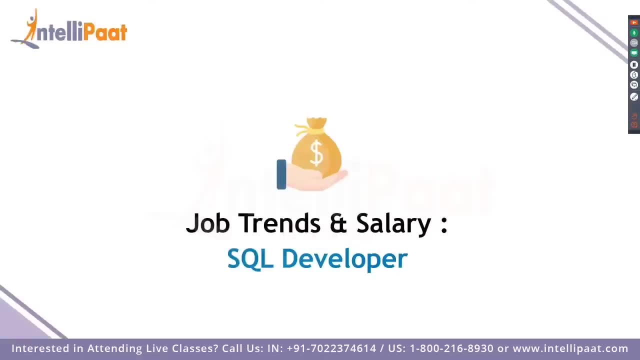 db or there are. there is a number of database engines out there. you can go ahead and check them out. so these are some of the popular certifications and highly recommended. okay, so we've seen that. now let's look into the most important part, which are the job trends, because obviously, at the end of the day, you will need a job and also salary. so first of 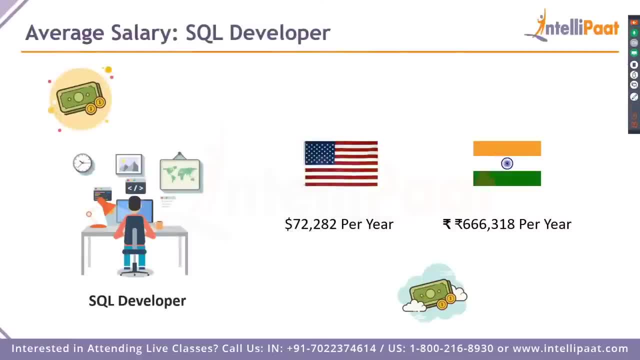 all sql developer in the usa. they are getting about seventy two thousand two hundred and eighty two dollars per year as an average. so this is the average amount. there is low, there is a low, there is a high to this and an. it goes around six point five lpa. so these are the two variants in us and india. so this is for an. 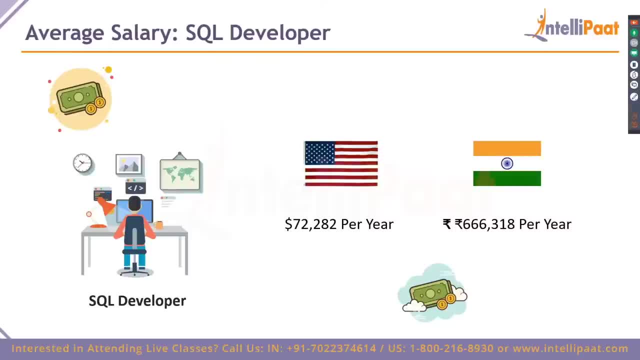 sql developer role and this is totally relative, because this is uh. this data is collected from glassdoor or p scale, and those data is based on the salaries. which other uh- let's say there are hundred users in glassdoor who are sql developers. if they post their salary, it is aggregated and the 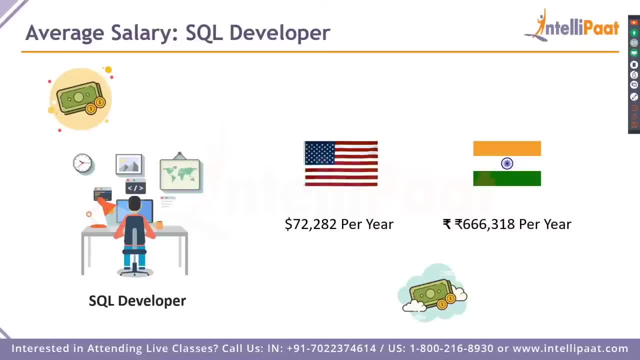 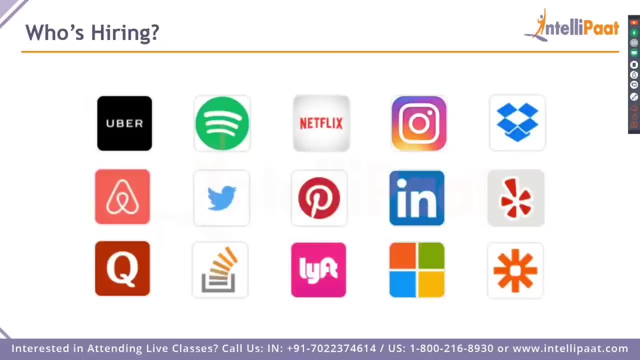 salary is given to you as the salary which is provided here, so it can vary. it can be a, it can be lower than this for a beginner and it can be higher than this for a experienced database professional. so we've seen that. so who's adding? so every single company which uses the database. 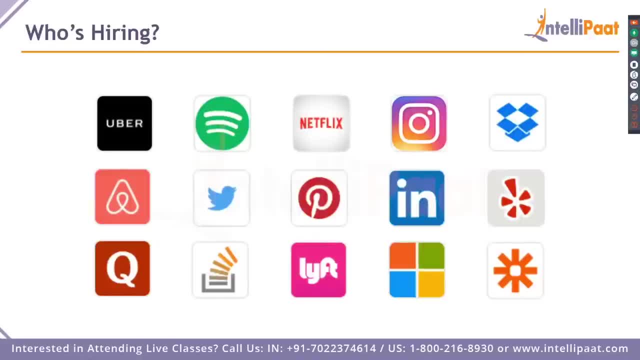 so that puts under uber, spotify, netflix, instagram, dropbox, airbnb, twitter and any other company. so you can go ahead, learn this and you will have to pick out. you will have n number of companies to pick out. you can attend a lot of interviews and, if you're talented enough, you will be able to bag a job in a couple of 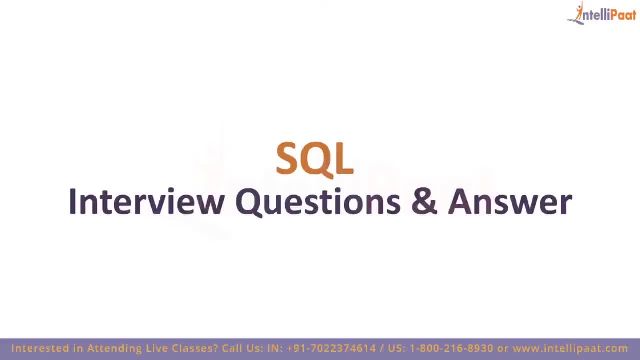 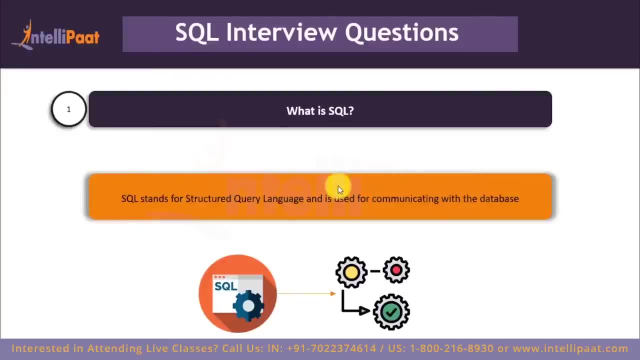 days or maybe weeks. so what exactly is sql? so this is a very basic question. so, to answer this, sql stands for the structured query language and according to ansi, it is a standard query language for relational database management systems which is used for maintaining the relational database. 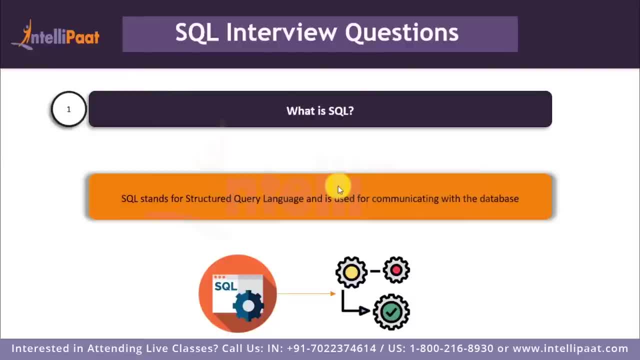 and also to perform different operations of data manipulation on different types of data. so sql is widely used language for maintaining relational database and in the year 1986 sql became the standard of american national standards institute or ansi. so basically it is a database language which is used for creation and deletion of databases and it can be used to fetch and modify. 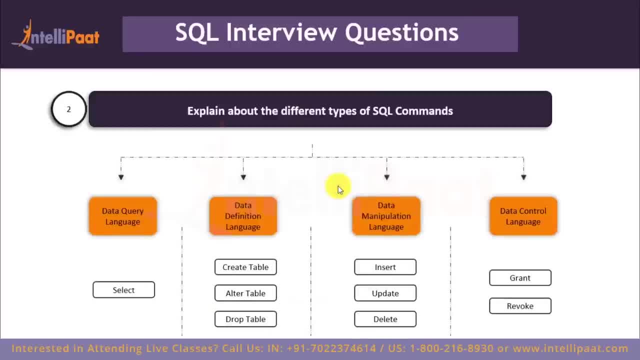 from the table and also multiple other things. so let's head on to the next question. so we are supposed to explain the different types of sql commands. so the sql commands can be divided into four categories. so we've got data query, language data definition, language data manipulation. 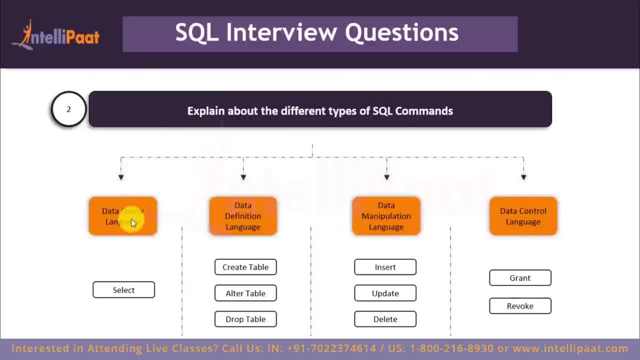 language and data control language. so the data query language comprises of just one command, select, though it can be accompanied with many clauses to compose queries on a database. then we have the data definition language. so ddl is that part of sql which defines the data structure of the database in the initial stage. 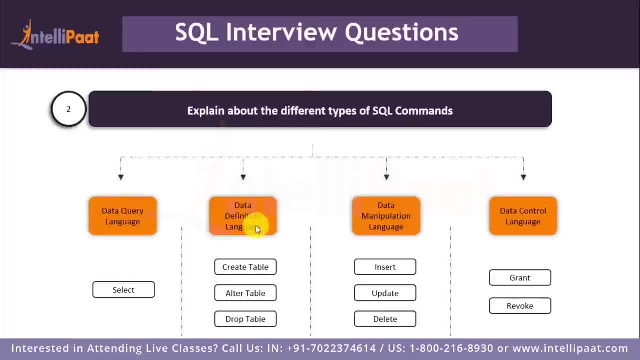 when the database is about to be created. so it is mainly used to create and restructure the database objects. so you can see commands like create table, alt table and drop table in ddl, and after that we have the data manipulation language. so dml is used to manipulate the. 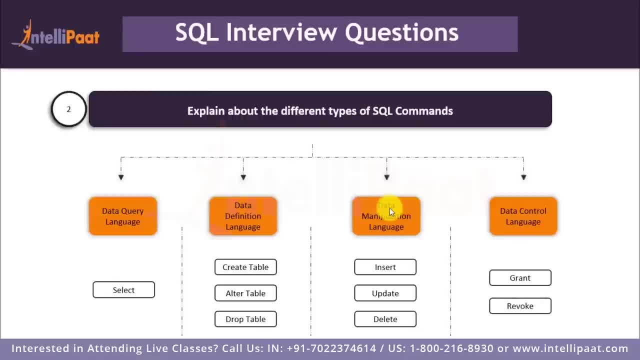 already existing data in the database. that is, it helps the user to retrieve and manipulate the data. is used to perform operations like inserting data into the database through the insert command, updating data in the database through the update command and deleting data from the database through the delete command. and finally, we have the data control language, which is used to control access. 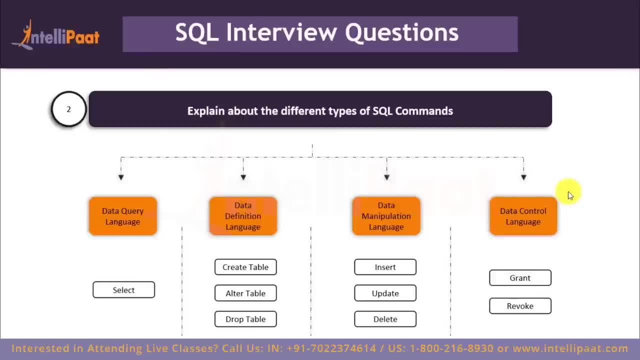 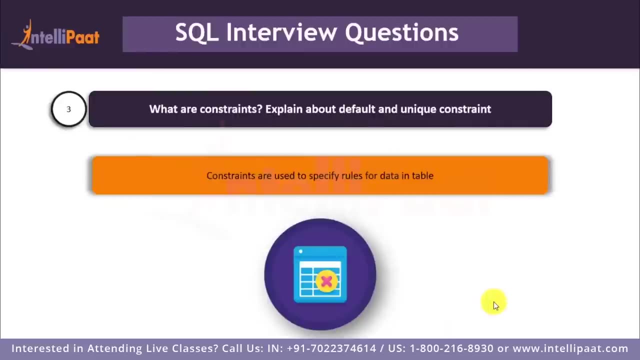 to the data in the database. so these dcl commands are normally used to create objects related to user access and also to control the distribution of privileges among users, and you see commands such as evoke and dcl right. so this is the next question. so what exactly are constraints and 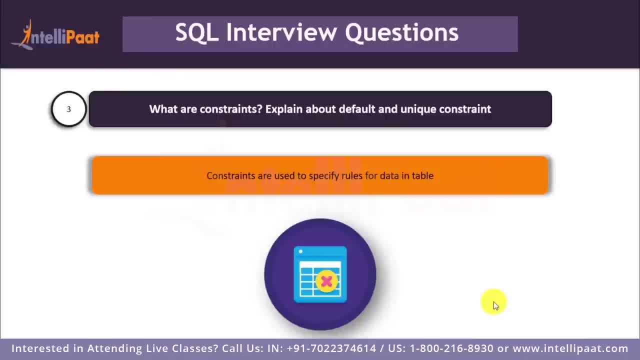 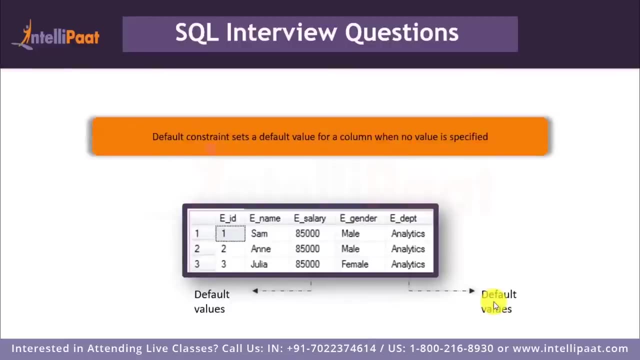 we are supposed to explain about the default and the unique constraint. so constraints are basically used to specify some sort of rules on the data and limit the type of data that can go into a table. right? so let's understand about default constraint. so the default constraint is used to provide a 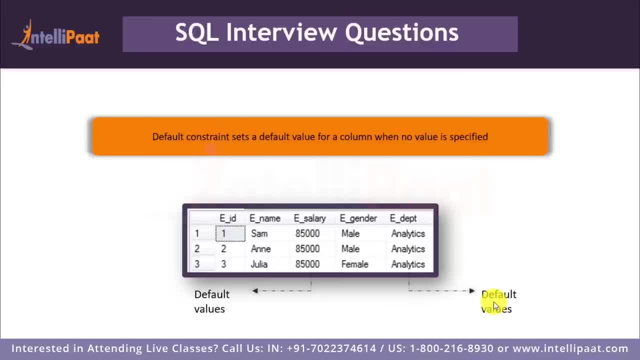 default value for a column. so the default value will be added to all the new records if no other value is specified. for example, if we assign the default constraint to this e salary column and set the default value to be equal to 85 000, then all the entries of this column will have a default. 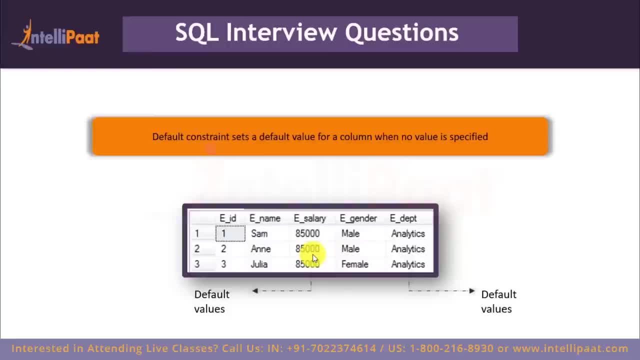 value of 85 000 if no other value is assigned during the insertion. so similarly, we can also assign a default value of analytics to this edept column, right. so now we'll go to sql server and we'll work with the default constraint. now i'll start off by creating a new table. 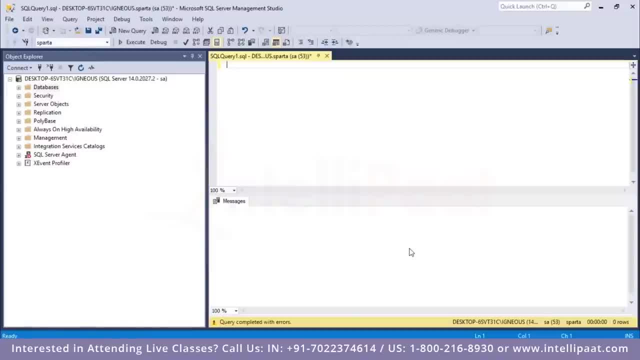 and i'll add the default constraint to one of those columns. so i'll create a new table and i'll name this table as stu1. so the syntax would be: create table stu1 and this would comprise of these columns, so that would be s id, which basically stands for the student id and the data. 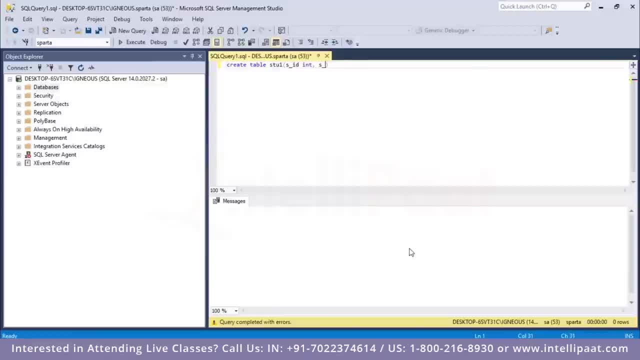 type of this column would be integer. after this, there is s name, which stands for student name, and the data type would be varchar, and the length of the string, or the maximum length of the string, would be 20.. and then i'll finally have the marks code by the student, which would be s marks, and this would be of integer type. now, after this, 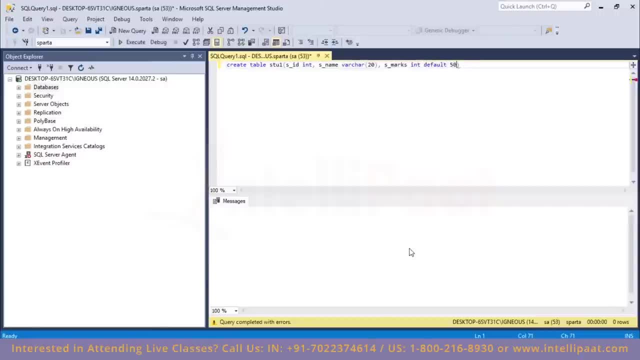 i will give in the default constraint and i will set the default value to be equal to 50.. right, so i have successfully created this table. now let me have a glance at this table first. so select star from stu1. this is our table, which is empty as of now. now what i'll do is i will go ahead and insert some. 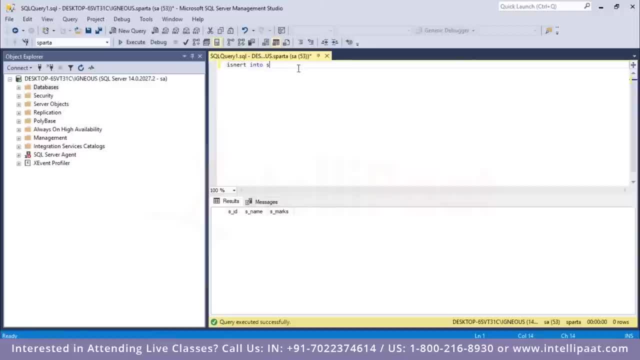 values into the table. so i'll type in: insert into stu1 and then i'll give in the name of the columns. so this needs to be i n s e r t. so the name of the first column is s id and then i've got s name. 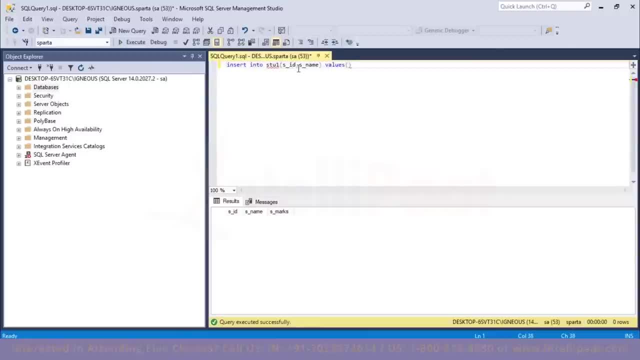 now i'll type in values and given the values for these two columns. so let's say the first id is 1 and the name of the student is sam. now i'll click on execute. now let me have a glance at this modified table. now select star from stu1. so now we see that we have this default value of. 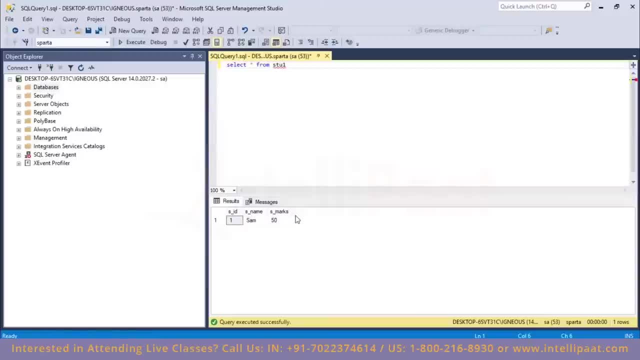 50 in this s marks column, and this is because we had assigned the default constraint to this column. now, similarly, let me add two more records into this table, so insert into stu1 s id s name. i'll give in values, so it'd be 2, and the name of the second student is bob. 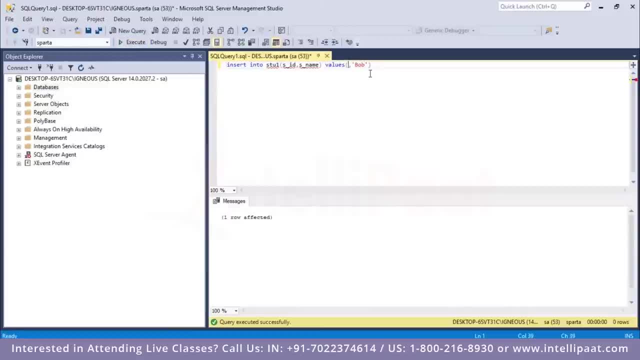 right. so i've also added the second record. now let me add in the third record. so the student id is 3 and the name of the student is matt right. so now i have three records in this table. select star from stu1. so these are the two new records and the default value is 50 for these two new records. 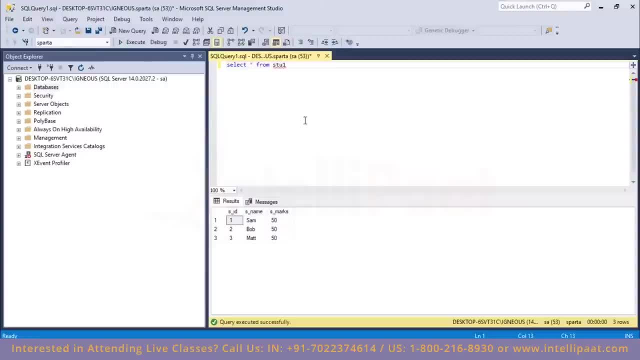 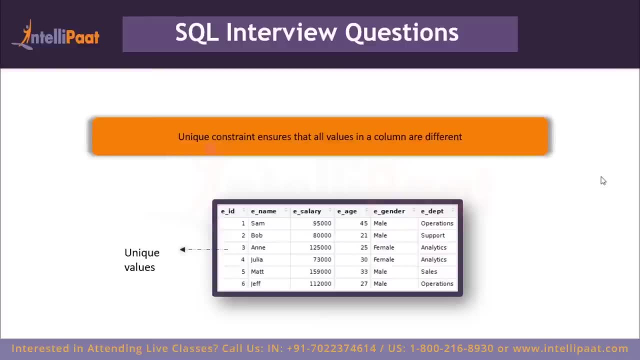 so this is how we can work with the default constraint. now comes the unique constraint. so the unique constraint ensures that all the values in a column are different. for example, if we assign the unique constraint to this e-name column, then every entry will be the same as that of the. 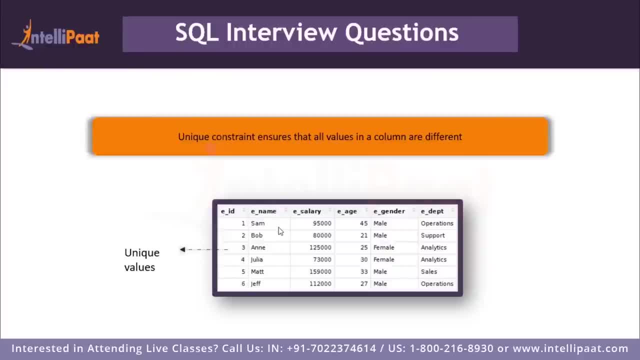 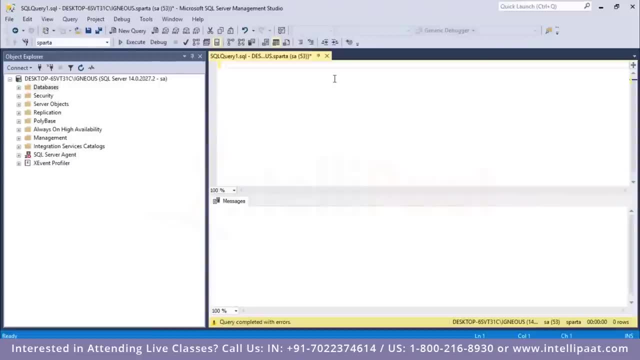 first column in this column should have a unique value. so here we see that all the names of the employees are different. now again let's go to sequel server and work with a unique constraint. so again I'll create a new table and add the unique constraint to one of the columns. create table and this time the name of the 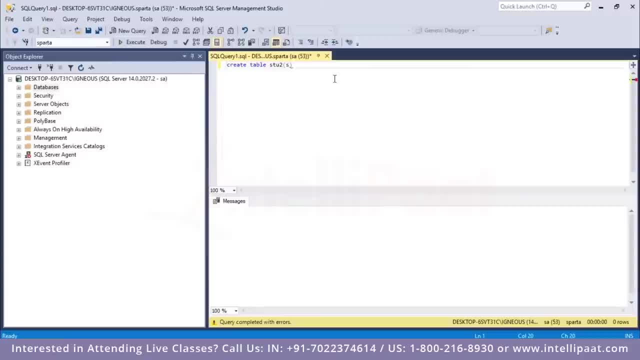 table would be stu2. again, there would be the ID, and this is of integer type. now I would be assigning the unique constraint to this SID column. and there would be a second column which is basically the student name, and this is of wirecard type. again, the length of the string would be 20. right now, let me have a glance at this. 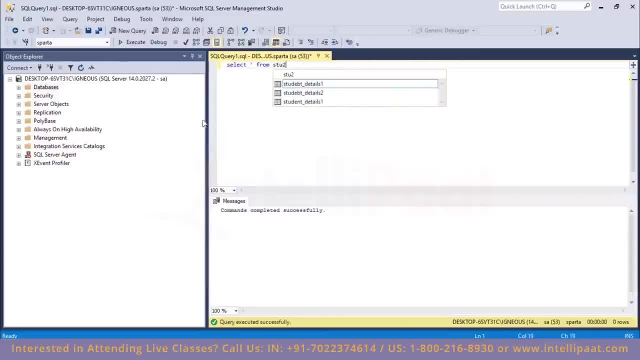 table again. so select star from stu2. so this is our new table, which is empty as of now. now let me go ahead and add values into this. so insert into stu2. so insert into stu2 values. I'll add in the first record, so one which would be the student ID name. 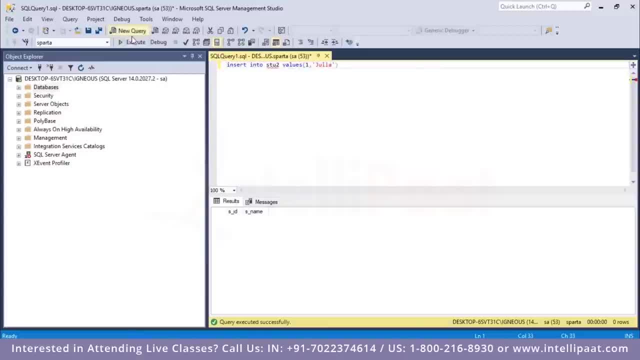 of the student is Julia. now let me look at this table. select star from stu2 right. so we have successfully inserted this record. now let me add a new record. so insert into stu2 values. so we have successfully inserted this record. now let me add a new record. so insert into stu2 values. 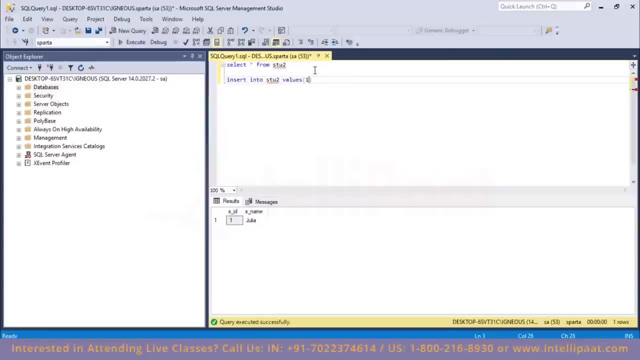 now what I'll do is I will again give the ID of the student to be one and the name of the student to be Matt, and let's see what happens. so this time we get a message, or a warning message, and this states that violation of unique key. 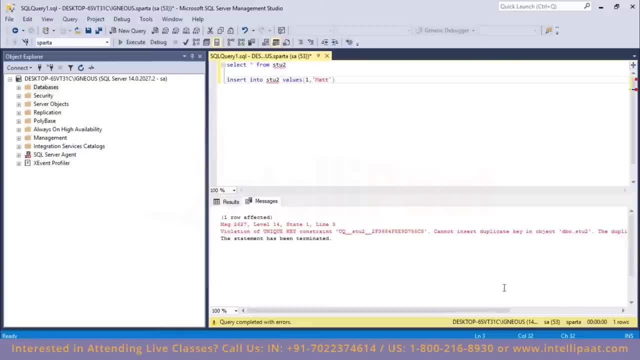 constraint and we cannot insert duplicate key in object DBO dot stu2, and that is because we had given the unique constraint to this SID column. that is why this has to be different. so let me change this to be 2 now. let me again run this right. so now, since this is a unique value, 2 is not a duplicate. that is why. 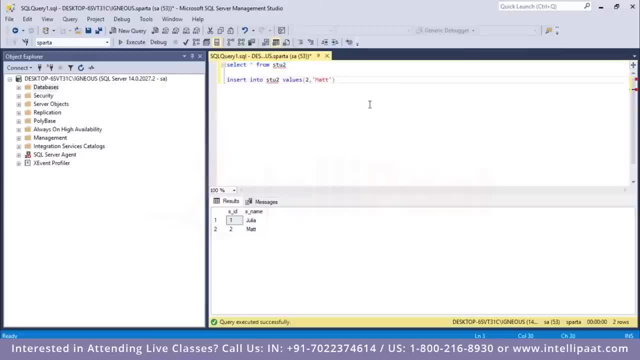 we were able to insert this record. now again, what I'll do is let me add another record with the ID 2. so let's say now the name of the student is Annie. now again we get this warning message because ID number 2 is already present. 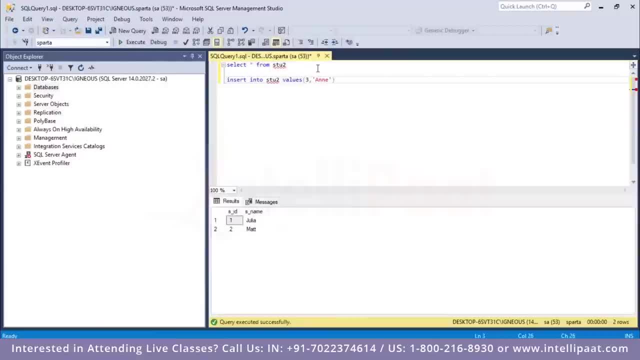 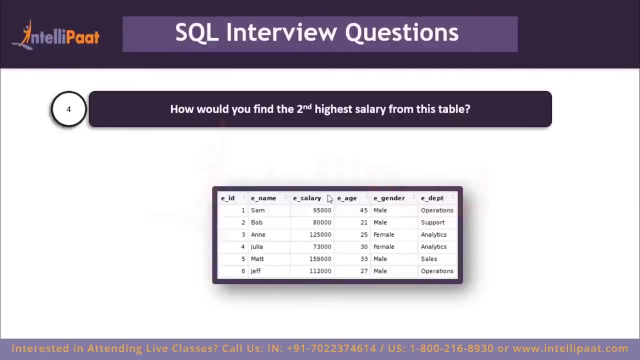 so let me change this to 3. now let me run this again: right, so now we are able to insert this record. so this unique constraint basically make sure that there are no duplicate records inserted into this column. so now we have the next question. so, again, we have this employee table with us and we are 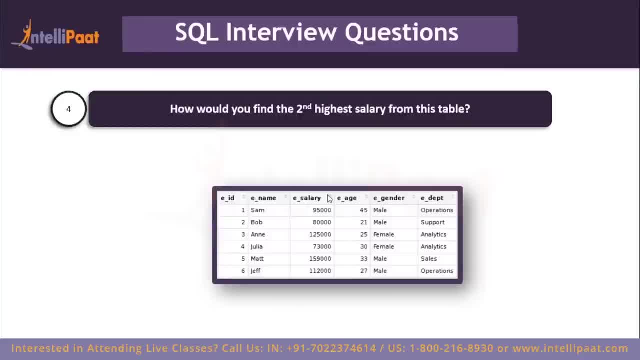 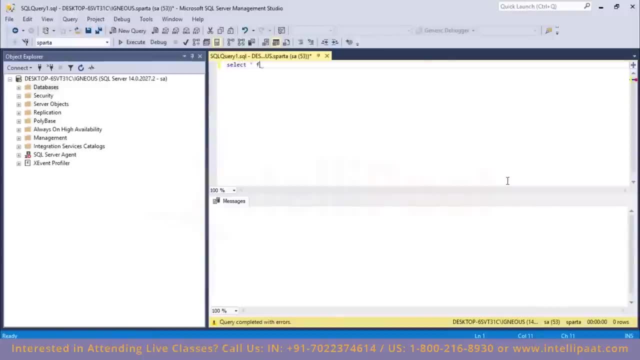 supposed to find out the second highest salary from this table, so let's go to sequel server and find out the solution. so let me start off by having a glance at the employee table. select start start from employee right. so this is our employee table over here and we see that. 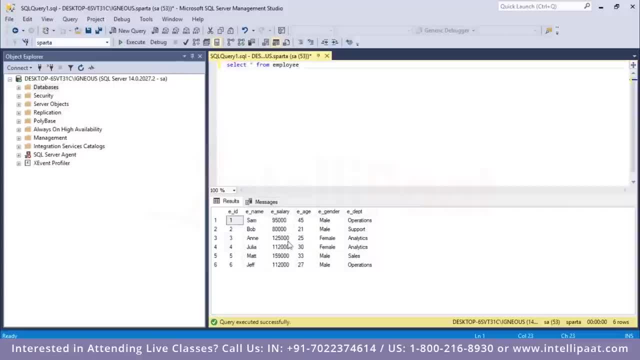 the highest salary is 159,000 and the second highest salary is 125,000, so we are supposed to extract this particular value from this data set. now let's see how can we do this, so we can perform this operation with the help of sub. 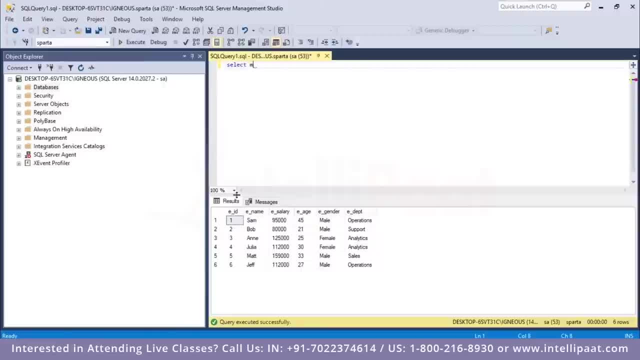 query. now let me just type in the command select and since you want the maximum value, I'll use the max aggregate function and this would be e salary. so I want the maximum salary from the name of the table is employee, I'll give in the where clause and, given the condition where e salary is not in after, 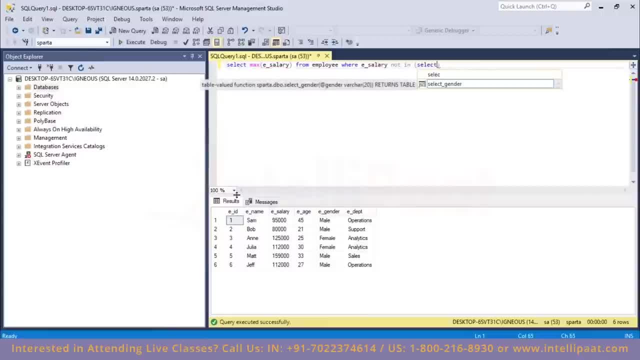 this I will give in the sub query over here. so the sub query again would be the same. so select max of e salary from employee. so now, if you have a glance at this, you would see that both of these queries are same. so select max of e. 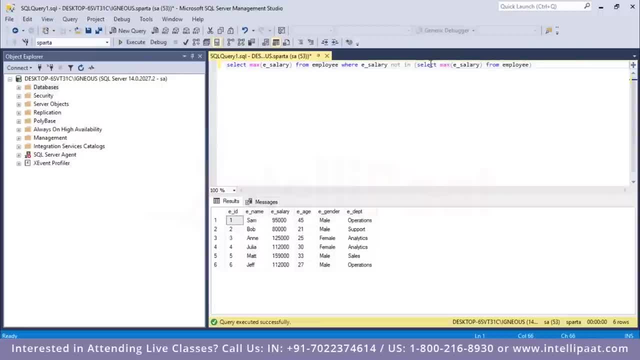 salary from employee and select max of e salary from employee. now this sub query would given this result, which is 159,000. so and then this main query would make sure that this salary does not lie in this. so this would give us the 125,000. 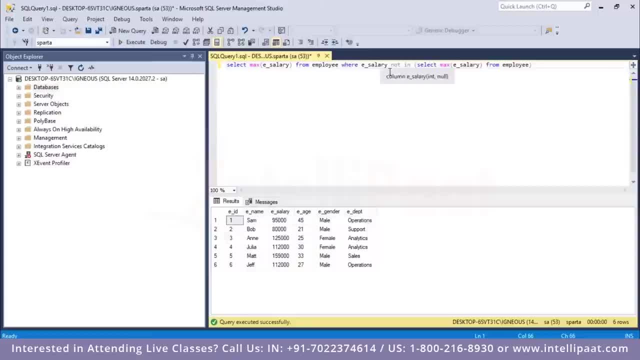 result. so select max of e salary from employee where e salary is not in 159,000. that would mean 125,000, so let me click on execute right. so we have successfully got the result, which is 125,000, and this is how we can extract the second highest salary. so we 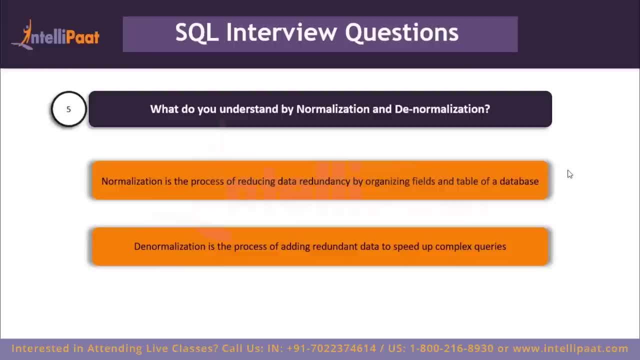 have our next question over here. so what do you understand by normalization and denormalization? so this is a question which is very frequently asked during the interviews, so let's get to the answer. so normalization and denormalization are basically methods used in databases, and normalization is: 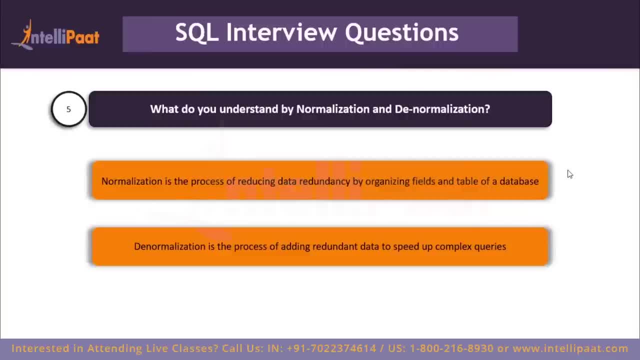 the process of reducing data redundancy and dependency by organizing fields and tables of the database. so it involves constructing tables and setting up relationships between those tables according to certain rules, and the redundancy and inconsistent dependency can be removed using these rules in order to make it more flexible. so I am repeating it again, guys. so simply put. 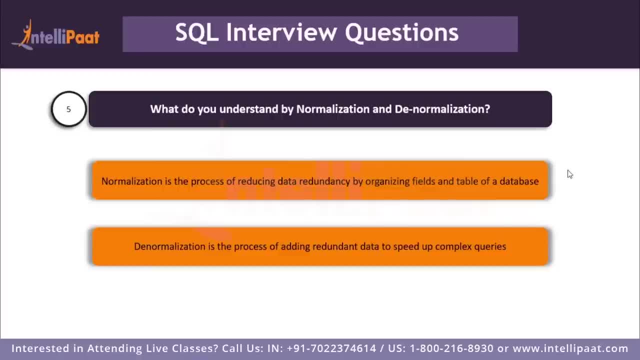 normalization is the process of reducing the data redundancy, and we are able to do this by organizing the fields and tables of the database. and then we have denormalization, which is a contrary process to normalization. so in denormalization we basically add redundant data to speed up complex queries involving multiple table joins. so in 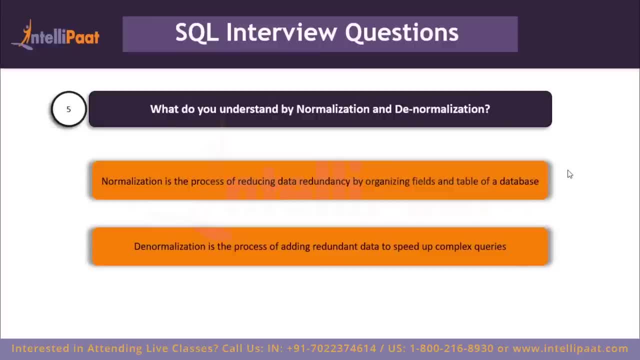 denormalization. we attempt to optimize the read performance of a database by adding redundant data or by grouping the data right. so this is our next question. now we are supposed to find out what exactly is wrong with the sequel query. so this is the sequel query over here. select gender average of age from: 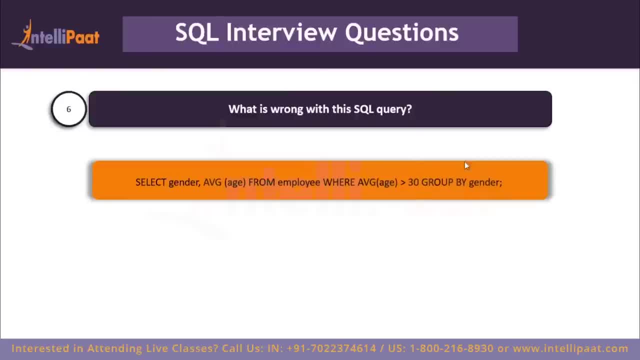 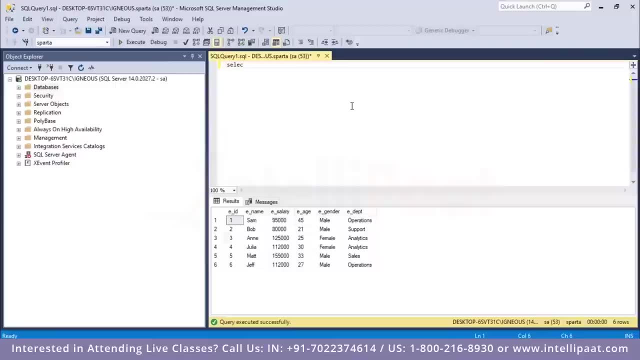 employee where average age is greater than 30. and again, this is the same same. we are grouping this with respect to gender. so this is our employee table over here. now let me go ahead and just type in the command which would be select e gender, and then I would want the average of age. so, average of e age. 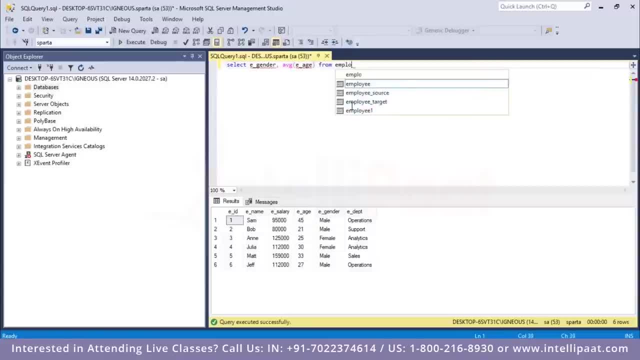 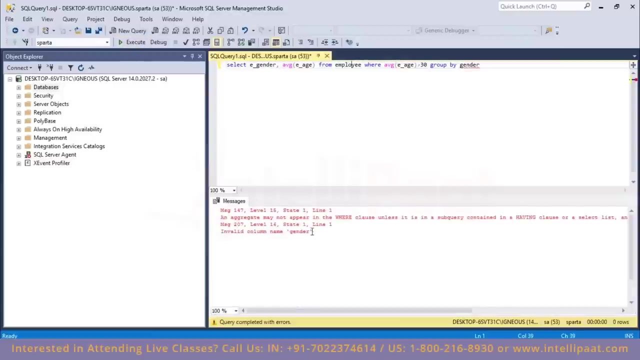 from the name of the table is employee, where, again, the average of e age needs to be greater than 30, and this is being grouped with respect to gender. now let me go ahead and click on execute. so let's see what is the error. so this warning message states that an aggregate may not appear in the where clause unless 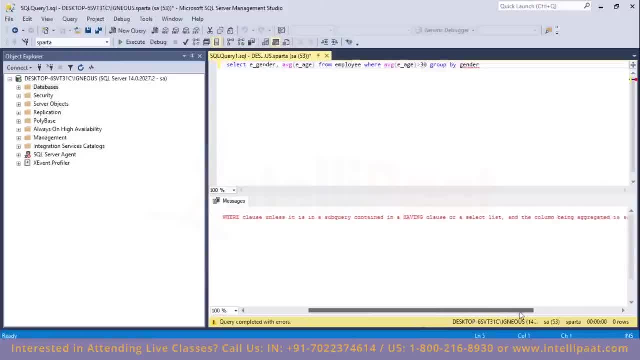 it is in a sub query contained in a having clause or a select list, and the column being aggregated is an outer reference. so this basically means that whenever we are working with aggregate functions and we are using group by aggregate, we are using group by the subquery and we are using group by the. 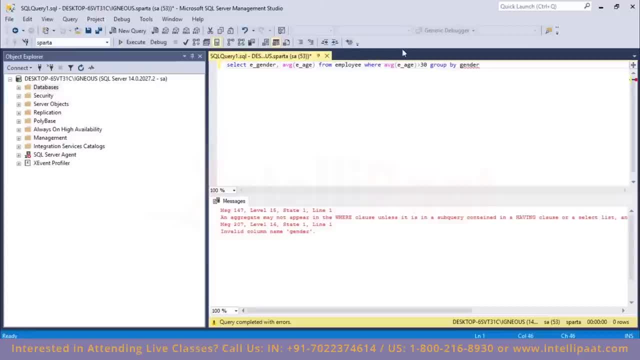 we can't use the where clause, so instead of the where clause, you would have to use the having clause. now let me change this to having and let me click on execute. so now again we get an error over here, and this error says that incorrect syntax near the keyword group, and this is because, if we are using the 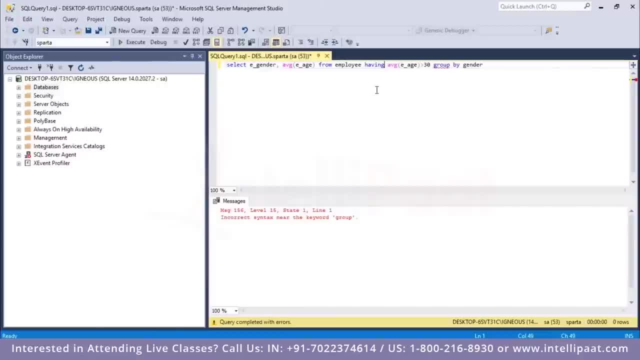 having clause, then group by would come first and having would come second. now let me cut this over here and let me paste this before having. alright, now I click on execute. so this has to be EGender over here. now we successfully got the result. so just to reiterate. the other was: wherever we are working with aggregate functions. 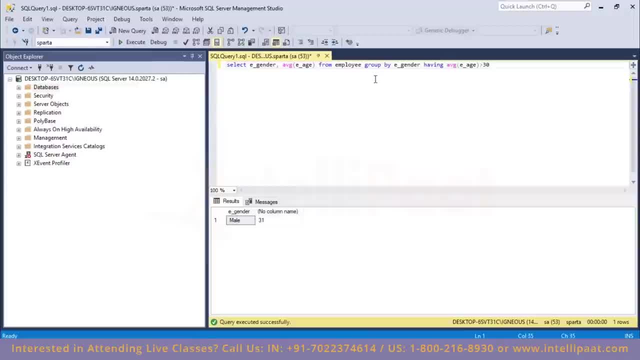 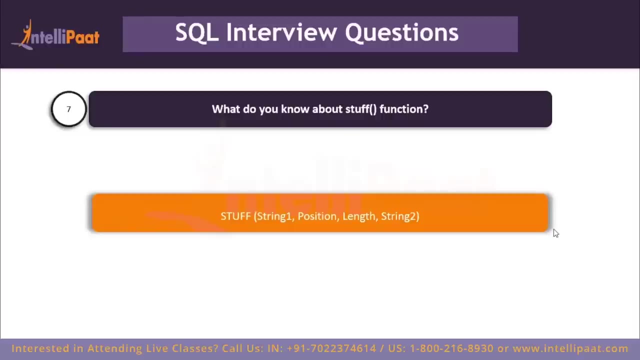 we cannot use the where clause and we would have to use the having clause. and if you are also using a group by with having, then group I would come first and having would follow it. so next question: so what do you know about the stuff function? The stuff function deletes a part of the string and then inserts another part into the string. 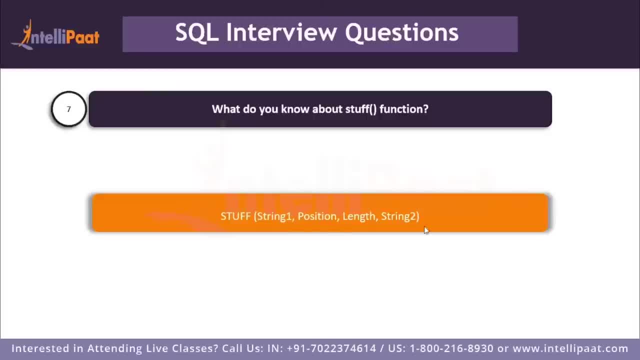 starting at a specified position. So this is the syntax of the stuff function. So stuff this takes in these four parameters: string one, position, length and string two. So the string one is basically that string which would be overwritten position would. 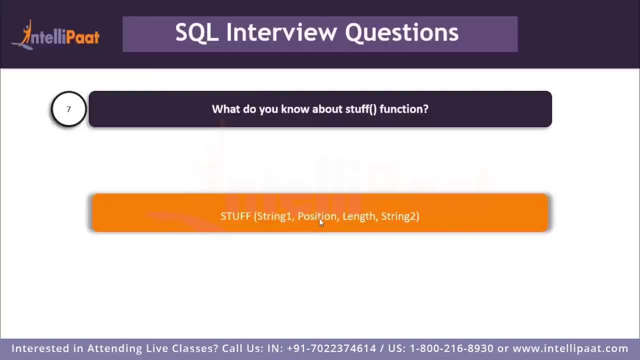 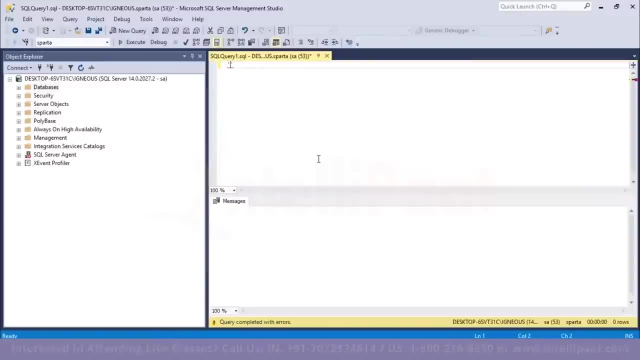 basically indicate the starting location for overwriting the string, and length is the length of the substitute string and string two is that string which would overwrite the string. So again let's go to SQL server and work with an example with the stuff function. So now let's say I have this string which basically stands like this: SQL tutorial. 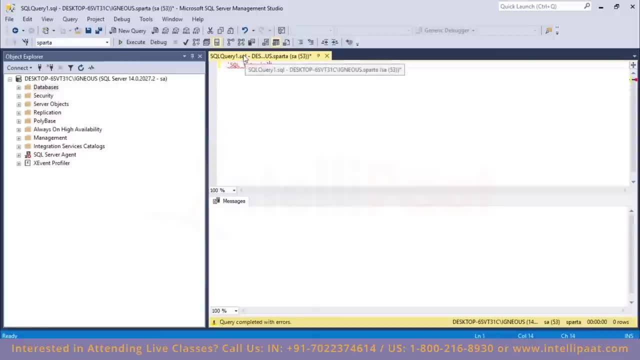 Now I'd want to replace this SQL tutorial with Python tutorial, right? So for this purpose we can actually use the stuff function. So let me go ahead and write the syntax for that. It would be select. I'll give in the function stuff. 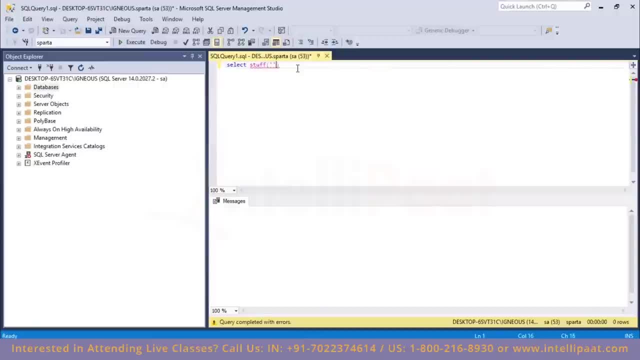 So let me start with the first parameter, which is the string which is to be replaced. So the string which is to be replaced is SQL tutorial, And then I'll give in the second argument, which is the position. So the position would be one, that is, I want to replace this. 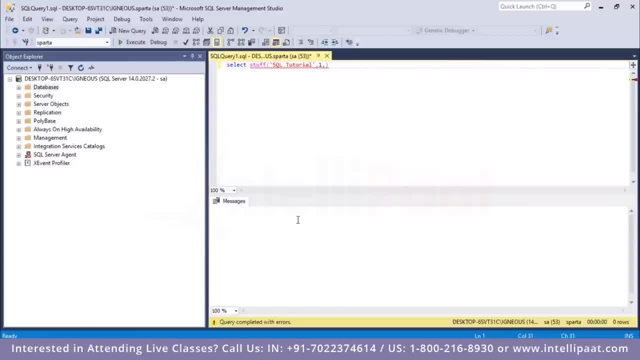 So this is position number one, And then I would have to give in the length of the string which is substituted right. So the length of SQL is three. I'll just type in three over here And then, finally, I will give in string two. 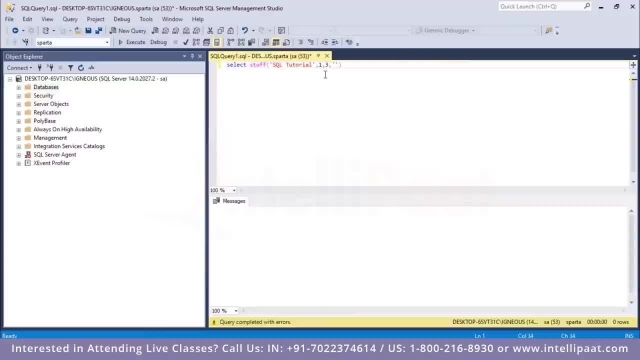 Which is basically that string which would replace this over here. So I would type in Python over here. Now I'll execute. So initially our string was SQL tutorial and with the help of the stuff function, you were able to change this from SQL tutorial to Python tutorial. 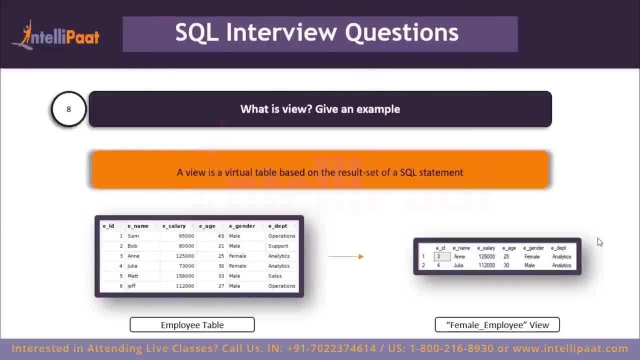 So next up, we'd have to explain about views in SQL- So what exactly is a view? And then we'd have to give an example of you, So you can consider views as virtual tables, which are used to limit the information that we want to display. 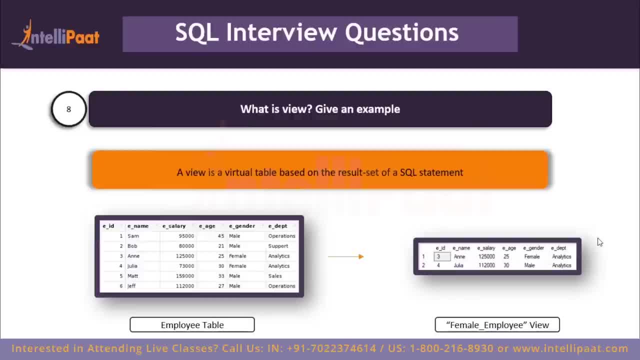 And these are actually nothing but the result of an SQL statement, which have a name associated with them, And since views are not virtually present, it takes less space to store. So let's take this example from this employee table. Let's say we wanted to perform multiple operations on the records where the gender is female. 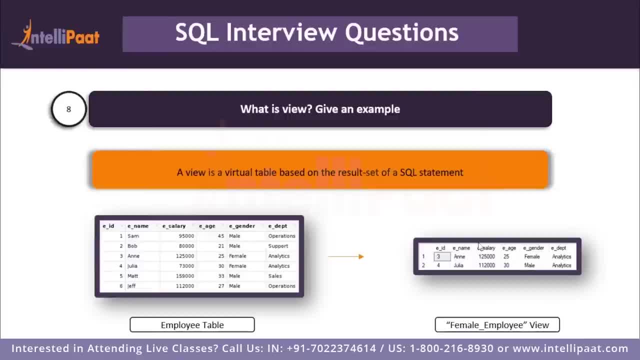 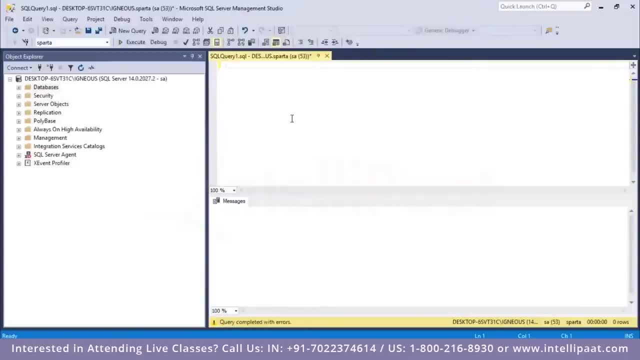 So we can create a view only for the female employees from the entire employee table. So let's go ahead and perform this in SQL server. Now let me type the syntax for this. So I would want to Create a view which would comprise of only the female employees from the entire employee. 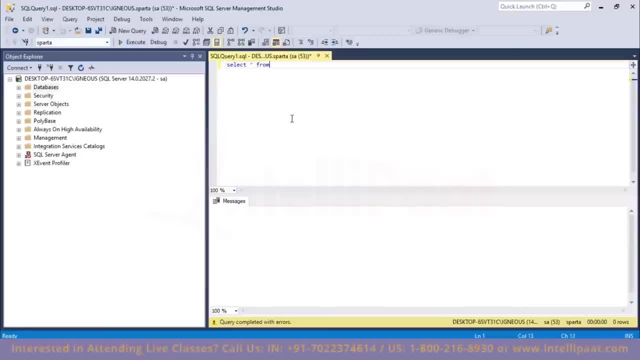 table. Now let me just have a glance at the employee table first. So select star from employee. Now I would want a view which would comprise of just these two records. Now let me go ahead and write in the syntax for the view. 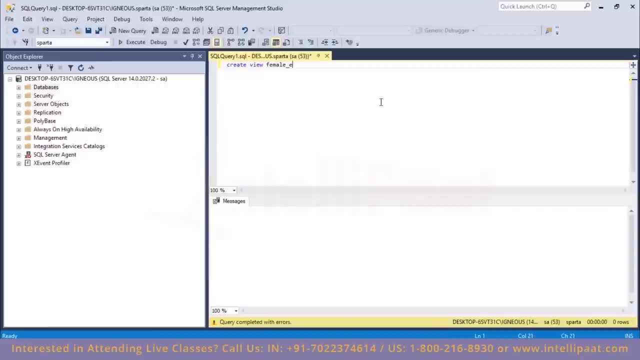 So it'd be create view and the name of the view would be female employee And after this I will given the keyword AS. After that I'll type in select and then I'll given the condition. So select star from employee where. after the where clause, I will given the condition. 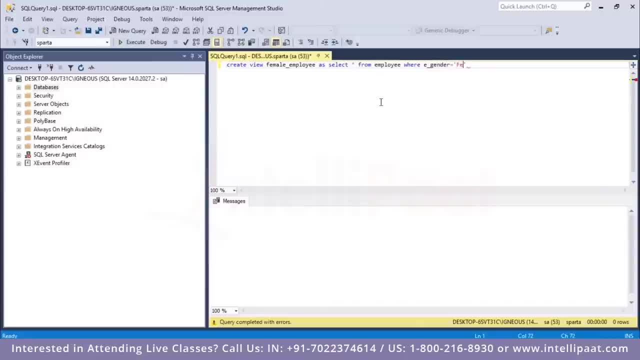 which actually matters. So gender needs to be equal to female Right. So I've successfully created this view with the name female employee, which would comprise of only the records of the female employees. Now let me delete this and let me have a glance at the view which I've just created. 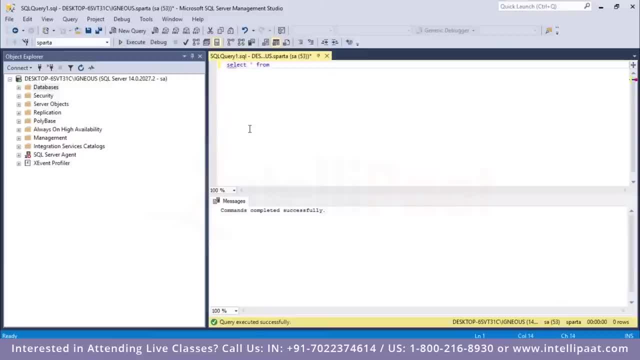 So I've successfully created this view with the name female employee, which would comprise of only the records of the female employees. So I've successfully created this view with the name female employee, which would comprise of only the records of the female employees. Now let me delete this and let me have a glance at the view which I've just created. 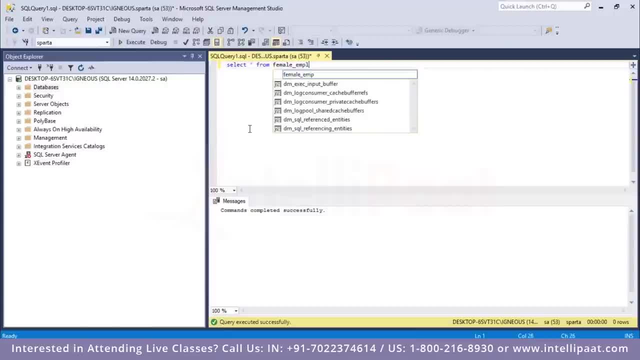 So select star from female employee Right. So this is our view, which comprise of these two records, and the names of the employees are Ann and Julia. Now, similarly, let's say, if I wanted, a view which would comprise of only those employees whose age is greater than 25.. 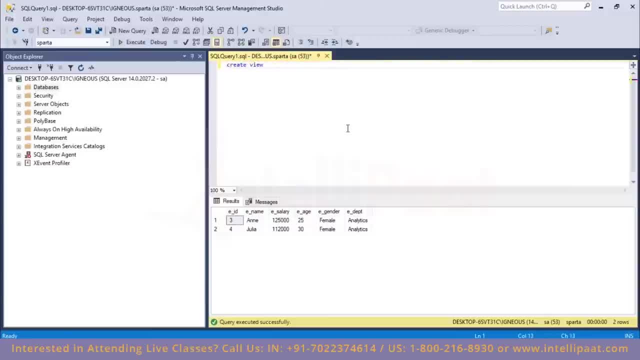 So let me go ahead and write the syntax for that. So create view. and then let's say the name of the view is H, And then I'll type in the keyword AS: select. now over here let me give in the statement: So select star from employee where. and then the condition would be: E, age needs to be greater. 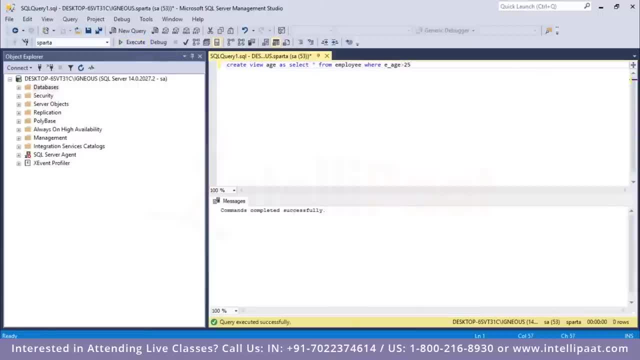 than 25.. So we have created this view. Now let me have a glance at this. So select star from age Right. So this is a view which would comprise of only those records where the age of the employee is greater than 25.. 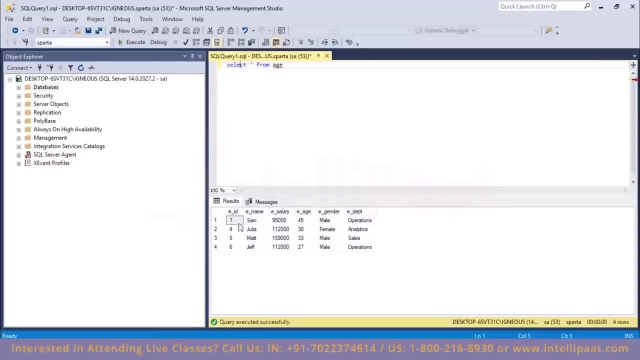 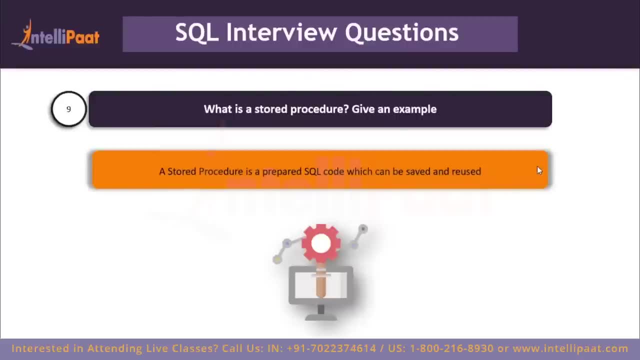 And we've got four records over here: Sam's age is 45, Julia's age is 30, Matt's age is 33 and Jeff's age is 27.. Right, So what is a stored procedure? And then we'd have to give an example of stored procedure. 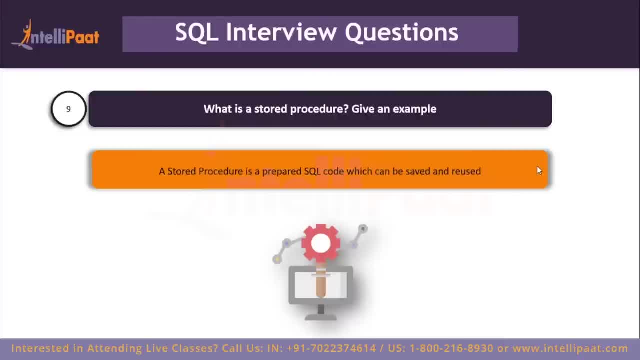 So a stored procedure is a prepared SQL code which can be saved and reused. Or in other words, you can consider a stored procedure to be a function consisting of many SQL statements. For example, you can consider a stored procedure to be a function consisting of multiple SQL. 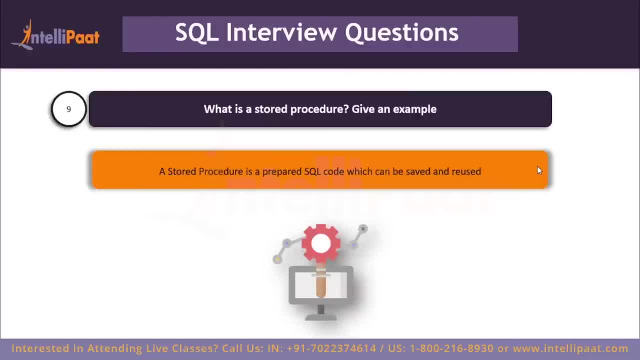 statements to access the database system. So we can consolidate several SQL statements into a stored procedure and execute them whenever and wherever required. And stored procedure can be used as a means of modular programming, That is, you can create a stored procedure once, store and call for several times whenever. 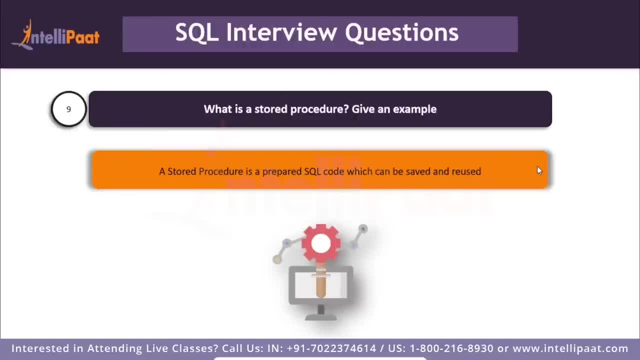 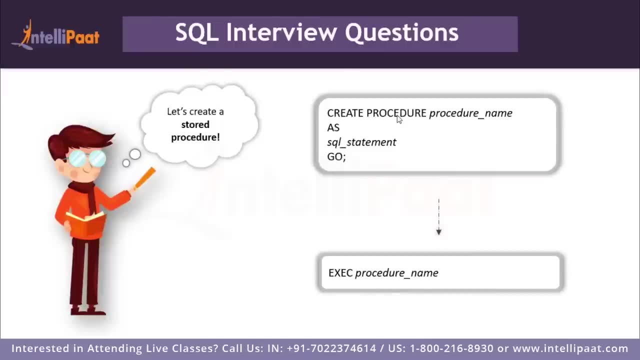 required. So this supports faster execution when compared to executing multiple queries. Now let's look at the syntax of a stored procedure. So well, given the keywords create procedure, And then we'll give the procedure name over here. After that we'll give in the keyword ES and then we'll give the SQL statement for which. 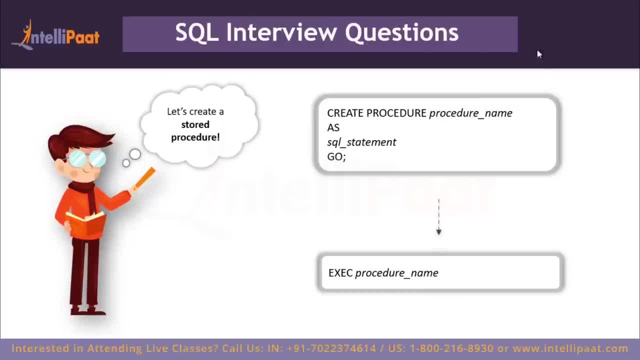 we'd want to create the procedure And then we'll end the procedure with the go keyword. Now, after we create a procedure, we need to execute it. So this is the syntax to execute the procedure. So we'll type in EXEC and then give the name of the procedure which is to be executed. 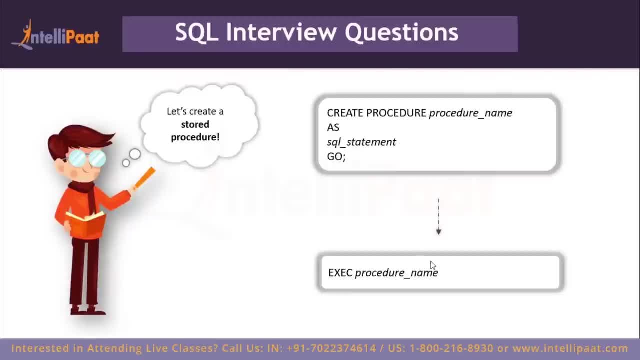 Right. So again, let's have an example with the stored procedure. So now I'm going to create a stored procedure which would help me to extract the EXEC from the stored procedure. This will help me to extract the age of the employees in a very easy way. 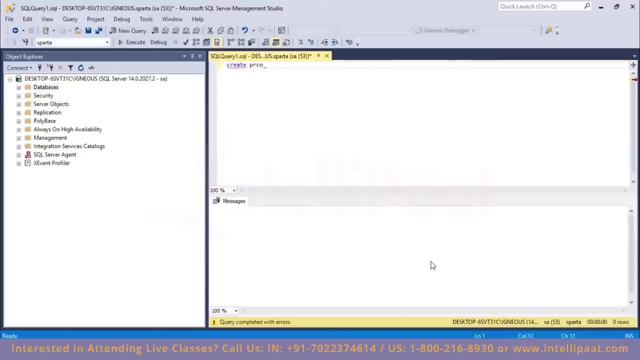 So let me type in the syntax for that create procedure, and then I'll give in the name of the procedure. So this would be employee age. After this, I will type in the keyword ES and then I'll give in the select statement. 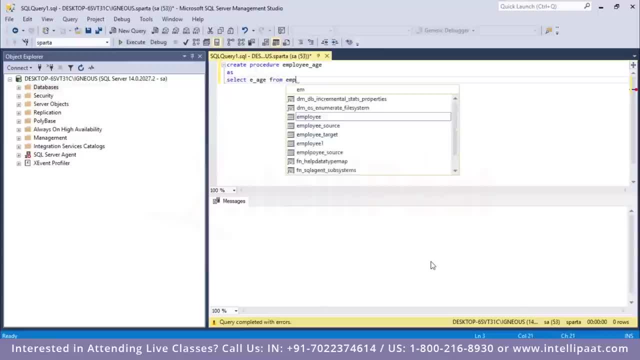 So select EH from employee. Now that this is done, I'll give in the go keyword Right. So now I have successfully created the stored procedure with the name employee age, Now I'll go ahead and execute this. So it'll be: EXEC or execute- employee age. 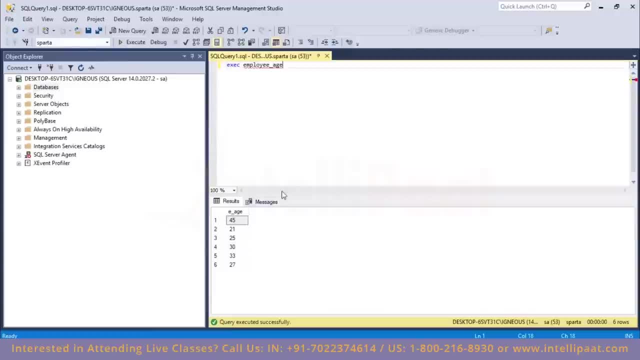 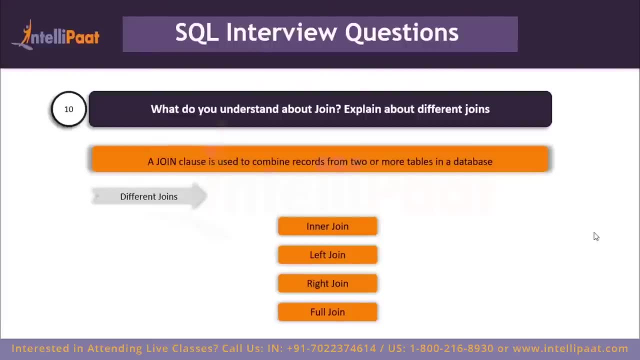 Right, So we have created the stored procedure which would help me to easily access the age column from this employee table. So next question: what do you understand about join and explain about different joins? So what do you understand about join and explain about different joins? 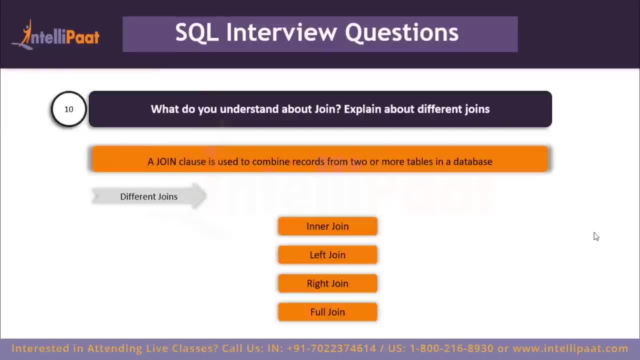 So a join clause is used to combine rows from two or more tables based on a related column between them. So there are various types of joins which can be used to retrieve data and it depends on the relationship between tables. So first we have inner join, which basically returns records that have matching values. 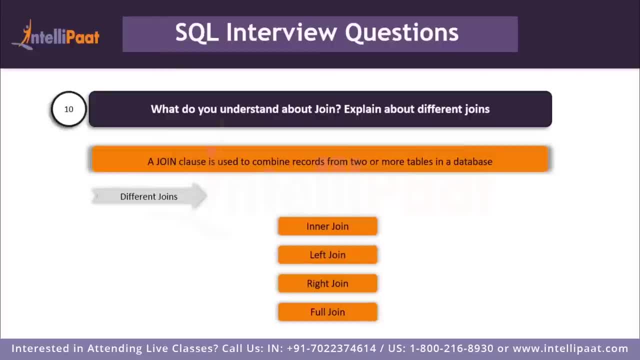 in both the tables. Then we have left join. So left join returns rows which are common between the tables and all rows of the left hand side table. That is, It returns all the rows from the left hand side table even though there are no matches. 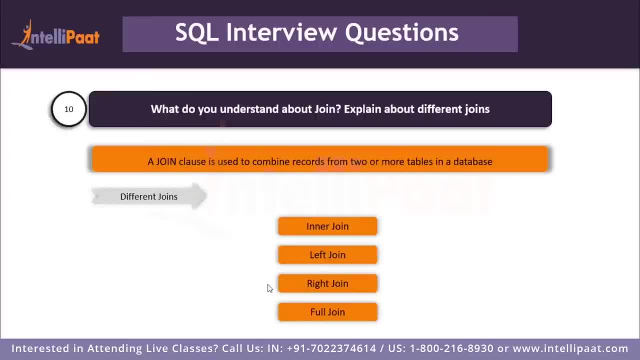 in the right hand side table. Then we have right join. So right join returns rows which are common between the tables and all the rows of the right hand side table. That is, it returns all the rows from the right hand side table, even though there are. 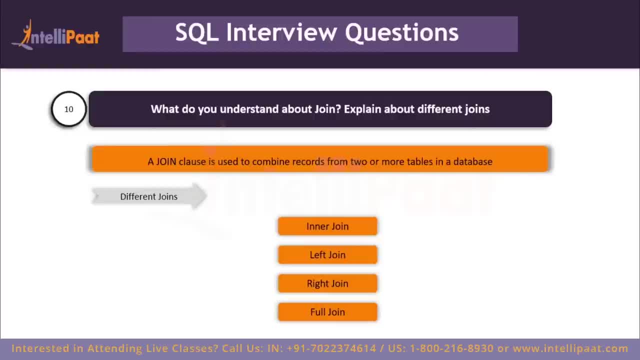 no matches in the left hand side of the table And finally we have the full join. So full join returns all rows from the left hand side table and all the rows from the right hand side table. So now we'll have to explain about inner join properly. 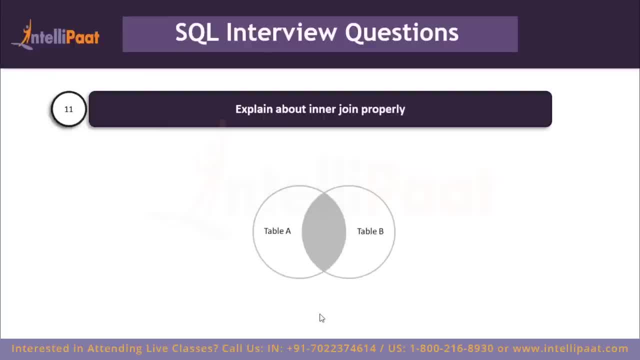 So the inner join basically gives us those records which have matching values in both the tables. So we've already learned this. Now let's say we have two tables, table A and table B, And when we apply inner join on these two tables, we'll get only those records which are common to both table A and 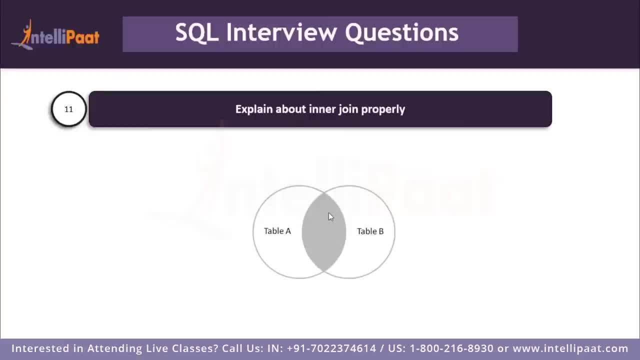 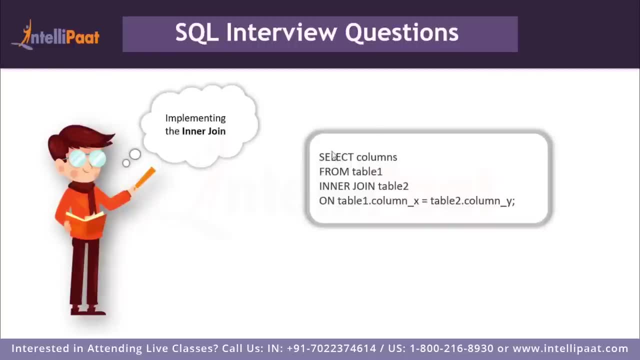 table B, So this grey portion which you see over here. So this would be the result of the inner join. Now let's look at the syntax of inner join. So we'll give the keyword select and then we'll give in the list of the columns following: 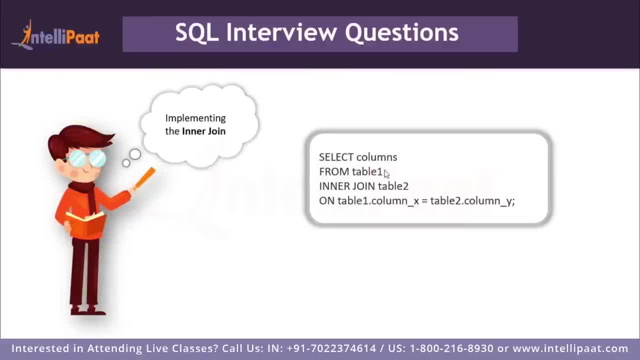 which we'll give the from keyword and then we'll give the name of the first table. Then we'll use the keywords inner join and then give the name of the second table, After which we'll give in the on keyword. So this on keyword tells SQL that this inner join needs to be done on some condition. 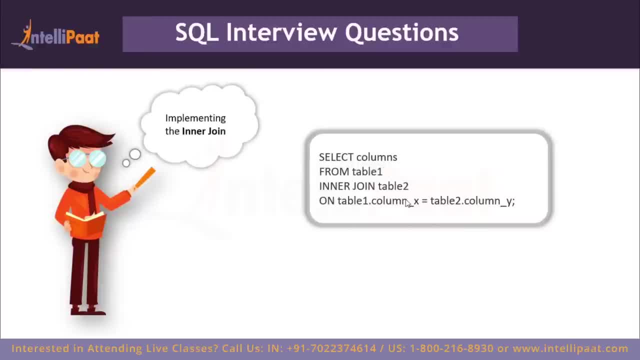 And the condition over here states that the values from column X of table one. So the values from column X of table one Should be equal to the values of column Y from table two. Let me just retread this: The values of column X from table one should be equal to the values of column Y from table. 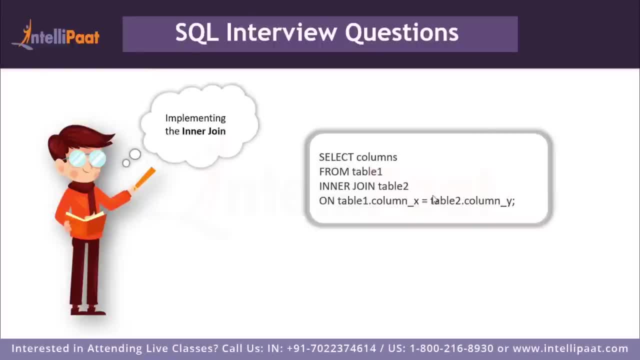 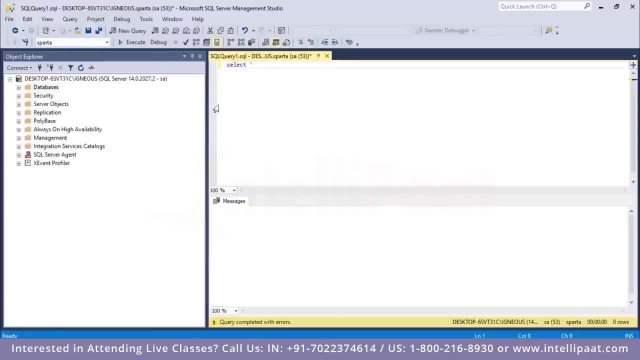 two. Now let's go to SQL server and work with this inner join. So I have two tables over here. So the first table would be the employee table and the second table would be the department table. So let me have a glance at both of the tables. 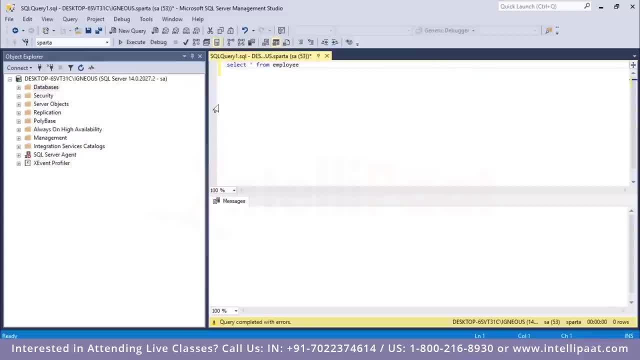 So select star from employee. Now The second command would be select star from department. So this is the employee table over here, which we've already seen, And then we have this department table. Now I'd want to have an inner join on both of these tables, where the EDPT column from? 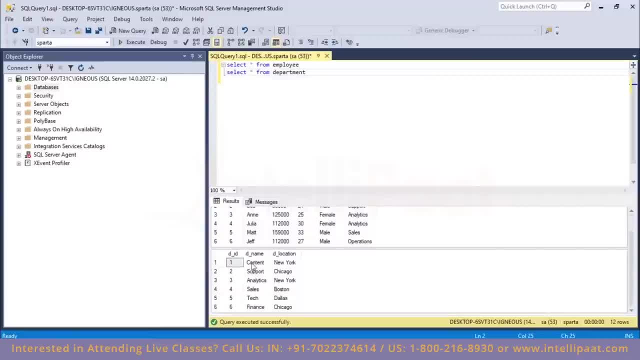 this table is equal to the D name column from this table, That is, wherever the values from these two columns match. I'd want only those records. Now let me go ahead and write the syntax for this, So I will type in select and then I'll give in all of the columns which I want. 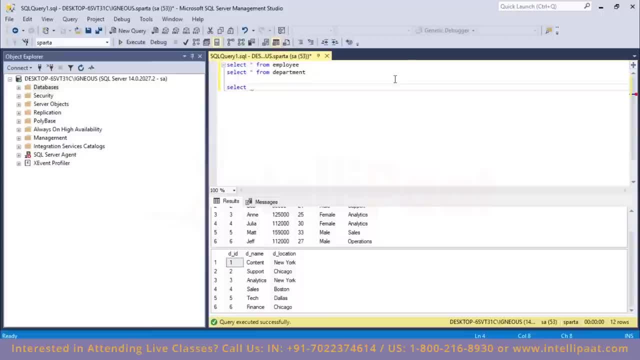 So I want the E name column and E department column from the employee table. So this would be employee dot E name. Then I would want employee dot E department. of that I would want the department name and the department location from the department table. 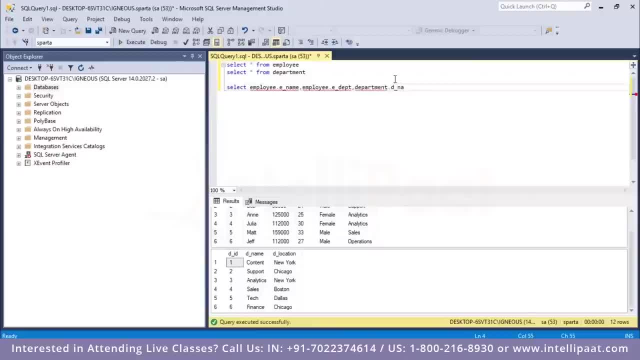 So I'll type in department dot D department, Okay, D name, And then I also want department dot D location, right? So these are all of the columns which I want from both the tables. Now, after this, I'll type in from, and then I will type in the name of the first table. 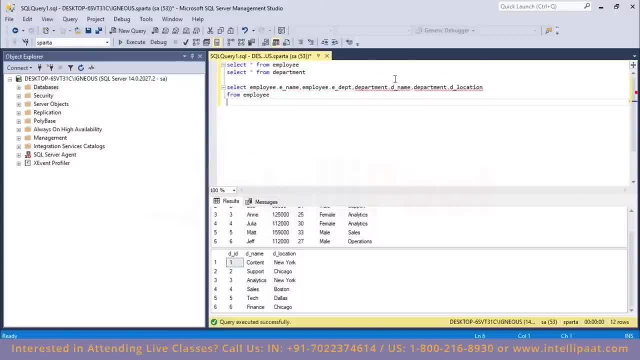 which is employee, And then I'll just type in inner join and then, given the name of the second table, which would be department, Then I'll give in the on keyword And then given the condition. So here the condition is the values of the D name column should be equal to the values. 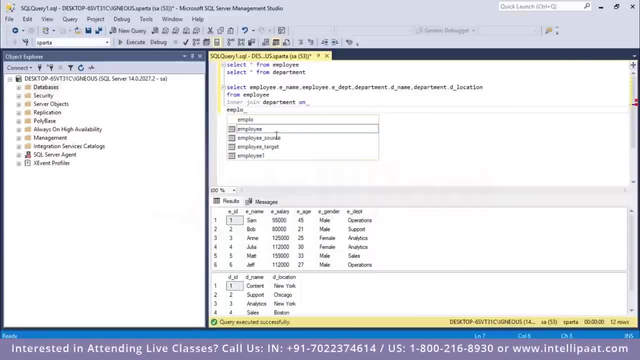 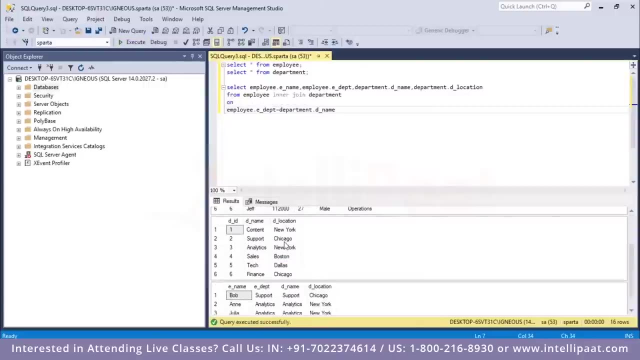 of the E, D, E, P, T column. So employee dot E name should be equal to department dot D name. Now I'll execute this right. So this is the result. So we have our employee table over here. This is the department table. 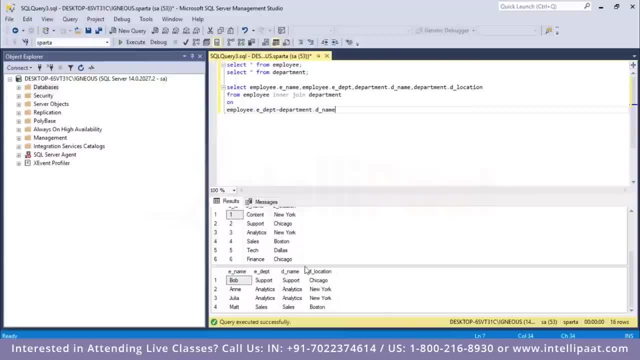 And finally, this is the result of the inner join. So here we see that we've got only those records Where Departments match in both of the tables. So the match departments are support, analytics and sales, right. So you've got support, analytics and sales from over here, because only those departments 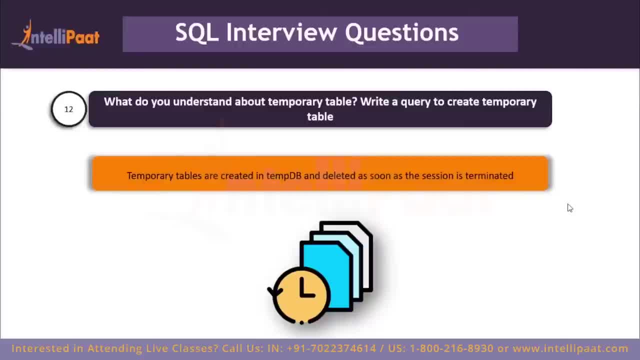 are present in this department column. So next question: well, what do you understand about temporary table? And then we'd have to write a query to create a temporary table. So, simply put, temporary tables basically help us to store and process the intermediate results. 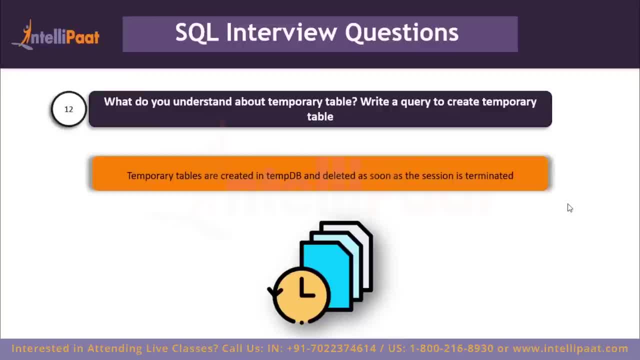 Now these temporary tables are created in the temp DB And are automatically deleted when they are no longer used. So the temporary tables could be very useful in cases where we need to store temporary data. Now let's look at the syntax of a temporary table. 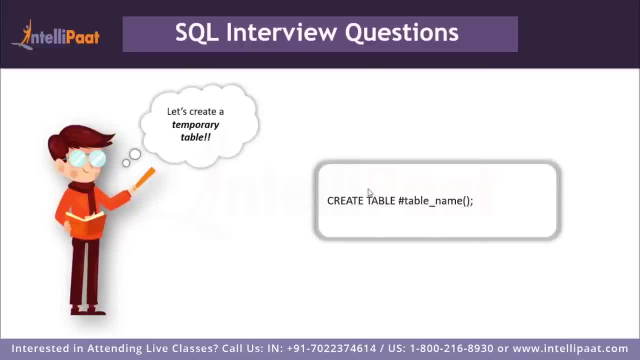 So first we will, given the keywords create table, And before we go ahead and give the name of the temporary table, we'll have to proceed it with a hash. So again, let's go ahead and create a temporary table. So now what I'll do is I'll create a temporary table. 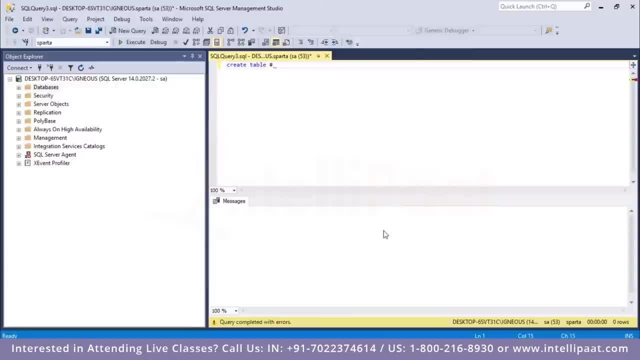 And I will name this as temporary table And I will name this as temporary table And I will name this as temporary table. Let's see book. And then before the name of the table, I'd have to proceed it with a hash. 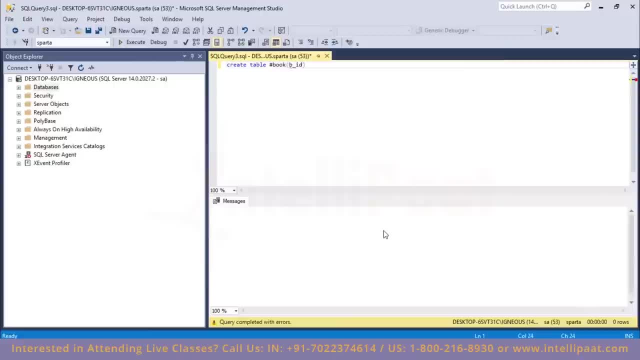 Right now, this would have two columns of: first would be the book ID, and this would be of integer type, And then this would have book cost, which is again of integer type. Now let me execute this Now. I'll refresh over here. 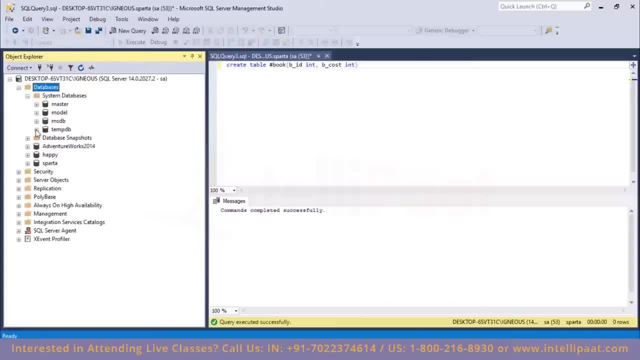 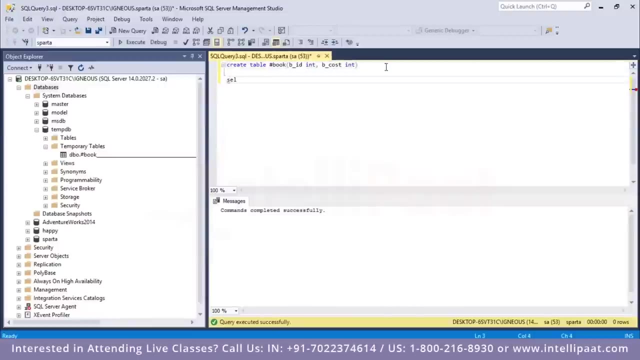 I'll click on the plus sign, I'll go into system databases and I'll go into temp DB over here. let me click on the temporary table so we see that we have successfully created this temporary table with the name book. now let me see what is present in this table, so i'll type in. 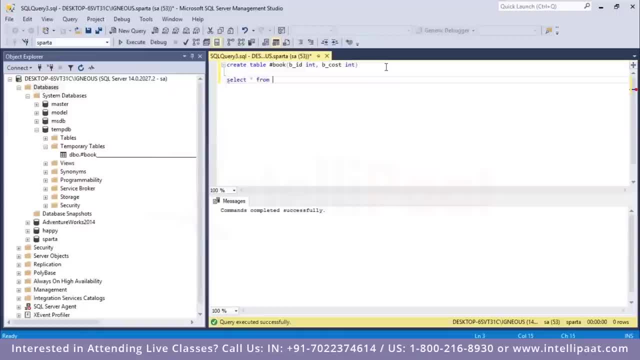 select star from. i'll put in the hash symbol over here and then i'll give in book right. so as of now, this temporary table is empty. now let me go ahead then insert something into this table. so the command would pretty much be the same. so insert into and then. 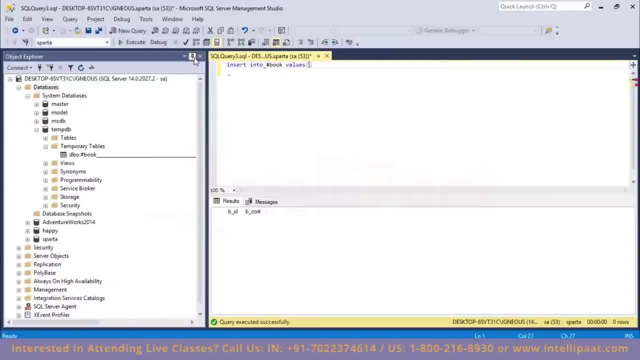 lb book. i'll type in values over here. so the only difference which you see when you're creating or working with a temporary table and the normal tables is you would have to precede the name of the table with the hash. so as simple as that. rest everything would be the same. and over here, let me. 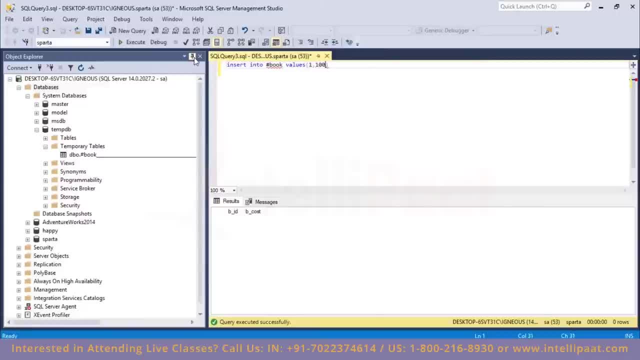 give in the values. so the book id is one and the book cost us hundred. right now let me also add another record. so the second id would be two and now the book cost would be, let's say, 232. all, right now let me have a glance at this modified temporary table. so select star from hash. 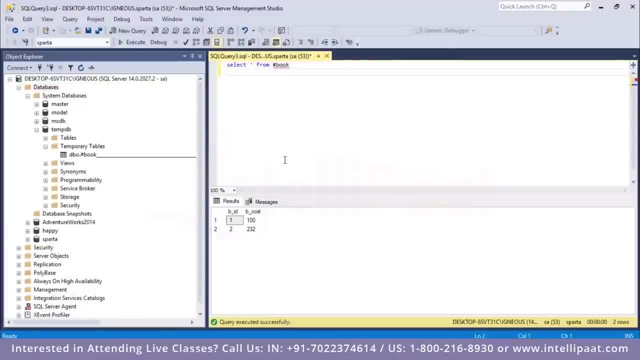 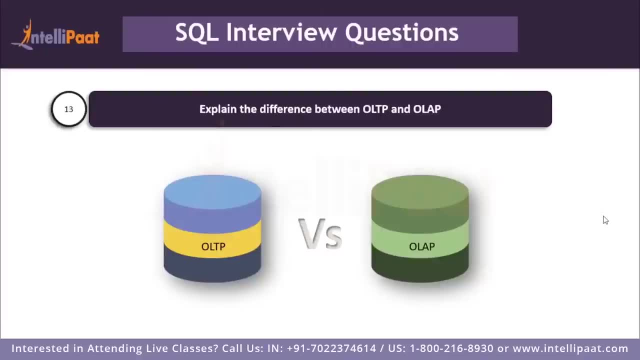 book right, so we have added two records into this temporary table. so now we'd have to explain the difference between OLTP and OLAP, so let's start with OLTP. so OLTP basically stands for online transaction processing, and you can consider it to be a class of software applications capable. 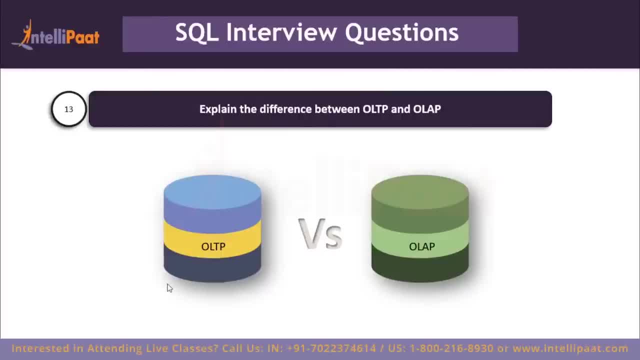 of supporting transaction oriented programs, and an important attribute of an OLTP system is its ability to maintain concurrency. so OLTP systems often follow a decentralized architecture to avoid single points of failure, and these systems are generally designed for a large audience of end users who conduct short transactions and queries involved in such databases are generally 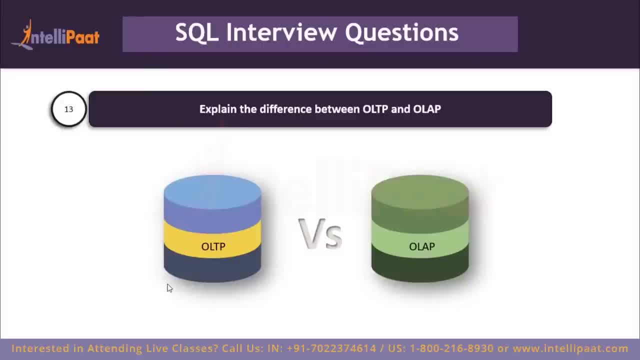 simple, need fast response times and return relatively few records, so the number of transactions per second acts as an effective measure for that systems. then we have OLAP. so OLAP stands for online analytical processing, and it is a class of software programs which are characterized by relatively low frequency of online transactions, so queries are often too. 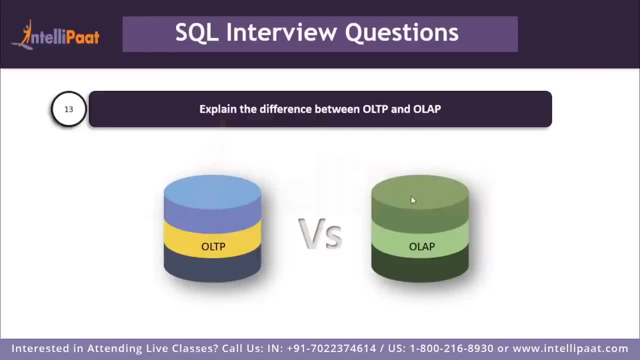 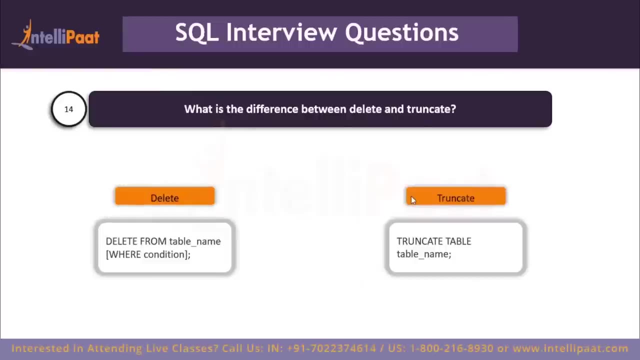 complex and involve a bunch of aggregations, and for OLAP systems, the effectiveness measure relies on response time. so such systems are widely used for data mining or maintaining aggregated historical data, and this is usually used in multi-dimensional schemas. so then we have the next question. so what is the difference between the delete and the truncate command? so again, keep. 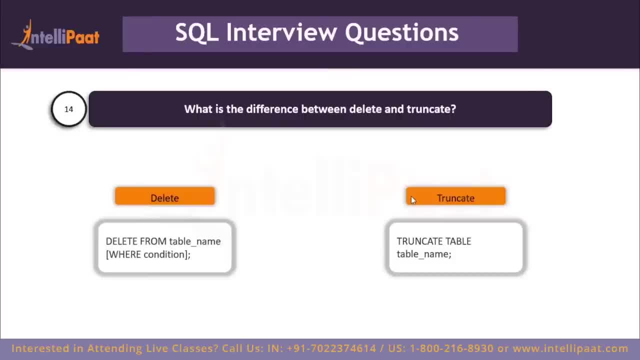 this in mind, guys, this is a question which is very frequently asked in interviews. so let's start off with the delete query. so the delete query is used to delete or remove one or more existing tables. so we'll start with the delete keyword and then we'll put in the keyword. from then we'll specify the. 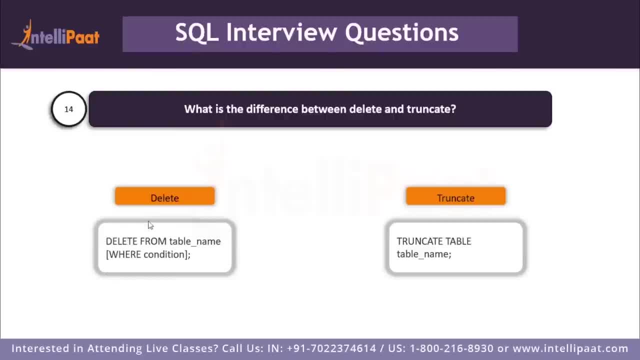 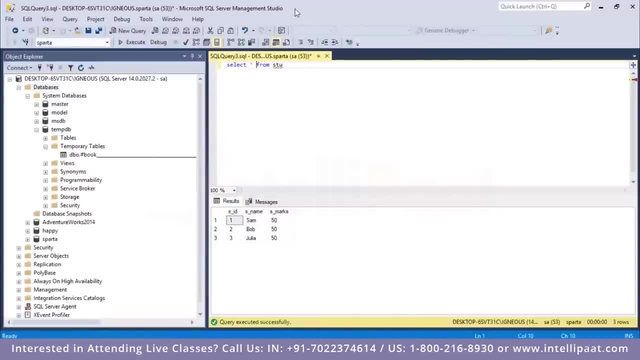 name of the table of that will specify the where condition, but then that's optional. so let's see an example of this delete command. so we have this table, so the name of the table is STU, which basically is the student table. now from this table I don't want to delete the record where 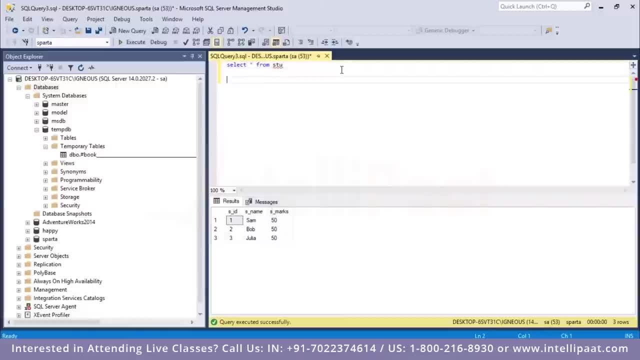 the name of the student is Bob, so let me write the syntax for that. so delete and then delete from, and then I'd have to give in the name of the table. so the name of the table is STU, so delete from STU. after that I'll given the where clause and give the condition where S name is equal to. 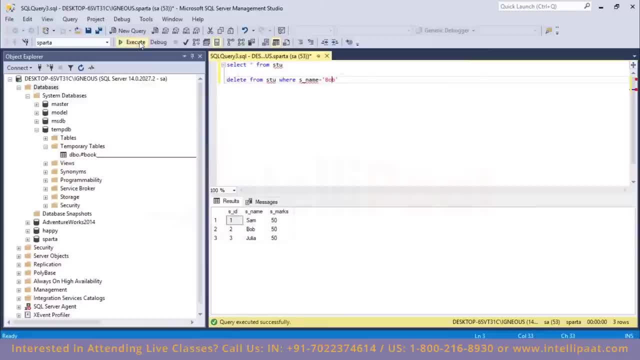 Bob. let me execute this right. so we have successfully deleted that record from this table where the name of the student was Bob. so similarly, let's say, if I want to delete that record where the student ID is, it's over here. the condition will change. so delete from STU where S ID equals three. so now this time. 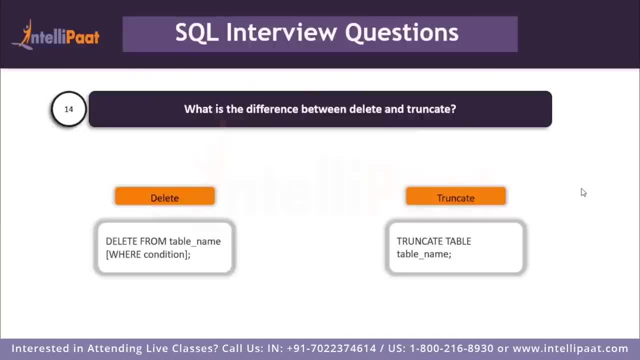 we have deleted that record where the student ID was equal to three. now let's look at the truncate statement. so the truncate statement deletes all of the data inside the table. so here we'll given the keywords truncate, table and then give the name of the table. so let's go to SQL server and 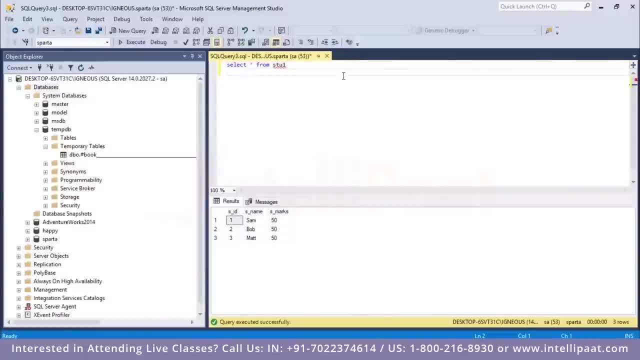 work with this truncate command. so now we have this two one table. so let me go ahead and create and use the truncate command of this table. so I'll type in truncate and then I'll given the name of the table, which would be STU one. so before that I'd have to type in tables of truncate table. 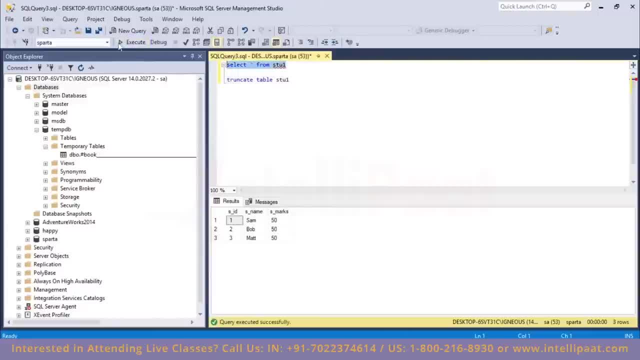 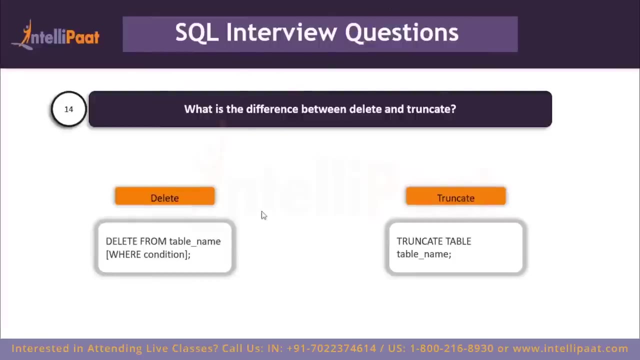 STU one. let me run this right. so we have deleted all of the records from this table, right? so this is how the truncate command works. now let's understand some differences between the delete command and the truncate command. so, when it comes to the type of language truncate would, 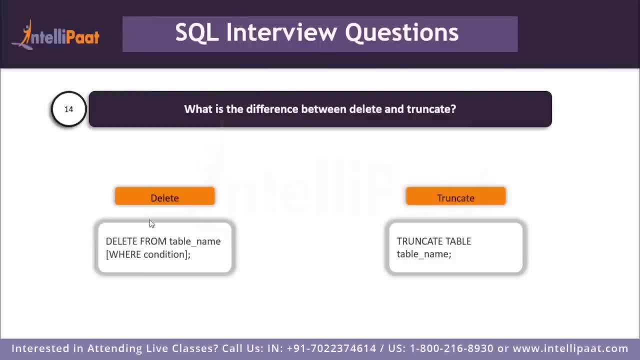 be your DDL command or a data definition language command, and delete is a DML command or a data manipulation command. now, another difference would be we can't really execute a trigger in case of truncate, while with delete we can accomplish a trigger now also if our table is different by 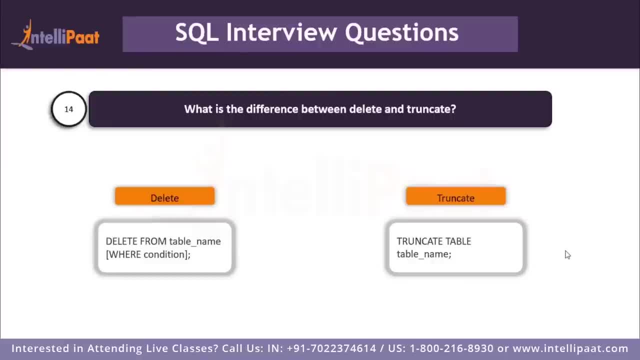 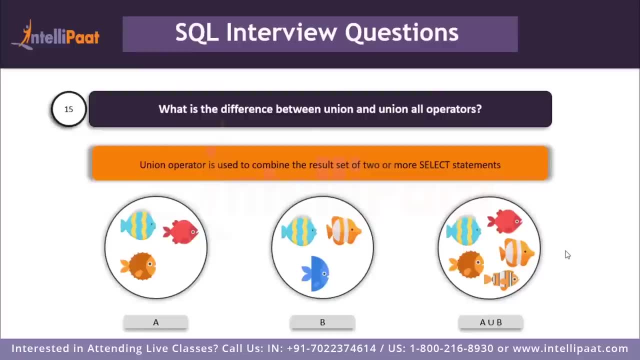 any foreign key constraints, then truncate won't work. so if you have a foreign key then you'd have to delete and you wouldn't be able to use the truncate command. so next question: what is the difference between union and union all operators? so the union operator is used to combine the 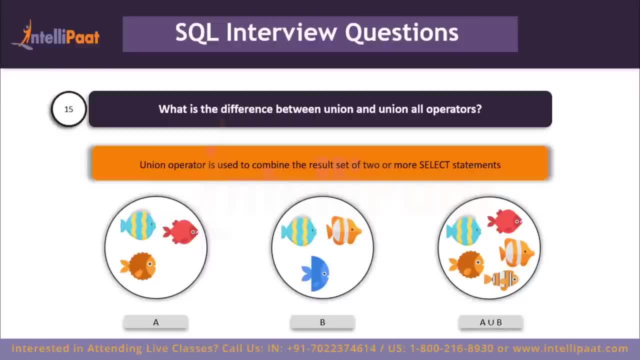 result set of two or more select statements. for example, if the first select statement returns these three fish and the second select statement returns these three fish, then the union operator would return the result of these two select statements and if there is a record which is tables, we'll get only one of them in the final result. So here we see that this 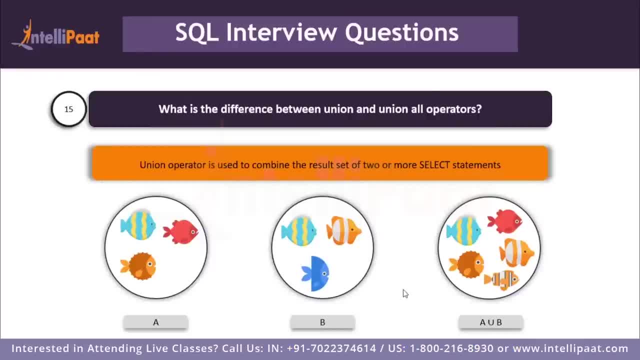 blue fish is present in both the tables A and B. Now when we apply the union operator on these two tables, the final result of A union B would have only one of these blue fish, And this is the syntax of the union operator. So we'll. 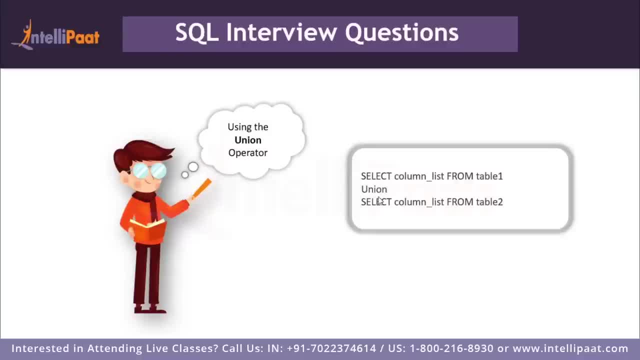 give the first SELECT statement. after that we'll give in the union operator, following which we'll give the second SELECT statement. Now you also need to keep in mind that the number and the order of columns must be same in both the SELECT queries. So let's work with this union operator now. So we have these. 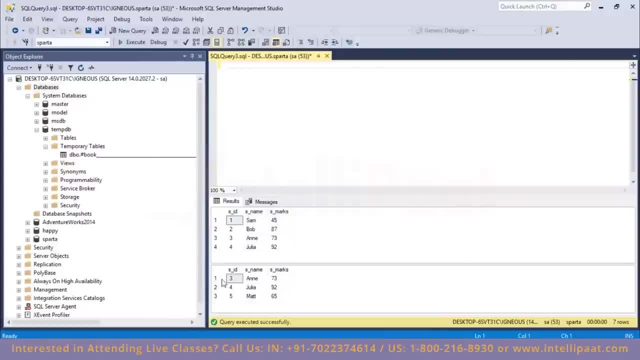 two tables over here. So the name of this table is student details 1 and the name of this table is student details 2.. And if we have a glance at the columns, we see that both of the tables have three columns and the names of the columns are: 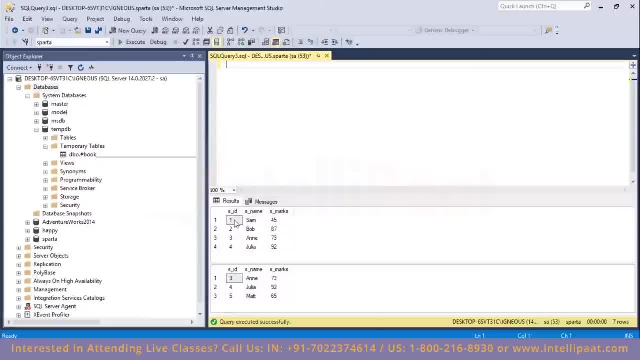 same and also the order of the columns are same. So here we have SID SNAME and DESMARKS. Similarly, over here we have SID SNAME and DESMARKS. Now let's go ahead and apply the union operator on this. So I'll type in the first SELECT statement. So 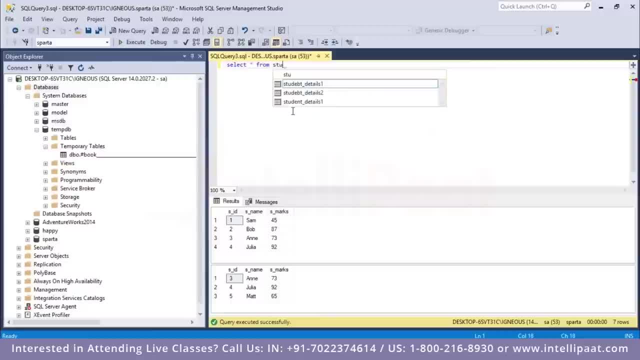 it'll be SELECT star from student details 1.. So let me change the spelling to student details. After this I will apply the union operator and then give in the second SELECT statement. So SELECT star from student details 2.. Now let me click on execute. So this is the result over here. Now let me also print: 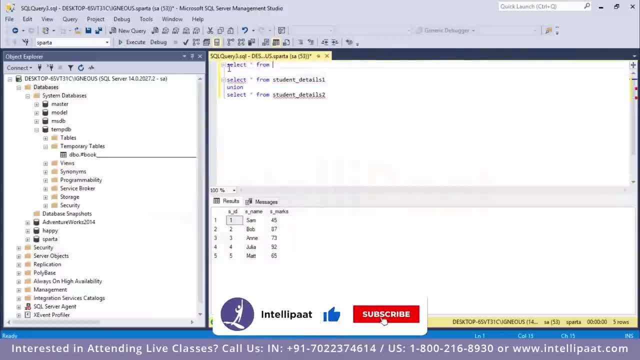 in the first two original tables. So SELECT star from student details 1, and then I'll also put in SELECT star from student details 2.. So let me just change the spelling to student over here. Let me also change this over here. So this will: 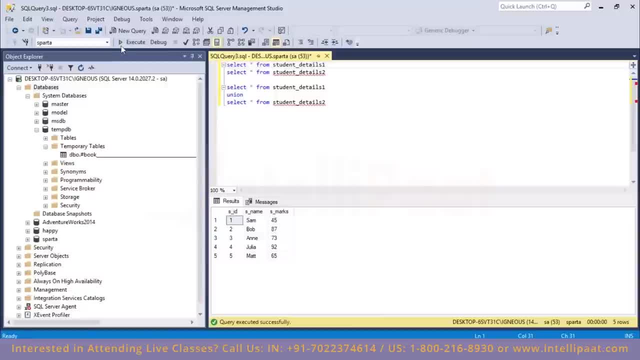 be student right. So this is student details 1, this is student details 2 and this is the result of the union operator. Now, if you have a glance at these two tables, then you see that these two records are repeating over here, right? So there's Ann and Julia over. 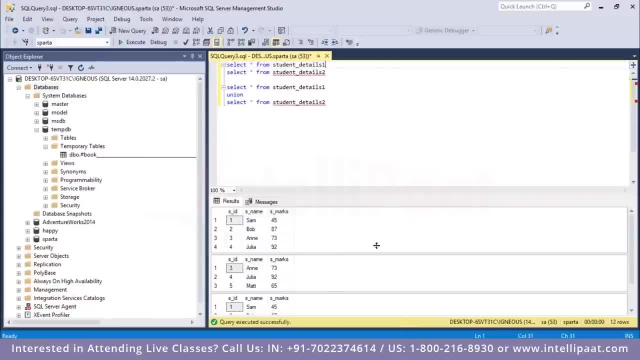 here in the first table and there's also Ann and Julia in the second table. Now, when we apply the union operator, then we'll just have one record coming from each of these tables, Right. So we've got Ann over here, we've got Julia over here, and then we have finally, 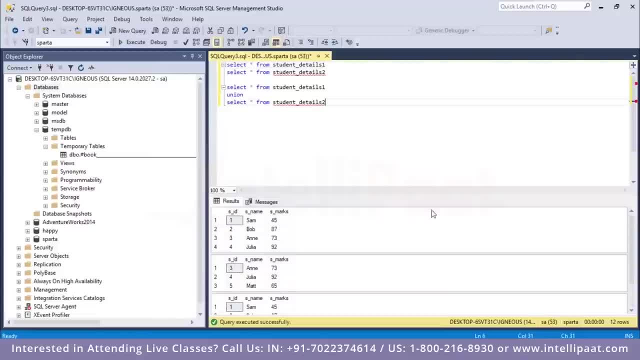 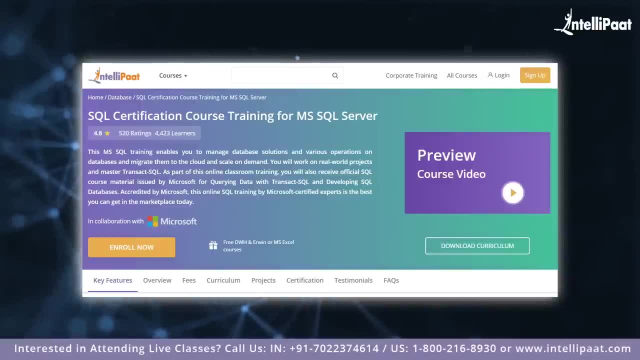 have Matt, which comes from the second table. This is how the union operator works. Just a quick info, guys. Intellipaat provides SQL online training in partnership with Microsoft and mentored by industry experts. The course link is given in the description below. Now, 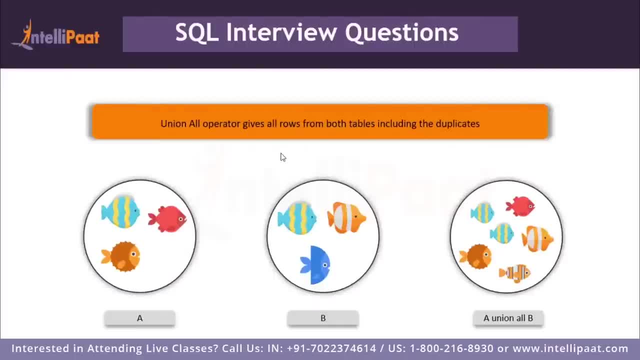 let's continue with the session. Right Now let's look at the union all operator. So the union all operator gives all the records from both the tables, including the duplicates as well. So here, since this blue fish is present in both the tables A and B, the final result: 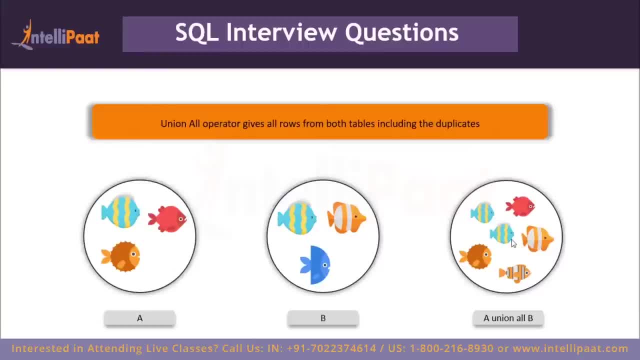 of A union, all B would also have the duplicate value. So here we see that we've got both of the blue fish from table A and table B. Now let's go ahead and implement this in SQL server as well. So here we have these two tables already ready, which are student details. 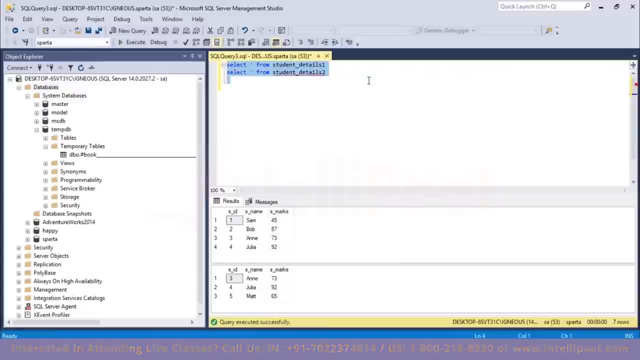 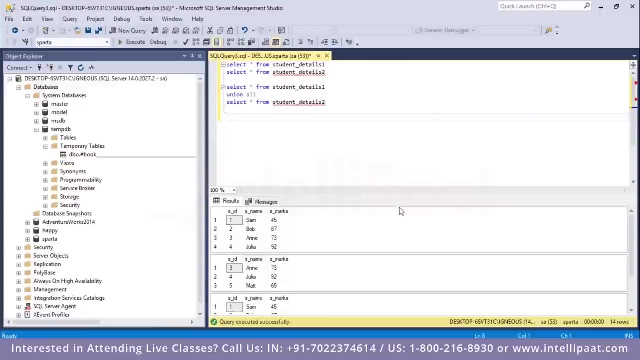 1 and student details 2.. Now what I'll do is I will copy this, I'll paste this over here and just type in: union, all So union, all. I'll click on execute. So student details 1, student details 2.. Let me just expand. 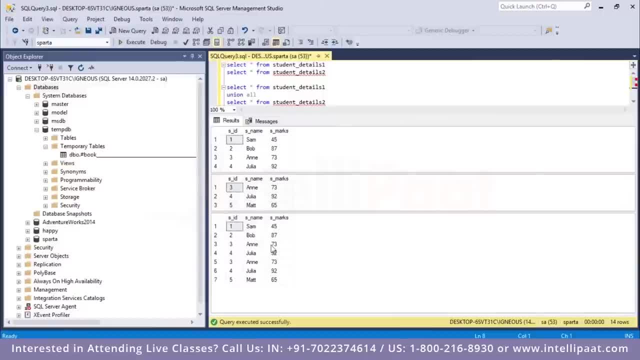 this over here, Right, And this is the result of union all operator, Right. If you have a glance at this, you'll see that these two are repeating, So we would have duplicate values. So we've got Anne twice over here and also Julia twice over here. So next question: 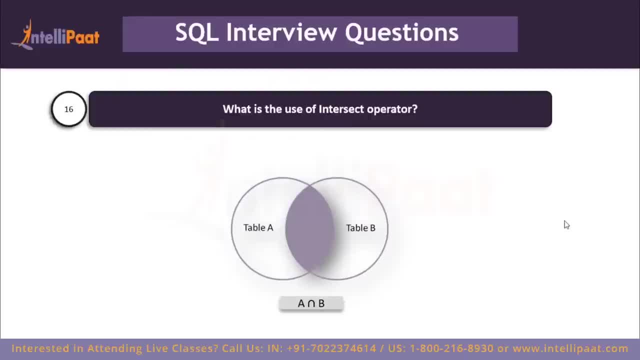 Well, what is the use of the intersect operator? So the intersect operator helps to combine two select statements and returns only those records which are common to both the select statements, Right? So if we've got table A and table B over here and if we apply the 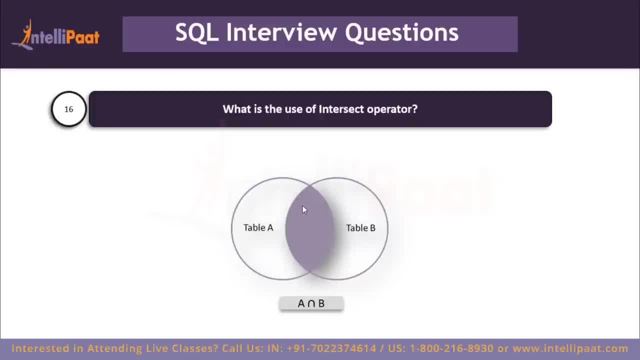 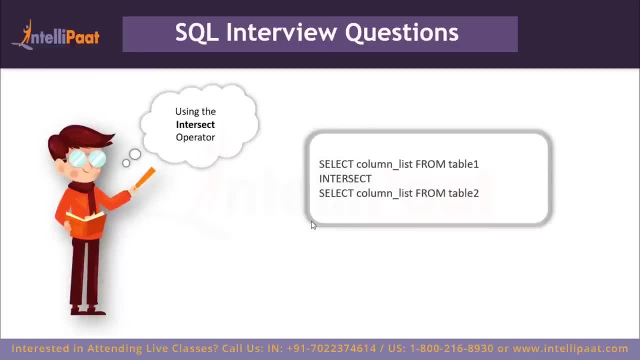 intersect operator on these two tables, then we'll get only those records which are common to the result of the select statements of these two. Now let's look at the syntax. So over here this is the syntax. So we'll start out by giving the first select statement and then we'll give the intersect. 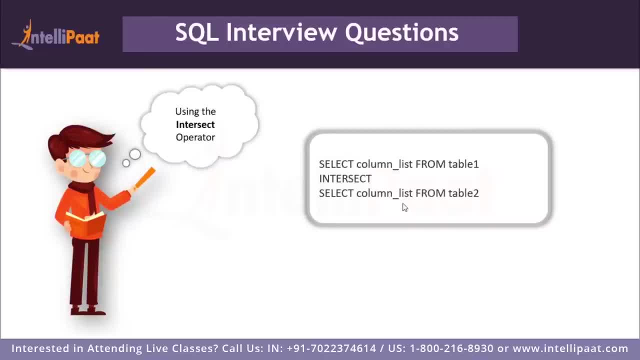 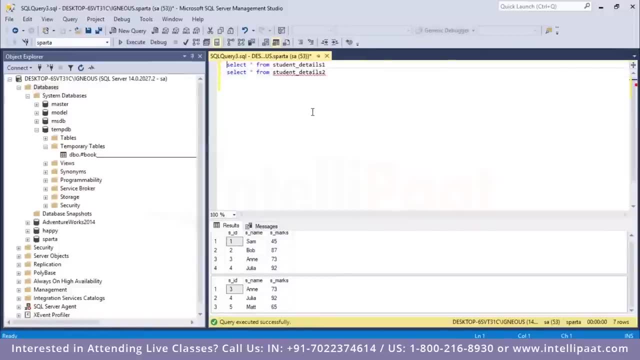 operator, following which we'll give the second select statement. Now let's see an example on this. So again, we have these two tables over here: student details one and student details two. Now let me apply the intersect operator on these two. So let me just type. 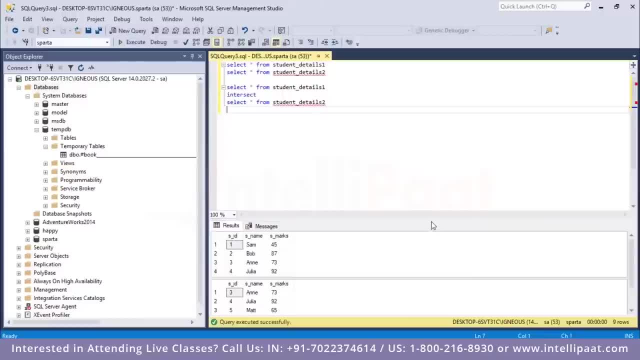 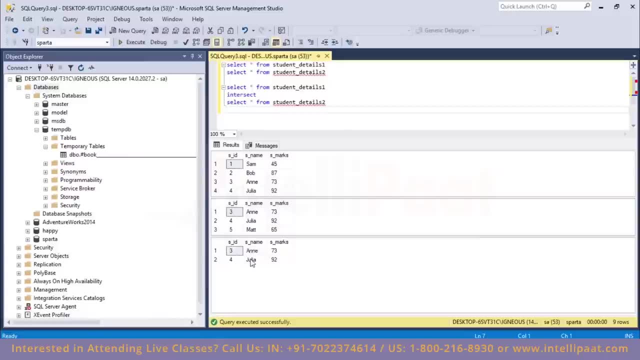 an intersect over here and I click on execute. Now let me maximize this over here. Right So, student details one. student details two. And this is the result of union. all Right So, student details one. student details two: result of the intersect operator. so we see that, since Ann and Julia are common, 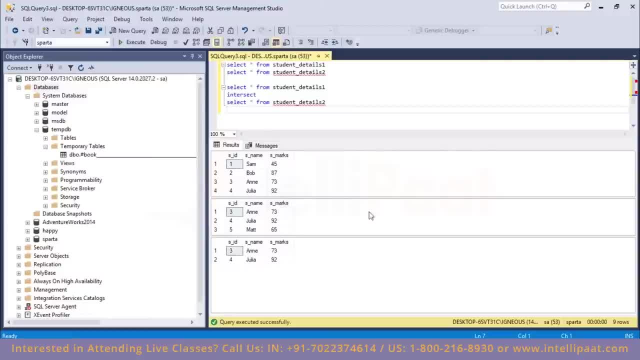 to both of these tables. this is the resultant of the select statement, right. so the select statement on the first table gives out Ann and Julia, and the select statement from the second table also gives out Ann and Julia, so the intersection of these two would be this. so we have our final question. now let's 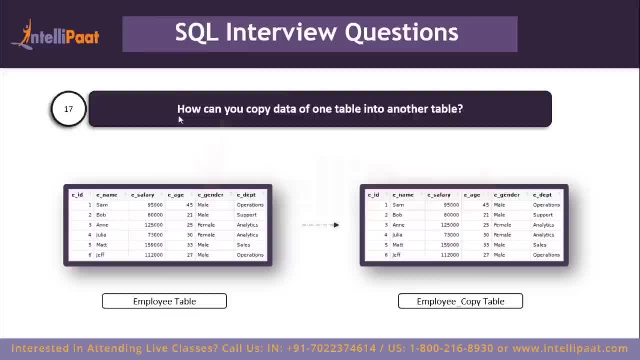 say, you are given a table. now you would have to copy the data of this table into another table. so you have this employee table. now you'd have to go ahead and copy the data which is present in all of this table into one of the table. so 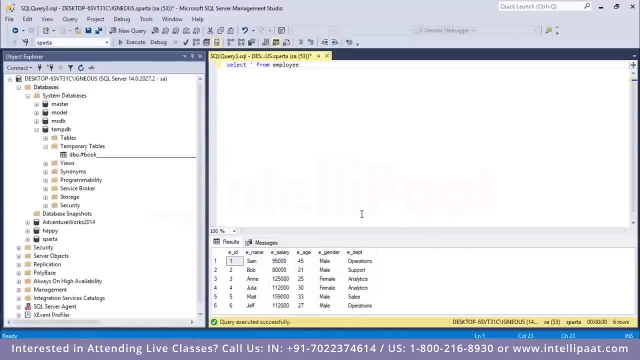 let's see how can we do this. so this is our employee table over here. now we would have two copy all of this into one other table. so for this purpose we can use the insert into select operative. now, before we go ahead and do that, we would also have to create another table which would have the same. 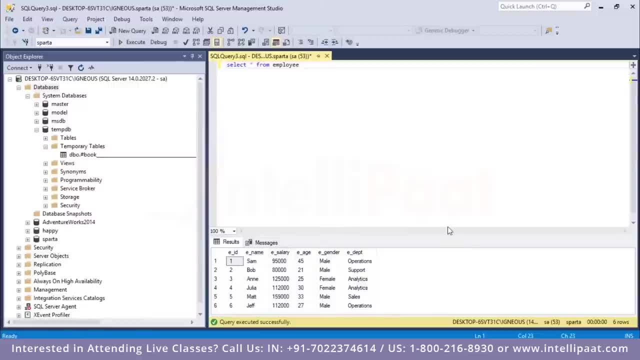 structure as this table, so the table doesn't have the same structure. then you wouldn't be able to copy the data. So let me go ahead and create the table first. So I'll type in create table and I'll name this as employee duplicate, And then I'll give in all of the values over. 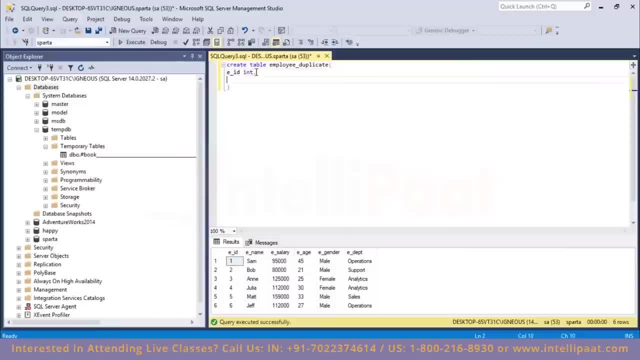 here. So my first column would be EID, and this would be of integer type. Second column would be E name and this would be of var char type And the length of the string would be 20.. And then I would have the E salary over here. This would be of integer again After. 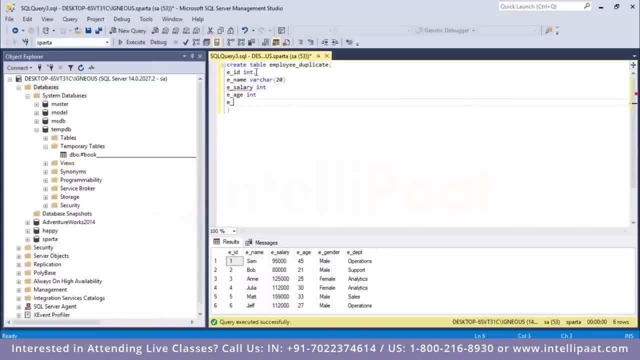 this. I would have the E age, which is of integer, Then I would have the gender of the employee. So the gender of the employee would again be of character type. Now I'd have to make sure that I give in commas after all of these, So let me just put in a comma after. 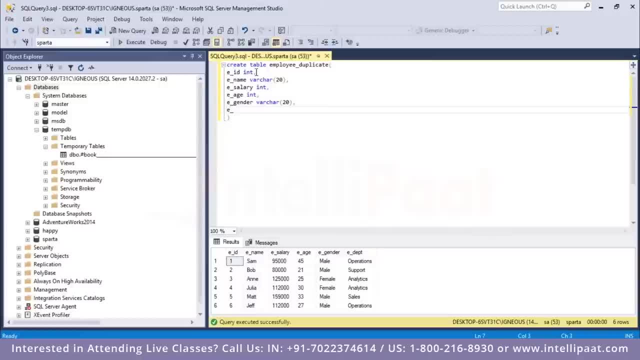 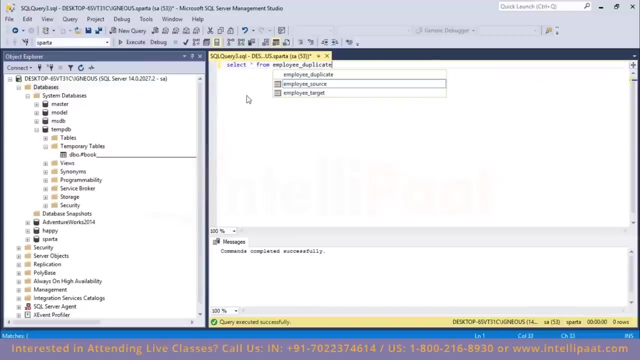 this as well, And then the final column would be E, D, E, P, D, And this again would be of variable character, of length 20.. Right, So I've successfully created this employee duplicate table. Select star from employee duplicate Right. So as 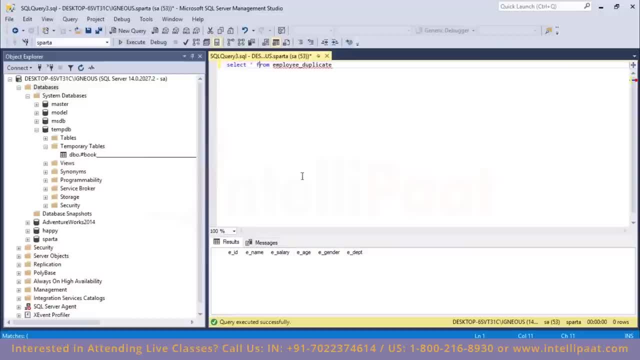 of now we see that this table is empty. Now I'd want to copy all of the table present in the employee table into this table. So let me write in the command for that. So I start off by giving the keywords: insert into Now. after that I'll give in the name of: 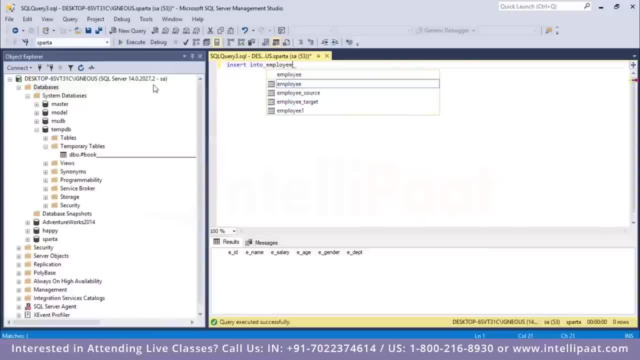 the table into which I want to insert. So the name of the table would be employee duplicate. Then I will type in select star from and then I would have to give in the name of the original table. So the name of the original table would be employee Right. So six rows.